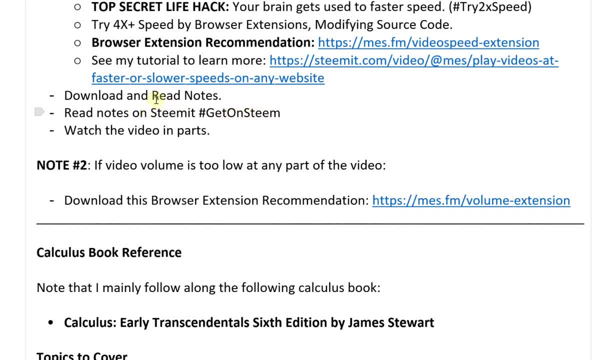 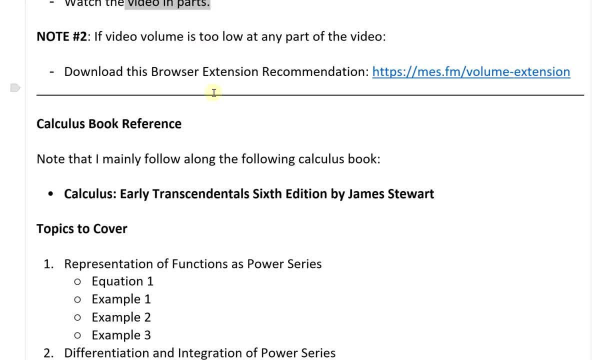 the notes. or you can read the notes on Steemit Hashtag: get on Steem. All the notes will be in the link in the description. Also, you can watch the video in parts. All right, so now let's go further. So calculus book. 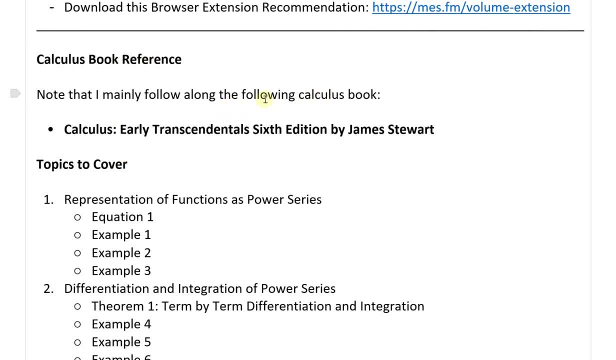 reference. Note that I mainly follow along the following calculus books, So calculus early transcendental, sixth edition by James Stewart, and this. this is from it mainly as well. So now let's look at the topics to cover. So we're gonna go over representation of functions as power series. 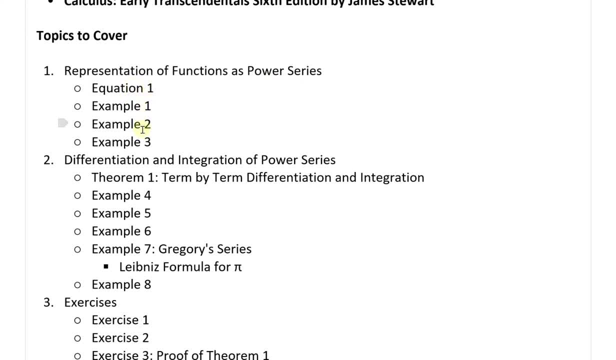 go to equation one and then go over example one, two, three, then differentiation and integration of functions as power series. So we're gonna go over representation of functions as power series. So we're gonna go over representation of functions as power series. So we'll go with theorem one term. 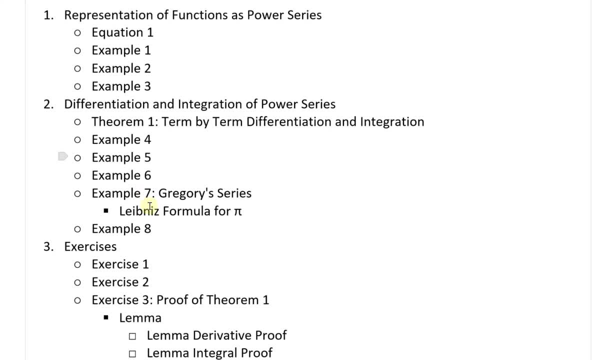 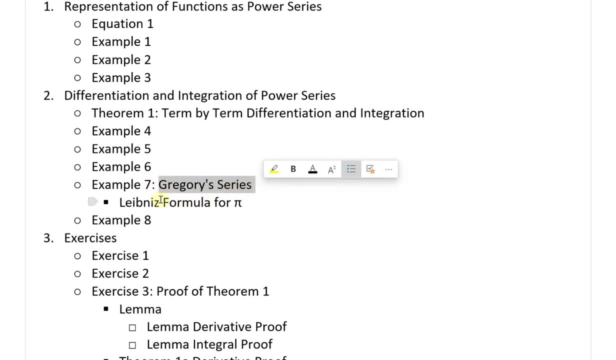 by term differentiation and integration, Then go over example four, example five, example six, then example seven, which involves Gregory's series, and then also look at Levin as formula for pi, which which derives itself from this example of this Gregory series, then go over 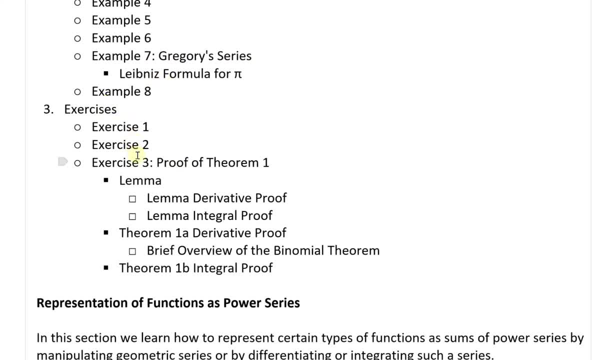 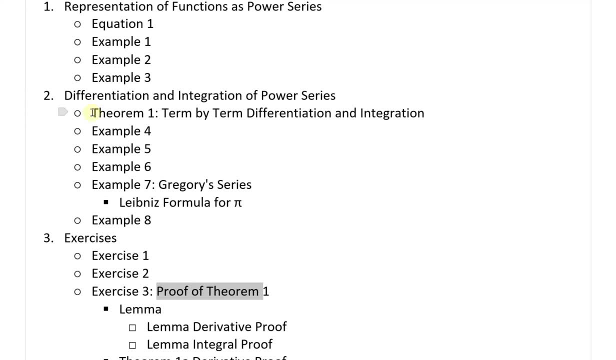 example eight. then go over some exercises: exercise one, exercise two, and then exercise three, which is proof of theorem one. So, and then go over some exercises: exercise one, exercise two, exercise three, exercise four, exercise five. So we're gonna go over some exercises, exercise six: 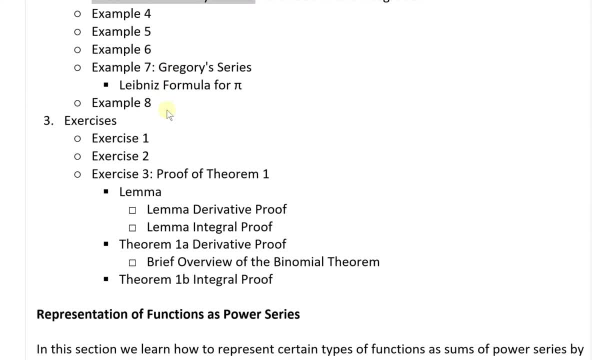 exercise seven. exercise eight: exercise nine: exercise twelve: exercise eleven: exercise ten: And this is where my calculus book doesn't prove it. Yeah, it doesn't prove, it just states the theorem. but then here at MES got a gotta find a, find a proof somehow. So go over the proof of 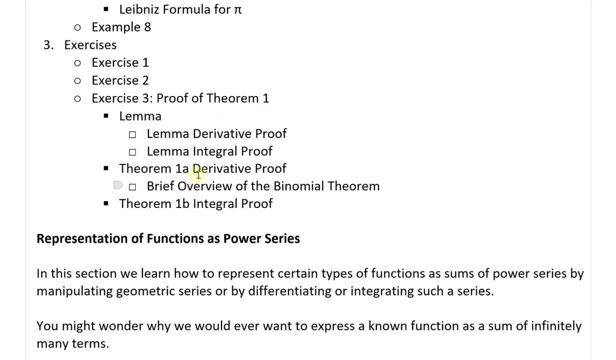 theorem one there's a lemma, and there I go over lemma derivative proof and lemma integral proof, and then go over theorem one a, which is a derivative proof, and then then, which involves a brief overview of the binomial theorem and also Pascal's triangle, and then theorem one b, integral. 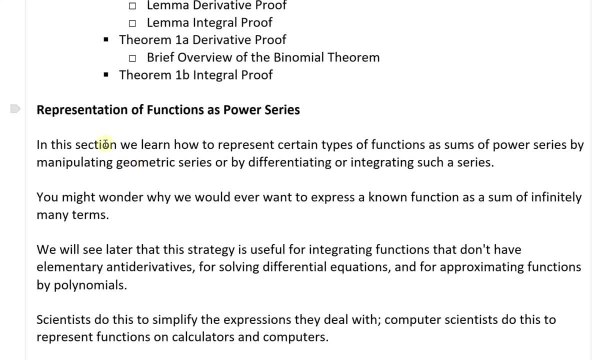 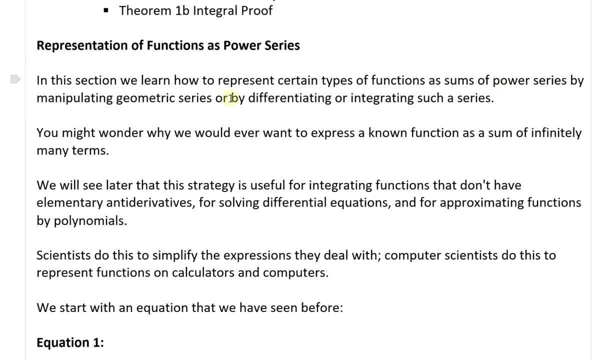 proof. All right, so now let's go for the theory of the drift. So let's get down to the common rule here for this. so representation of functions as power series. so in this section we learn how to represent certain types of functions as sums of power series, by manipulating geometric series or by 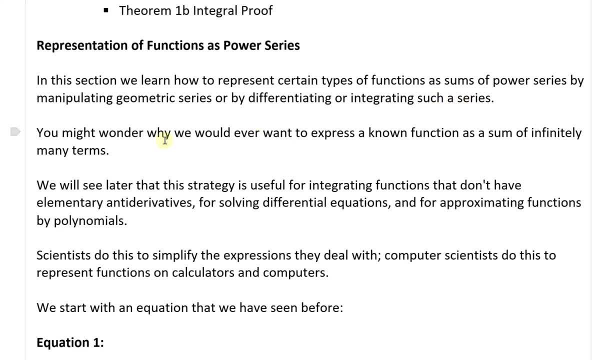 differentiating or integrating such a series. so you might wonder why we would ever want to express a known function as a sum of infinitely many terms, because, yes, when you're dealing with series goes infinity. uh, we will see later that this strategy is useful for integrating functions. functions. 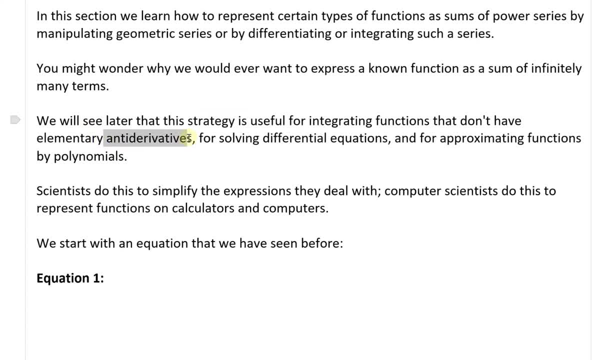 that don't have elementary anti-derivatives, or basically the basic ones that we're uh used to uh for. yeah, and also for solving differential equations. this is useful for that and for approximating functions by polynomials, yeah, so scientists do this to simplify the expressions. 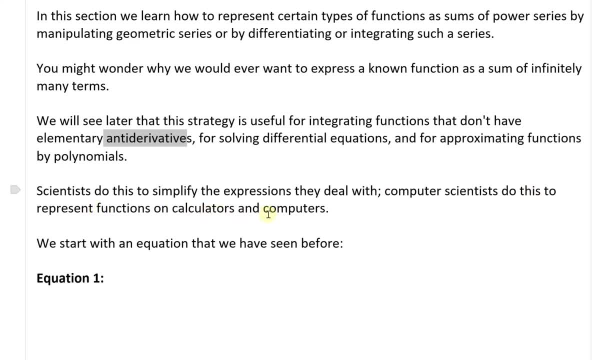 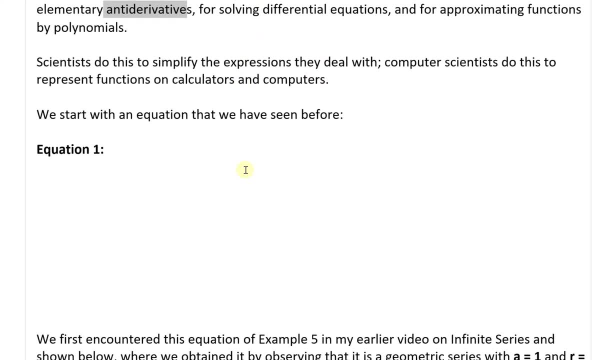 i deal with computer science, do this to represent functions on calculators and computers. so, yes, most of it is just pretty much using this. uh, we start with an equation that we have seen before and since i'll be referencing this equation uh, many times in this document. 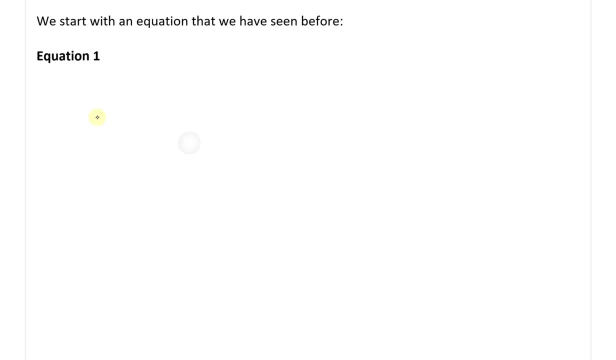 in this video. i'll just call it equation one and uh, here, uh. so the equation i'm gonna- it's actually working backwards, but we have one over uh. one minus x. yeah, this equals two. yeah, this equals to one plus uh x, plus x squared, plus x cubed, and then plus dot dot dot. this equals to: 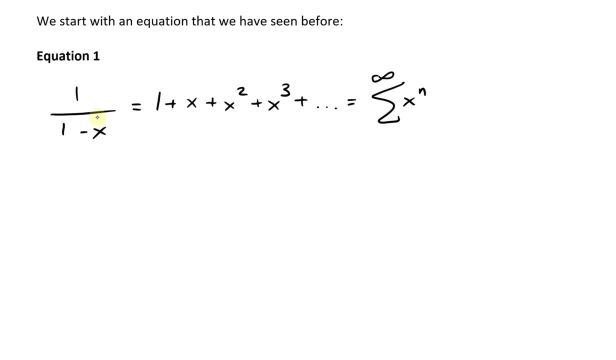 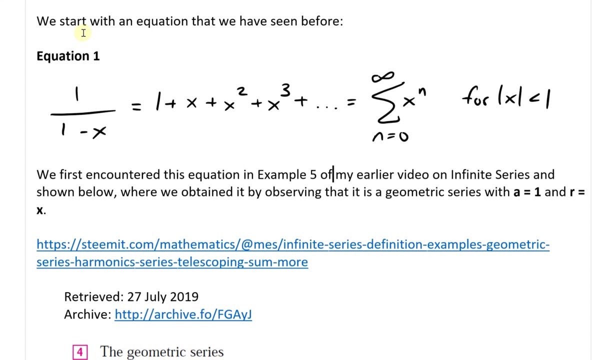 the summation of x to the n, this is up to infinity, starting from n equals to zero, and this is four. uh, when the absolute value of x is less than one. so, yeah, so for these values of x, when the absolute value is less than one, it's convergent and we get this. yeah, now recall that. 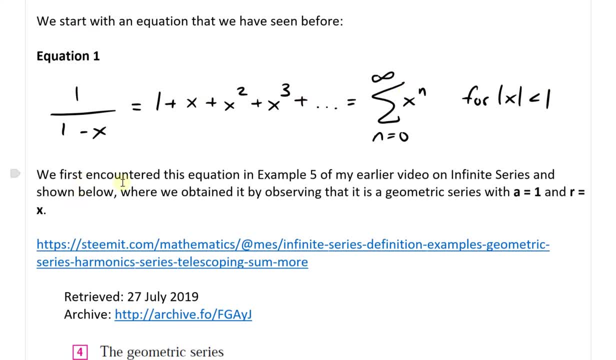 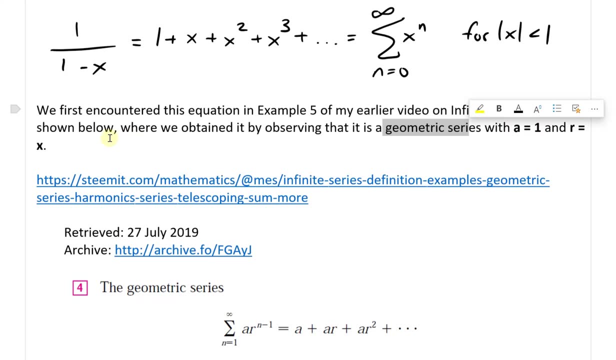 i went over this uh equation in my earlier video, so we first encountered this equation in example five of my earlier video on infinite series and and shown below where we obtained it by observing that it is a geometric series, also reference ball, with a equals one and r equals to x. yeah, so recall. 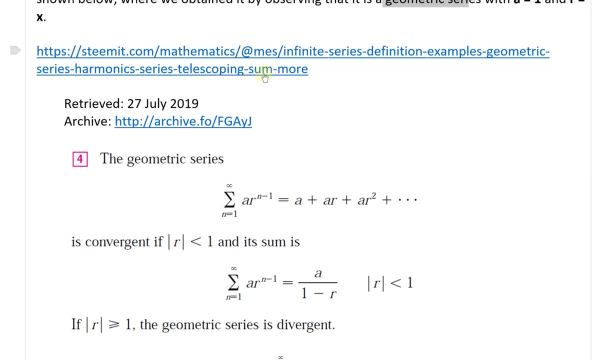 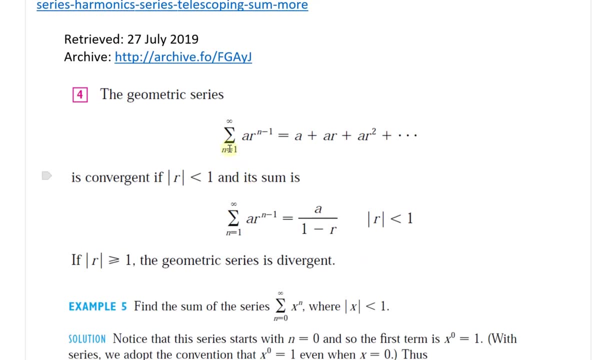 this, and then we can ramen it and then compute by. does it? uh, Carolina, yeah, et al, does that make sense, or or anything? yeah, let's just go ahead. let's just break this down. i think this is one. okay, one more time, and let's think about this. so how about what we might do, whether it's that, 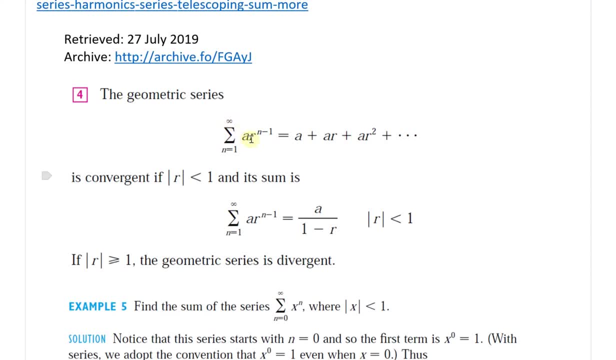 the r when r equals zero, and so on. and we want to make this one horizontal axis by starting from this function of the three ranked engine associated with the r她. so par수가, and where's the mesons and ubiquities? also, row, just box plays around with it delivering. 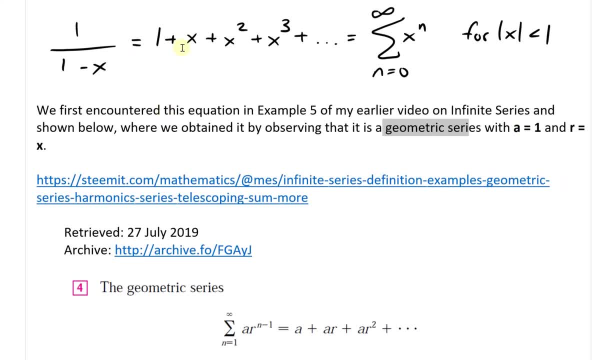 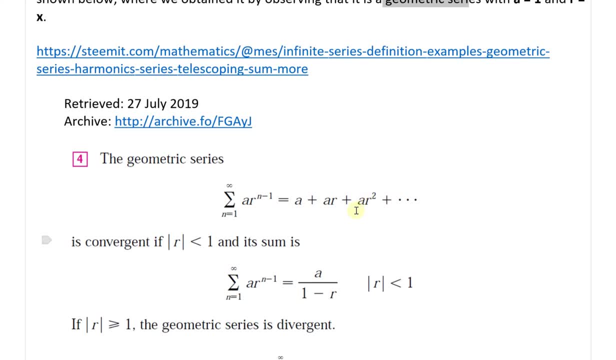 to the wonderfulness of the formula today. so we're going to go ahead and analyze the prognosis here and then we're going to look at thewhat charles v placebo's value is over here. when you do the x, uh, yeah, yeah. so a plus a x would be just one plus x, plus x squared and so on, and this is a. 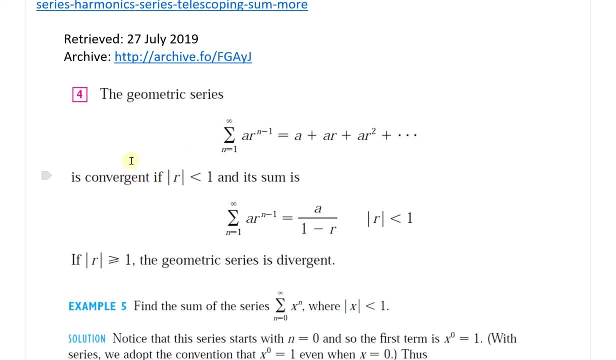 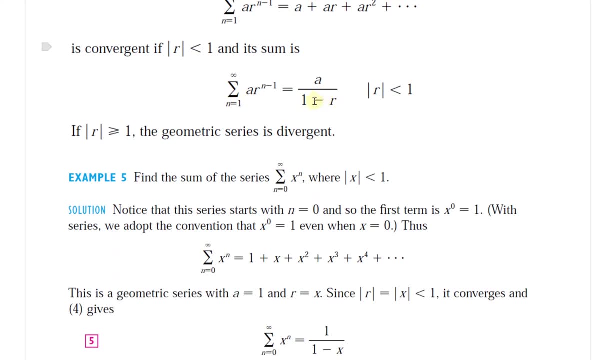 r squared, keeps going on and on and and recall that i proved that it was convergent if the absolute value of r is less than one and its sum is. when it's convergent, uh, equals to this a over one minus r, and this is for uh, uh, absolute value of r is less than one. so when a is equal to one, 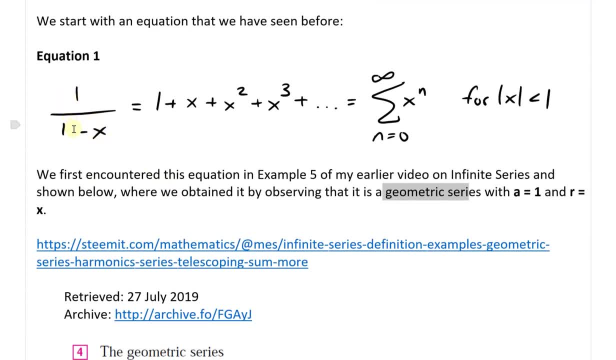 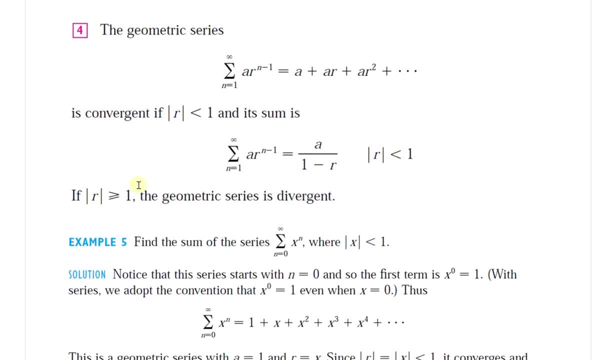 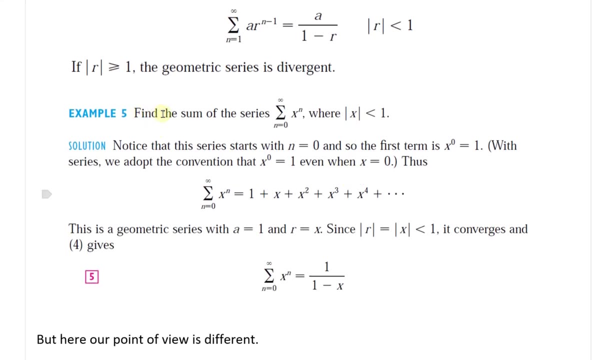 we just get our one minus one over one minus uh one, i mean one over one minus uh x or r. so this case, x equals r. if r, if the absolute value of r is greater than or equal to one, the geometric series is divergent and in example five i showed that uh. well, yeah, i showed that. uh, this one right. 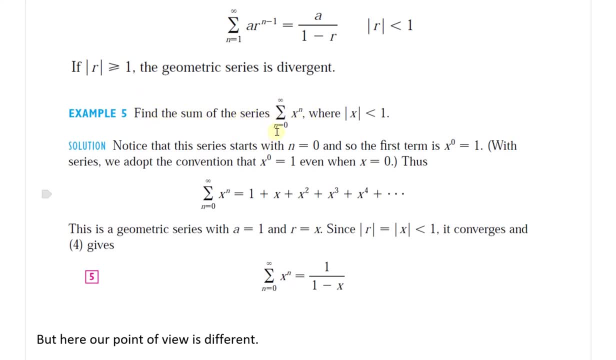 here, where we were asked: find the sum of the series. uh, the summation from n equals zero to infinity of x, and where absolute value of x is less than one, and then again notice that this series starts with x. and then again notice that this series starts with x, and then again notice. 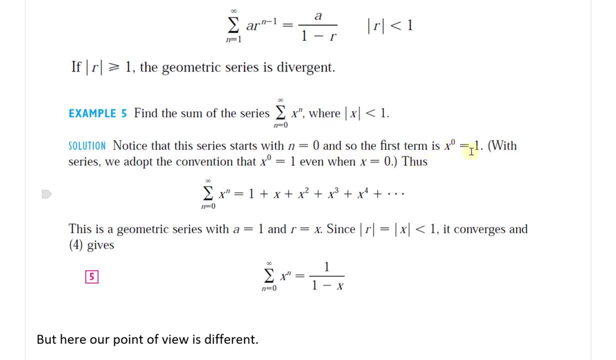 with n equals zero. so the first term is: x to the power of zero equals one. so yeah, put x equals the power of zero is equal to one. so with series we adopt the convention that uh, x to power of zero equals one, even when x is equal to zero, and also in this i referenced uh. this is the convention. 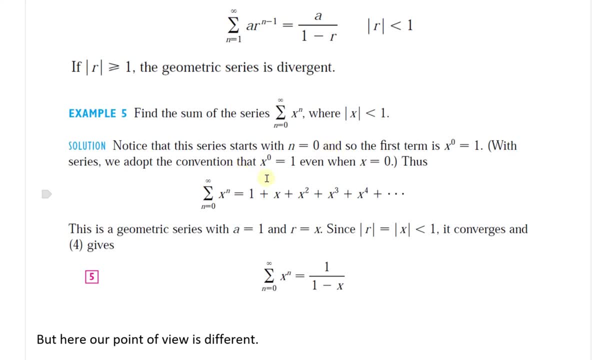 that's usually used for uh, powers of zero, and zero to power of zero, and so on. so yeah, thus what we have is the summation from n equals zero to infinity, of xn equals to uh one, x to the zero, then x to the one, x to the. 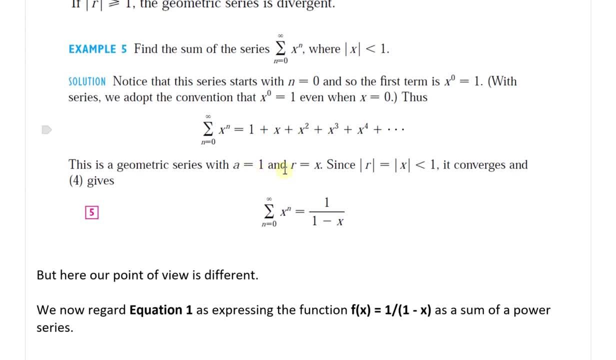 two extra three and so on. this is just a geometric series of a equals one and r equals x. since all absolute value of r is uh equals to absolute value of x and is less than one uh, it converges and gives this right here. so then we have just replace that by one, so we have the sum of this uh, of this series. 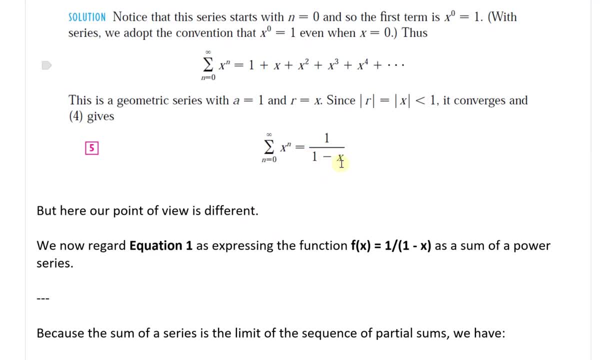 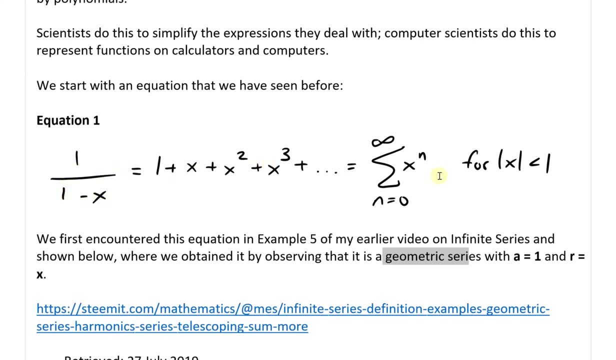 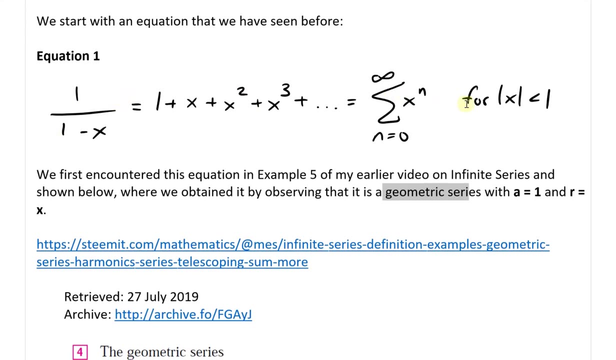 equals to one, one divided by one minus x. so here i just wrote this on the other way. so i wrote this: this one minus one divided by one minus x equals to the series. and this is get the idea that this is a function being written as a series. so here's a function being written as a series, an infinite. 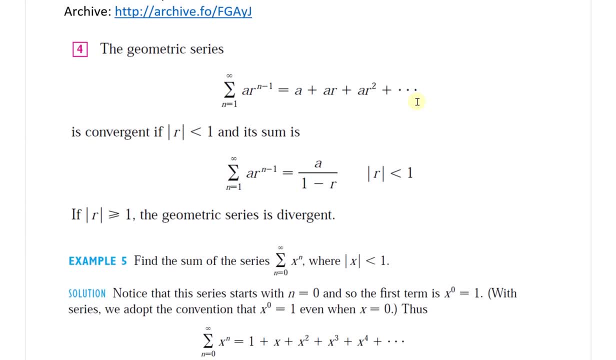 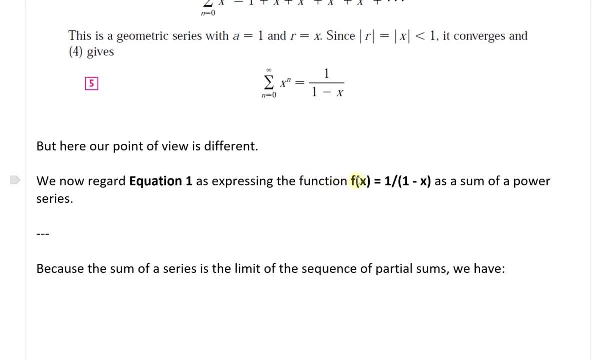 series or infinite, in this case power series, because x to the n. yeah, so here so, but here our point of view is different. we now regard equation one as expressing the function- f of x equals to one divided by one minus x- as a sum of a power series. so yes, it's a function. 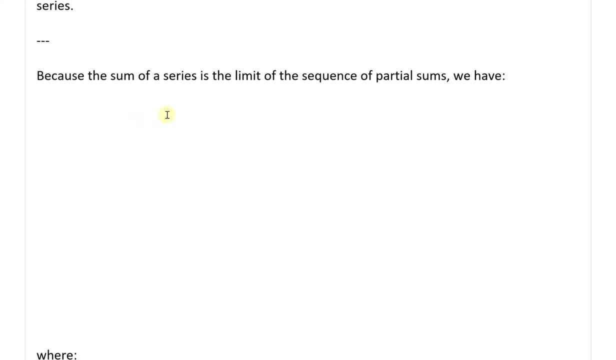 representing the function f of x equals to one divided by one minus x as a sum of a power series represented by power series. so, because of the sum of a power series, the limit of the sequence of partial sums, yeah, we have that f of x, so we're writing this- a function equals to one over. 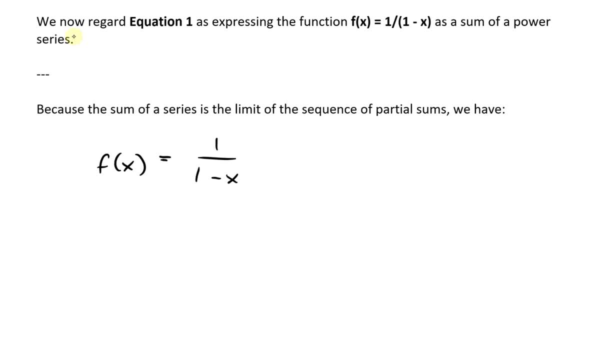 so one over one minus x, and now this equals to the limit of the partial sums and approaches infinity, as approaches infinity of s n of x, and where this uh s n is partial sum is equal to s n x, and this equals two, one plus x. this is, this is just a power series, plus x, squared, plus dot dot. 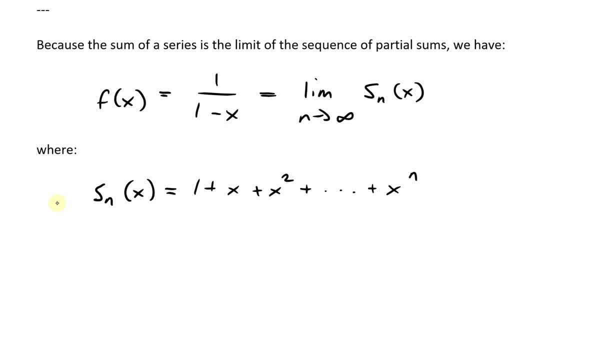 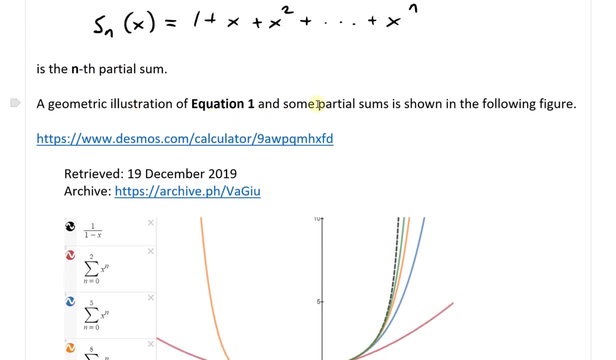 dot plus x to the n. so as this goes to infinity, we have our power series goes to infinity, then we can. then then it's going to equal to this one one divided by one minus x. so yes, and this s? n of x is the nth partial sum. so a geometric illustration of equation one and some partial 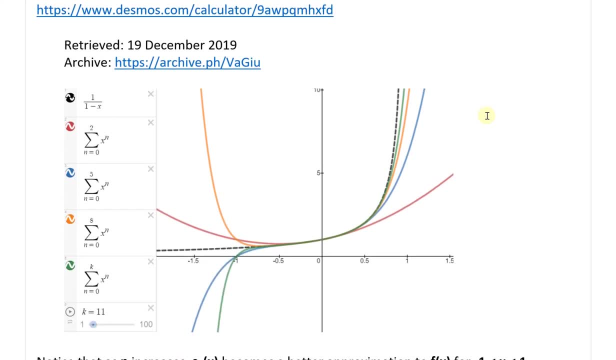 sums is shown in the following figure. so if we have, yeah here, if i just use the uh decimals calculator, it's pretty amazing. yeah, so in the dashed line right here, this is the exact uh function. so we'll call this one right here f of x and yeah, so let's put it on this side actually. so. 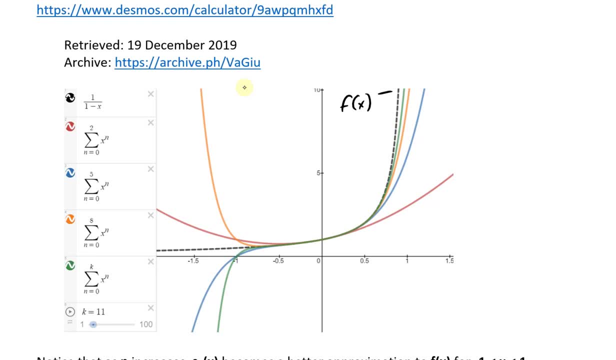 this is our f of x, and the dashed uh line right here, and then the, the first though, or the partial sum s two. so this is: from n equals zero to to uh two of x. n, that's the one arranged in red. so this one right here is s uh two, so it goes like this. so it's uh pretty far away from. 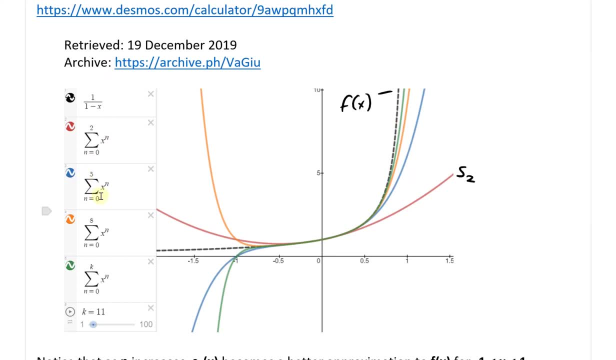 this f of x. then if you go to s five in blue and uh notice how it gets closer and closer, this one becomes negative and goes positive up there. this is going to be s five, and then the, then this uh orange one, s a, is getting closer and closer and this is uh eight. so it's positive, so it looks. 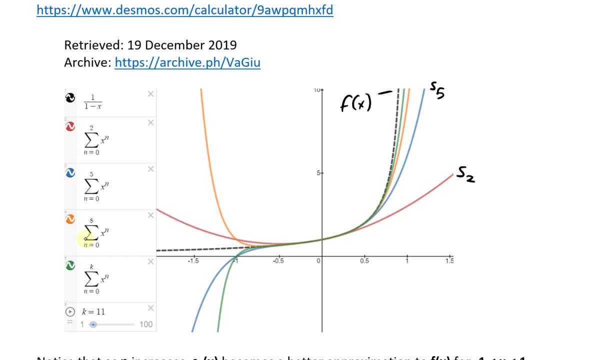 like it's going to scroll or fly up there. this is going to be our s eight. then i have uh. right here this: you could also write this in decimals calculator like this: you go n equals zero to k and where k equals to 11.. so right here is s 11. notice how it's getting. 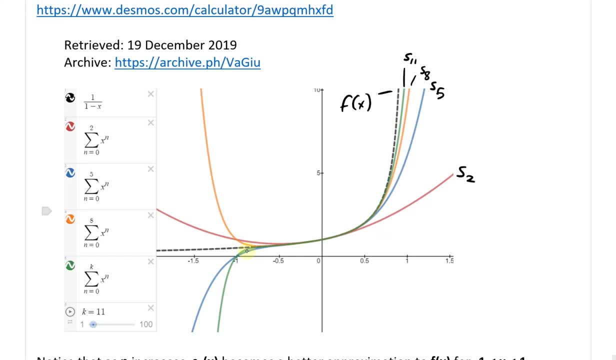 closer and closer to it. and then, uh, yeah, so obviously yeah, so it's getting closer and closer to this uh dotted line, which is our f of x function. and then, yeah, so, if you're summing up this, up to infinity, it's going to get closer and closer and closer, and and uh approach f of x and uh also note: 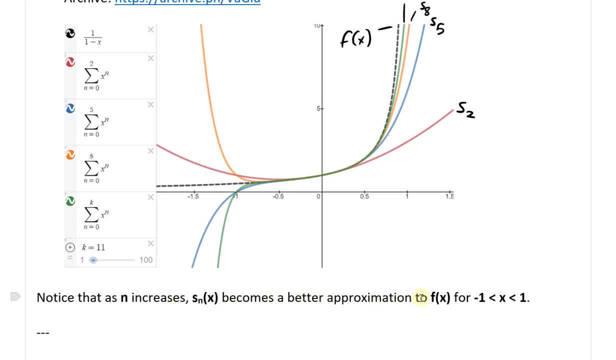 notice that as n increases, s, s n of x becomes a better approximation of x for uh, the uh interval of convergence. so where uh, x is between negative one and one and uh and one, or in other words, absolute value of x is less than one. so in other words, uh between this, this and this. so, as you can, 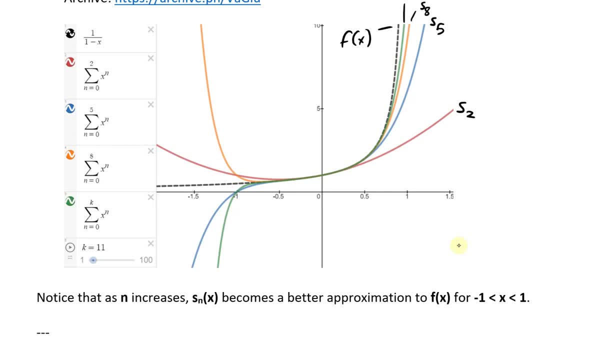 see here it diverges away from once you get past this one, but right right next to this, this line, right here and here. so between this and this, you can see it's getting decent approximation to this dashed line, right here and here. so that's our absolute. x is less than one and you can see here at x equals. 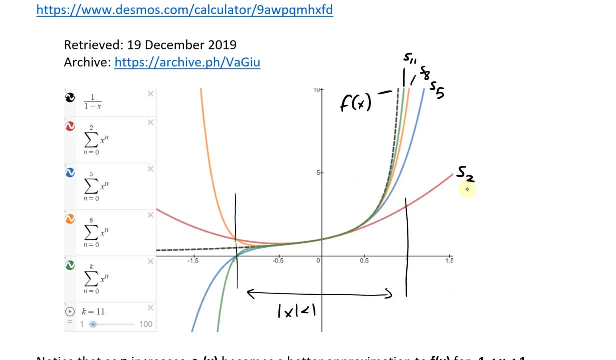 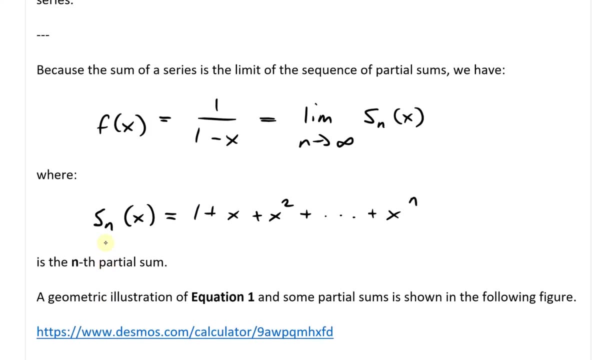 one here. it diverges up uh a positive there and here at uh negative one. yeah, the approximations are diverging, uh, the function isn't there. as you can see here, f of x equals like here, if you plug in one here, so you'll have a one divided by one minus zero. so the function is going to go to: 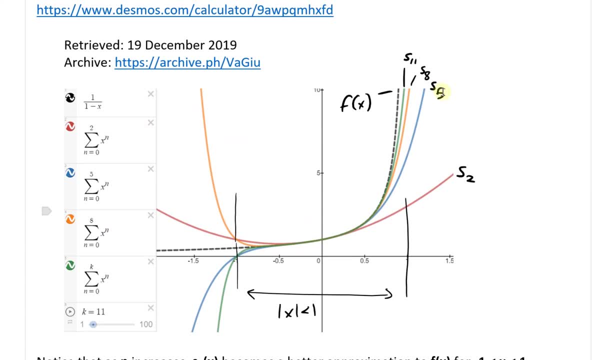 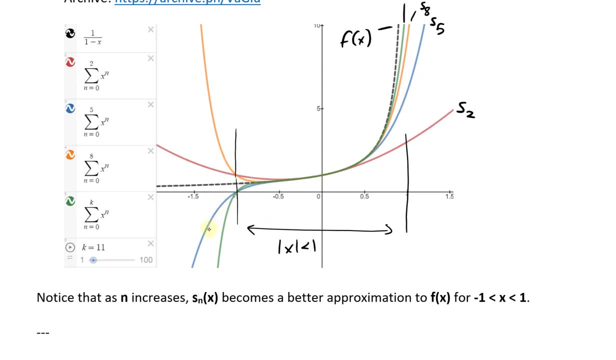 infinity there and then, interestingly, here, whenever you have the odd power s5. so when you plug in one, it's going to go into negative infinity there. so it's just getting smaller and smaller, though yeah, i mean yeah, as you get past this, uh pointer, as you get larger and larger negative value it's. 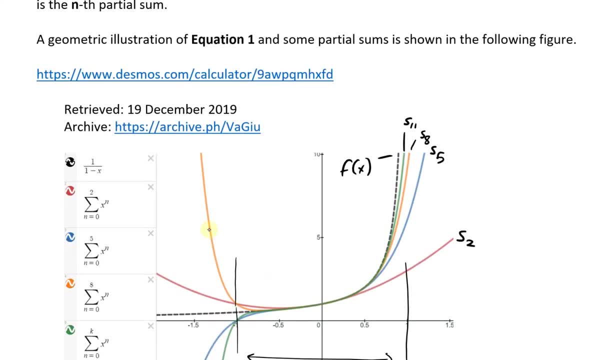 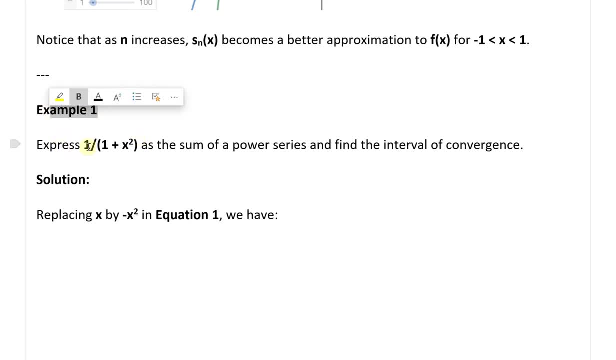 going to go more and more negative as opposed to, yeah, more and more positive there. so anyways, i digress. let's just uh skip over to now example one. so example one is: say it's express 1 divided by 1 plus x squared as the sum of a power series, and find the interval of convergence all right. so this: 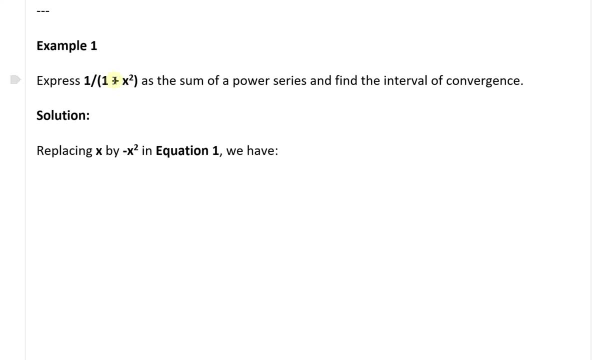 thing, what we have- uh as equation one. so what we could do is: yeah, but but instead of negative x, we have x squared. so or plus x squared, so what we'll have is replacing x- uh by negative uh, x squared in equation one we have. so what we could do is, if this is this function as equation one, we could. 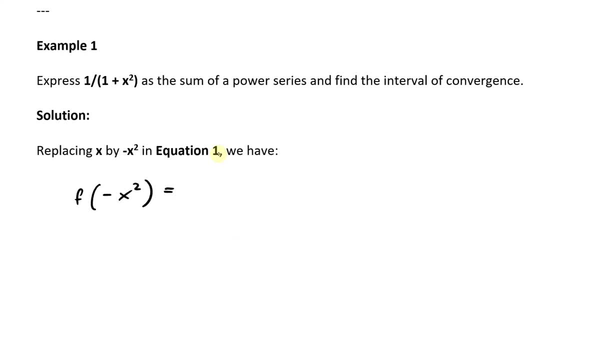 we could do f of negative x squared, so then we could plug this inside. this becomes one minus negative x squared. so now that this is in the form of equation one, we could write this as power series. so this equals to summation of: from n equals 0 to infinity of negative x squared n to. 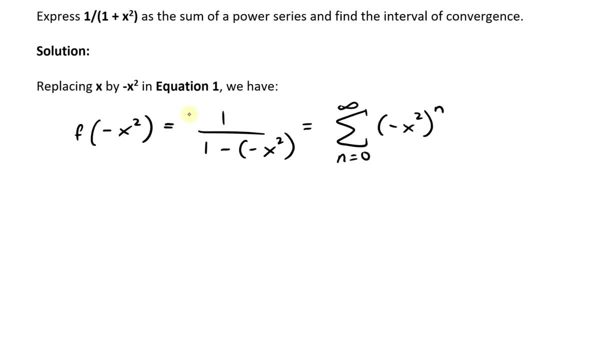 power of n like that. so what we have here- so this part right here- is just our equation: 1 divided by 1 plus x. so this is what we end up having is just this: uh, let's write this equal sign. so equals to 1 over 1 plus x squared. what we were starting off with, this equals. to now simplify this: 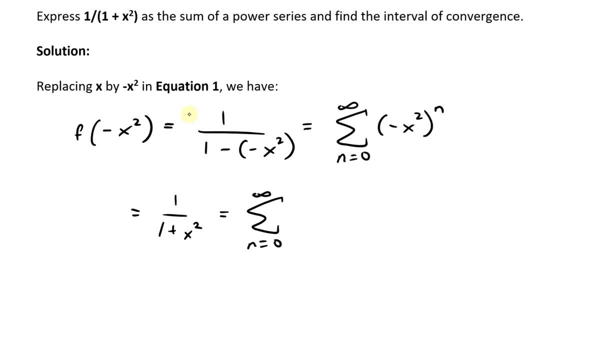 summation infinity and equals to 0. so now what we can do is this negative right here, though that's just negative 1 times x squared. so, uh, expand this power there, so it's going to be negative 1- n, and then times it by x to the 2n. 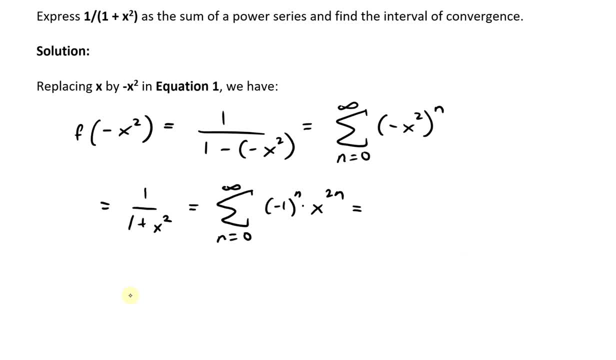 and uh, yeah, what this equals to if we expand this series. so negative 1 to power of n. when n is 0, this becomes 1, and then this one here: x to the 0 is going to be 1, so we'll have 1. 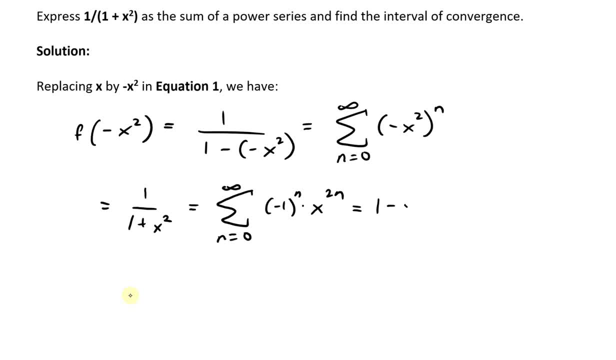 then. then we have n equals 1. this can be negative x squared. and then we have n equals to 2. this becomes positive, positive 1. this one, because 2 times 2 times 2 is 4, so we'll have plus x to the 4.. then, when this is 3, what we end up having is: is: this becomes negative. 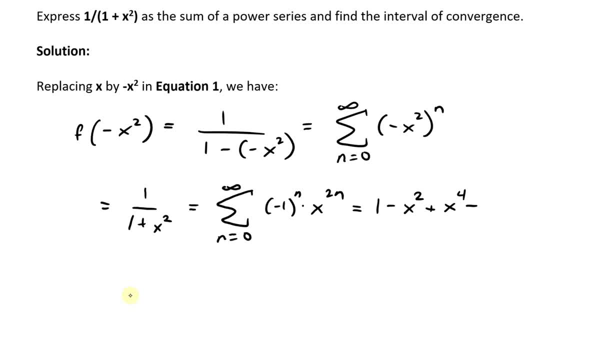 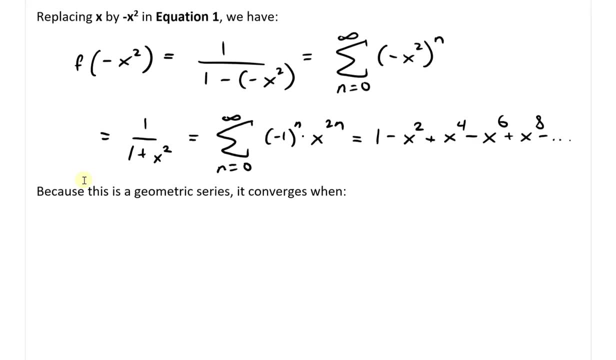 1, and then x to the 2 times 3 is 6.. so you can see the pattern. next one's going to be a plus x, 8, and then minus dot dot, dot. all right, so now, because this is a geometric series, it for it. 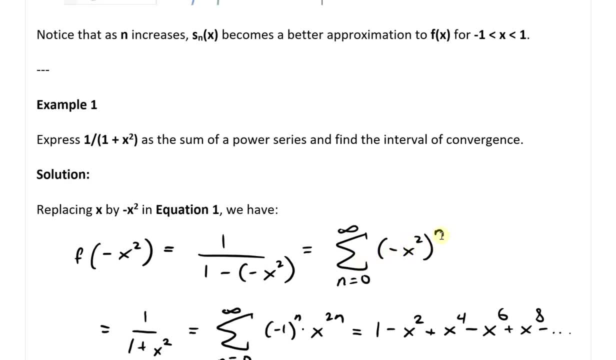 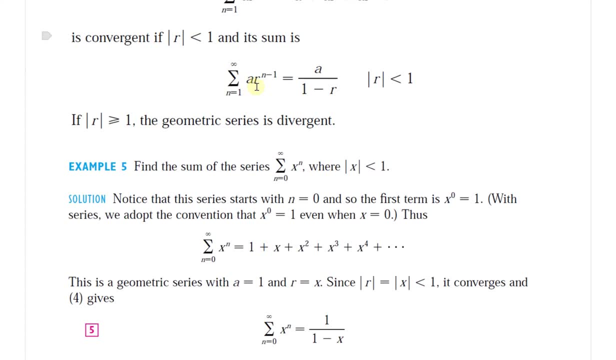 when. so that this is? yeah, this is just a geometric series. now we have negative x squared power of n, so scroll up to what we have our reference right here. so this is just a geometric series where a equals to one and our r is our negative x squared. so, in other words, instead of the absolute value of 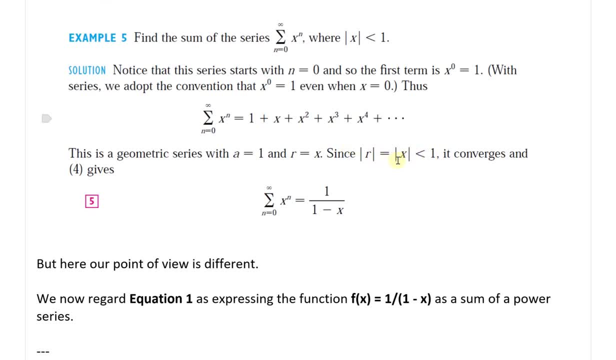 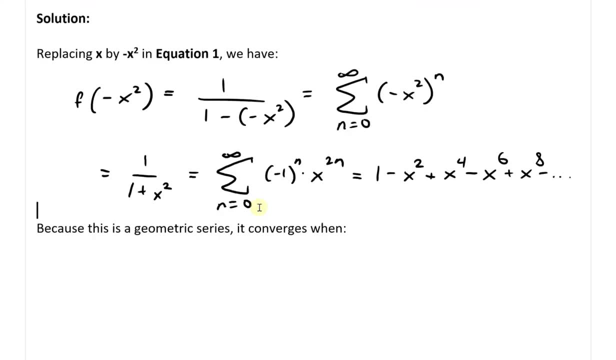 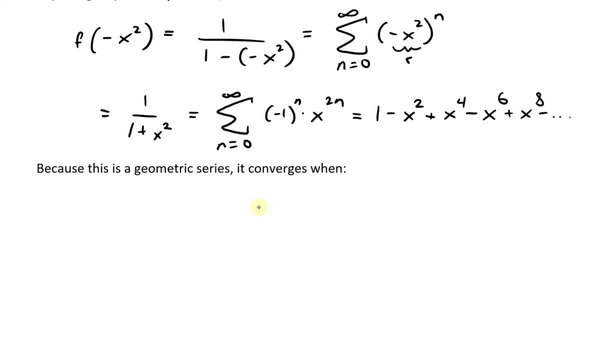 x is less than less than one, we have negative x squared. so score here. so absolute value of r is: is the one inside this power there, so this. so what we have is: so it converges when the absolute value, absolute value of this, this is our new r. so absolute value of- uh, i'll just 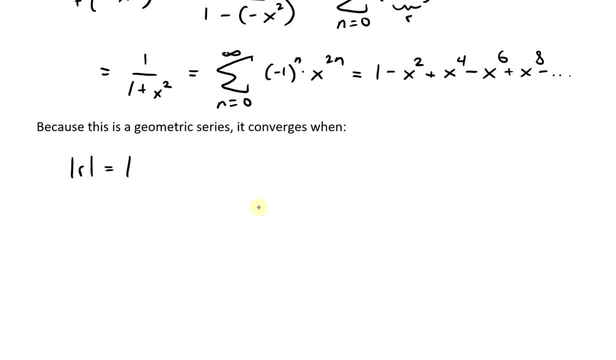 write: absolute value of r equals to absolute value of negative x squared, and this is less than one, and the absolute value of negative x squared that's just going to be. well, uh, just remove this negative, so this just becomes x squared. and x squared is always positive, so it's when x squared 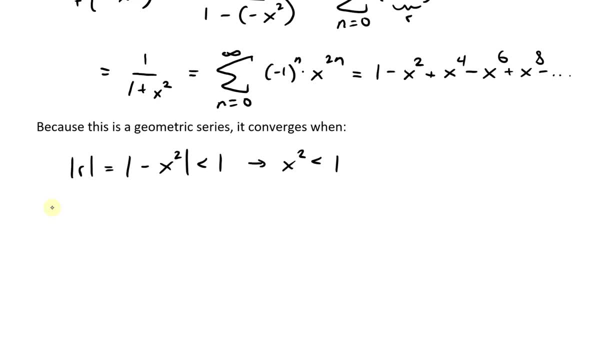 is always uh, less than one. and now this right here is our negative x squared. and this is our negative x squared. and this is our right here, x squared. the only time it's less than one is when the x inside of it is, when the absolute value of x is less than one. if x is two, x two squared is four, etc. if x is uh, 0.5, uh, yeah, for. 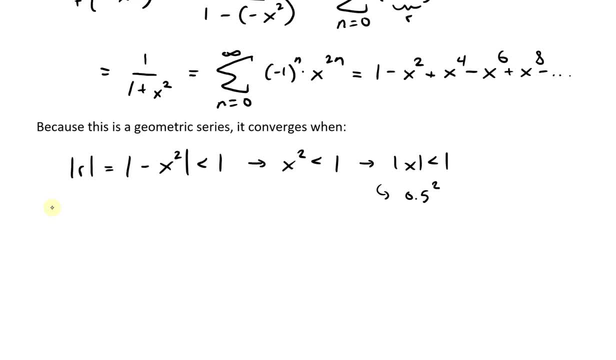 example right here: 0.5 uh squared equals to one over two squared, which equals to one over four. let's put uh i e. or, for example: yeah, we have that. or we could even put this: uh, plus or minus, it doesn't matter, it's always going to be. 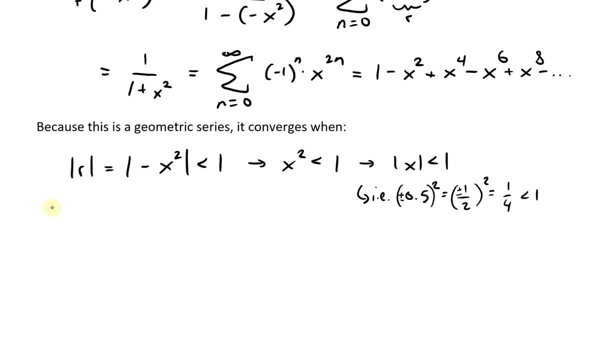 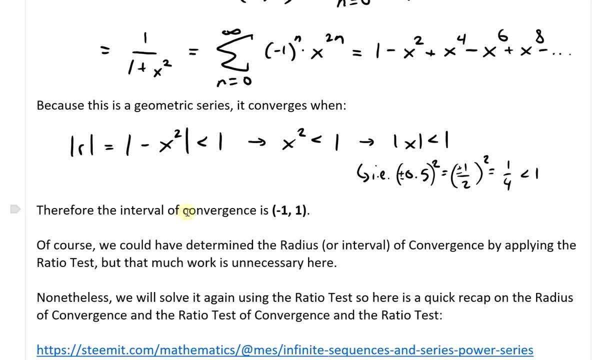 uh positive there. yeah, when you square it's always positive, so you can do plus or minus, doesn't matter. and then it's going to end up becoming uh positive, uh, one over four, and that's less than one. yeah. so therefore, the uh interval of convergence right here, because this absolute value of x less. 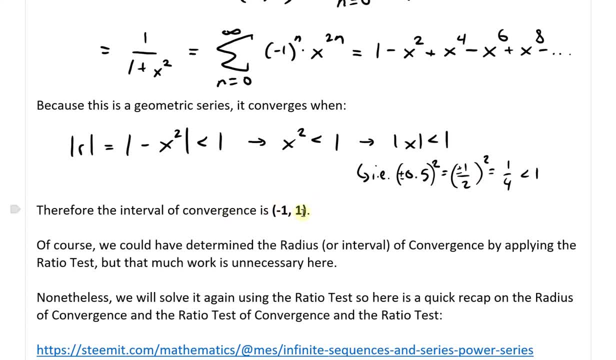 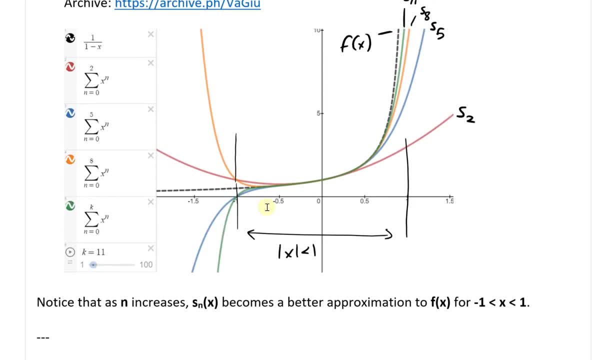 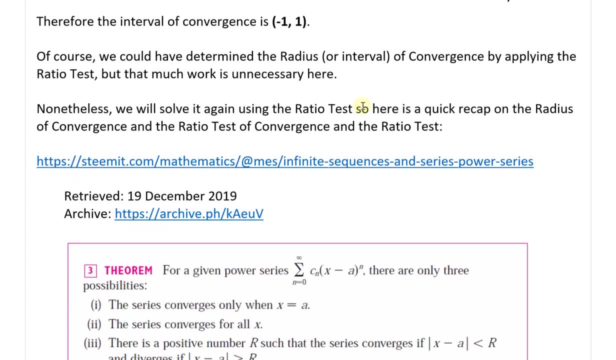 than one. uh, that means that it's, uh, it's going to be between negative one and one. this is open bracket. um, yeah, so not at these points. as per the geometric series, uh, theorem above for my research for my earlier video, it's right there. so when this is less than one, so going further, uh, of course, uh. 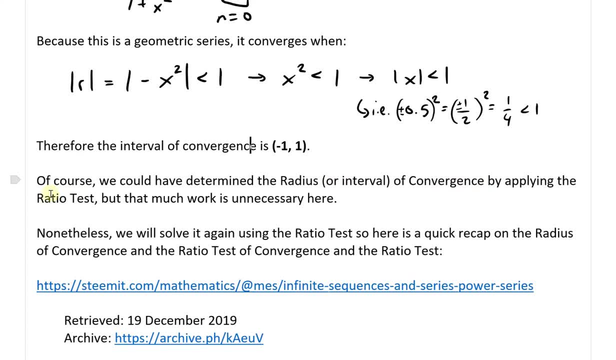 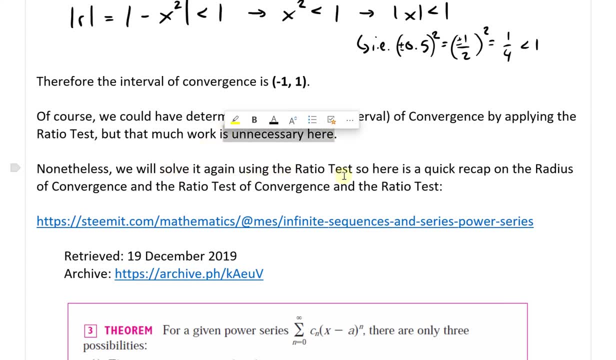 we could have determined the radius or interval of convergence by applying the ratio test, but that much work is unnecessary here, uh, nonetheless, this is what calculus book says. nonetheless, we will solve it again using the ratio test. so here's a quick recap on the radius of convergence and the 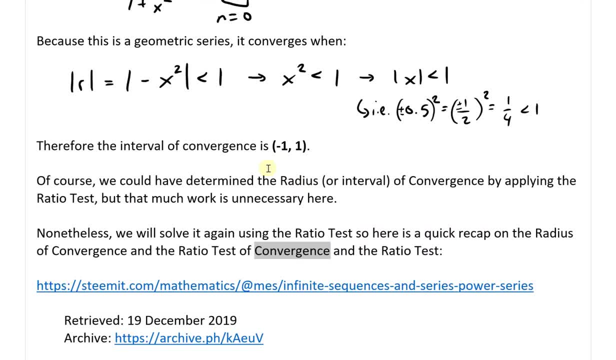 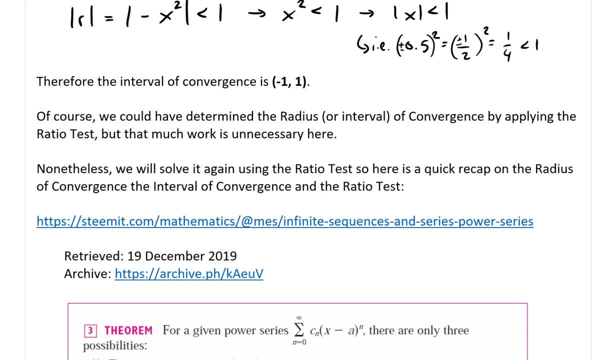 ratio test of convergence- actually ratio test too, too many times so- and the interval of convergence on the difference is uh. so the uh recap on the radius of convergence and the interval of the convergence and the ratio test is probably better to put this bracket. yeah, so recall from our other. 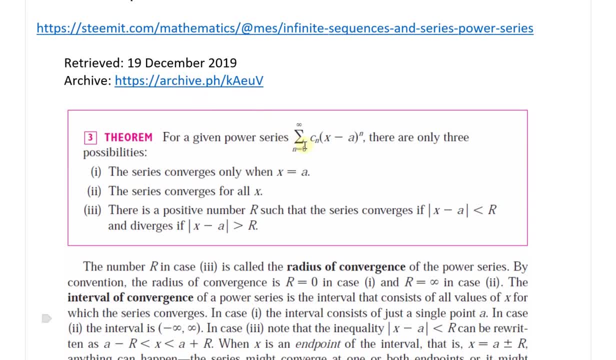 earlier video. so a theorem for a given power series. we have power series like this: uh, from n equals zero to infinity of s of c and the constant x minus a to power n. there are only three possibilities. the series converges only when x equals to a. that is, uh, everything goes to zero. 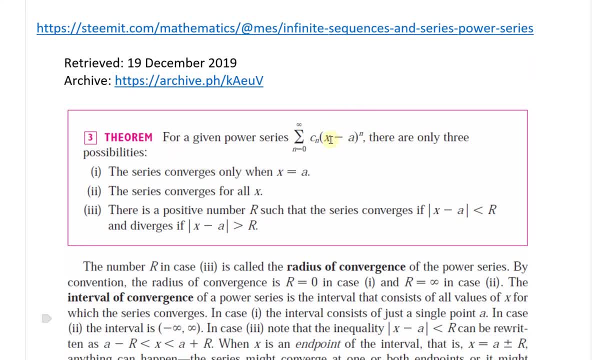 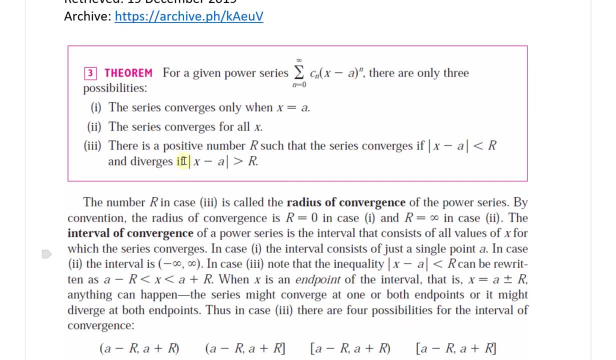 there, except i would assume then, uh, except here, x minus a zero, but zero to power of n when zero, so it depends on the convention- it could equal one. so, uh, then here the series converges for all x, or there is a positive number, r, such that the series converges of x. absolute value of x minus a is: 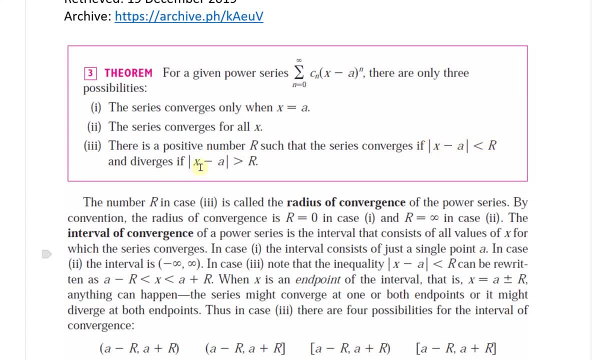 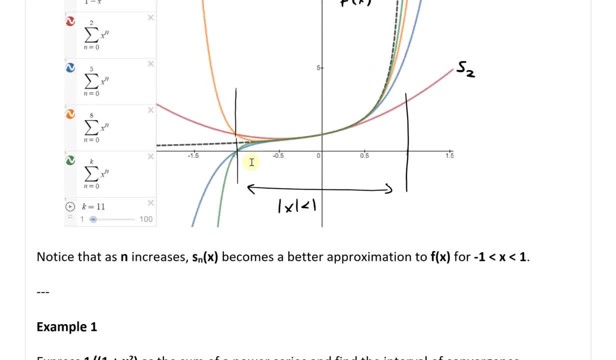 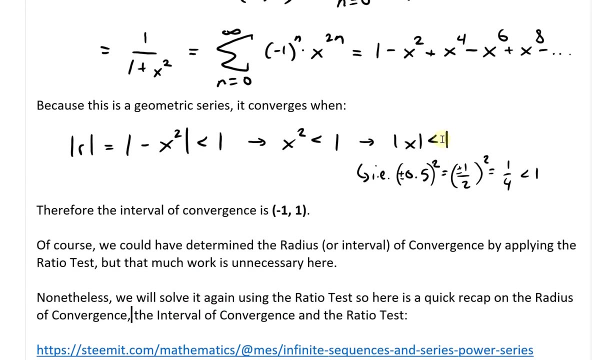 less than capital r there and diverges if absolute value of x minus a is greater than r. in other words, this is the radius of convergence and this value would be the one in the geometric series. so in this case this is less than r. so in this case here, the radius of convergence is one. so this uh, this one, here, where uh a is zero. 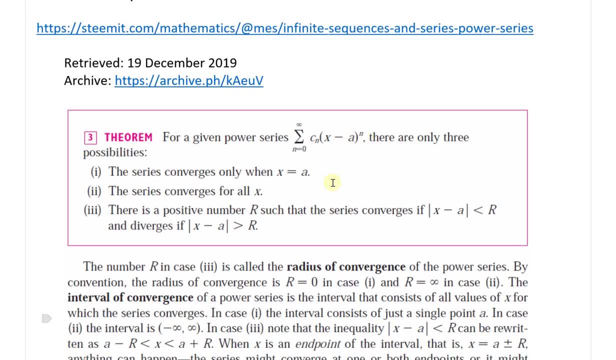 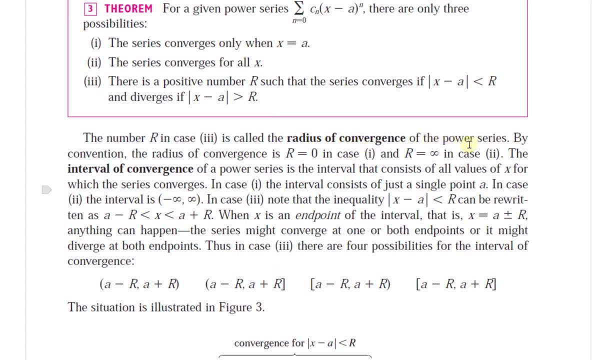 so in this case we'll have this part- is zero. x minus zero is absolute value is less than one. so one is the radius of convergence. yeah, so the number r in case three is called the radius of convergence of the power series. by convention, the radius of convergence is r equals zero. in case. 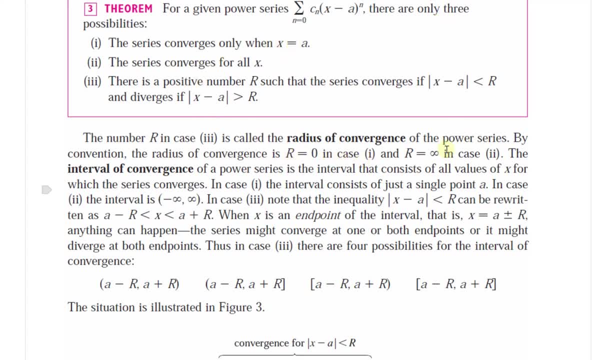 i. so here, when x equals to a and then here r equals to infinity, one in case two, of the convergence for all x, just by convention, and uh, the interval of convergence of a power series is the interval that consists of uh, consists of all values of x for which a series converges. in case i, the interval. 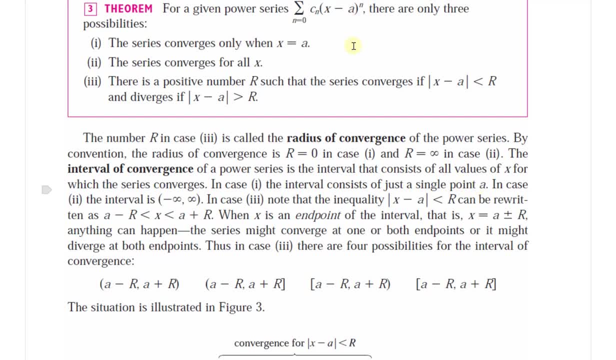 uh consists of just a single point, a, so that's just when a equals to when x equals a and in this, in the, in the, in case two the interval is from negative infinity to infinity. and in case three, note that the inequality x minus a uh absolute value is less than r, can be rewritten such that 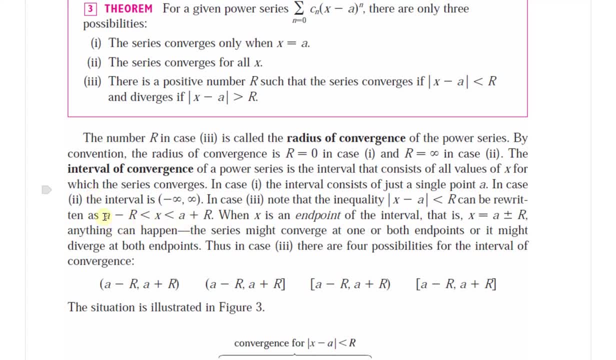 we can get an integral of the interval of convergence where a, uh, if, where x is going to be between uh negative, yeah, it's going to be greater than a minus r and x is less than a plus r, so you just rearrange this and uh, when x is an end point of the interval, that is, x equals to a plus or. 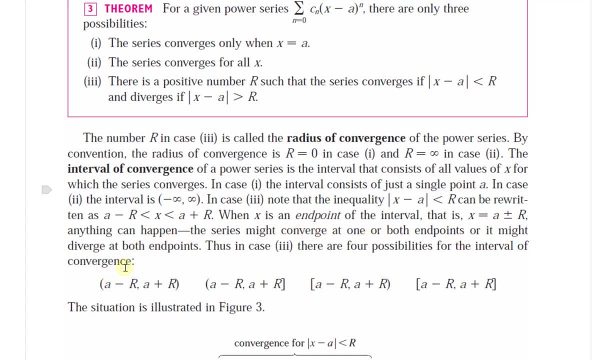 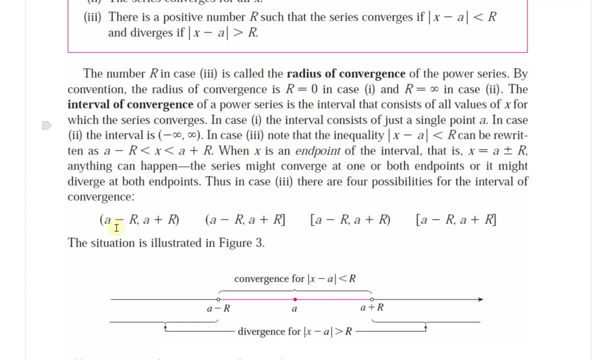 minus r, anything can happen. the series might converge at one or both endpoints or might diverge at both endpoints. thus, in case three, there are four possibilities for the interval of convergence. it could be here with the open bracket where it doesn't converge at the point. so 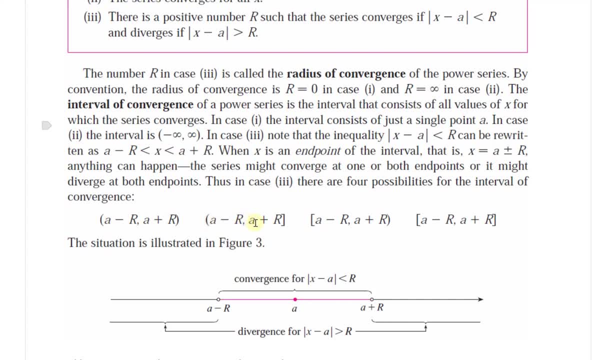 it can be convergent at a plus r, or it can go from a minus r to a plus r, but it can equal this: uh, it can be convergent at a plus r, so. or it could be convergent, uh, at, i guess, remember, at a minus r and all the way up to uh, up to, but not including a plus r. and then here is includes both. 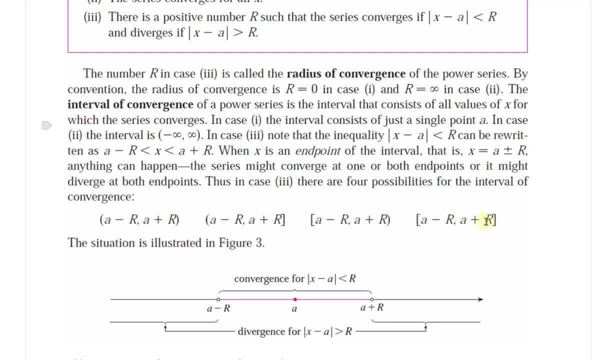 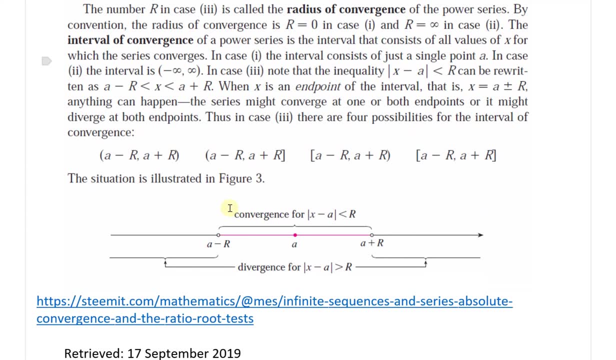 the endpoints: uh, a close bracket- a minus r and uh, up to a close bracket. yeah, up to a plus r. so the situation is illustrated in figure three. yeah, so we have right here, x minus a is less than r as a convergence, and this is closed brackets, and we 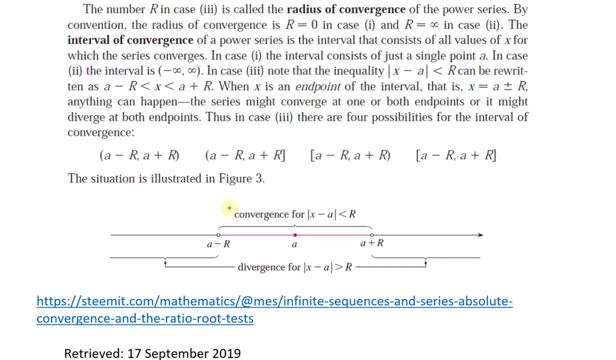 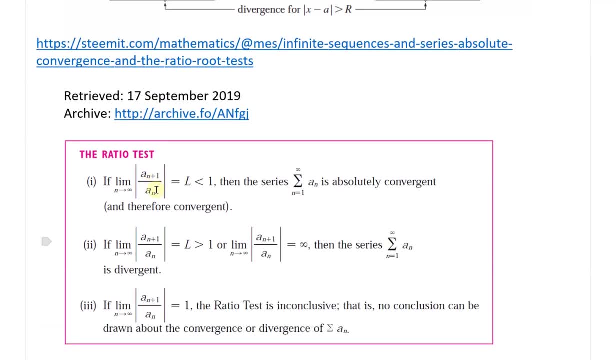 converge, uh, between between this, uh, this, this interval right there, but it diverges when it's greater, but then when it's at here, it could or couldn't. so, going further, now, look at the ratio test and uh, yeah, just a note, i'm, i'm uh revisiting all this because, mainly for myself, because uh, 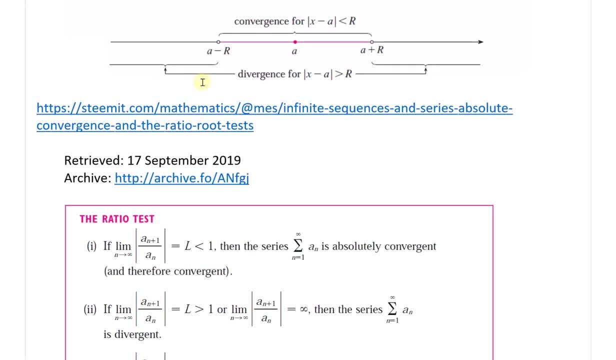 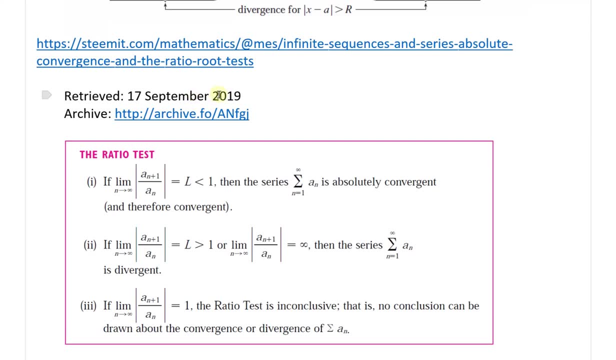 sometimes i go a long period without doing these power series or just uh without doing a calculus book. i'm calculus uh or math video because i'm doing uh, researching other things, such as uh hashtag free energy and hashtag anti-gravity- if you see my gyro videos anyways- so i'm just 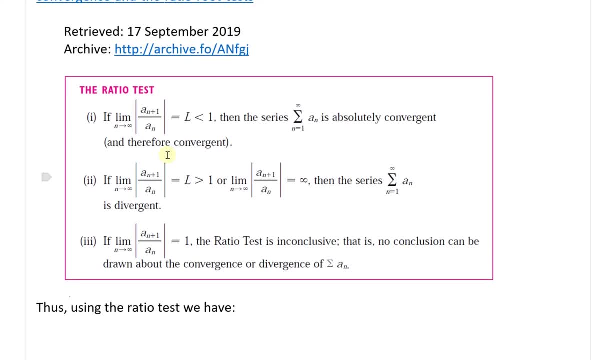 getting a refresher right here, so uh recall for the ratio test. so the ratio test is: if the limit of, as an approach, infinity of absolute value of a n plus one, uh, divided by uh, a n equals to l and it's less than one in the series right here, uh, summation of n equals to one, to infinity of a n. 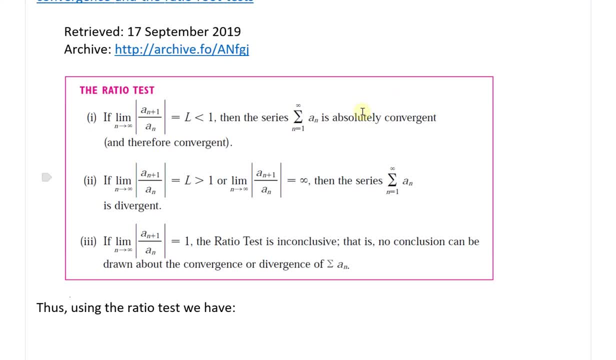 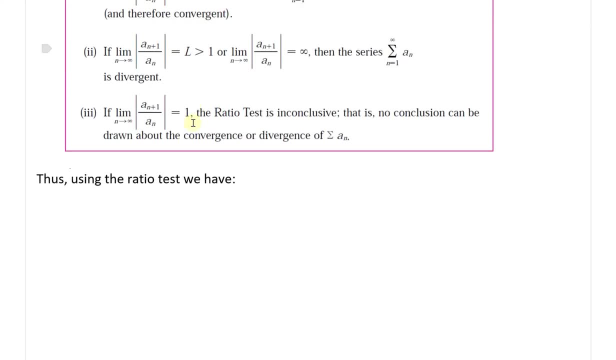 is absolutely convergent and therefore convergent. if it's absolutely, absolutely convergent, as i'll use the comparison test, which also reference later- and that's converged, uh, and then here, if the limit, uh, right here, is equal to l, but it's greater than one, or this goes to infinity, which. 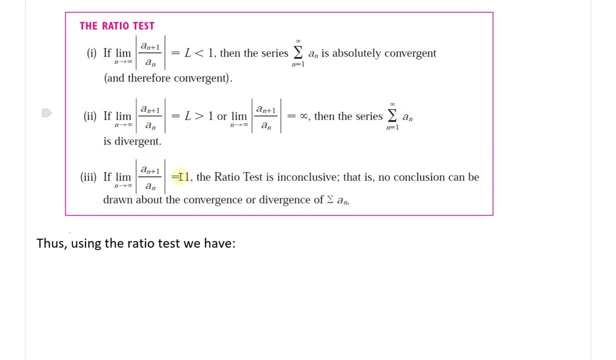 is the same thing, both greater than one, then the series is divergent. but if it equals to one, the ratio test is inconclusive. that is, no conclusion can be drawn about the convergence or divergence of the summation a? n. all right, so thus using the, the ratio test we have, so our a? n. so let's just. 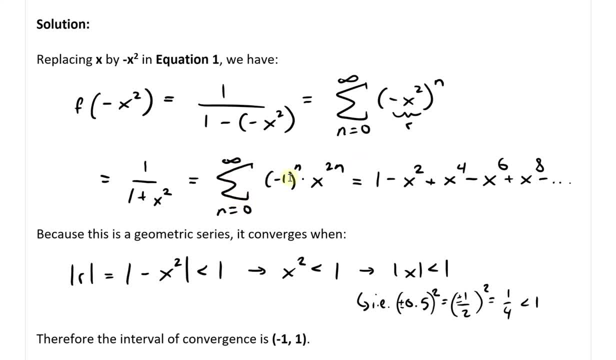 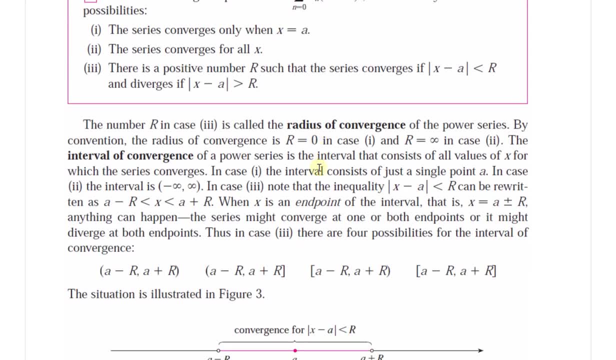 write this out, so let's just write it down over here. so we have- let's start from this one. here's a summation of uh from n equals 0 to infinity of negative 1 power of n times x to the power of 2n. so thus we have is- let's write this down here: infinity n equals 0. 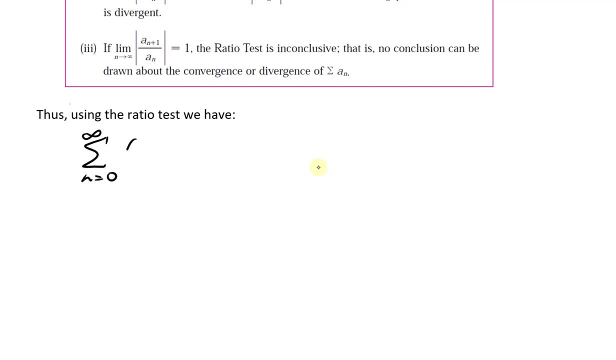 and i'm gonna let- actually we'll write that after. so this is going to be negative 1 to the power of n times x to the 2n, so we'll call this a n. yeah, so thus what we have is: uh, so we have right here. 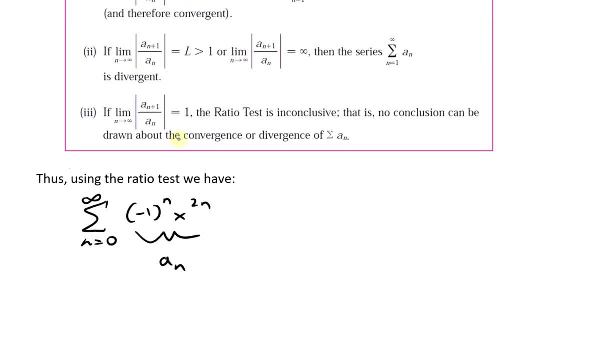 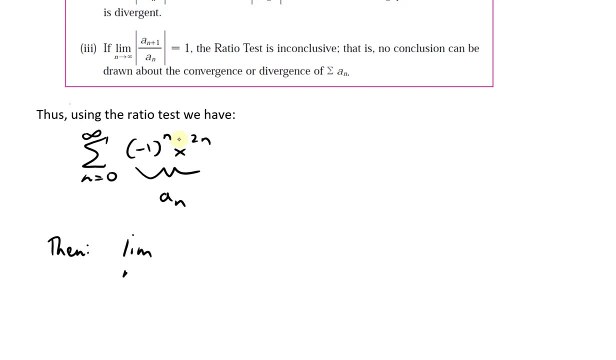 we just apply the ratio test limit at a n plus 1 divided by a n, absolute value as n approaches infinity. so i'll just write then: limit as n approaches infinity of uh of this is going to be a n plus 1 over a n equals to limit. yeah, 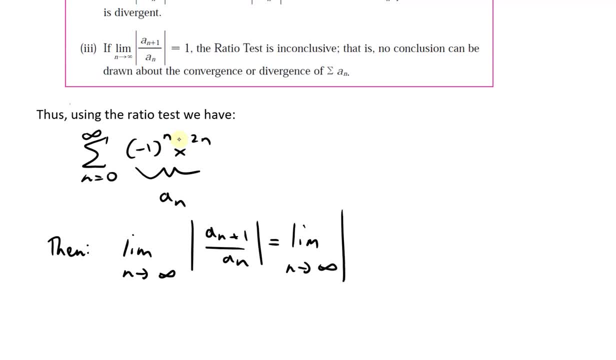 limit as n approaches infinity of. and then let's plug this inside: so negative 1 to power of n plus 1 times by x to the 2n plus 1, that's going to be 2 plus 2, so you can just go 2 times n plus 1. 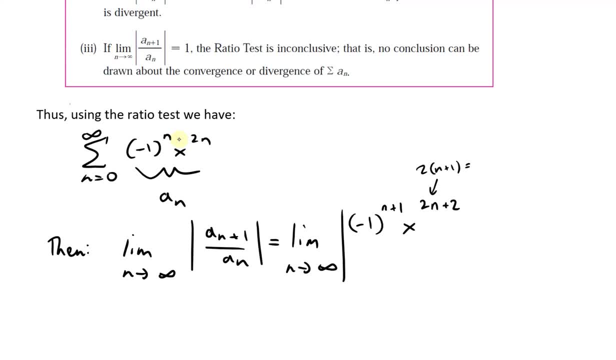 expand that this is going to be equals to um. i'll put it like that: this just equals to 2 times n plus 2.. just write that over there like that. all right, so we're going to be dividing this by: i just are a n, so negative 1 n. and we're going to be dividing this by: uh, just our a n, so negative 1 n. 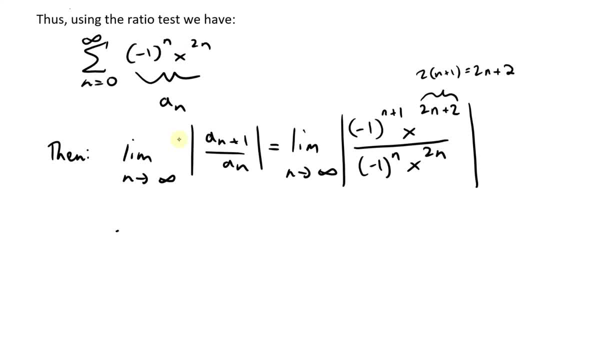 x to the 2n. so now what we can do is subtract, so this equals 2. let's write the limit again. limit is n approaches infinity, and then absolute value. so let's see what happens here. we could just combine the power, so n plus 1 minus n, this is going to be power of n, i mean the power of 1. so 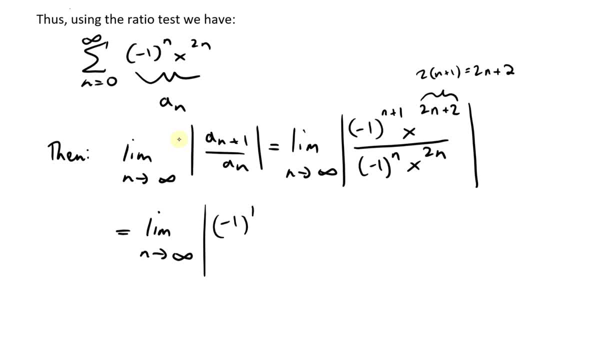 this can be: equals negative 1, power of 1.. uh, yeah, so we actually don't need that big of a sign, so we just go negative 1. this is going to be 1.. this is going to be now: x 2n plus 2 minus this: uh 2n. 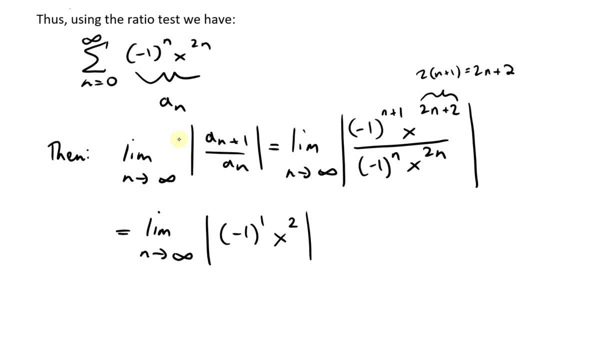 because you could just subtract them like that and then this is going to be just the absolute value is that x squared is always positive. this is the only thing that could be negative. so we and this is just going to be positive, then it's positive. 1, just get rid of it. this is equals. 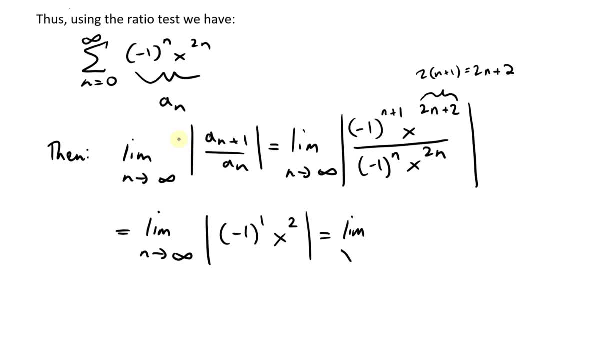 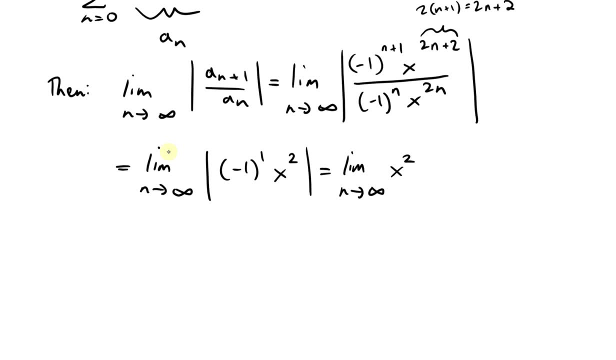 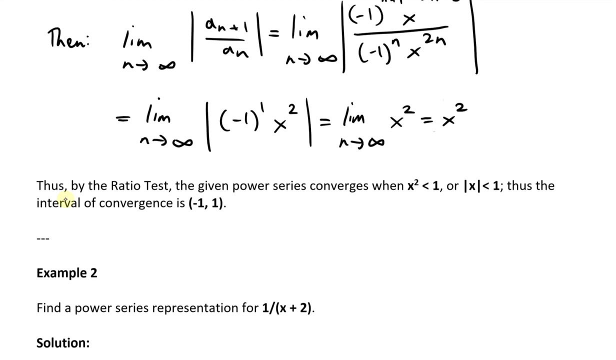 to the limit, as uh n. to limit, as n approaches infinity, of yeah, of x squared. and notice, here there's no n, so this is just x squared. it's not dependent on n, so this just equals to x squared, yeah, yeah, here i'll just box this out. so then by the ratio test, only time that this is. 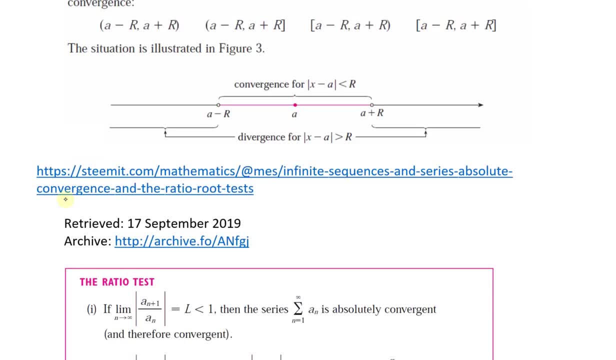 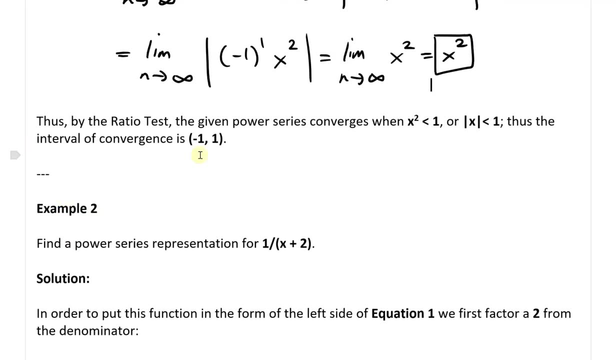 uh, convergent is when this, uh, this limit is equal to l- yeah, so we equals on- is less than one. that's only time it's convergent. so what we have is so, thus, by the ratio test, the given power series converges when x, squared, is less than one, or the absolute value of x is less than one, exactly as i. 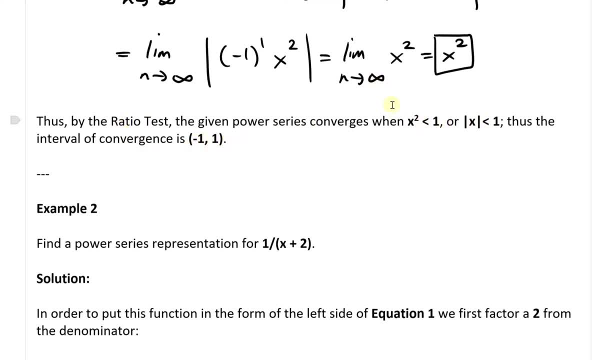 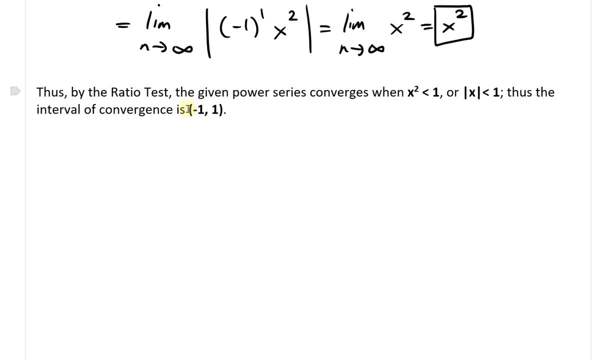 showed before. thus, the interval of convergence is negative one and one, and the radius of convergence actually uh. here i made a slight mistake here. this could be, uh, negative one to one, uh, or could be. so it could be negative one to one. it could also be uh, use the close bracket. 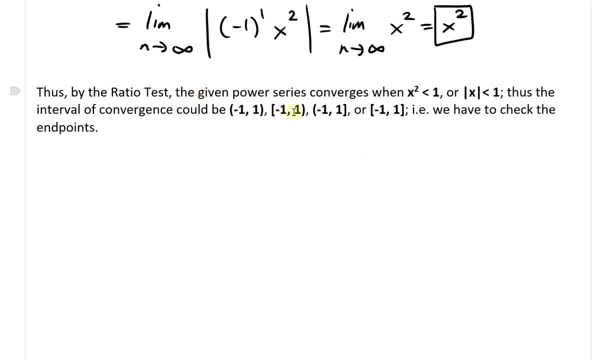 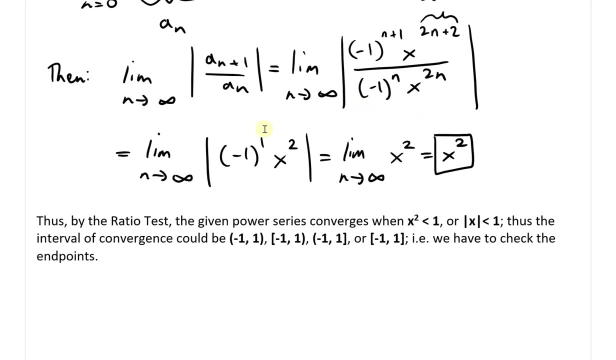 yeah, it could be a negative one to one, or it could be at negative one two, one there, or uh, negative one, uh, two, including, uh, yeah, square bracket one, or we'll have square bracket negative one and one. so at the end points: uh, we have to the end point. yeah, I just while making this video, I just realized that. so this: 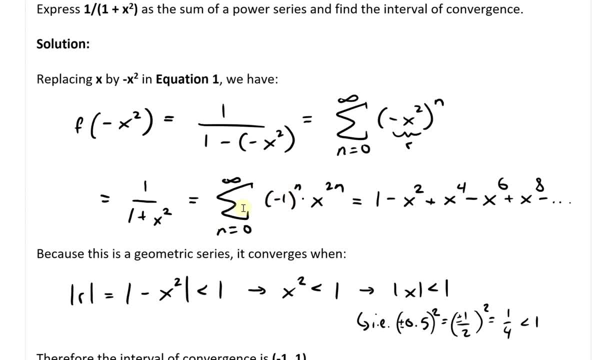 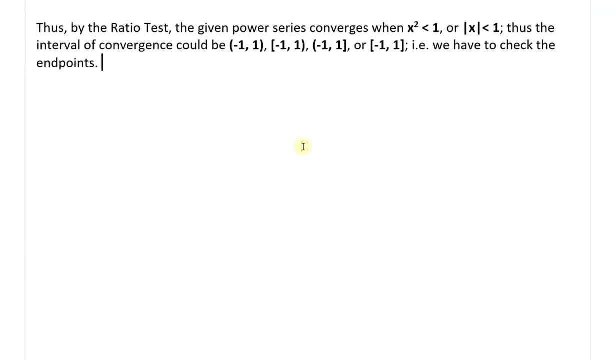 is actually pretty easy for this case because we can look at this formula right here. so summation from n equals 0 to infinity of negative 1 n times X, 2 n. so this equals 2 now. so I'll just write here at: let's just start at the end. 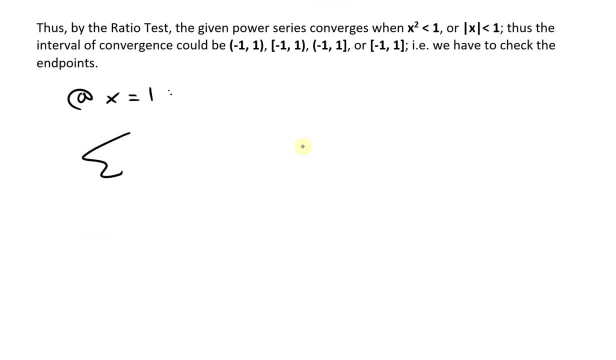 point at X equals to 1. we have summation, so summation of up to infinity of n equals 0, of negative 1, and and then this is going to be now 1 to the 2 n. this is just equals to 1, so this just equals to. also I'll put like here: 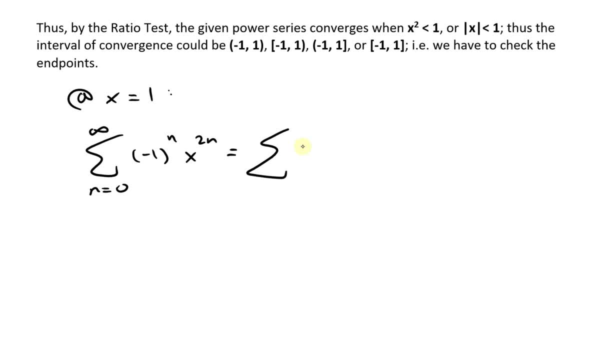 actually X, 2, n, and this equals to summation right here and equals to 0, and this is going to be negative 1, and and this is going to be times 1 to power of 2, and that's just gonna be 1. so all we have is is negative 1 to power of n. this 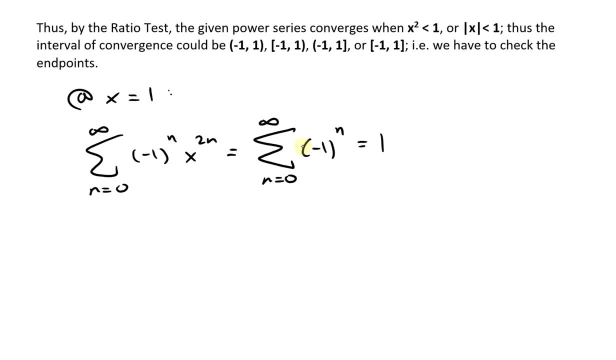 equals to 1 egg n equals to 0, that's going to be 1. when it n equals to 1, we're going to have a minus 1. when n equals to 2 is positive 1, then 1. n equals 3 is negative 1. so what we end up? 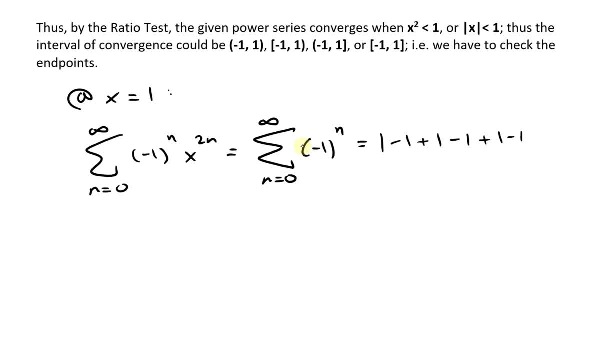 having is a plus 1, minus 1, etc. and then plus dot, dot, dot. so, in other words, the partial sum right here. so if right, this is the partial sum s 0 is equal to 1. then the partial sum right here up to this point is going to be s 1. yeah, a 0. 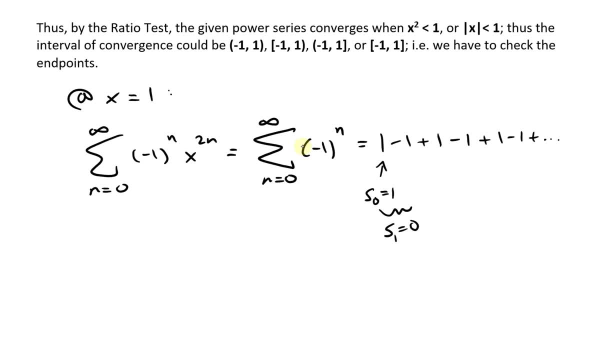 is 1. s 1 is equal to 1, minus 1 is 0. and then this one right here is going to be from, from all the way across, their partial sum of this- this, these three terms- is gonna be s3, or I mean s2 equals to this. 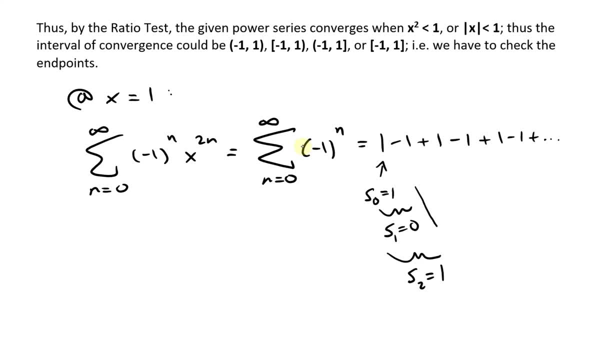 is gonna be plus one, then you always minus one. so it goes to yes. so it goes basically to one zero, one zero, one zero. in other words, this is, and then dot, dot, dot. this is divergent, it does not converge, it just goes from ones and zeros non-stop. and likewise music, exact same thing. at X equals to negative one. 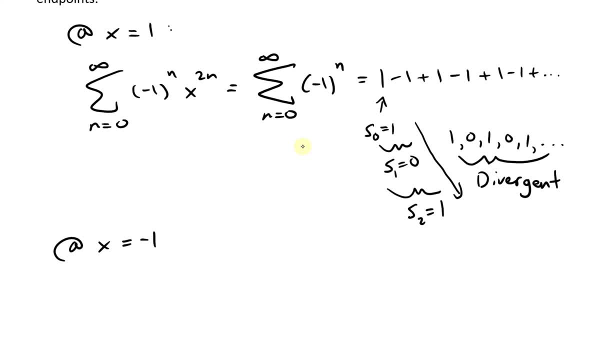 so at the other endpoint, at X equals negative one we're gonna have instead of this right here, we'll have negative one. actually, I don't need to write this one here, we just put this on all into one. so this is plus or minus one if you plug. 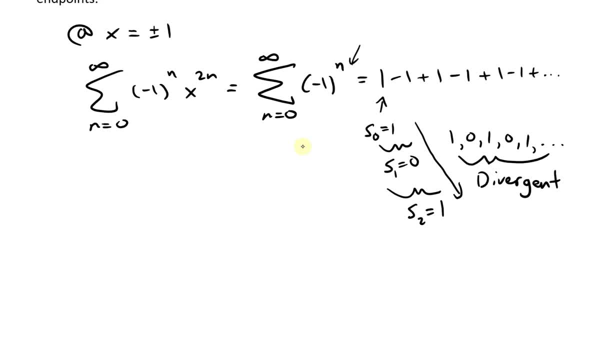 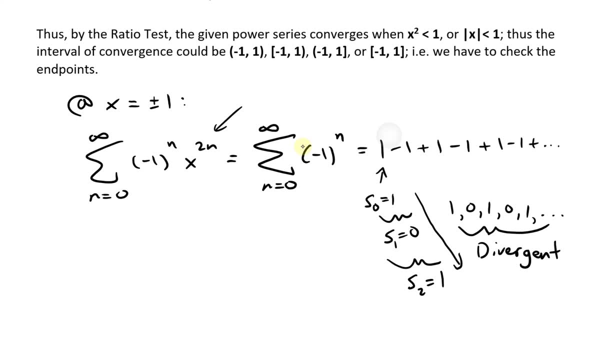 this inside. what we end up having is this right. here is- or just put it here at you- at X equals to plus or minus one. we have. move this here: plus or minus one to power of two, and this is because this is always gonna be. even what if you have two? 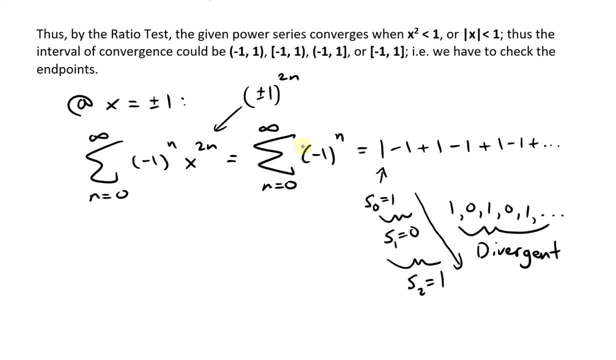 times one is two times twos is four, etc. this is always gonna be positive. it's always gonna be positive. one doesn't matter if it's plus or minus inside, so this is gonna be divergent, so it's right here. this is also part of the 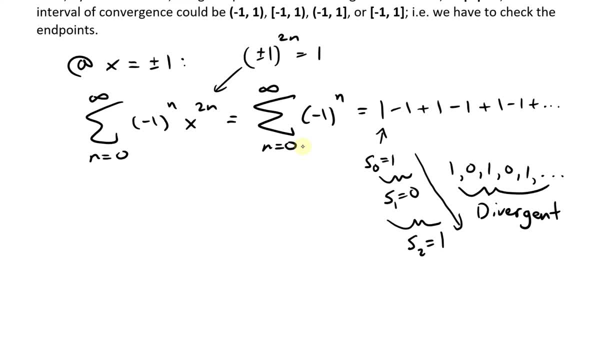 alternating series test to be more formal or just to be more in line with the, in line with the theorems that I did before, but I'll go over that later in this video. and yes, so thus it's divergent on the endpoint. so this is: 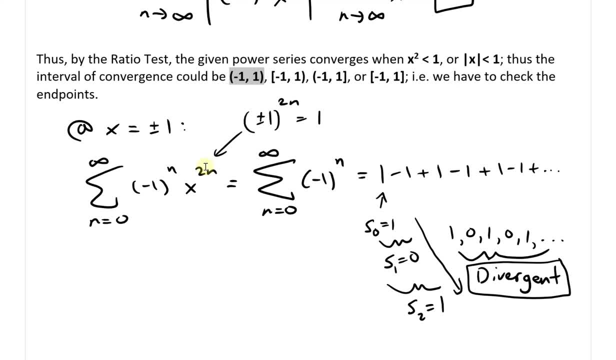 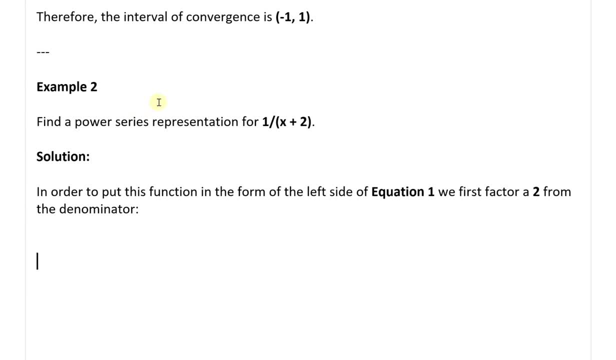 going to be the interval of convergence. so yes, therefore, the interval of convergence is negative, one to one. so now let's look at example two, and this example states: find a power series representation for one divided by X plus two. and this is yes. so, in order to put this function in the form of the left side of a, 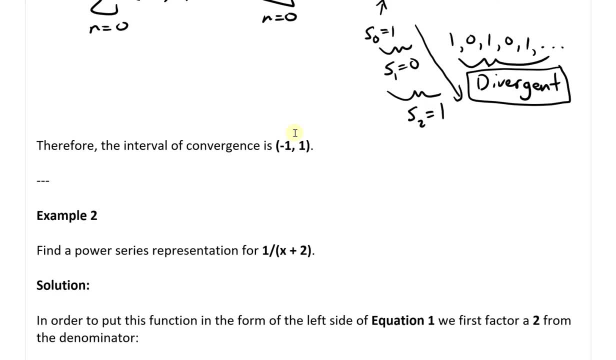 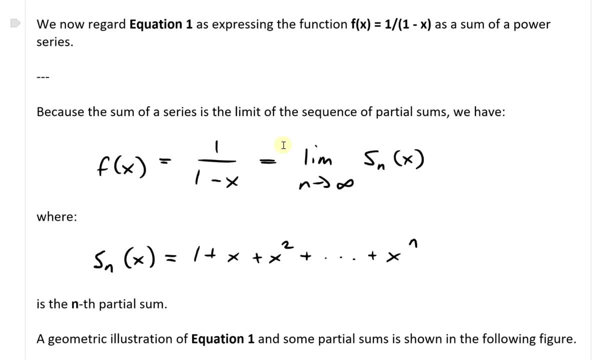 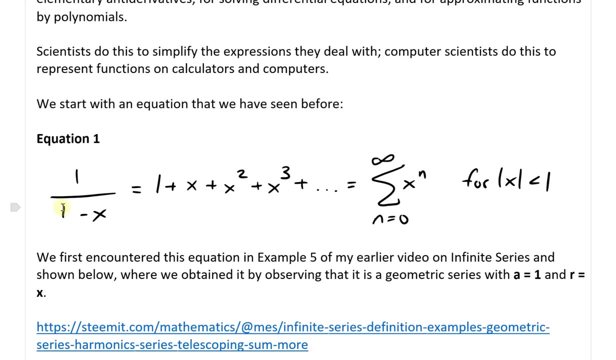 equation one. yeah, because the number equation one has one minus X. let's just scroll all the way up to equation one right here, so this one. keep this in mind. so we have our equation right here: one minus X, but the other one we have X plus two or two plus X. so what we can do is factor out a two, and so let's just scroll. 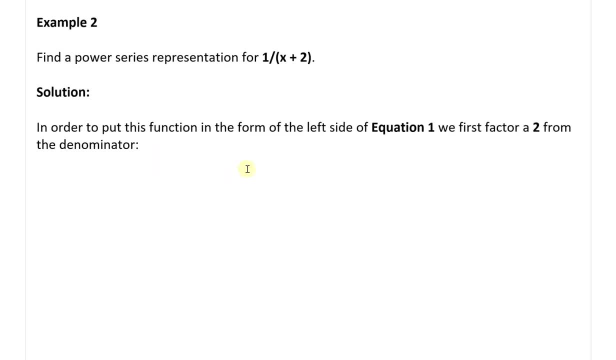 up here. I'm scroll down here. so in order to put this function in the form of the left side of equation one, we first factor a two from the denominator. so what we could do is write one over N. X plus two equals one, and then rearrange this, just factor out a two from the 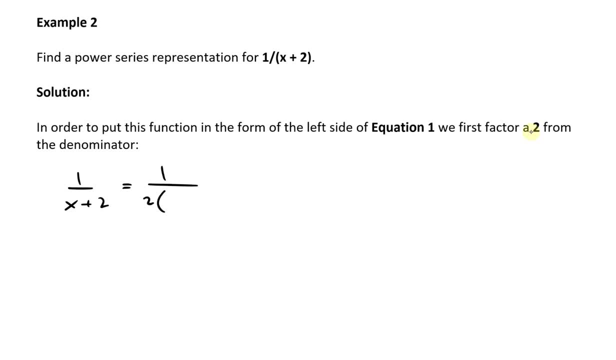 denominator take a two out, so that means we could factor out two- this is going to be one there, and plus this is me- X over two. so here, if you multiply this out two times two and then twos, cancel here. it will back. so all we're doing is: 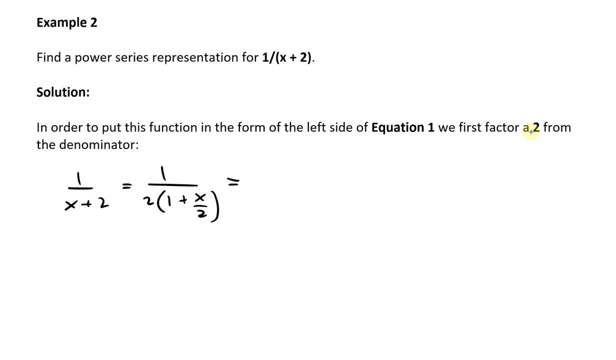 factoring out a two like that. so now what we have is: and then write this in the form of equation: one: this can be one over two, bracket one: this is going to be now a number supposed to be minus X, so this can be the same thing as writing. 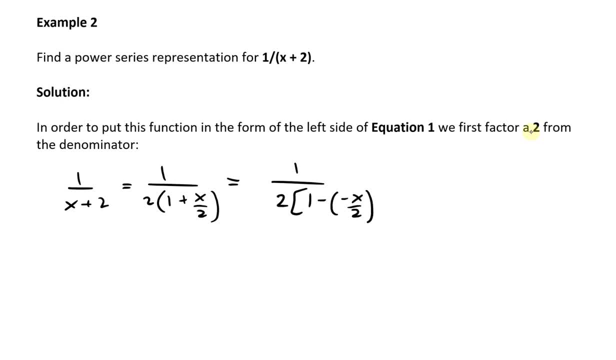 minus minus X over two. let's put a double negative there, so that's. it's in the form of exactly equation one. yeah, so that's. this equals to F of this is the equation one actually can be. take the one over two out, so this can be equal to. 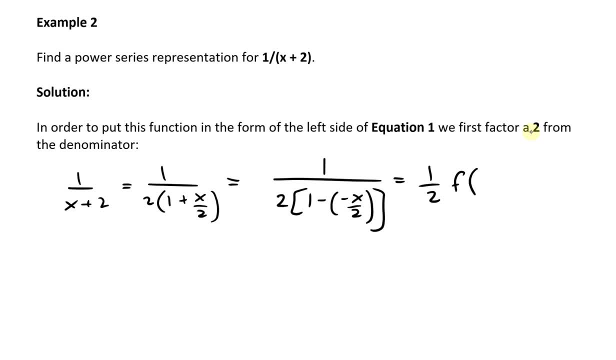 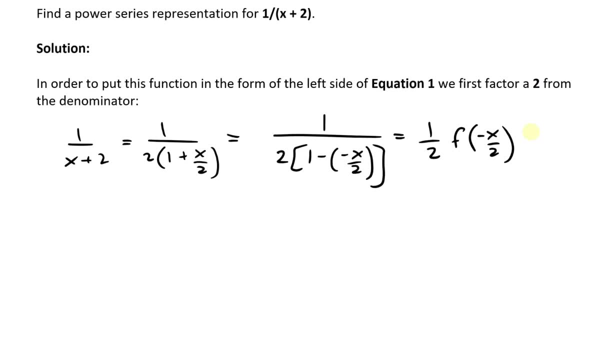 one half of equation one, negative equation one, but with this negative X squared inside. so that is our of equation one and plug that inside. we get now into the power series we get. this is gonna be equals to summation up to infinity of n, equals to zero, and this 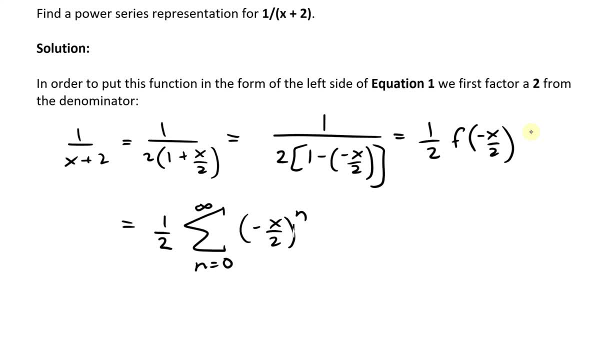 is gonna be negative X over two and it's just replacing X with negative X over two, and now this equals two. yeah, we're gonna. we could stop here, but let's just keep writing it further. we could expand this out into summation and summation up to: 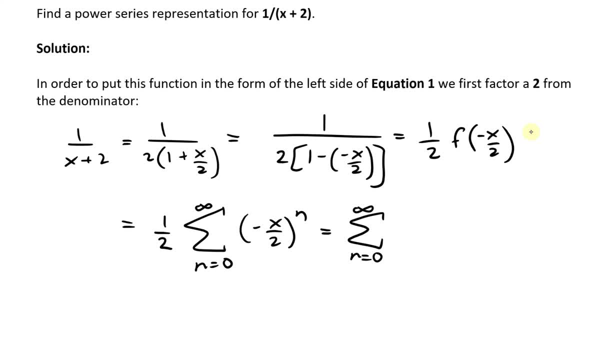 infinity from N equals to zero, and then we're going to put this in the form of equals to zero. this is going to be a. I'll put a giant division like here, because we have a to the power of n and we have a to the power of one. there's 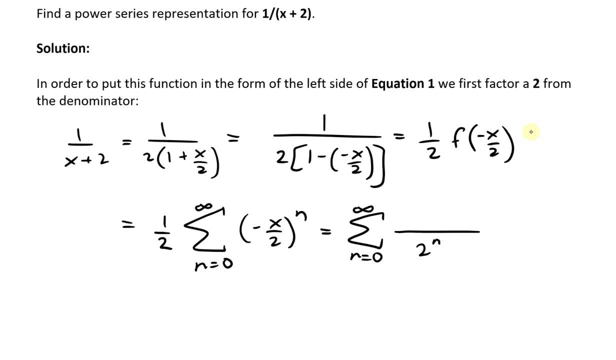 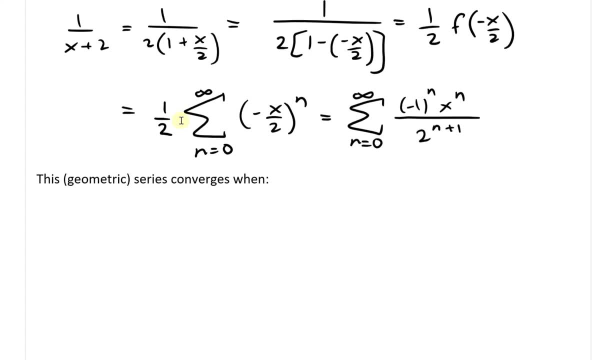 we've combined those, move it inside. it's gonna be two to the n plus one, and then we'll have a negative one to power of n and an X. and yeah, now this geometric series. yeah, this is just a geometric series number, it's just our equation one. 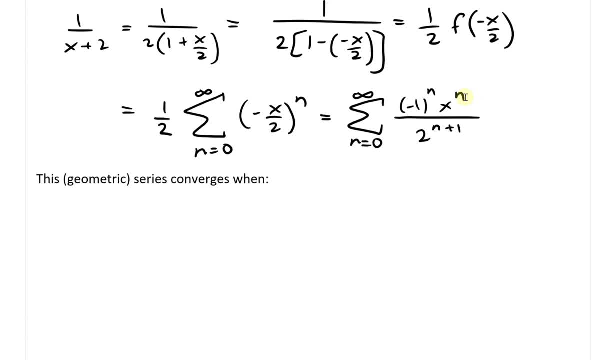 but just varied by changing the input there. so this geometric series converges when, when we have the R value, absolute value of R is equal to, in this case, absolute value of negative x over 2 is less than one. yeah, so this, this, this just means that, well, the only thing that could be negative is the X, so we could check the. 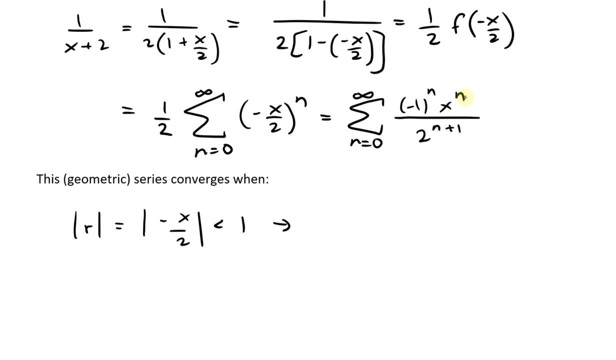 absolute value of it and remove the a negative there. so this is the same thing as writing absolute value of X over two. this is constant. less than once move the two multiplied over onto the other side. so we get absolute value of X. this is less than two. this is when it converges. so radius, radius of convergence is two and by the geometric, 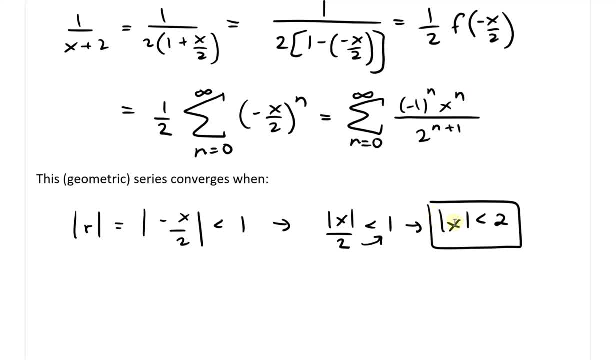 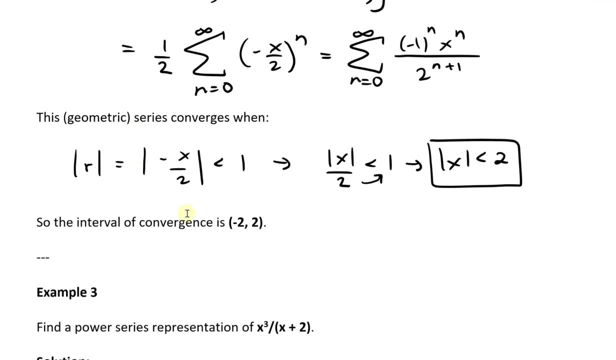 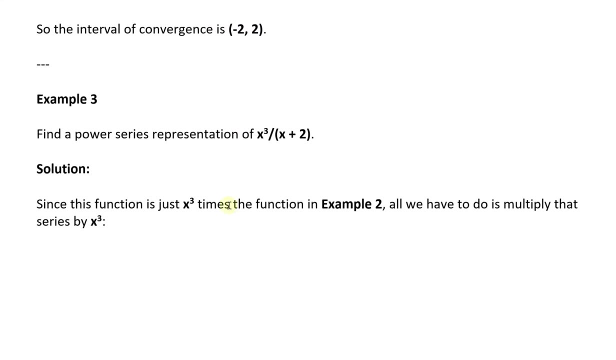 series, uh, theorem above, uh, from my earlier video, then the um, then this means that the interval of convergence can be from negative two to two. and uh, yeah, to write this down, so, uh, so the interval of convergence is, uh, from negative two to two, and not including the endpoints. so going uh on, uh so. 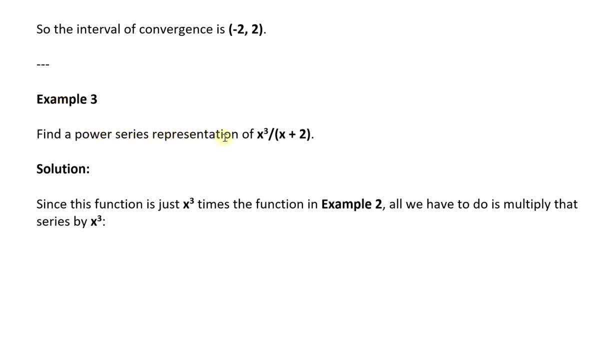 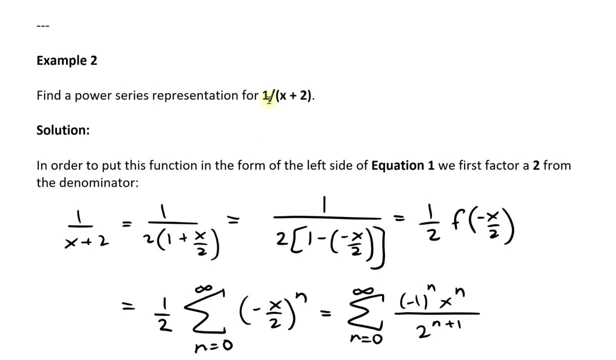 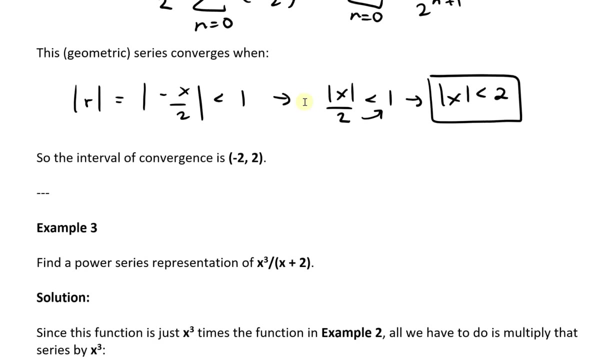 now let's look at example three, and this one states: find a power series representation of x cubed divided by x plus two. now, this is exactly the same thing as example two, except we have an x cubed. so we have an x cubed multiplied by one, divided by x plus two. so, uh, let's look at the. 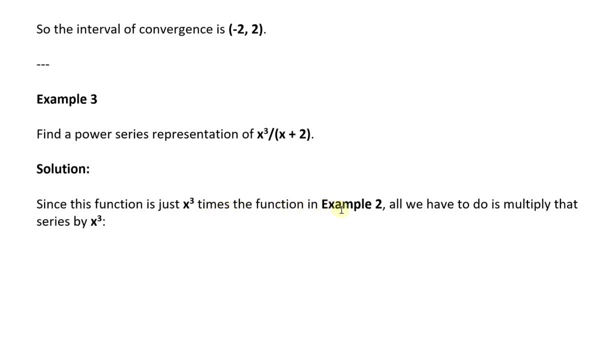 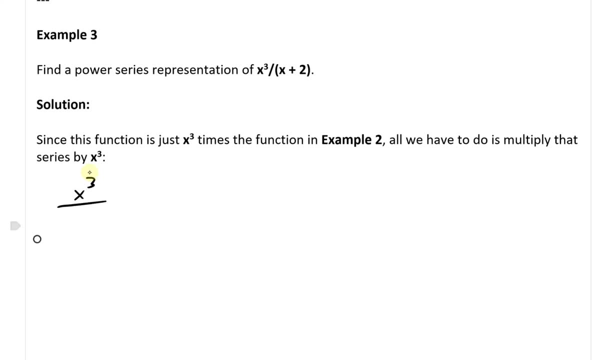 solution. so since this function is just x cubed times the function in example two, all we have to do is multiply that series by x cubed. so what we have is x cubed over x plus two. this one is going to be equal to x cubed multiplied by just one over x plus two. 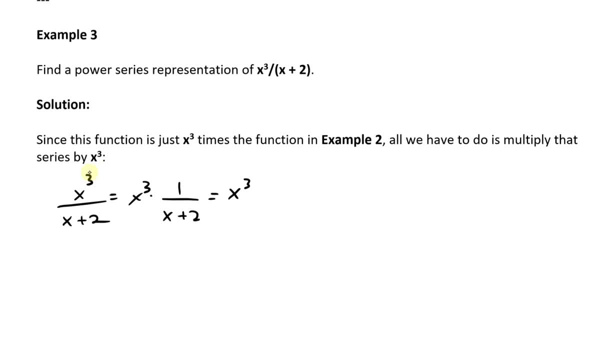 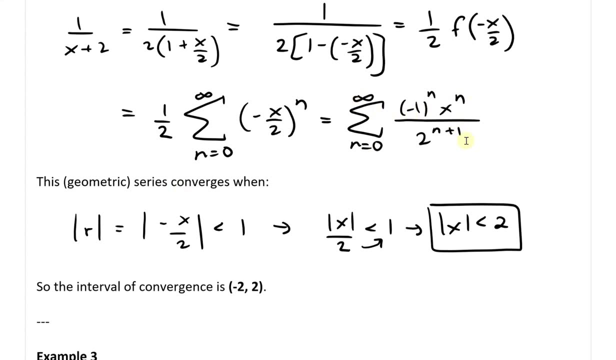 and now we already know this one. this is x cubed multiplied by, and we know what this is in: one over x plus two in power series. now notation, that's this one, right here. so as a power series that one over x squared plus two is equal to: from example, two n equals zero to infinity of negative. 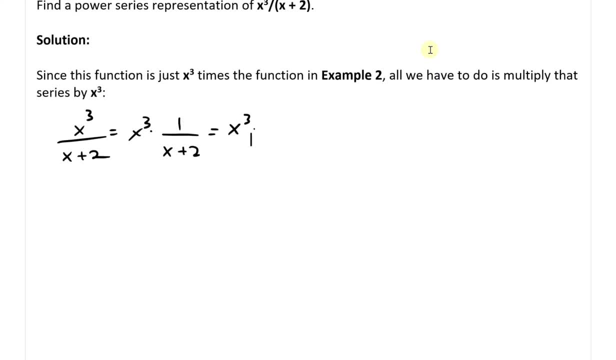 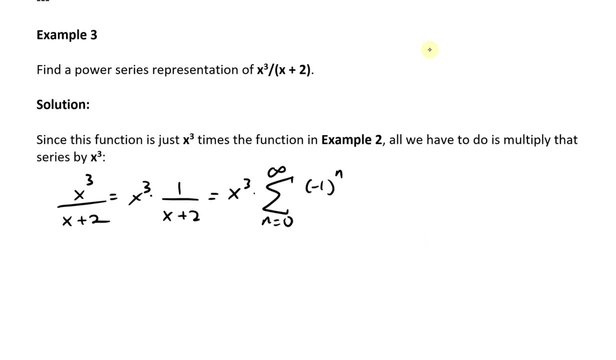 one n times x n divided by two n plus one. so let's write that down. so this is going to be the summation from n equals zero to infinity, of negative one n, x, n over two n plus one. just double check, that's right, so that's right. so now what we? 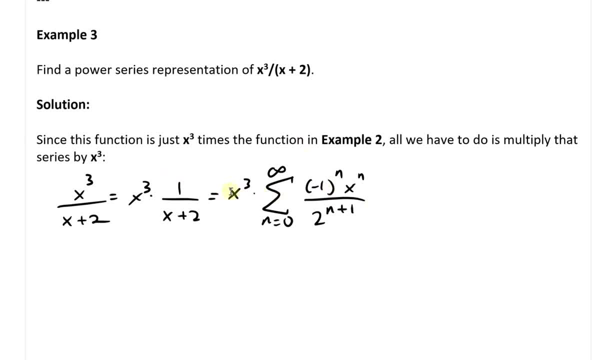 could do is: well, this is x cubed, this is x and this is uh. for any value of x, it's just a constant, so we can multiply that inside and this is going to be equal to the summation. uh for up to, up to, from n equals zero to infinity. 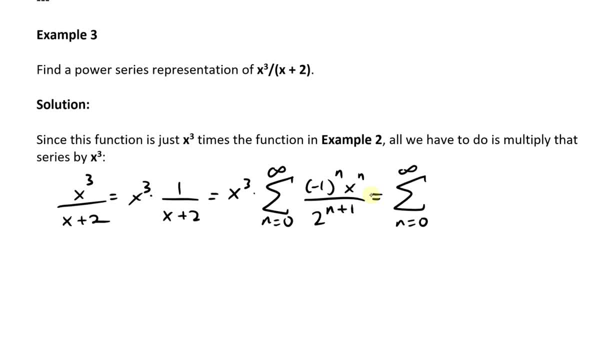 and this is again, this is not dependent on n, so it's equivalent to a constant. we can move that inside this x, so that, and i'll write this in this form: uh, negative one, n over two, n plus one, and now we'll have, is this x n times it by x, cubed is going to be well, x n plus three. 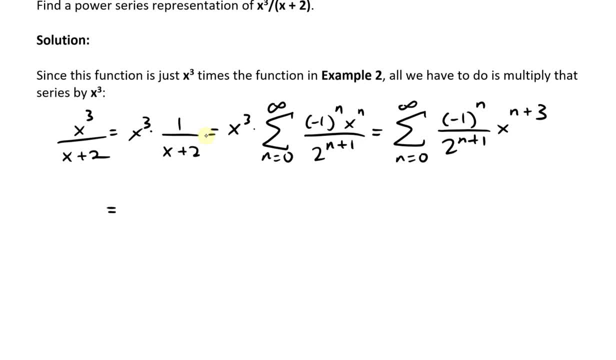 and now, if we were to expand this out, this is going to equal two. when n equals zero, negative one, n is negative one, zero is going to be just one. and then two. so two to the power of zero plus one, that's just two. and now here, x to the n plus three, so n is zero. 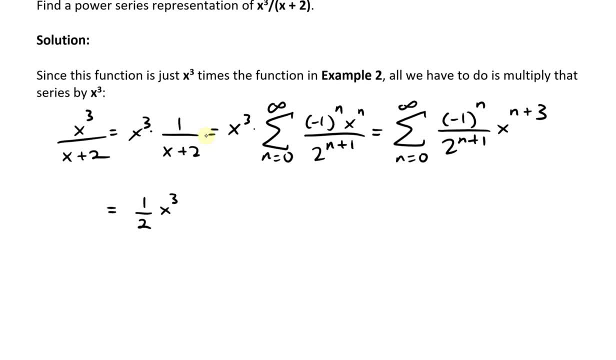 we'll just- let's just be uh x to the three and then plus uh, or the next one's going to be actually a minus. when n equals one negative one, power of uh one is going to be negative one, and then this is going to be divided by two to the power of one plus one, that's two. so that's two to power two. 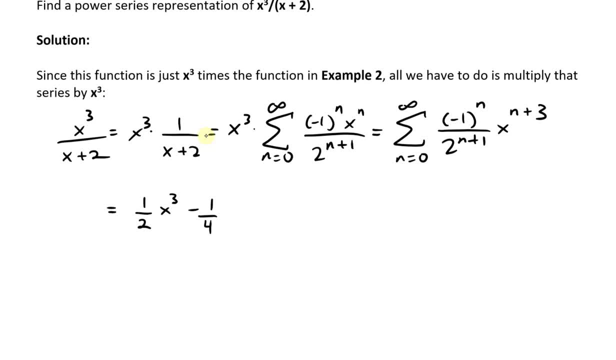 that's just four. and likewise, here, this is going to be x to the one plus three, which is, uh, four, x four, and then x. one. when x equals to two, yeah, when x equals to two, what we end up having is negative. one to the power of two. uh, that's going to be well positive. it's an even power, so positive. 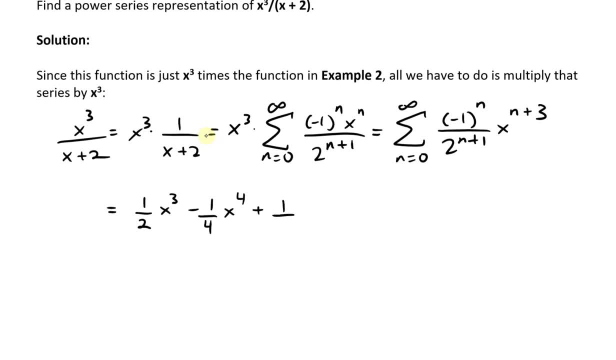 two or a positive one over now. this one's going to be two to the three, because it's just me. two plus one and it's two, so two to the three, that's just going to be well. four over this. this one times two, so that's going to be eight. two to three is eight or four times two, like that we just carry. 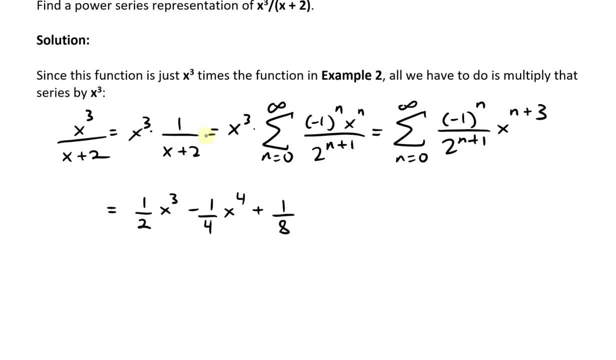 that, and then this is going to be x to the uh. two plus three, that's five. now we do is the next one's going to be uh. this is the n is equal to three. that's going to be odd, so it's going to be negative. 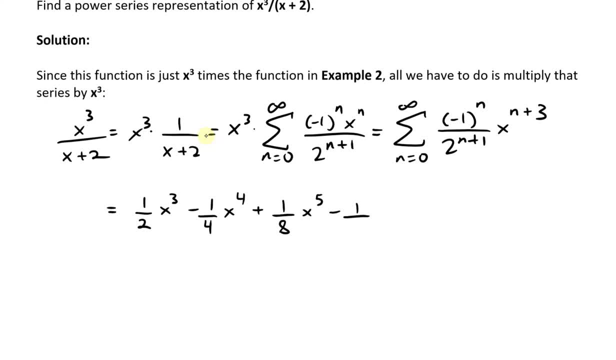 one over, and then this is going to be two to the three plus one, that's two to the four, or eight times two, and that's just going to be sixteen. then this one right here, x to the three plus three, is six, and so on. so then plus, and continues on and on. and now, to simplify this even further, 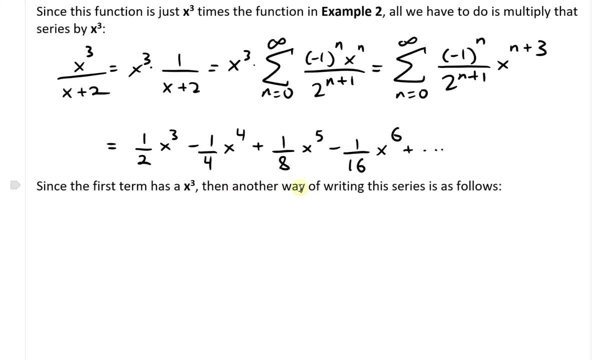 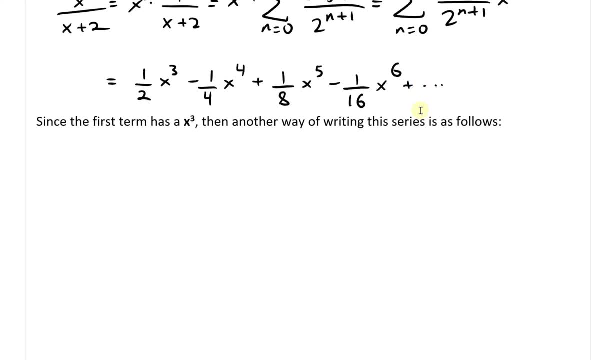 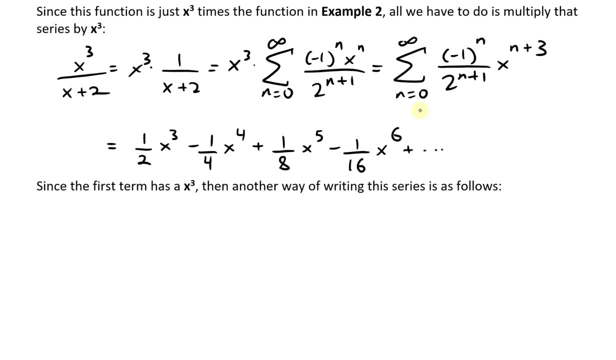 since the first term has a x cube, then another way of writing this series is as follows: instead of dealing with x- n plus three, we could just use x- n by starting instead with n equals to three. so what we could do is let's just write this all from the beginning, so we'll have x cubed just right here. 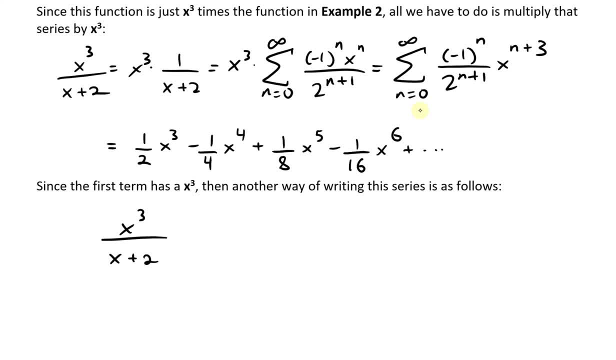 x cubed over x plus two, this is going to equal two. so if we're going to start with, n equals three, so we go from here. this is up to infinity and n equals to three. so when we have this, n equals to three, uh, we're going to write it like this, so that 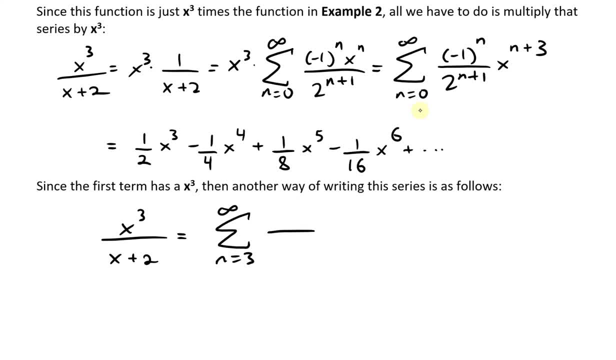 uh, this x, uh to the n. so we'll start and start with x to the n instead of x to the n, plus three. so this is going to be x, and so when n equals three, this is just going to be x, cubed there, and then uh, the bottom one is going to be two, so that's two to the power of one. so we can't do uh. 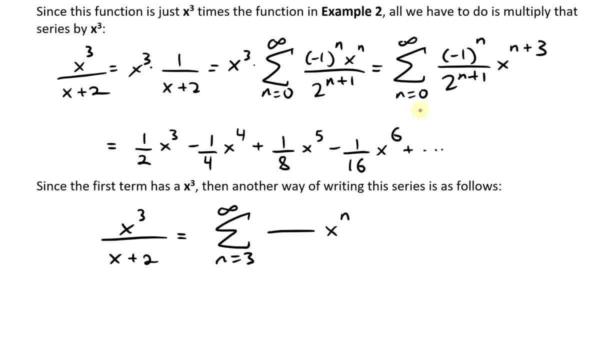 two n plus one, because when we have a three there that starts at four. so what we could do is, well, we could do two to the n, so two to the n of the initial one's gonna be three, so we need to get to the one, so we minus two. 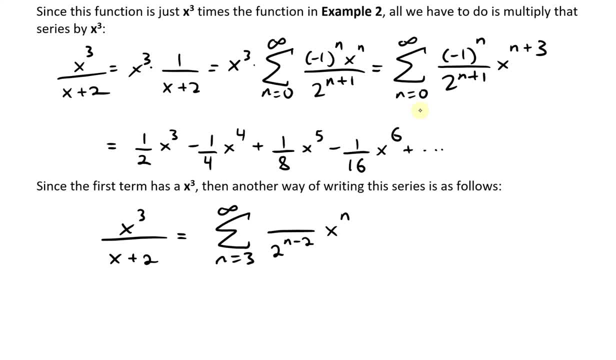 so two to the three minus two, that's gonna be two to the power of one. and then, when n is four, we'll have two to the four minus two, which is two, that's two to the power of two. and then now for the uh top part here. this is going to be the initial is going to be positive. 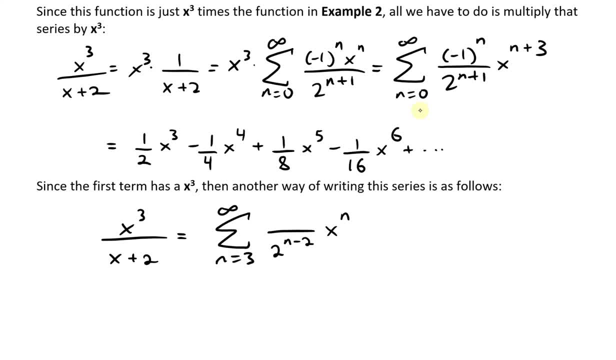 so we can't do uh n, because that's going to be an odd power, that's going to be negative. so we'll do is negative one, n. and now, if this is odd, to make it even, we just subtract by one, so that when n is equal to three, we have n? uh three minus one, that's two. so this is gonna be. 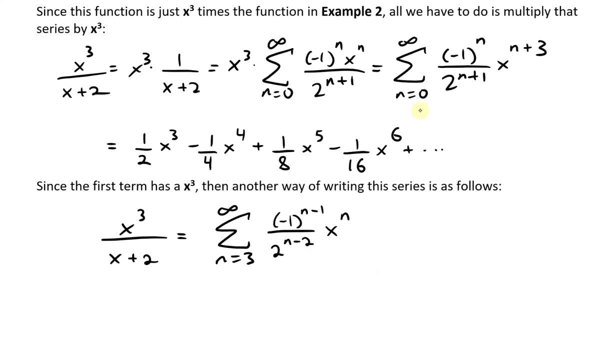 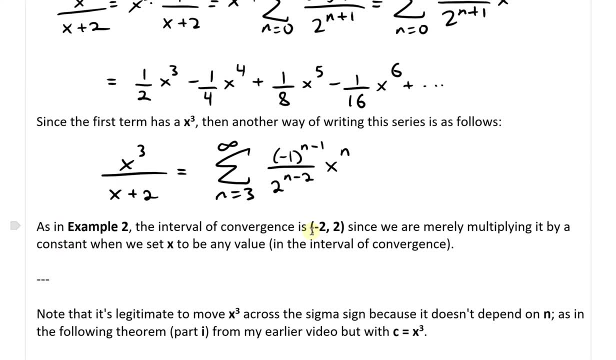 positive, then when n is four, we minus one, that's three, that's gonna be negative, and so on. so we could just leave it as is like here and uh, yeah, as an example two, the interval of convergence is going to be from negative two to two, and not including the end points. uh, since we are 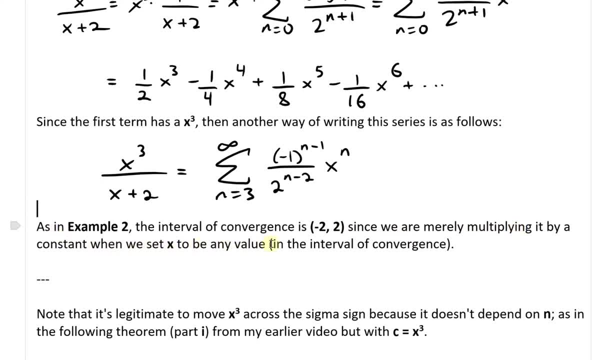 merely multiplying it by a constant. when we set x to be any value and bracket, uh yeah, in the interval of convergence for this convergence to occur. but any value that you set x, it's just a, it just can be considered as a constant because it doesn't depend on n in this series and note. 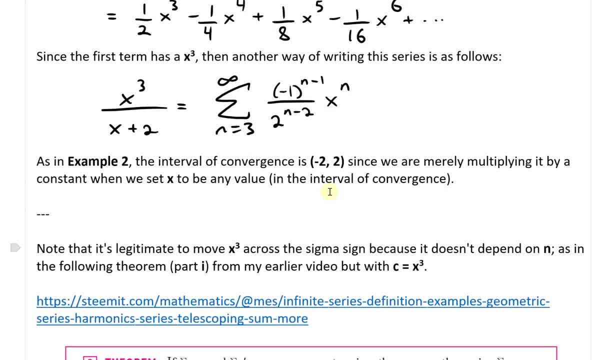 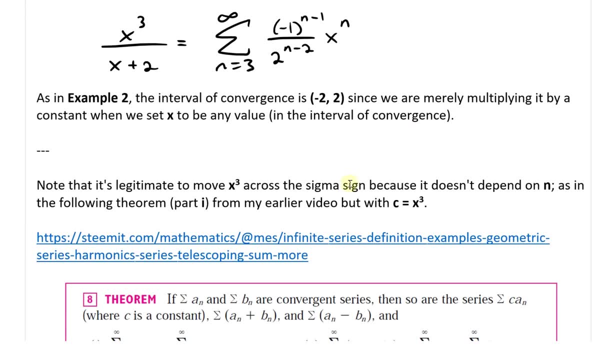 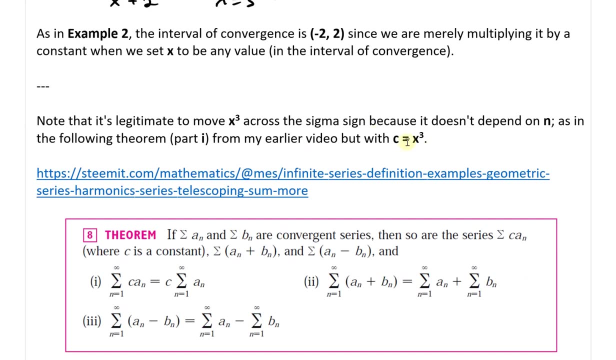 that it's legitimate to move x cubed across the sigma sign. so we have x cubed here and move it inside this summation like this: x, n plus three. we can do that because it doesn't depend on n, as in the following theorem as part i from my earlier video, but with c equals to x cubes from: 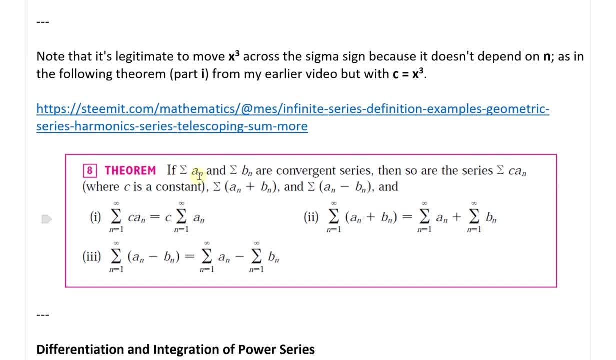 my earlier video theorem. if the summation a? n and the summation b? n are convergent series, then so the series summation c times a? n, where c is a constant, and likewise we have here the summation a? n plus b? n or a n minus b n. subtraction of these or addition is also going to be convergent. 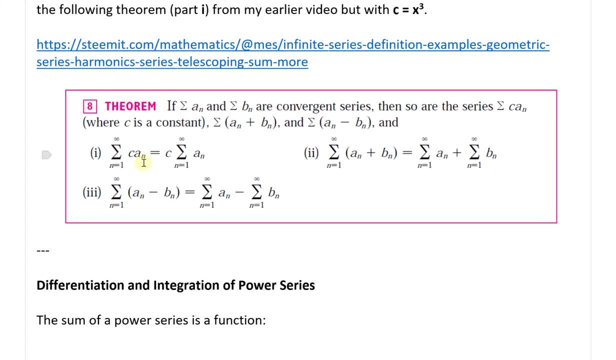 and this is part i, when you have summation, n equals one to infinity c of c times a n. we just move the c outside or inside, it doesn't matter, and these are equal to each other. so the, in our case c, is going to be x. 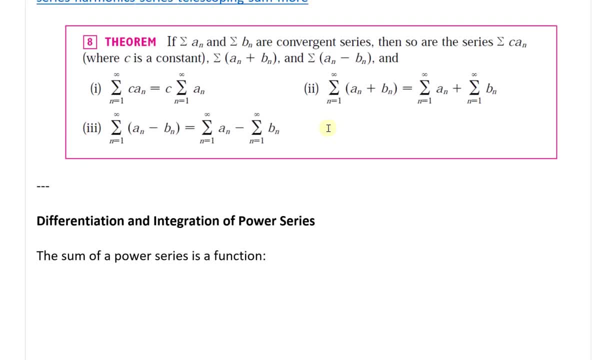 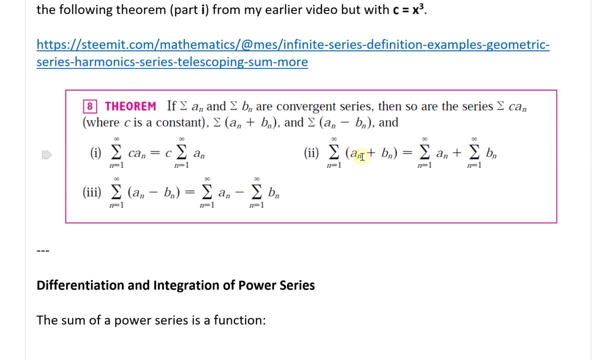 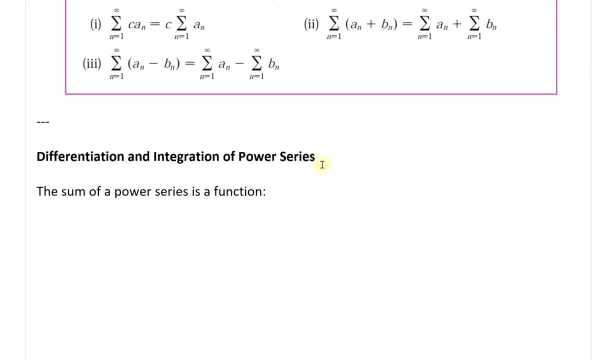 cubed. so yes, this is x cubed, move it inside. and then likewise other part uh, part two and part three, or part i- i and part i- i i, uh. this is just uh, the addition and the subtraction. you could separate these uh terms into their own separate series, like that. so that's very, very interesting. 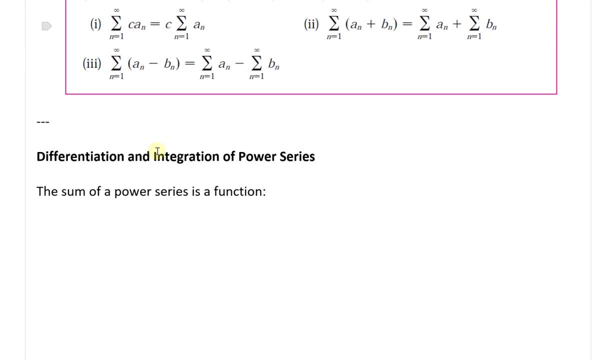 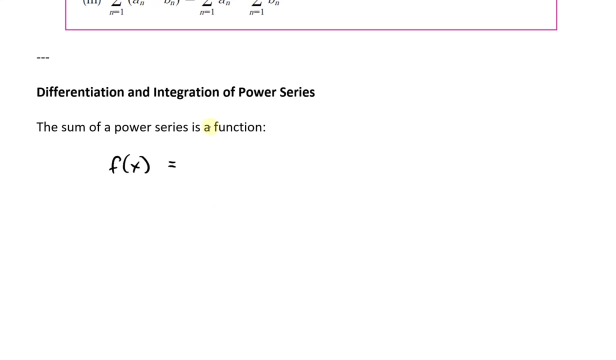 so now let's continue further. yeah, all right. so now let's move on to differentiation and integration of power series. yes, so the sum of a power series is a function. uh, right here. f of x. and now, to be more general, write this as a summation: 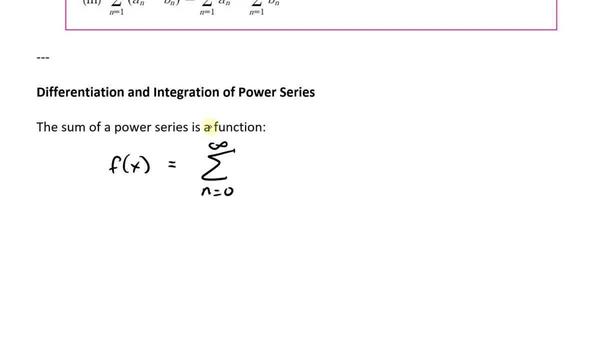 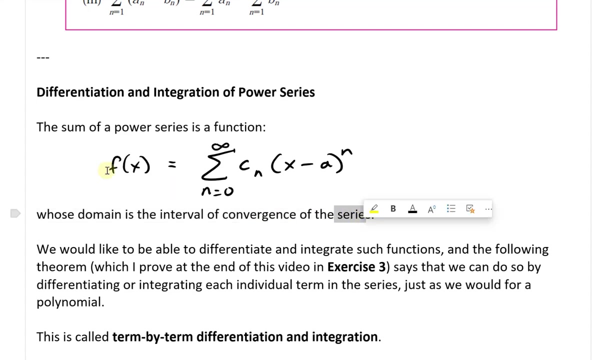 infinity, n equals zero of the coefficient c, n, and i will have x minus a. yeah, just to be more general than to the power of n and uh, whose domain is the interval of convergence of the series. so, yes, we'd write this as a function, and uh, what? and we would like to be able to. 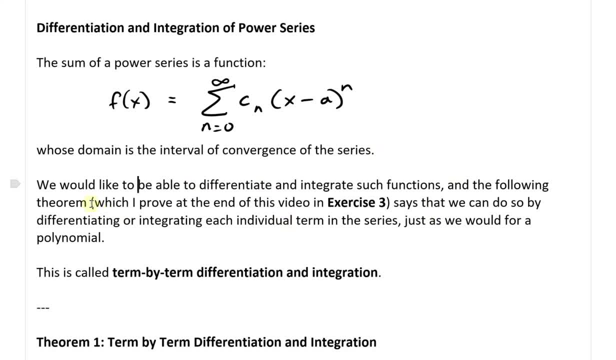 differentiate and integrate such functions. and we would like to be able to integrate such functions, and the following theorem, which i prove at the end of this video, in exercise three- and it's a pretty extensive uh, says that we can do so by by differentiating or integrating each individual. 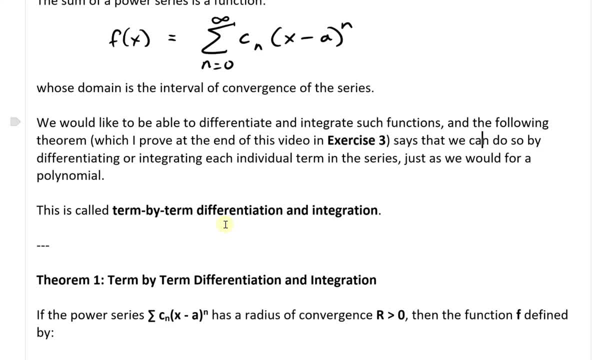 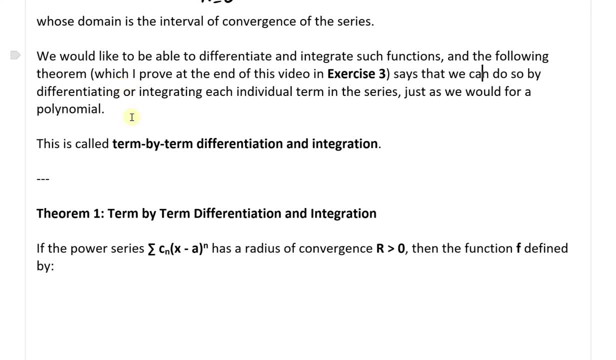 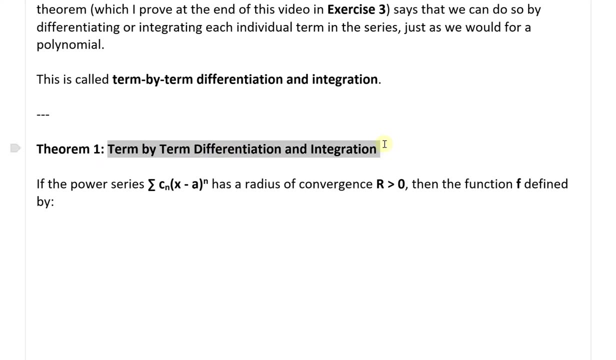 term in the series, just as we would for a polynomial. the difference here is that it's an infinite polynomial which keeps going on. we can nonetheless still differentiate it. this is term by term, differentiation and integration. so let's look at theorem. one is one most important theorems in all of calculus and science. 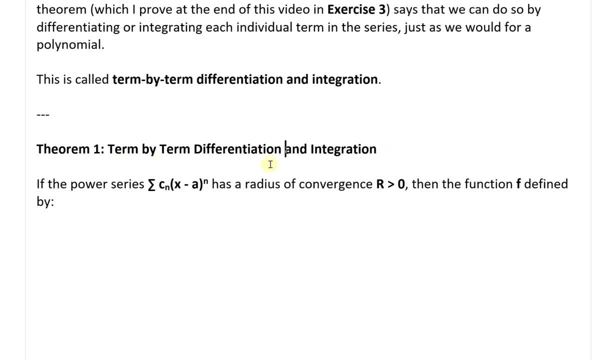 in general. uh, so theorem, one term by term: differentiation and integration. so if the power series, uh, the summation c n times x minus a to the power of n, has a radius of convergence, uh r is greater than zero, then the function f, defined by yeah, defined by f of x, which equals 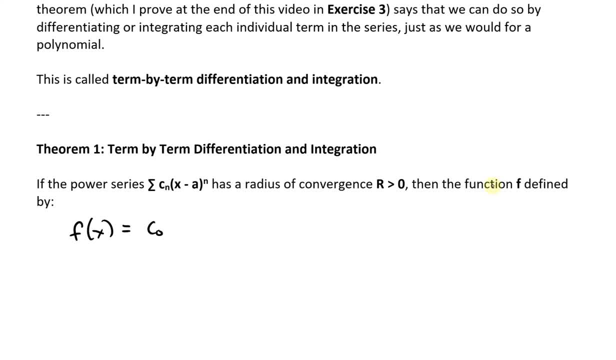 to c zero. so when x minus a to the power of zero is just one. so just have c zero there, plus c1 x minus a, plus c2 x minus a power of two, and so on. so plus dot dot dot equals two. and then write this: 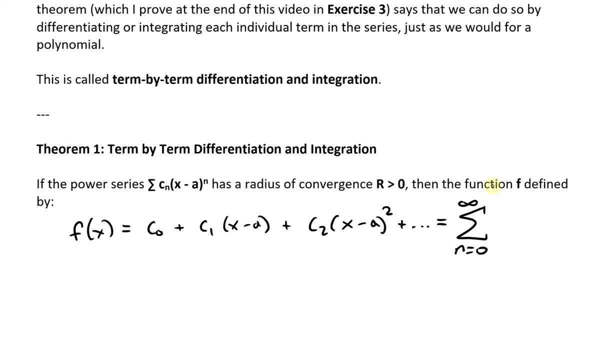 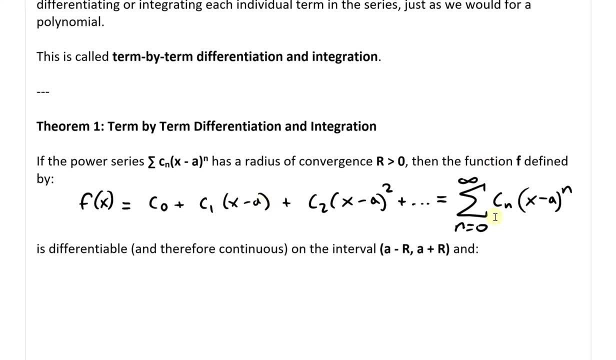 in series form or summation form, uh, summation from n equals zero up to infinity of c, n, x minus a, n, yes, uh. thus this function is differentiable and therefore continuous, as in my earlier video suggested- and i'll put a link to it soon- on the interval from a minus a to the power of n. 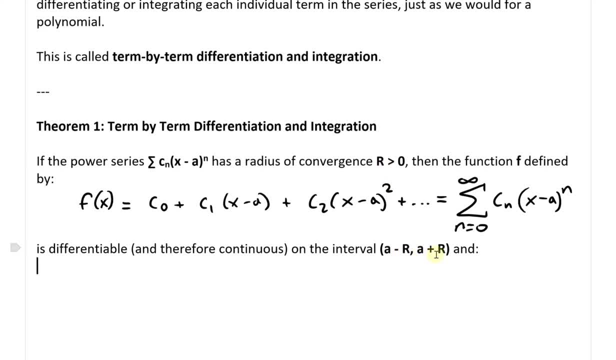 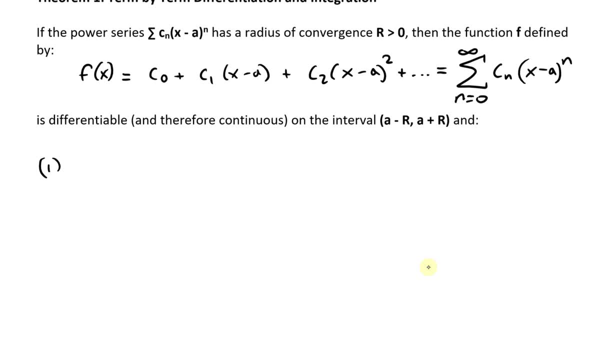 and then i'll put a link to it soon- on the interval from a minus a to the power of n. so the derivative of this function, f, prime of x, is going to equal to the derivative of every single term. so for the first one, c zero is going to go to zero. so then c1, the derivative of c1 times x. 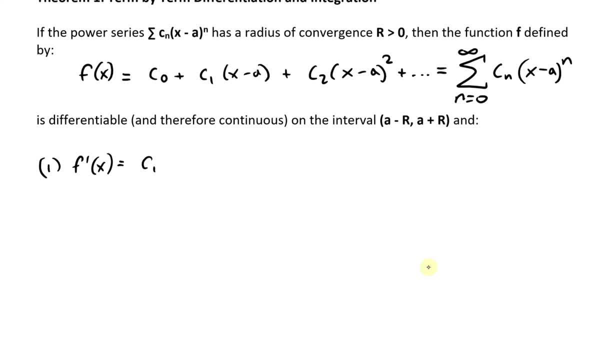 minus a, that's just c1, and derivative of c2 x minus a. squared, that's going to be plus two, c2 x minus a. and likewise the next one's going to be three, c3 x minus two, two, and this one's going to keep going on plus, dot, dot, dot. this equals to the summation up to infinity from n. 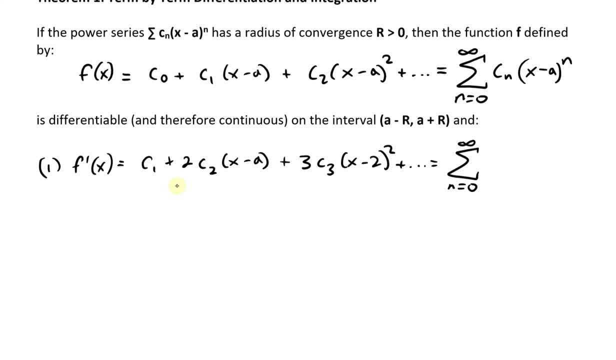 equals to zero and, yeah, what this equals to is just the n goes down just using basic derivatives. so it's going to be, uh, right, here, n. and then this c? n is going to be the derivative of c? n, x minus a, to be, yeah, actually it's still going to be cn. but here we're, instead of starting from: n equals one. 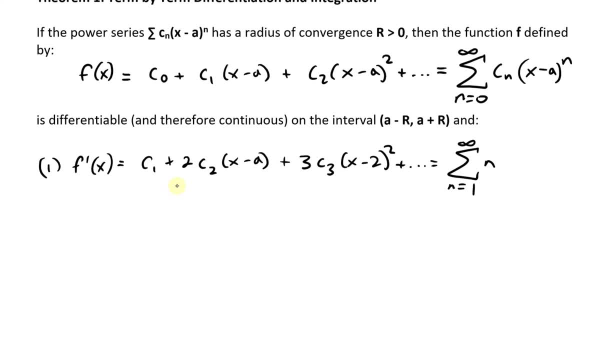 we start from n equals zero. n equals uh one. i mean, instead of starting from n equals zero, we start from n equals one, because notice, here the derivative of c, zero goes to zero. so then we have a c1 over there. but even if we put n equals to zero, the times this n is going to be zero and 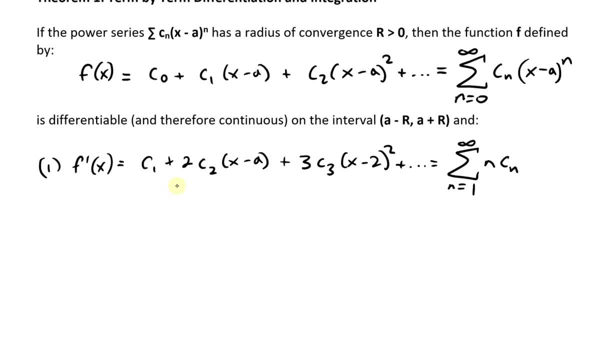 it's going to be gone. so now, this is going to be c, n, so c1 to make it line up, and then we'll have x minus a to the power of the power of. initially, this one's going to be x to zero, this is x, and 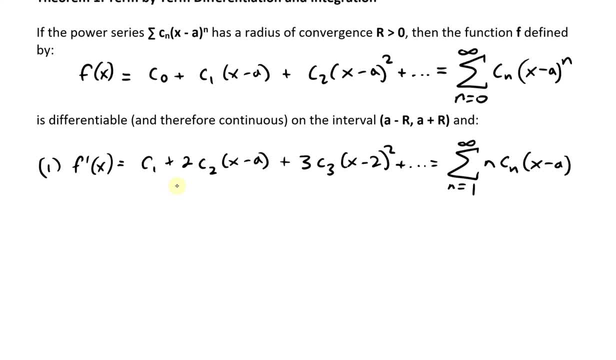 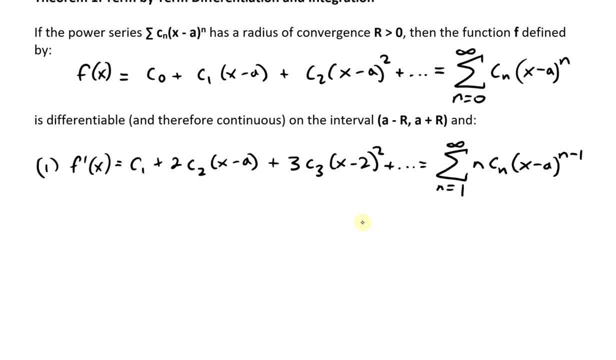 x minus a to the power of one. this is x minus two to the power of two, so this can be one less than it. so it's going to be n minus one. yeah, so that is the uh derivative, and now, likewise the integral, where this, i, i, this is going to equal to the integral of f of x. so f of x, dx, now, uh, this is. 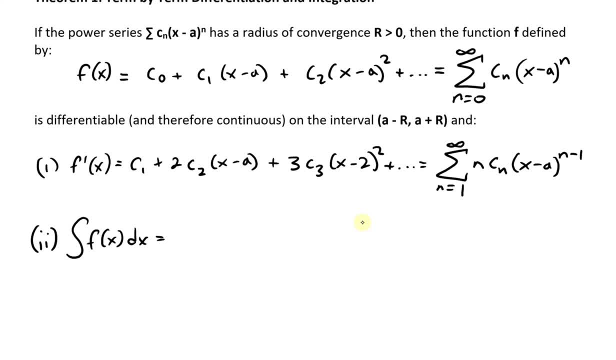 going to equal to well, the integral of c zero there, this one here. um, what i'm going to do? i'm going to write this as: uh, this is going to be c zero, and then i'm going to write this as c zero. i'm going to be written as c zero. actually, no capital, c for a constant, because you also add a. 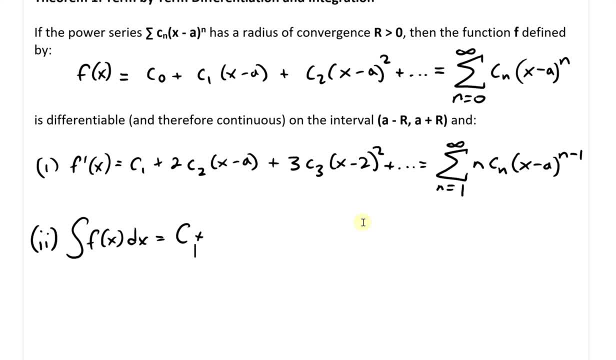 constant, and i'll explain this one in a bit. i'm just going to try to make it the same term. so we're going to have c zero, x minus a and i'll write: so this one, this particular one, i'll write the difference or how we get this form. uh, soon, but but then basically let's just skip that part. 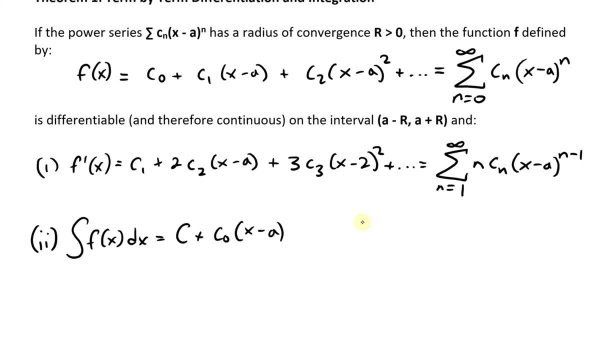 right there, so right now. then the next one over here: c1 x minus a. the integral of that is going to be: well, we just raise this a power, then divide this by two. so this is going to be plus c1 x minus a power of two over two, because, remember, you just take the derivative. now this two take. 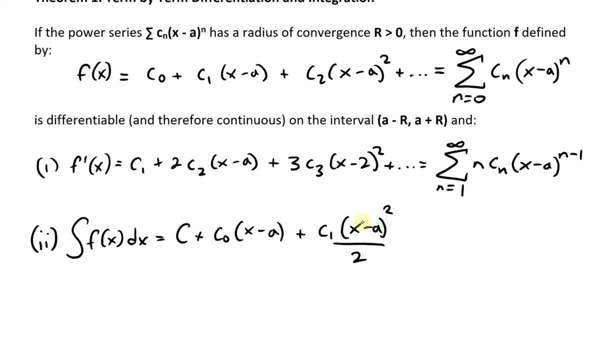 derivative two goes down, this cancels and minus one, so we'll just have this exact term, and then likewise over here, plus c2, and now we have an x minus a and the integral is going to be three. divide this by three. so add, add a power there and divide. and now this one keeps. 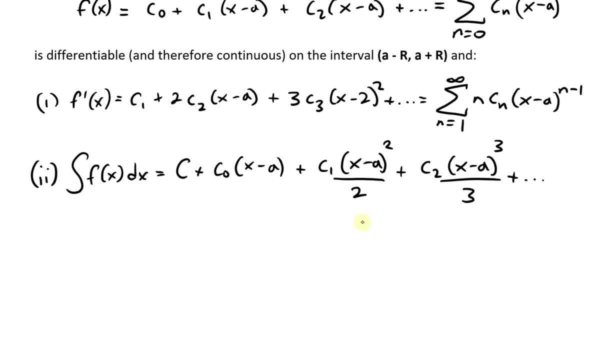 going on plus dot, dot, dot, and now this equals two, uh, and this equals two. basically, you know, what we have is we'll just add a constant outside of this uh. first, because we also have a constant integral. so plus c, uh, and then divide them, plus, i mean c, plus. now this is going to be the integral actually. 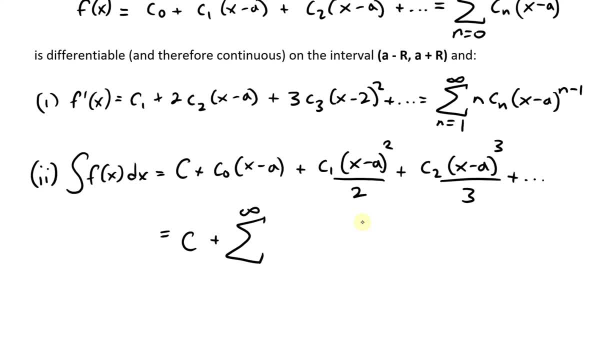 we already have the integral. now this can be a summation right here. summation: n equals to zero. up to now we just write a summation of this one. so we have c zero. this starts from n equals zero, c0 is cn, and now what we have is a x minus a like that, or better yet, let's write it up here: so x minus. 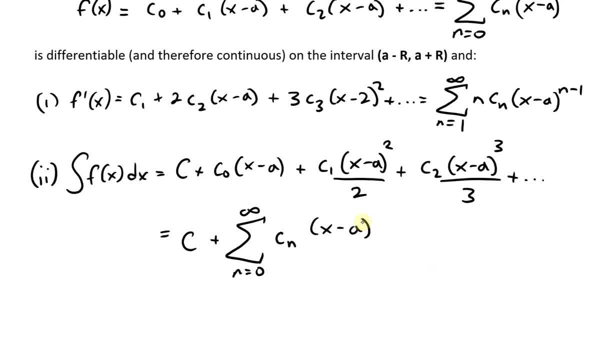 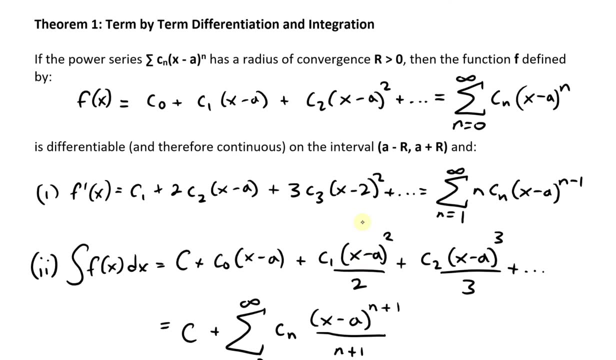 a to the power of the same power of one, so it's going to be a n plus one. because you have zero there, then one n is one, we have to have two and likewise divide this by n plus one. so when n is zero, uh divided by one, so we get that term there. yeah, note here: this is just the uh integral of. 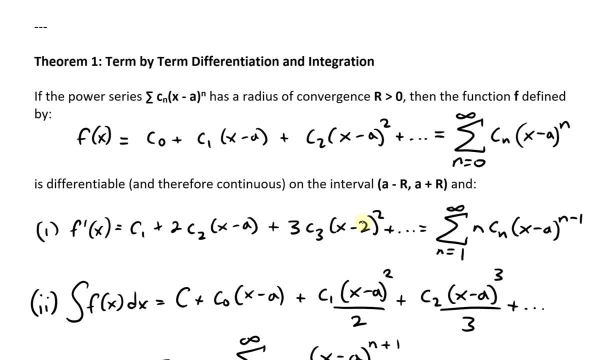 this right here cn. so we have uh n plus one, so we get that term there. yeah, note here: this is just the uh integral of this right here, cn. so we have uh, n, uh plus one and then divided by n plus one, and then we have a constant uh afterwards, because 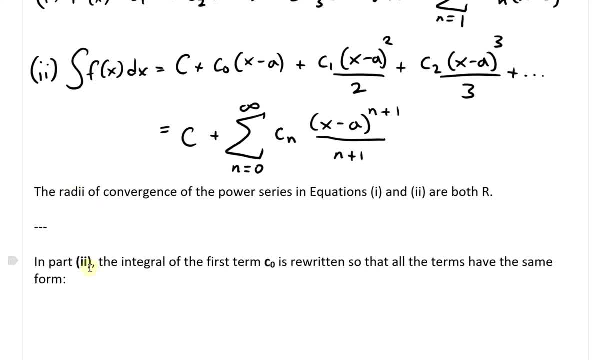 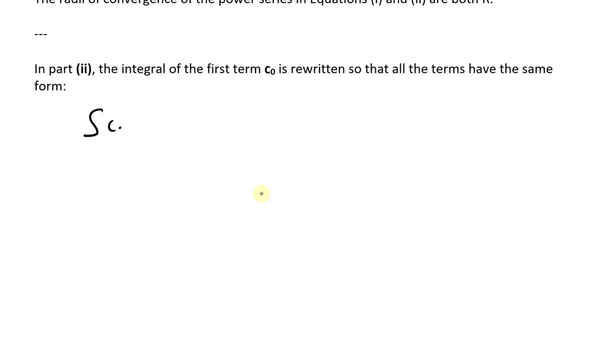 we've taken integral, yeah. so here, uh, in part two, or part i, i, the integral of the first term, c0, is rewritten so that all terms of the same form, that's, to get this c0 times x minus a, somewhere a is a constant as well. and to do this, uh, what i did was well, if we take the integral of c0, 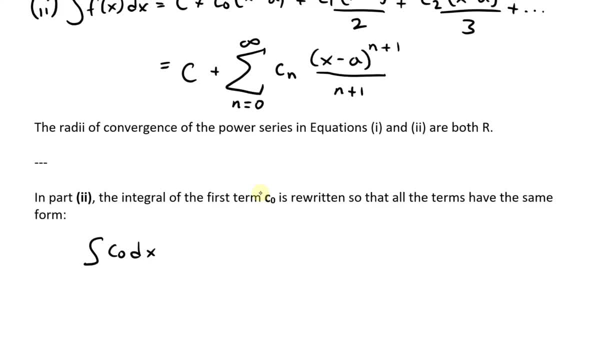 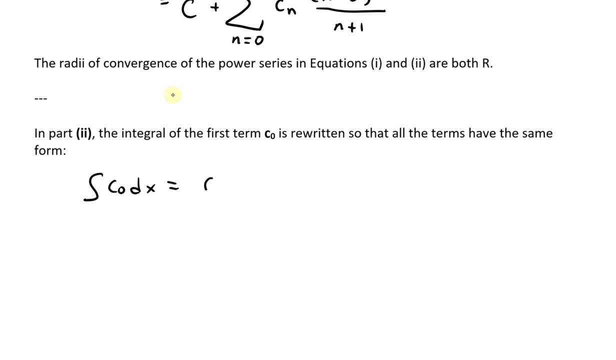 uh d, uh, dx. yeah, so c0 dx- that's this one right here. so we take integral of this one separately- is going to be equal to. that's just a constant. so if c0 times x, then we have a plus constant of integration. i'll just write this as one like that. yeah, so we have it like this form. but what we want. 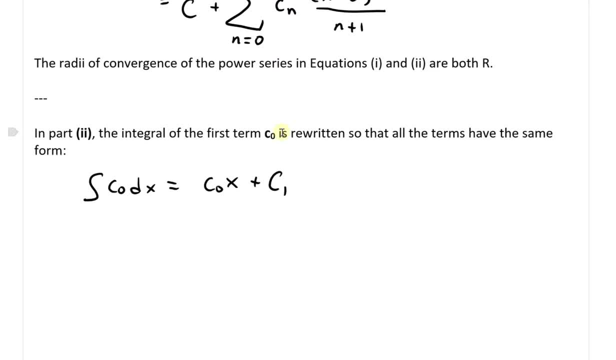 is a c. well, we want this x minus a, like that. so what we could do is: uh, let c equals to c1 plus this is going to be now a c0. if we do this, then we can move this over to the other side, so that 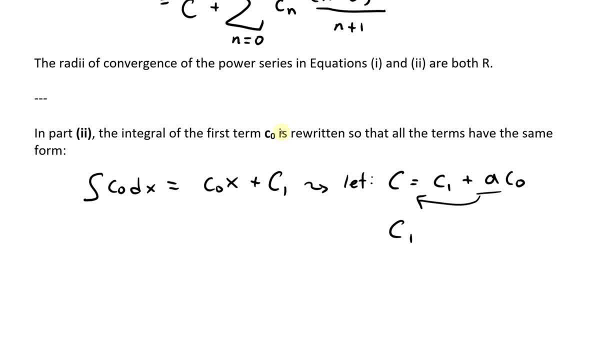 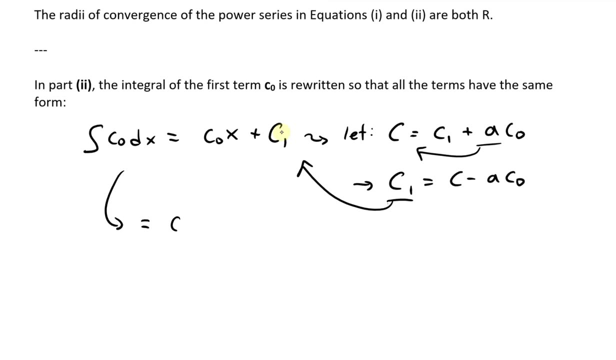 c1 equals 2, or large capital c1 equals 2 c minus a c0, and then we could throw that inside this one. so what we end up having is this equals 2 c0 x. this is going to be. now let's move this. 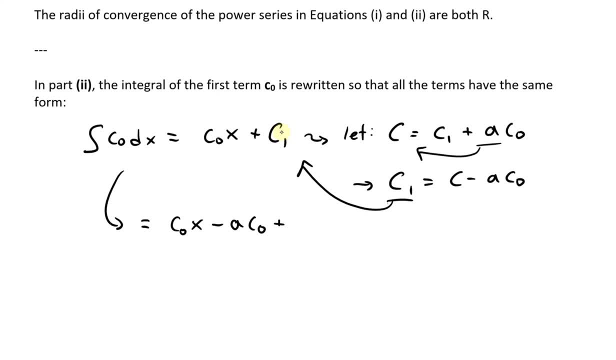 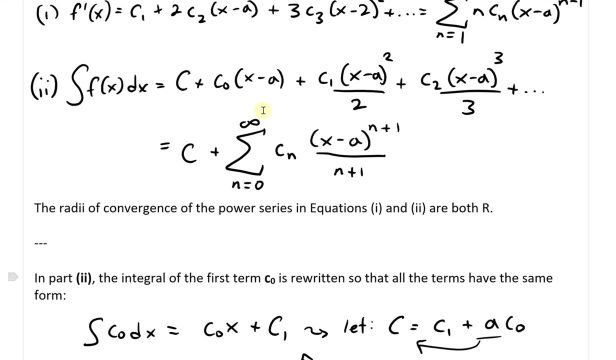 right here, minus a, c0 plus c, and then we can just factor out the c0 there and also move the in front. so c plus c0. uh times it by x minus a, like that. and also what happens is when we take the integral of all of these terms, we're always going to get a constant and we just we can combine. 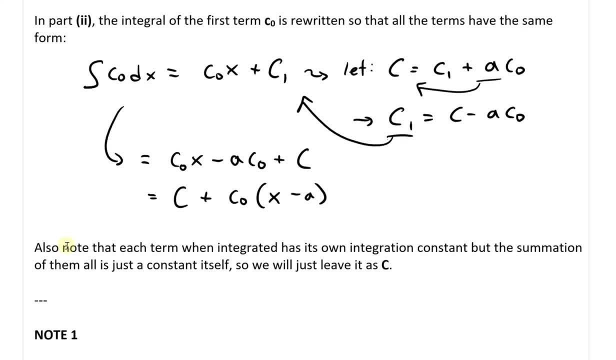 all the constants into this uh, just to see one right there. and i also note that, uh, each term, when integrated, has its own uh integration constant. but the summation of them all is just the constant itself. so we'll just leave it as c and just leave it like that. so c plus this uh. 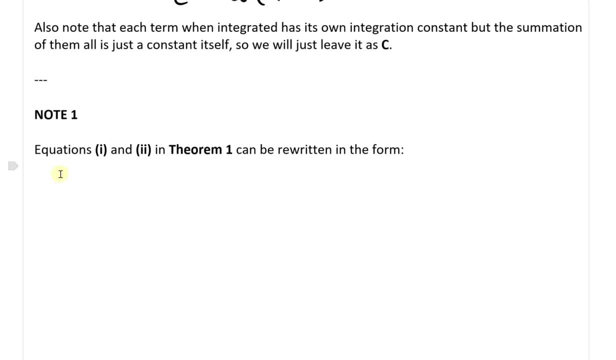 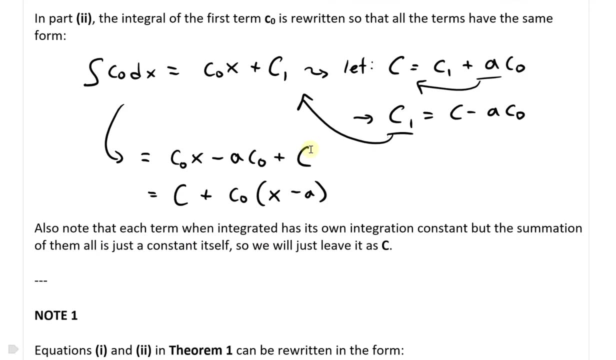 series right there and uh. now i'll make a note one, uh, the note number one for my calculus book. this one states: uh, equations one and two in theorem one can be rewritten in the form. so what? the? what this is saying is that the derivative is equal to this one right here. but that's just again. 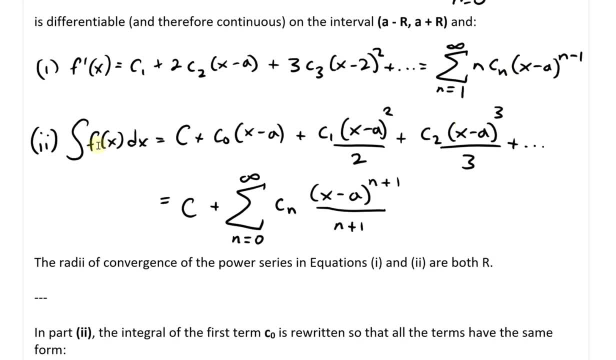 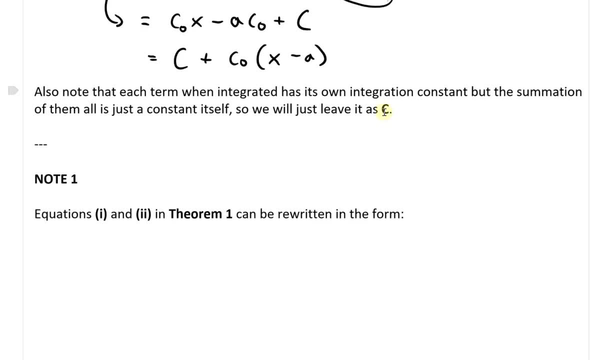 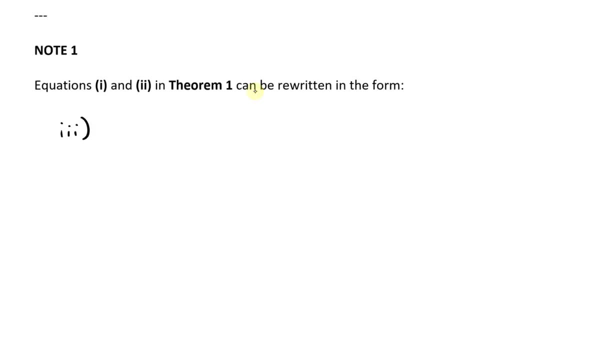 that's just taking the derivative directly from this series and the integral. you can take the integral directly from this uh, this uh series cn x minus a to power n, so we could rewrite this as yeah and i'll write this as uh, for i'll call this i, i, i, uh, so we'll call this one like that, and this is uh. equal to this is. 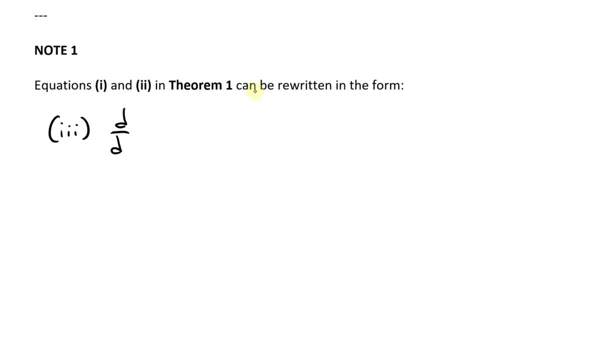 the derivative part. so we could write this as: the derivative d over dx of the square bracket of the series n equals to zero of c, n, x minus a of this power series, this equals two. put a close bracket, this just equals two. well, this the the summation from. 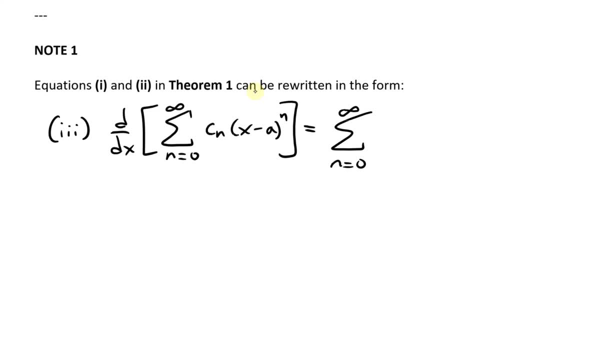 uh, up from n equals zero to infinity of. just. well, then now we could take the derivative of the inside term, or the or the inside terms. like this this is going to be. i have to put a bracket like this: so this just equals to the derivative of the whole series, equals to the summation of the. 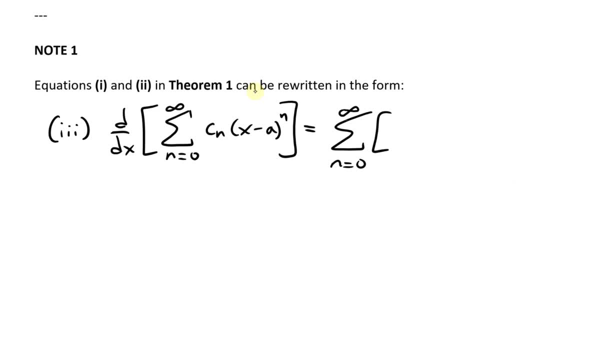 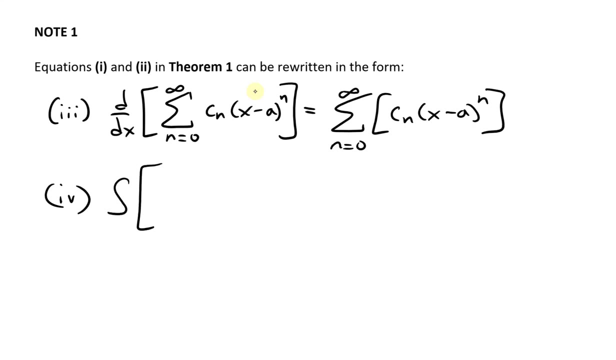 individual derivatives. so, uh, right here, this is going to be c n x minus a n, like that, and likewise we'll write this as i v for four and the integral of this all. so the integral of this, uh, summation of the series n equals zero up to c n x minus a n. bracket, close bracket uh is exactly as expected. this is just. 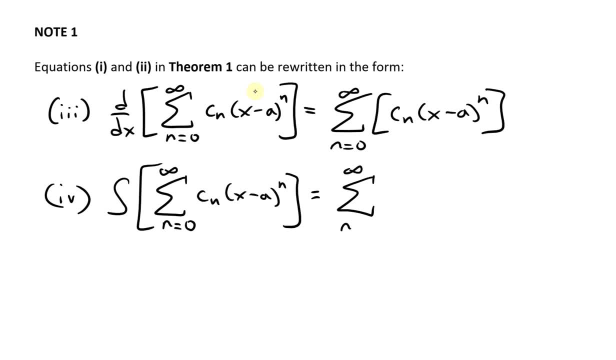 going to be the summation, just exactly like above, but integral instead of derivative. n equals zero. the integral now of: and also- actually i've forgotten this side, we'll just move this over- uh, include the dx here, taken, because we've taken, uh, integral. this is going to be now. 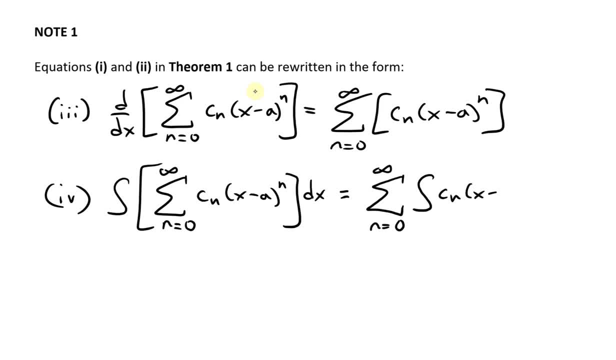 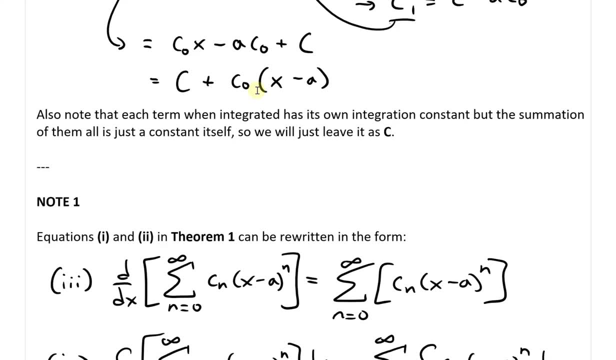 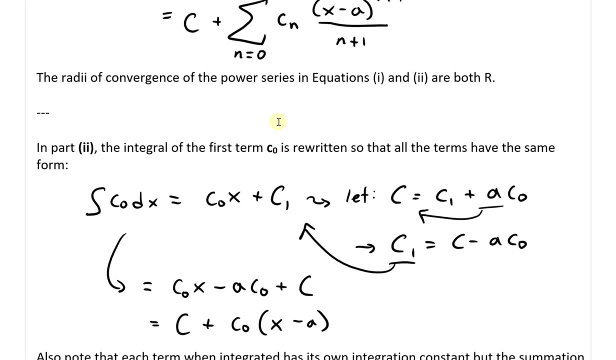 uh, this is going to be integral from c, n, x minus a, n, dx, like that and uh, this term right here. the derivative just so happens to be uh. this right here. uh, x minus a power of n plus one divided by n plus one times c, n and plus is extra constant c and uh. now continuing further: yeah, we know that. 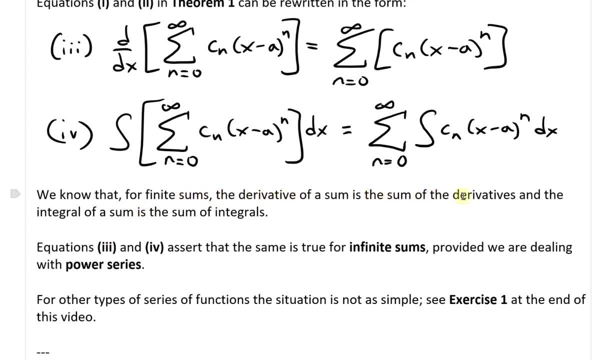 for finite sums. the derivative of a sum is the derivative of the sum of the derivative of the sum is the sum of the derivatives, and the integral of a sum is the sum of integrals. yeah, this is finite sums, uh, but uh, for this, equations, uh, this? three and four assert that the same is true for. 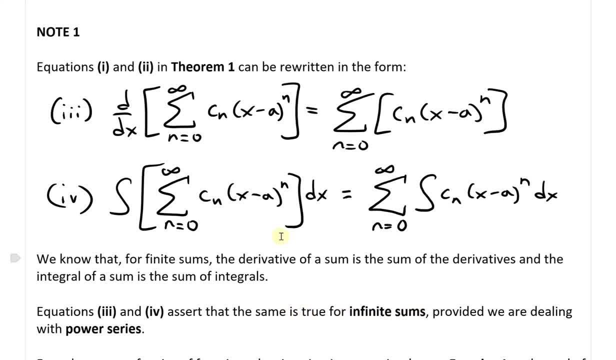 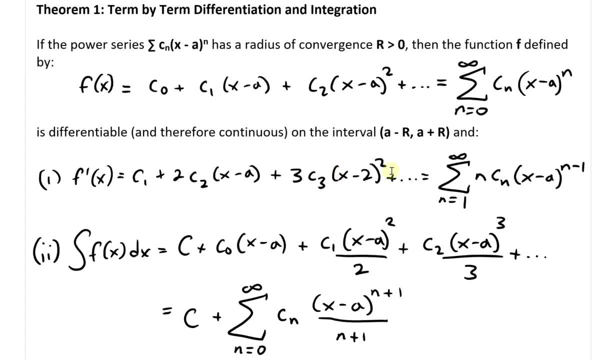 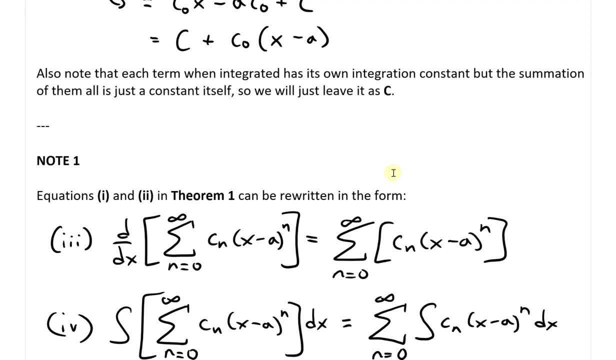 infinite sums, provided we are dealing with power series. so yes, when dealing power series, we could do this: uh, integral or differentiation for infinite sums. so notice, uh, exactly like these right over here. uh, but if this was uh just finite, we already know we could do that, but now we're uh. 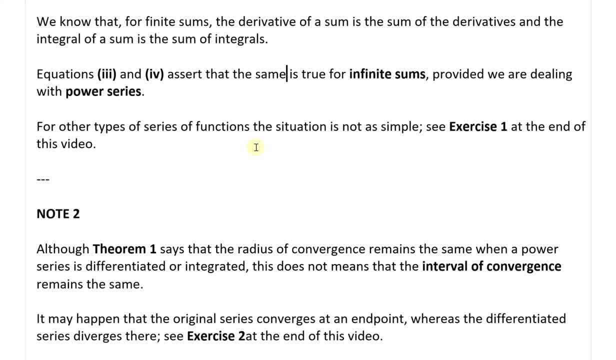 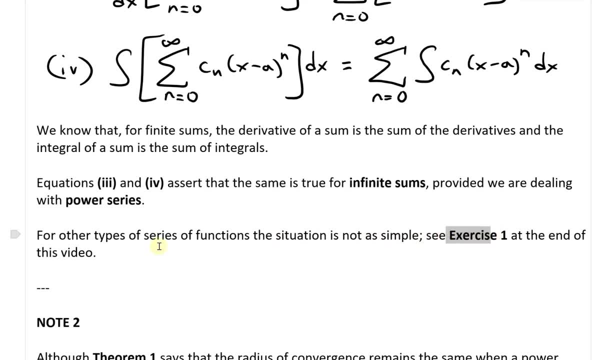 asserting that even for infinite sums- and again i'll prove this at the end of this video, and it's pretty epic- for other types of series of functions the situation is not as simple, and see exercise one at the end of this video. so remember this is dealing with power series for other functions you 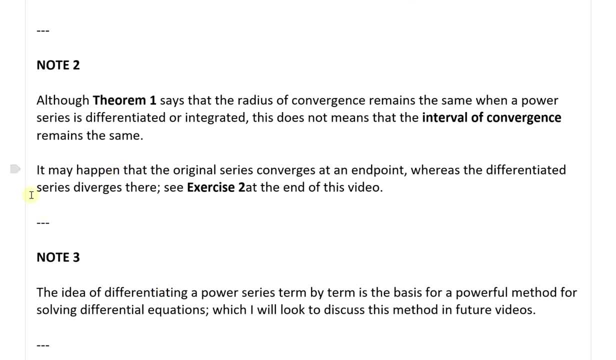 gotta look at those specifically, uh. so now let's look at another note. my calculus book makes note two: although theorem one says that the radius of convergence remains remains the same when a power series is differentiated or integrated, yeah, so, uh, scroll up here. so this is saying that. 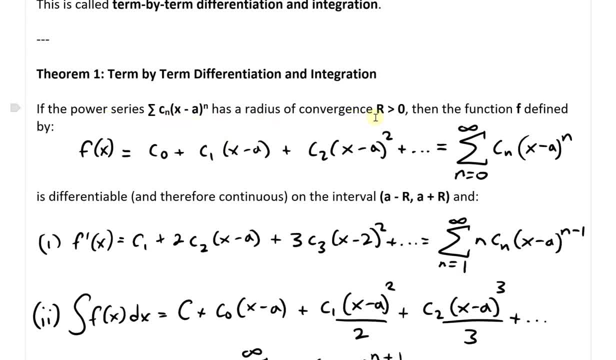 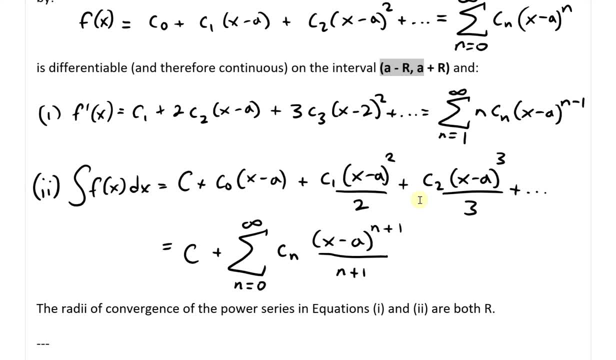 the radius of convergence is the same. so if the power series has a radius of convergence r is greater than zero, then the function is differential and therefore continuous on this interval. and yeah, and we're given right here as bold these ones, uh yeah. so the radius of convergence of the 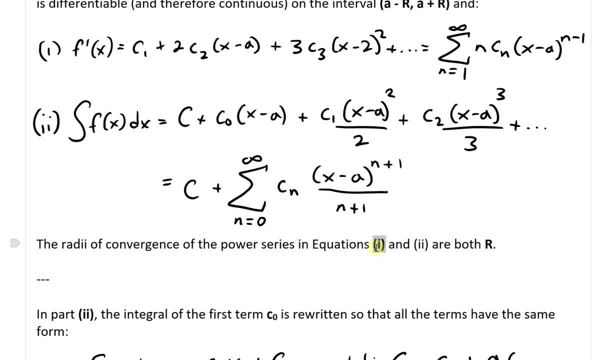 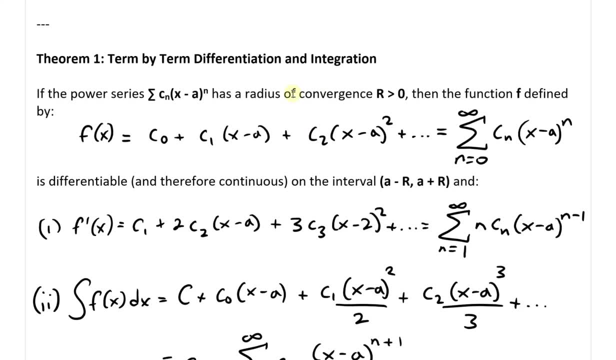 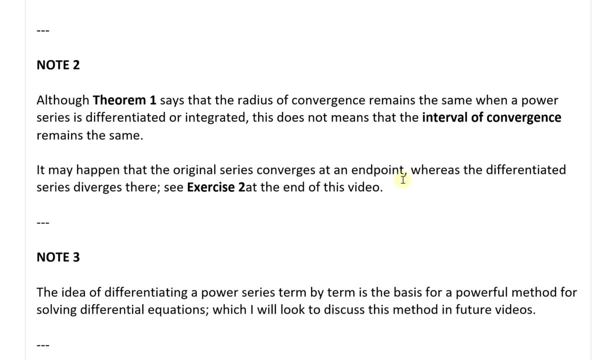 power series in both of these equations- and i forgot if i read this or not, uh, yeah, in both of these equations- are, are, r, so these have the same radius of convergence as this power series, fx. so derivative integral have the same. so the theorem states- and again, i'll prove that at the end: and yeah, so this theorem one says that: 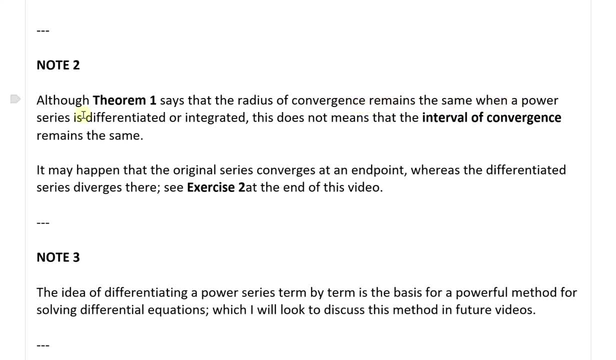 although the radius of convergence remains the same when a power series is differentiated or integrated, this does not mean that the interval of convergence remains the same because, remember, the end points are different. uh, you have to check those. it may happen that the original series converges at an end point, whereas the differentiated series diverges there, see exercise. 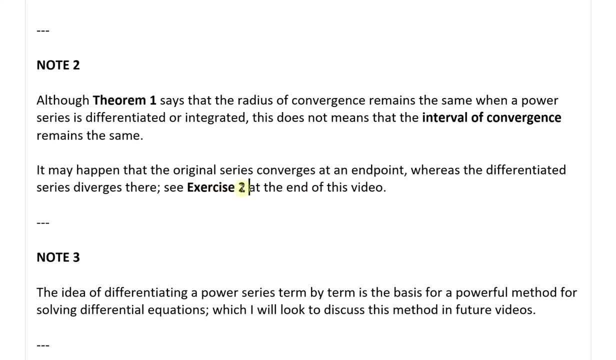 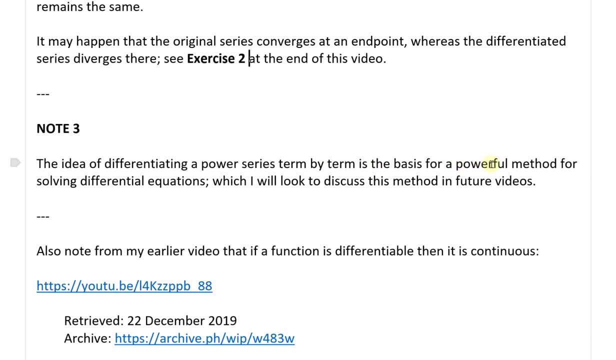 two at the end of this uh video, which i'll go over, that one there and now go over another note in my note three. the idea of differentiating a power series term by term is the basis for a powerful method for solving differential equations which i will look to discuss uh this method in future. 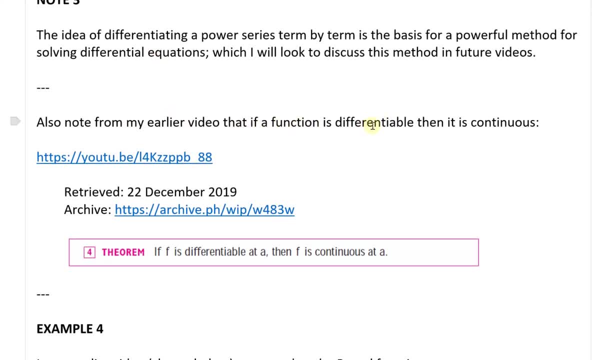 videos. uh, also note from my earlier video that if a function is differentiable, then it is continuous, and this is a just copy and paste from my calculus book, but there's a video on it. if f is differentiable at a, then f is continuous at a, and it's basically because we are when you're taking 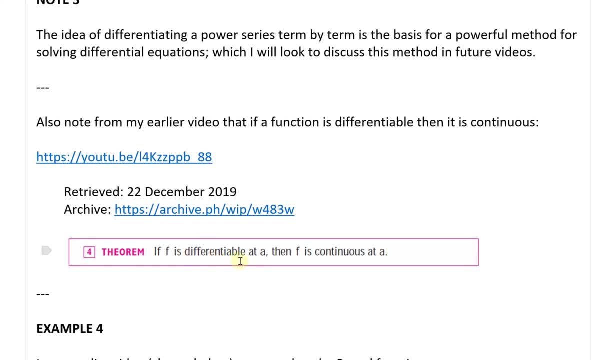 derivative. uh. you're essentially taking the limit as a difference as the slope is approaching. is exactly, uh exact rate of change, or uh, basically, you're dividing by uh infinitely very, very small, or i mean, uh, the rate of change that you're looking at or the slope that you're looking at. 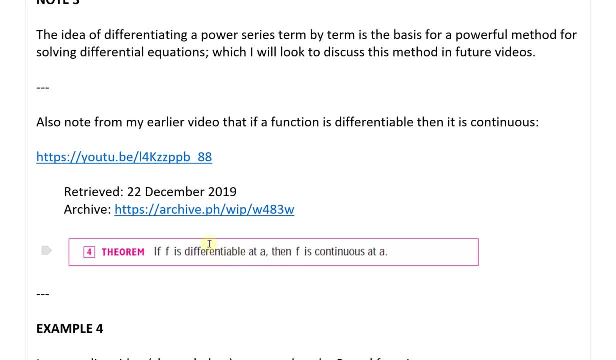 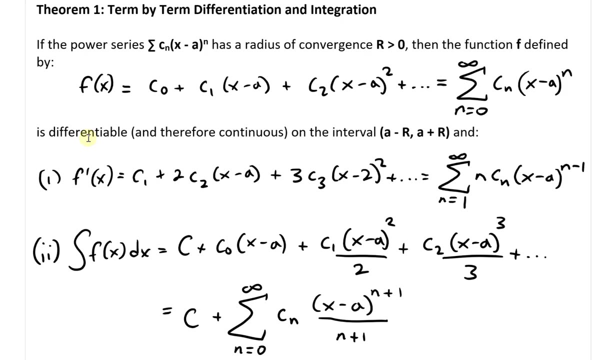 is becoming more and more fine. so that requires, yeah, obviously taking a limit. and we take a limit, it's eventually gonna. yeah, it essentially means that it's continuous at a if the limit exists at a. so it's very, very interesting and that is, yeah, noted here. so scroll up in the theorem. so 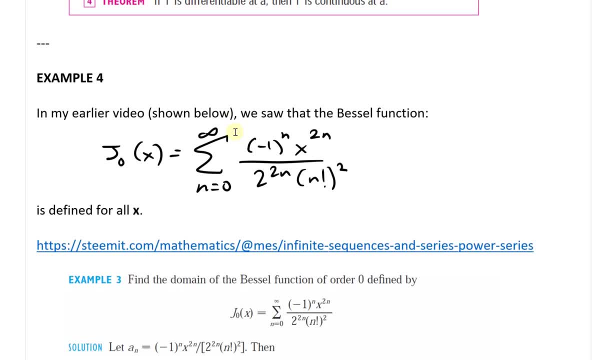 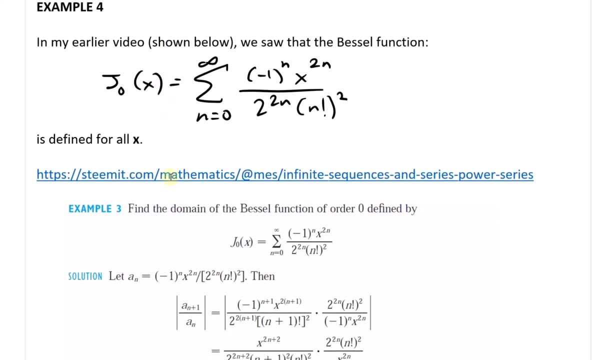 it was differentiable and therefore continuous. as in my earlier video, i'll put a link there. all right, so now let's look at example four, and this one in my earlier video was shown below or linked below: uh, we saw that the yeah, that the uh bessel function. 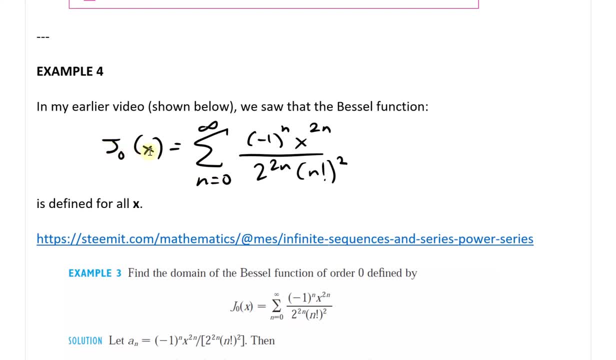 and written here: j zero. j zero of x is equal to the summation- n equals zero, up to infinity- of negative one. the power of n times x to the power of n. again, there, it is right, there, uh, divided by two to the power of two n. and then, uh, this is times it by n factorial. 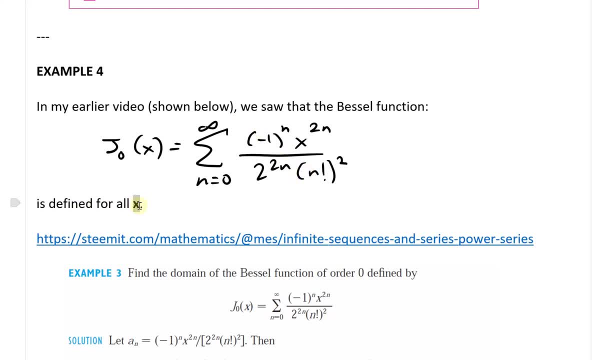 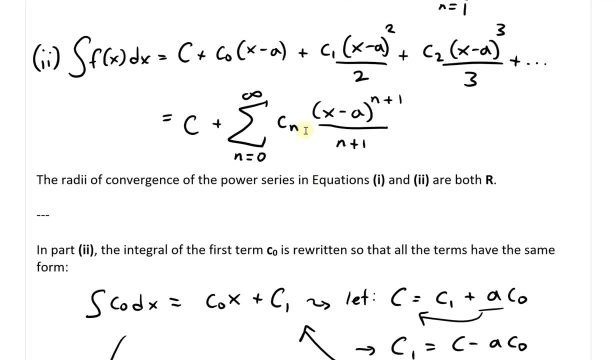 all squared and i showed that this is defined for all x as radius of convergence is, uh, infinity there and it's a power series, uh, number, uh. the note that in this case, right here, this power series that we're defining, these c zeros, these are just coefficients. they could be anything. 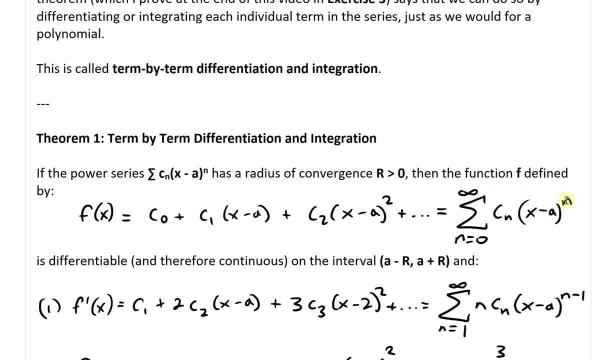 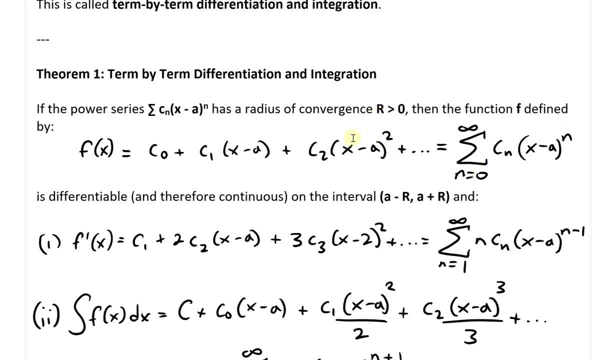 uh, we want them to be. uh, and then this power of n right here. yeah, just a power series. but if it's two and three, and it doesn't matter, because essentially all it means is we're inside these each terms, we're just gonna have a different power there. 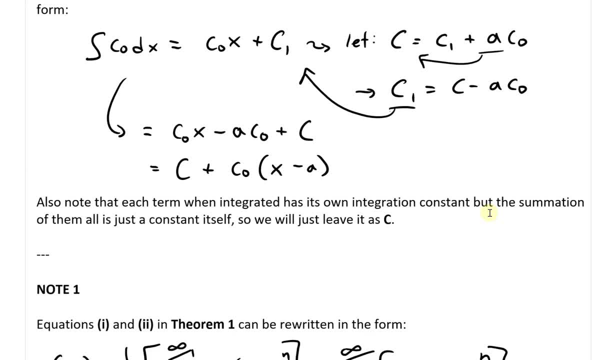 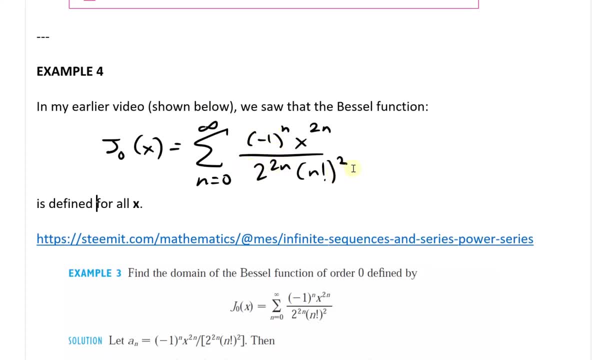 eventually, even this gets every single power when it's just n like that, and this one will just skip some if it's uh 2n and so on, yeah, so then this vessel function has a bunch of these uh n terms right here, but but uh, for each n value you're just going to get a coefficient times it. 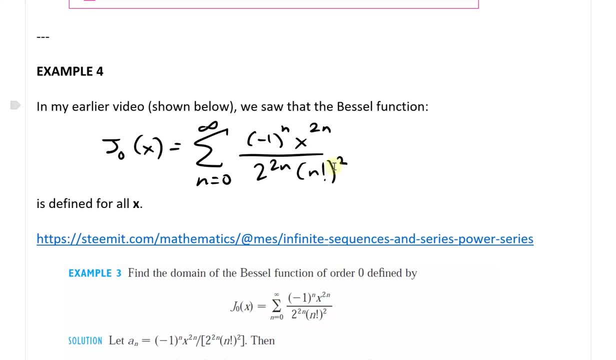 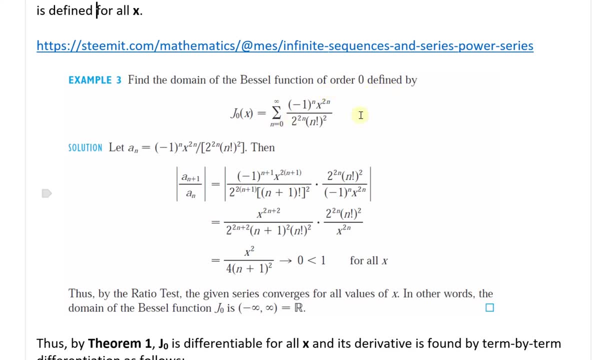 by x the power of a number. so, which is exactly what our power series is. so this is defined for it, and here's just a link to it, where i should find a domain of the best function of order zero, defined uh by uh, this function right there, and then i i let this one here and i use the ratio. 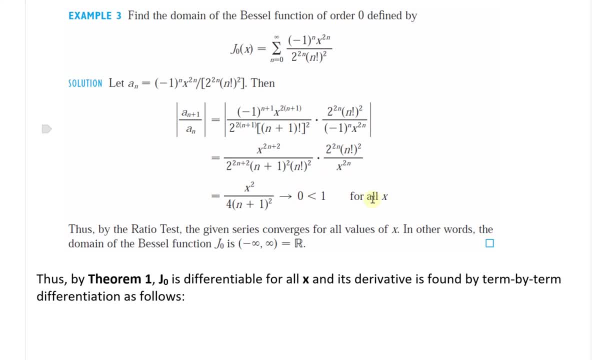 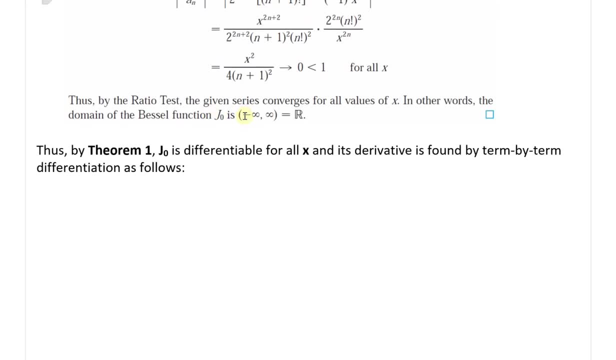 test and uh solve that it's equal zero, less than one for all x, uh, that's by ratio test. convergence is uh, so on, and it's uh. radius of convergence is infinity, and it converges from negative infinity to infinity. so thus, by theorem one j zero is differentiable for all x and its derivative is: 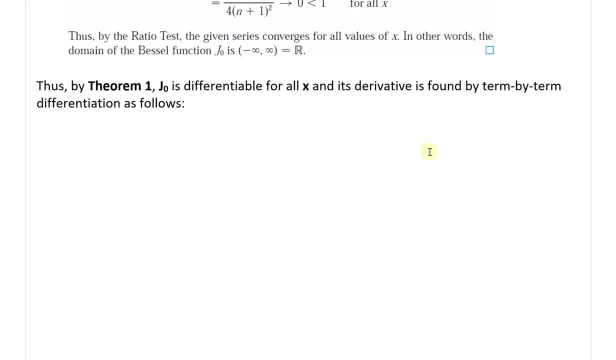 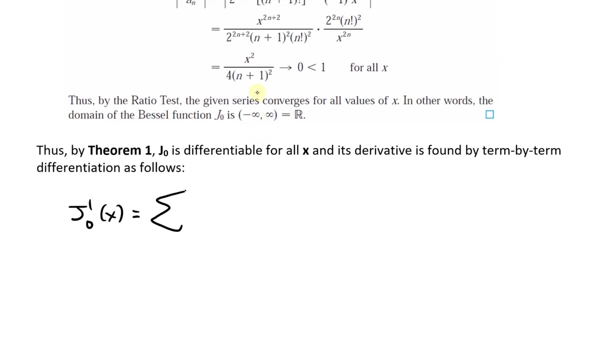 found by term by term differentiation as follows: so we can just write this down as the derivative of the best function: uh, j prime j zero. prime of x is equal to. so this is equal to- and i'll just take a summation right here and then times the derivative. so we can write this as summation: 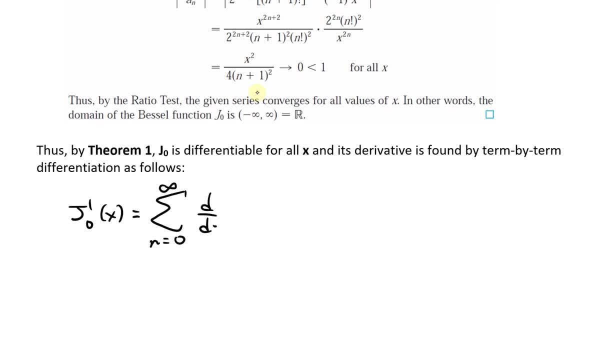 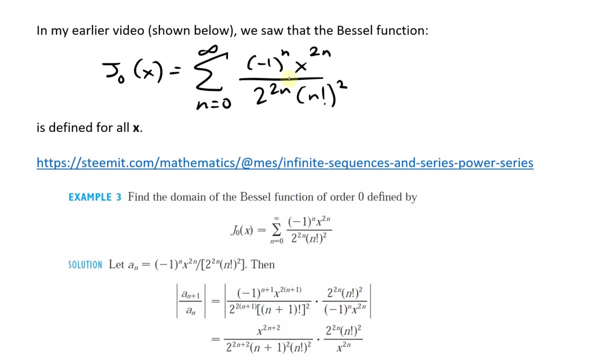 up to infinity of n equals a zero d over dx, and then right over here. so this is, uh, negative one n, x to the two n. so, uh, we just write this as negative one n, x to the two n. and what else do we have? as is two and two to the power of two, and then n, factorial squared two to the power of two. 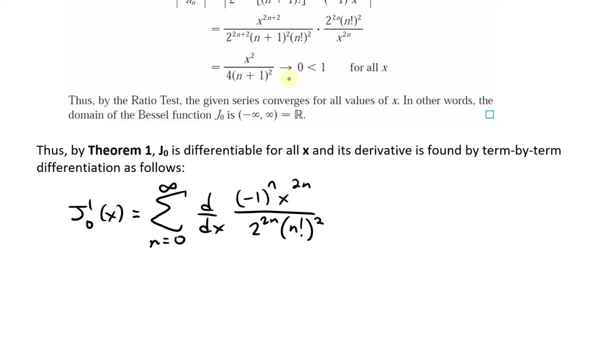 n, and then n- factorial square, and now the derivative of this one here. well, these are all. just, these are all. we're taking order in terms of X. so then, the only one that matters is this: X right here, X to the power of 2, n, so we can keep all these inside. this is. 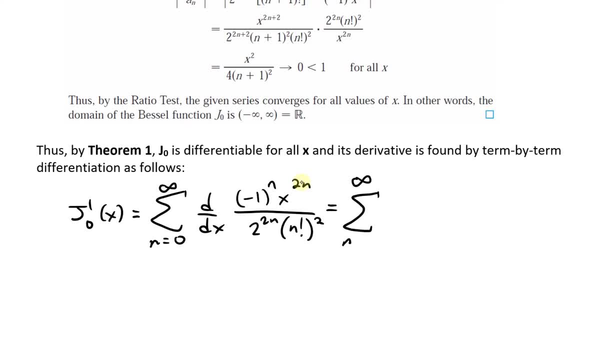 going to equal to the summation up to infinity from n equals 0, and then bring this down here, bring this 2 and down we get negative 1 and like this: let's put this to the power of 2: n times it by expand this out: times by n factorial n. 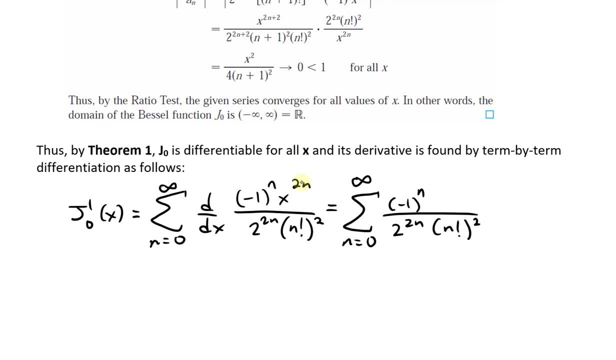 in fact I go n factorial and squared and this is 2 n. this guy is gonna go down, so we'll have a times 2 n, times it by X, 2, n minus 1, like that. this basic differentiation rules. and now this is n: 0. but then when you plug inside here: 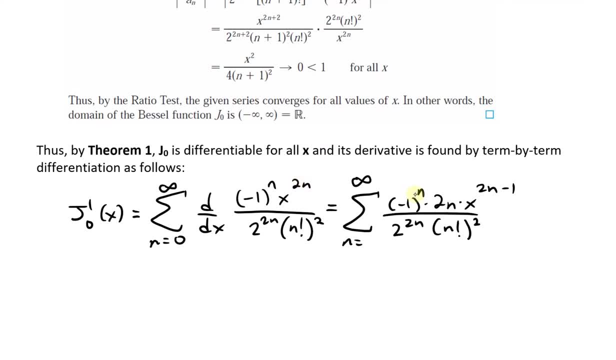 there's a twos times 0, that the two times n. you just put a 1 here for everything and then we're going to take this and we're going to take this and being specific, but you could put 0 to just have a 0 term. so, yes, this is it all. 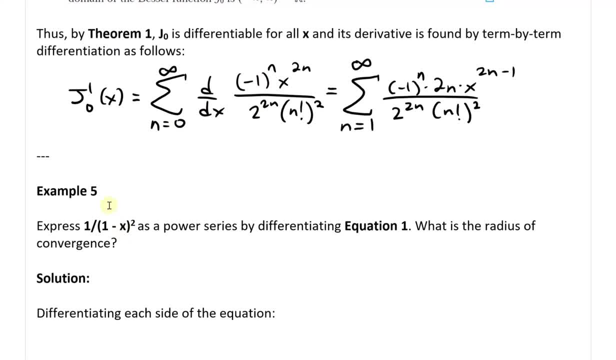 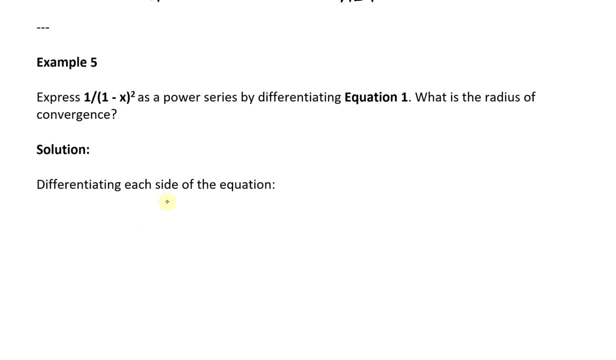 right. so now, going further, let's look at example 5. this one states: express 1 divided by 1 minus X, all squared as a power series. by differentiating equation 1, what is the radius of convergence? so, solution of differentiating each side of the equation, and remember, equation 1 was, if we remember it, just 1 minus X, 1 we. 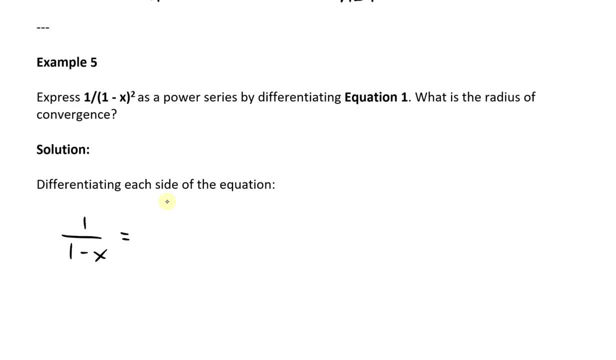 are 1 divided by 1 minus X, and this was going to equal to 1 plus X, plus, as a power series, X squared plus X cubed, plus dot dot, dot, and then this equals to the summation up to infinity of N, equals 0 of X, N and 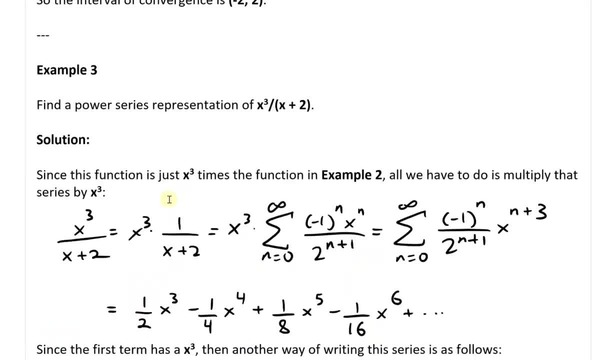 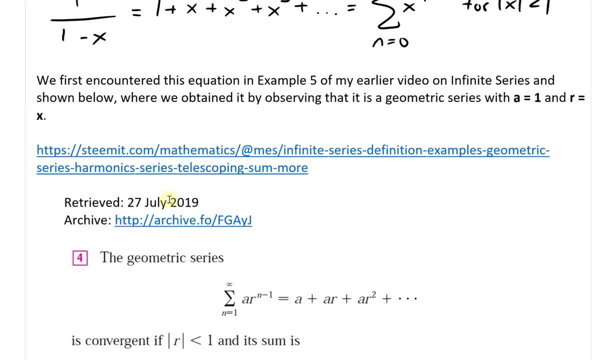 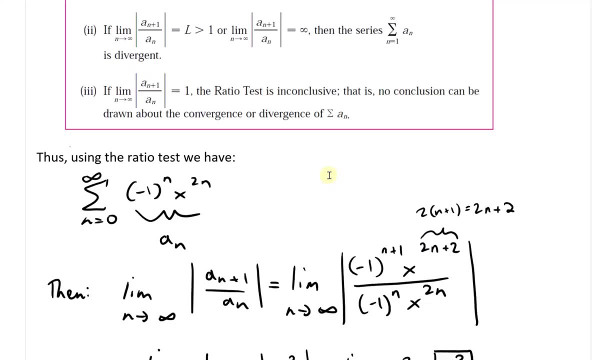 to double-check. let's just scroll up, because I don't see what we wrote. there was the equation 1 and that should be it, so scroll up higher. so yeah, there is our equation 1. this is it. so X n 4agh. so value of x less than 1, like that. just scroll down. yeah, let's just keep going down. yeah, so that is. 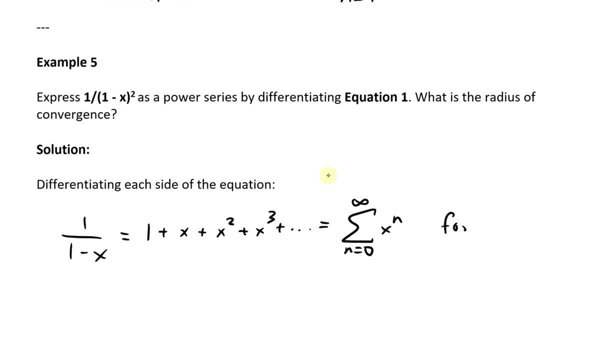 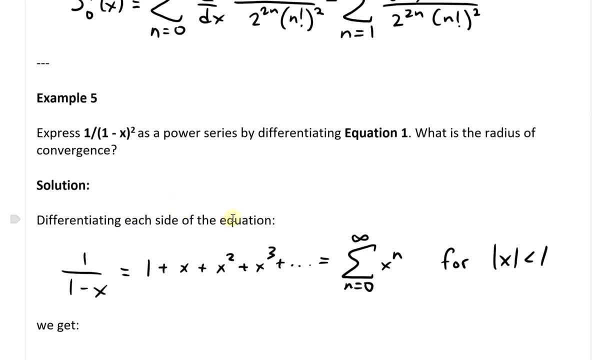 for absolute value of x is less than 1, so let's write for the radius of convergence less than 1, like that. yeah, so now differentiating, uh, each side of the of this equation is again that we were asked to differentiate the equation 1 to get this term. so we can notice, we can get that. 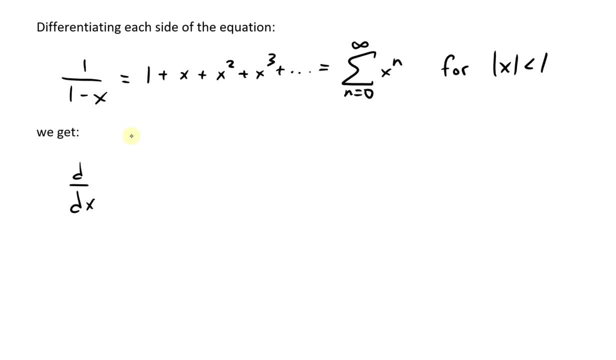 if you take the derivative d over uh, dx of 1 over 1 minus x, like here, so derivative of this is going to be equal to well, you could write: rewrite this as d over dx. uh, write this as a notation. i'm used to 1 minus x, to the power of negative 1, so if it's like this, we just bring down the negative 1. 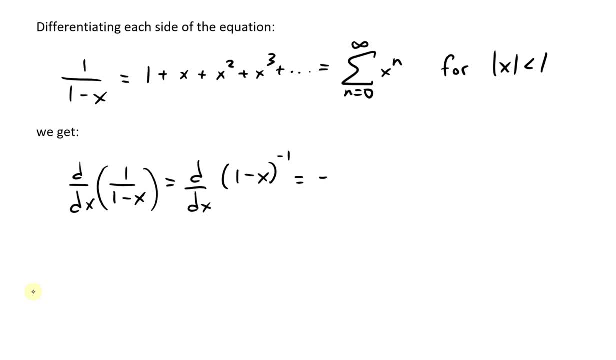 yeah, so we just bring down the negative 1, and then this is going to be a 1 minus x, and then this is going to subtract the power negative 2. you, but also using chain rule. now we also apply chain rule. so this is the derivative. uh, we've. 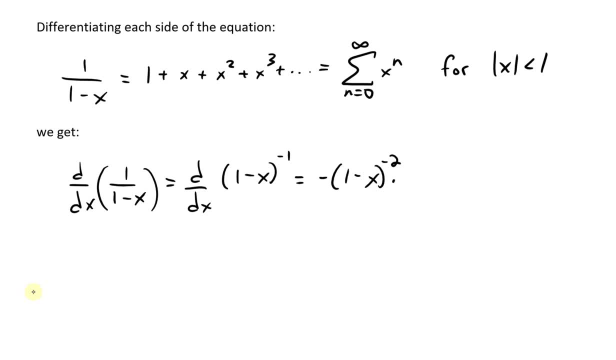 taken derivative of this inside function, which is negative x. yeah, the derivative of negative x is going to be negative 1, like that. so, in other words, this negatives cancel. so what we're left with is: uh, yeah, what we're left with is just 1 minus x to the power of negative 2, or just flip this. 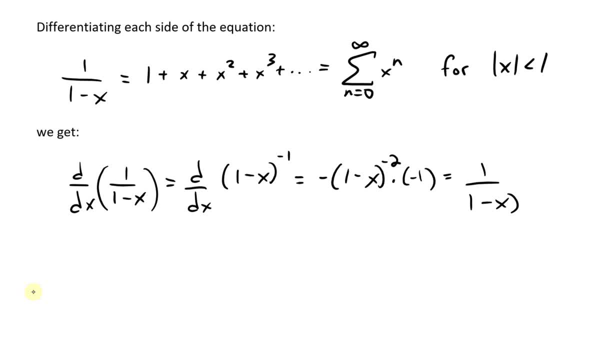 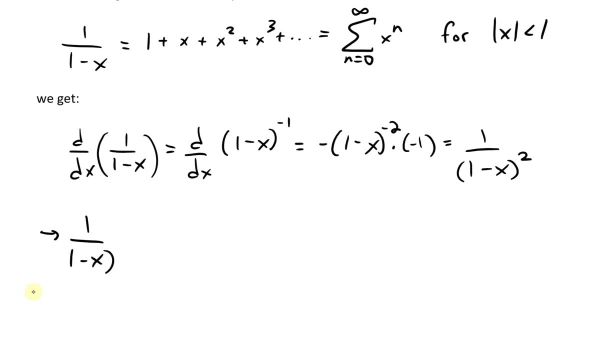 upside down, this just equals to 1 minus x squared. so that's the left side. so this equals to 1 over 1 minus x squared. and now this, uh, each term we take, to take the derivative derivative of 1 is equal to 0. derivative of x is equal to 1, derivative of x squared is going to be equal to 2x, and then it's. 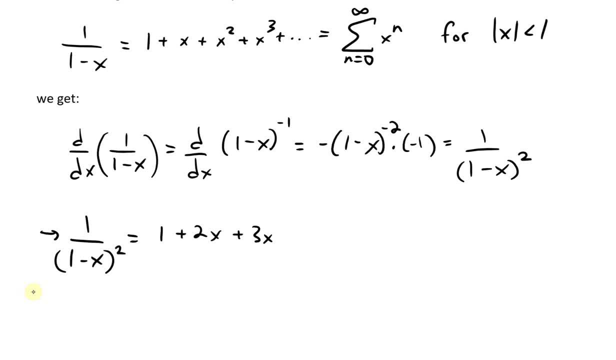 like a derivative of x cubed, it's going to be 3 x squared, and so on. we can keep going on and on. and now this just equals to the summation, uh, up to infinity- of n equals 2. unless it's right, n equals 1. because we know what happens at derivative of x: n: n goes down. so we're going to. 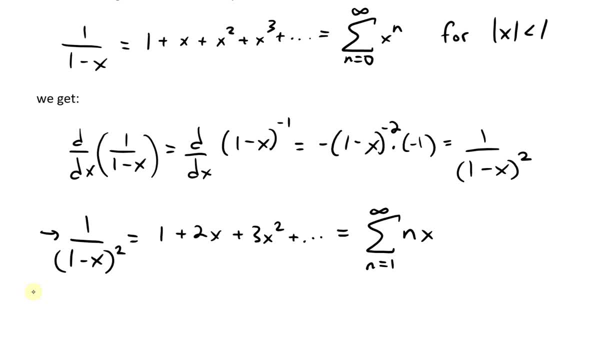 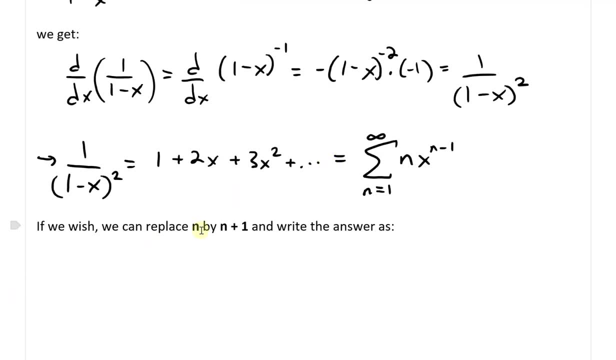 n like that, because if it's 0 we just just have a 0 term. so n x and then n minus 1, like that. and now simplifying: uh, if we wish, we can replace n by n plus 1. so this, right here we have this n minus. 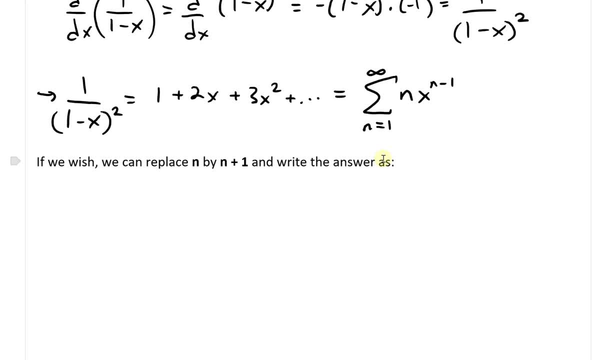 1 like that. what we could do is we could rewrite this whole thing. as this is going to be the left side, it's going to be 1 minus x. 1 divided by 1 minus x squared equals 2, and in this series, right here, we could take the summation. 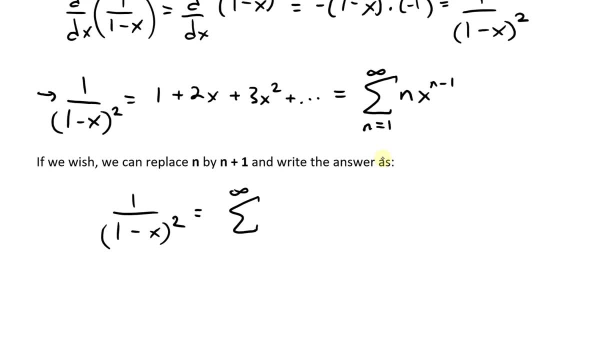 it's always up to infinity. and then, yeah, here, if we're replacing uh n with uh, yeah, we're replacing n with n plus 1. so in other words, what we get is an n, so right here, n plus 1. if it equals to this, 1, right there. so then these cancel. what we have is n equals 0, so we start over there. now, this n. 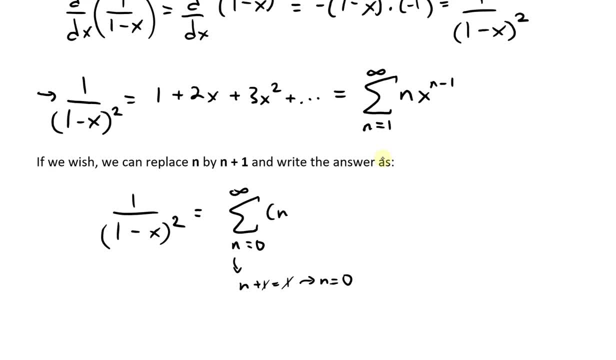 is going to be n plus 1, like that. and then this x is going to be x, n plus 1 minus 1. so we're going to. so it's going to be n, like that. so just all it does is get this negative 1 out of there, just. 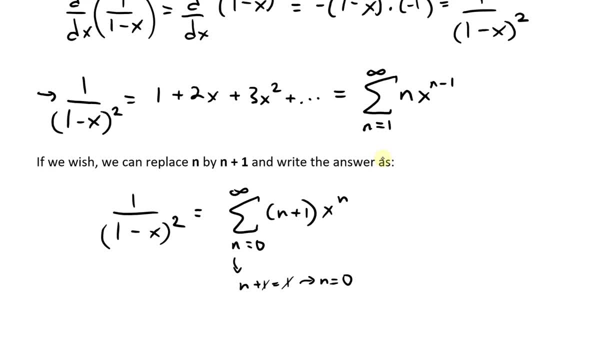 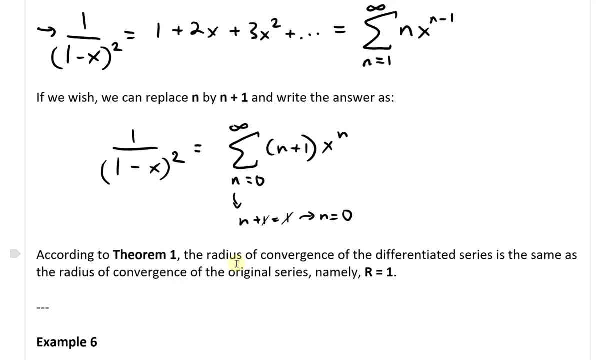 leave it in this n plus 1 term, and then we have a nice little x to power n. yeah, and according to theorem 1, the radius of convergence of this differentiated series is the same as the radius of convergence of the original series, namely r equals to 1, or this absolute value of x is less. 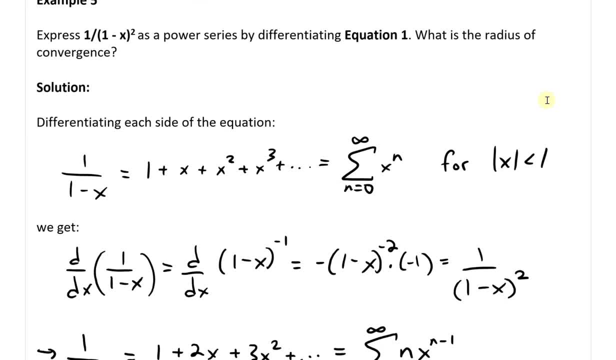 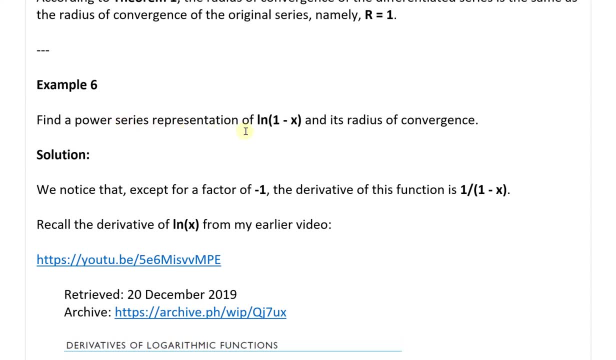 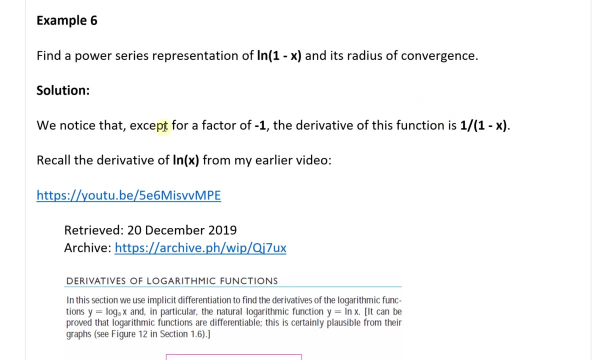 than 1, which is the r value right there. so yes, continuing further. so now let's look at example 6, and this one states: find a power series representation of ln of 1 minus x and its radius of convergence. so let's look at the solution now. we notice that, except for a factor of negative 1, 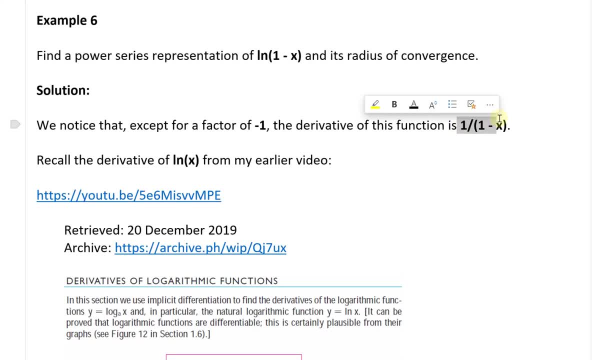 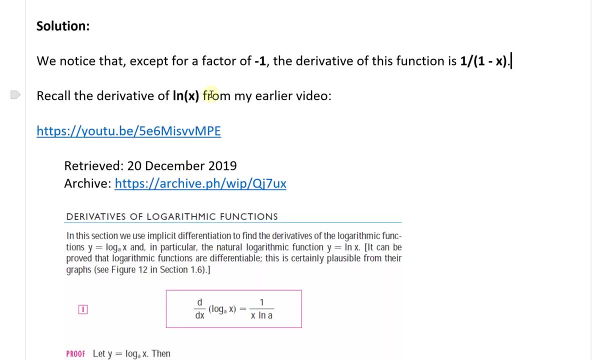 the derivative of this function is uh 1 divided by 1 minus x. in other words, negative 1 uh divided by 1 over x. this is equation 2. so first of all, recall the derivative of ln of x or natural log of x from my earlier video and this one here derivative of logarithmic functions i showed. 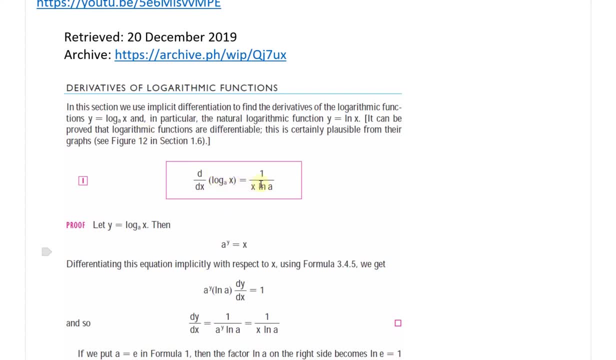 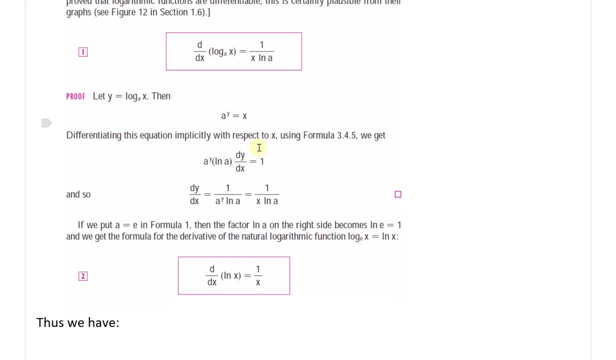 that d over dx is the derivative of ln of x and this one here derivative of logarithmic functions. x of log a. x equals to 1 over x. ln a, yeah, where lon is just log base e. so if we uh let, or if we put a and a equals e inside this ln of uh of a, so we'll get ln e, that's just uh, by using log rules. 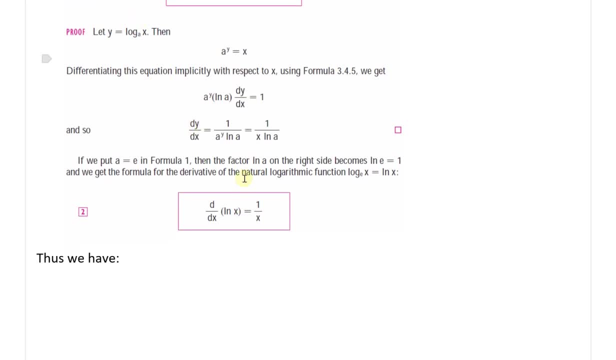 that's just equals to 1, so we just have 1 over x. so again, you could watch a video for the proof and my earlier video. so we'll have d over dx of ln x equals 1 minus x. so that's, in our case, what. 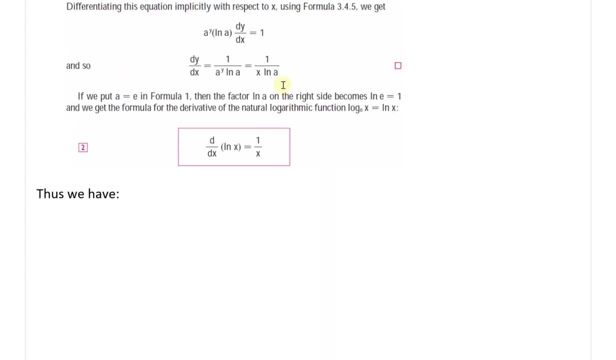 we have is this: 1 minus x. we have to put it in the derivative of ln of x and this one here, derivative of 1 minus x, is just going to be negative uh 1. so we just put a negative there. so we're going to. 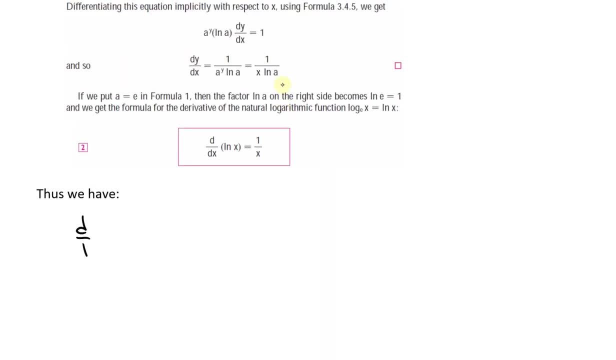 apply chain rule and so on and substitution. so thus we have is d over dx of of uh lon, 1 minus x equals 2. this is going to be your substitution. this is going to be now 1 over 1 minus x, and then using uh, uh, using chain rule, this negative x derivative of this inside function, there's going: 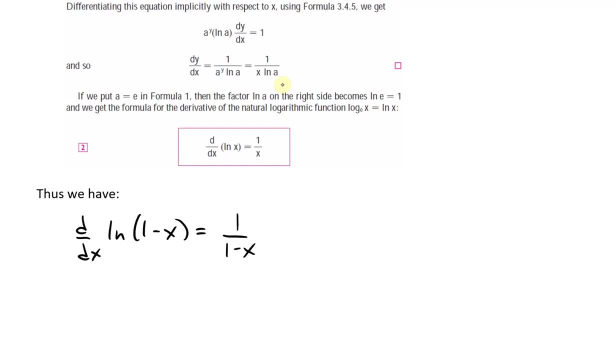 to be 1 negative 1, or this derivative of 1 minus x is just going to be negative, uh, 1. so we just put a negative there, like that. let's put a negative, yeah. so that's what we got, what we have as well, what we can do. 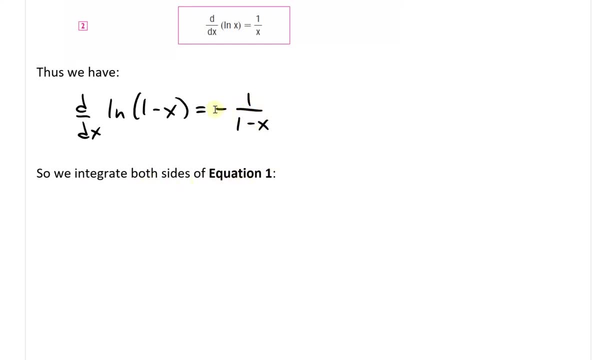 is, we can integrate both sides of equation one, because this is just equation one, but but then we have a negative term there. so what we can do is just we can move this dx on the other side so we get the integral of d, uh lon 1 minus x. like that it has to be uh complete. this is going to be. 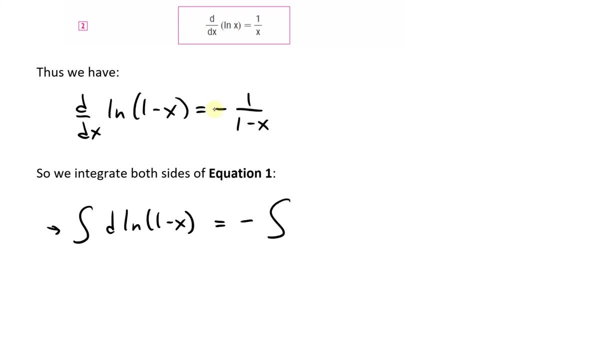 move this dx on this side, it's going to be now negative integral of negative integral of uh 1 minus x dx, like that. and again recall equation one and i'll just uh move this uh negative inside there. i'll just move this negative on the other side. we just multiply negative one on both sides. 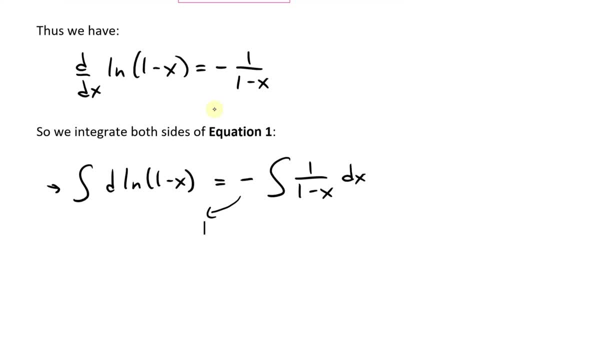 so move it across and integrate this. that is just yeah. this is just uh. this is going to be negative lon. integral of this just mean negative uh. integral of uh. d lon 1 minus x of using like this: let's use d of this. we're integrating this with this integral of d of x, so we're going to 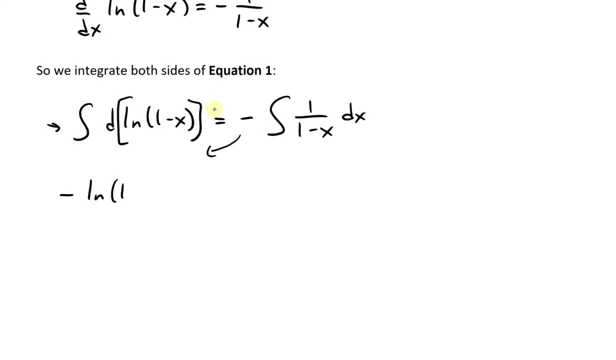 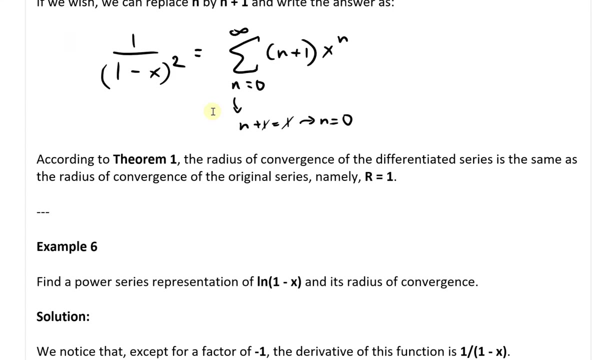 be moving this entire term. uh, that's just going to be well, lon 1 minus x. now here i'm just moving this negative sign across here, uh, all the way across to this side, so that we have here, to make it easier, right now we have the integral of this is equation one. so recall equation one. we already 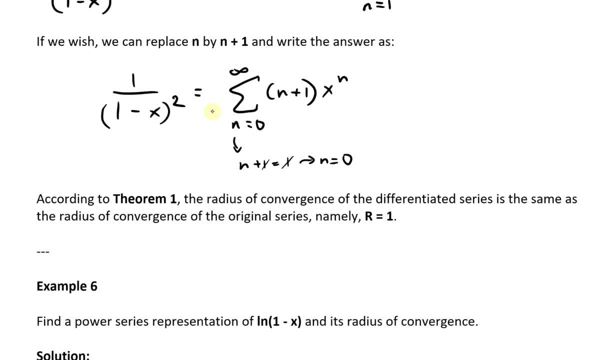 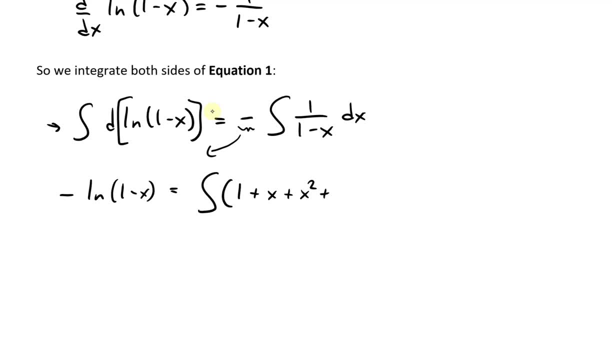 recalled it earlier. so this is going to be one plus x, plus x squared, plus x cubed, and so on. so we just uh put this in the bracket. so one plus x, plus x squared, plus x cubed, plus dot, dot, dot, and then I'll put a bracket. this will be DX. so now, if we 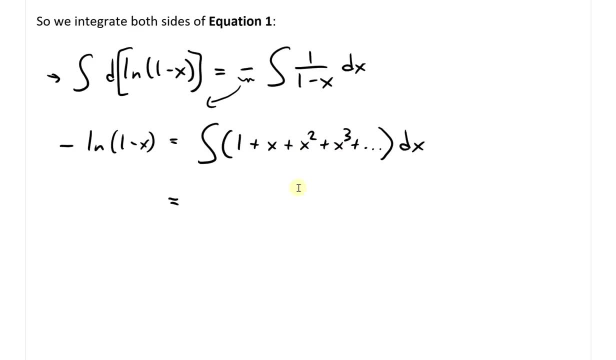 integrate this each term. if we integrate each term, the root of an integral of 1 is just gonna be X, and integral of X is gonna be, well, x squared, and then over 2. integral of x squared is gonna be x cubed over 3, and then likewise that the 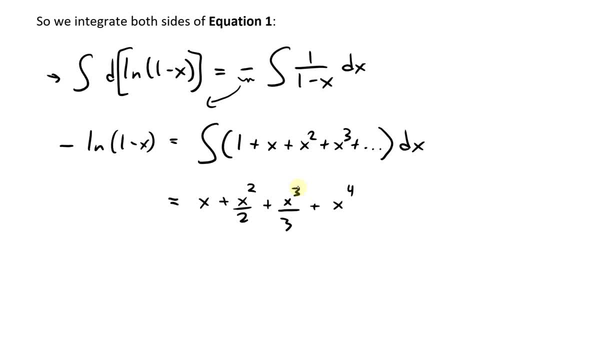 integral of x cubed is gonna be x 4 over 4, and it keeps going on and on. and then also, what we have is the constant of integration. I'll put this capital C. and now what this equals, 2 is well, this just equals 2 and power series notation: we'll 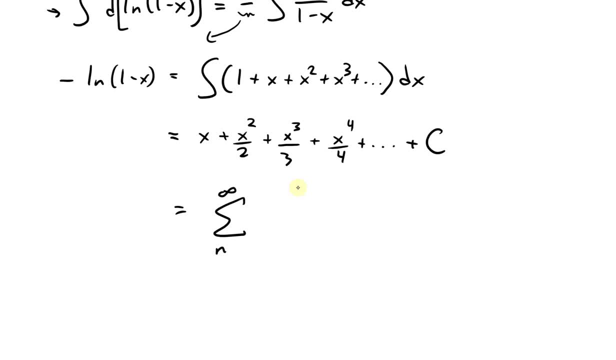 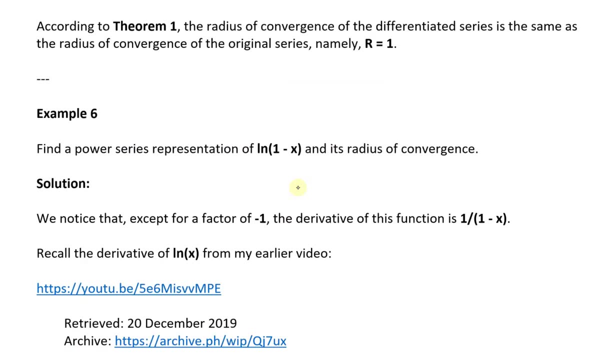 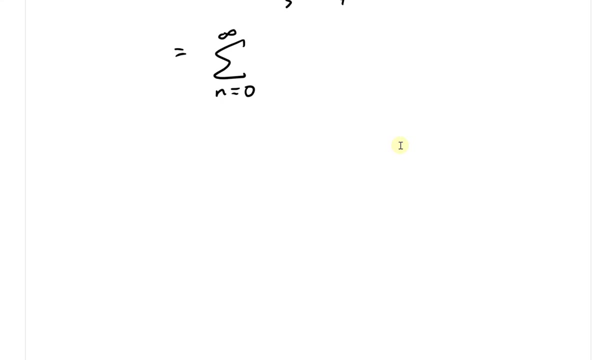 put a summation up to infinity on this one. we'll start with: n equals to 0. yes, since this is just the integral of the integral of the power series from equation 1, scroll up here. this is X- n, so this can be X n plus 1 divided by n plus 1, and you can just 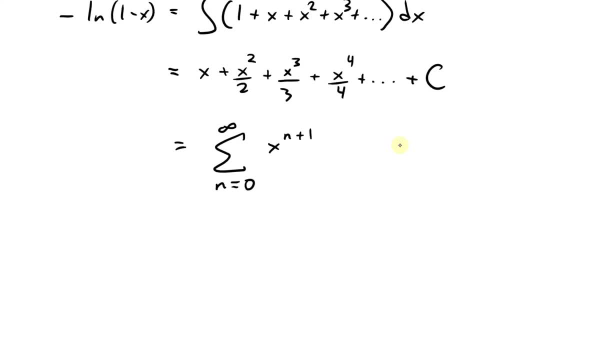 look at it right here. so this is gonna be X, n plus 1. so when n equals 0, we'll have 1, and this is divided by n plus 1, 1, X I mean. when n equals to 2, I mean it wouldn't n equals to 1, we'll have the first term, or this. this is your term. 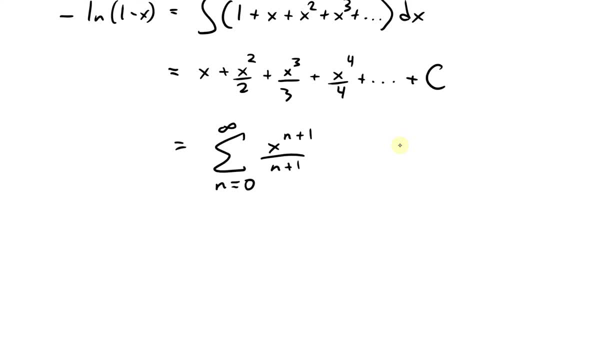 this is the first term. so 0, 1 we'll have. when n equals 1, we'll have 1 plus 1 is 2 there, and then divided by 2. so divided by 1 plus 1 is 2, and well, you've got n equals 1 if you go through it, theynet, and right then. 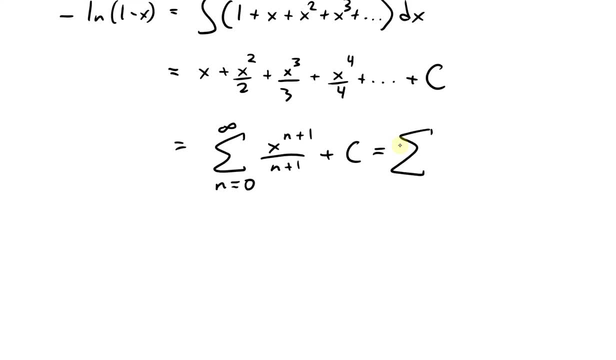 we'll have n equals 2, so we're putting out the walking tables here. we're supposed to be in 45ures. well, the set that we're assuming can't be dropped, so never mind. and it would have one, that's fine. we're going to have some in toins that height for. 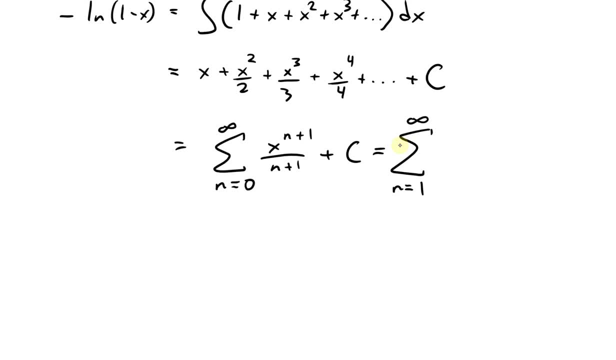 Theatre. and then if we would write this as n equals nothing? I'll just leave that for later, since I don't suppose that's a fancy plan now. at some of the points we make a 0, 0, and we'll add in to this 1, because true, then what we're doing here. 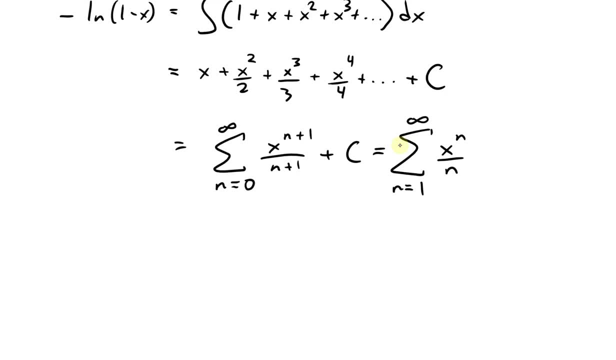 n, 1 and 1. X is 2, 1, n is 2. this can be an X to the n, X to the 2, divided by 2, exactly that, and then plus constant C, and this is all, for I'll move this over. so move this over to here and this is for again. this is the same as the. 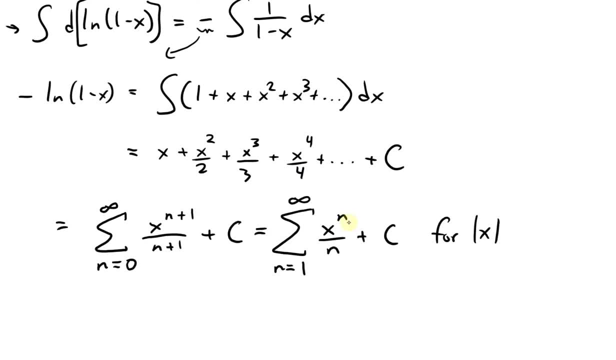 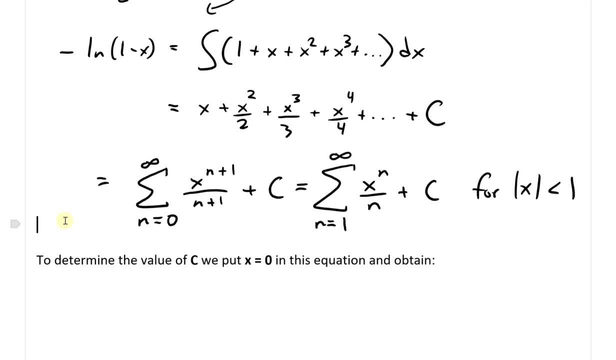 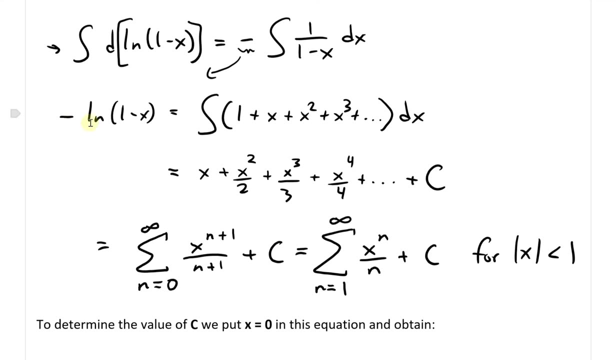 function we started with. yeah, so as the same radius of convergence. so this radius convergence is 1, so absolute value of X is less than 1 and to determine this, the value of C. here what we could do is we could put X equals 0 and into this equation and obtain so what we have here. we have this negative. 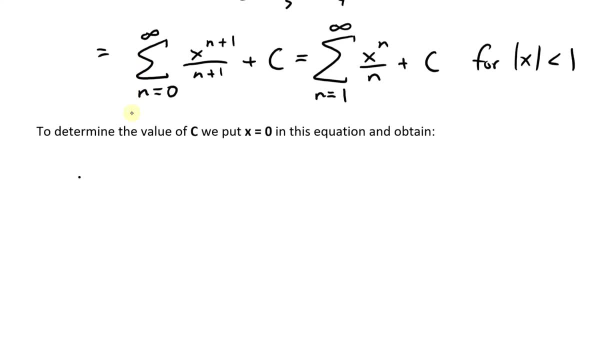 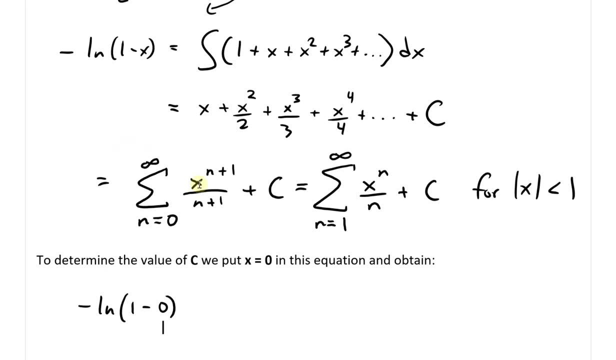 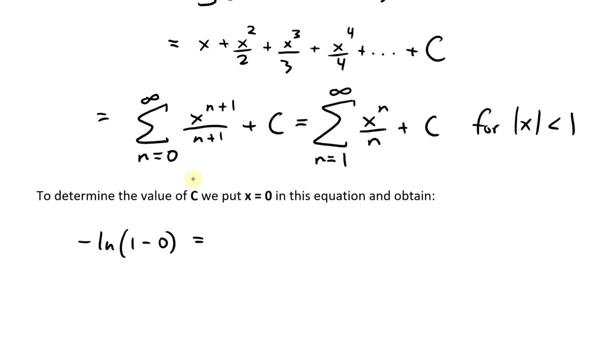 lon 1. it's what it will do is write negative lon 1 minus X 0. so 1, 1 minus lon 0 equals 2, and then just write this over there: equals to: this is summation of 0. yeah, this is gonna be well. we just, for completeness, just write this whole. 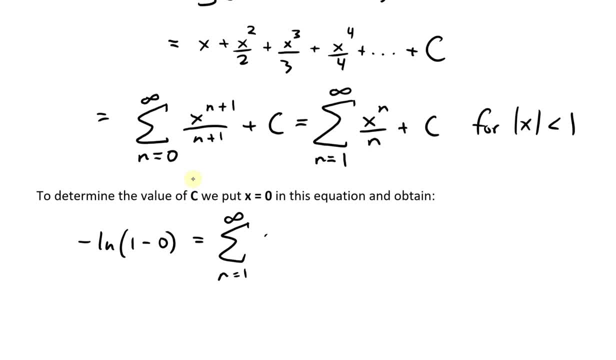 series, infinity, infinity. from n equals to 1. now we'll have 0 power of n. 0 power of n is just gonna be 0 divided by n. yeah, so this is just this, is this is just going to 0, like that, and this is again: this is a plus C, so what we have is C equals 2. yes, so then this. 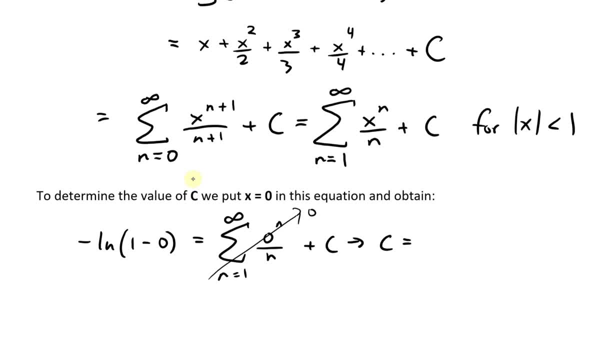 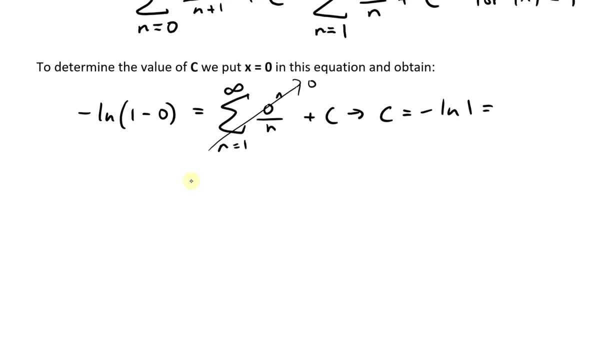 equals 2. yes, C equals 2. so we'll just write here: C equals 2, negative lon 1. now this in fact just equals a 0. lon 1 is just equal to 0. let's circle that in. you can recall from earlier videos on natural log. so recall, if you draw a graph out, the 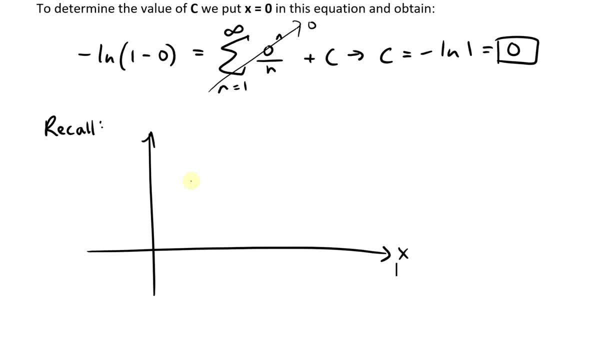 natural logs and it looks something like this: yeah, recall here if this is lon of X, like that, so that that vertical axis, so now the remember we called the curve- looks just like this, where at this point is 1, so this is gonna be equal to 0 and 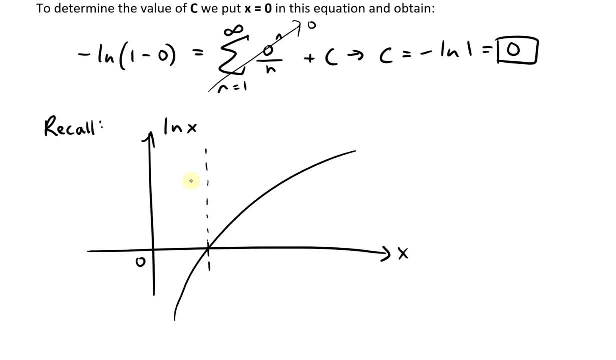 let's put a dashed line all the way cross here. so at this point we're right. here we have ln of 1. if we let this equal to y recall that this just means what we have is e to the y. so we're solving here is like the inverse of this exponential. 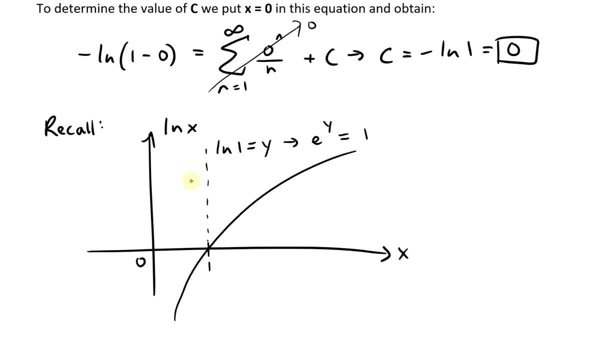 function. so e to the y equals to 1 is the same thing as writing that and the only way this is true is if e to the 0, so e to the 0 is equal to 1. the same thing is writing out. e to the y equals. 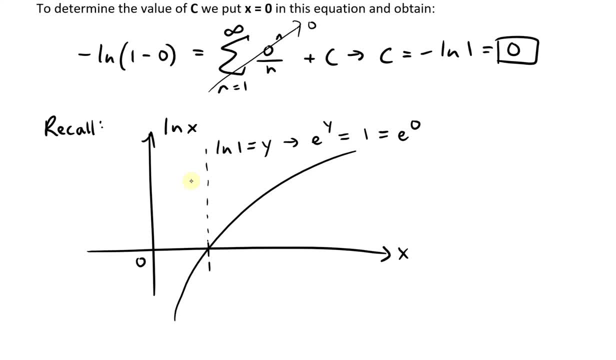 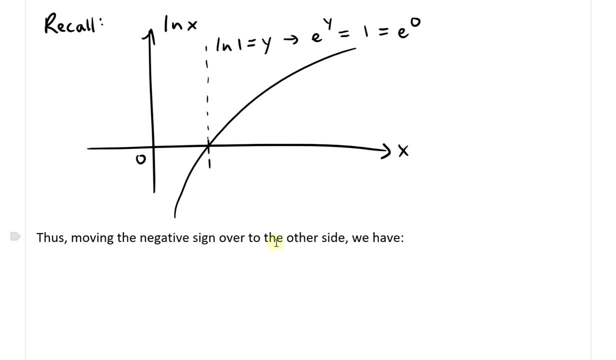 1. the same thing is writing: ln 1 equals to 0, so that equals to negative 1. negative ln 1 just equals 0, yeah, so thus, uh moving, uh, yeah moving this, uh the negative sign over to the other side. we have, so we have number. this is negative ln 1 over uh 1 minus x equals to all this stuff. 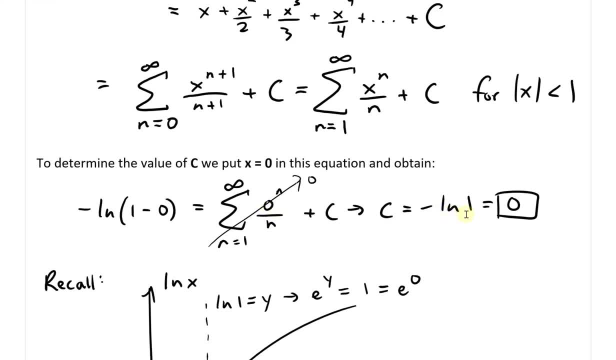 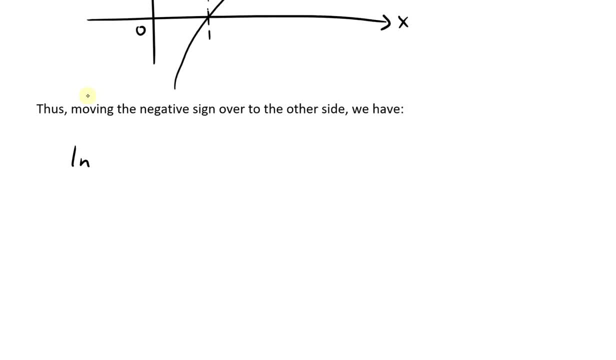 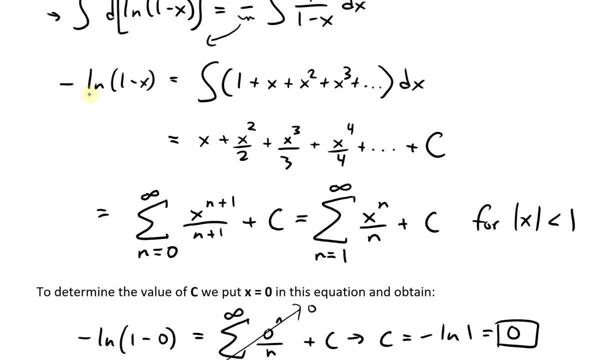 so what we're seeing now is equal to 0, because number negative, uh. 0 is equal to 0, uh. so what we have is move it over to the other side. we're going to have ln of 1 minus x equals 2- yeah, equals 2. so instead of uh, instead of having x, we have negative. 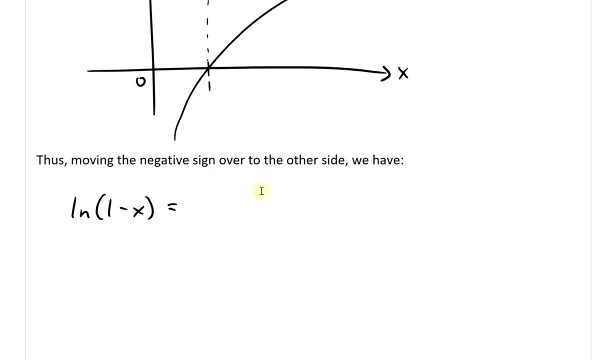 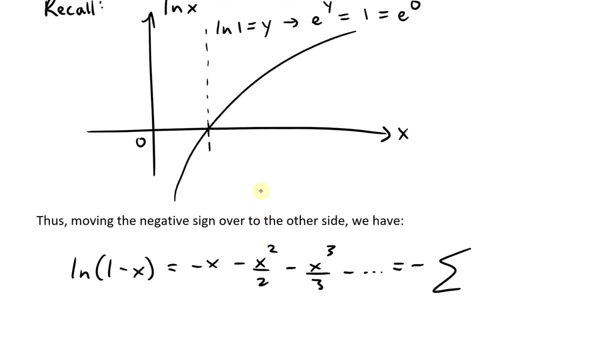 x instead of having x squared. oh yeah, so everything just becomes negative. so we have negative x minus x squared over 2, minus x cubed over over 3, and then minus, dot, dot, dot, all the way until we have negative, and then negative in this series right here. so n equals 1 up to infinity of. 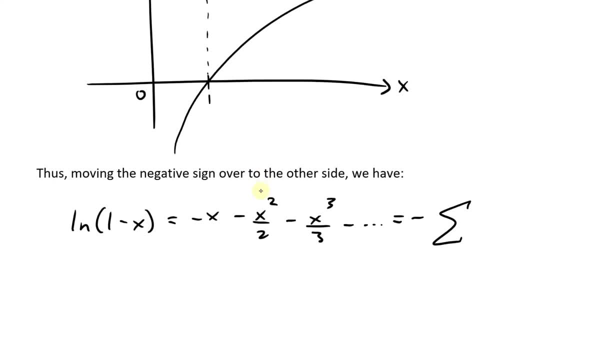 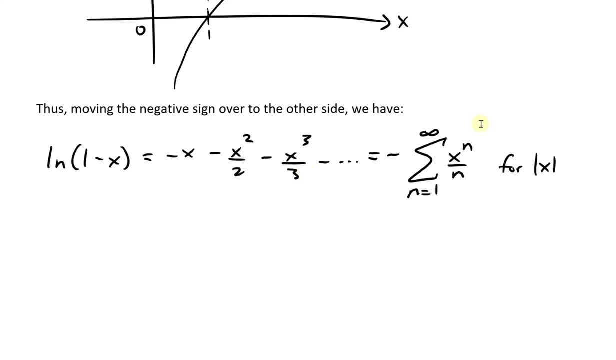 of x, n divided by n, like that, this is n equals to 1, up to infinity of uh x, n over n, where c is equal to 0, and this is again for absolute value of x is less than, yeah, less than 1, like that, which is again the radius of convergence and, yeah, so the radius of. 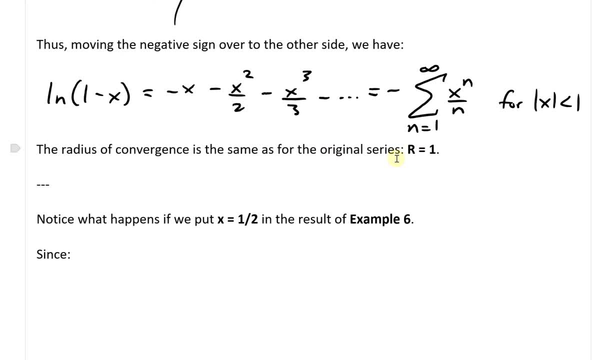 convergence is the same as for the original series or of equation 1 or negative of equation 1, so r equals to 1.. and also notice what happens if we put x equals 1 half in the result of example 6.. so what we have here, if we put uh, x equals one half, what we get is ln of. 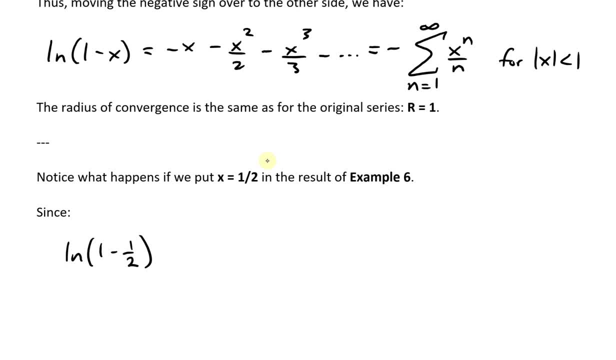 1 minus 1 half, this equals 2. so 1 minus a half is the same thing as writing. now this is the same thing as writing 2 over 2 minus 1 half. so this just equals 2 ln of 1 over 2. and now this just equals to the same thing as writing ln 2, power negative 1 and. 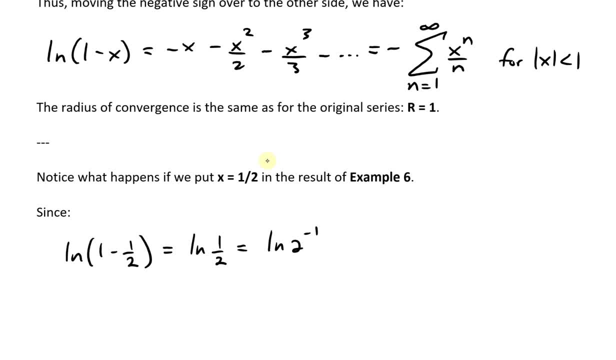 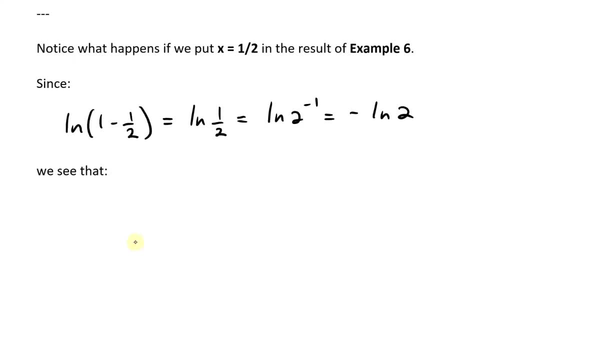 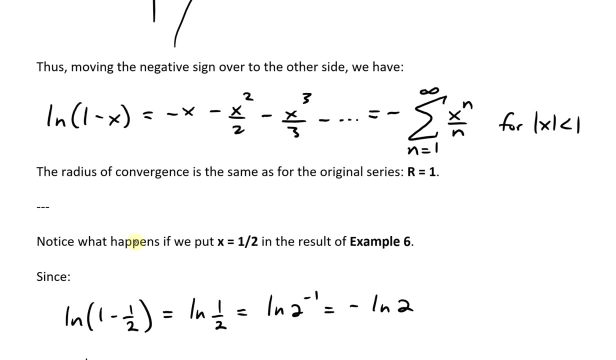 using the logarithmic rules, we can move this negative 1 down or this power down, so this is equals to negative ln 2.. yeah, so that's what we see is. uh, yeah, we see that when we're also moving this negative one to the other side, we get a ln 2 equals 2, and then we're just going to make this all positive. 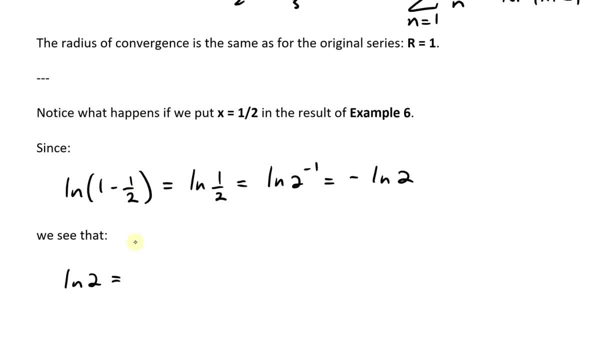 now, because we have the negative sign again, is make this all positive and now plug in this, uh, yeah, this one half for the all the x, uh, for here, for all the x's. so what we get is everything's gonna be positive. so x, uh, x is gonna be one half, so it's gonna be one half. 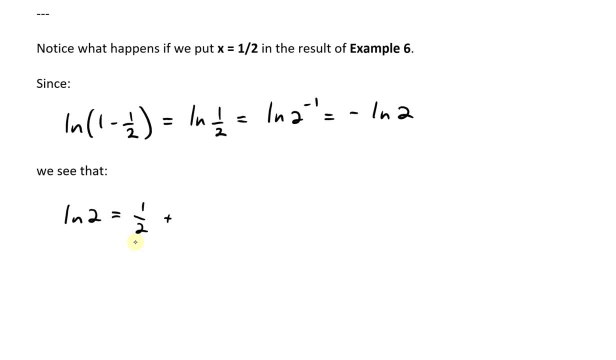 and then over here is gonna be: uh, i have plus everything's plus plus one half, uh, squared times 2, that's just gonna be 2 times 4.. that's just 8.. so also, yeah, this is my head, uh. and then next one. 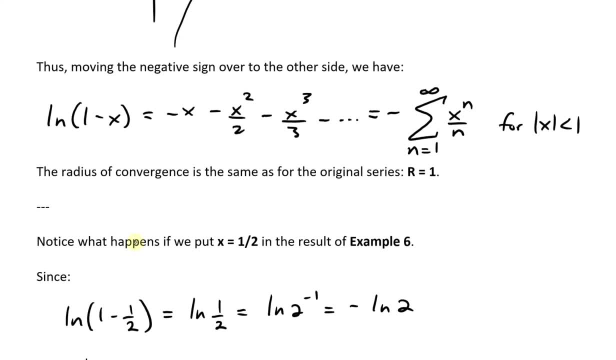 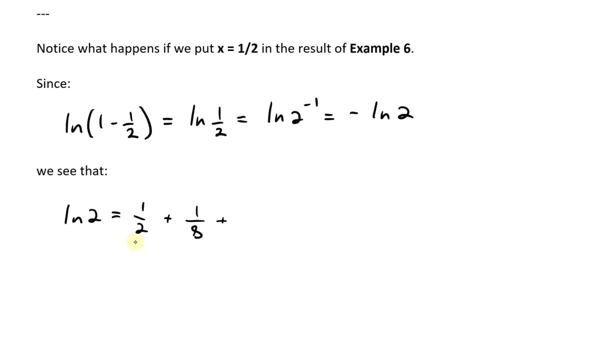 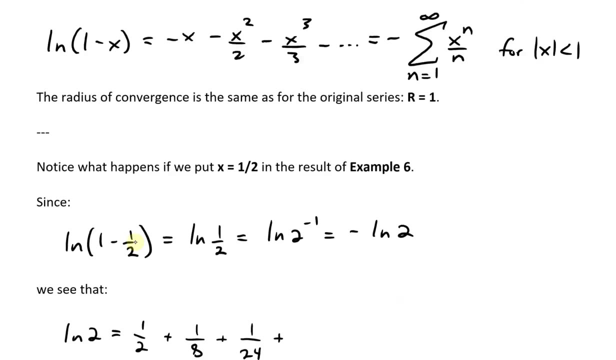 right here, plus here's x cubed, or in other words 1 divided by x to the uh, i mean 2 to the 3, and 2 to 3 is a times 3 is going to be equal to 24.. this is going to be 24, and then uh, plus again everything's. 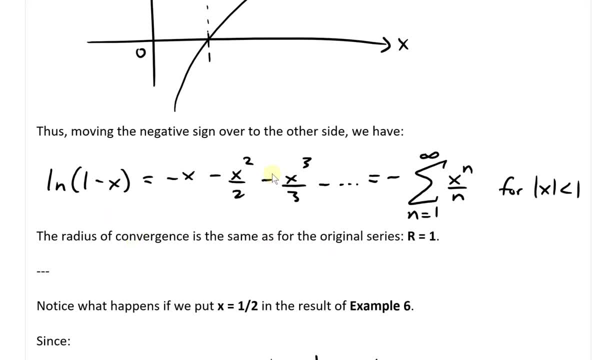 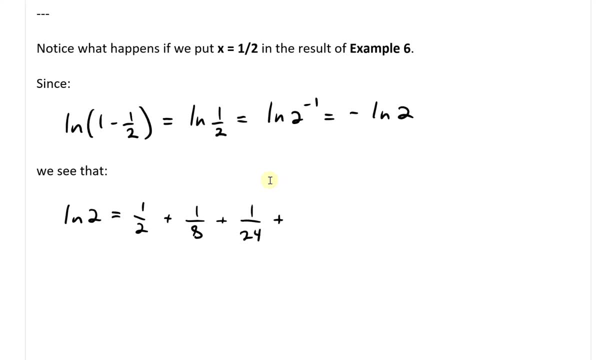 gonna be plus, and then the next one is going to be: well, let's do one more to the four. so is it going to be 1 half to power 4? 1 half to power 4 is going to be 16 times it by 3.. so this is going to be: 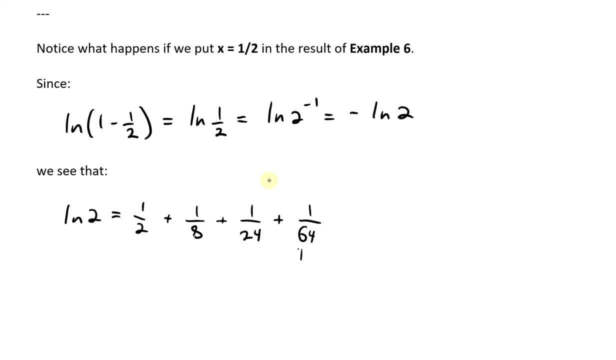 16 times 3 is going to be 64.. this is: uh, yeah, this is just 16 times it by 3.. which equals to 3 times. uh, yeah, i'll just leave it like 16 times 3.. 16 times 2 is going to be 32. 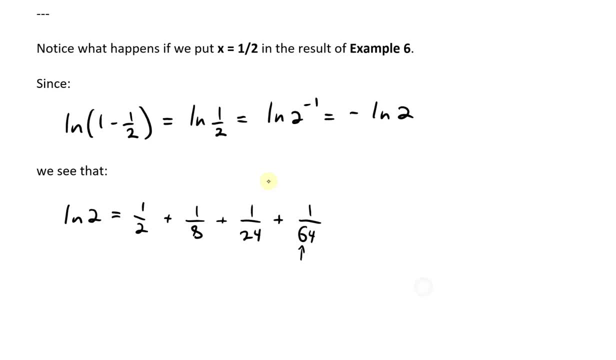 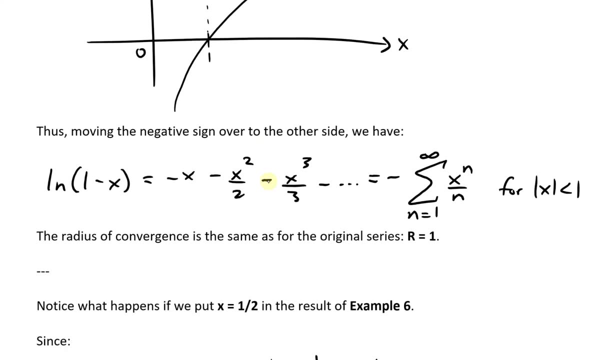 and then uh last. no, yeah, i got that wrong. i think we wrote that wrong. it's 16 times 4.. so, yeah, get this right here. so the next one's gonna be four. so x to the four is gonna be one. one over two times two to the power, four times it by uh four. yeah, so what we'll have is uh, a 16. 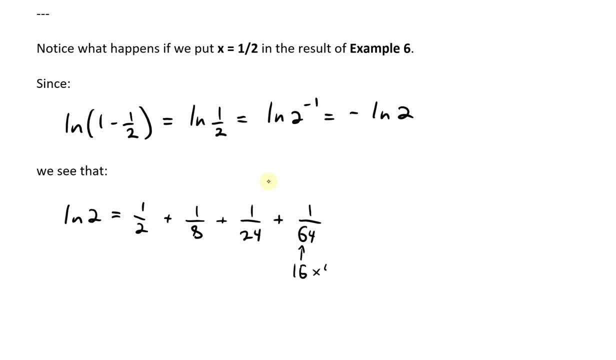 times it by a four, so 16 times 2 is 32 and 32 times 264.. so, yes, and anyway, just keep going on and on, and then this just equals two. yeah right, this has a series summation up to infinity of n equals two one. so, yes, my calculus will just uh once you notice this little pattern. so uh, this. 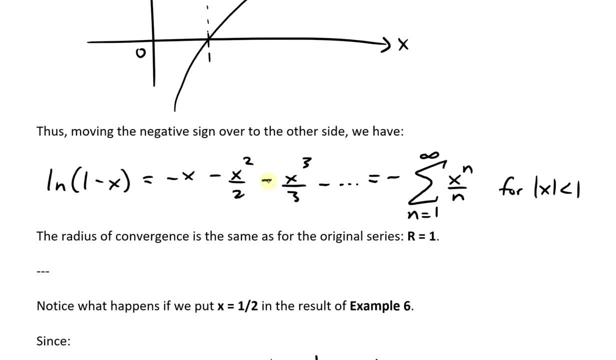 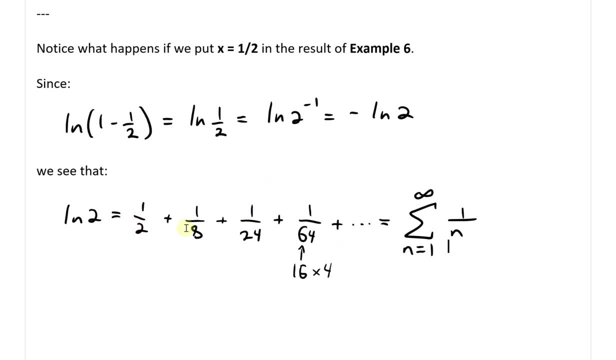 equals two, from starting from n equals to one. uh, similar to here. so what? instead, what we have is now a one over n. yeah, this is uh. so when, when n equals to one, we have one like that and then divided by- yeah, divide, this is going to be: yeah, two to the power of n, and this is uh. yeah, when x is. 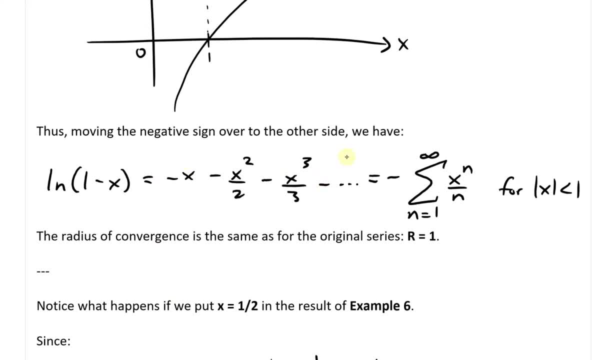 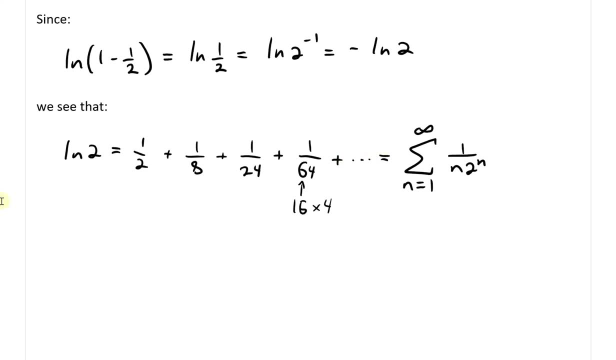 equal to one half. so this is going to be: yeah, one half, the n goes down. so, yeah, so we'll have one over n divided by two to the power of n, like that. and you can see here: so we'll have: uh, when n equals to two, we get two times two to the power of two. that's two times four is eight. when n equals to: 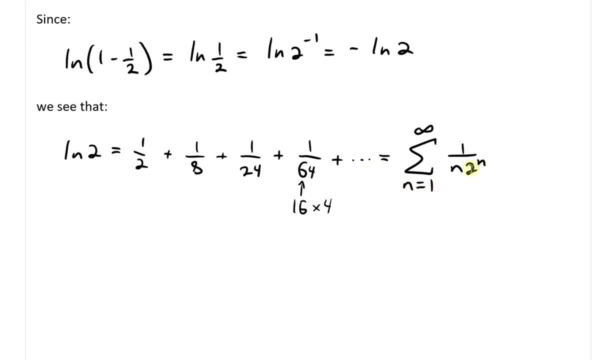 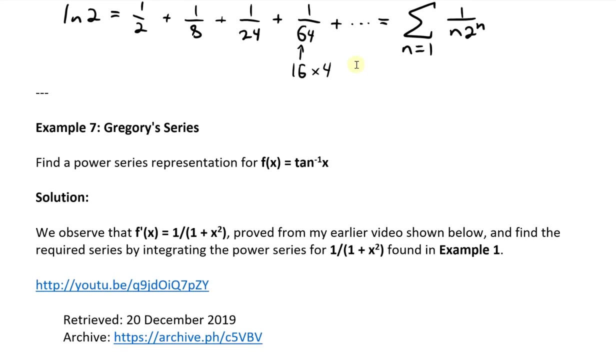 three, we have three times two to power of three, which is three times uh, three times eight, which is 24.. and then the next one is: n is equal to four, so four times two, to the power of four, which is sixteen times four, so 64.. so that's very, very fascinating, all right, so now let's uh continue. 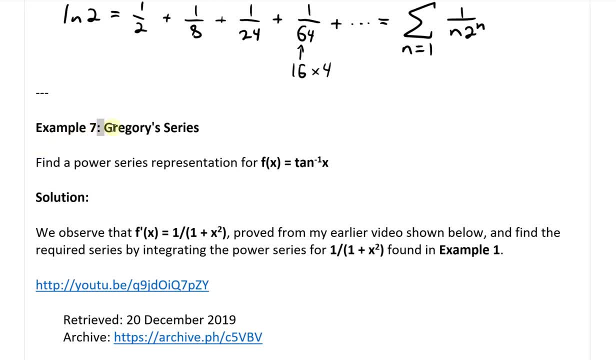 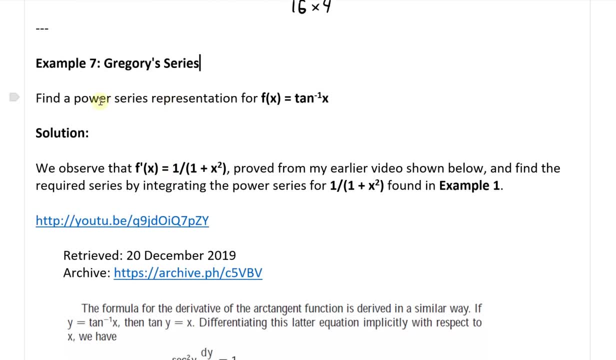 further and we'll do another example. this one is on example seven, and this involves the famous gregory's series. so let's uh jump right in. so this example asks: uh, find a power series representation for the function f of x equals to the inverse tan of x. and now let's 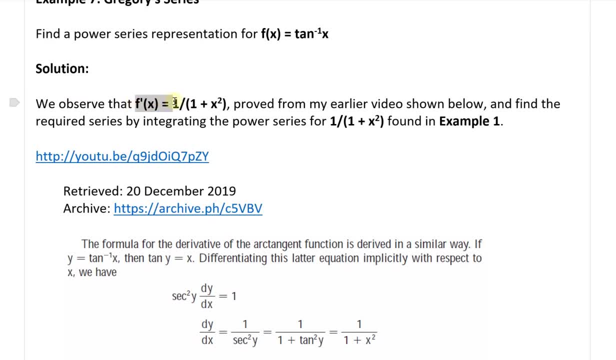 look at the solution first: uh. we observe that the derivative of this, uh, this function, fx the f prime of x is equal to 1 divided by 1 plus x squared, and i proved this from my earlier video, which is shown below, a reference below, right here, and we can find the required series: 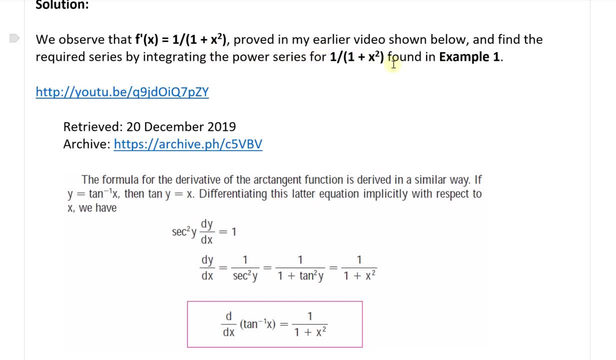 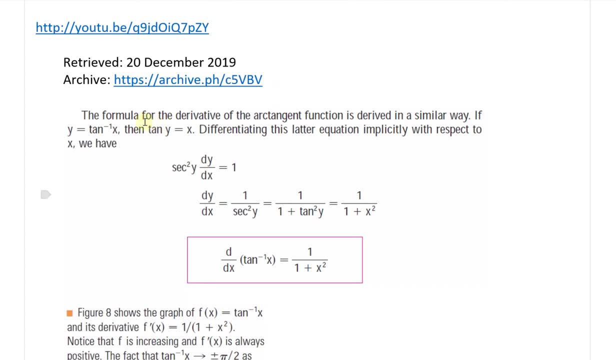 by integrating the power series, uh, for 1 divided by 1 plus x squared, and this was a. this was the function that we looked at in example one, and i'll uh scroll up there soon. uh, so basically here, from my earlier video, uh, the formula for derivative of the arc tangent or inverse tangent is derived. 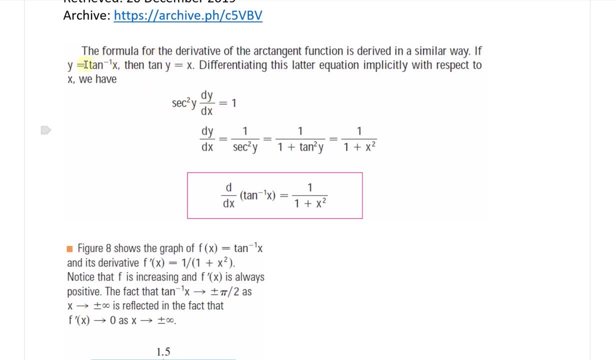 anyway. so you could, uh, basically, uh, rearrange this, write this out, uh, so if this is y equals inverse tan of x, then the same thing is writing tan y equals x, differentiating, and then moving things around: uh, differentiating tan, tan y, you will get here, which is a secant squared y and 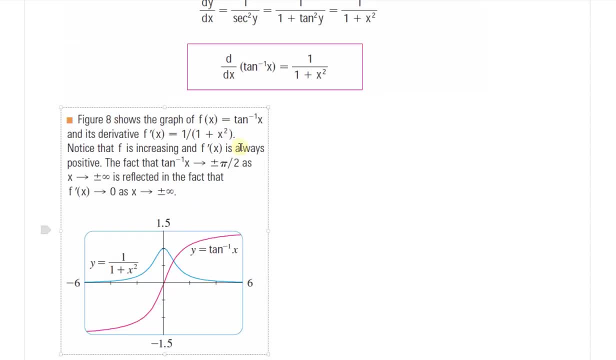 then derivative and move it around. we get this function right there. and then, uh, yeah, then the graph of this looks something like this: so this is the inverse tan of x, uh, in in pink right there. then the blue one goes up like that and goes down, yeah, which is the derivative. so initially it's a, it's a flat slope, then it goes. 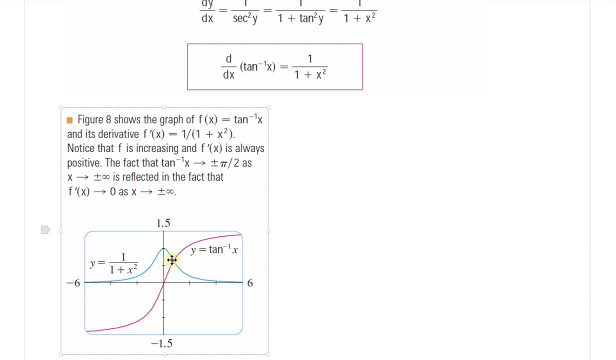 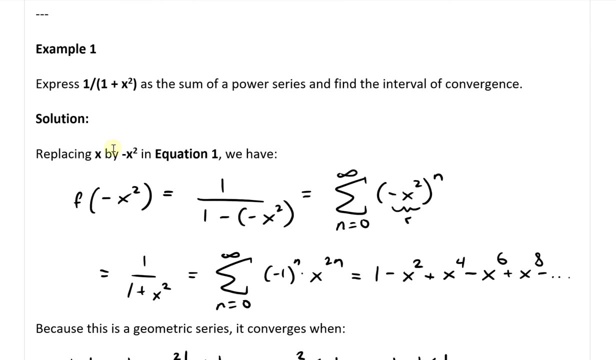 increases until it uh reaches a peak here, and then it's gradually, the slope starts decreasing. so yeah, it's very interesting. so thus, from example one, let's just scroll up here- i just uh quickly scrolled up here's example one. we uh express this as a power series: 1 divided by 1 plus x, squared. 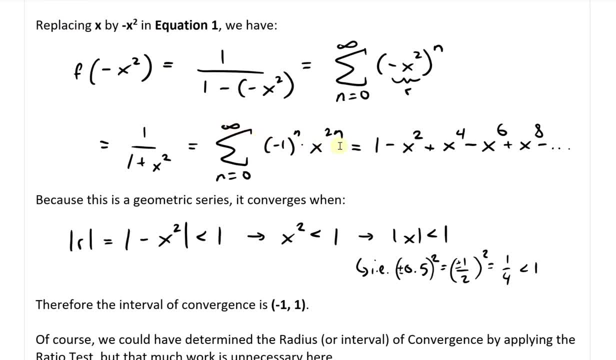 basically manipulate equation one, then we get this form right here: yeah, which is this: uh series or the summation from n equals 0 to infinity of negative 1 n times x 2n, and this equals to 1 minus x squared plus x 4, minus x squared minus x 6 plus x 8. so 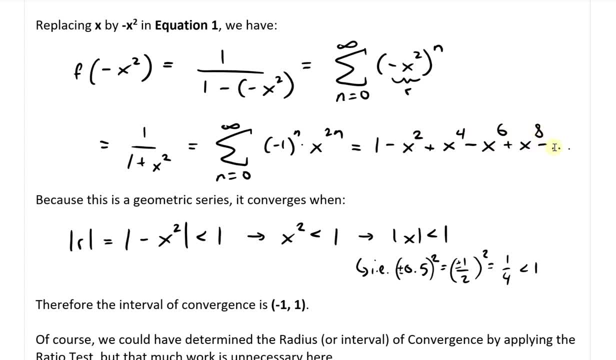 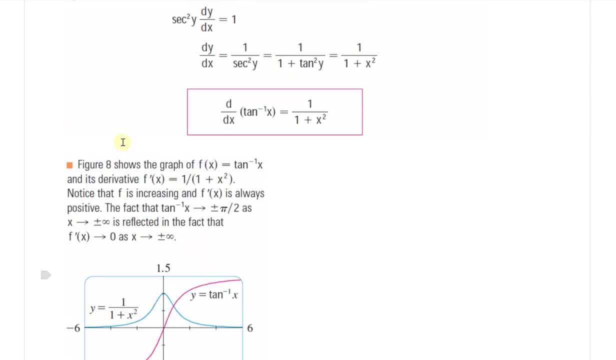 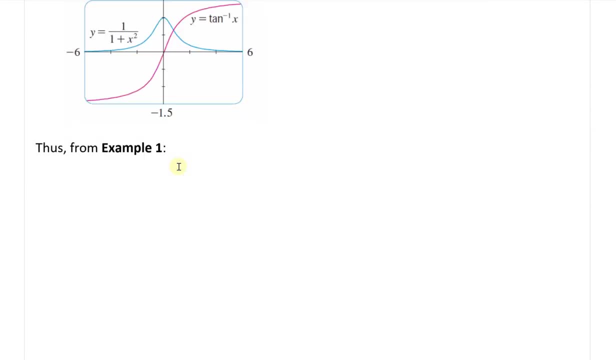 this, the powers go up by 2 and then, and it's alternating, yeah, so to teleport right back here. so thus, from example one, what we have is, well, the derivative of this function. so f prime of x equals to uh, the, the function in example one. so what i'll do is here is write d over dx of uh inverse. 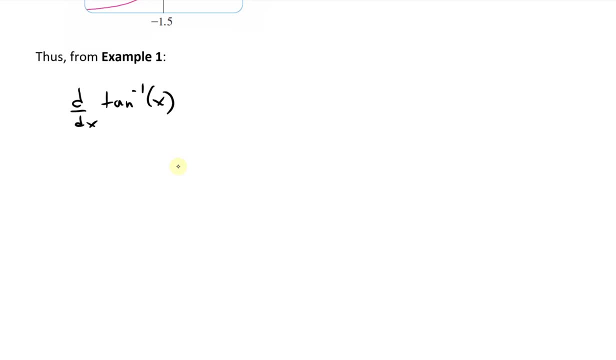 tan of x like this: this is the same thing as writing f prime of x. now this equals 2. this is going to be equal to 1 over 1 plus x squared. yeah, so what we could do is just move the dx to the other side, take the integral and yeah, just for completeness sake, just want to write it like this: 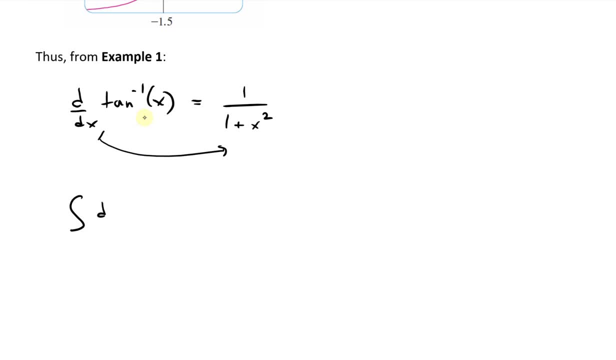 and then take the integral. what we'll get is the integral of d, uh. put a square bracket like that of uh, inverse tan of x, like this, and then dx. actually, i did no, i mean, this is the dx. yeah, so this is the retain derivative of it in for. 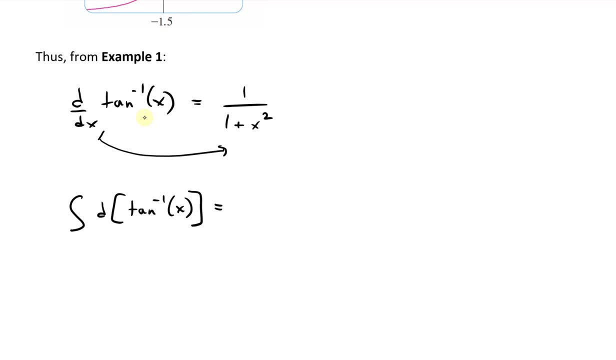 in terms of inverse tan of x. uh, this equals to well, this derivative of the integral, this is just going to be tan of x. tan inverse- um, yeah, it's just going to be the function inside here. so inverse tan of x. just for completeness sake, write it out like this: and now, this equals to now. 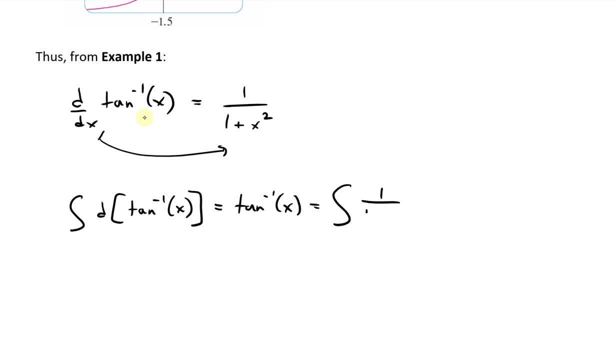 the integral, yeah, the integral of 1 over 1 plus x squared dx. yeah, that's what we have is uh, tan, inverse, inverse tan of x equal to the integral. let's put this all into 1. we're going to get 1 minus x squared, uh, and then this is: yeah, this is from. 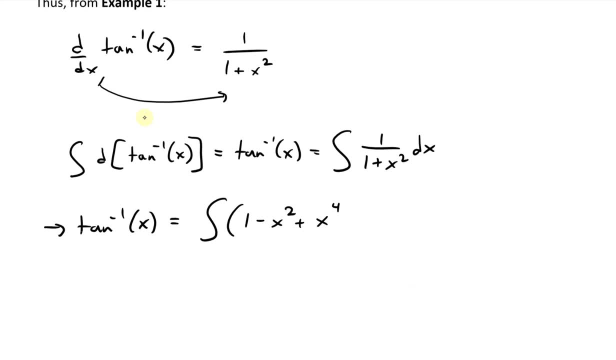 example: 1 plus x4- remember it's alternating- starts at 1 and the powers go up by 2. uh, initially it's x0 and this is x2, and it's going to be minus x6 and then plus uh, etc. dot, dot, dot, dx. yeah, and if we 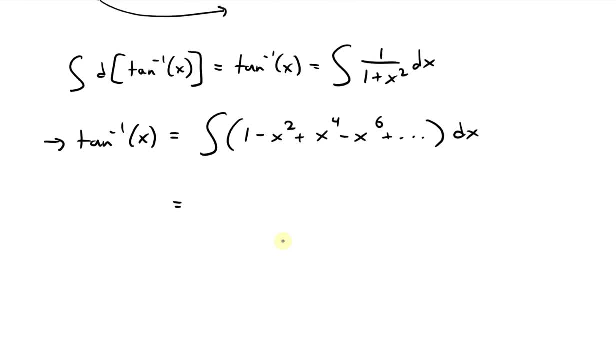 each term. and also we also combine all the integration of constants and into just one giant, one swallow. well, a giant integration of constant. we take this integral as well, accounts for this integral as well. there's an inverse tan of X right here, so so we have a constant integration right there. C, the integral. 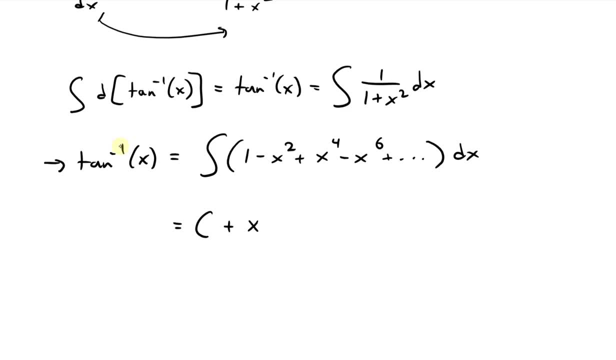 of one is just gonna be X integral of negative X square is gonna be well negative X cubed over 3, and then this one's gonna be plus X 5 over 5, and then this one's gonna be negative X 7 over 7, and it's me plus dot dot dot and I have. 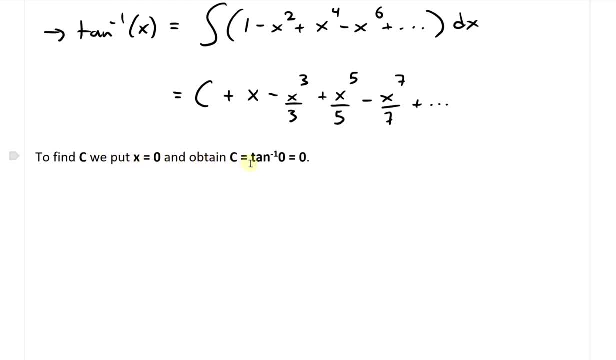 to find C. we put X equals 0 and obtain C equals 2, inverse tan, yeah, inverse tan of 0, and this just equals 0. so C is equal to 0 because when you plug in 0 inside here, all these X's and Y's are equal to 0. so we have a constant integration of. 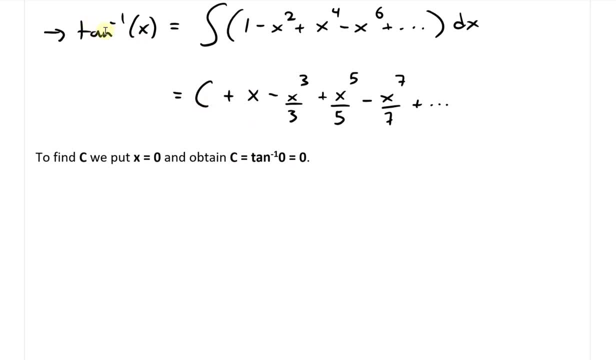 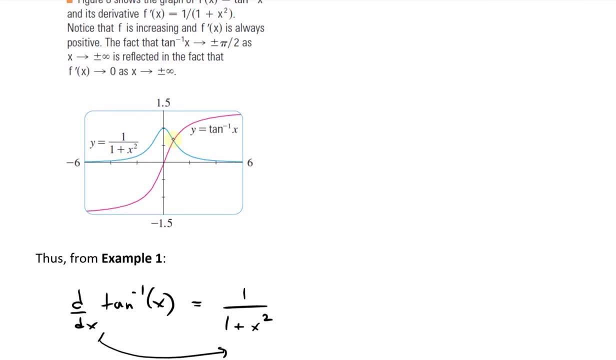 this is go to 0, so we just have C equals to this and an inverse tan is of 0, is just 0 and interestingly, yeah, this is also from the graph right here. so this inverse tan recall that the it goes like that. so this is gonna be at 0, this is at. 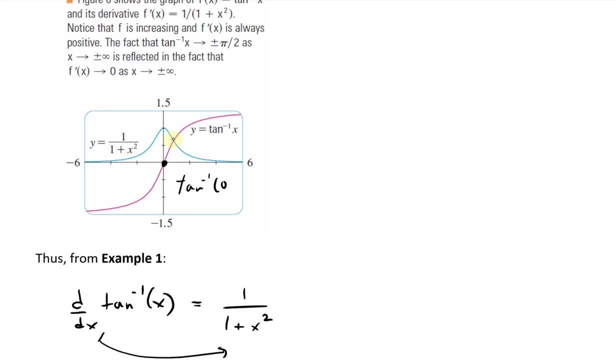 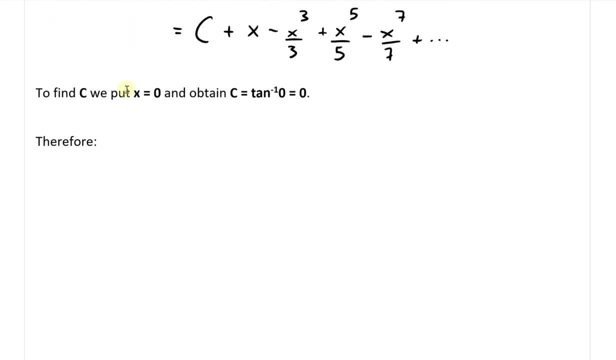 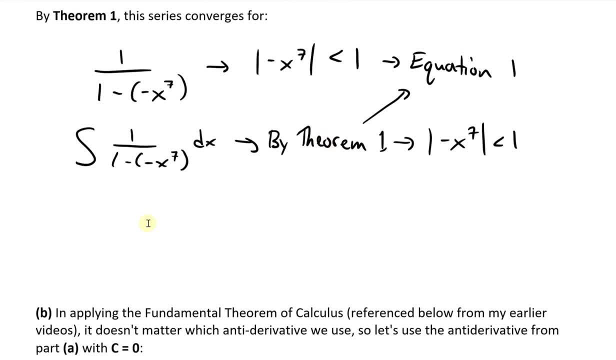 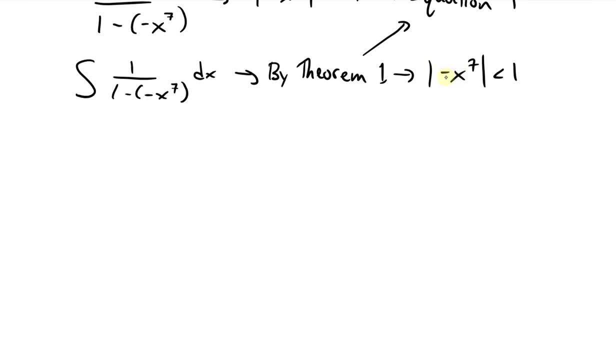 7 less than 1. and now, uh, this one here. it can simplify: here we're only taking the absolute value, so we can get rid of this. uh, this one right there, this negative there, and the only thing that could be positive, i mean that could be negative, is this absolute value of x. so we could write this: 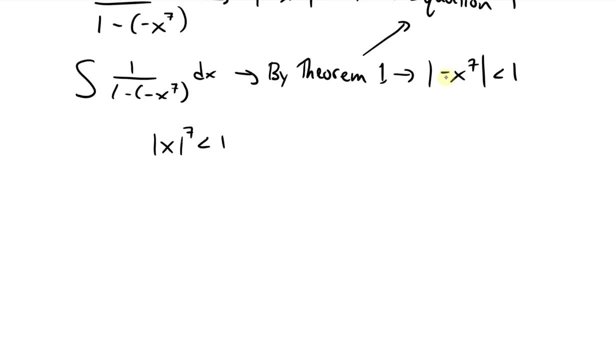 as absolute value of x to the power of 7 is less than 1. but if you take the uh seventh root like that, just take 1 over 7, 1 over 7. out of there this is still going to be 1. so 1 to power of. 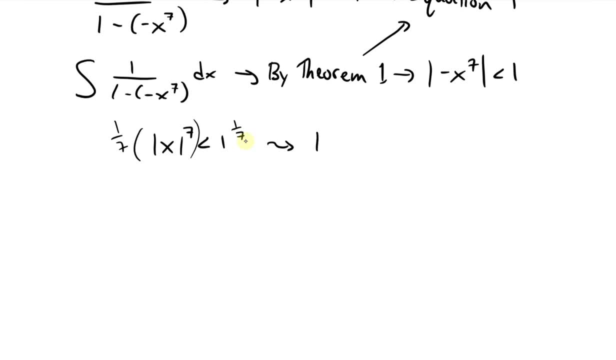 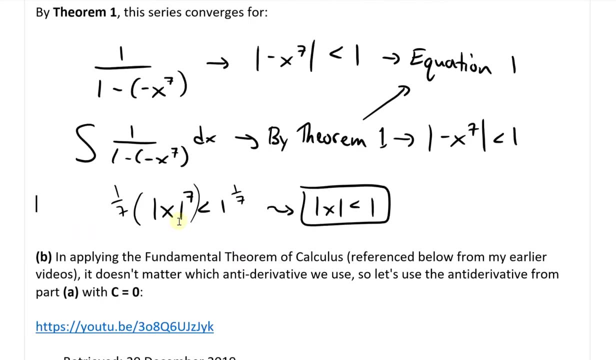 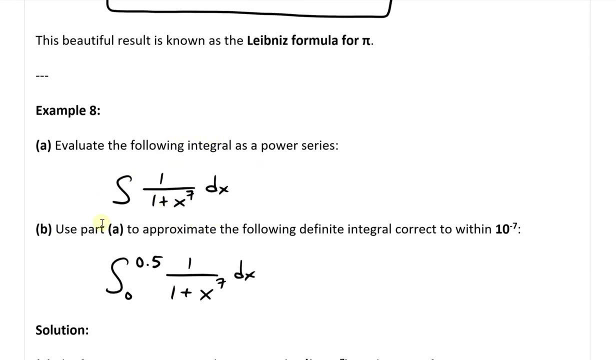 anything is always going to be 1. so then what we end up getting is absolute value of x is less than 1. so there is our radius of convergence is 1. all right, so we got that solved. now let's look at part b, scroll up here, so part b. so first we got this as a power series in part a, and then part b says 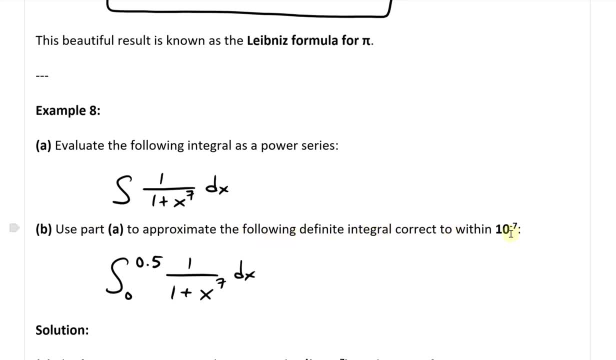 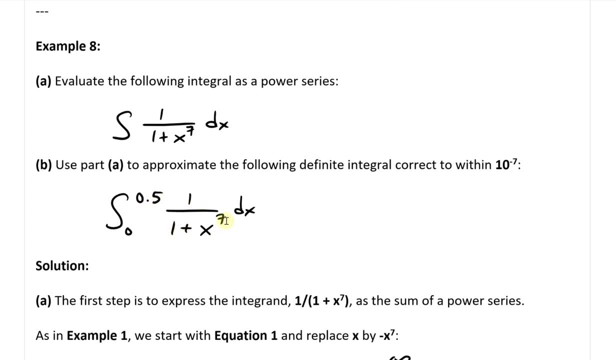 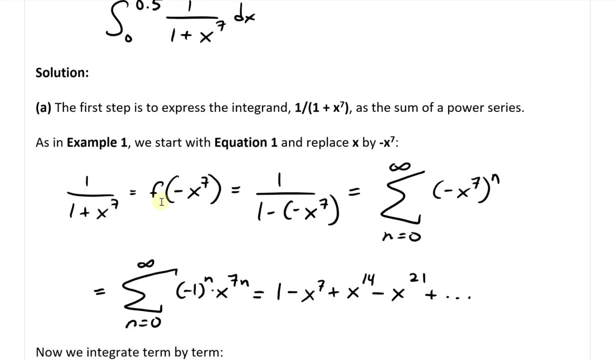 use part a to approximate the following definite integral, corrected within uh 10, to the negative 7. here we're going from 0 to 0.5 of 1 divided by 1 plus x to the 7 uh dx. and again this is within our radius of convergence because it's 0.5, which is less than 1, so let's just go over. 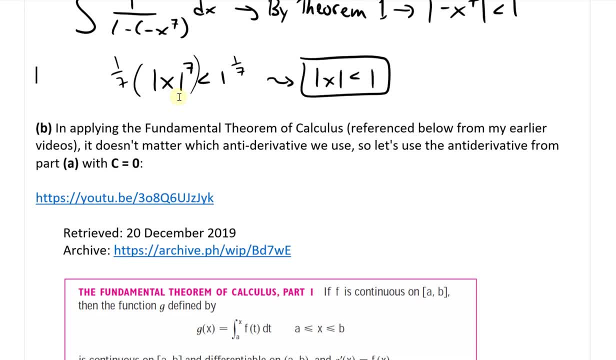 yeah, so here, scroll over here what i've written. so uh. so, in applying the fundamental theorem of calculus referenced below from my earlier videos, it doesn't matter which anti-derivative we use, because we're taking the integral from uh 0. yeah, we're taking a definite integral, so we're taking. 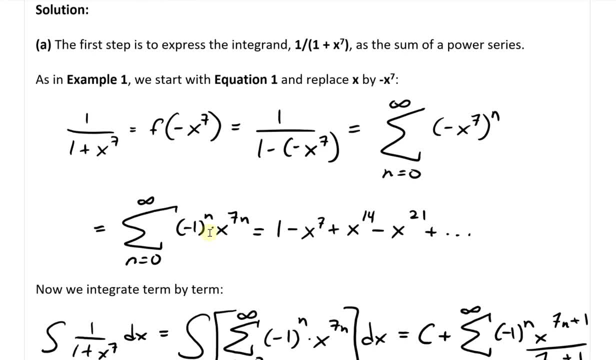 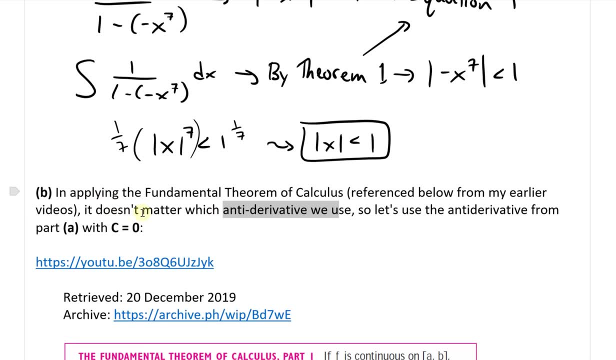 from here to here and we integrate from either one. you're going to get a uh, you're going to get a constant of integration and but they're going to cancel out. so it doesn't matter which energy anti-derivative we use, so let's use the anti-derivative from part. 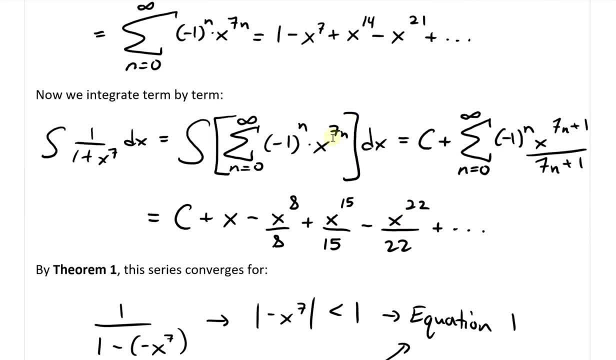 a with c equals to 0. so we can just pick this one here, because this integration constant would cancel out when we take a definite integral. so then this: this would just set that equal to 0. and again here's recall from earlier videos. so this one here: the fundamental theorem of calculus. 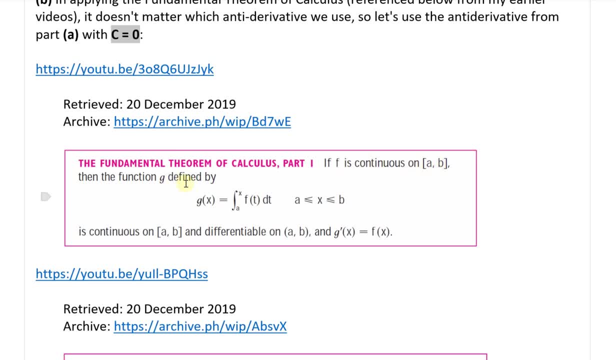 part one. if f is continuous on a and b, then the function g is defined by g of x, equals to integral from a to x of f of t, dt, where x is between a and b. yeah, then this integral, uh, is, is continuous on a and b, and. 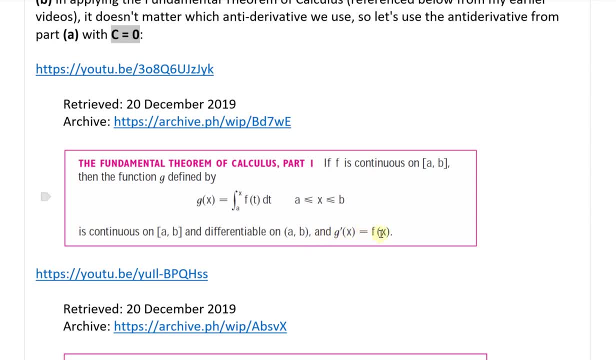 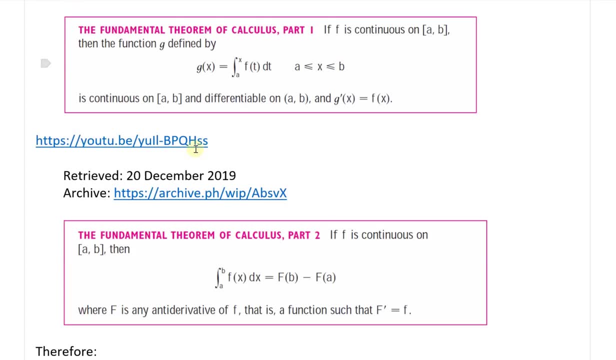 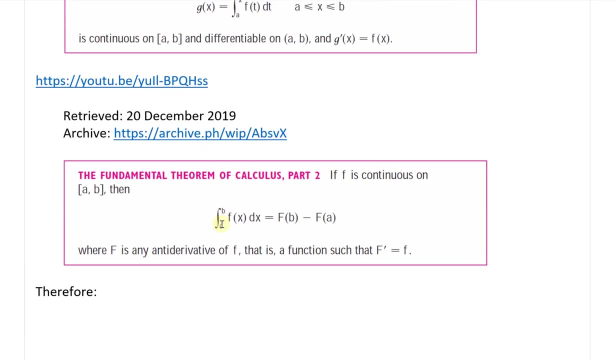 indifferentiable on a and b and g. prime of x equals to f of x. so, in other words, a derivative of g of x equals to uh, f of t. in other words, or f of t, that the anti-derivative is this g of x. and then the fundamental theorem of calculus, part two, where we look at uh, uh, the definite integral. 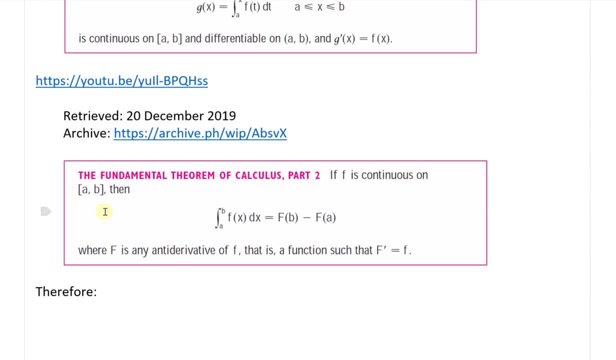 as opposed to just the variable x. so what we have, if f is continuous on a and b, including the end, integral from a to b of f of x, dx equals to capital f of b minus capital f of a, where f capital f is any any anti-derivative of f, that is a function such that the derivative of f equals to f. 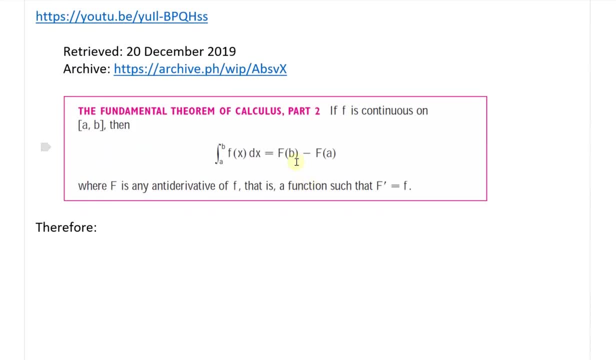 so yeah, so this definite integral just equals to this f of b minus f of a, which are anti-derivative. so therefore, and we could pick any anti-derivative, because here we would cancel out because we're subtracting. so therefore, let's take this integral zero. two point five: 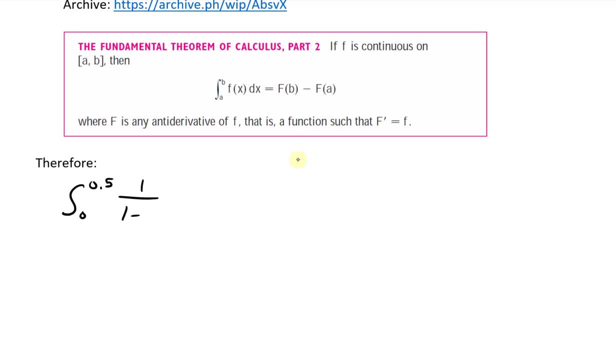 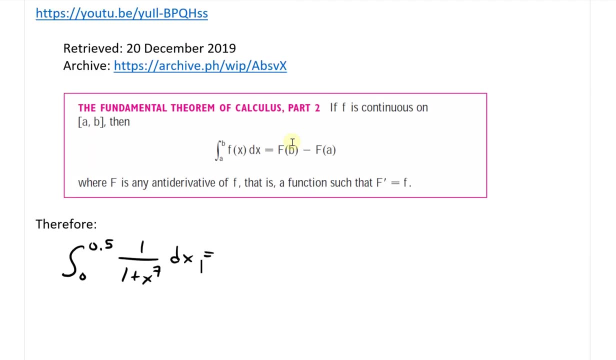 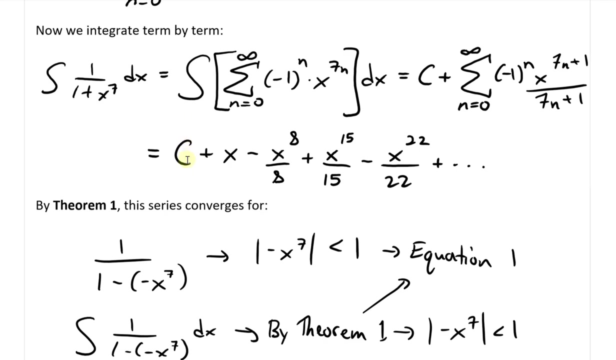 it's same thing as writing: uh, one over two, so one over one plus x to the seven, uh, dx. so now this equals two. yeah, let's just take any anti-derivative. so we're just going to pick this one right here. this is anti-derivative, is just the integral there: uh, so where c is equal. 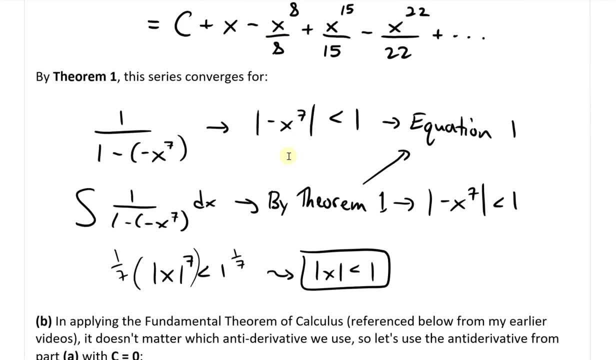 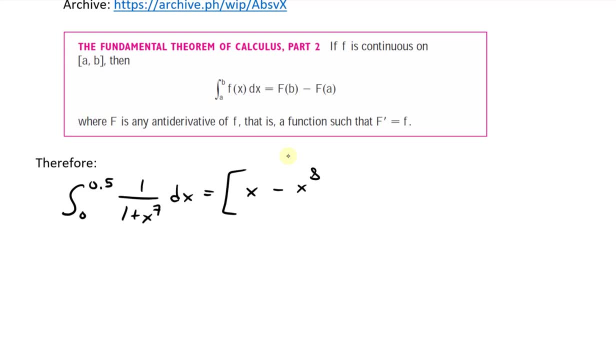 to zero, so x x, minus x 8, etc. x 15 x 22. so this is going to be equal to x, and then it's going to be x 8 over 8, plus x 15 over 15, and then minus x 22 over 22. and this is 15, yeah, plus dot dot dot. and then this is: 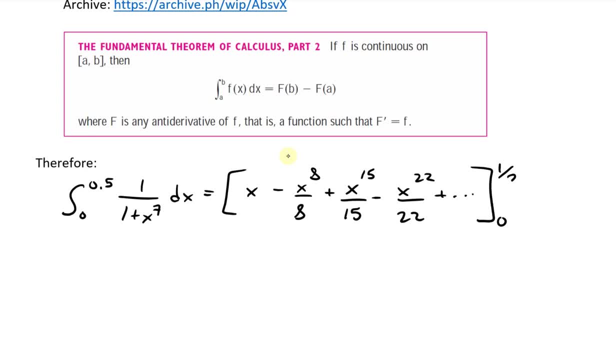 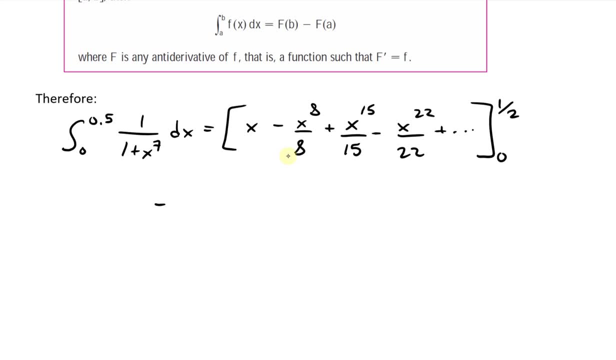 going to be the from. we're going to take it from zero to one half or 0.5, and now this is just going to be. i just plug this inside and subtract by the zero one, so this equals two. but notice the zero one's always. it's just going to go all to zero. so only one that matters is this, right here, this. 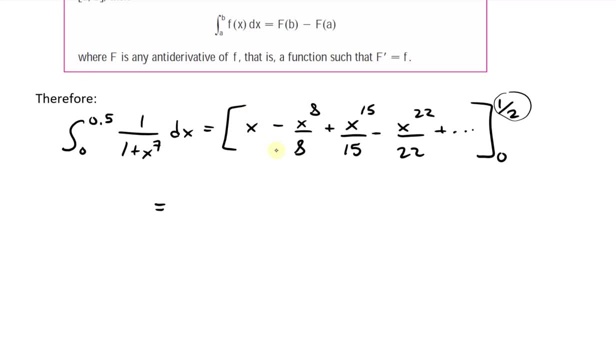 is a trivial one. this gives you minus zero. so uh, or if we had our integration constant will equal to c, but then they'll cancel out of the first c. so plug in one half. we're going to get a one over two, then minus one over eight. yeah, i mean one over uh, one over two to the power of eight. so we're. 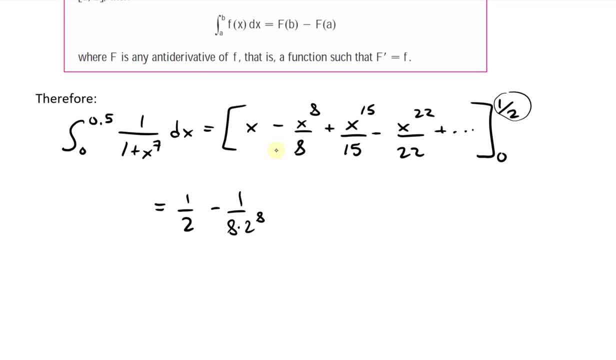 going to have this eight times two to the eight, and then, plus this is going to be a one over 15- yeah, times it by two to the 15.. and then this is going to be one over um 22 times by uh, two to the 22. so there's big, giant numbers. 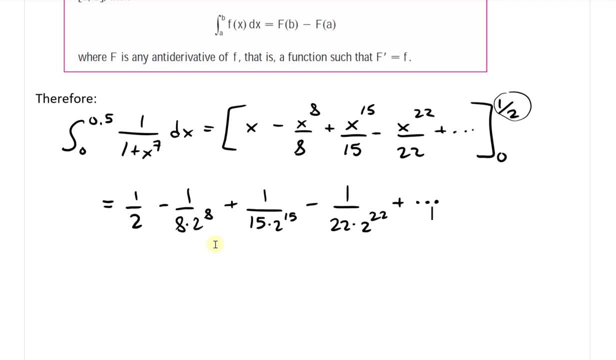 there, plus dot, dot dot. it keeps going on and on. yeah, it keeps going on and on. but uh, here let's just write this: uh and yeah for the general one. so now for the general term. it's going to be one over um, one over, yeah. so the general term, this one, this number, right here, that's just going to. 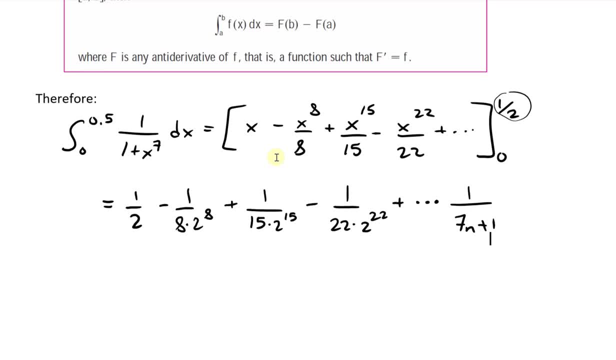 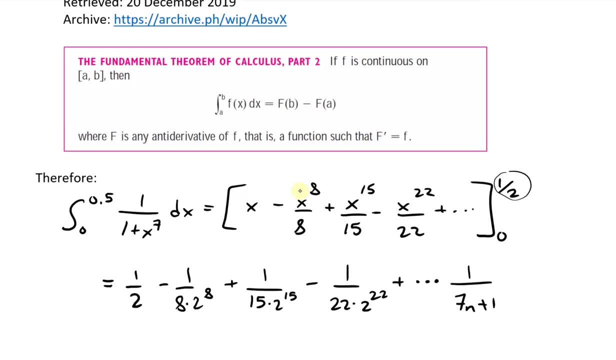 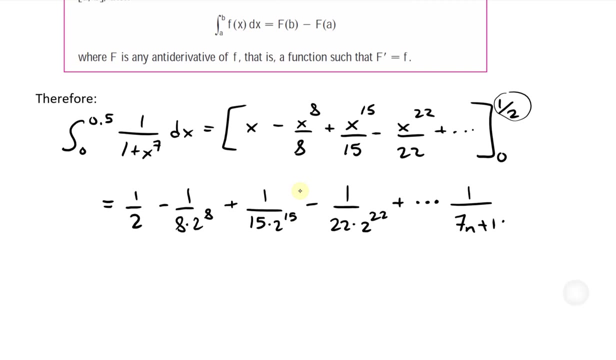 be our seven and plus one. that's the same thing as our anti-derivative right here. uh, this is our seven and plus one. so eight, 15, 22, and so on. so eight, 15, uh 22, and then this is going to be times it by: notice your eight and eight. so this is going to be times it by. let's. 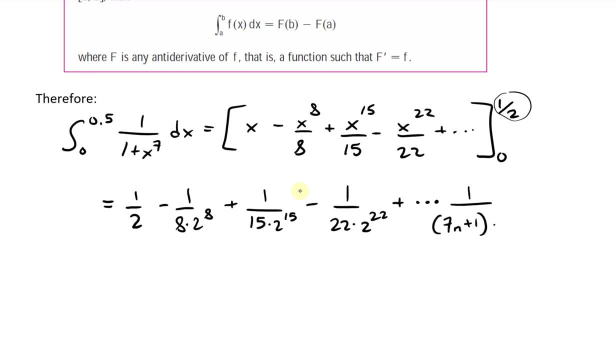 put this in bracket. yeah, times it by. uh, this is two to the seven and plus one, and likewise it's going to be plus dot, dot dot. it's going to keep going on and on. so, yes, yeah, this keeps going on and on. so, uh, also, we get a look at this one here. so if we have n equals zero, 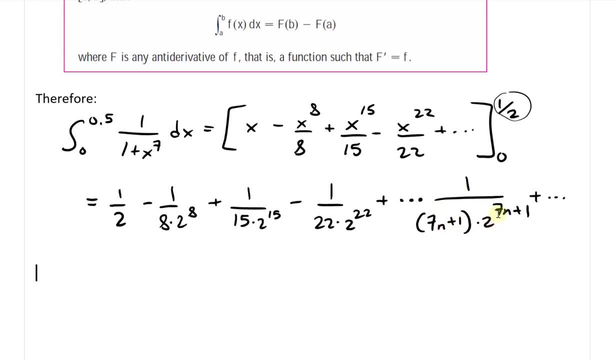 uh, this is going to be one divided by uh, one and then two to the power of well, one, that's going to be one over two, and and if n is one, we get, this is going to be eight. two to the eight, eight and two to the eight, and so on. if it's three, this can be, or, uh, let's say, if it's two, this would be 15. 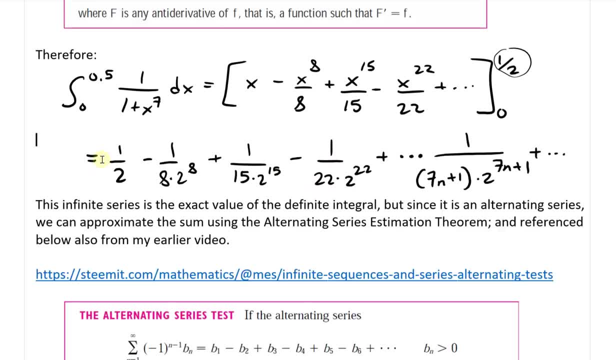 and then two to 15. so, yes, very, very fascinating. all right, uh, yeah, so now this uh infinite series is the exact value of the definite integral right here that we're uh trying to solve. but since it is the same, we're going to have to approximate the sum using the alternating series theory, as 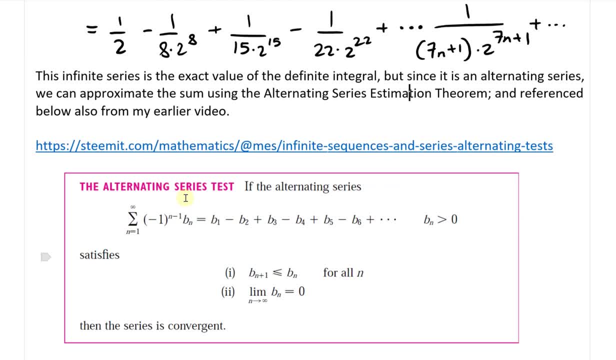 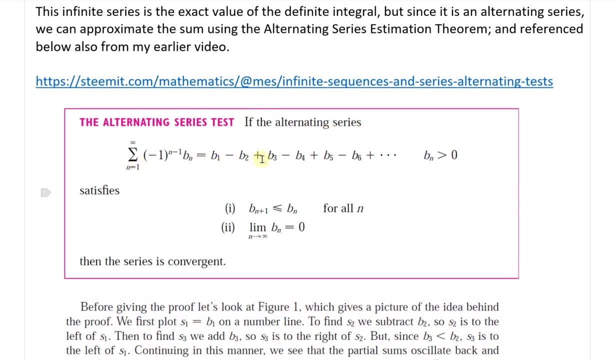 alternating series estimation theorem and reference below from my earlier video: uh yeah, so here was the alternating series test that i referenced earlier as well in this video. so if the alternating series we have this b1 and minus b2, plus b3, etc. satisfies bn is greater than zero. 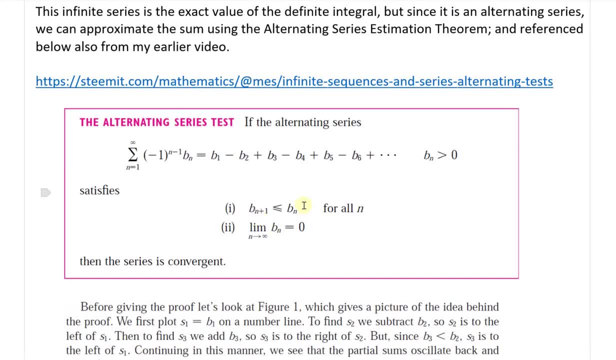 and we have this case. this was, this was the alternating series test, where the bn's uh become increasingly smaller than equal to that. this is just for convergence and the limit is approaching zero. so this is convergent. we already have a radius of convergence. here is for absolute value of x is less than one. 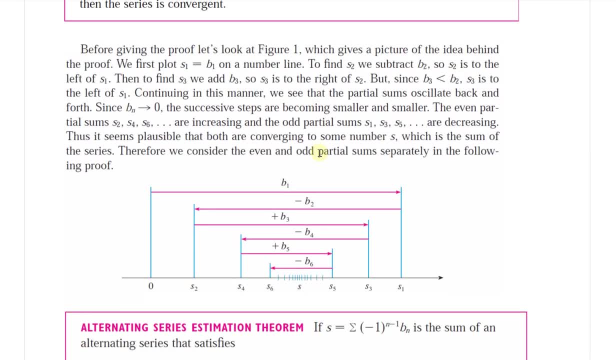 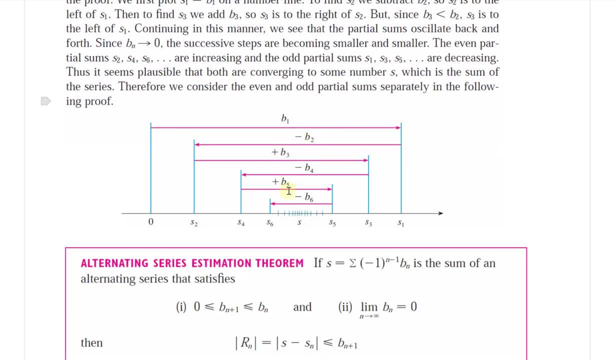 which this will converge. uh, so going further. yeah, so, since we have an alternating series, it's going to be alternating like that. essentially, what we end up having is we're going to have, let's say, we're going to have it converge to a sum s, but then for each term. so if we have the first, 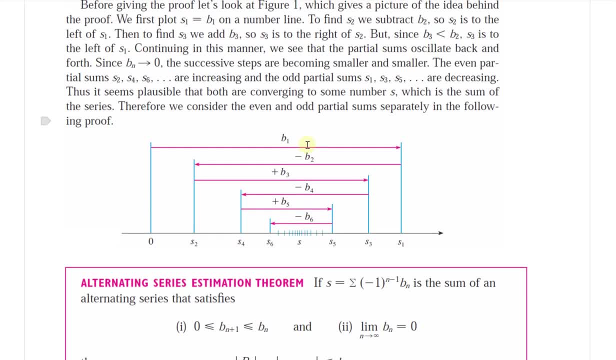 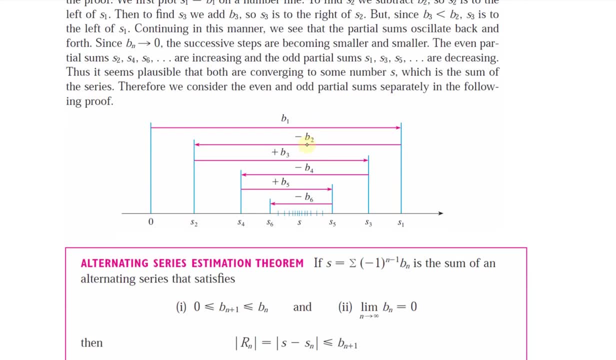 partial sum. that's just going to be, yeah, the first partial sum. for example, we're going to have a b1, so we'll have a b1, so this is going to go such that here is going to be 1 over the b1 value in here and the least. 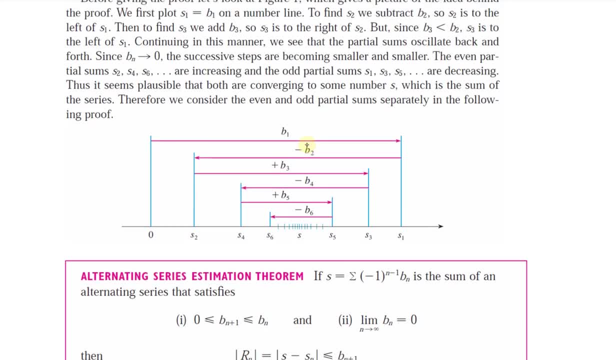 you're going to be on in the right-hand corner, so it's got a b1-b2 minus 2b2, and then our next one, in our case, is going to be 1 over 2, so it's going to go all the way across here and then the 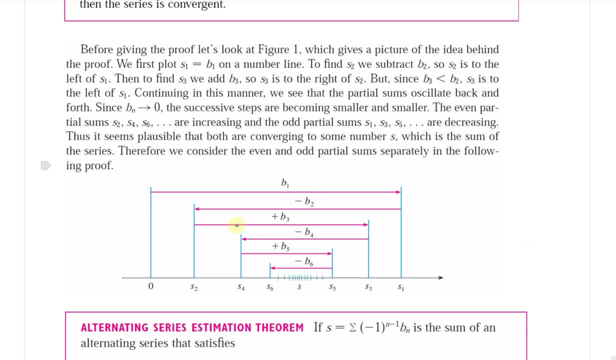 next one minus b2. it's going to go all the way across here and it's always going to be less than it. so this alternating series test will be satisfied when for when it converges. so it's always going to be less than equal to this bn for all n. so then it's going to go over here and then 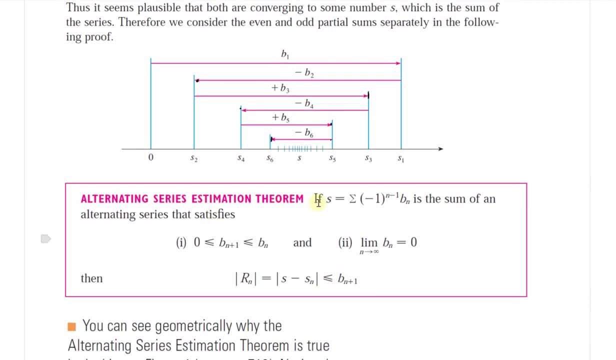 this b3 is going to go over, or what do you add? it's going to go there. when we subtract and go there, we add b5 and go. Gustav Wolk series. theorem states: if s equals to this alternating series, uh, right, here a summation. 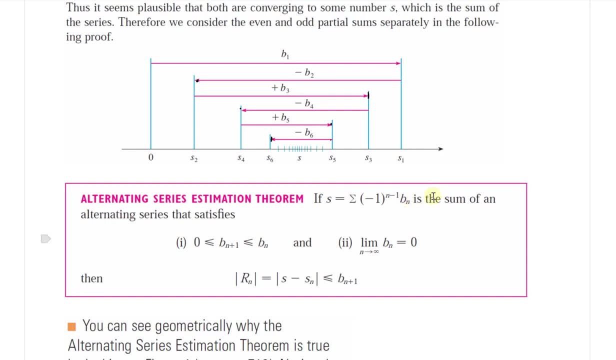 of negative one, power of n minus one bn is the sum of an alternating series. that satisfies, uh, the alternating series test there where absolute value, oh no, where bn plus one is greater than equal to zero and less than equal to bn. and yeah, and uh, right here also, yeah, this. 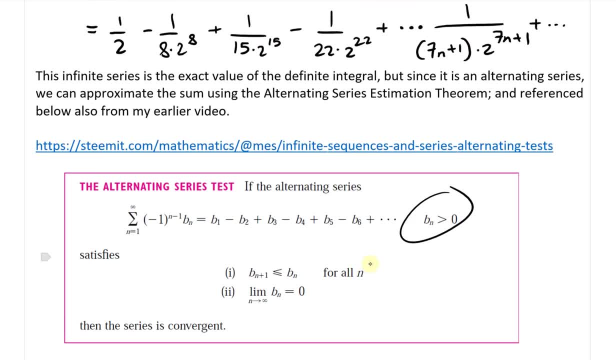 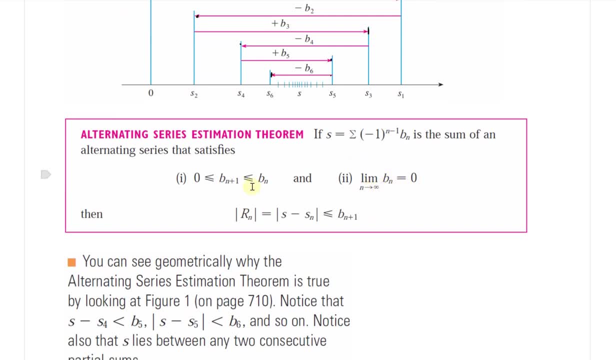 is greater than zero. it's same thing over here: alternating series test. this is for non-zero values and the second case limit is approaching zero of bn. as n approaches infinity, then the remainder, rn, is going to be. the absolute value of the remainder is equal to the actual sum minus. 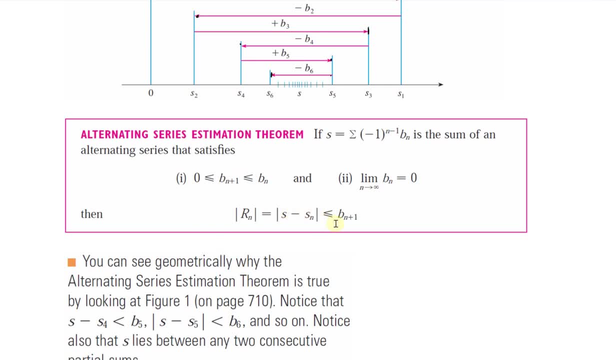 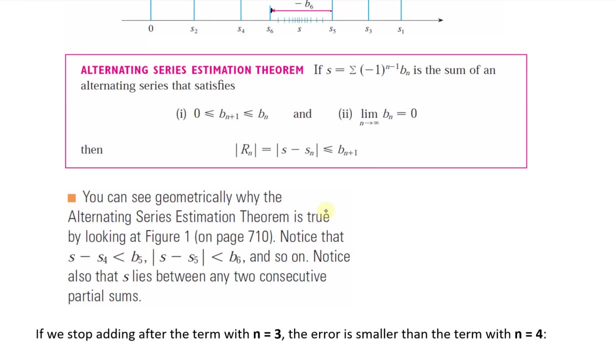 the partial sum of n absolute value of the difference is going to be less than or equal to bn plus one or the next term. yeah, so that is our estimation. we could use the next term and you can see this. you can see geometrically why the alternating series theorem is. 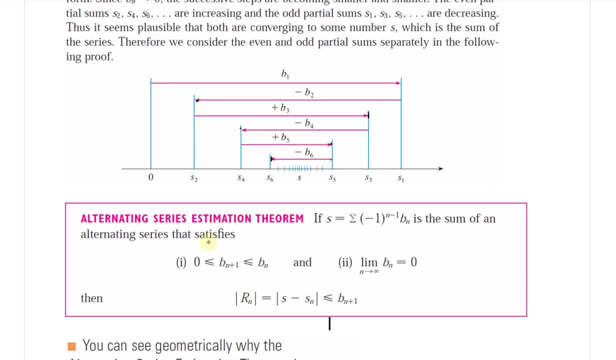 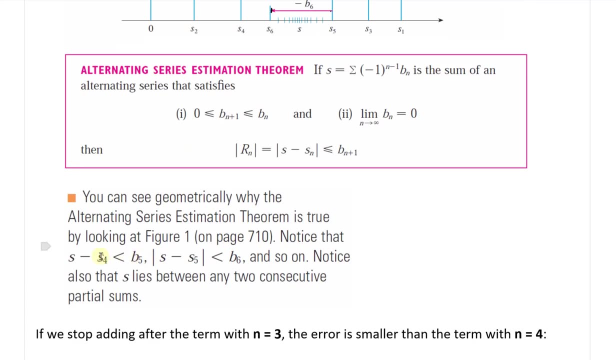 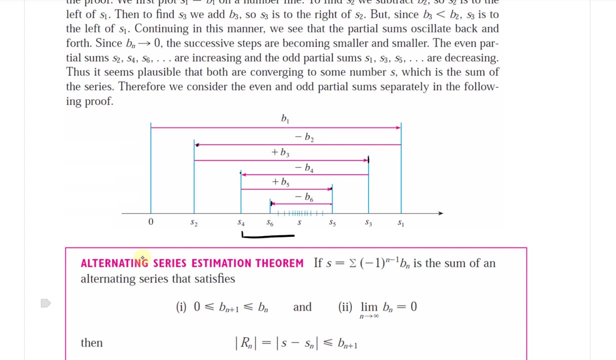 true by looking at figure one. uh, that's this one right here, that's this our figure one here. oh yeah, on page 710. so notice that s minus s4 is less than b5. that is right here. so s minus s4- right here is going to be less than when you add this next one. this is b5 because this crosses it. 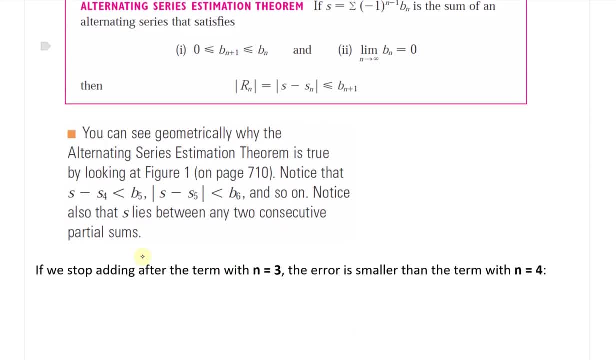 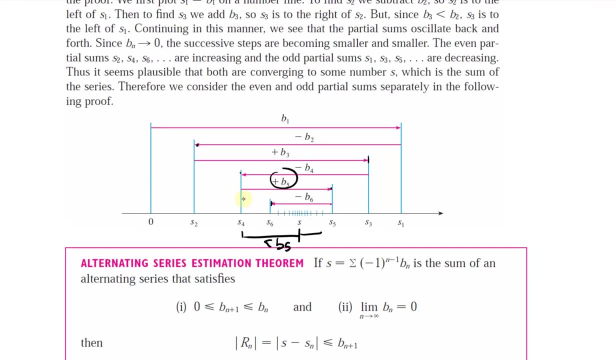 this is less than our b5, right there, and, uh, yeah, notice that also s minus s5 is less than b6. so s minus s5 right here, from here to here, is going to be less than the absolute value, is going to be less than this b6, which crosses our s. so this is going to be, this is. 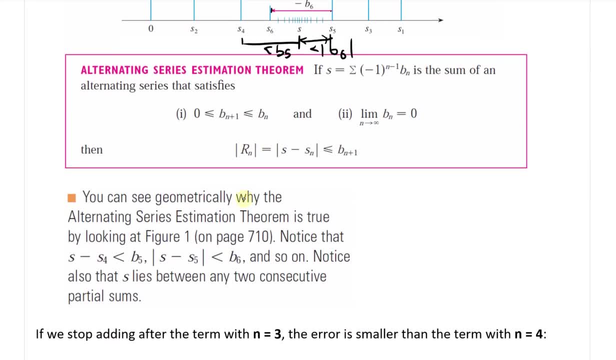 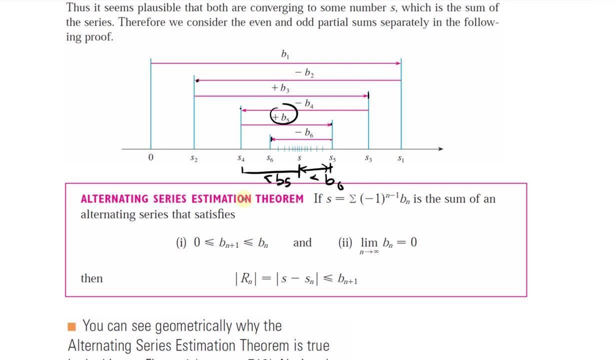 going to be less than absolute value of b6, like that. well, actually, in this case, yeah, we're just looking at b6. yeah, so it's less than b6, ignoring the sign, because these b6 are always positive. the signs take care of the rest. so this difference, right here s minus s5- is going to be less than. 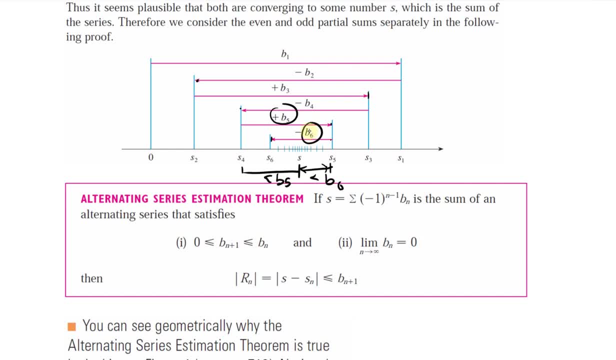 the next term, b6. likewise, if we look at: uh, delete this, so again, watch my earlier video too, where i go over this in depth here, here i'm kind of refreshing for myself. so what we have is a few recall. if we look at this one, s3, if you look the difference between s3 and s4, so s3 and s4, i should know the. 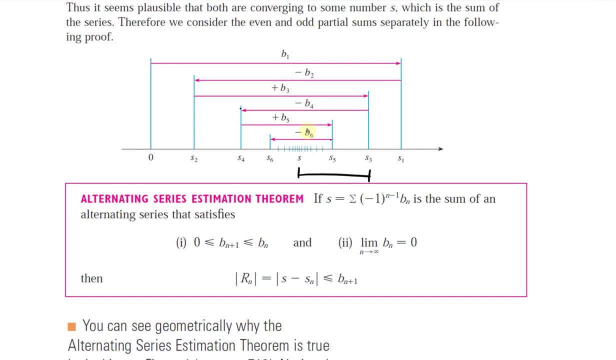 other way around. if we look at the difference from s and s3, this is going to be well less than b4. that's b4 crosses the entire uh s right there. so this is always going to be bigger than b4. so we could use that as our estimation. yeah, so and so on. we can keep doing that. so notice that. 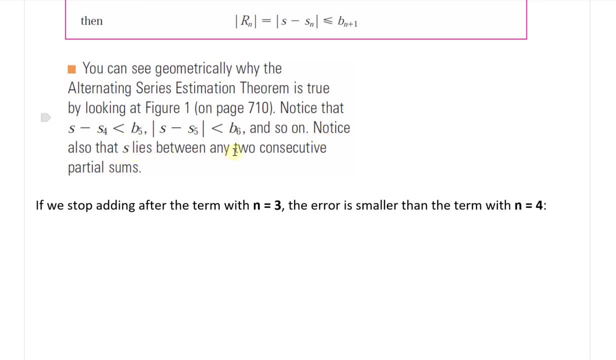 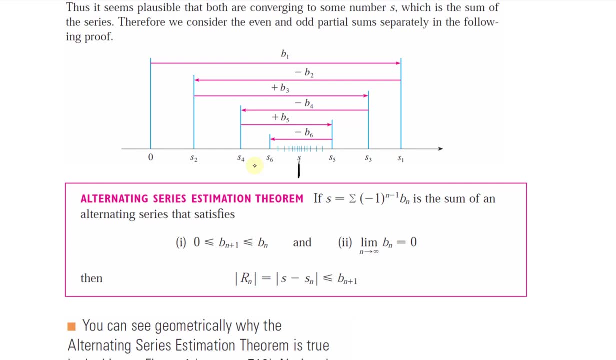 also the notice also that s lies between any two consecutive partial sums. so if you have uh s, if you have s1, then s2 s is in between. so if it's in between, it's it's going to be less than or equal to uh. the actual difference, uh, yeah, the actual difference, which is the term, it's, from b, from s. 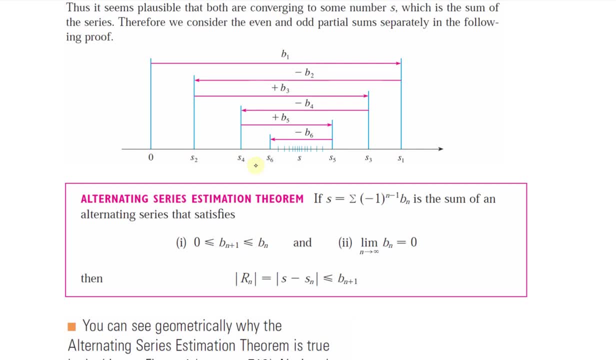 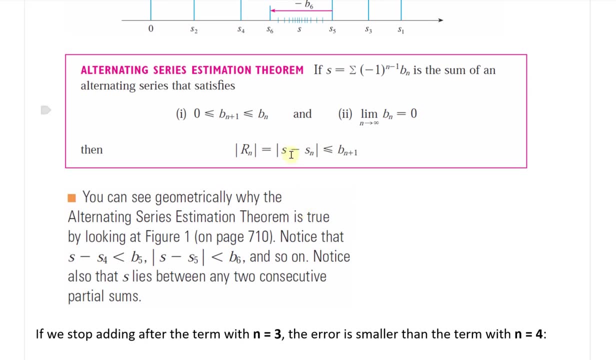 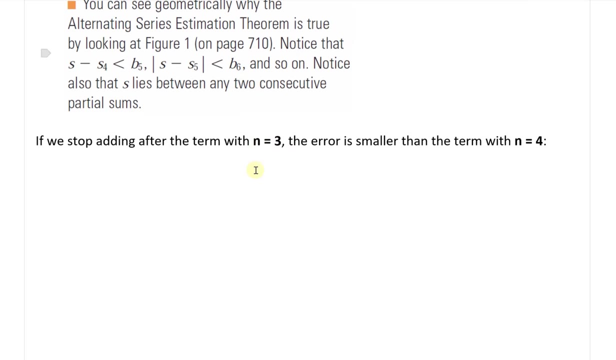 to s2, we would go a full b2, which is going to be greater than that. so so our real difference is going to be less than or equal to, uh, the next term, bn plus one. that's the remainder. so if we stop adding after the term with b through b- the b i mean not b, so after. so if we stop adding after, 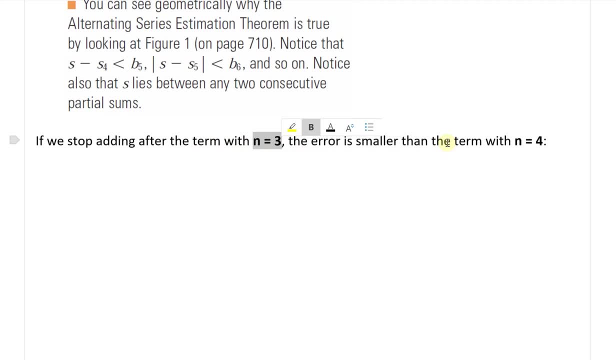 the term with n equals to three. the error is uh, smaller than the term with n equals to four. so let's just calculate this out to see what we have. so this remainder, uh three. this remainder is the error. so let's write this as remainder, remainder, or remainder or error. 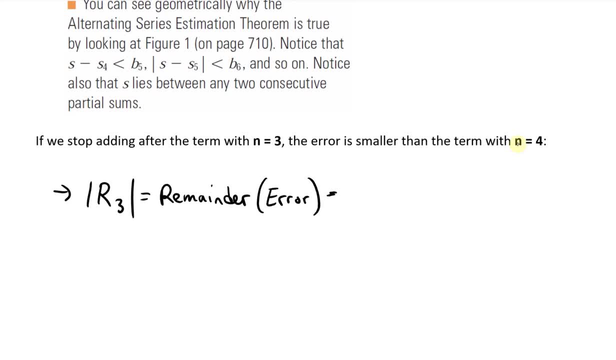 equals two. this is the remainder when we take it all the way to the partial sum. so the remainder is going to be equal to absolute value of s minus the absolute value. i mean, yeah, that's the value of the actual sum. this is uh actual sum which is our uh definite integral, actual, 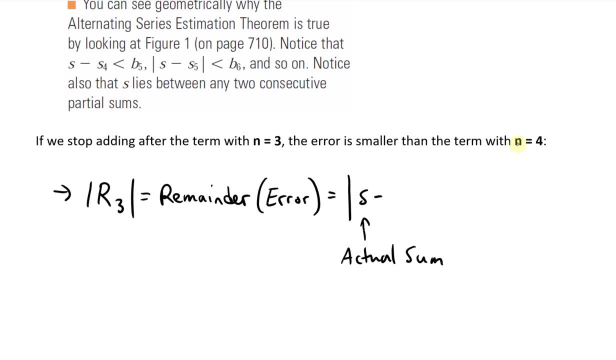 sum, uh. and then, yes, that's actual sum, or the uh- definite integral, definite integral. and then this is s minus our s3, which is our partial sum- uh, the third partial sum. like that, this can be less than, less than or equal to the next term, which is b4. 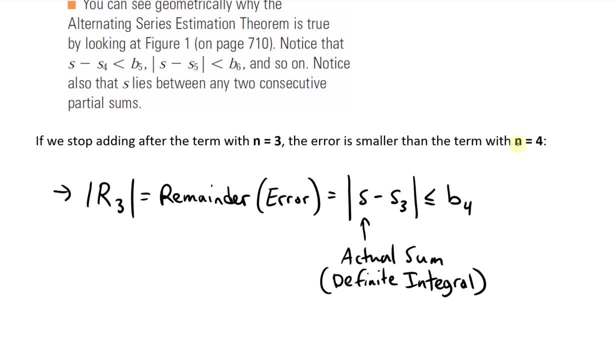 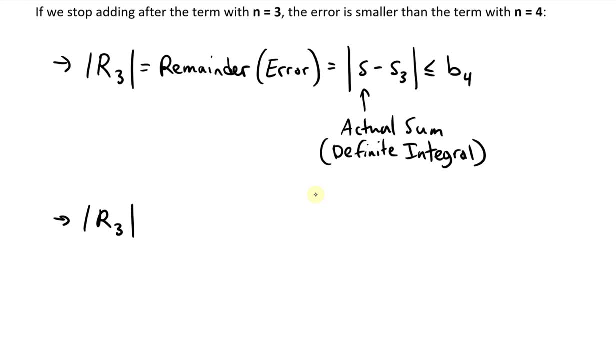 yeah, so that's what we have. is this right here: uh, absolute value of uh r, or the remainder absolute value of the remainder, um r3, like that, or the error is going to be less than or equal to b4, which equals two. yeah, so let's look at our b4. 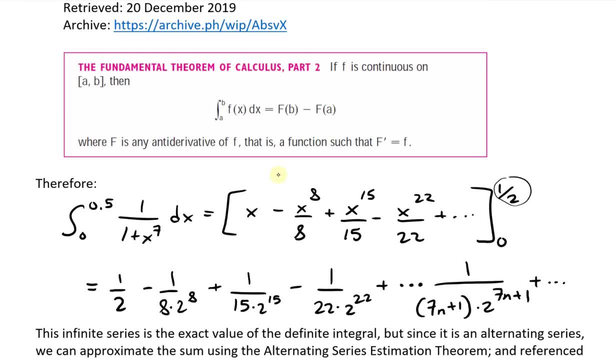 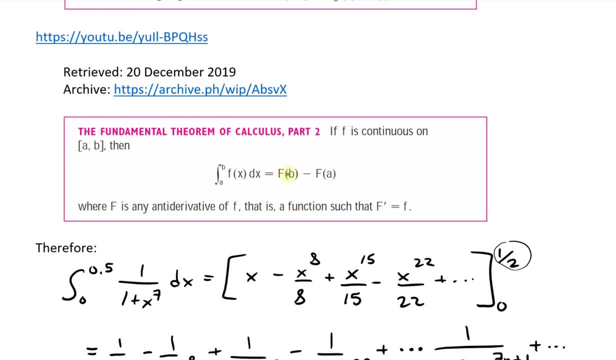 so the b4- because, remember, this is always positive- uh, the alternating, um, yeah, the alternating part of the, the negative signs that take care of the rest. so let's scroll up what we have here. so, therefore, we have this right here now. let's just scroll up. so this one number, this one's a. 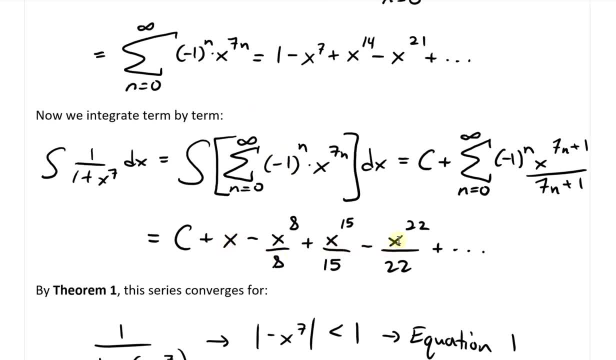 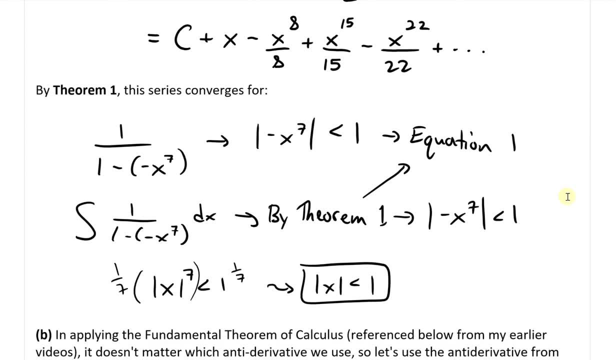 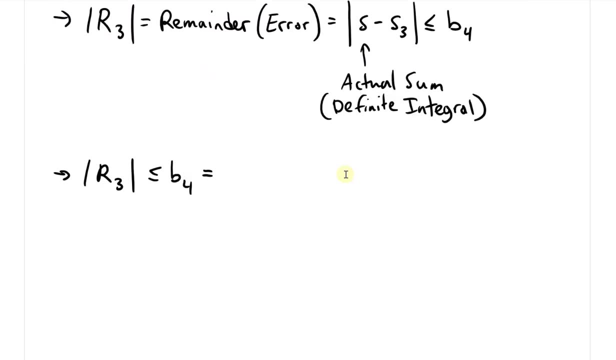 n equals zero, is n equals one, n equals two, n equals three, so the next one is uh. n equals to four, so that's going to be seven times four is 28, and then that plus one is 29, so this is the 29th one. so, yes, this is uh, so this. we have to go one more of this, so that's going to be. so this equals: 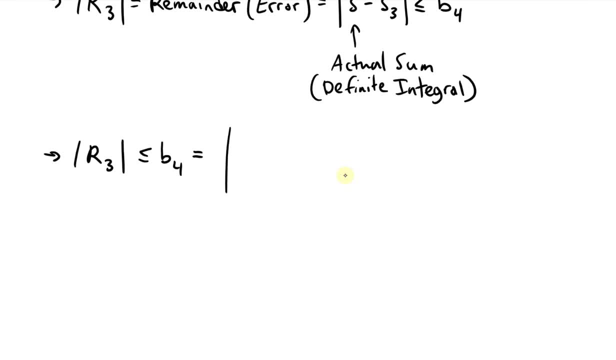 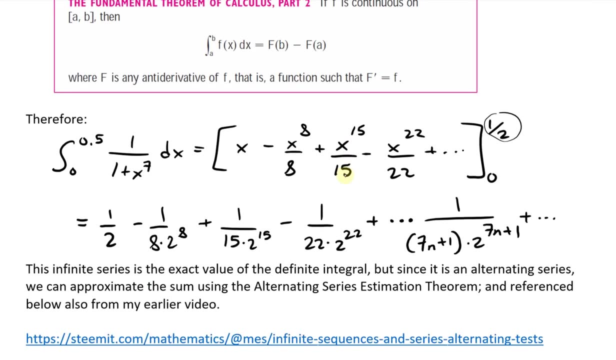 to: yeah, this equals to the absolute value of. actually, we don't need to write absolute value, we could just remove this. uh, we're only looking at bn, so that's going to be. yeah, this right here. one divided by seven n plus one. yeah, times, uh two n uh two. the power of seven n plus one. or else scroll up here: 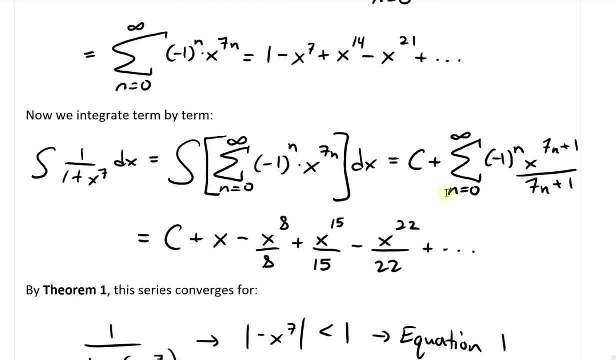 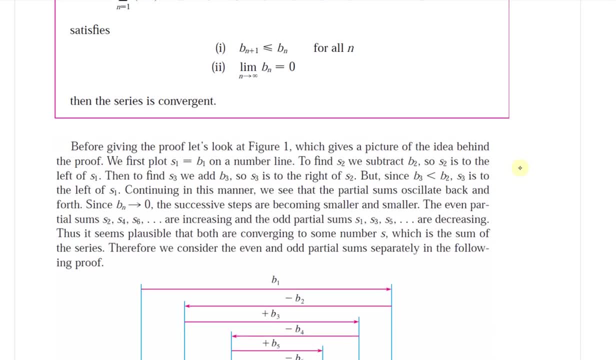 so we have this right here. um, yeah, we have this, but yeah, but yeah, remember, x equals to one half, so let's just look at this one right here. let's look at our definite integral. so we just plug this one inside with: n equals to four. so, yes, i was a bit overthinking, so this is going to be. 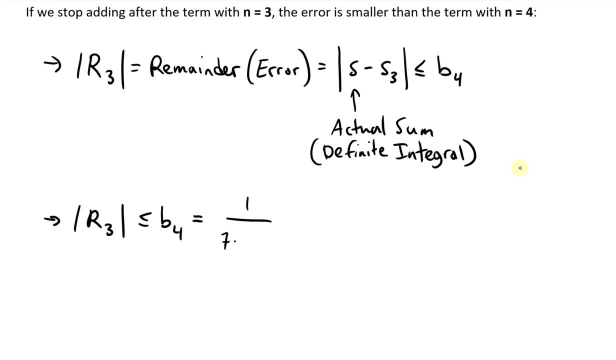 equal to one over uh, seven times four plus one, and then the set seven times four times two, and then this can be two to the yeah multiplied by uh to two of. so when i put an xğini to thext and this can be two to the yeah multiplied by two to the. 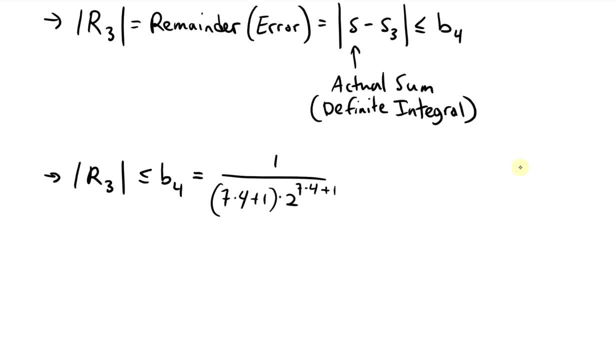 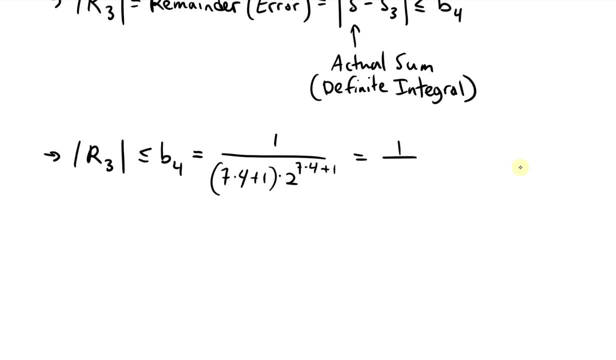 yeah, two to the power of of 29. yeah, or seven times four times seven times four plus one, where this equals to: so, seven times four is 28 plus one is 29.. so we got one over, um, yeah, one over, uh, 29 times by two to the 29.. 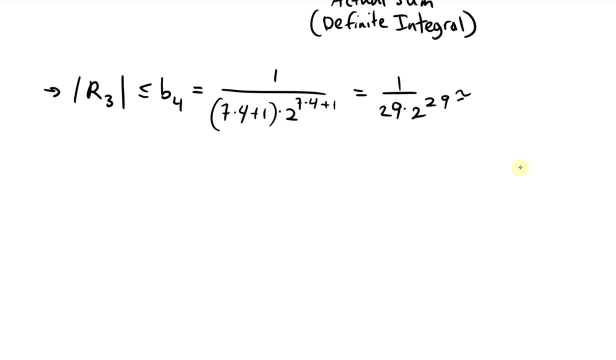 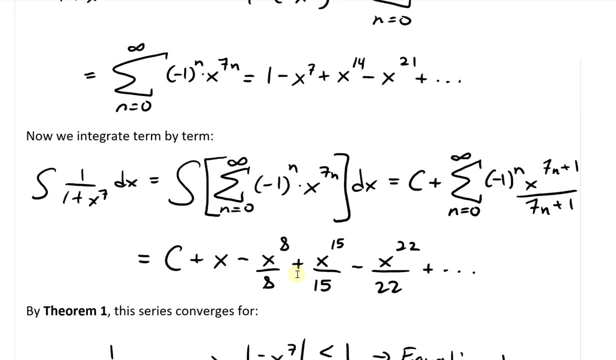 equals two. if you plug this in a calculator, this is in fact equal to roughly 6.4, as my calculus book has times 10, power of negative 11.. and we were asked: let's scroll up what we were asked to do. so that that is the error. and here we were asked to solve it. for let's scroll with: uh, yeah, so. 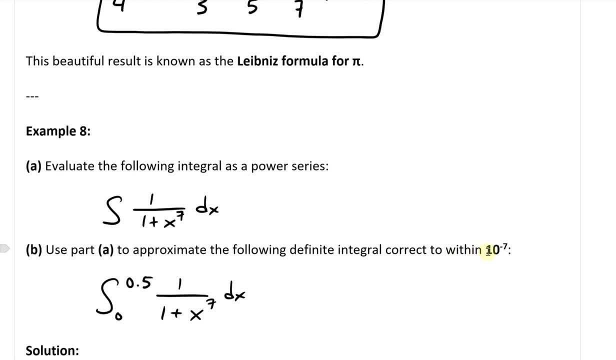 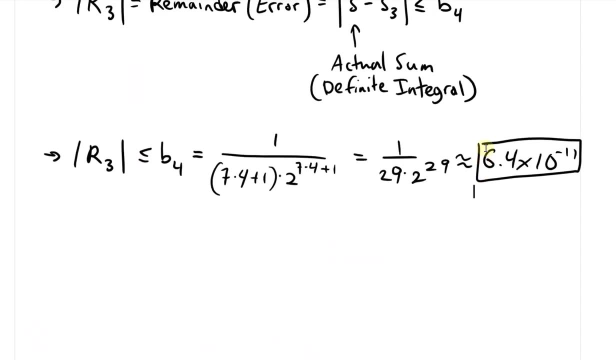 approximate to uh to within 10 to the negative 7.. so this one is: uh is smaller than 10 to the negative 7.. so we've got that part right here and this right here is that's correct. this is less than uh 10 to the negative uh seven. yeah, so we're going all the way to the uh negative 11.. and uh. 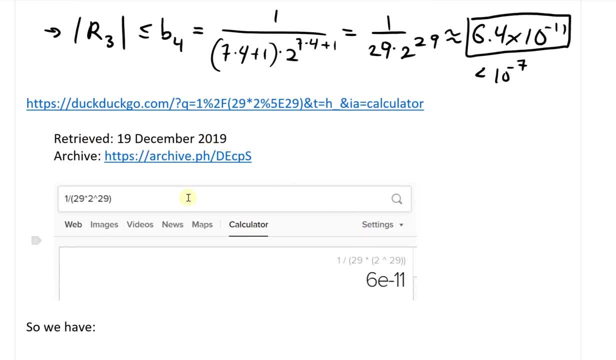 here. i just did a calculation check uh, just use dot dot, go here. so if you go, one divided by uh, 29 uh times uh, or you know, bracket, 29 times uh times two to the power of 29, we get 6 e negative 11, or 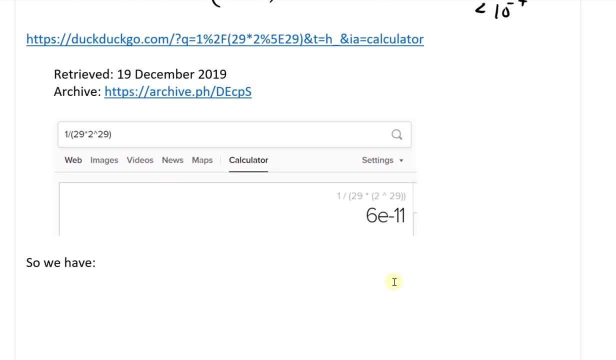 6 times 10 to the power of. uh, negative 11 is the notation for it. so yeah, this is a little bit more complicated, but it's a little bit more complicated, but it's a little bit more. this one doesn't have the 0.4, but i assume that's right. so this is the same ballpark. so negative 11. 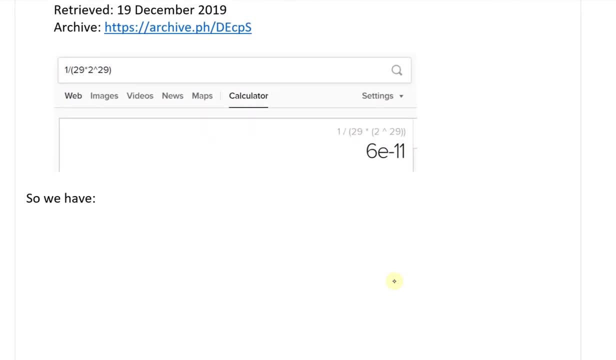 there's a negative 11, there's a six, so i assume this is right as well. so, uh, so we have. what we have now is the actual, uh, the actual definite integral. so the integral from 0 to 0.5 of 1 over, plus x to the 7 and dx, this is going to be equal to, roughly. let's just add up the first four terms. 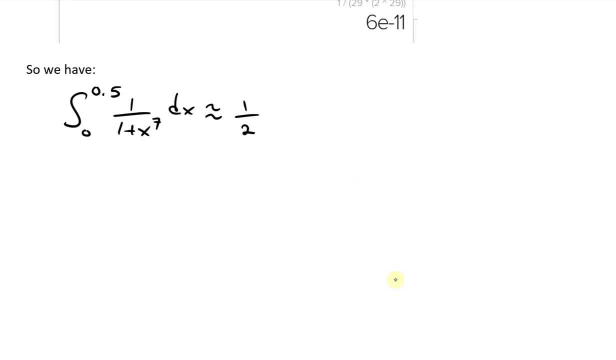 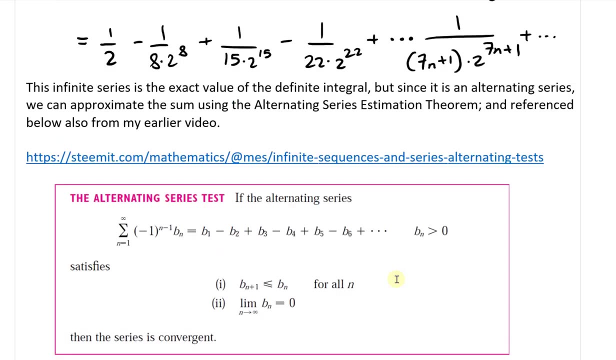 i mean first, uh three terms or uh, yeah, actually first four terms, when we include this, starting off at zero. so this is n equals zero, so this can be negative. uh, yeah, this can be 1 over 2.. scroll up here: so 1 over 2 minus uh, 8 times 2, 8 and 15 and 22 and uh, then we know what our error is. 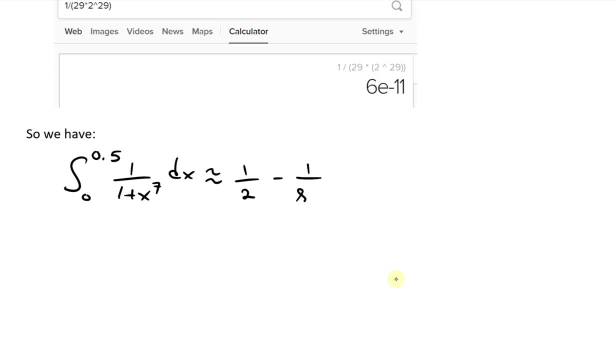 so it's going to be minus 1 over 8 times 2 to the 8, plus 1 over 15 times 2 to the 15, then minus 1 over 22 times 2 to the 22. and now this right here, this right here, if you plug in the. 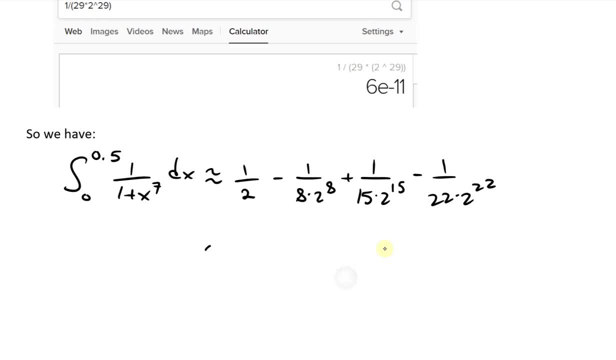 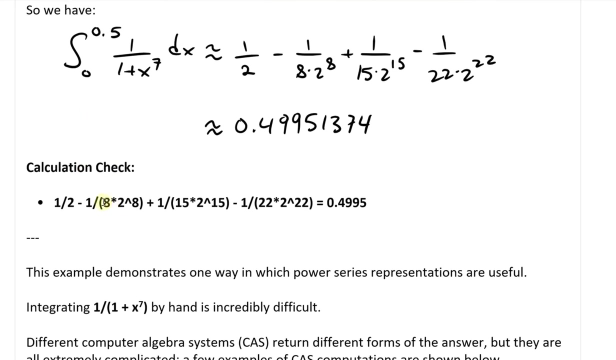 calculator. this equals to uh. this equals to roughly approximately uh point four, nine, nine, uh, five, one, three, seven, four and uh. now do a quick calculation. check: you just use my one node built in uh calculator. right here you just go: one divided by two minus one divided by eight. 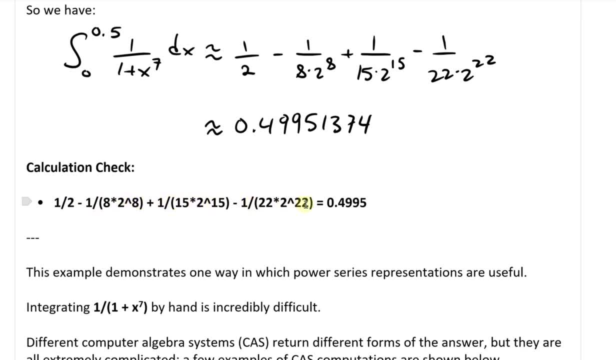 times two to the power of eight, and this is uh, so on all the way to the. this last term right here, the 22 term, so equals two. let's just uh delete this and calculate again. so just press equal and press space and automatically calculates, which is quite amazing. so 0.4995. so yes, i assume the rest is right. this is from. 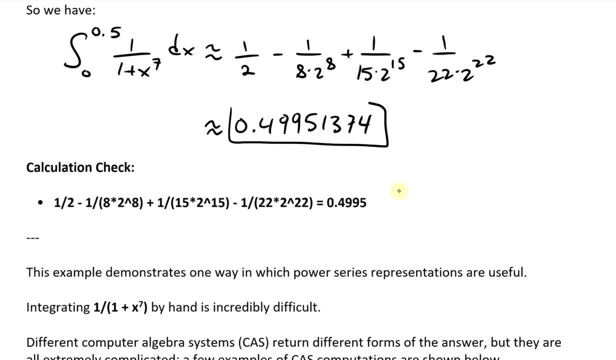 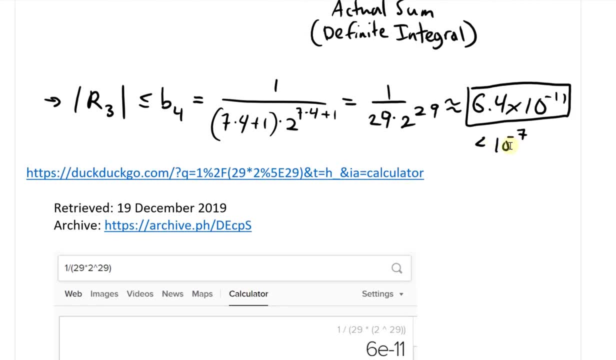 my calculus book and so, yes, very, very epic stuff. i'm just going to circle this like that. so that is our answer and that is approximate the end, that is, within the margin of error that we were asked to solve that which was 10 to the negative 7, and we got it accurate to within 6.4 times. 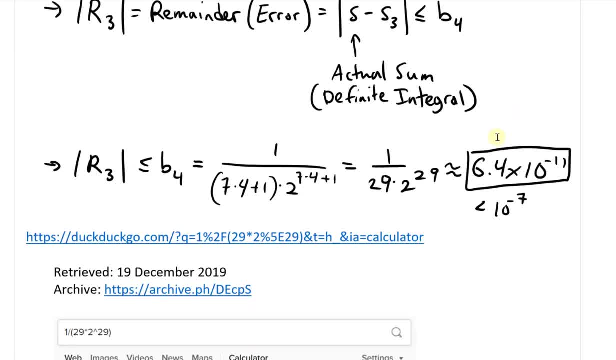 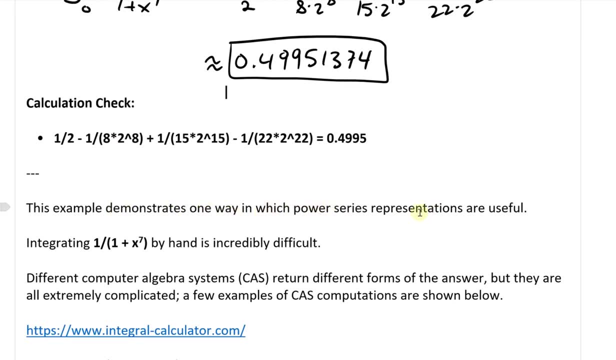 10 to the negative 11.. so, yes, fascinating stuff. so yeah, so yeah, that's pretty, uh, a epic stuff. so now let's keep going further. so, uh, this example demonstrates one way in which power series representations are useful. integrating one divided by one plus uh, x to the seven by hand is 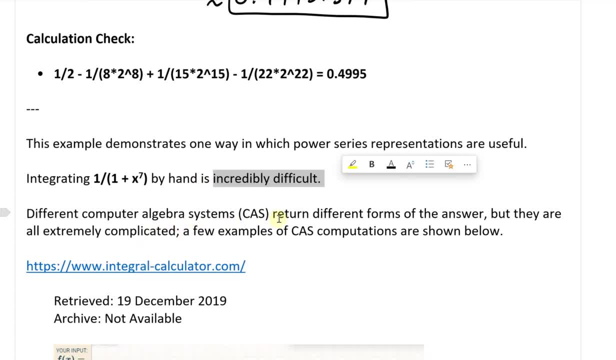 incredibly difficult. uh, different computer algebra systems, uh, or cast, uh return different forms of the answer, but they are all extremely complicated, since if you're integrating this actually by hand, it's actually pretty ridiculous. i didn't know this, was this called this complicated? so if you a few 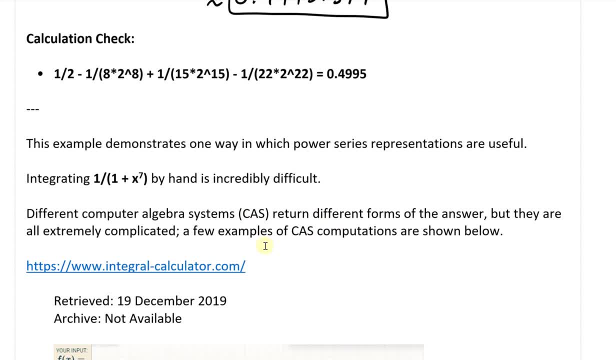 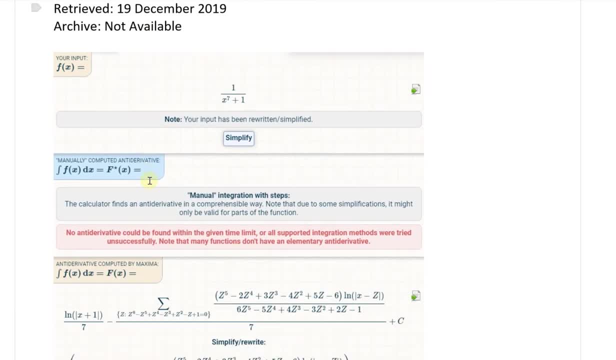 examples of uh cast computations are shown below. so the integral calculator. so this form seems to forward. this is one divided by one plus x to the seven. but if you wanted to find the definite integral of this uh, this uh, using this integral calculatorcom, that's a pretty uh epic calculator. 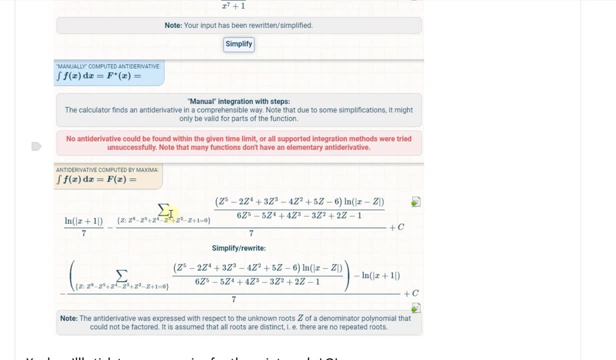 so it gets this, this formula here. so we got summation. you got a bunch of zeds, uh zed six minus uh set five, etc. the anti-derivative was expressed to the unknown root set of a denominator polynomial that could not be factored and assume that all roots are distinct either are no repeated. 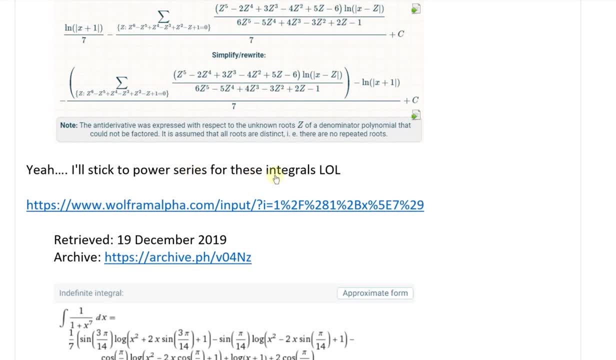 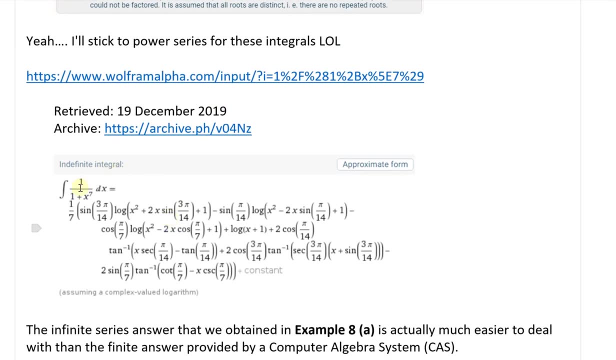 roots. so we get this giant uh integral. yeah, i'll stick the power series for these uh integrals lol. and here if you use wolfram, alpha uses a bunch of logs and signs. so integral of one over one plus x to the seven equals to one divided by seven times sine. three pi over fourteen, log x squared plus two x sine. 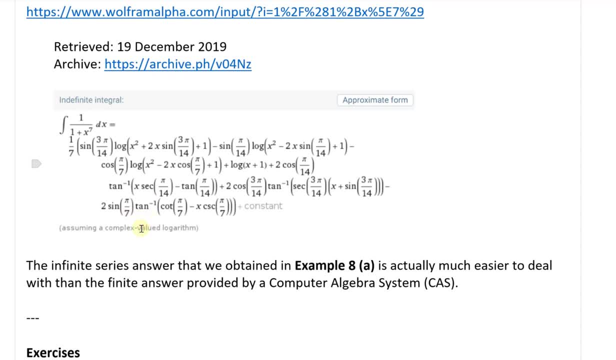 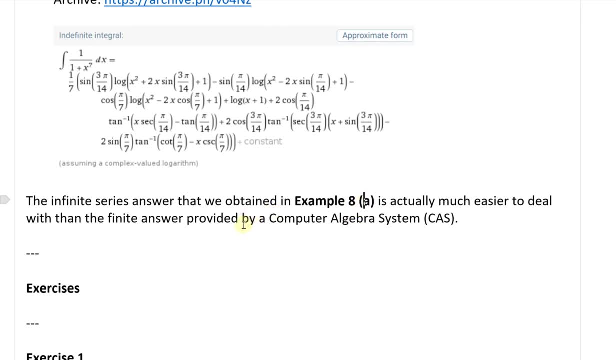 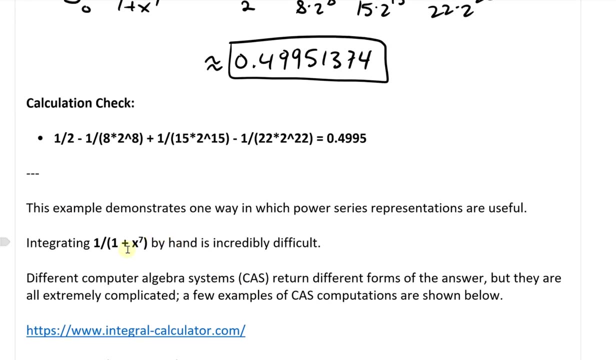 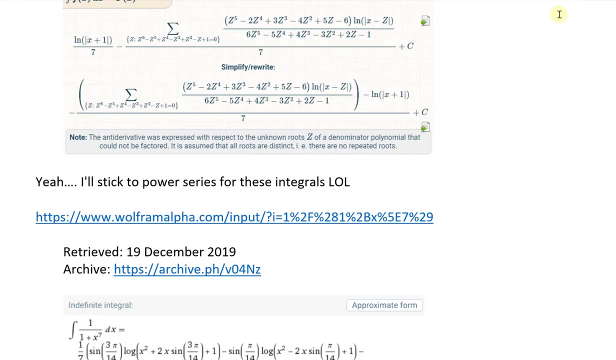 etc. keeps going on and on. so that's absolutely ridiculous. so the the infinite series answer that we obtained in example uh 8a is actually much easier to deal with than the finite answer, because the infinite know how to do it well. what it's very interesting and very important. 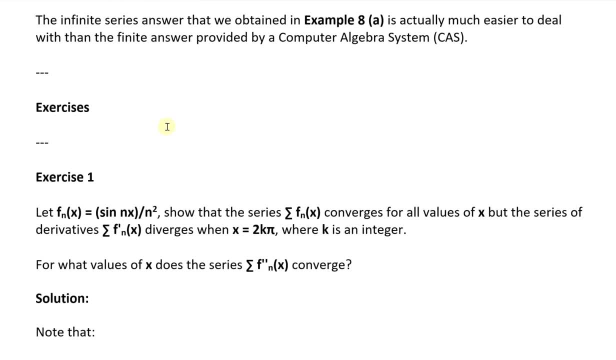 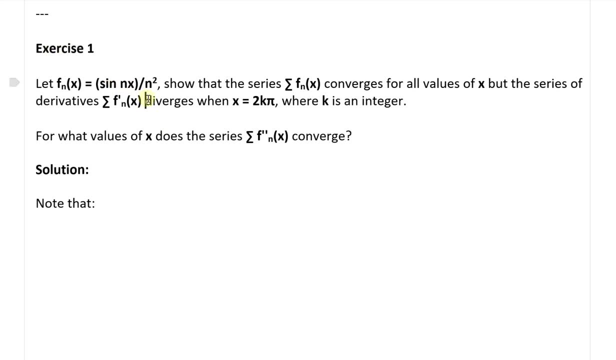 so, by the way, uh, this guy lines up in here like this Tackle extremely well, uh, okay, now we don't see it. you don't see it here. you'll see reести jean's Graylin kahn. that's positive. nothing to allow it to work, so why don't? uh, let's find out more about it. 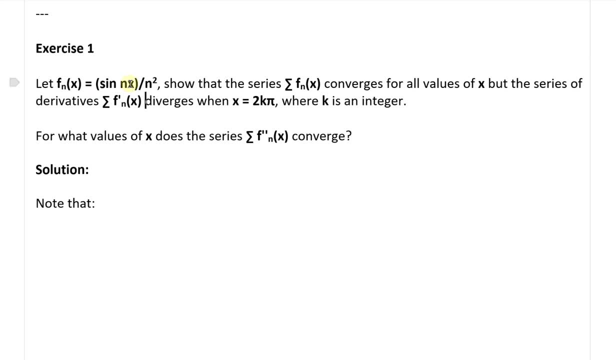 fn of x equal to sine of n of x, I mean sine of nx divided by n squared. and we're asked to show that the series, the summation of fn of x, converges for all values of x, but the series of derivatives, summation of f, prime, n of x, diverges when x equals to 2k pi, where k is an. 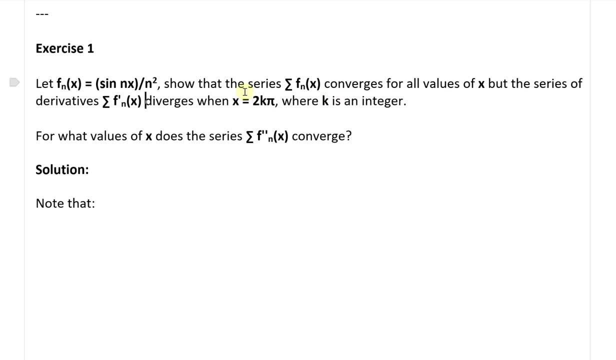 integer. and this is to show that theorem one is not necessarily applicable to other power series. I mean other series where this one is a trigonomic series, right here. and in theorem one states that for power series that the derivative has the same radius of convergence. but in this 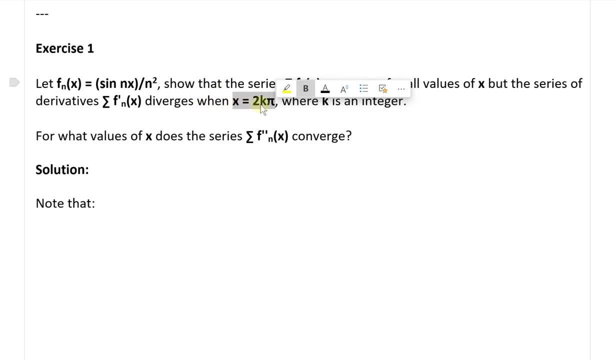 case. here we're going to have it diverge for these values. in other words, the radius of convergence is not going to be the same as the function itself, since this converges for all values of x. in other words, radius of convergence is infinity. Yeah, so thus for non-power series. 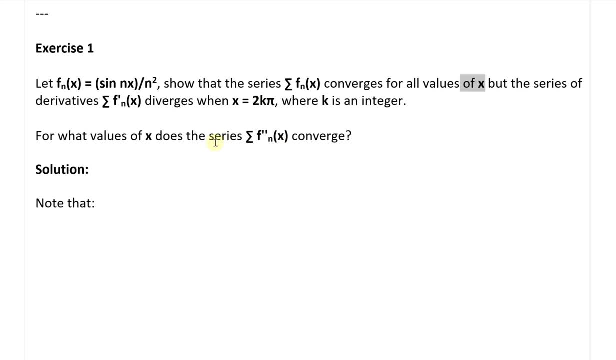 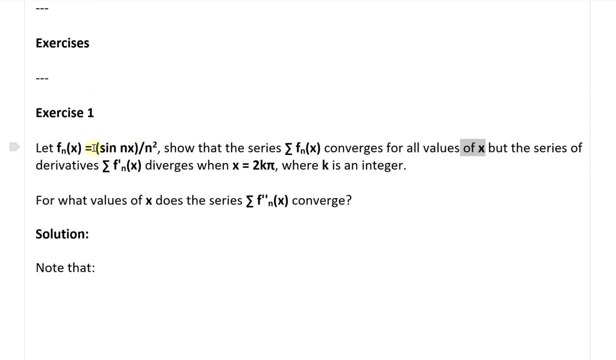 we have to check where it converges, specifically For the derivatives and integrals and so on. So let's look at the solution. So note that. let's look at this right here we have sine n of x divided by n squared, and when we're dealing 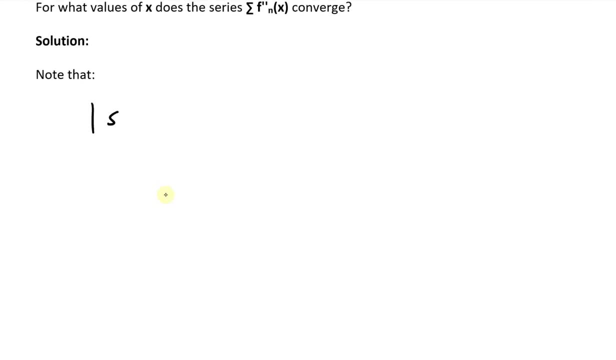 with sine, or it's a trigonomic function. if we take the absolute value of it, absolute value of sine, n, of x, like here, over n squared, this is going to be well less than or equal to 1 over. 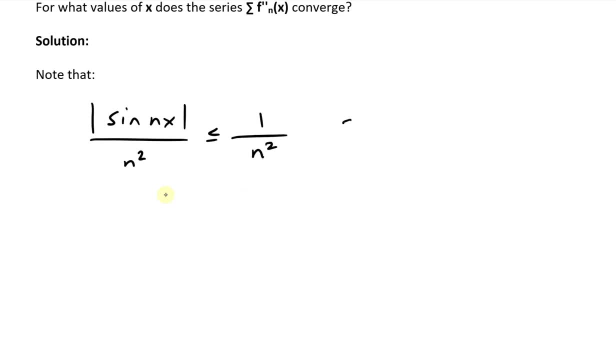 n squared. and that's because, yeah, that's because, right here, since when we're dealing with trig functions, this is, this sine is going to be well, less than or equal to 1 over n squared. this is just going to be oscillating from maximum 1 to minimum negative 1, so it's always going to be. 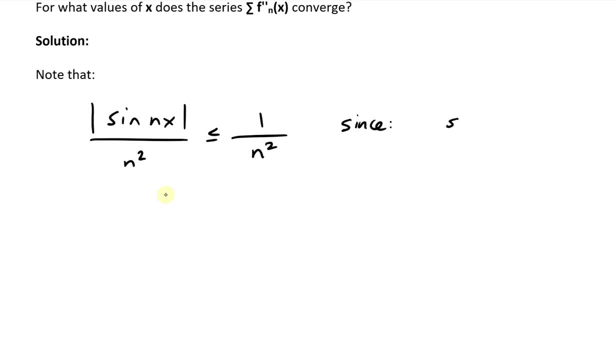 between absolute value of 1.. So, in other words, I'll write here a sine theta just to distinguish from this x there and this n in front there. so we're going to write this as so: sine theta is equal to, is less than or equal to 1, and greater than or equal to negative 1.. In other words, 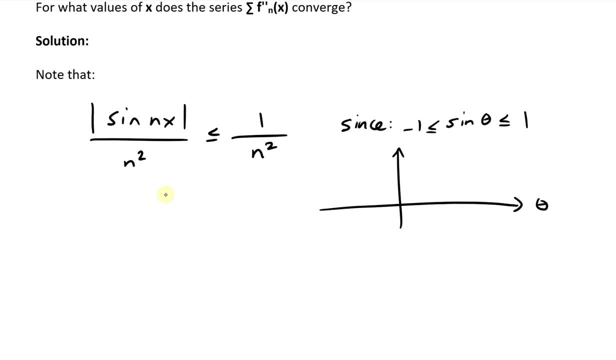 if you were to graph this out, this is going to be theta sine theta, like that. it's going to look something like this, and so on. It's going to keep going on and on. where the yeah, the maximum here is 1, and the minimum is: 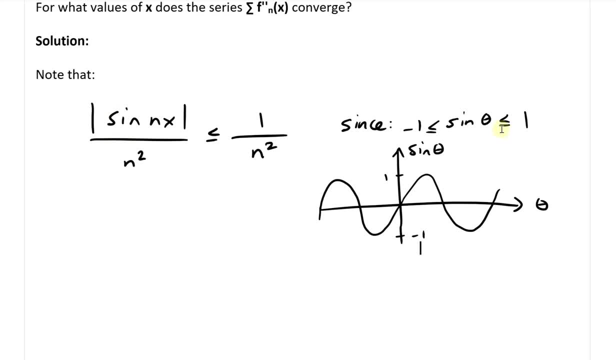 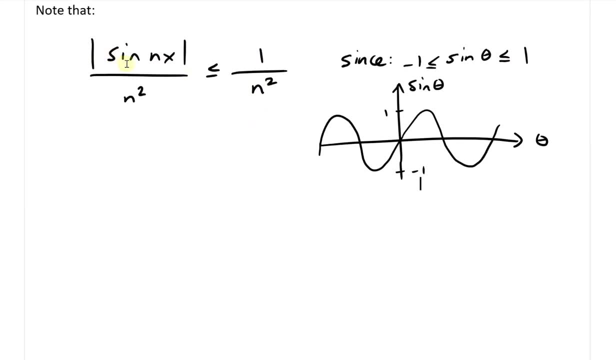 going to be negative 1.. So it just oscillates back and forth. so then we can now cap it at between: or. the absolute value is going to be well less than or equal to 1 there. So in other words, this function right here, sine n of x, divided by n squared, is going to be less than. 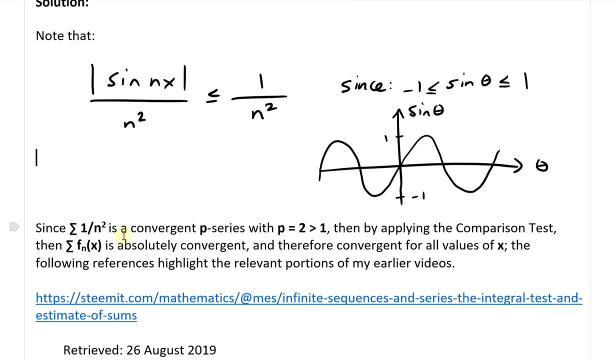 or equal to 1 over n squared. Yeah, so now going further. so, since if we take the series of this one- 1 over n squared- this is just a convergent p-series with p equals to 2, which is greater than. 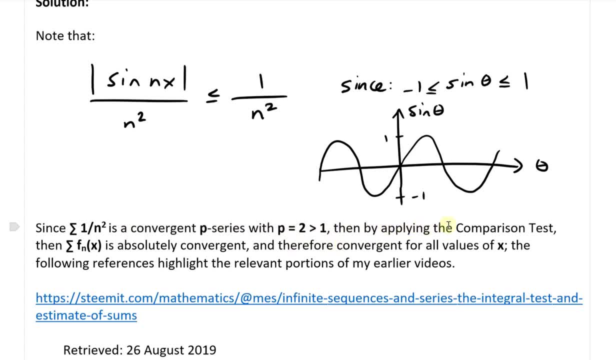 1, and I'll show the link to it first. I mean in a bit. So then, by applying the comparison test, then the summation of fn of x is absolutely convergent, because this is the absolute value, and therefore convergent for all values of x. The following references highlight the relevant: 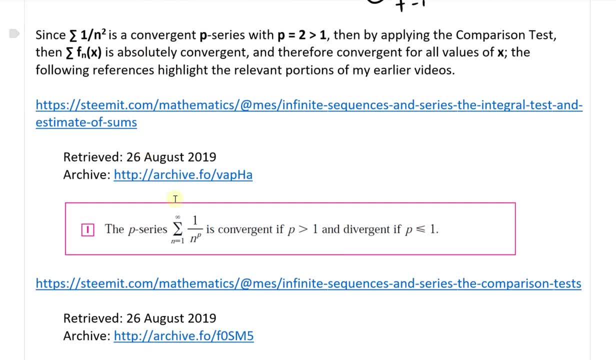 portions of my earlier videos for statements I just made there. So the p-series right here. I recall from my earlier video that if you have n equals 1 to infinity of 1 over np, this is convergent if p is greater than 1, and divergent if p is less than or equal to 1.. So in our case, 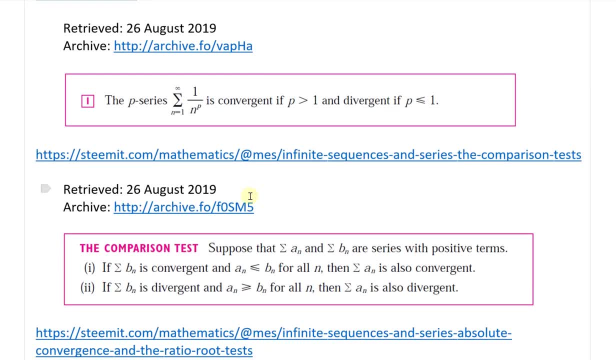 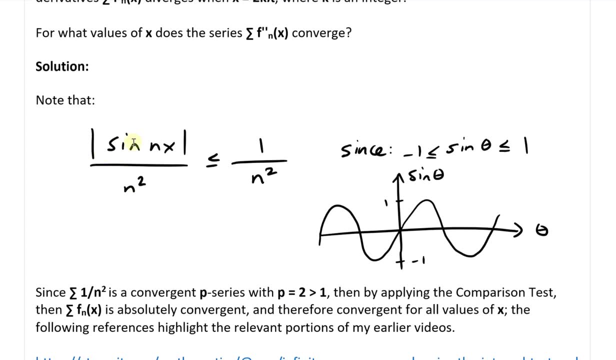 p equals 2,, which is greater than 1.. So it's going to be convergent. And then using the comparison test, so suppose that the summation an and summation bn are series of positive terms. and here we're going to: yeah, this is all positive terms, right. here we're going to. 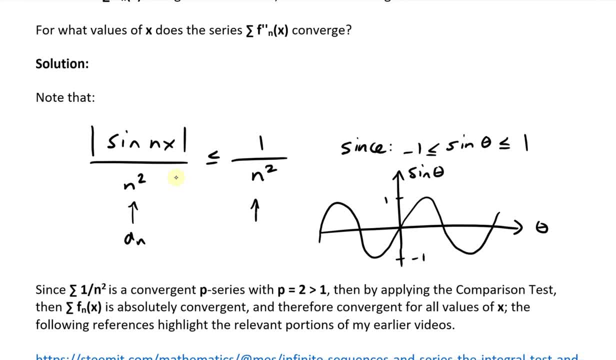 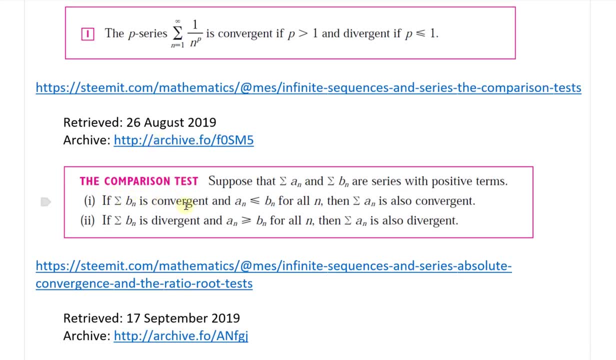 consider this as our an. this is going to be our bn, like that, so we're taking the absolute value of it. So if the summation bn is convergent to the series and an is less than or equal to 4,. 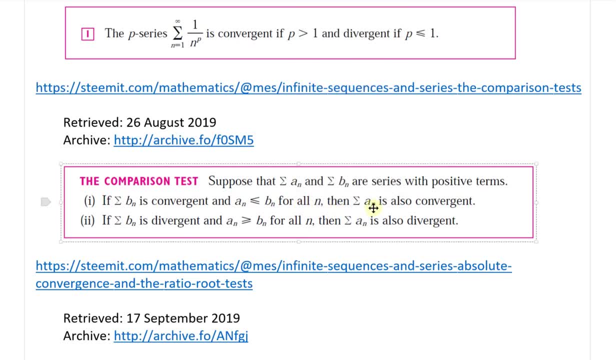 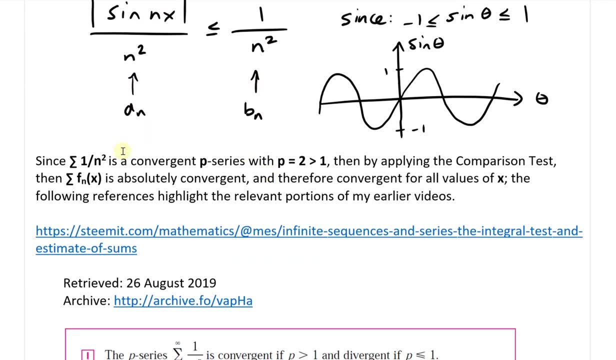 less than or equal to bn for all n. then we have the summation: an is also convergent. So that's the part a of it, And this one is going to be less. this is: an is always less than or equal to bn, And this summation of bn is convergent. p-series. 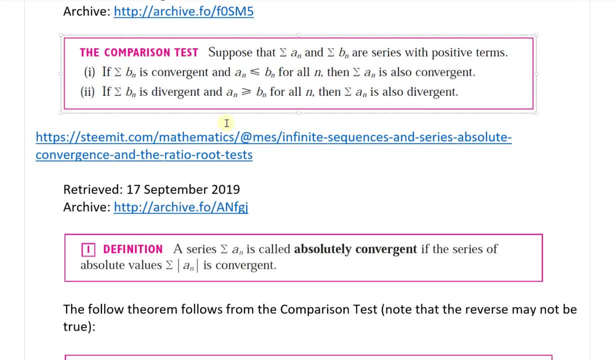 thus fn of x. this right here is going to be convergent, So the absolute value of it, And also likewise I recall that the opposite is also true. So if the summation of bn is divergent and an is greater than or equal to bn for all n, then the summation an is up as. 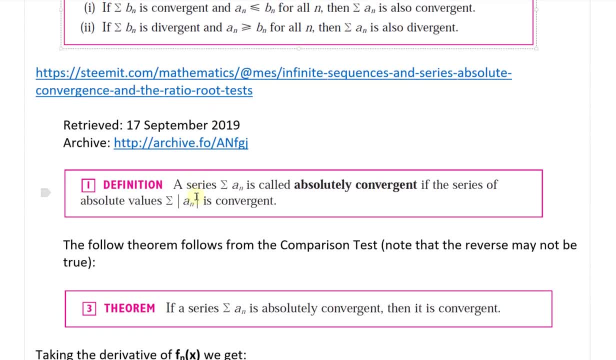 also divergent And also going further here, since we did a absolute value sign, a series summation, an, is called absolutely convergent if the series of absolute values, right here, a summation of absolute value, an, is convergent, And the following theorem: 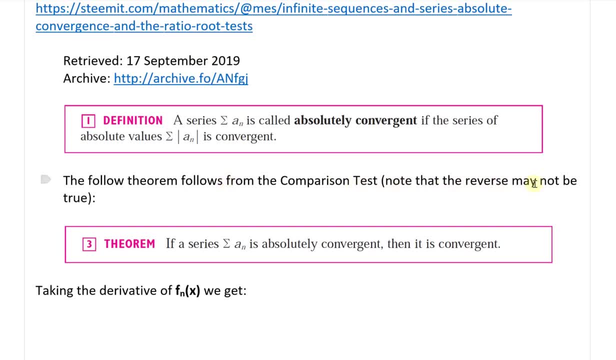 also again, all this from earlier videos follows from the comparison test. know that the reverse may not be true. So here we have: if a is just a comparison test, if a series summation, an, is absolutely convergent, then it is convergent, In other words. so if this is absolutely convergent, 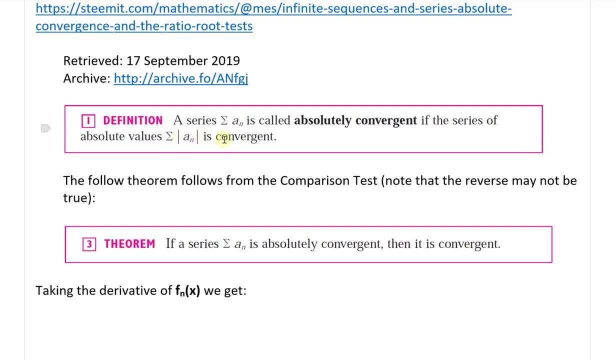 that means this: this summation of this absolute value is convergent. And then this right here: can. it can't be bigger than this. it can. each term. an is going to be either. it's going to be either equal to absolute value of an or less than it. it could be negative and so on, but still. 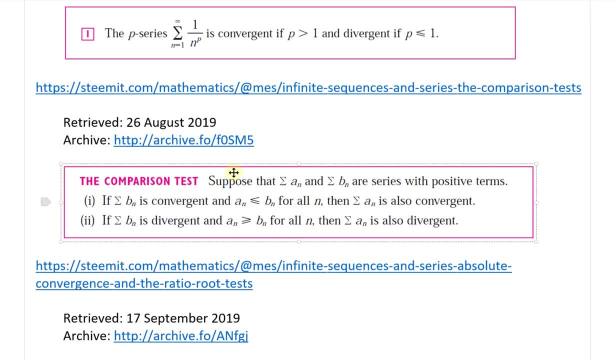 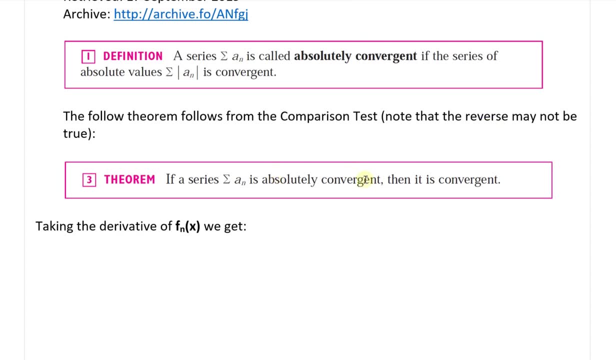 going to be less than it. So apply the, apply this right here, the comparison test, And then we have this. then we have that it's convergent as well. But the reverse may not be true. So if a series convergent, it does not necessarily mean it's absolutely convergent, Because, for example, 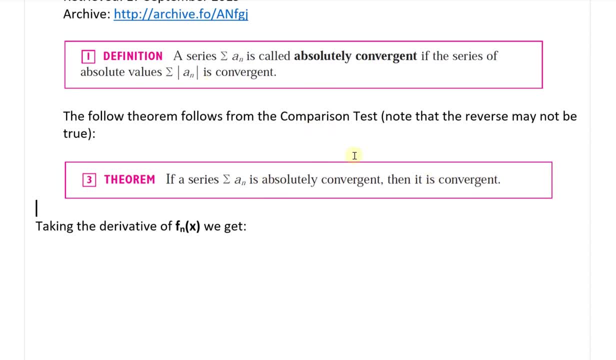 an alternating series, like the alternating harmonic series, it's going to be convergent, but if if you make it all positive is gonna be divergent. So yes, so keep that in mind And I'll, in fact I'll talk about the alternate the wall, just the harmonic series, soon, And that. 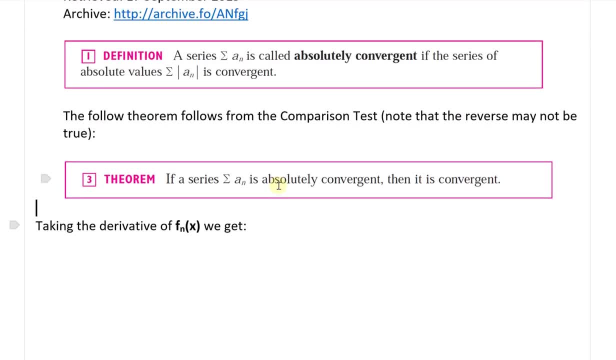 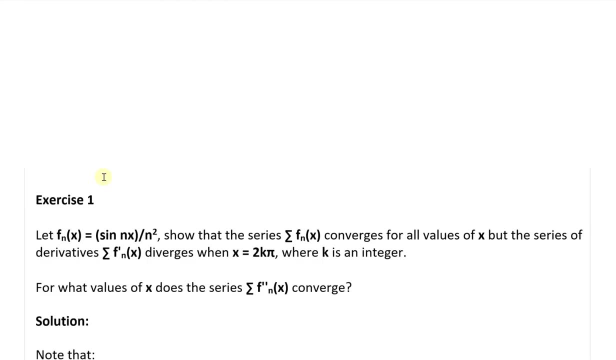 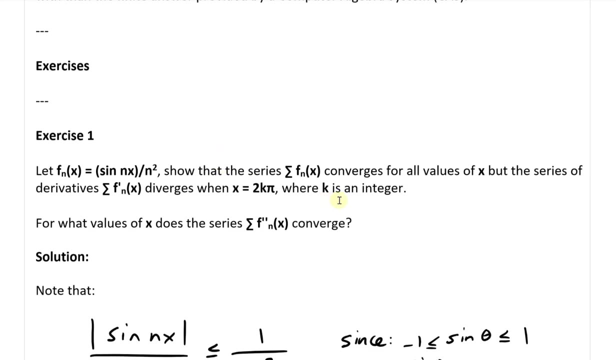 is what it's just a p series with p equals to one and that's going to show that in this derivative. So now that we have, we have showed that this series, the f? n of x is, converges for all x, just using comparison tests. So, for all x converges, let's look at the derivative and show. 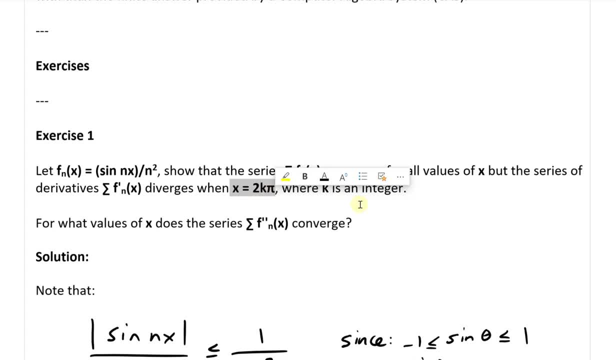 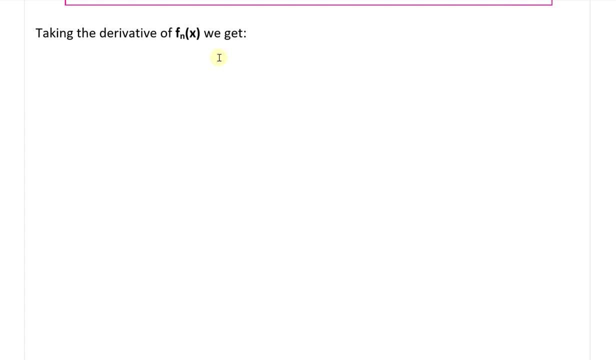 that it diverges for all x. So let's look at the derivative and show that it diverges for all x. this case, right here, x equals a two k pi, where k is an integer. So let's look at that, Alright. so taking the derivative of f and of x, we get so the derivative f n prime of x. 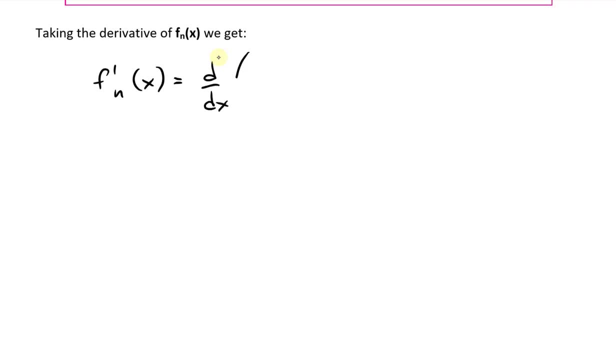 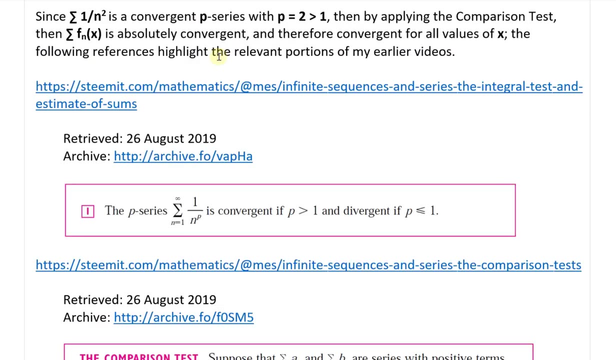 is equal to. this is just going to be D over dx, and let's just plug in our sign and x over N squared. double check, that is what our function is. So, yeah, we have a sine and x over N squared. that's right here, So let's go down. 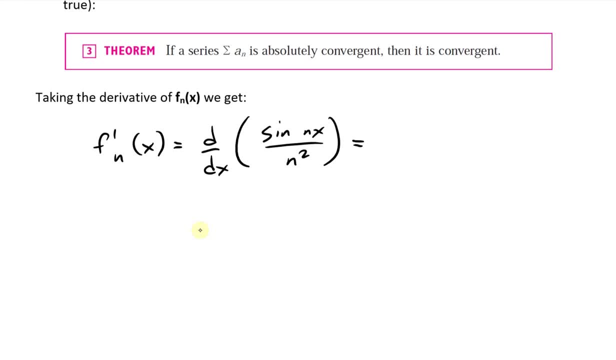 let's take the derivative and recall: the derivative of sine is just going to be cosine, so that's just going to be cosine, n, x. and then, using the, let's divide this by n squared and then chain rule: derivative inside of n. x is going to be n. so this is going to be cancelled. it's going to cancel. 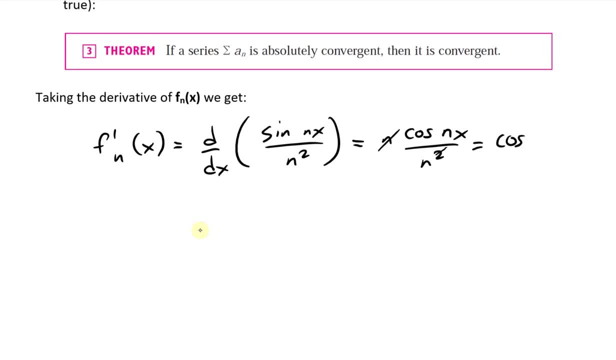 this is going to be equal to cosine, yeah, cosine n of x over n, like that. so that's what this derivative is equal to. yeah, so thus we're asked to show that divergence for this case. so that's, when x equals to 2k pi, where k is an integer, we have- let's just write this down- what we end up. 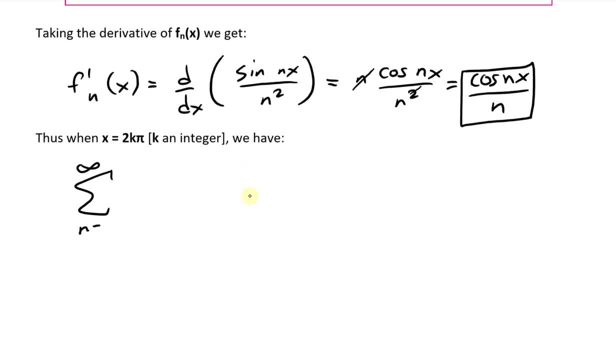 having is the summation: n equals to this, n equals to 1 of f, n of x. yeah, we're putting 1 here, because when you plug in 0 here, you're divided by 0 goes to infinity. so it's undefined. so we'll start from. 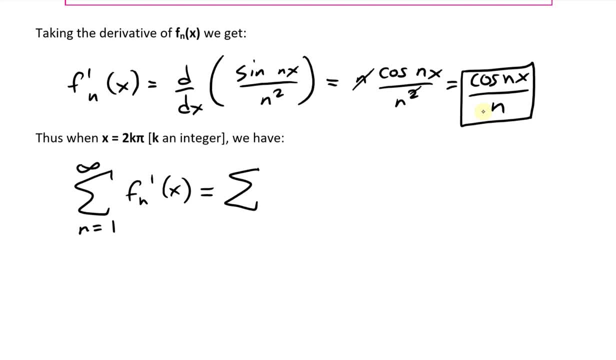 1. this is going to equal to the summation right here of n, equals to 1 of cosine. and now let's just plug in our 2k pi, so we'll have cosine 2, 2. yeah, let's write 2k. you know, let's write your 2k n pi, like that, over n. now notice what happens here, yeah and here. 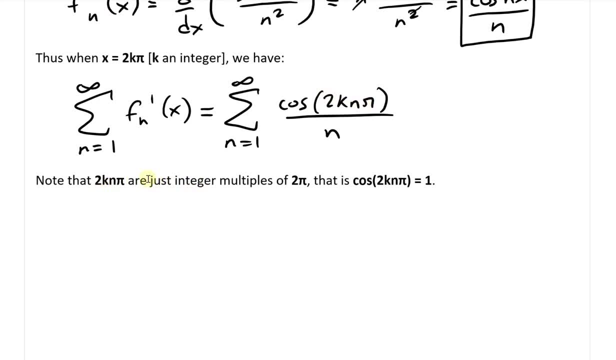 note that 2k and pi are, are just or is just. yeah, i'll just write: are just integer multiples of 2pi, because if this is an integer, this could be a negative and so on. this is: n is integer starting from 1 to infinity. so whenever you multiply anything by 2pi, you're still multiplying it by. 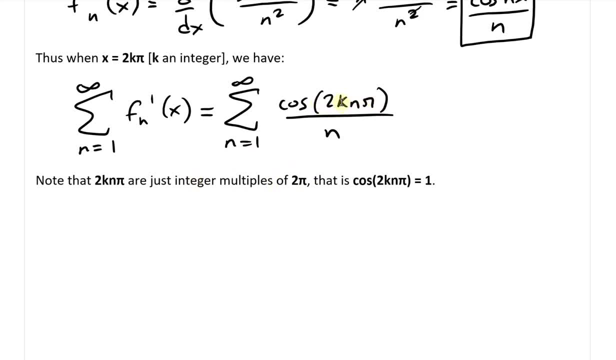 2pi. so then it's just an integer multiple. this is, for example: if k is equal to negative 1 and n is 1, that's just going to be negative 2pi. and this is uh. if n is 2 and k is negative 1, this is going. 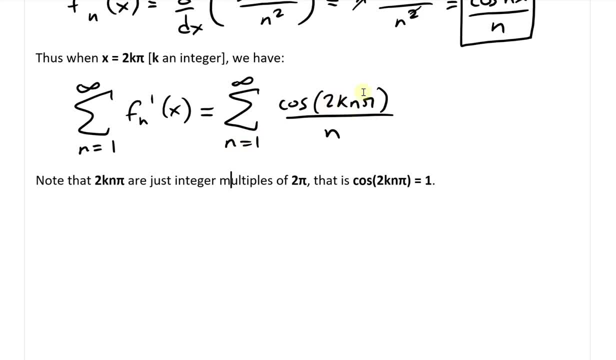 to be negative 2 times 2, that's going to be 4 times uh pi, or in other words, negative 2 times 2 pi, yeah, 2 pi. so in other words, that is cosine 2k n pi equals to 1, and you can see this by just. 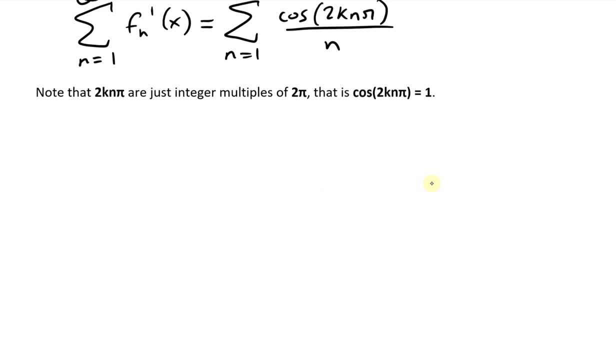 graphing this out. so if you graph this out like this, so again i'll just write theta, just to avoid confusion between the other terms. so we have this: delete this thing. write it like that. it's a cosine theta. this one starts off over here and then goes up like this and keeps going on and on. 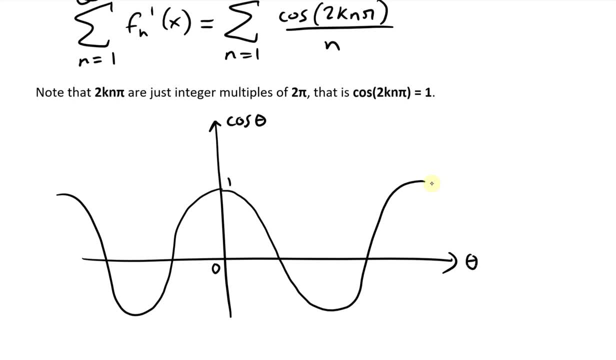 and then where here is a zero, this is going to be a highest value is one, lowest value is going to be at a negative one, and then it's going to become: uh, it's going to equal to one. we're interested when it equals to one, so that's going to be right here. so this is going to be zero. this, this goes all. 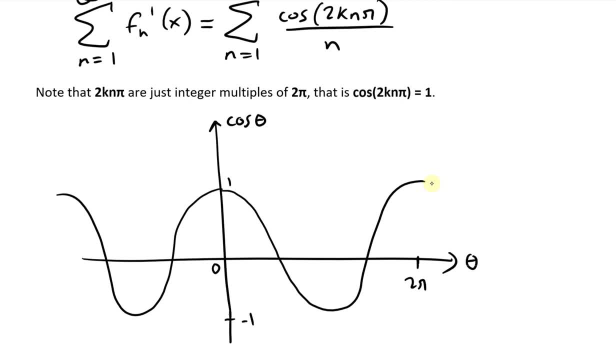 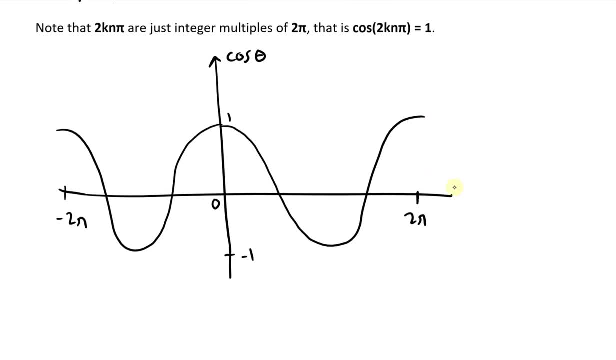 the way to 2pi, like that, and likewise you go backwards one period, this is going to be a two, a negative 2pi, and so on, and this is going to, this is going to repeat itself. and here we can just expand this out further and let's say it goes up like this, and then we're going to have 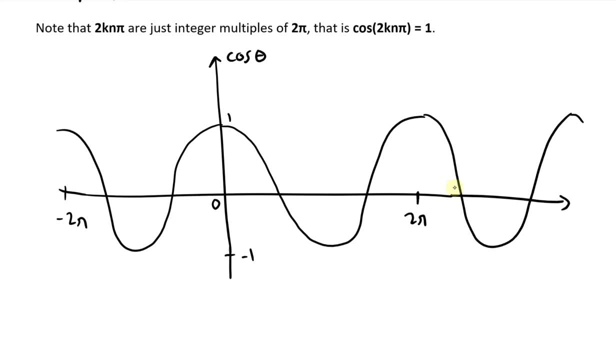 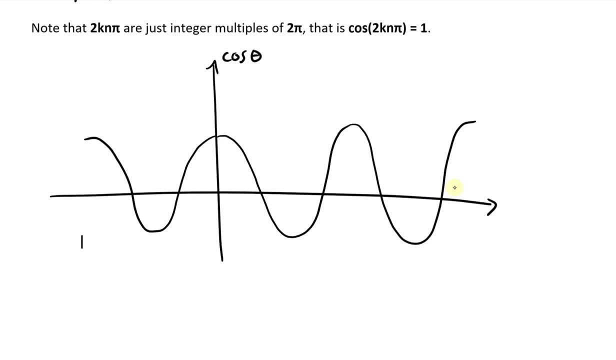 this and it goes back to this 2pi there, so that we have like: here let's keep going even further. this is theta, and here i just got quickly: uh shrunk it, every shrunk everything. we wrote it, so we have zero there. this is going to be at uh 2pi. this highest value is one. lowest value is: 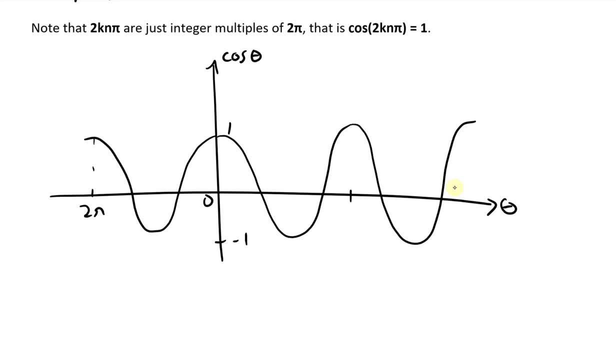 negative one and so on. yeah, and it's not the scale, but anyways, this is going to be 2pi there. here's going to be our 4pi. so at this point, this point, this point and so on, these are all integer multiples of 2pi so we have: this is negative. 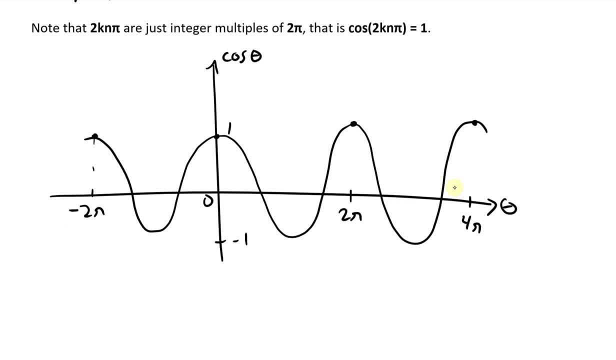 2pi. this is 2pi is 4pi, and so on. yeah, so that's what we have here. is cosine negative 2pi equals to uh. well, just one, which also equals to cosine zero, which equals to uh, cosine 2pi, which equals. 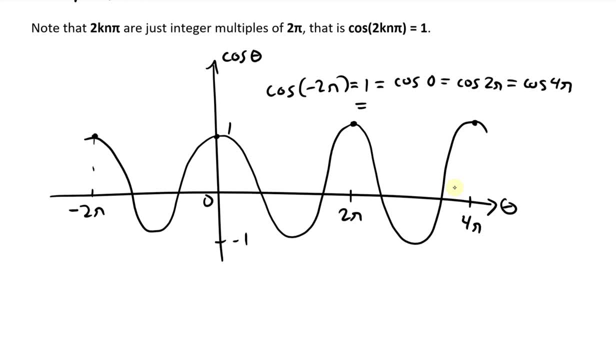 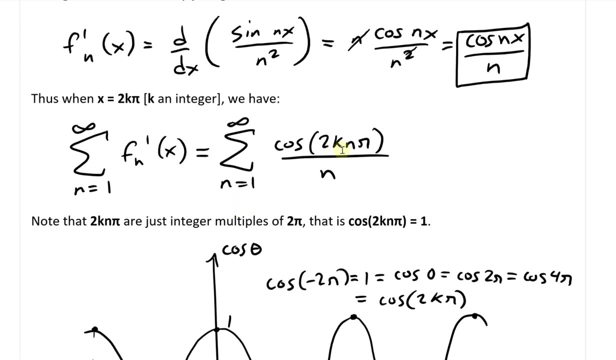 to cosine 4pi. in other words, this just equals to cosine uh, 2k, pi, like that. yeah, where k is an integer. and then if you plug this inside uh, this, uh, this right here, this x value, i mean inside this series, right here, where it has an n there, that increases that. 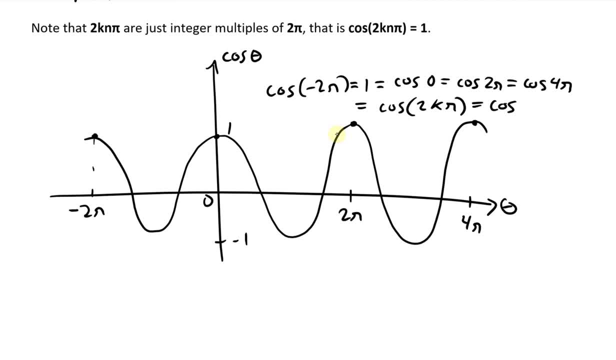 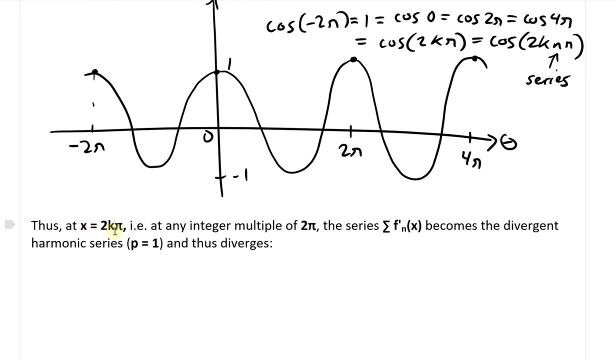 increments, that it's still going to equal to cosine 2k, where n, uh, 2k, n, pi, where this is from the series. so n is the series where it increases, but it's still going to be an integer multiple 2pi. yeah, so thus uh, we could state that uh at x equals 2k pi, uh ie. 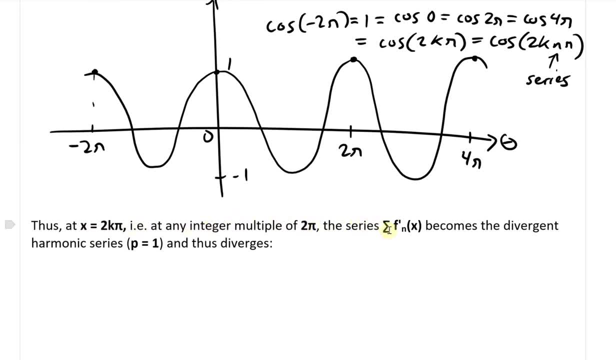 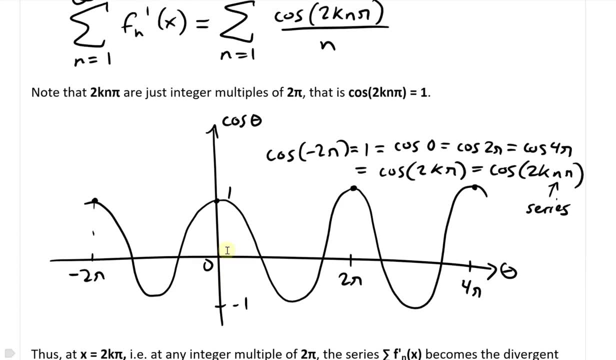 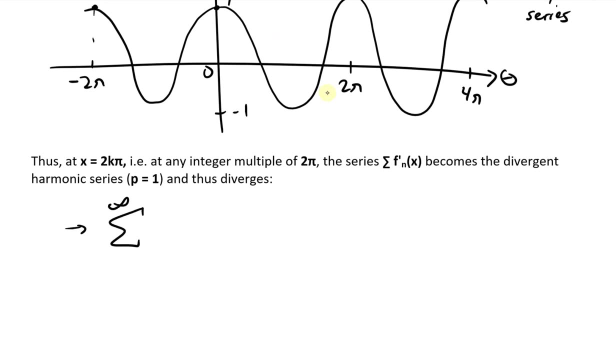 any integer multiple of 2pi, the series uh some, the summation of f, prime, uh of n of x becomes a divergent harmonic series. p equals 1 and thus diverges. in other words, this becomes equals to 1, so we could write this as: uh, the summation uh infinity n equals to 1 of f, n of x. 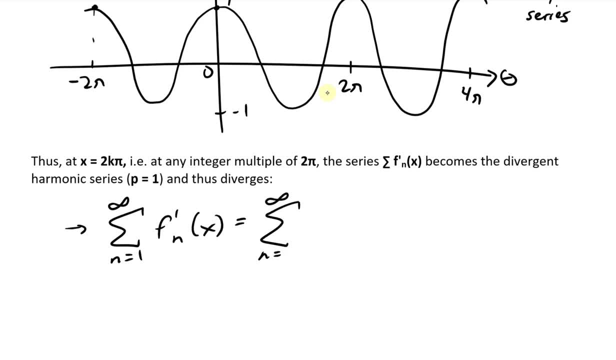 this equals to summation, n equals to 1 infinity. uh yeah, up to infinity, and this is going to be our 2k n pi desen, and this is going to be two k and pi over. endness just becomes right here. this is going to be 2k n pi over, and this becomes right here. 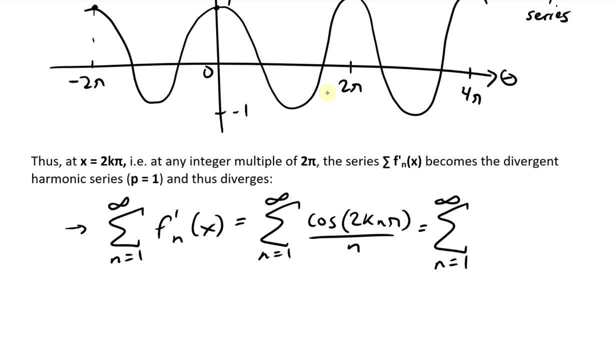 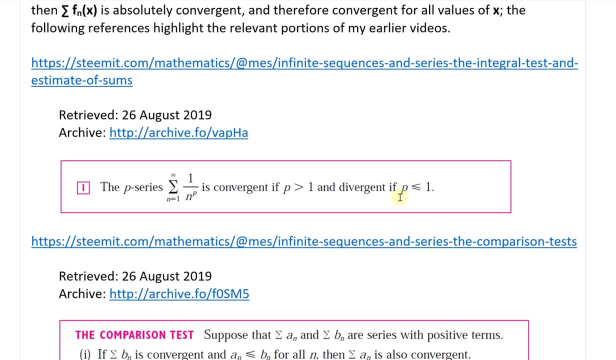 this is the harmonic series. the harmonic series, recall this, the harmonic series. this equals to 1 over m. this is divergent, theta or diverges: yeah, so this is a harmonic series and this is, yeah, diverges because this p equals to one. so that's 1 over n. and recall, this is database. 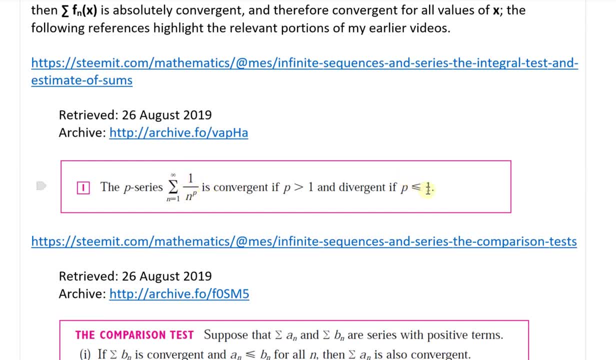 from this early reference. uh, this piece series, summation n equals one to told me this pie series and he goes one to infinity. a probabilityutt and p. this is a diversion if p is less than or equal to 1. in our case that equals to 1, that's. 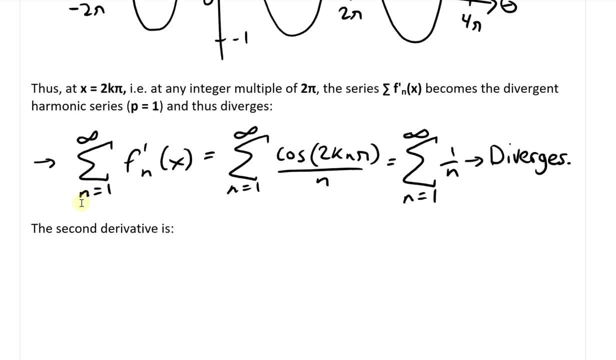 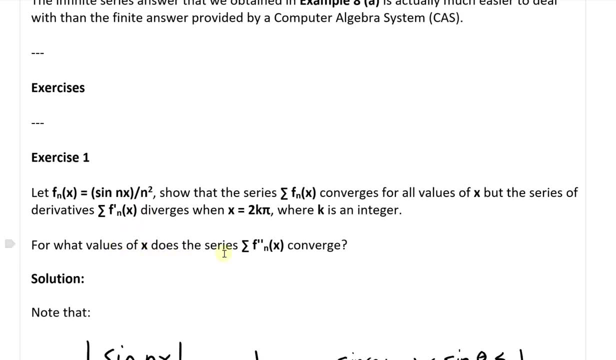 harmonic series and that is divergent. all right, so now let's look at the second derivative and let's just uh refresh what the question says. uh, so now? yes, now it's asking for what values of x does the series summation of the second derivative, uh, converge? so let's look at that. so the second. 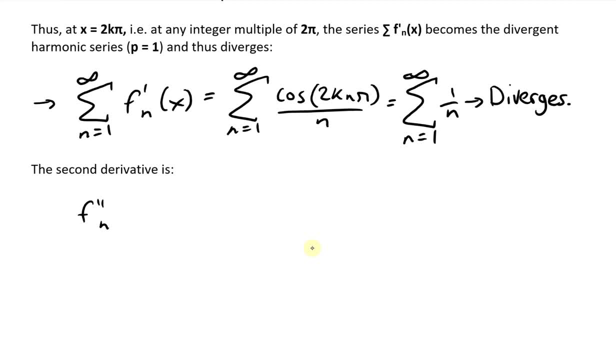 derivative is that's just going to be f double prime n of x, and this equals to well d over dx of the first prime n of x. this is going to equal to well the derivative of that d over dx of cosine. right here let's put a bracket. actually that's just going to be n of x, and actually i hear it. 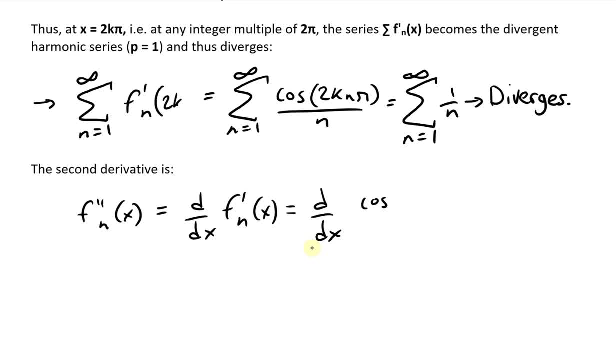 from. for more completeness here, this is going to be at 2k pi, or actually i'll just leave it there. we already state that that at x equals to 2k pi, which we'll place in there. so, anyways, this is going to be uh cosine, uh this. 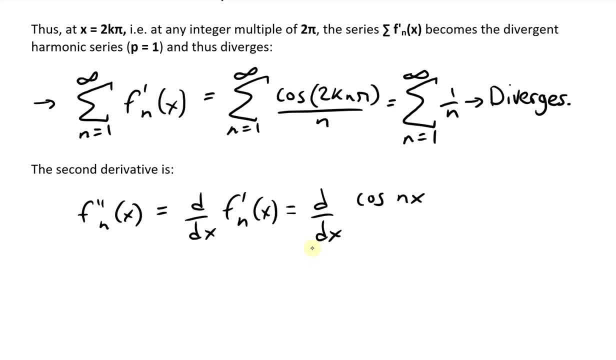 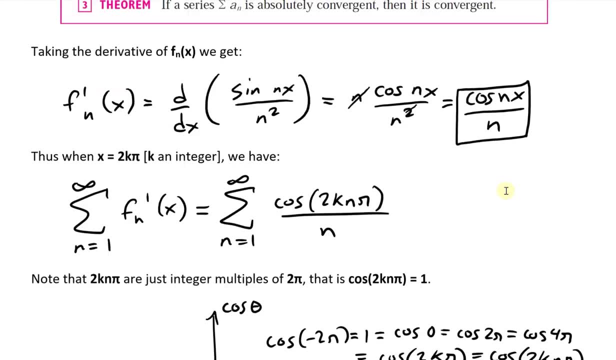 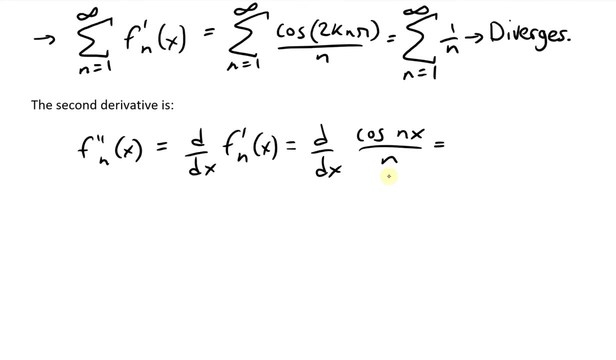 is going to be cosine number. this is going to be n? x, yeah, so n x over n. and just to show you that again, just to um show it here. so it's going to be cosine n- x, like that, over n. so to take the derivative of this recall, the derivative of of cosine is going to be well negative sine. so this: 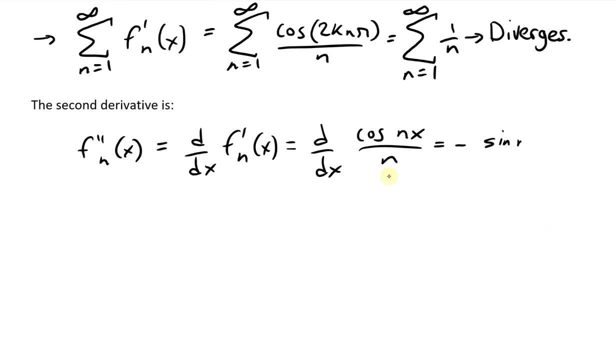 is going to be equal to negative uh sine, so n of x, and then the n will go down and will cancel. so take the chain rule divided by n: this cancels, like that. i'm just going to leave it as a negative sine n of x, like that. and this has no. 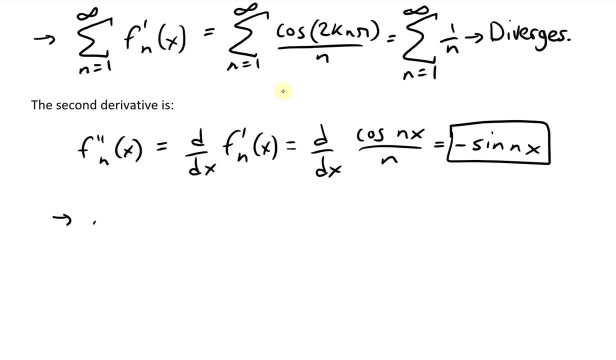 divided by n. thus, if we write this in serious notation, thus we can write this as a summation: n equals to 1, up to infinity. and now we're going to get a sine n of x, or i'll just write this as comparison function to this. you only have a sin x here. i'm just going to take the selvedge function. 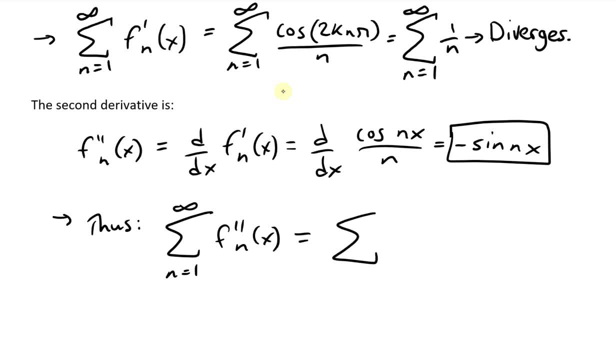 Anen, start the state area of f, Braille Come fully. so we're going to f double prime and of x. we got this equals to summation and put this negative sign outside of it. so outside of that we'll have it n equals to 1 and then it's just sine an of x and uh, this right here, this is a sine function. 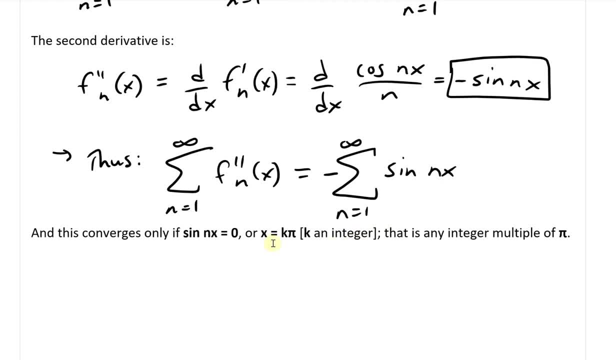 and this converges only if sine n of x equals 0, or in other words, x equals to k pi, where k is an integer, that is, any integer multiple of pi, because, remember, the sine is all slides back and forth. so the only way we could have it converge is we determine that the sine period 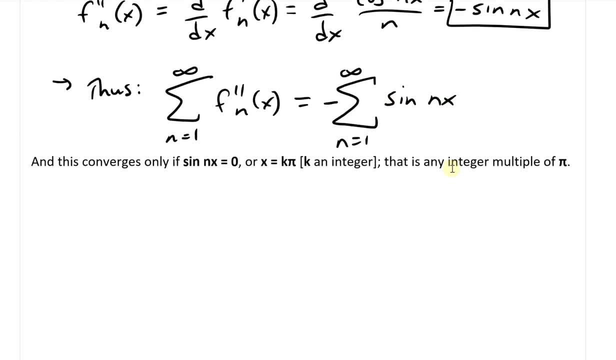 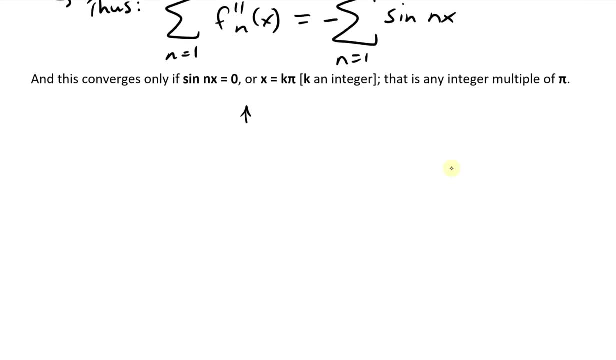 minus one times n is the sin of x, or p times x plus the sin of x- the sineкие names here merge- is if this just equals to zero. so in other words- and this is this can only be done when it's going to be: x equals to k, pi or integer multiple of it. so if you write something like this or try: 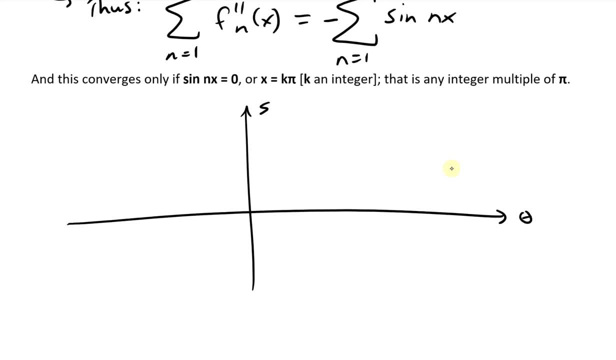 this out over here. so this is theta, this is going to be our sine theta, and this is going to be start from zero. instead of um, instead of one, like the sine function, i'm the cosine function, and so on. so it's going to go like that: uh, this right here is going to go on the negative side, and so on. 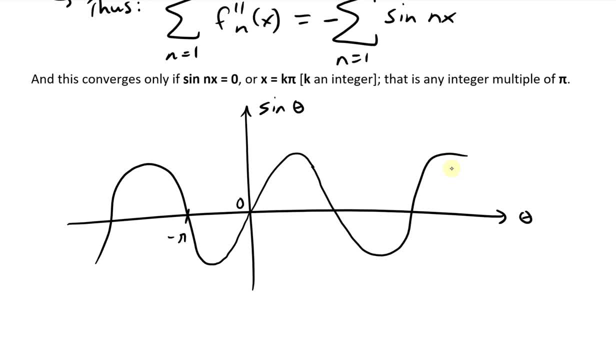 this is at zero, then this, this right here, is going to be negative pi. this right here is going to be, uh, negative two pi. so that's a full period. likewise, uh, go all the way over here. this is going to be our two pi, this is going to be our pi, and then the next time it's zero, it's going to be. 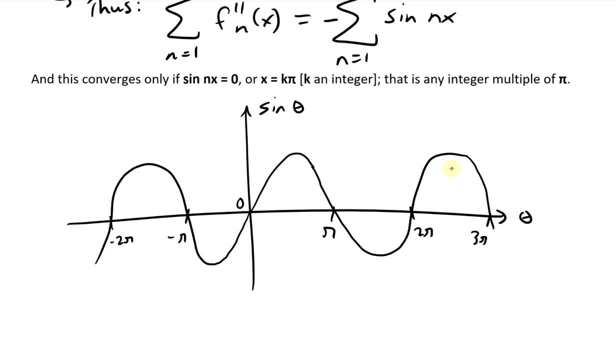 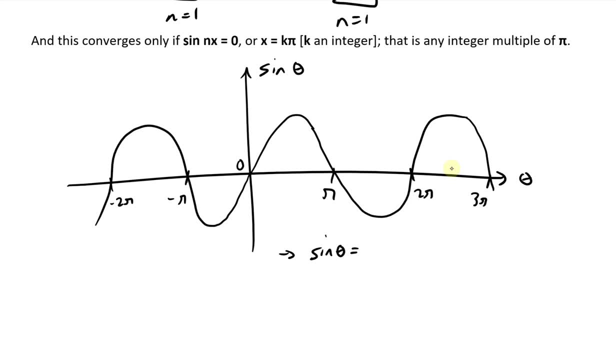 at this is going to be three pi like that. so, in other words, it's going to be zero, and then the next time it's zero, it's going to be at this is going to be three pi like that. zero, yeah, right here. so we're going to write this as uh, so we can write sine uh. theta equals to: 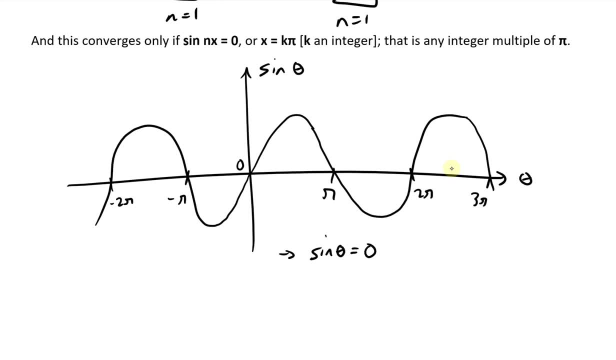 zero, uh, and this is at, yeah, this is at. uh theta equals to all zero. you could have negative pi, pi, two pi, three pi, etc. uh, negative three pi, or uh, and it keeps going on and on or uh. more specifically, at uh, theta equals to just integer multiple of pi. so in other words, 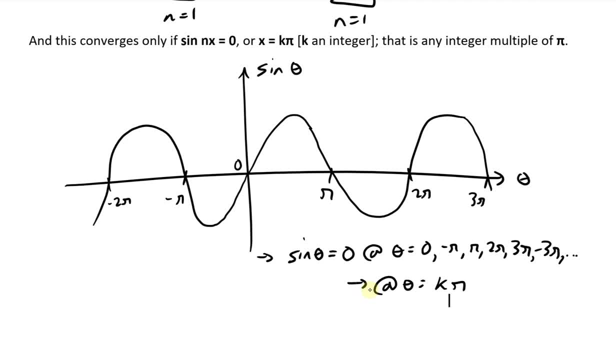 this is going to be at k pie, like that. yeah, so when, uh, this theta equals to k pi, the same thing is writing over here: x equals to k pi, and even when you have an n there n times k, it's just going to be another integer multiple and so on. so with the x is just equal to k pi. then yeah, so long as. 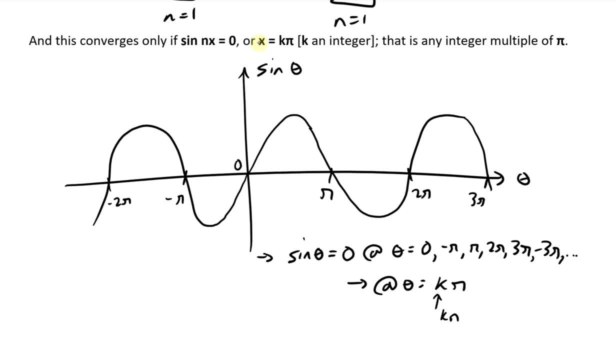 this k, right here, this could be k times and uh. so in other words, we can have uh, yeah, yeah, k, and pi, yeah, k n times pi, as long as we have an integer multiple, and we are all right. so we're going to have, and we are fine. yeah, so, yeah. so this second derivative, though, when you write: 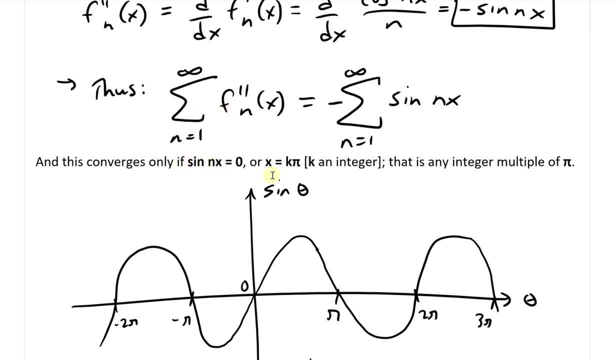 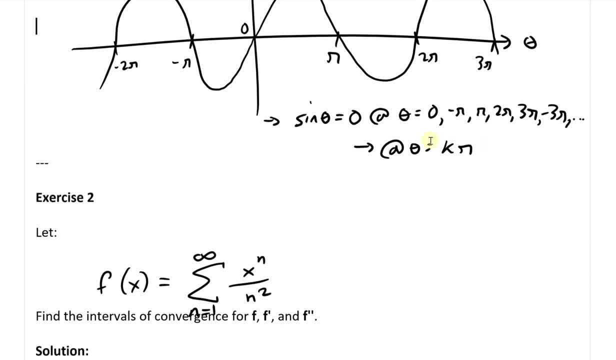 in series formation. this only converges when sine n of X equals 0, or in other words X equals 2, K, pi, like that. so those are where it converges again, which is different than the infinite radius of convergence in just the function F, F and. 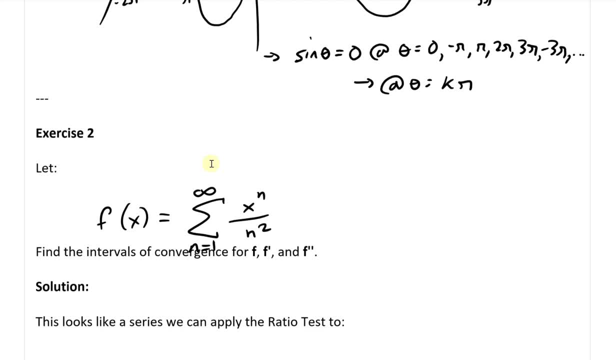 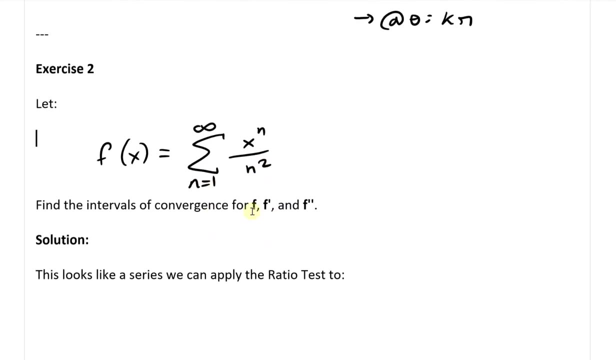 of X. so now let's look at another exercises, exercise 2, and this one states: let the function F of X, equal to the summation, n, equals 1 to infinity of X, n over n squared. and we're asked to find intervals of convergence for F, F. 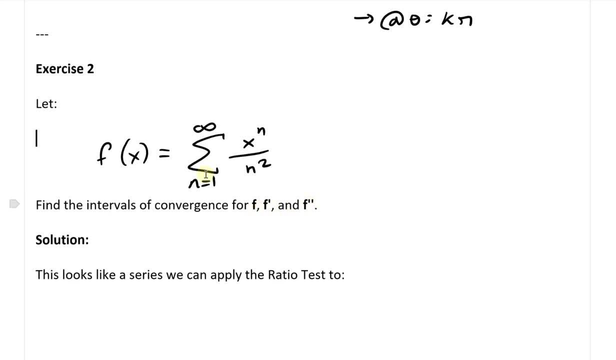 prime and F double prime, or the first derivative and second root of, and so on. so let's look the solution now this: let's look at the function F, so this, this looks like a series. we can apply the ratio test to remember the ratio test, to take you the limit of the absolute value of a, n plus 1 divided by: 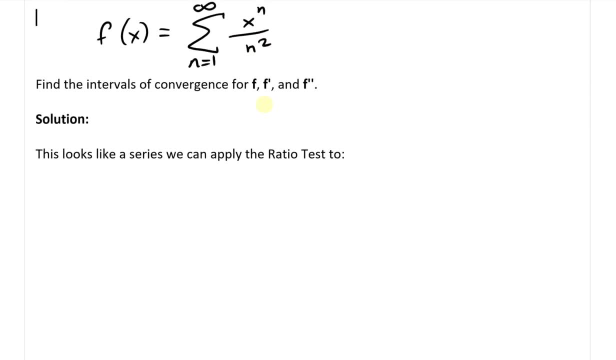 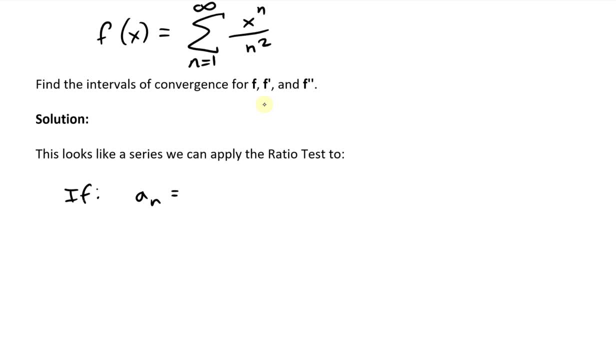 the ratio test. so if a n- and I referenced it earlier in this video, but I've memorized, so let's leave it here- so if a n equals 2, X and over and squared, then then let's just take the difference first, then we'll take the limit. so a n. 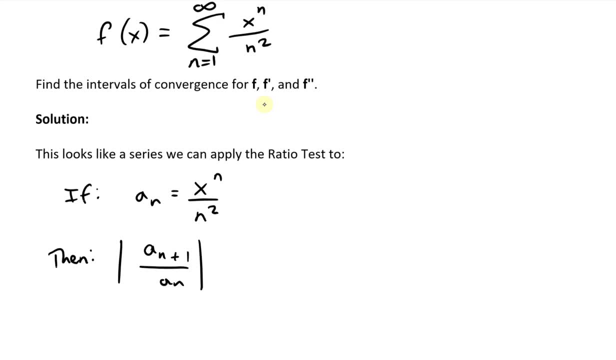 plus 1 over a n. this has to be number. the limit has to be less than 1 for convergence, so this equals to absolute value. right here, this is going to be X and plus 1 over n, plus 1 squared. and now when we divide it by a, and this is going to go at the bottom, or this X, n is going. 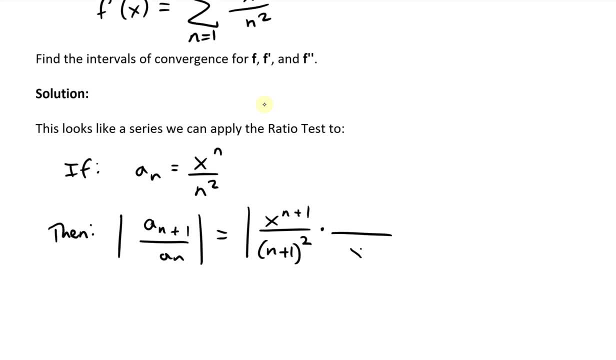 to go at the bottom and then this n squares new on the top. so this can be X and that's gonna be n squared. and now we could do absolute value, this K. we can combine these two and also the ends always positive when we do the series. so we could get that. 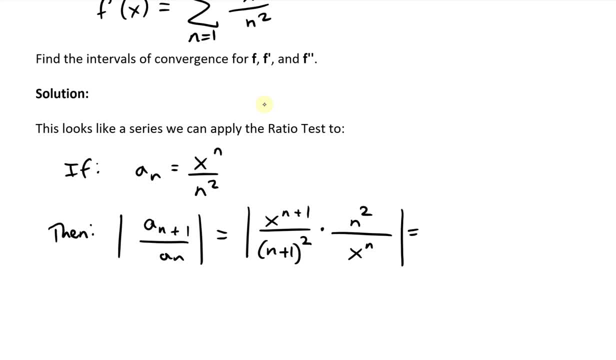 out of the absolute value sign, make it only inside the X, the only thing that could be positive or negative, I mean that could be negative. so, and then also we can combine this, so X, n plus 1 minus n. so combine those powers can be just power of X, I'm just power of 1, so this can be equal to X. times it by and then 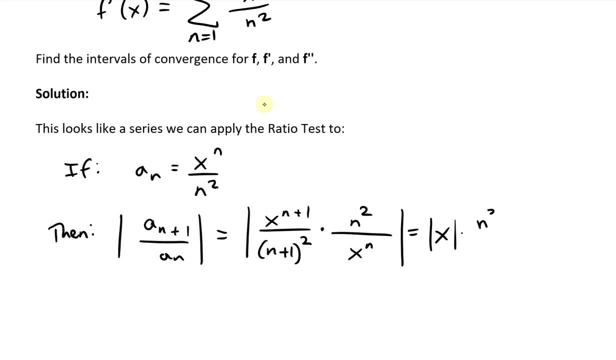 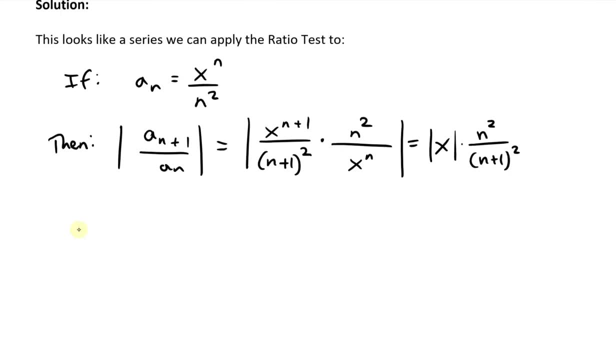 we have multiplied by n squared over n plus 1 squared. yeah, so thus to take the limit now. so thus, or just write limit limit. as n approaches infinity of this series, this is gonna be of a and should take the limit of a n plus 1 over a n. this equals 2, right here, this X is not. 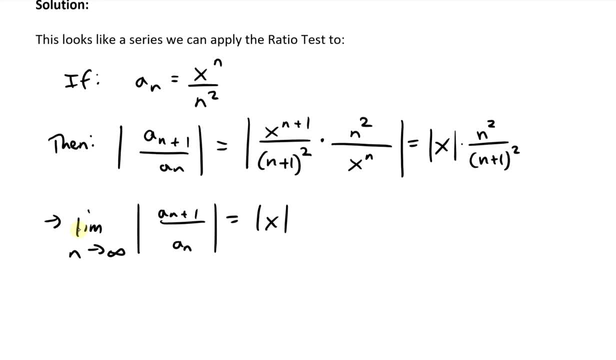 dependent on, and we just factor that out of the limits is going to be X times it by limit, as n approaches infinity, of n squared over. and now we have n plus one like this: uh, n plus one. yeah, this is actually a squared squared. we just uh, remove the squared and put it all together. just write this as n plus one. 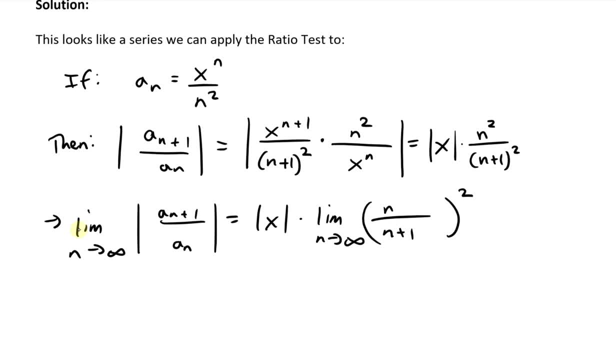 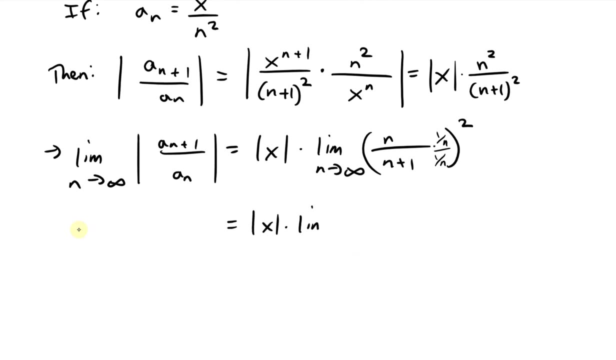 like this, and i'm going to square this all together and also just so we could do here, we can multiply the top and bottom by uh, one over n, divided by one over n, so that this right here ends up equaling absolute value of x times by limit. as n approaches infinity, let's write this: 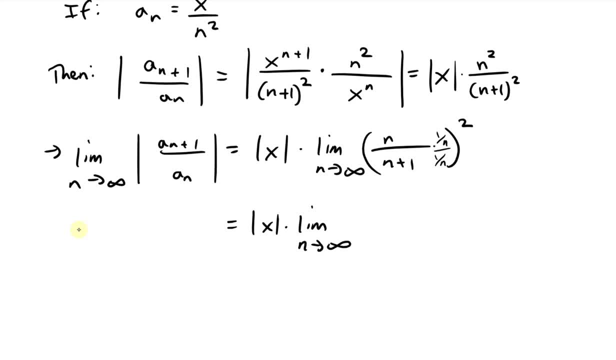 neater and approaches infinity. and now we have: um, this is this: n is going to cancel, so we're going to be left with a one over. this is going to be the end. this one cancels becomes one plus one over n, squared like that. so, in other words, what we're going to have is this, right here. 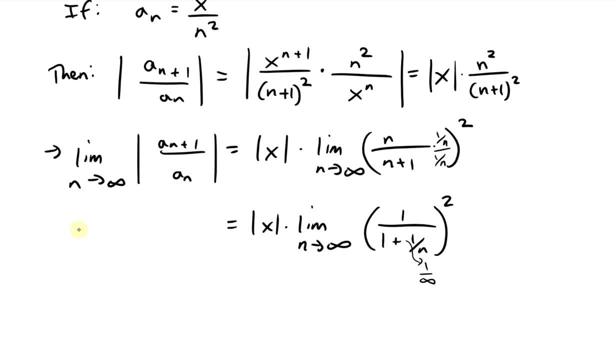 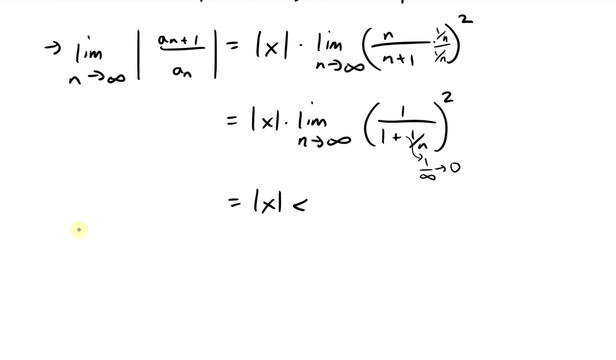 and as this goes to infinity, we have a one over infinity approaches zero. so in other words, we're going to have a one divided by one plus zero. in other words, it's going to be one when we all squared. so this just equals to x, so equals to x, and uh, with the ratio test. recall that this. 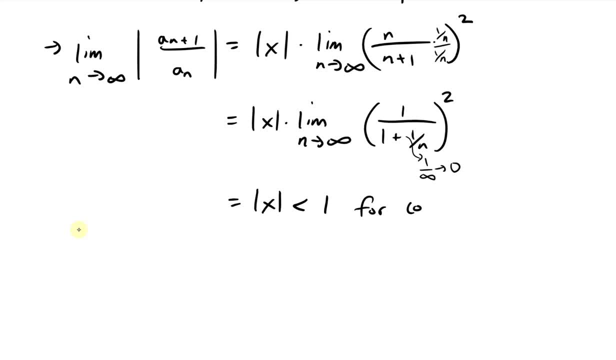 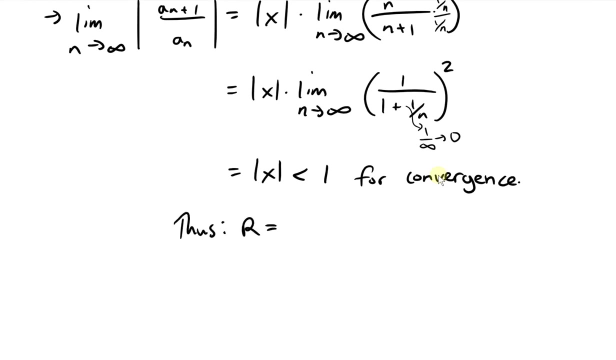 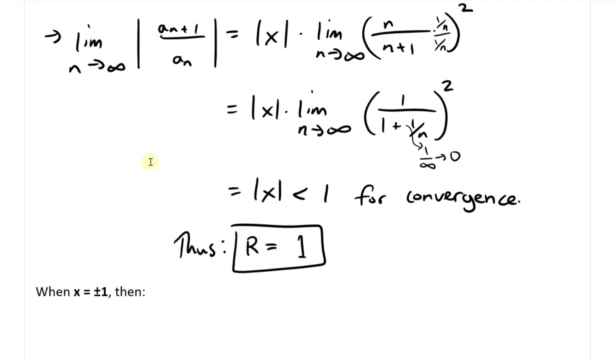 has to be less than one for convergence. for convergence like that, yeah, so, uh, thus, the convergence are is: uh, yeah, so thus r is radius of convergence. this equals to one. just square this, so yeah, the ratio test just gives us the radius of convergence, but doesn't tell us the interval in terms of the. 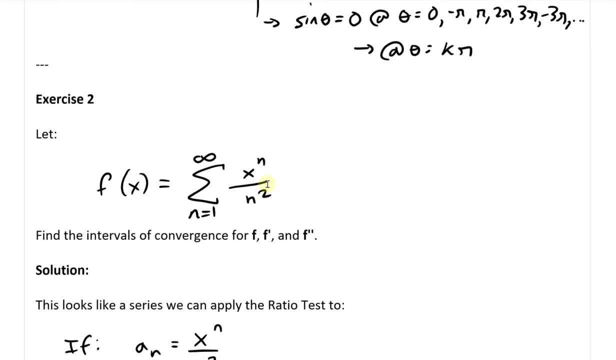 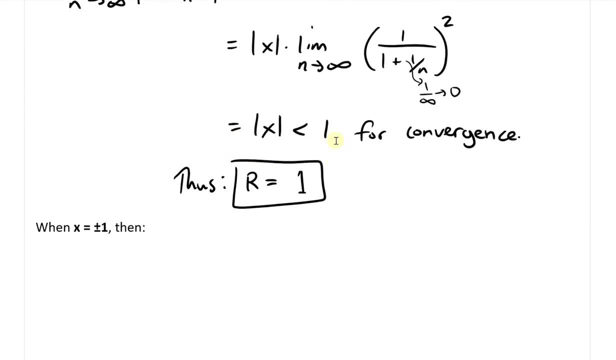 endpoints. we just know this radius, we don't know the endpoints, so we have to check the endpoints ourselves manually. so this is a function right there, and so the endpoints are at: x equals one, so or uh plus minus x equals one, or the absolute value of x is equal to one, so 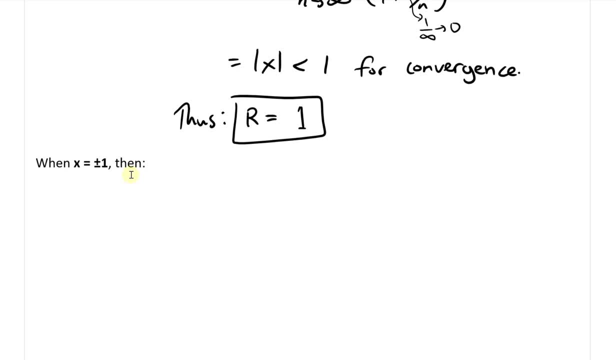 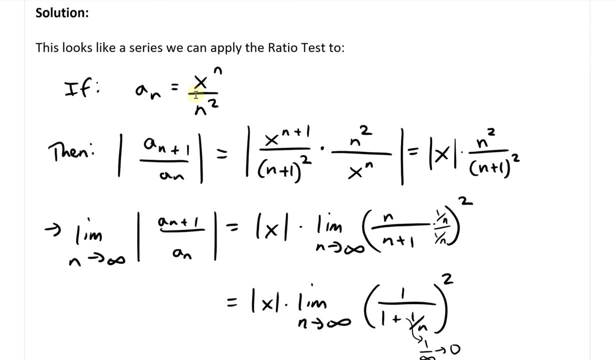 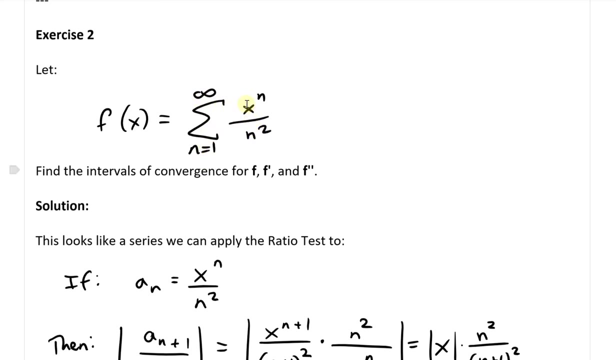 when x equals to plus or minus one, then what we end up having is: if we take the absolute value of this series or uh of the terms, so we have this function, fx equals to a series of the summation, n equals one to infinity. so we'll go with the absolute value of this uh whole thing. so what we? 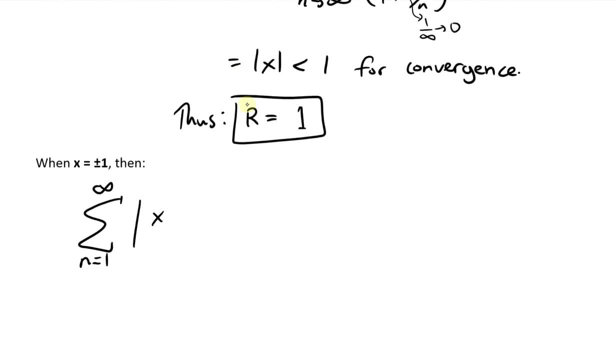 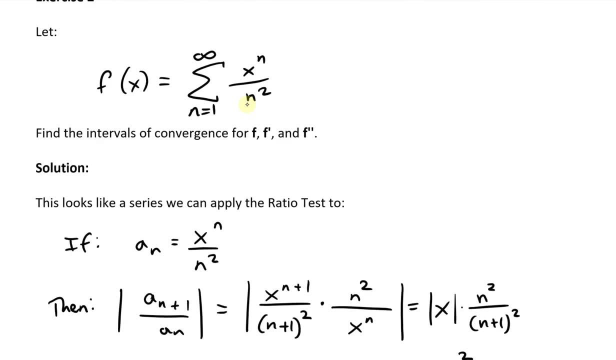 get is: yeah, so the absolute value of x to the n over uh n squared this is: yeah, see if i got that right. yeah, so this is x over n squared. so the absolute value of x to the n over n squared. this is divided by n squared. this right here, when this is equal to plus or minus one, we're just going to get. 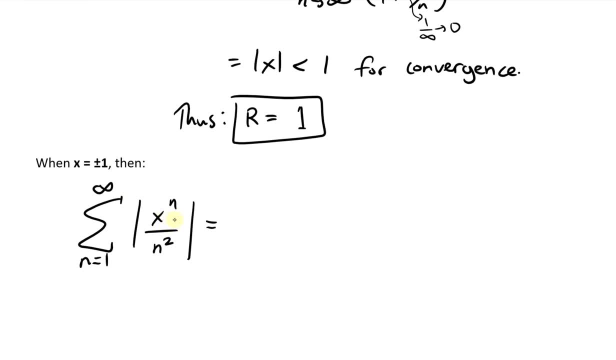 a plus or minus one to power of n, which is going to be either plus or minus, but we're doing absolute value, so it's going to be equal to one. so this just equals to n, equals to one. one over uh, n squared, this is just a p series, uh, a p series of p equals to two, and this is convergent, yes, this. 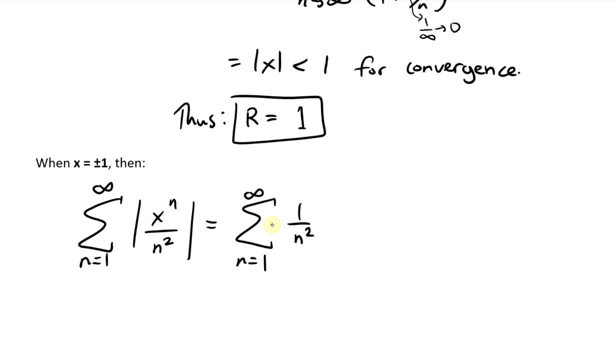 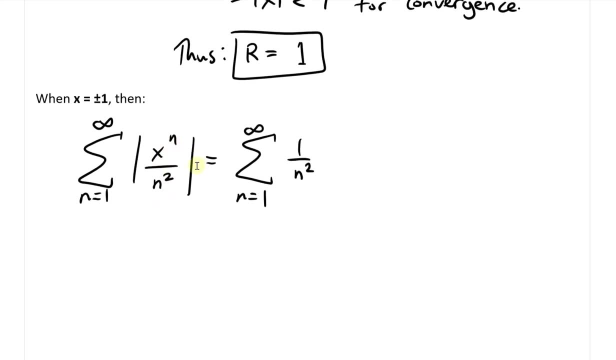 is a convergent p series. so then, by the comparison test, or by, uh, the uh, absolute, uh, absolute convergence, uh, theorem, this is going to be convergent: the x, n divided by n squared: if it's absolutely convergent, it is convergent. so, yes, uh, this is just a convergent p series. p equals two. 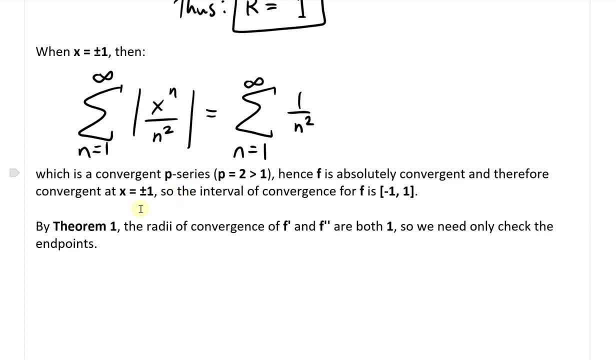 is greater than one. hence f is absolutely convergent, and therefore convergent at x equals plus or minus one. so the interval of convergence for f is just going to be well, from negative one to one close bracket. so this includes the end point. so now going further, by theorem one, the 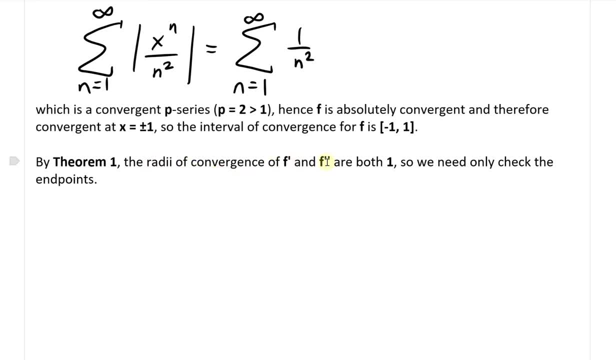 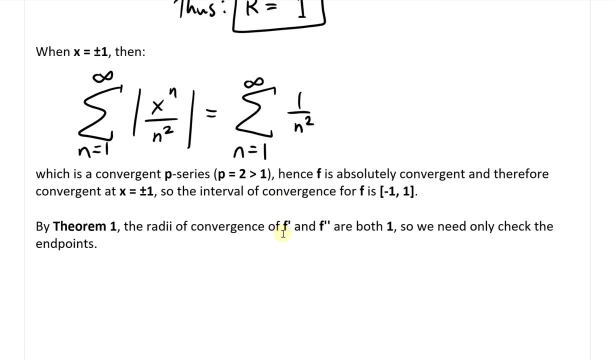 radii of convergence for f prime and f double prime. this is, this is just a. you know, this is just a power series, this uh x, power of n. so thus the radii of convergence of the derivative and the second derivative are both uh one, just be exact same. so we only need to need to check the end. 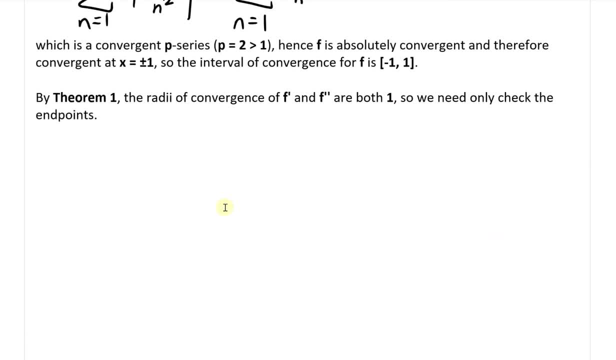 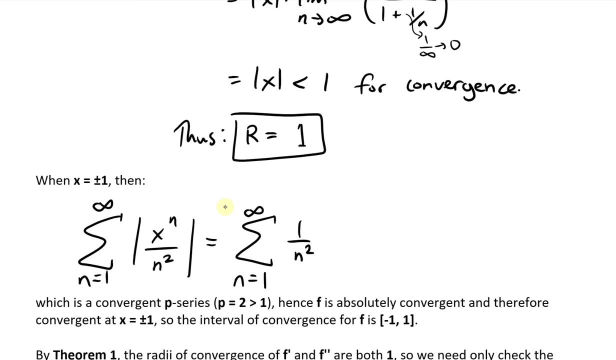 points. so so let's consider the first derivative, uh. so thus let's just check this first: uh f prime of x, so f prime of x. this equals to d over dx of f of x, and f of x is equal to uh, just x n over uh. 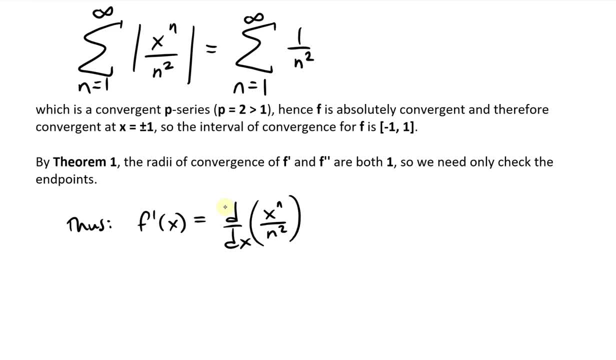 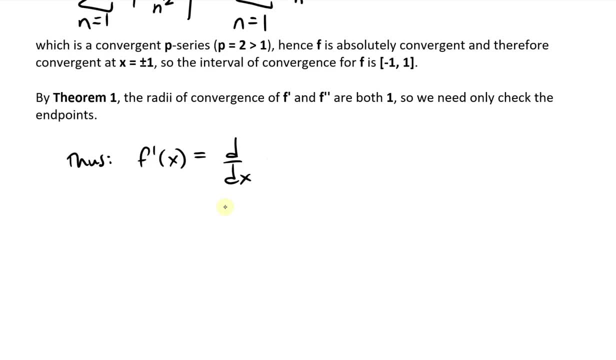 so x, n over n, squared like that, and then the derivative here is going to equal to: actually, uh, we have to put the whole entire derivative here, i mean the entire series. so this is equals to when you put it inside, this is equals to summation: n equals to 1 up to infinity. 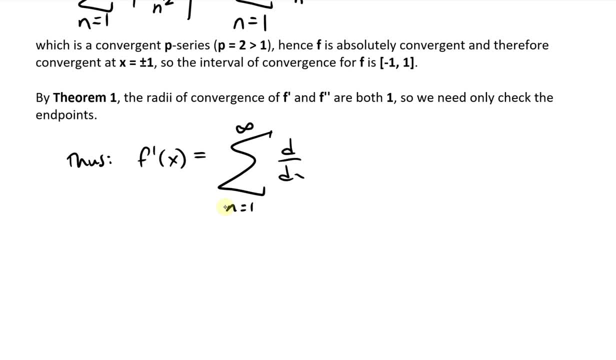 of uh, this is going to be the derivative d over dx, of x to the n over n squared. so again, it's just theorem one, and this is just term by term differentiation. and then we could plug this inside. we get infinity: n equals to one and this is going to be: n goes down, so we get a n over n. 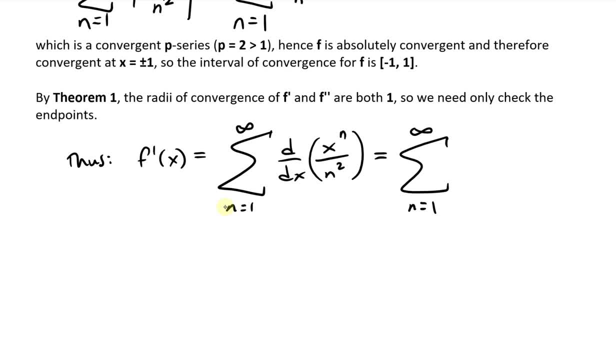 squared, that's just going to cancel out, to become: uh, yeah, this is, this is- i'll just put that down anyway- so n over n squared x and minus one. so just subtract it like that: yeah, so now this would cancel this. and uh, yes, this cancels with this square, so we're just gonna have it over n and. 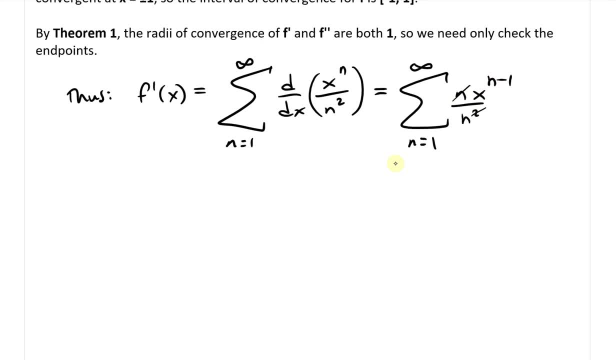 also. so right here. uh, this x to the n. uh, my calculus book just simplifies it further. the solution manual does and puts n equals to zero here and just to get rid of this n minus one there. so we'll put this to infinity and it starts off at n equals to zero. 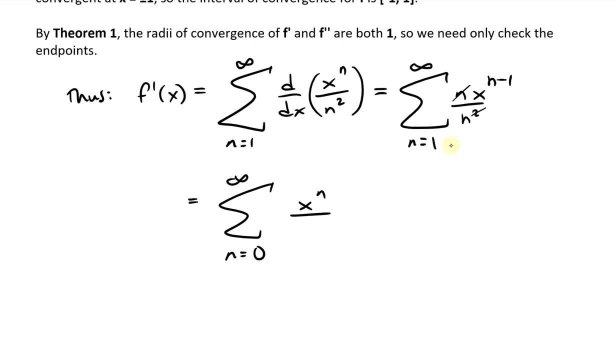 and this is going to be uh x, n over, and here's going to be n. it's going to be uh n plus one. actually, before i do that, let's just put this: uh equals one. this is going to be n and minus one, so uh, to get this equal to yeah, the same thing, but have this n equals to uh zero. 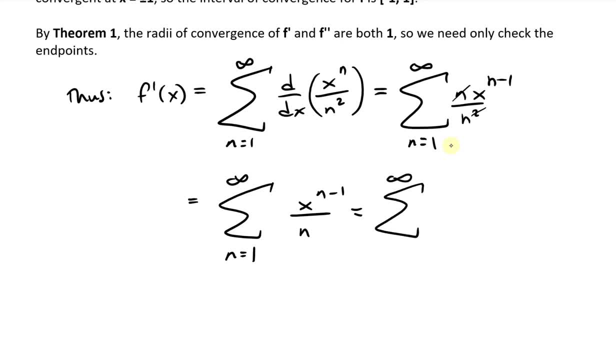 there. so calculus, we just writes it down like this: uh, this is going to be n equals to zero. in other words, what we're doing is we're subtracting, actually not subtracting. we're going to be writing uh and we're going to replace it with uh, n plus one. 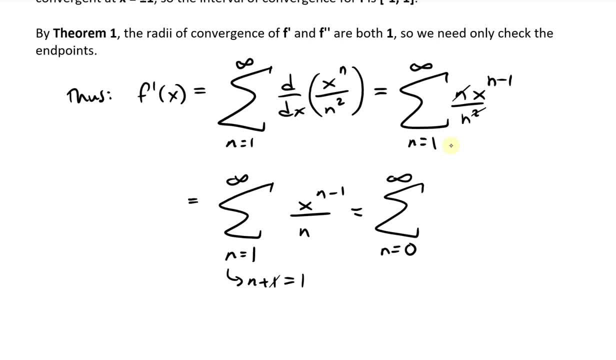 so n becomes n plus one equals one. so then this cancels, et cetera. so replacing: yeah, then we get n equals zero, so we're gonna replace it with n plus one, so it's gonna be n plus one, And so that we'll have x, n plus one minus one is going to be n, like that, And yeah, so this. 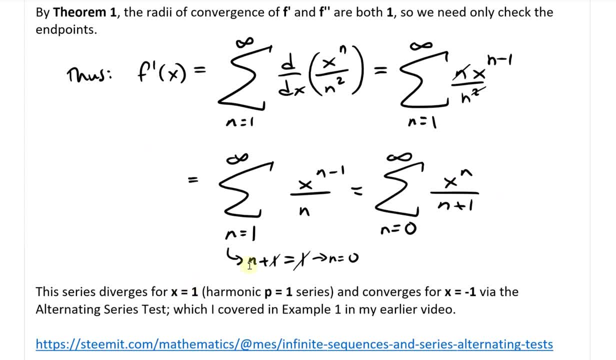 series. right here it diverges for x equals one. So when x equals one we're just going to have a harmonic series and harmonic p equals one series. And it converges here when x equals negative one, because then we're going to get the alternating harmonic series And then this is via the. 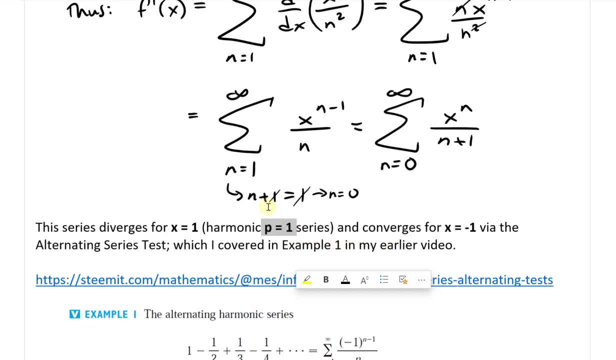 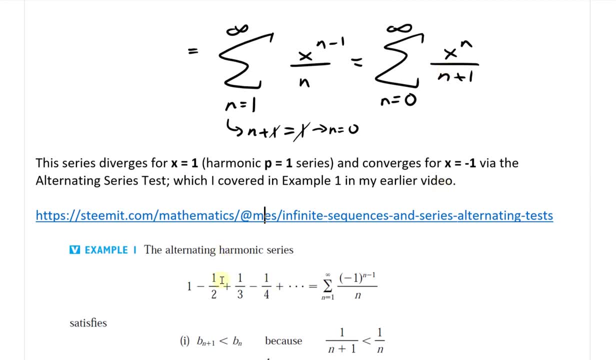 alternating series test test, which I covered- an example one, in my earlier video And again scroll down here. So, when this is going to equal to negative one, this will not equal to negative one. we, what we're going to have is the exact same formula as this right here. So, and I'm in x, n, minus, 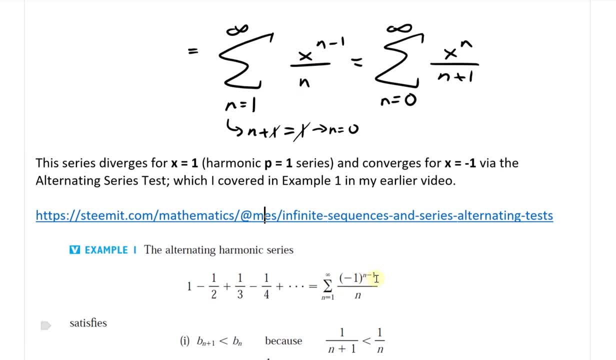 one over n. this is going to be n minus one over n. And this is when we plug in negative one for x. and we plug in negative one for x when, when we have n equals to one- here, which, using this, this one, because it looks like this formula, n equals to one, we plug that in. we're going to get. 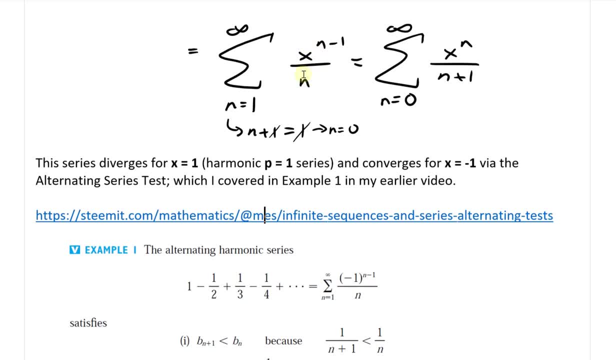 a x to zero divided by as, divided by one, which is going to be well one, one over one, So that's gonna be one, the next one is gonna be negative, And so on. Yeah, this is exactly this form. So when you plug, 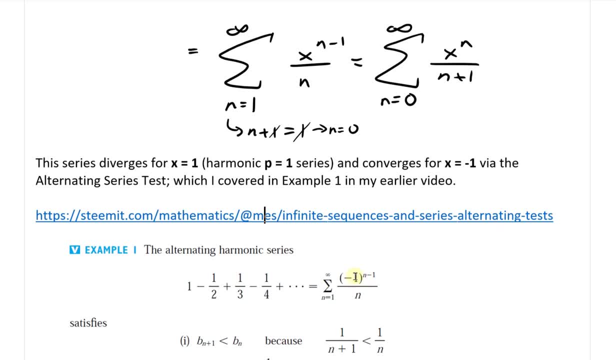 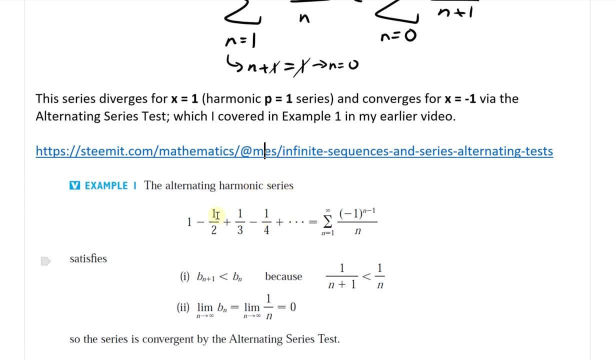 in two, we're going to get negative one. power of two minus one, that's the power of one. that's me negative and then divided by two. so negative one half and so on. So the alternating harmonic series recall that from my earlier video I showed this, that it satisfies using 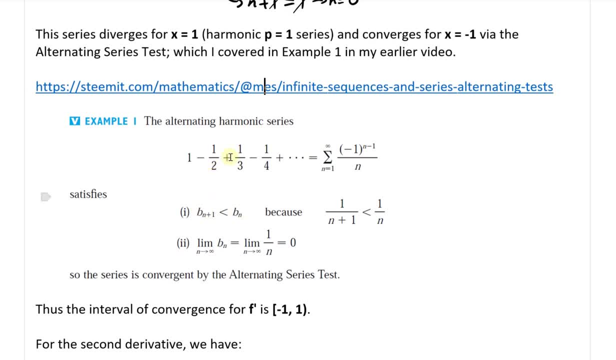 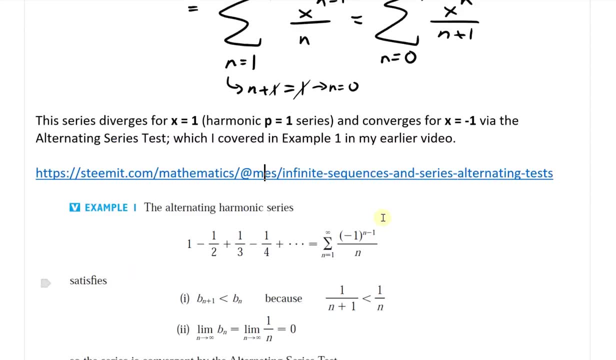 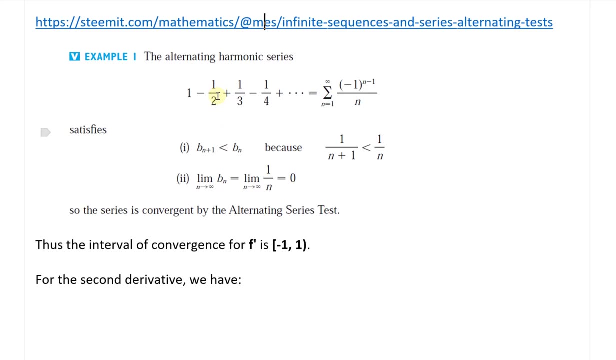 alternating series tests where b? n plus one is always gonna be less. it's always gonna be less than b? n And because, yeah, because one over n plus one is less than n, that's n plus one there. And then the second case is that the limit approaches zero. So one over n this this term. 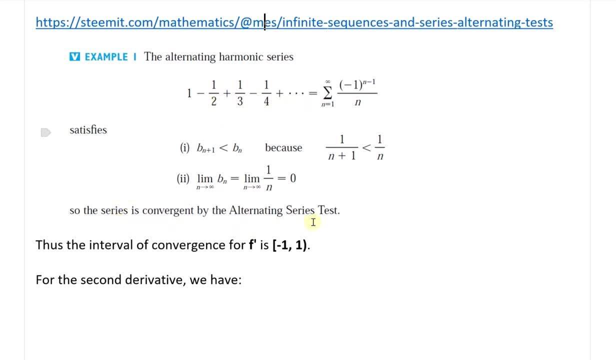 right here- goes to zero. So the series is convergent by the alternating series test? Yeah, because the term is always gonna be less than the next term and it's approaching zero And this is not proved that this alternating harmonic or alternating series test in my 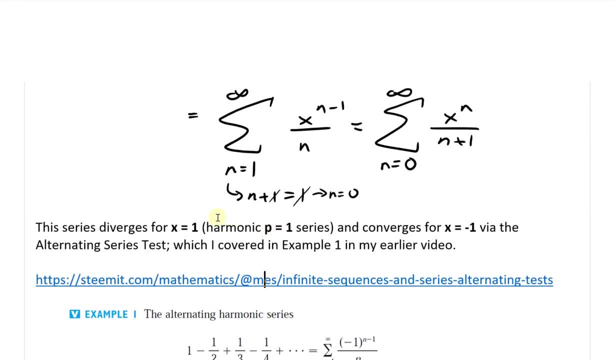 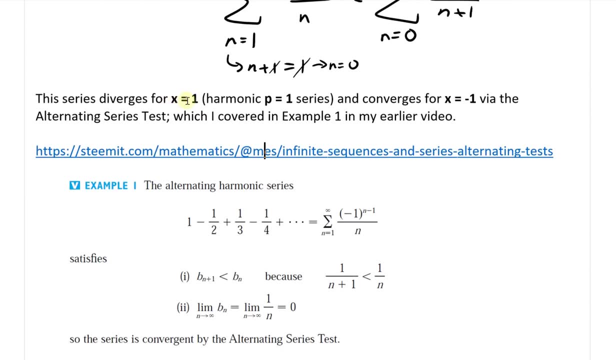 earlier video, the theorem. And so yeah, that's alternating harmonic series. And but the harmonic series, when it's not alternating, is equal to, is divergent. So in other words, we have divergence at x equals one and convergence at x equals negative one. So thus, 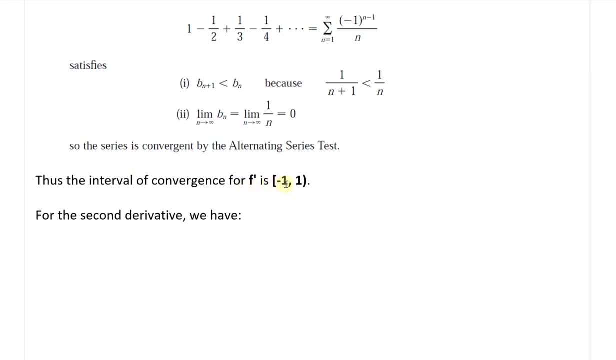 interval for convergence for f prime is going to be closed bracket, negative one, up to open bracket one. So in other words, at the negative one endpoint, but not the one endpoint. And now for the second derivative we have. well, let's take the second derivative. 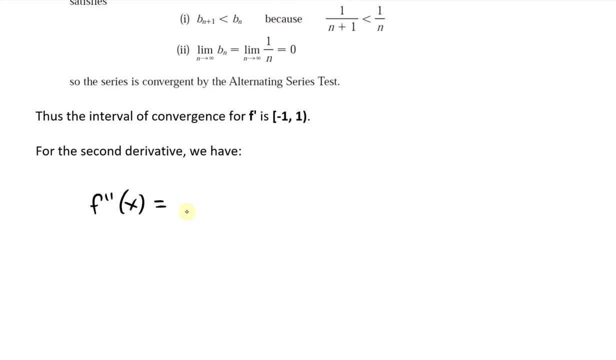 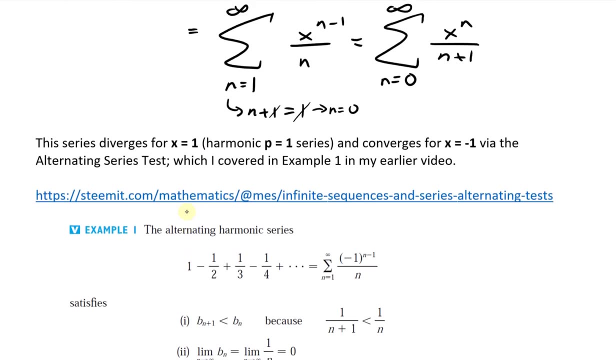 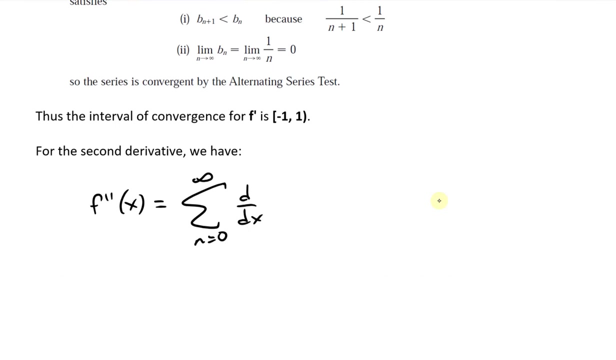 f double prime of x is going to equal to. well. the summation and up the up to infinity from n equals zero, because we rewritten it like this, So let's just write it like that. And then take the derivative of this one inside, So d over dx of x, n over n plus one, this is going to equal to. 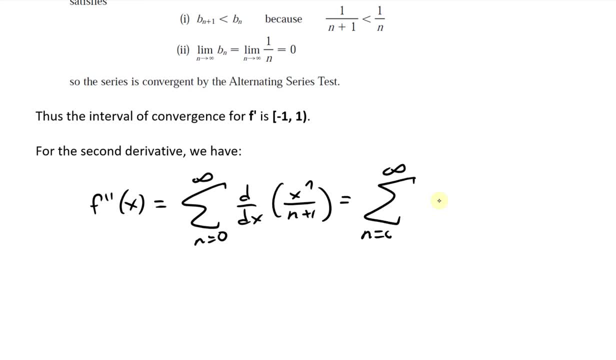 the summation. Again, it's just theorem, one, zero, and then this is gonna: the n is going to go down, And then we're going to have a n over n plus one and then times it by x, n minus one. So now to find. 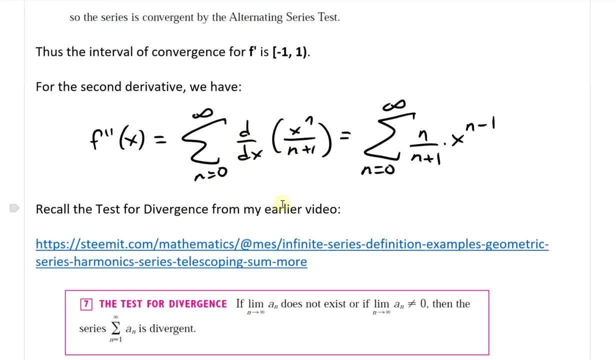 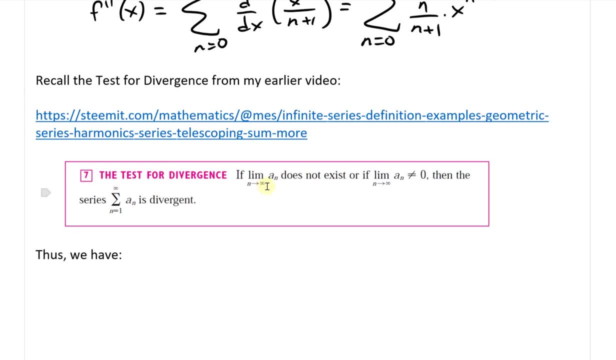 the interval of convergence. here first recall the test for divergence from my earlier video And here is a screen cap from it. the test for divergence. So if limit as n approaches infinity of a, n does not exist. or if limit as n approaches infinity of a, n is not equal to zero, has equal to. 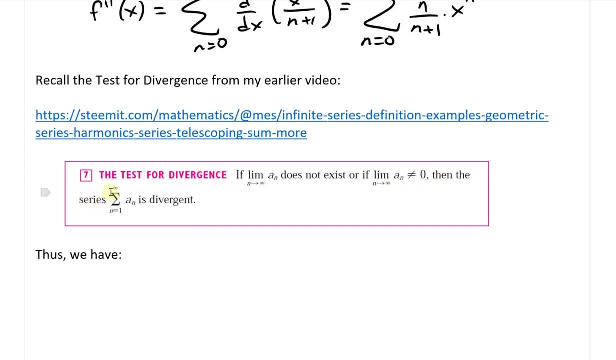 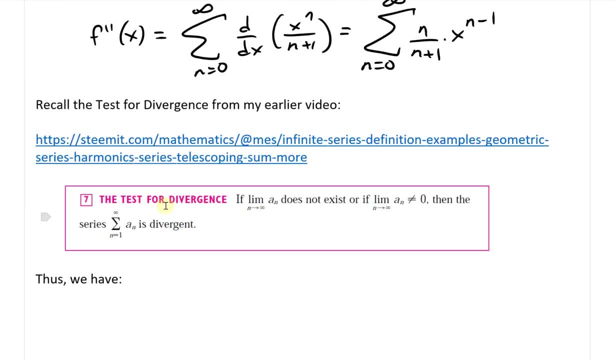 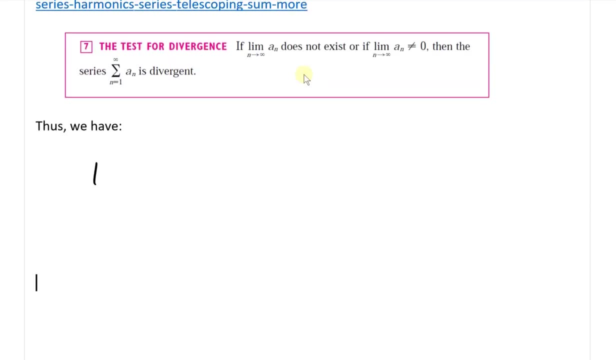 zero, then the series n over n plus one is going to be equal to zero, And then we're going to have a n over n plus one, x minus x, power of n minus one. So that's what we have is limit as n approaches. 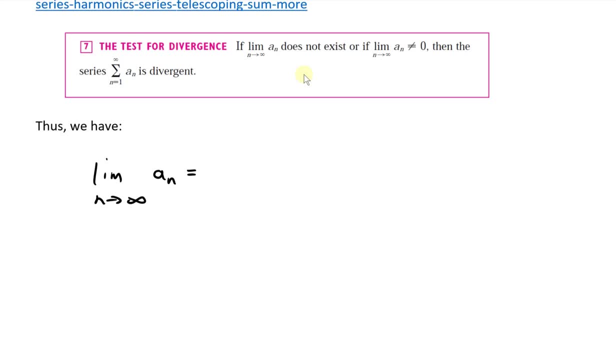 infinity of a n equals to the limit as n approaches infinity of right here n over n plus one times by x to the n minus one right here. Yeah, so now, since at x equals plus or minus one, the term x to the n minus one alternates between plus one and negative one, because depending on what power it. 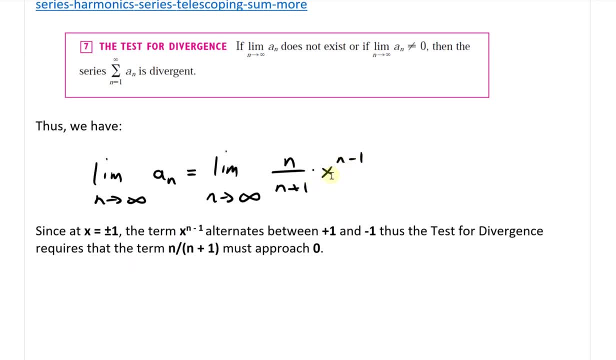 is if it's either odd or even, and this is either negative. either x is negative, one or one, then it's going to. it's just going to alternate between one plus one and negative one. Thus, the test for divergence requires that a n to be zero. in other words, requires that the term, the only term, that 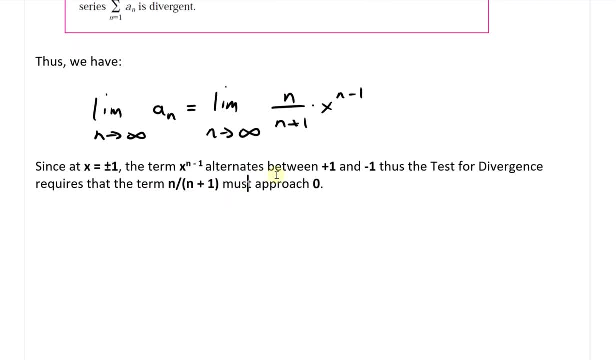 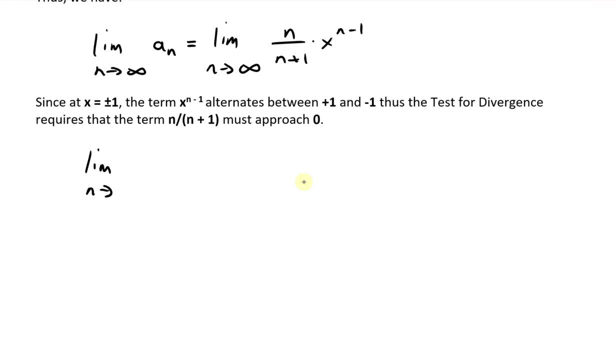 is n over n plus one, So requires that the term n over n plus one must approach zero. So thus what we have is limit as n approaches infinity of this n over n plus one. Now, if we multiply top and bottom, one over n, one over n, what we get is limit as n approaches infinity of now this top. 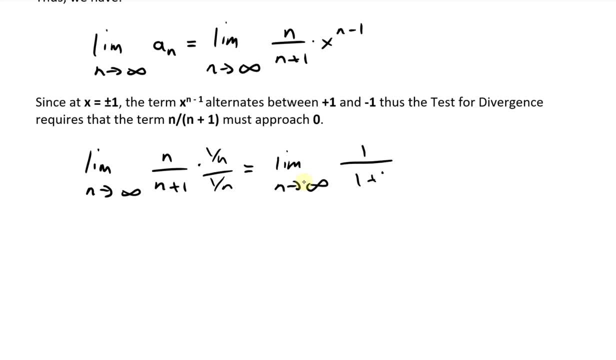 cancels be one, And then this one here is going to be one plus one, one Over n, like that. then as you plug in infinity, this becomes- or yeah, this becomes one over infinity and approaches zero. So in other words, we have one plus one divided by one plus zero In. 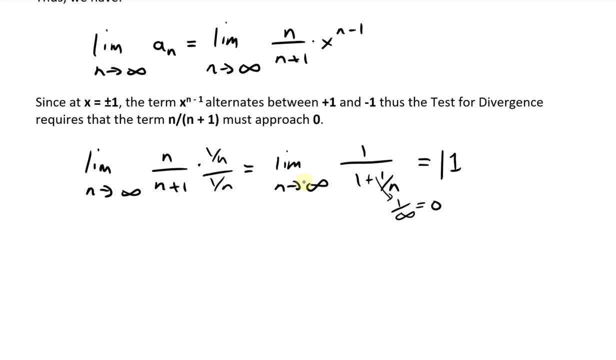 other words, we just get equals to one, which is not equal to zero. So this is not equal to zero. So thus it's divergent, because this, this, doesn't approach zero and this x, x to the power of n minus one, doesn't approach zero. for the endpoints, x equals plus or minus one. Yeah, so thus by the 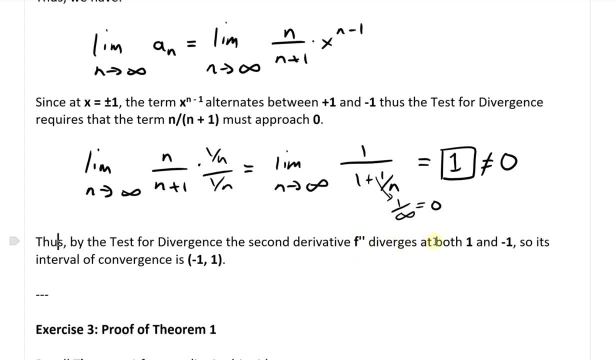 test we get the term n to be zero, And then we get the term n minus one, And then we get the term x to be negative one. So this test for divergence, the second derivative f double prime, diverges at both one and negative one, because this test for divergence doesn't approach. 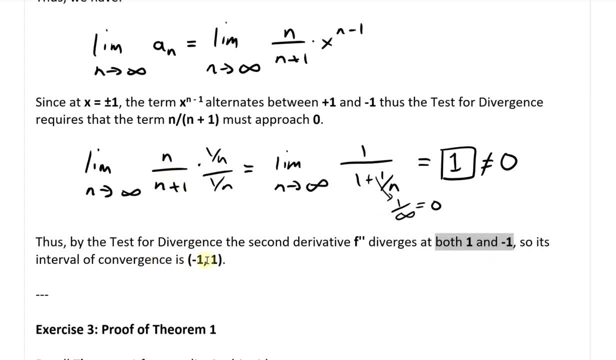 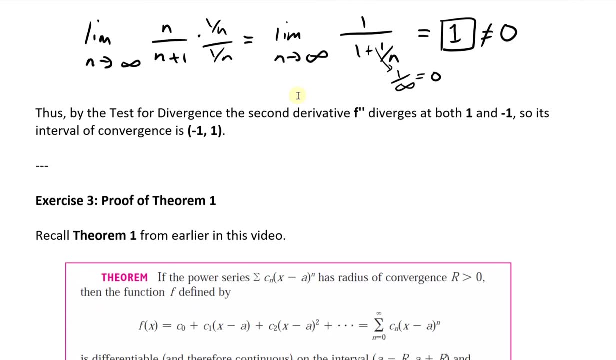 zero. So its interval of convergence is: open bracket negative one to open bracket negative positive one. So not at the endpoints, just anywhere in between. So, yes, very fascinating, fascinating stuff, Alright, so now that we finally finished all these exercises and examples, and so, 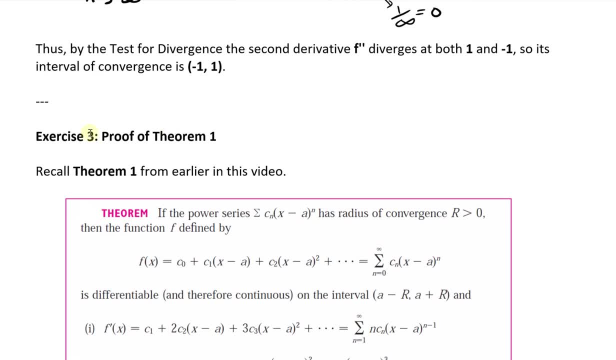 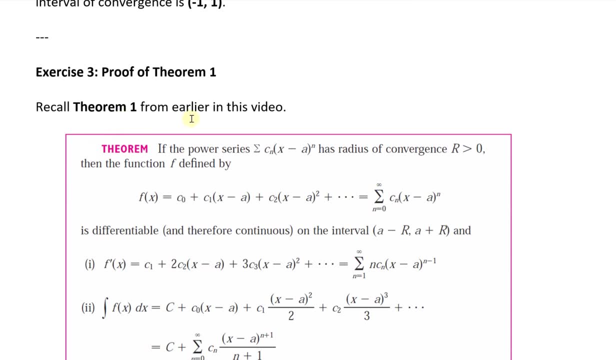 on. I'm going to go to the last part of this video and it's actually the most intense And that is proof of theorem one. So this is exercise three and recall theorem one from earlier in this video, which I didn't prove then, but I'm going to prove now and my calculus book: 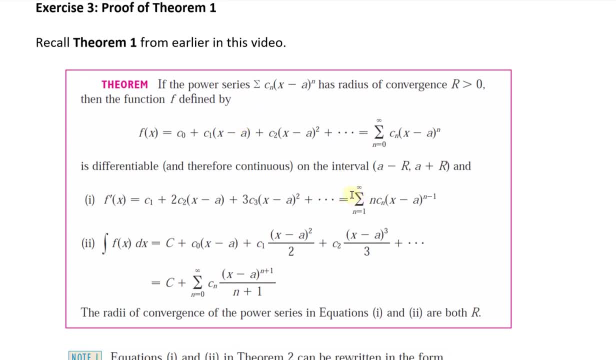 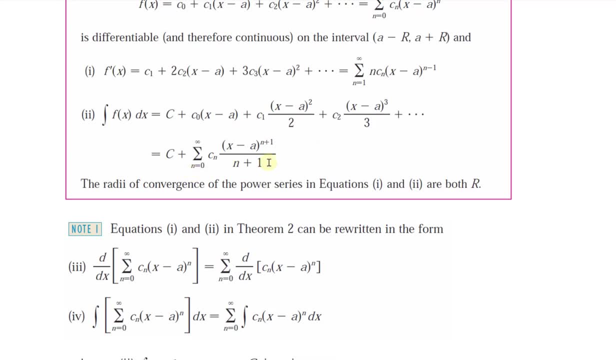 doesn't even prove it. So I found one online and had to manipulate it my own way because it's- even then it's a bit complicated. So so theorem one here. I just took it from my just copy and paste it from my calculus book, just because it's more condensed than my write up earlier. But anyway, 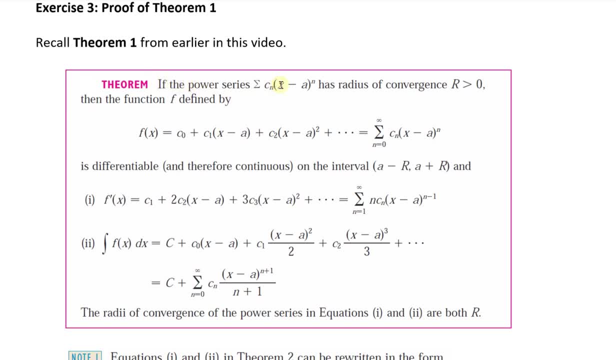 so theorem is theorem one. if the power series is the summation c n of the summation c n times x, minus a power of n, as it has radius of convergence, convergence r, which is greater than zero, then the function f, defined by f of x, equals to c zero plus c one. 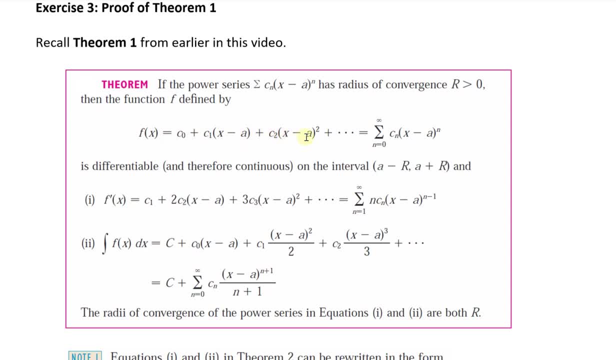 times x minus a plus c. two times x minus a, square plus dot dot dot, which equals to the summation n, equals zero up to infinity of c. n times x minus a to the power of n, And so, if this function is differentiable and therefore continuous, 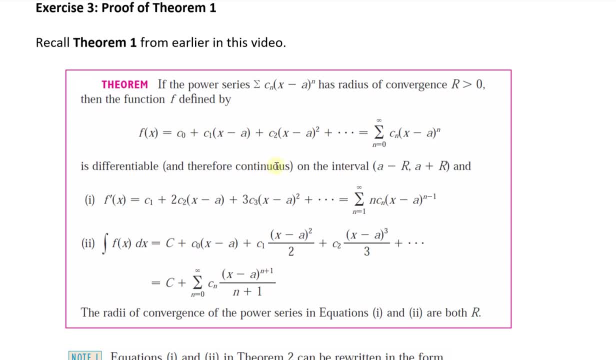 as also stated earlier, for reference my earlier video: Yeah, so it's a differentiable and therefore continuous, on the interval from a to negative r. no, I mean a minus r to a plus r. In other words, this is the interval of convergence, but without checking the endpoints, And we have i, which equals: 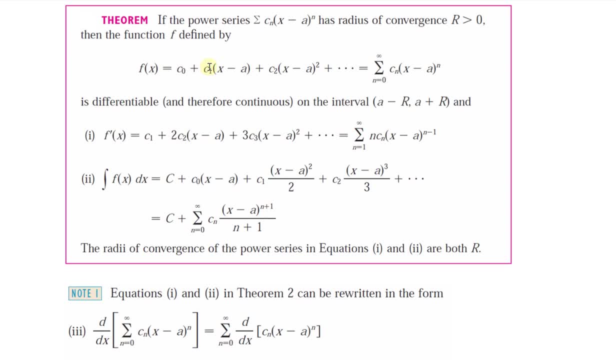 to f. prime of x equals to c one plus two, c two. this is just taking the derivative of these ones right there: c two times x minus a plus three, c three times x minus a plus three, c three times x minus a squared, and then plus dot, dot dot and this equals to summation. from n equals one to: 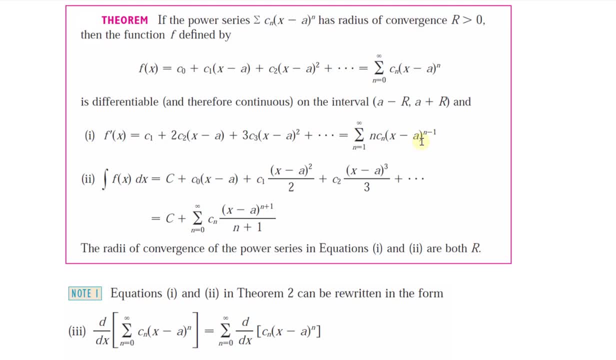 infinity of n c n times x minus a power of n minus one. And yeah, that's just the first rule, That's just the derivative of this to n down and we have n minus one, And this is it from n equals one. 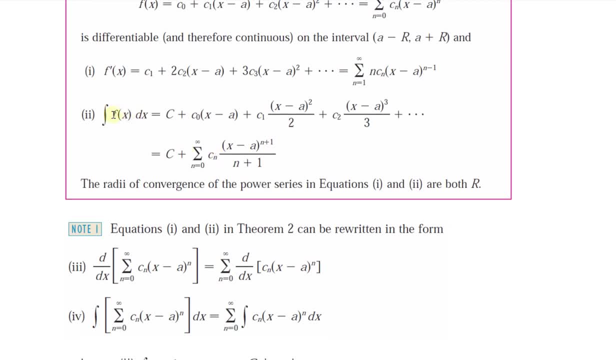 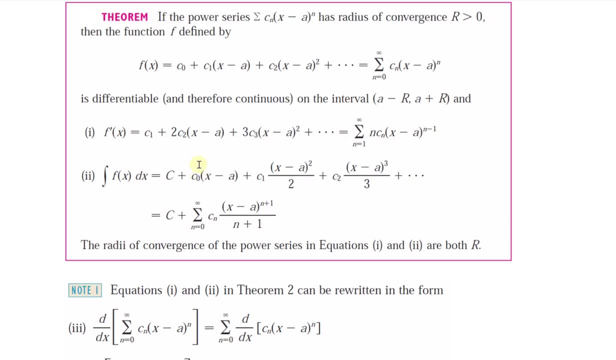 you can put n equals to zero. just have a zero term. But anyway. so the and also case case two or case i, i and integral of f of x, dx is also term by term. So this is just a derivative of n. 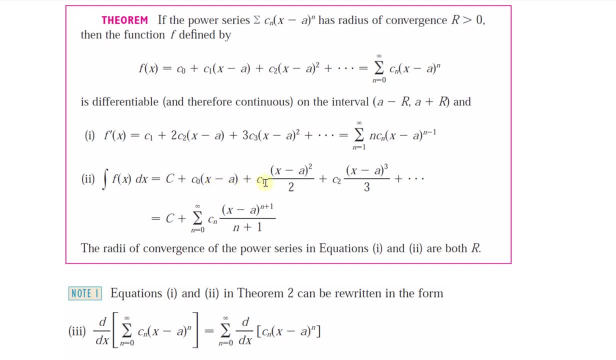 plus one. This could be c plus c, zero times x minus a plus c. one times x minus a. squared over two, this one's going to be three over three. it's a power of three over three, and so on. So c two times. 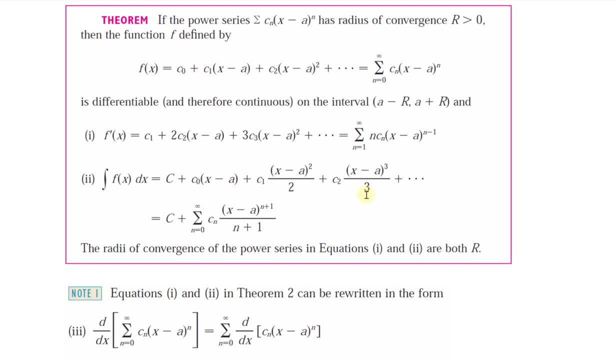 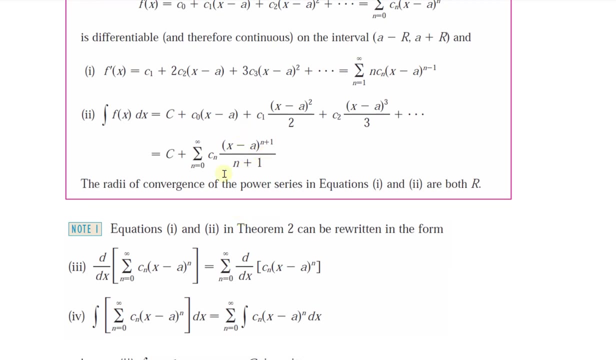 x minus a power of three over over three. n plus dot, dot, dot, which equals to plus the integration constant or constant of integration plus the summation from n equals zero to infinity of c? n times x minus a power of n plus one divided by n plus one, or all divided by n plus one. So and: 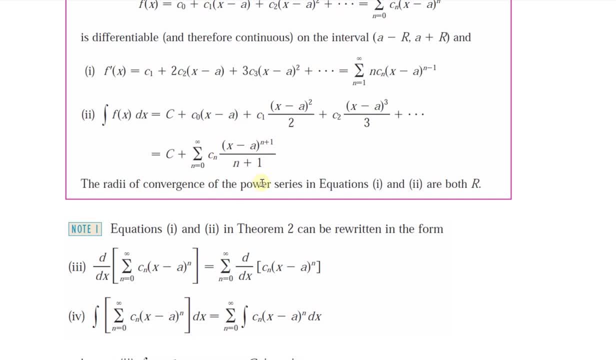 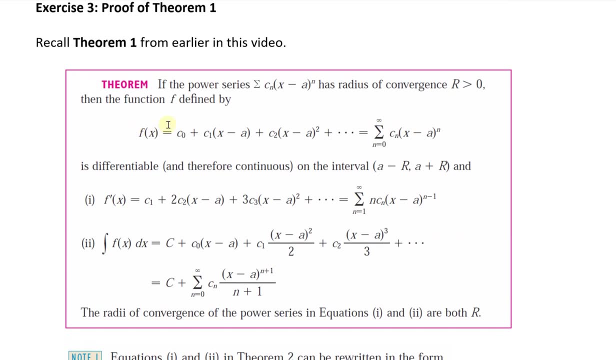 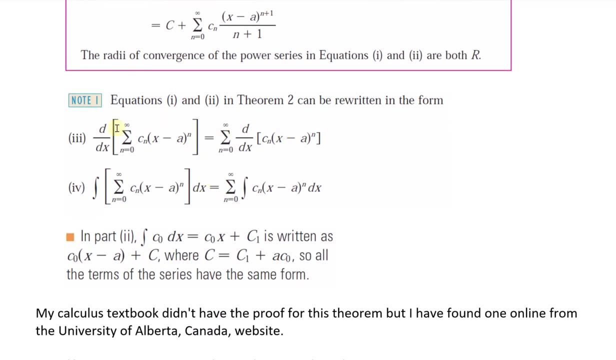 of conversion and, yeah, and the radii of convergence of the power series in equations uh one and two r, or i and double i are both r. in other words, the exact same as uh. this theorem, i mean as this function above there, and we'll prove that as well as here. we also took a screenshot of uh note one. 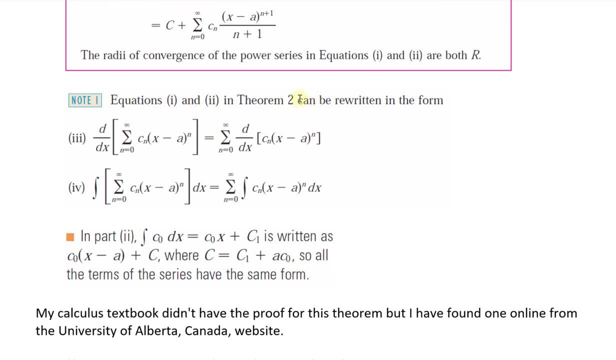 which uh equations one and two and theorem theorem. uh, this actually should be written as theorem one. yeah, i'm kind of looking at it as theorem two, but it's called theorem one, so anyways, i'll uh edit this uh after this video. yeah, so, uh, those case, uh, equations one and two above here. 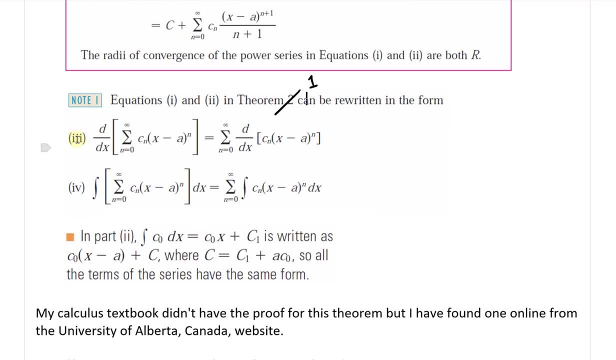 can be rewritten in the form: uh, the triple i or case three. so d over dx of this, uh entire summation equals n. equals zero to infinity of c. n times x minus a to the power of n equals to the summation. n equals zero to infinity. and then the derivative of the inside term, uh, d over dx c. 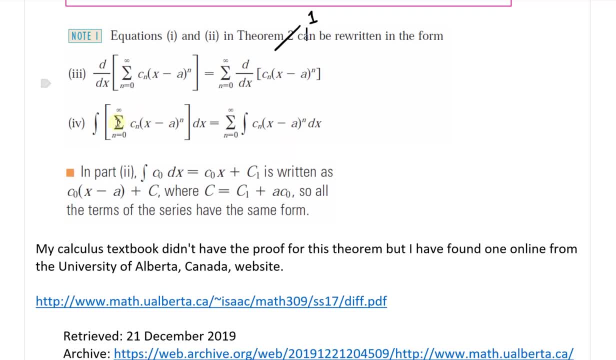 n times x minus a, to the power of n and uh. likewise, the integral of this entire uh summation, and from n equals zero to infinity, uh and so on. uh, dx equals to the uh, the series of summation n equals zero to infinity of the integral of the inside. so you just rewrite. 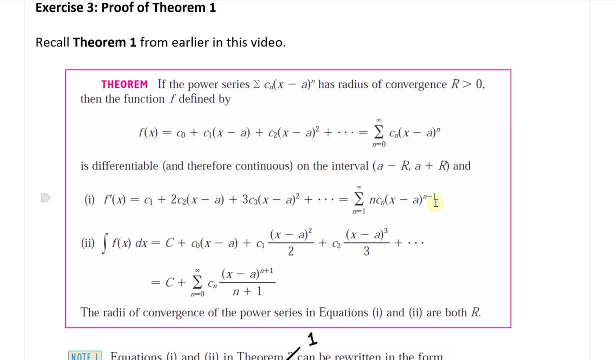 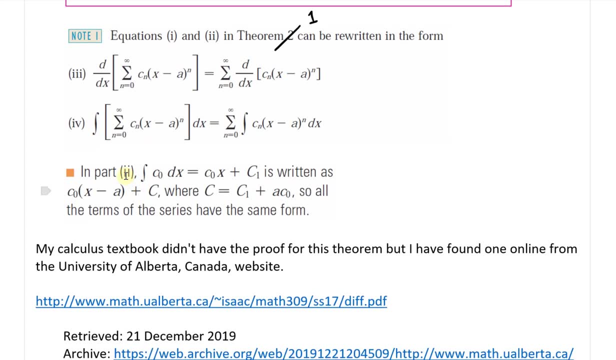 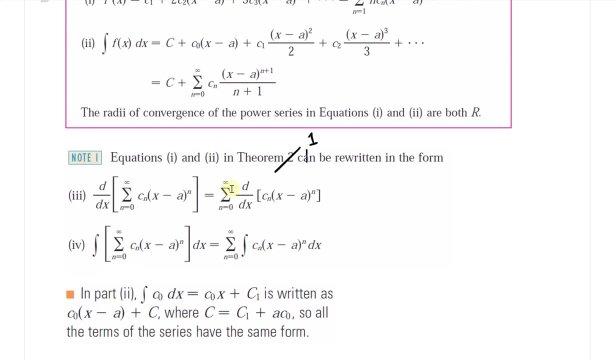 it like that and that's: this term is exactly just this, and this term and c, n, etc. is exactly this one. right here, when take the derivative of it. and also for completeness, oh yeah, for in part, uh, i, i, we had this, uh, integral of c one, we made a, rewritten it as c plus c, zero times x minus a. 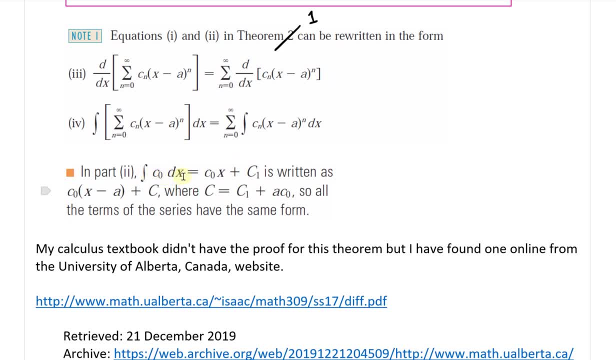 and that's this right here. uh, integral of c, c o d x equals to c o x plus c one and is written as c o x minus a plus c, where c is equal to c one plus a c zero. so all the terms of the series have the 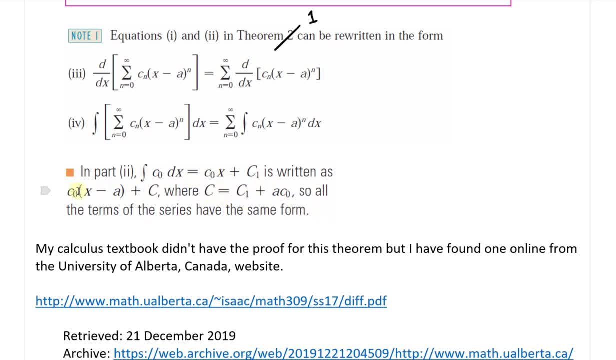 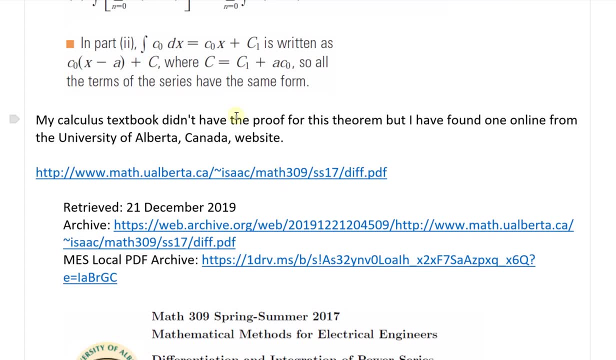 same form. so, yes, you just wrote it like that's exactly as this one, because a and c are just constants, are just manipulating as such, so c will just change relative to the c one. anyways, let's keep going further. so my calculus book didn't have the proof for this theorem, but i found one. 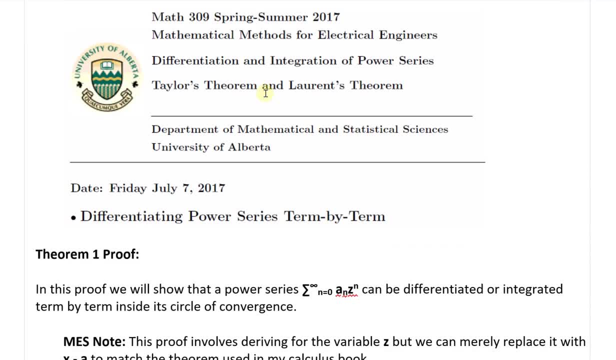 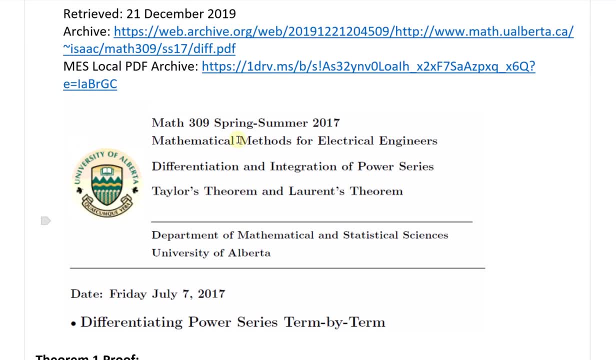 online from the university of alberta, canada website and here i'm going to go over it mainly, and plus some of my own uh, own mes uh write-ups. so this is from it. here's pdf: uh, there's the archive pdf of it and also mes local. 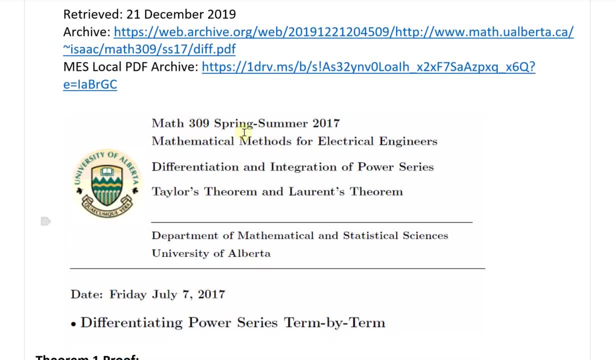 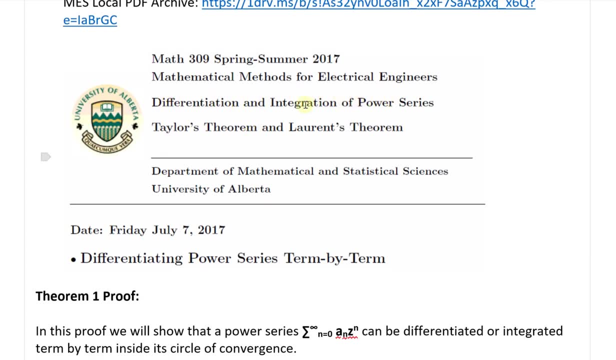 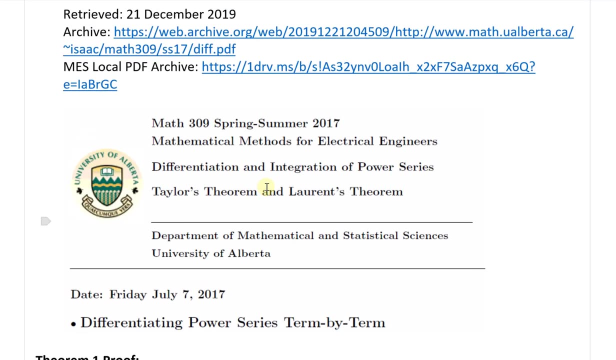 pdf archive and so on. so this is actually from a math 30309 uh course 2017 method: mathematical methods for electrical engineers. interesting, uh, different differentiation, integration of power series. so again, yeah, electrical engineers are using this. uh, this is why, uh, this is one of the most important concepts in all of science, not just math, just just, not just calculus. 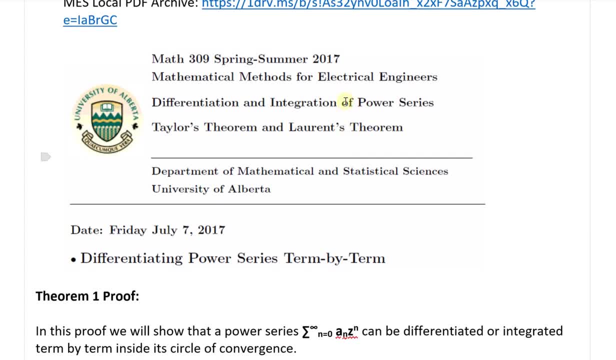 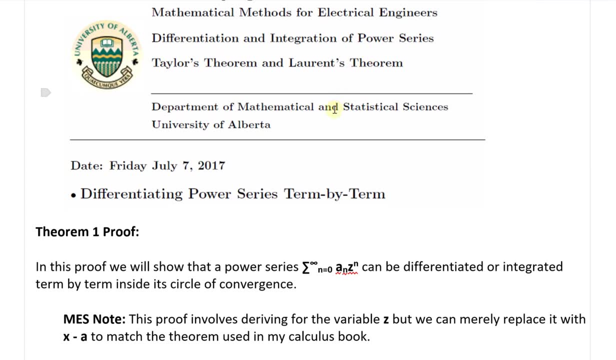 not just math but all of science, including electrical engineering, because it just simplifies calculations, yes, of uh functions and so on. so, uh differentiation, integration of power series, taylor's theorem- this also goes over there, but i'm not going to go over this- and it's department. 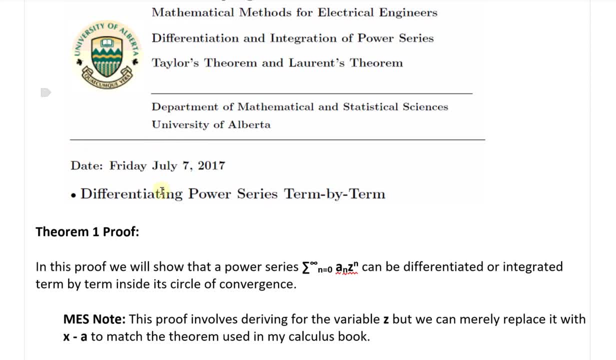 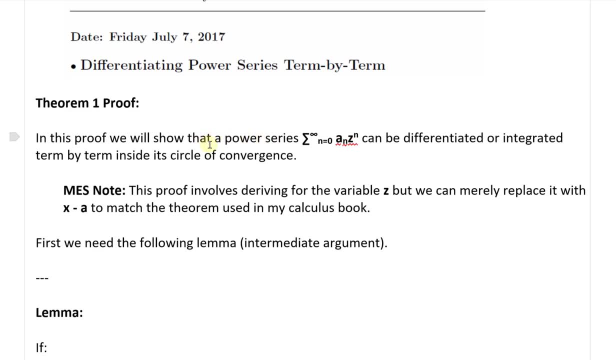 of mathematical and statistical sciences, university of alberta. and this is friday, july 7th 2017. so differentiating power series term by term. so let's look at theorem, one proof. so in this proof, we will show that a power series, or this uh summation n, equals zero to infinity of a and z and can be: 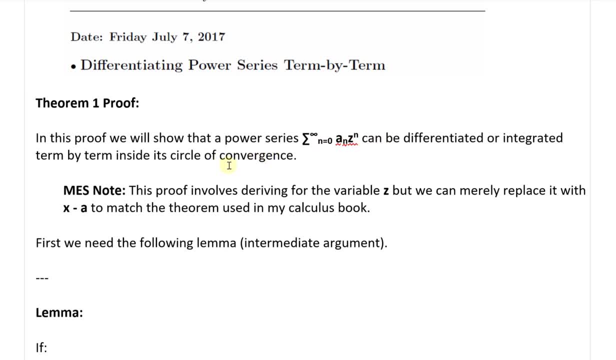 differentiated or integrated term by term inside its circle of convergence. and uh, yeah, just a mes note. this proof involves deriving for the variable z, but we can merely replace it with uh, x minus a. uh, let's pull this uh to match the theorem using my calculus book, and it's gonna be the exact same. 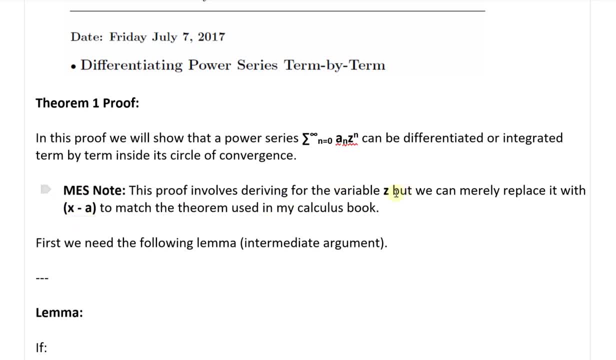 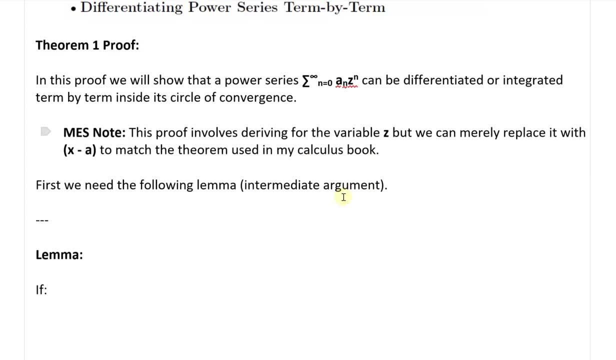 things. when you take an integral derivative of this, it's gonna be uh, the same thing as uh z. when x minus a is just gonna be one derivative of z, it's gonna be one. so it's gonna be, it's the same thing. so this is uh. you can just replace that. let z equals x minus a, and so on. so anyways, just to. 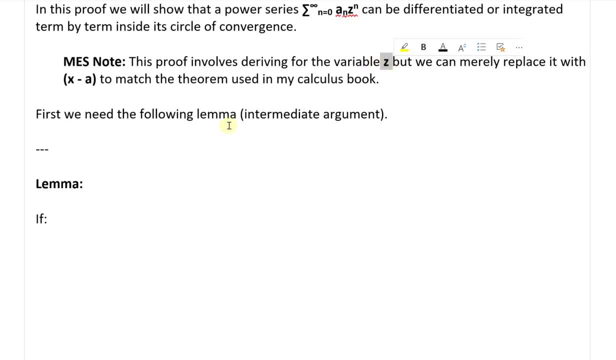 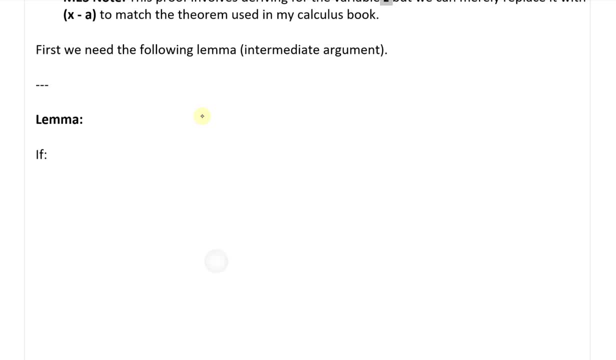 let you know. the proof uses this. so first, uh, we need the following: uh lemma or or uh intermediate argument, just what it means. so we'll use this first and uh. this lemma states: if we have, uh, the series or the summation, n equals zero. up to and from n equals uh zero. summation from n equals zero. 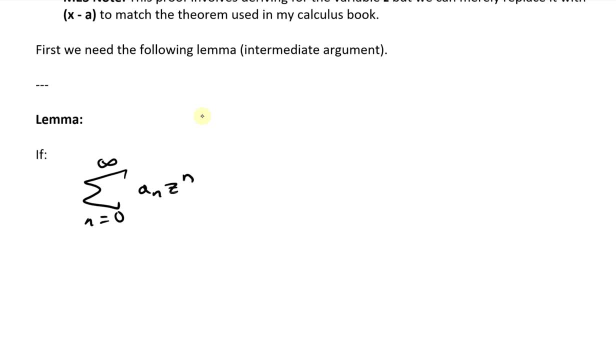 to infinity of a and z. n. yeah, so this first lemma. so if this series has a radius of convergence r which is greater than zero, then the following series: uh, right here, uh, this is if we have. uh, the summation from n equals to zero up to n. a. uh, yeah, n a n z. let's just take the derivative. 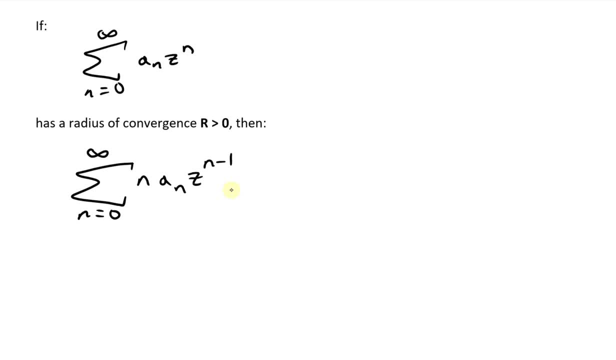 bring it down to z and minus uh yeah and minus uh one. and now words: this is uh, i, e, uh the derivative, or just write this down: yeah, so this function right here, this is just a derivative derivative, and here uh, next one here, and this series which writing it. 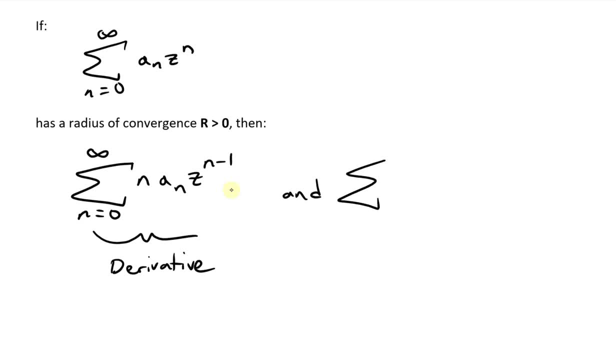 like this: uh, because, yeah, these are the integral derivatives, but we got to prove that we can do this, so let's write these. here's then the following series and then following series. this is a and z. now here, take the integral n plus one divided by uh, yeah, divided by n plus one, like that, uh, in other, 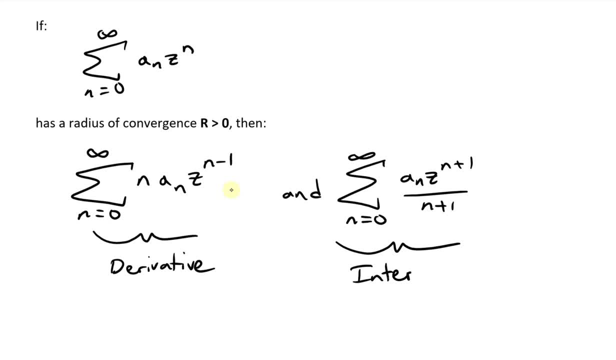 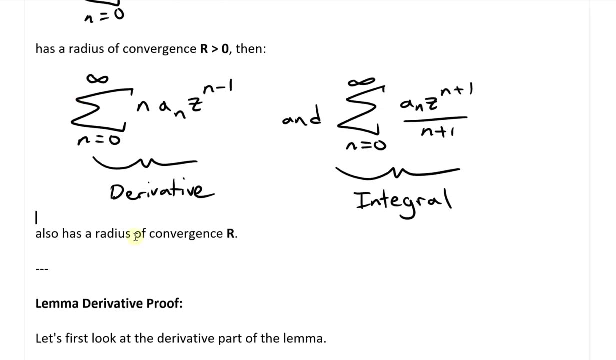 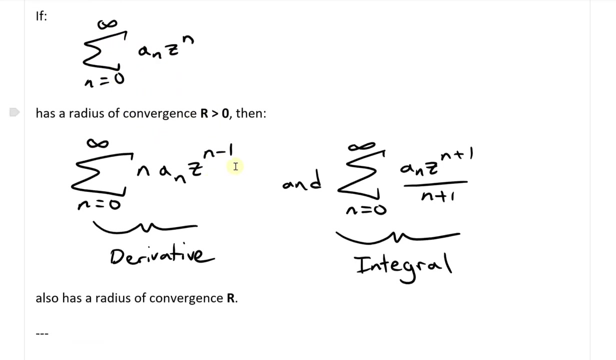 words. this is the integral, the integral part into, yeah, integral right here. yeah, i'm just spelling wrong. this is a g r a l. yeah, so this lemma uh states that, uh, if we have this series a and z n has a radius of convergence r is greater than than zero, then the series, this one, right here. 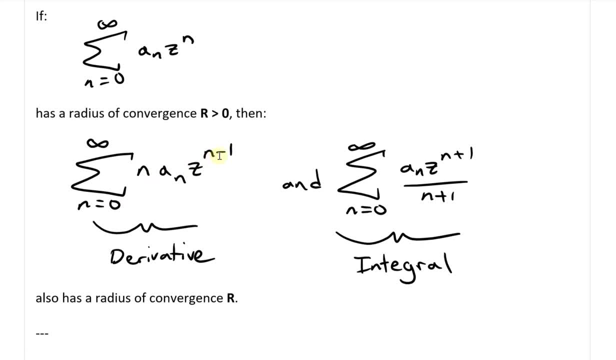 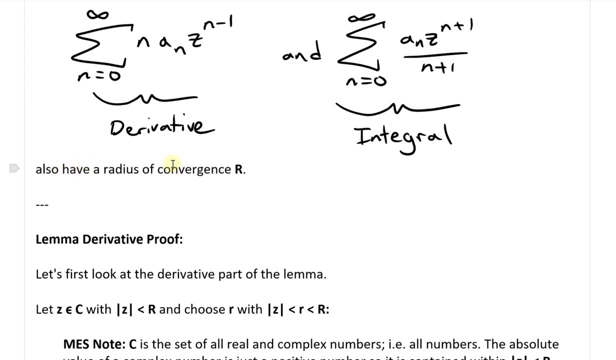 of n times a, n z, n to the power of, i mean z to the power of n minus one, and the series with the terms a, n z, n plus one. uh divided by n plus one, also, uh has a radius of convergence, or also have, yeah, a radius of convergence. r, and this is again part of theorem one, but let's just 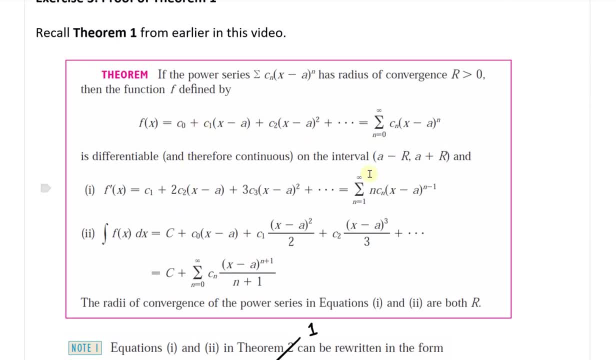 prove this theorem or a part. prove this part of the theorem. so if differential and has a radius convergence r right there and then then, uh, then case one and two, or i and double i also are both r. so that's our lemma. before we prove the whole theorem that you can take term by term. 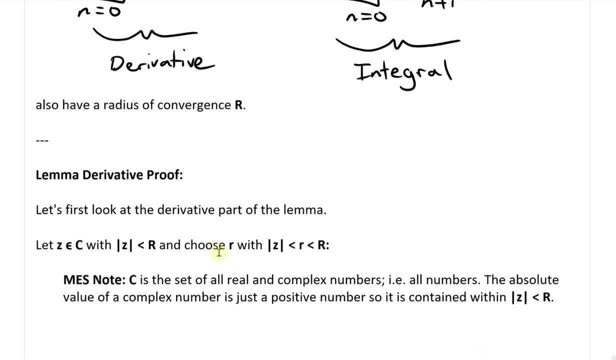 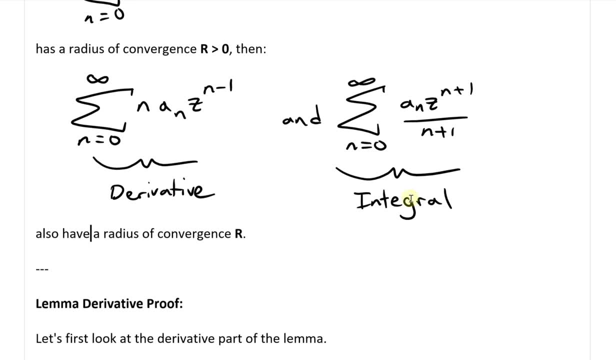 derivatives. so let's first prove this. so, uh, lemma: derivative proof. so for let's first, uh, look at the derivative part of the lemma, which is this: this uh part. here i'm just going to categorize this derivative as integral and integral, just because that is what they are, uh, anyway. so let's first. 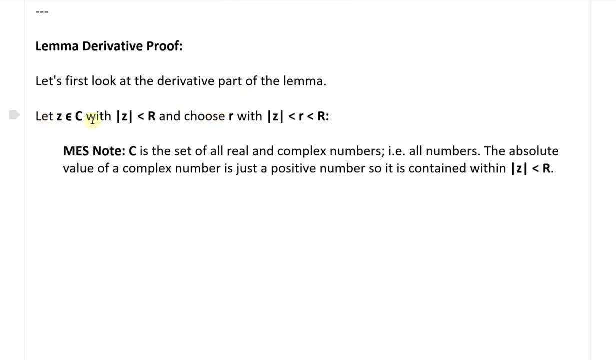 look at that. let's let z be an element of c and mes node. c is the set of all real and complex numbers. it's also, it's actually uh, written. it's uh, it's actually written like this, uh, like that, i think something like that. yeah, it's actually. 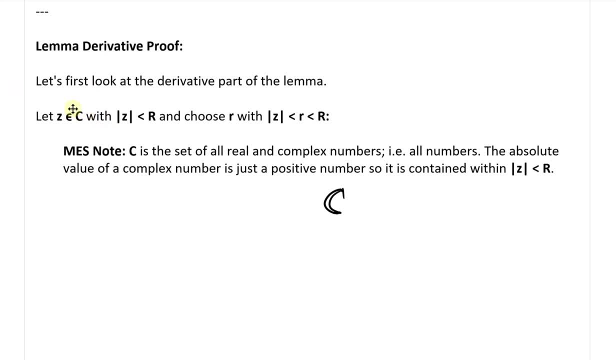 written like that, but uh yeah, i didn't bother checking if there's an actual symbol for that and i'll just use c instead. it's better, just like when i use my element of all real numbers are. so in this case, uh yeah, it's just going to be a set of all real and complex numbers, ie all numbers. 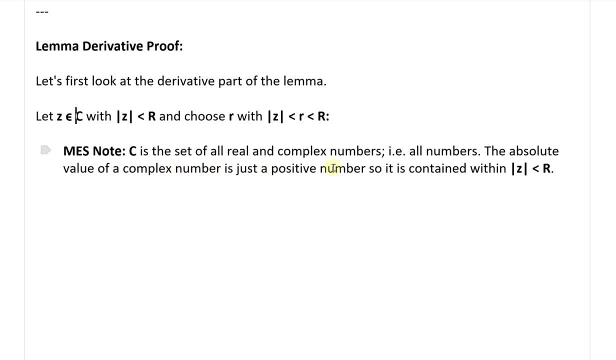 and then the absolute value, of the absolute value of a complex number, of a complex number, is just a positive number, so it is contained within over here. this uh absolute value of x is less than r, and uh, yeah, that complex numbers and stuff, uh and uh, the square of the, i mean the uh absolute value. 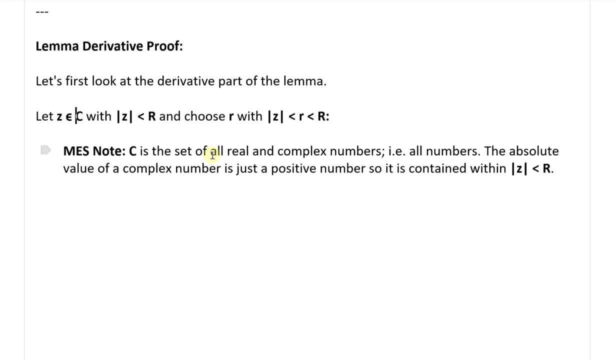 of them are for another video, for another day. i believe that that's a bit beyond what i've covered so far, but anyways, uh, this is all contained within this, so let's see be an element of all numbers, all real and complex numbers: c, uh, with absolute value of z. 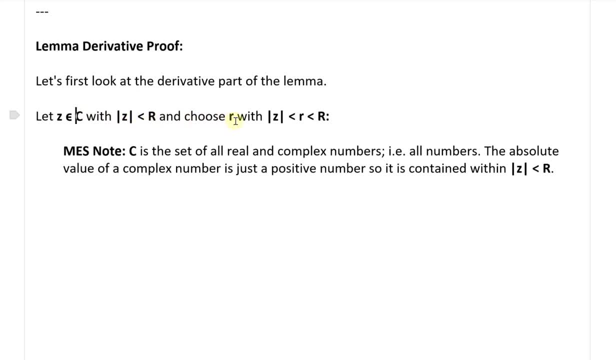 is less than the radius of convergence, r, and choose r a little r, with absolute value of z is less than r, little r, which is less than capital r, which is the radius from convergence. then what we could do is what we could do is let's let's start off with the derivative part. so let's look at this. 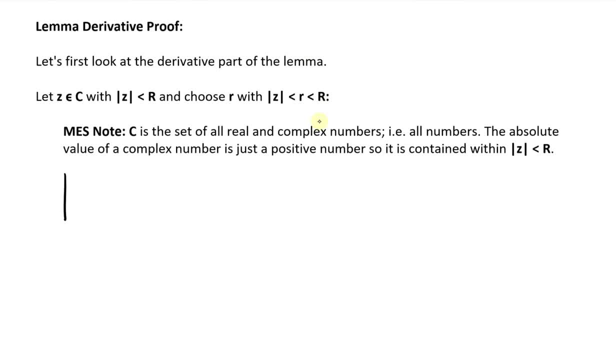 term n a n z uh n power of z to the power of n minus one. so we'll write the absolute value of this. remember, absolute value is always useful because we could take absolute convergence. so, and then which? which proves which? uh implies the convergence whenever we deal with series. so let's look at uh. absolute value of n times an. 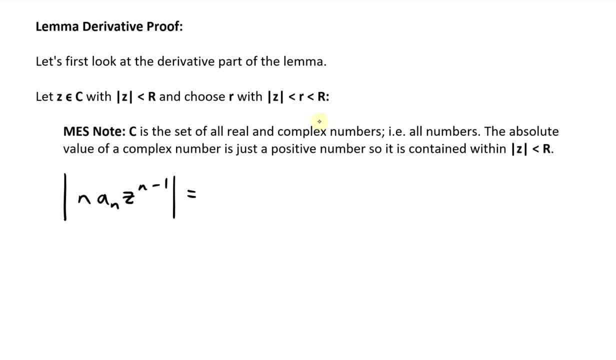 z to power of n minus one. now, this equals two. yeah, this equals two. and what, my what the pdf proof does? uh, it does this. so it does, uh n abs the value of n times a n o n minus 1. then what it does? it multiplies the top and bottom by r to power of n minus one, or little r power n minus. 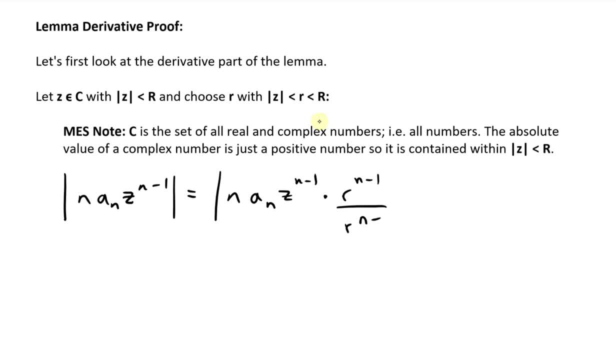 1 and then divided by: yeah, top and bottom by one, and that's two and that's one. well, if we go to the, so it times it by r, and r to the n minus 1. divided by r to the n minus 1, yeah, so absolute value of. 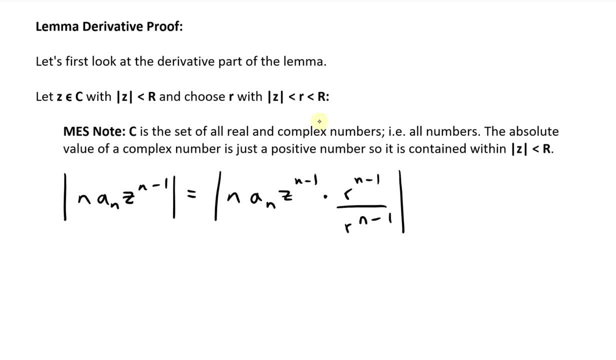 this. and now what this equals to. we can combine the z and this r together because of the same power, so we could do this: equals to n, a, n, and then this is going to combine these z with the denominator there r. so that's why we had the same power, and this will start to make sense as i go. 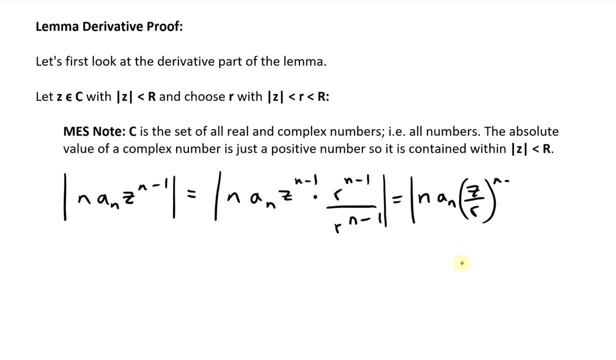 through it and then, and then, yeah, just write this n minus 1, and then over here we get what we can actually do with this r and minus 1, where i'll just write this down first actually just write it down, do it afterwards absolute value, like that, and then this part right here: r to the. 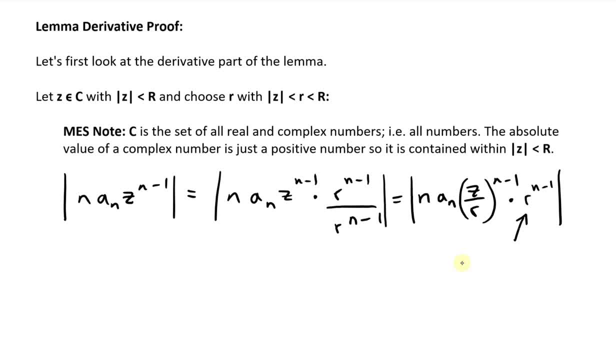 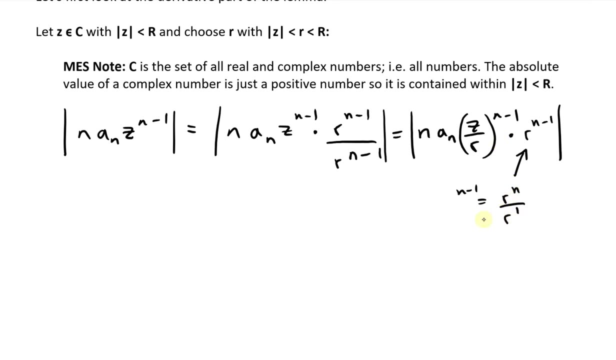 n minus 1, this just equals to uh. right here, r n minus 1 equals to r n divided by r 1, because when you subtract the powers uh over, when you combine these, it's same same base is gonna be our n minus 1, so that's the same thing there. so now, 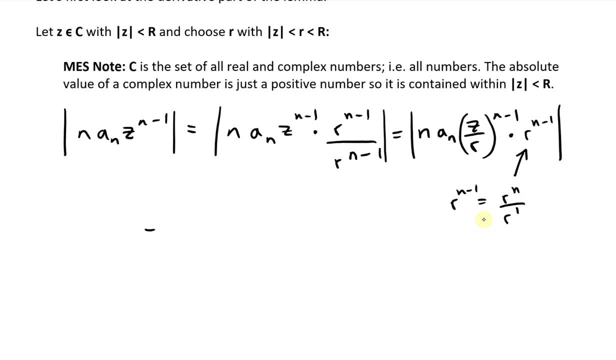 what we could do. what we could do is now this equals 2 and just simplifies: move this R over to here, so we'll have an N over R, a n actually afterwards I'll put this in front: Z over R and minus 1. then move this a n to the other side and then 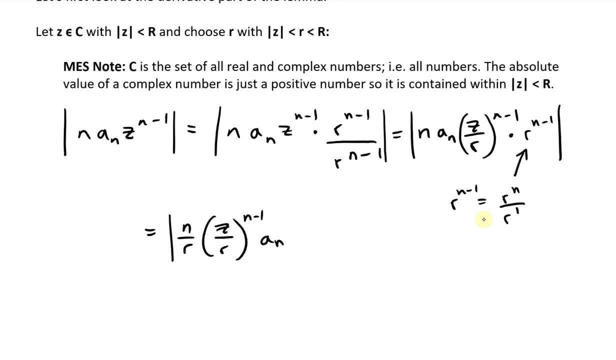 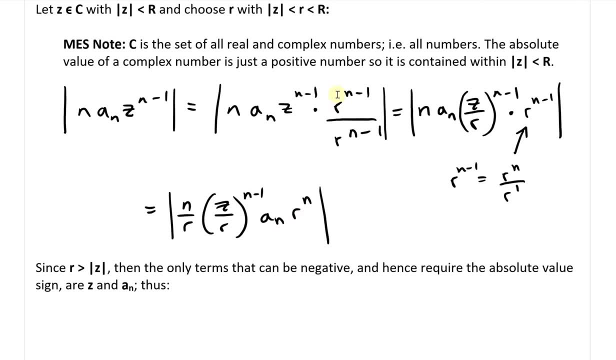 we're gonna get an R n, so we're gonna have a n R n like that, and move it over there, and, effectively, what we're trying to do is: well, we know that R is greater than an absolute value of Z, so then, this R, we're trying to make it a form of this. 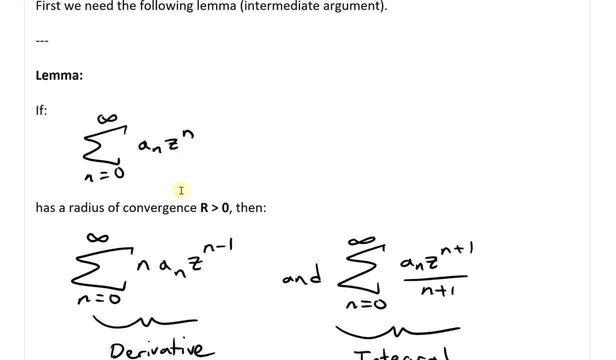 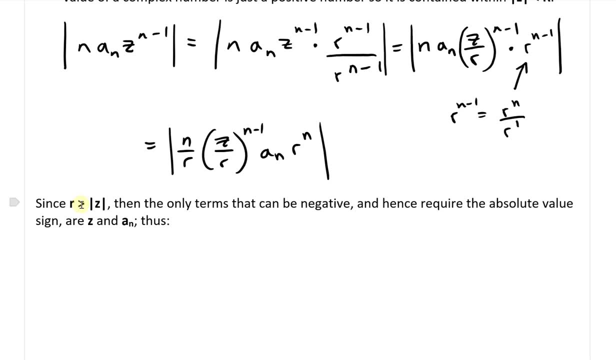 earlier function a and Z, and but now we're gonna have a, n, R, n, so that's what we're gonna do. and now, since R is greater than the absolute value of Z, in other words, it's gonna be always positive- then the only terms that can: 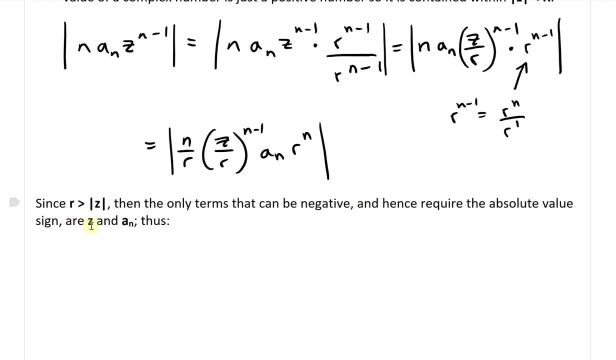 be used are the ones that are positive, and the only terms that can be used are can be negative and hence require the absolute value sine R, Z, so this one could be negative. the R is always gonna be positive and the and the a, n the coefficients, so those coefficients can't be negative, so we have to absolute value. 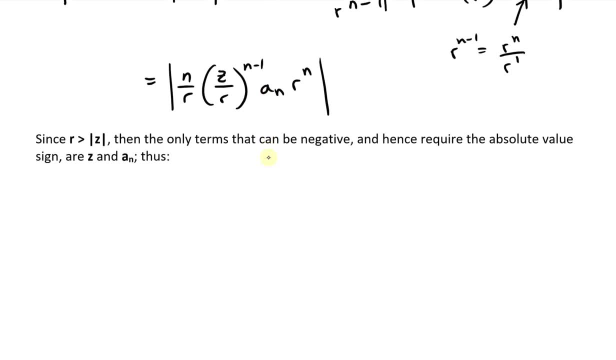 of them. so what happens is, you know, we could write this top part there. now this is gonna equal to: this is just this part. so now it's gonna equal to n over R times it, by absolute value of Z over R. power of n minus 1. 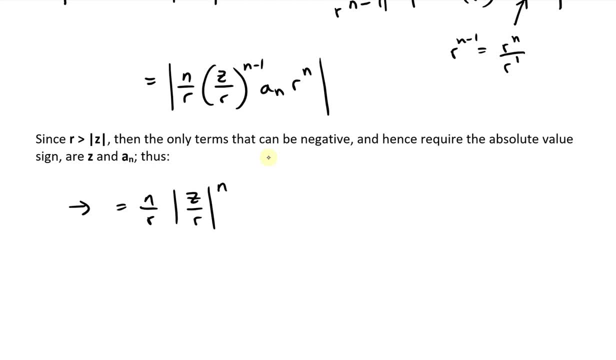 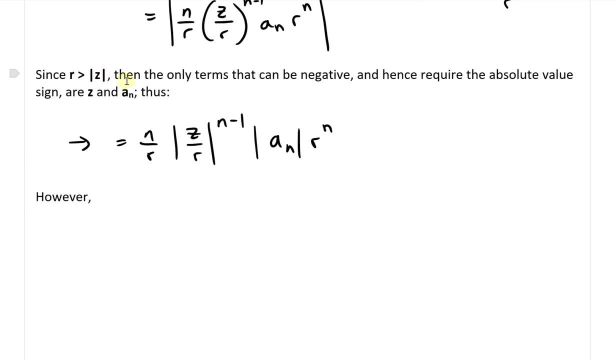 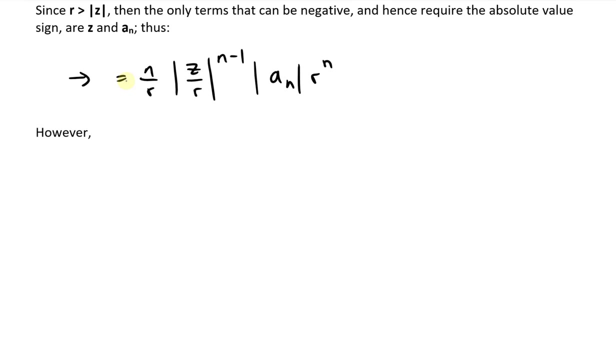 like that. and then we also have absolute value of a n times it by R n. alright, so now, however, notice what we have here is this part right here, and we can ignore this R radio or my. the PDF proof ignores R and what I'm about to do, just because it will be a constant for whatever value it is when. 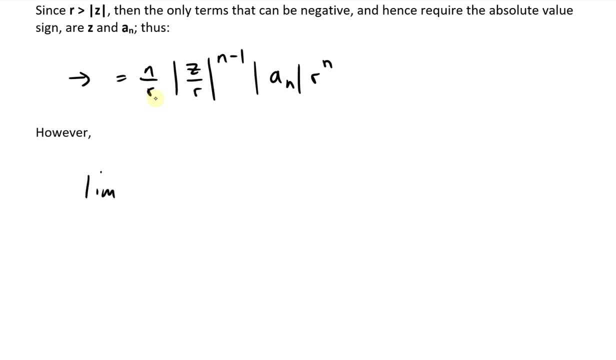 we do a limit. however, if we take a limit, so notice what we're gonna have. so if we take a limit and a approaches infinity of this first term, ignoring r, because you'll just factor it out, so if you had r, just put it over there, etc. so just leave it up. so now we have n times z over r and then 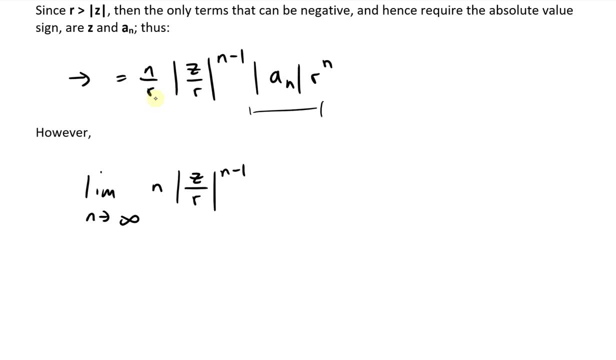 n minus 1. so we ignore this a, this term right here, just ignore that. so the limit of this one this is going to equal to. that's a very interesting uh derivation technique. so so what my, the pdf proof does in this part of the proof, so what it's going to do is this is equal to n. now this part. 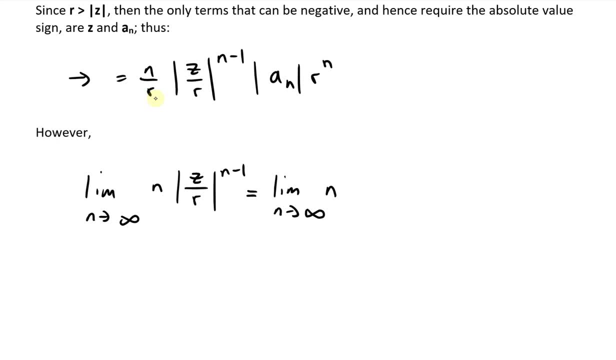 here it wants. what you could do is take the exponential and we'll take the logarithm, natural log of this or the lawn, and then take it to the exponential power. so what we'll do is e to the lawn. so we're not changing anything, because e to the lawn will just cancel and we're just left with. 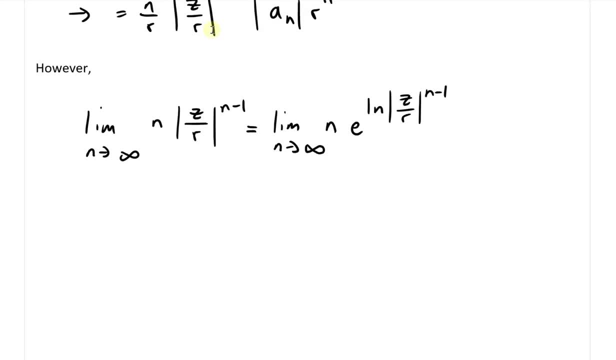 this part right here of n minus 1, like that. so, yes, i'll recall the you natural log rules or just logarithmic rules. this would cancel and uh, this would go. yeah, this would cancel. just have, uh, exactly, uh, this right here, but what we could do here now, because taking the 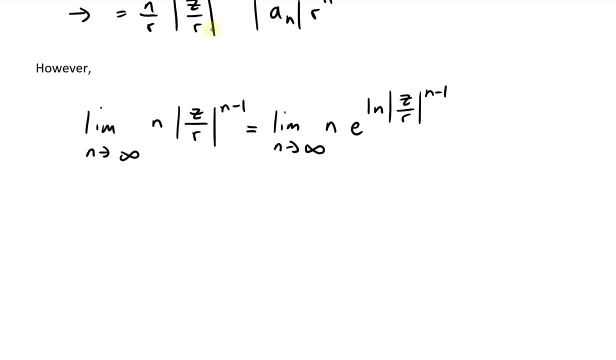 power of this to natural log. we can move this downwards. so this equals to: yeah, so i'll just write it here. this equals to the limit as n approaches infinity of n, and now we're going to have a e to the, and then we can bring that in that power. uh, yeah, so now, with this one down, we just 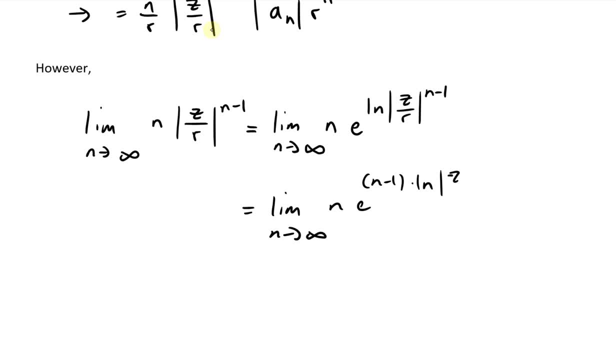 have the multiply, the top and the power there, by absolute value of z over r. and now, since absolute value of z is less than r, then what we end up having is this absolute value right here, absolute value of z divided by r, which is going to equal to just absolute value of z divided by r, because 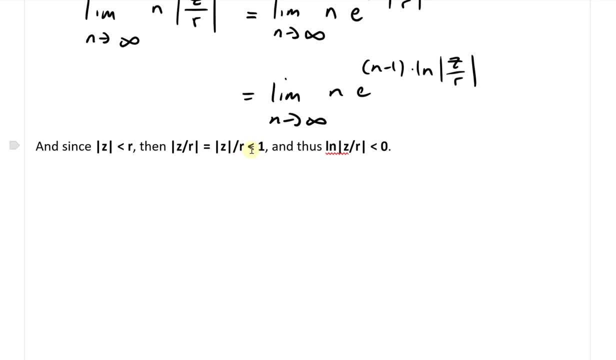 it's always positive anyways, this is going to be less than one, since this r is greater than this absolute value of z, as we had it defined there. so r is less than one, and then we're going to have: this is greater than this. so now though? now, what we have is: so thus lawn so dictionary, so lawn of. 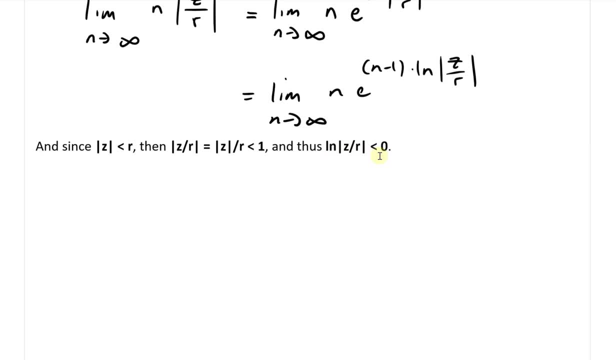 absolute value of Z over R, this is gonna be less than zero. and this is again. just recall the logarithmic chart. yes, if you recall, the logarithmic charge looks something like this: we have move it over here, so it's gonna be. if this is X, this is gonna be our lawn of X for the Y, so it's gonna. 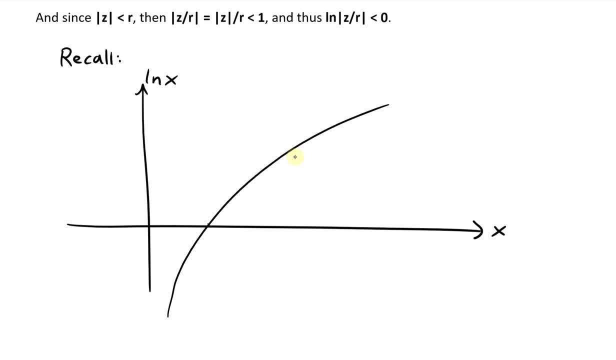 look something like this, where it goes like that, and this part right here at this point is: this is our one, so when it equals to one, it's the lawn of X is zero. yeah, so thus, at this point, just recall what it looks like over here. so let's just scroll up here just for reference. so at this, 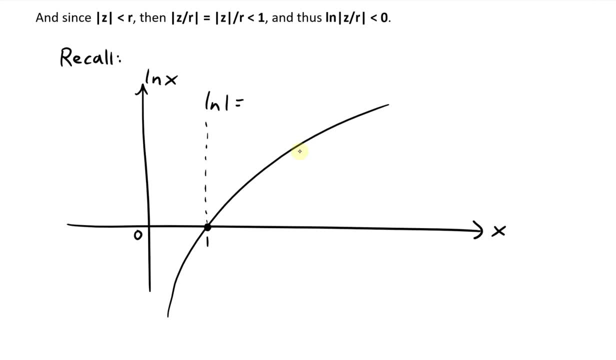 point we have: lawn of one is equal to zero and the same way as writing is. it's just an inverse function. so it's the same way as writing e to the zero, because that's the lawn is just log, log, base e. so this is: e to the zero equals to, well, one and the same thing is writing: lawn of one equals to. 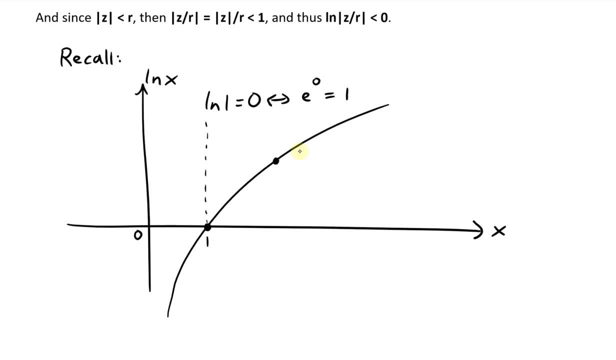 zero. and also just for further reference at this point right here, this would go up to e, and then this value is going to be one. so they- these are, there's X and y-axis are not different to scale, but anyways, we have it like that. this is all the way across there. and then, at this point, 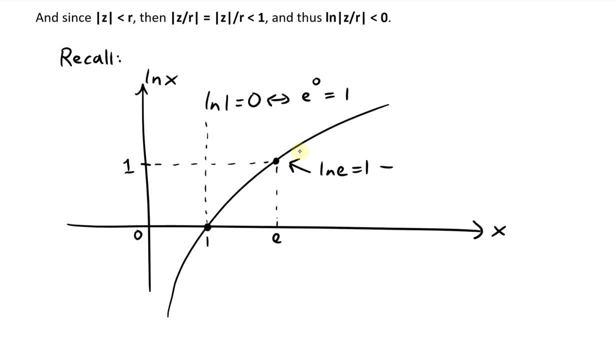 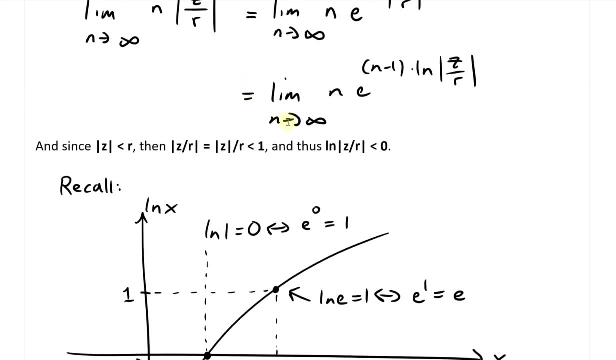 right here lawn, e equals to one, or same way as writing e to the one equals to e. yeah so, anyway, so I digress. so, since this absolute value of Z divided by R is less than one, that means well, that means it's going to be less than this value. 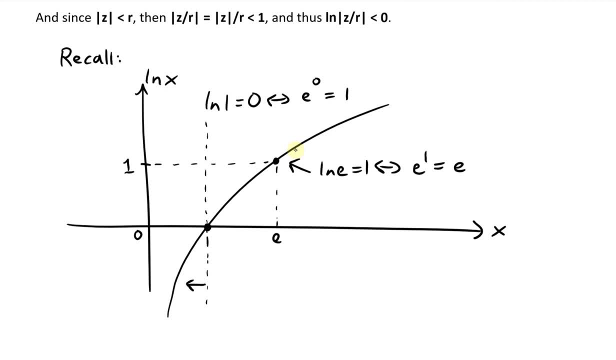 so let's scroll it all the way down. it means it's going to be to the left here, so this is negative. so what we have is negative values right here, or better yet. yeah, so it's going to be to the left of this, so we're going to have negative values. 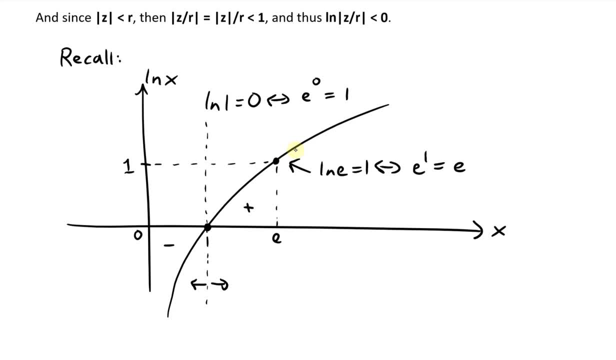 as opposed to if you were to the right of this. we get positive values, so those are all positive, but here we're going to get everything's going to be negative. yeah, so thus, what we have is thus: lon of Z over R is going to be less than zero. yes, so thus, if it's less than zero, then if we take this limit right here, let's start. 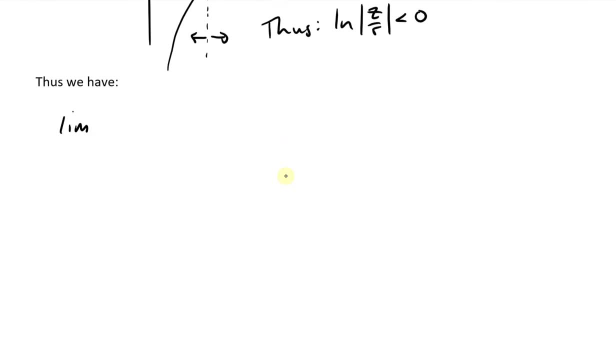 off there. so thus we have the limit, as n approaches infinity, of n over e to the n minus 1. this is going to be lon absolute value of Z over R. that's just this part, this, this, all this term, right right over there. but since this is going to be less than zero, we could just take the absolute value of this. 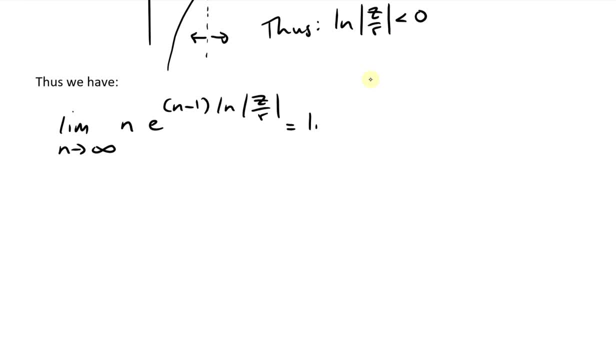 and move it below this function. so this is going to equal to the limit, as n approaches infinity, of n. I'll just write this as: yeah, let's write n over here, divided by e to the n minus 1. so now that, yeah, this n minus 1 is always going to be, yeah, the n minus 1 is always going to be positive when we 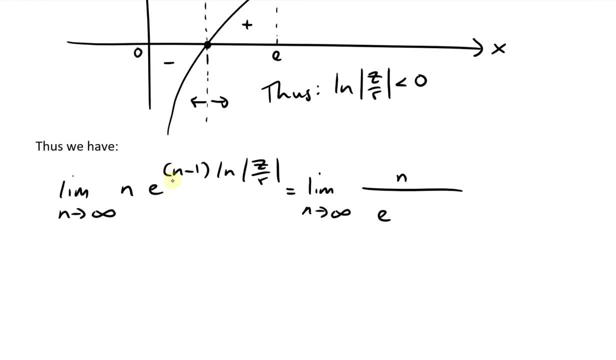 have n is 1 or greater. if n is 0, well, this is gonna be 0, that's, this all goes to 0. so when this is equal to 0, and that'll just all make it 0, but when it's greater than 0 is always gonna be. 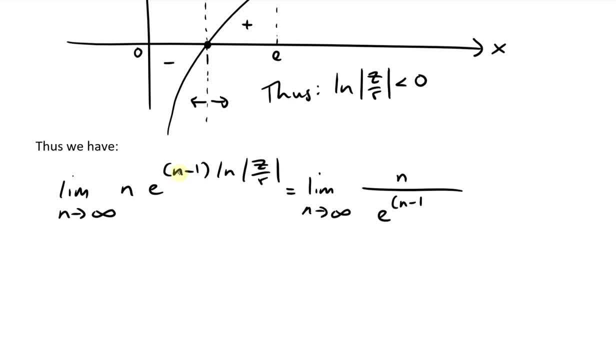 positive. so for our case, this is: yeah, it's always gonna be positive, because when n is 0- that's trivial- the whole, all the whole series can be 0 because of the sand, but anyway. so this is going to be. we're going to make this at the bottom, and then we take the absolute value of lon and then 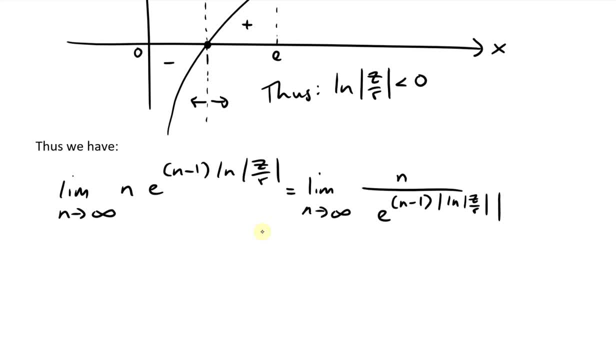 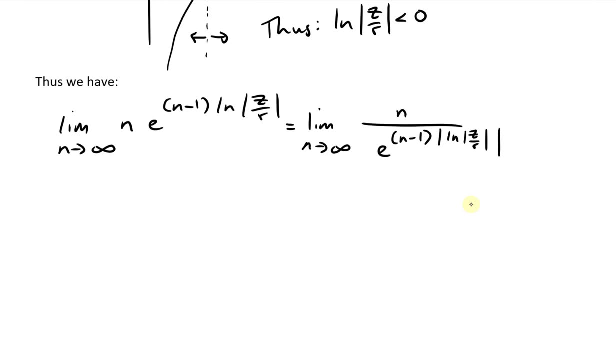 absolute value of the inside, Z over R, like that. so now we have two absolute values, but this one's below it, because this is always going to be negative. so this inside lon of absolute value of Z over R, those can be negative and since it's the power we're gonna, we can just flip it out at the bottom and make it a positive, like that. so 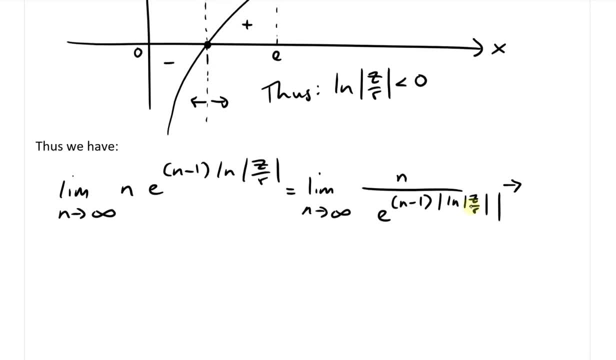 now, when you take the limit here, this, what we're gonna get is a scenario where n approaches infinity and then, divided by the bottom- well, this, right here, lon Z over R, the absolute value of it, is just going to infinity, as you can see here. just going to infinity, and then this e to the n minus. 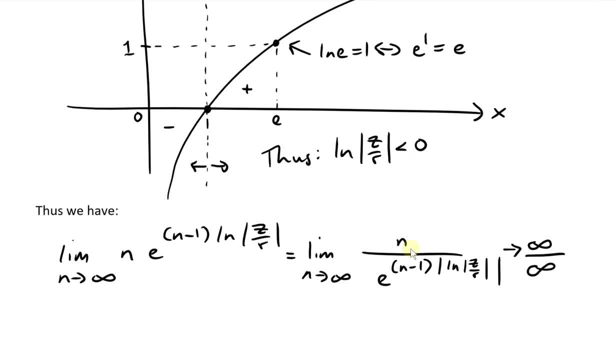 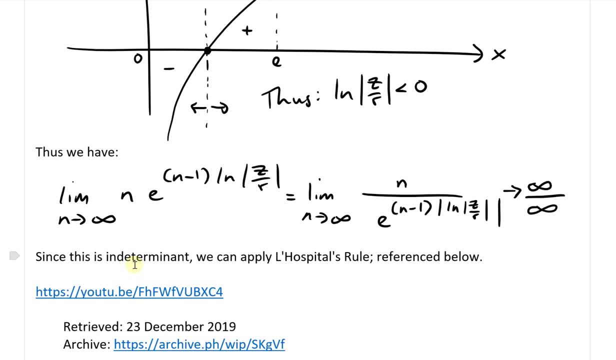 1 is also going to finish, so we'll have an e to the infinity, which is just infinity, and yeah, so this infinity over infinity that's not defined or that's indeterminate. so, since this is indeterminate, we can't determine whether it converges or not, because it's a infinity divided. 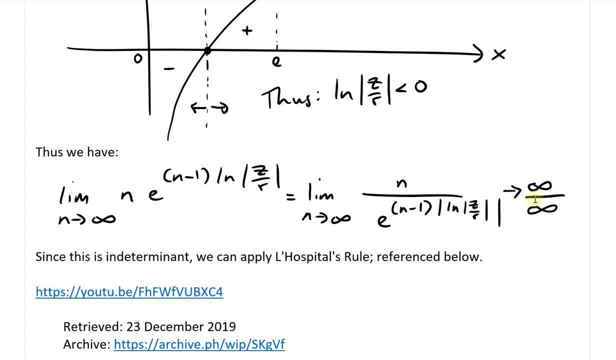 by infinity. basically, we're trying to see which infinity is going faster, yeah, which one's increasing faster: the the bottom or the top? it's the top, then it's going to be approaching, approaching infinity. if it's a bottom, then it should be. it could be approaching a limit, or 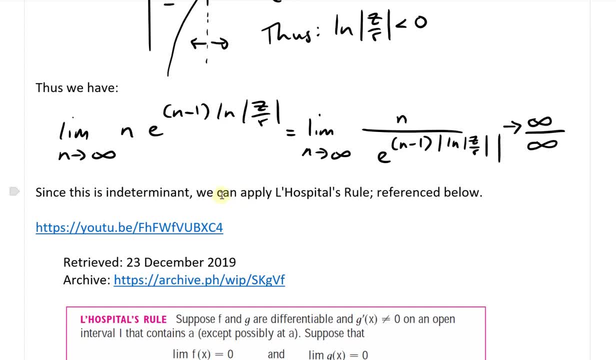 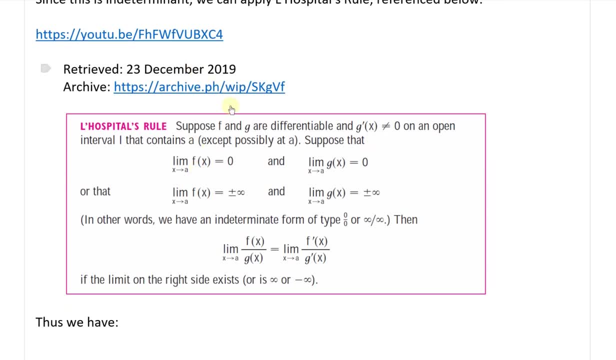 zero. so since this is, since this is indeterminate, we can apply the hoppy tells rule referring to below. so yes, so recall this from earlier video. so hoppy tells rule, suppose F and G are differentiable equations and or functions and the derivative of G of X is not equal to 0 on an open interval. 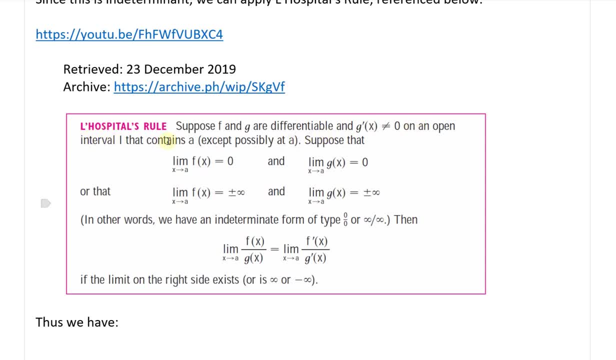 the open interval I that contains a, except possibly at a, does not be a differentiable at that. I mean, it doesn't have to not equal to 0 at that point, as long as the limit it doesn't, or I mean the other point near it's on an open interval that contains a, except possibly at a. so suppose, 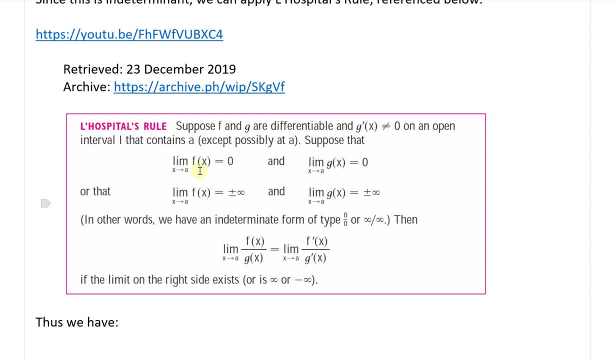 that the limit as X approaches a of f of X equals 0 and limit as X approaches a of G of X equals to 0. yeah, or that the limit as X X approaches a of FX equals plus minus infinity and limit as X approaches a of G of X equals to plus or minus infinity. in other words, we have an indeterminate. 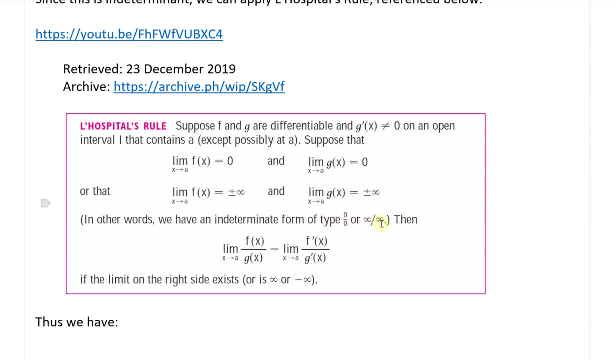 form of yeah, of type zero, zero over zero, or or infinity over infinity, the limit as X approaches a of FX over G of X. so if we have any of these scenarios where you have, yes, 0 over 0 or infinity of infinity, then then what we could do is take the limit. so then limit. 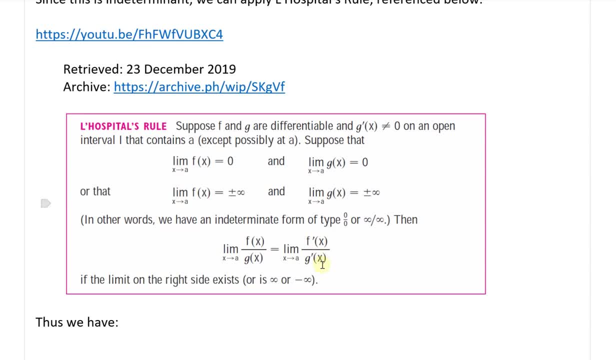 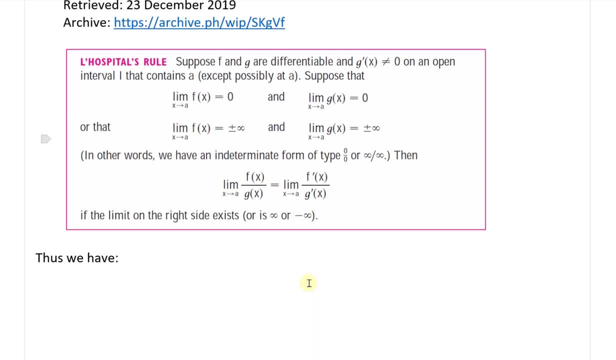 as exports a of F prime of X over G prime of X, if the limit on the right exists or is infinity or negative infinity. yes, in other words, we could take the derivative. so that's essentially the hoppy tells rule. when you have this indeterminate form- and this is again- 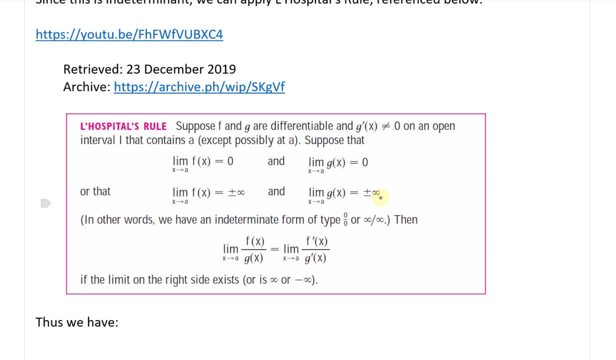 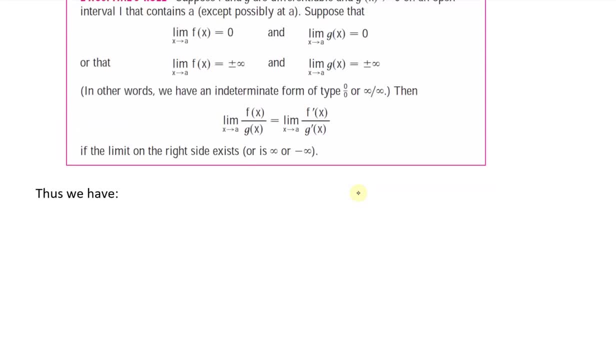 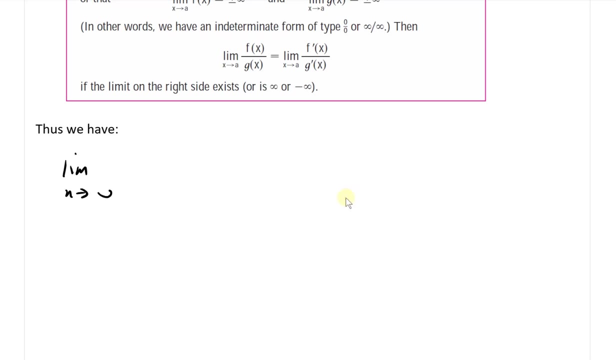 where the derivative at the denominator it does not equal zero. so that, yes, so that if it's dividing by zero can have an as infinity scenario anyway. so that's what we have is the limit as, yes, the limit as n approaches infinity, of d over d n, and this is gonna be our n, so that's d over d n of. 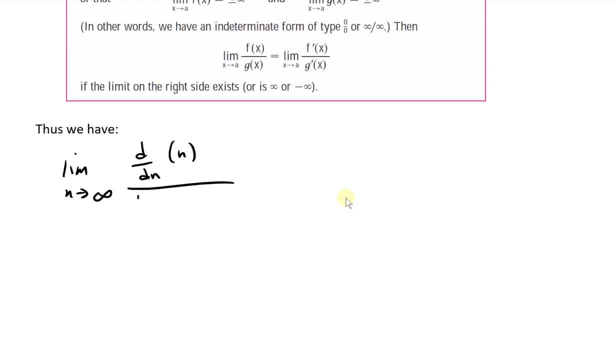 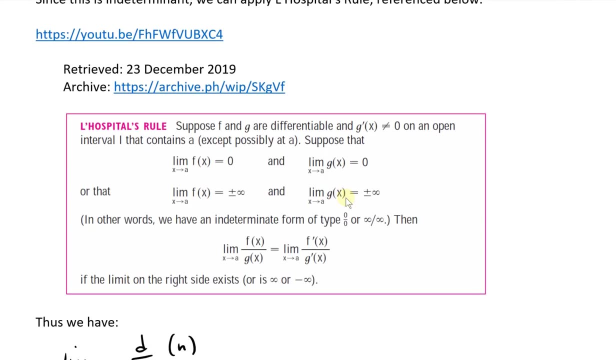 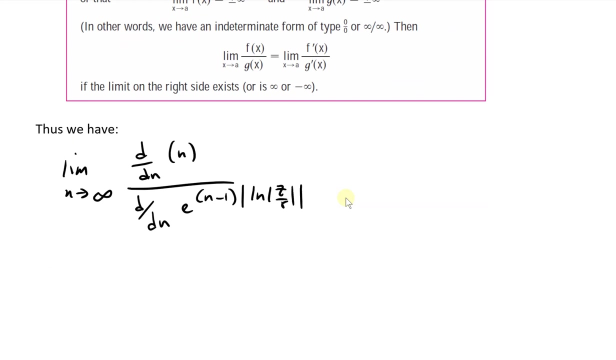 this one, and then divide this by D over D, end 3 of this big giant one, e to the n, minus 1 times epsilon value of yeah, ln, epsilon value of z, epsilon value of ln, epsilon value of z over r. just so it's all positive there. 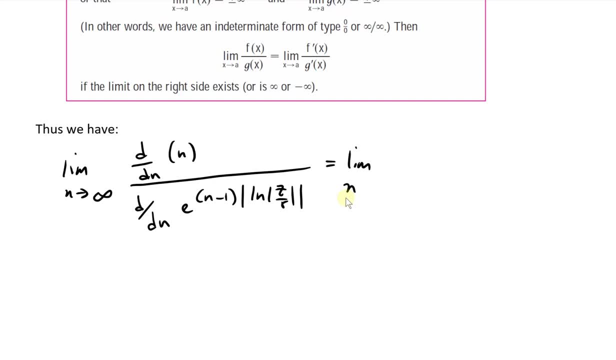 So now, if we take the derivative, this just equals to limit, as n approaches infinity, And the derivative in terms of n on this one n is just 1.. Then the bottom right here, what ends up happening is: so what we're going to have is this: this is e to the n minus 1,. 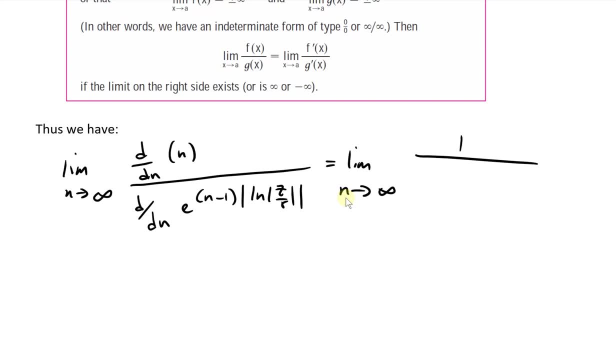 and this one's not based on e, so that could be viewed as a constant. So then the derivative is just going to be itself and then bring it down, so using chain rule. So then this just goes down and we're going to end up with a epsilon value of ln. 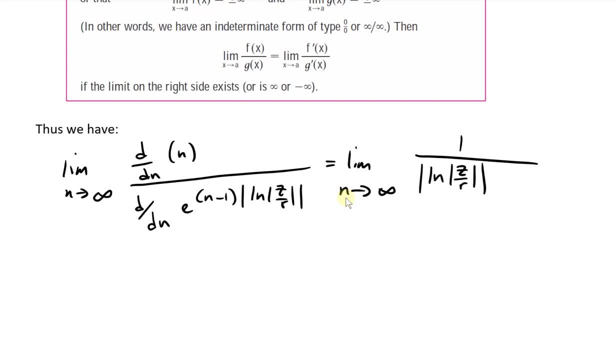 epsilon value of z over r, epsilon value like that, e, and then this is going to be n minus 1, and then this is going to be e to the n minus 1, and then this is going to be n minus 1,. 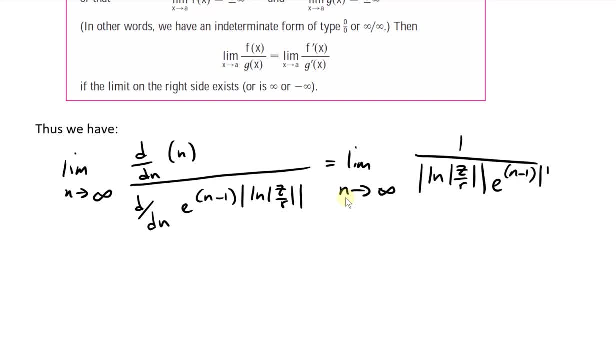 yeah, n minus 1, and then epsilon value of ln, epsilon value of z over r, like that. All right. so now this scenario: well, this is all just positive at the bottom. and then this ln, this z of r. this is approaching infinity. 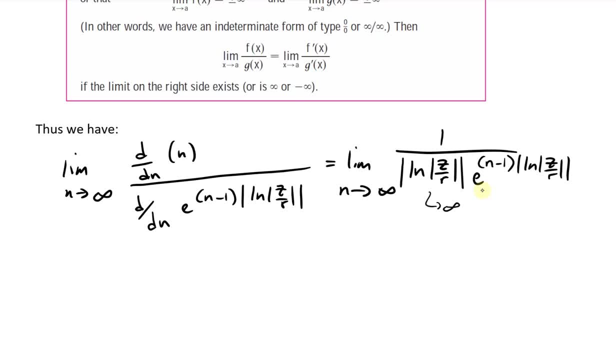 So this is approaching infinity. and then this right here is going to be: yeah, this is approaching infinity, this right here, this whole thing's e to the infinity, that's just infinity. So what we end up having- infinity times e to the infinity- is going to be infinity. 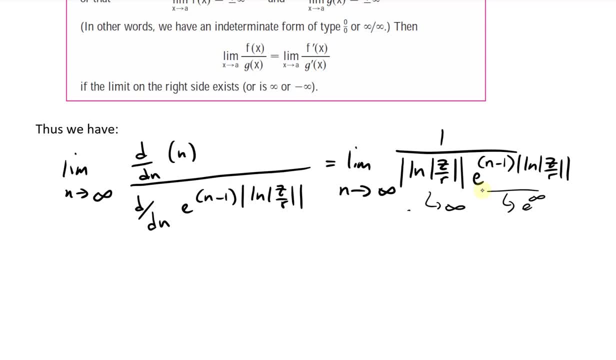 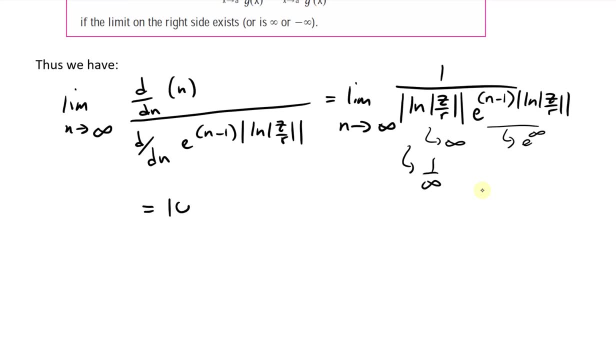 and then 1 divided by infinity is just going to be. well, we have a scenario of 1 divided by infinity. So, in other words, this whole thing equals to 0.. Let's box this out: yeah, 0,, like that. or let's write it better: 0, and then box it. 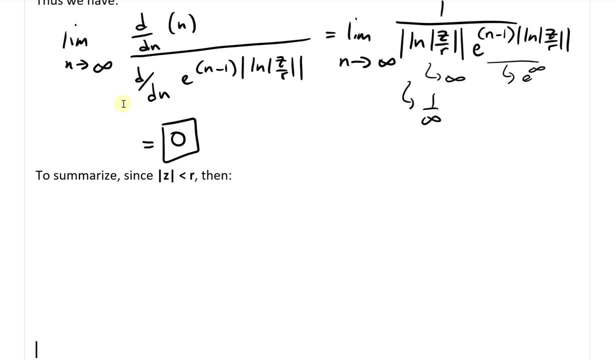 All right, so now to summarize, because that's a derivation within a derivation, within a lemma of a theorem. All right, so to summarize. since epsilon value of z is less than r, then what we have is well, we have a derivation of 1 divided by infinity. 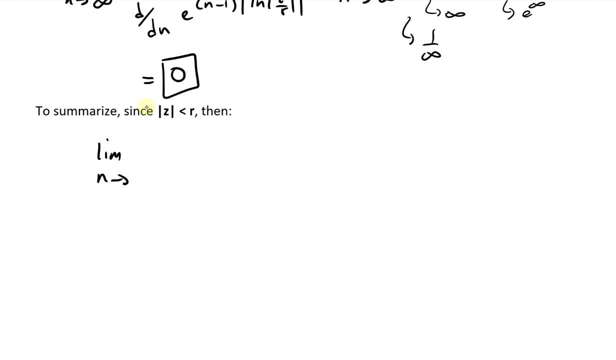 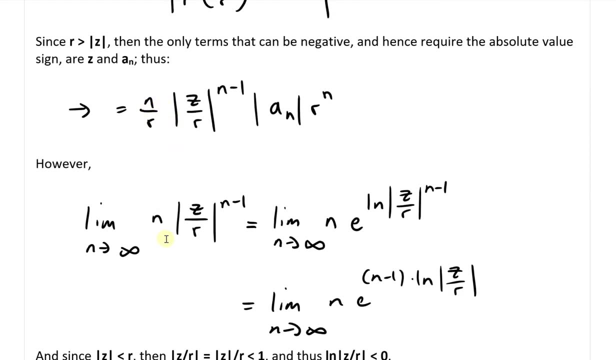 and what we have is the limit, as n approaches infinity, of the earlier limit that we were doing. and that earlier limit is just this one, right here, of n times epsilon value of z over r, then n minus 1, so that all equals to 0. 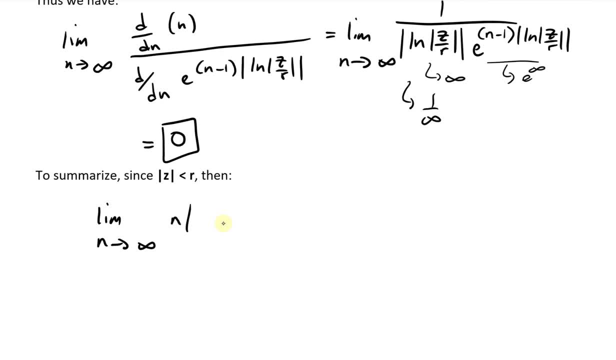 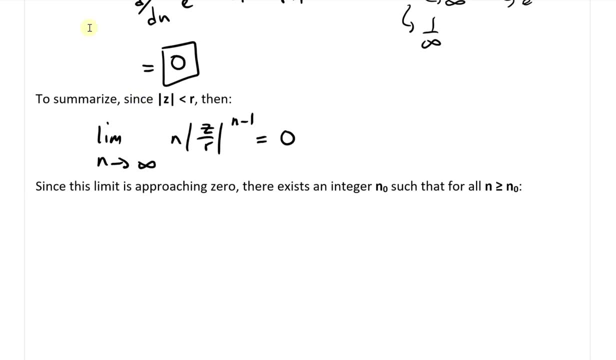 So this is going to be right here. n then z over r epsilon value of n minus 1, this equals to 0.. Yeah, so since this limit is approaching 0, there exists an integer n0, such that for all n greater than or equal to n0,. 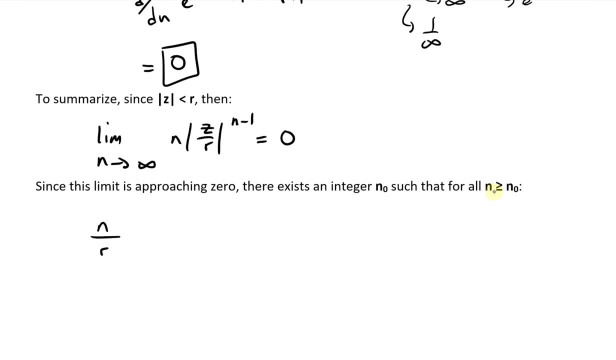 then we'll have this scenario: n over r of this is going to be epsilon. value of z over r, n minus 1 is going to be less than 1.. Yeah, this is for all. yeah, this is for all. n is greater than or equal to n0.. 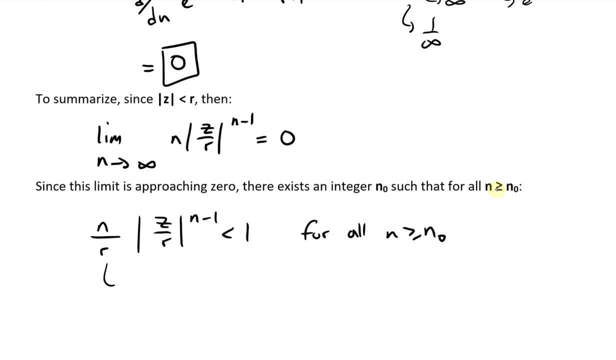 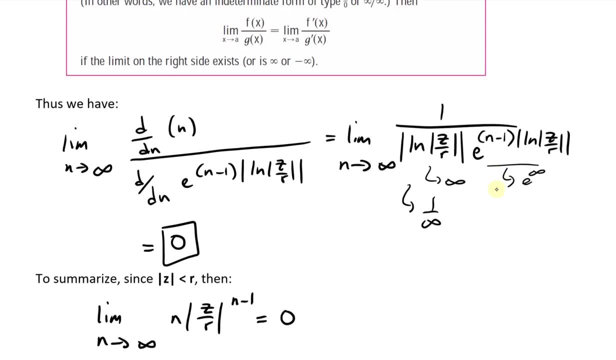 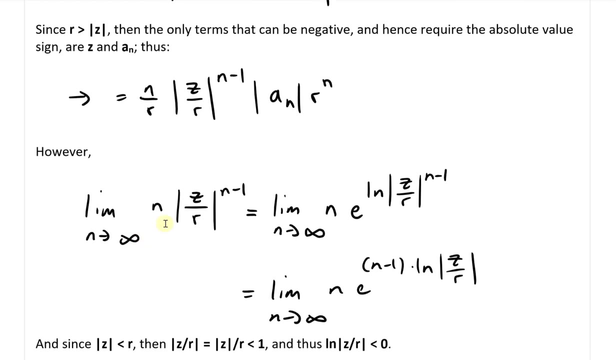 And again, this r r right here. this is just a constant. this r is just a constant that we defined earlier. and the reason we're putting it there is because, scrolling up, we had this scenario: so n over r. and then the PDF proof: just ignore the r there in the proof. 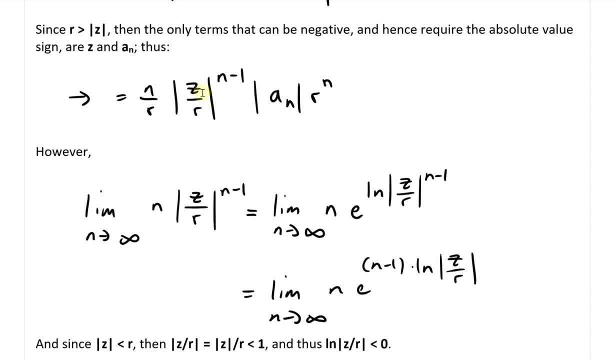 because it doesn't matter, it's just a constant. So what we're doing is essentially taking apart this and showing that this is going to be less than 1 for a specific number, n greater than and n0, or n0, and then we'll see what happens. 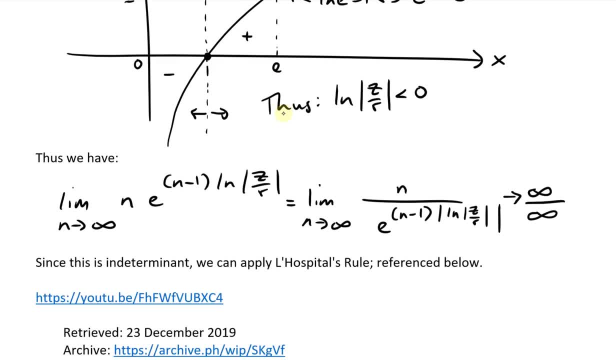 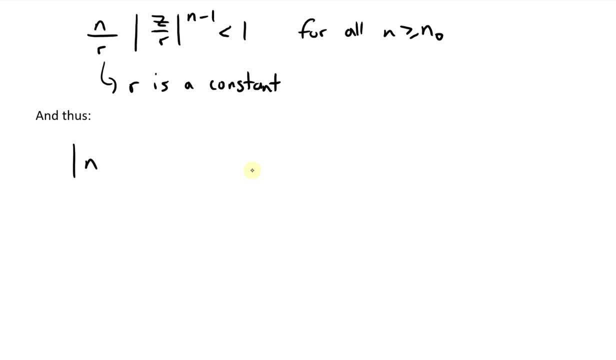 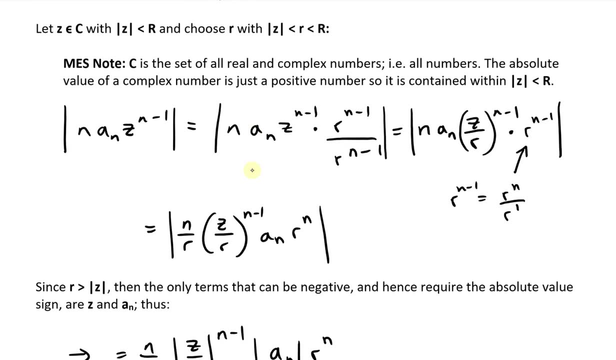 and we can use a comparison test, and, yeah, it should be making pretty self-evident soon. Yeah, so, and thus what we have is the absolute value of n, a, n, z to the power of n minus 1, and let's just scroll up what we have where we last showed that. 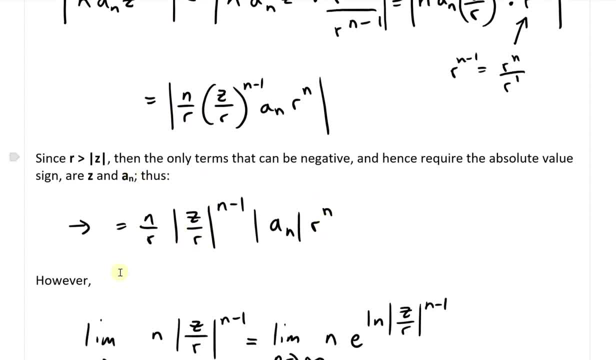 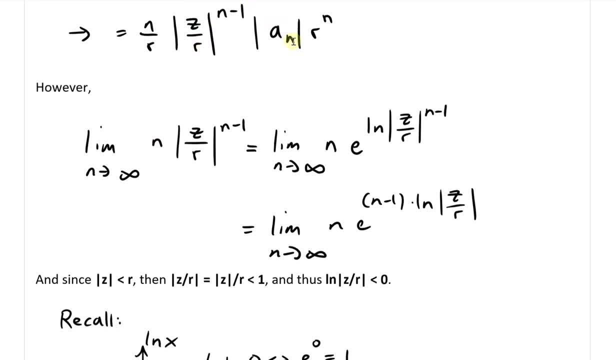 So that's this part right here. we showed that it equals to this part right here. So this: where it equals to n over r absolute value of z over r n minus 1, then we have absolute value of a n times r n. 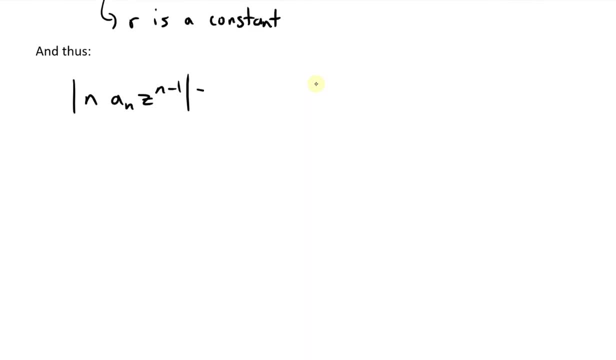 So let's go all the way here. So, where this equals to n over r times absolute value- which is exactly this part right here- z over r n minus 1, and then this equals to, or I mean multiplied by this: 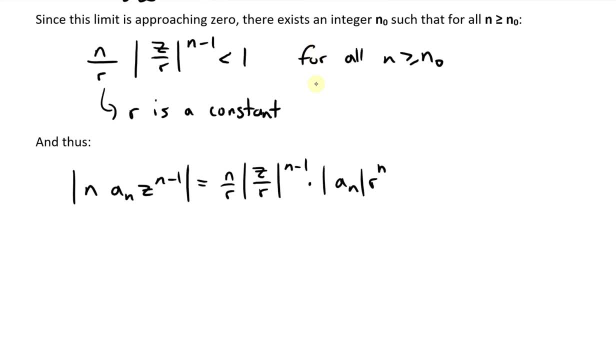 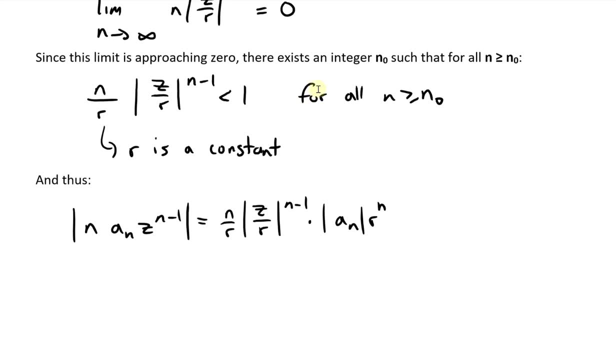 a n over r? n. So now what we have is: well, since this scenario- this one is for n- is greater than equal to n0, since this limit is approaching 0, this whole thing is going to be less than 1,. 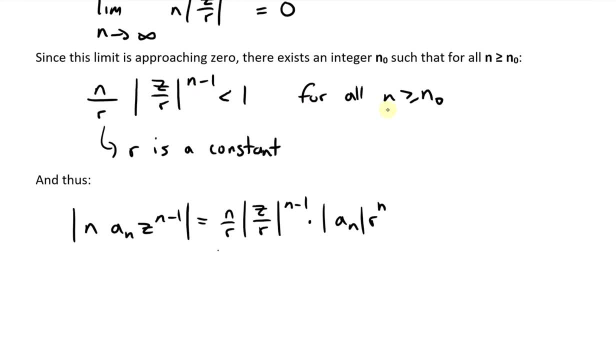 for a specific value there. So that means this right here. so I'll just look at this one. So this one is less than 1, for n is greater than or equal to n0.. So then this means that this whole value is going to be less than. 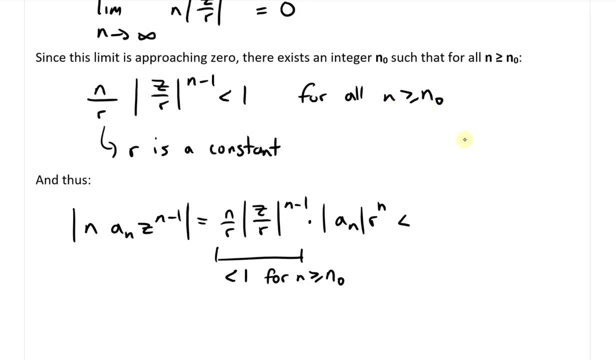 this is all, for n is greater than or equal to 0, less than just having this a n times r right here, Because you're going to be multiplying this in this scenario, that this scenario for n is greater than n0, is going to be multiplying it by less than 1.. 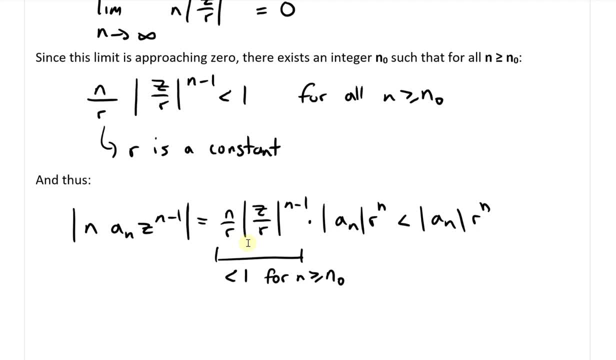 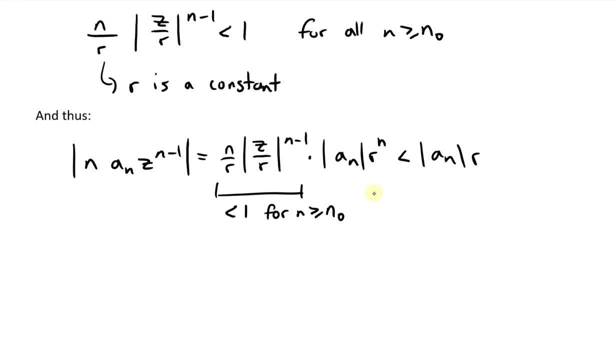 So when you multiply it by less than 1, the overall is going to be less than if you didn't multiply it by less than 1.. So it's less than this part. So that's less than this right here, And then, as you can see, we could apply the ratio test. 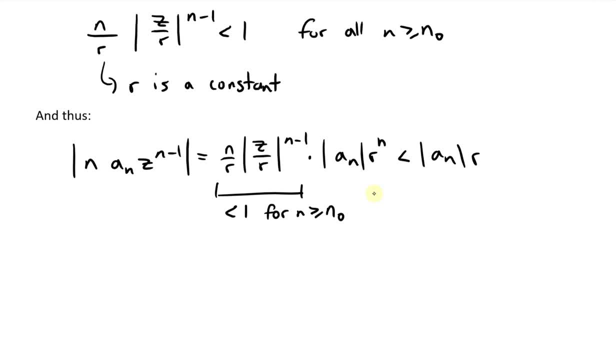 So this is r? n. like that, Let's write this a bit better. Yeah, so that's what we have. is this part right here which is a derivative part? So we could have right here, this is going to be n absolute value of n a n z to power of n minus 1.. 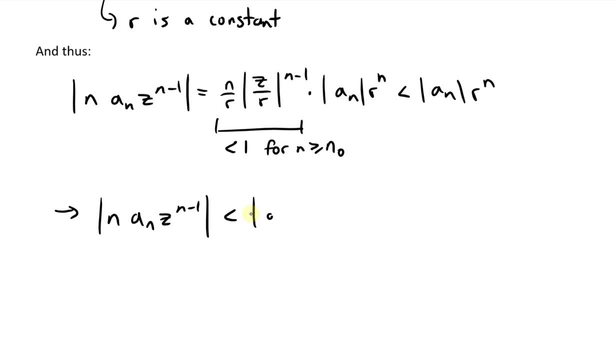 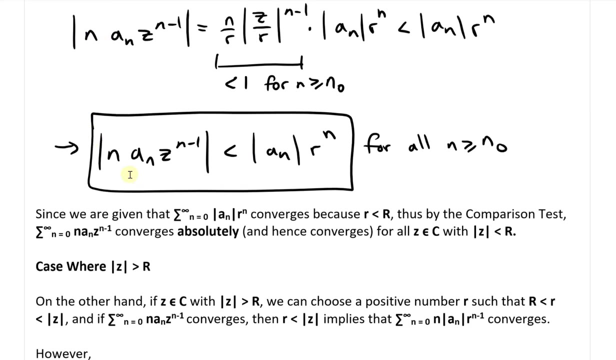 And then this absolute value of it all is going to be less than a n absolute value of a n times r, n, for if for all n greater than or equal to n0.. So let's just circle this part. And now, since we are given that, 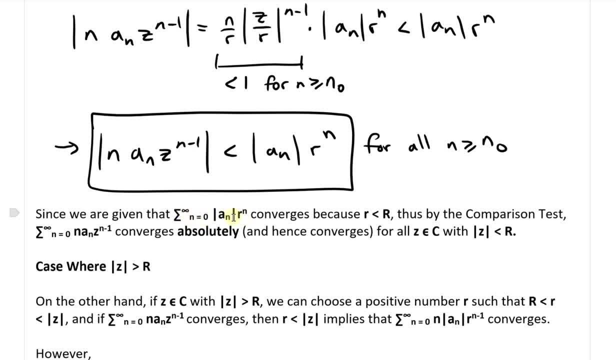 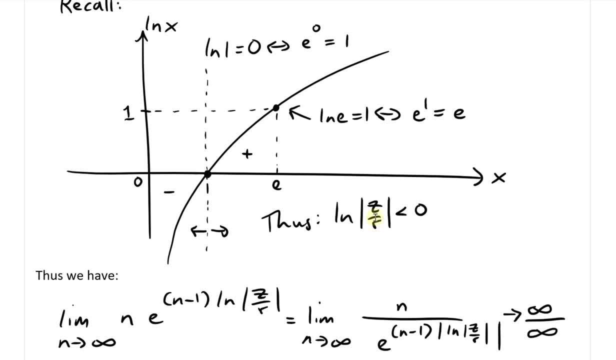 the summation from n equals 0 to infinity of absolute value of a, n is going to be less than the radius of convergence. So this is because r that we chose is less than the radius of convergence. So let's scroll up to what we were given here. 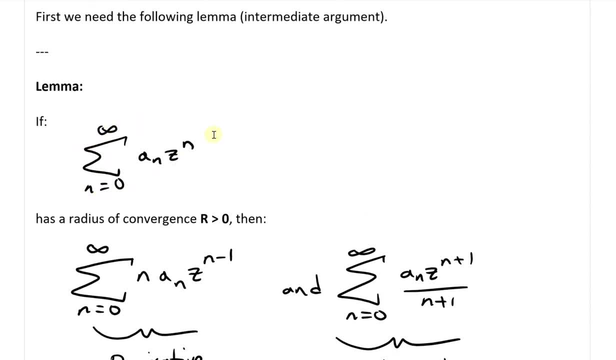 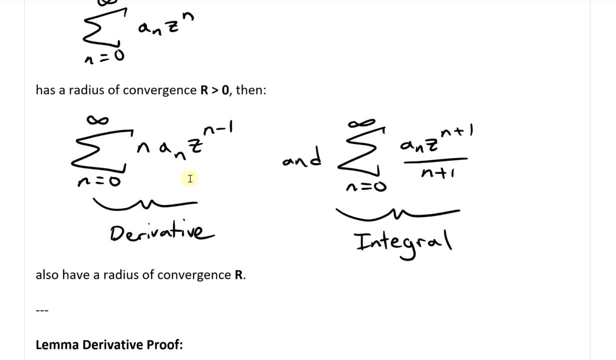 So in the lemma we're given. so if we have this power, series a and z- and if this has a radius of convergence, r is greater than zero. So in other words, in other words, the radius of convergence where absolute value of z is less than r. 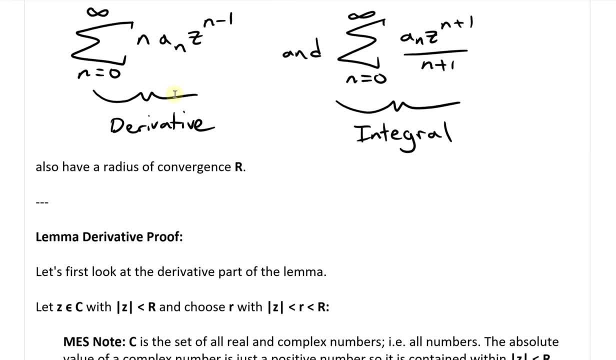 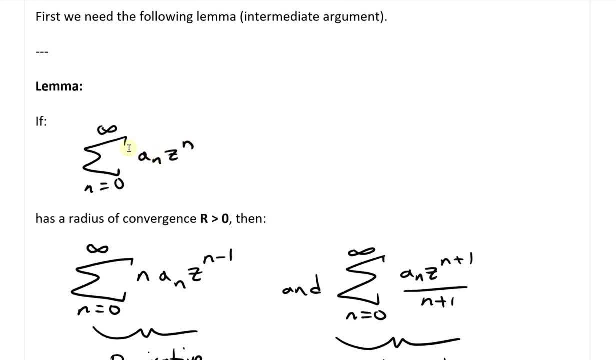 So that's just what this radius of convergence means, right there. And since r is going to be less than this radius of convergence, and but just it's just greater than absolute value of z, then a n, even absolute value of a n or a n, is also a n, r to power of n, is also convergent. 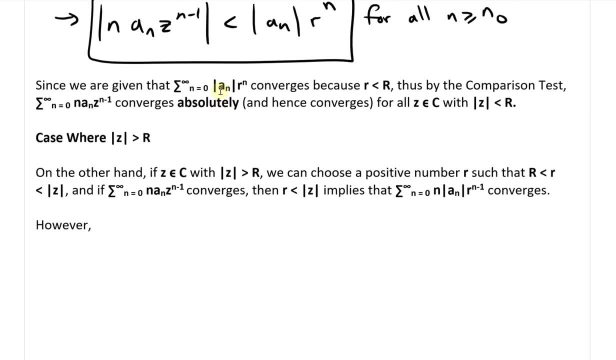 Absolutely and therefore convergent. So yeah, so we're given that this converges because, again, r is less than the radius of convergence. The lowercase r is less than the capital case r. Thus, by the comparison test, since this is less than this, for n is greater than or equal to zero. 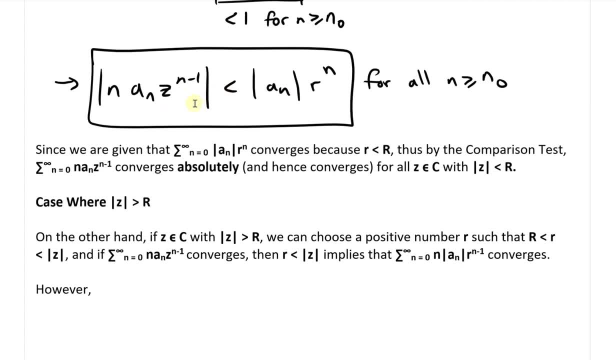 And again we're taking to infinity. So eventually it's going to, Yeah, it's going to always be less than. therefore, the summation from n equals zero to infinity of n, a, n, z to power of n minus one. In other words, 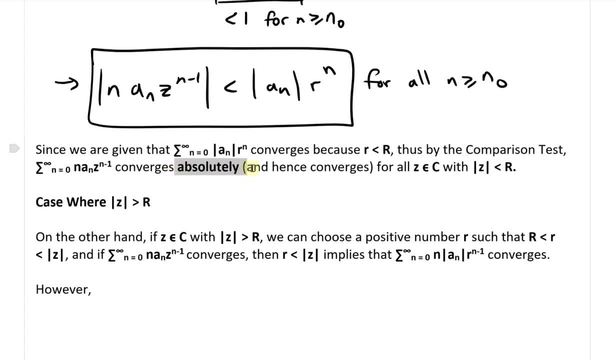 the derivative part converges absolutely and hence converges. Yeah, this is the absolute one and hence converges overall. because of the earlier theorem, for all z, as element of all numbers, real or complex, with absolute value of z, is less than r. So now let's let's look at the case when the absolute value of z 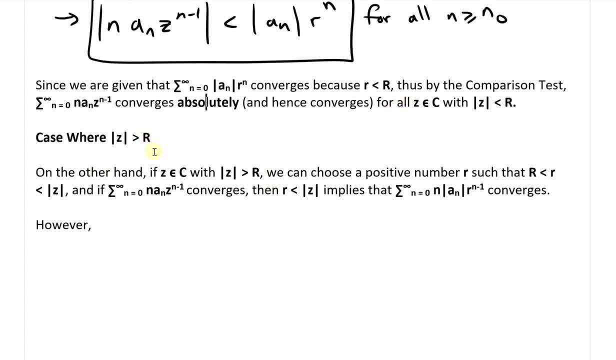 is greater than r. In other words, it's beyond what we chose as the radius of convergence, what we were given for the a n z to power of n. So, on the other hand, if z is an element of all numbers, real and complex, with absolute value of z is greater. 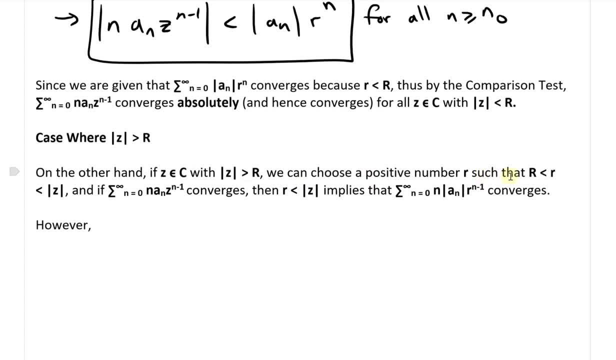 greater than r instead of less. we can choose a positive number, r, such that r is less than capital. r is less than r, which is less than absolute value z. So we're always choosing this r in between. So we're always choosing the absolute value of z and the radius of convergence. 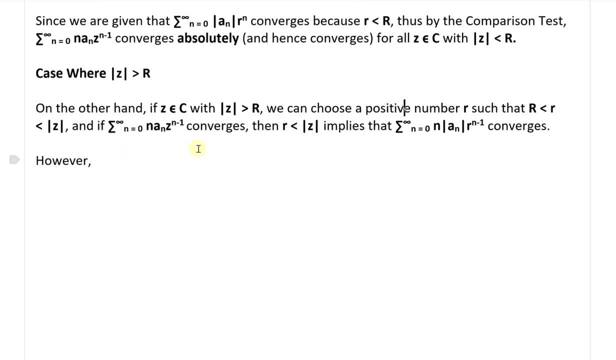 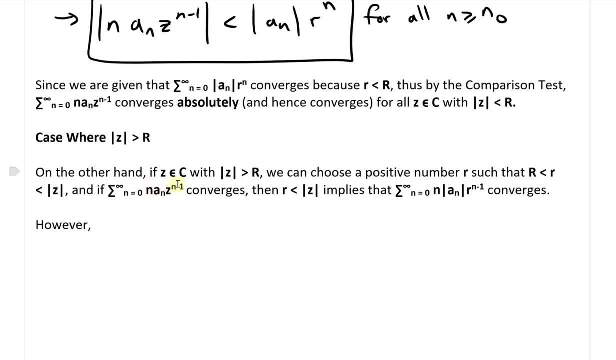 And if we're given that, if we're given that and there's a series n equals zero to infinity of n, a, n, a, n, z, to power of n minus one converges. and also here actually my PDF uses n equals one, Because if you put zero, there is going to zero term. and does that also for here, for the derivative part there, just be more complete. 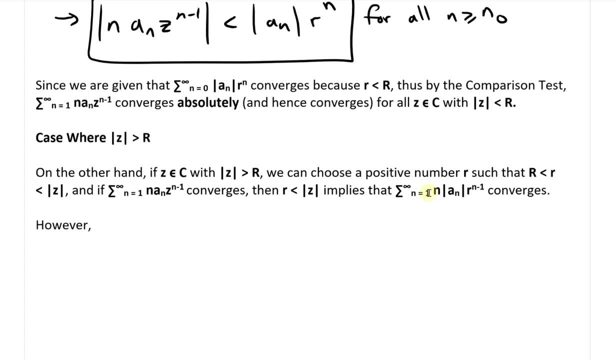 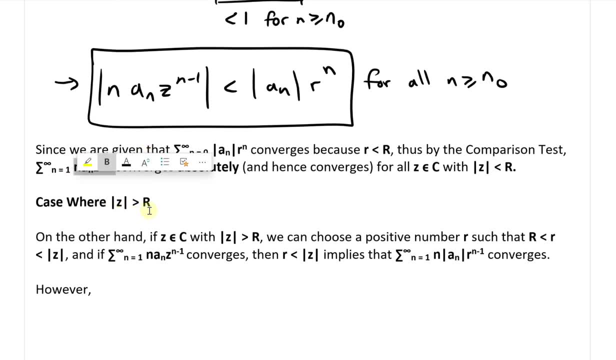 So whenever you have this n in front there, we split this one there. Yeah, So if we're given that the derivative part converges from above here, so we're assuming absolute value of z is greater than r, then that means yeah. So if this is convergent, then that means, since r is less than absolute value of z, since we chose it between the radius of convergence and this, z implies that this is also convergent. 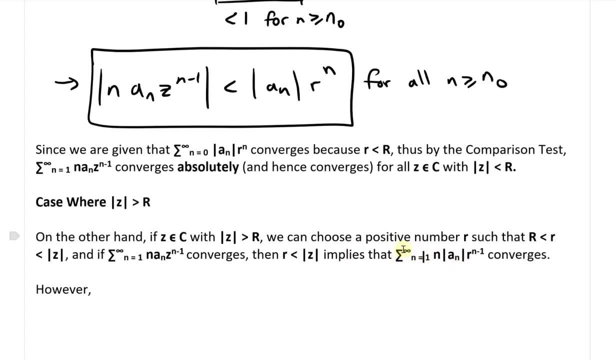 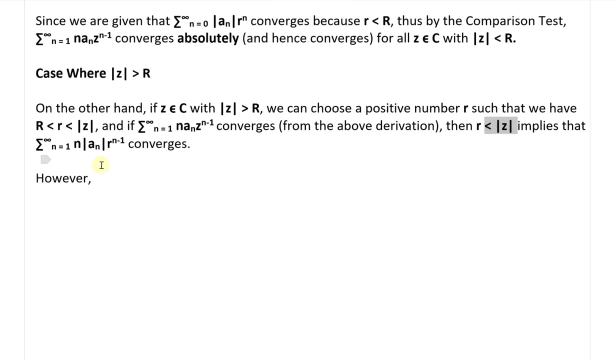 So absolute value, I mean a series from n equals one to infinity, infinity. and also here is put a note here, from this one, here, if this converges from the above derivation and also just type some stuff up to move it here, So it looks a bit better. so then that means yeah, if we're given that this, this converges from the above derivation, then since r is less than absolute value of z, implies that as well, the series from n equals one to infinity of n times absolute value of a, n, r and minus one also converges. yeah. so it implies that this also with this absolute value sign and using this absolute value sign, just because I can follow up with it. 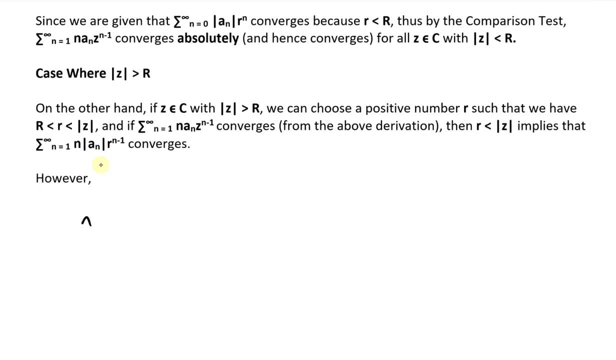 So, however, what we have here, this n absolute value of a, n r to power of n minus one. so this is why. so, if it's absolute value, then we could set some equality signs, because otherwise we couldn't do this. so this is going to be: this is greater than or equal to a n times the absolute value of a n times r and minus one. that's because this n is always means that this is going to be greater than or equal to it. this one doesn't have an n. 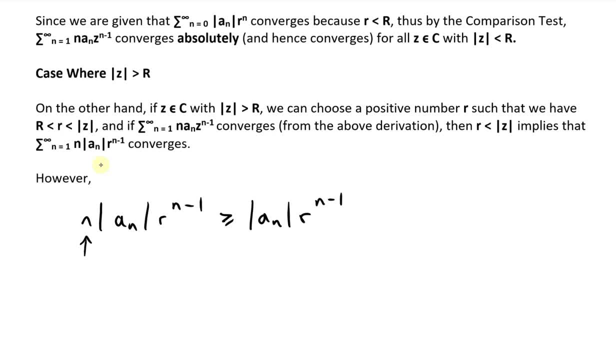 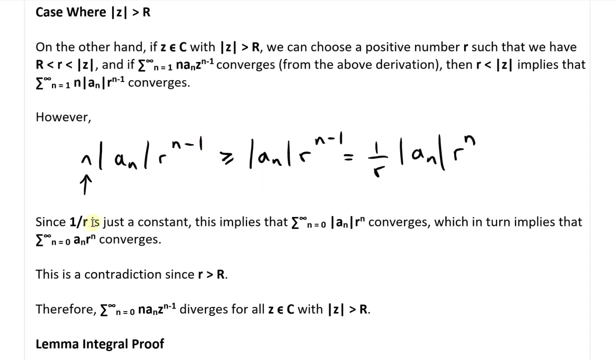 So this is just a highlight here. So this, This one just makes it always greater than or equal to. and now this part right here, just factor or just just take this down or expand this power right there, so this becomes the same thing as writing one over r a n, like that: this is r to the n, absolute value of a n, r to the n. and now, since one over r right here is just a constant, this implies that the summation from n equals zero to infinity of absolute value of a n. 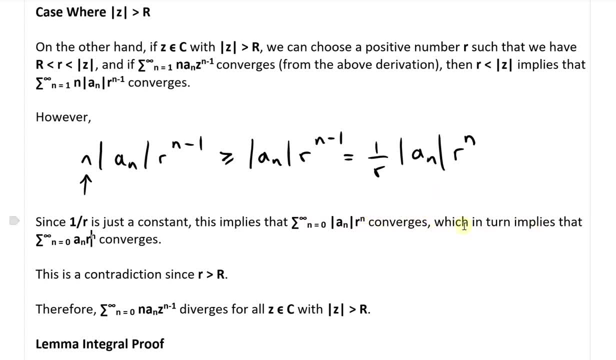 r and converges, which, in turn, because it's absolute convergence. This is absolutely convergent which, in terms, implies that the summation from n equals zero to infinity, of a, n, r and converges. this is a contradiction, since r is greater than the radius of convergence, capital R. 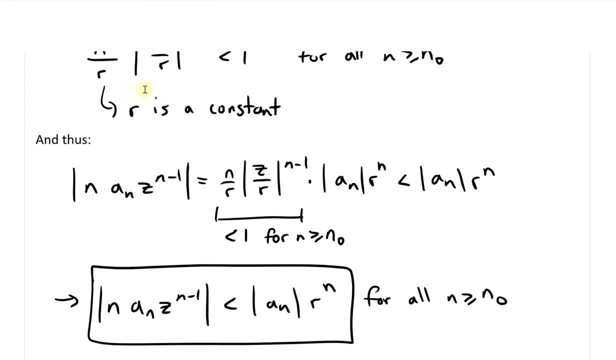 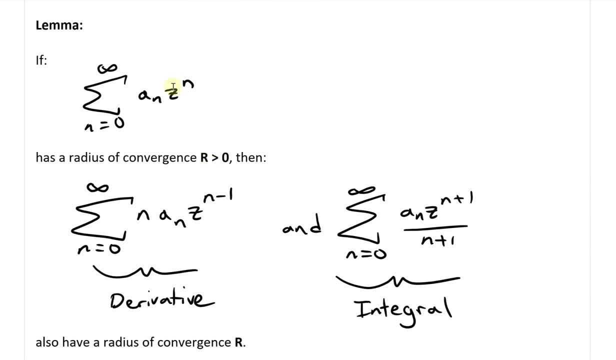 Remember this is the case where absolute value of z is greater than r, where the starting point of the lemma is always going to be this scenario, where r, where the radius of convergence is r, right there, but we have r- is greater Than absolute value of r. so we have a contradiction there. 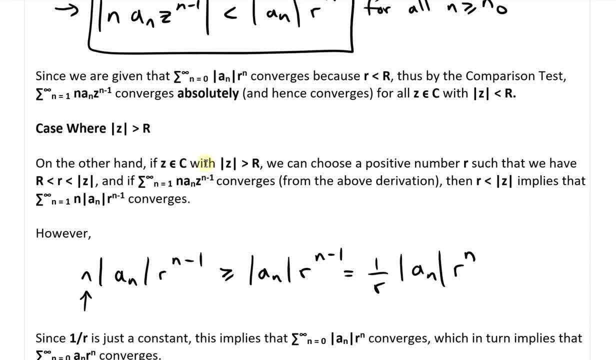 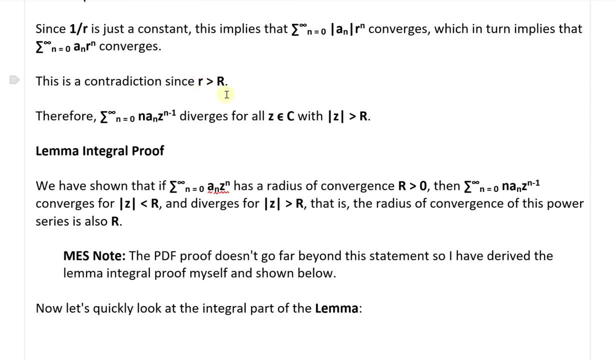 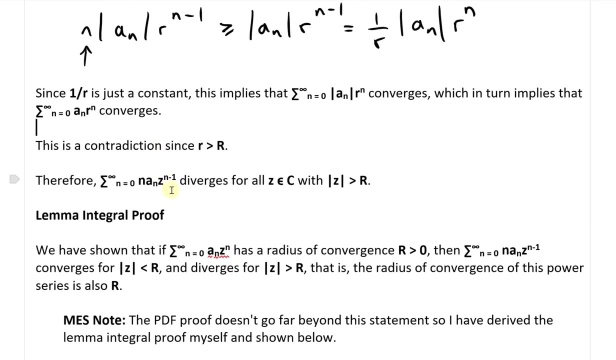 Yeah, greater than the radius of convergence there. So it offsets our, our basic lemma that we had. therefore, this is: there's a contradiction, since r is greater than capital R or the radius of convergence. therefore this: the summation from n equals zero to infinity, of n, a, n, z power, n minus one, diverges for all z element, of all all numbers, real or complex, with absolute value of z greater than r. 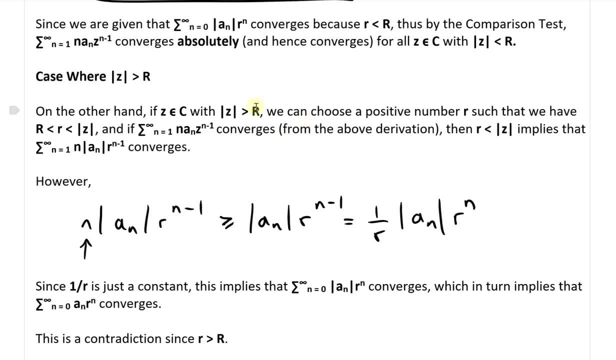 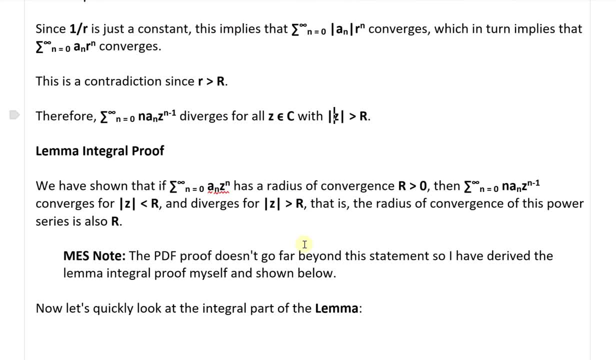 So, in other words, Of convergence is r and you can go greater than it. is a contradiction and hence it's the same as same radius of convergence of the function. that weekend or you quickly or a move things around to put this in a proper place. 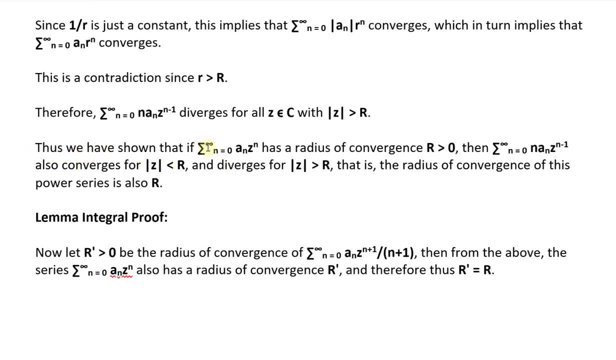 On our now to read what I just did. so thus we have shown that if The summation from n equals zero to infinity of a sub and times, that then has a radius of convergence all which is greater than zero, then this, and so does over this one, here is then: 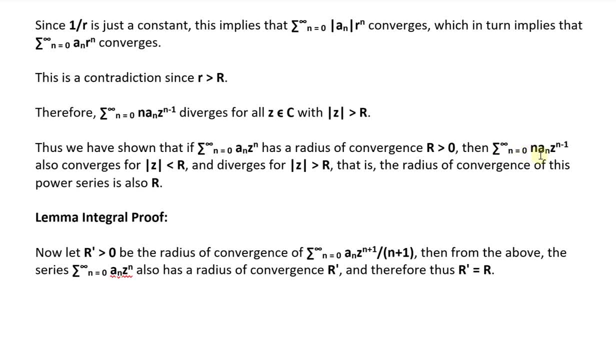 Then the summation from n is from: n equals zero to infinity, of n times a n times z to power of n minus one. also converges for absolute value of z is less than r and diverges for absolute value of z is greater than r, as in this case. right there, that is the yes, that is the radius, radius of convergence of this power. 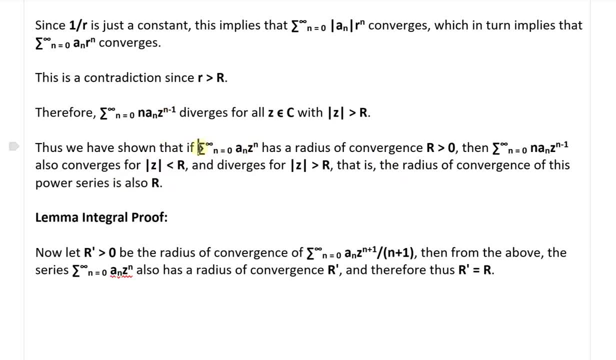 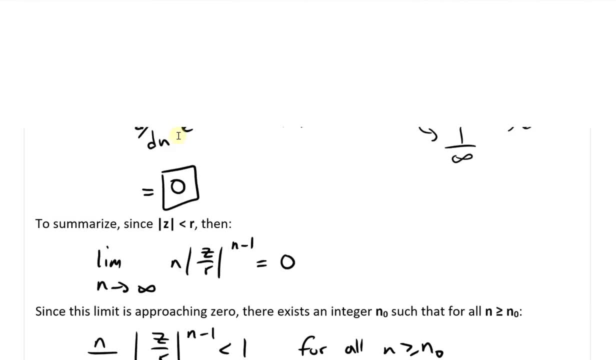 series is also r. so hence we have just proved the first part of the lemma, or the derivative part. so now let's take a look at the lemma and integral proof and let's just quickly recap on the lemma. so the lemma here states that, uh, if we have a series like this, n equals zero to. 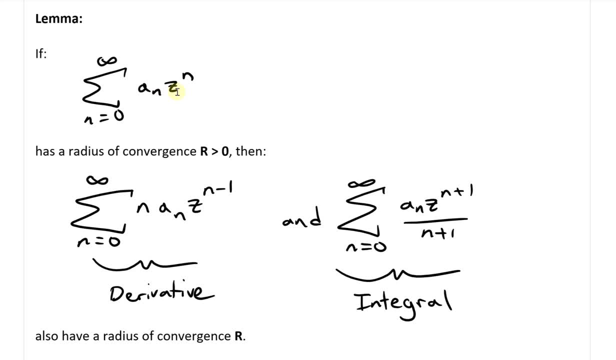 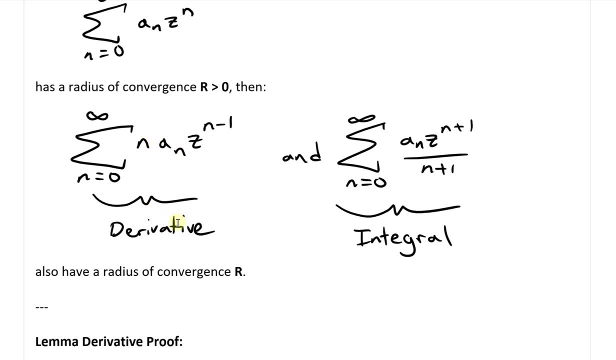 infinity of a n times z to power of n and it has radius of convergence capital r greater than zero. then so do these two series, where this one, i'll call it the derivative part of it- but remember, i'm not proving that this is the derivative of this entire series- is this function? this is this. 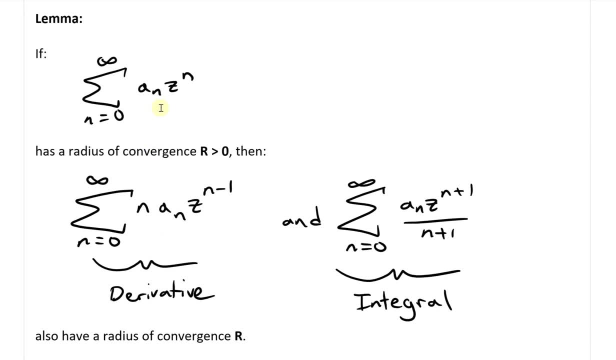 is theorem one, and that's that's what i'll prove later in this video. but here i'm just showing that these have the same derivative part of it. so i'm just showing that these have the same derivative part of it. so i'm just showing that these have the same radius of convergence. so this series and 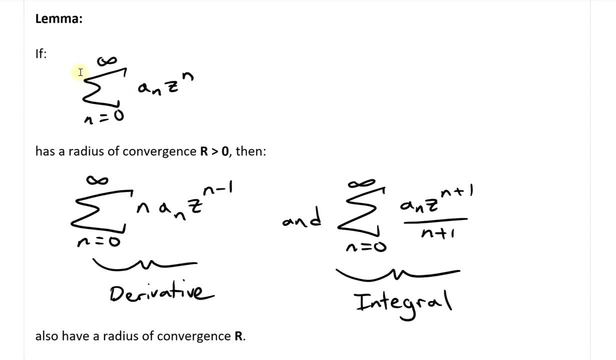 this series. and then theorem one just shows that you can take a derivative of the from outside of this uh, of this power series, and then it's the same thing as taking derivative of each, each term like this: so uh. so basically, this says: if this has radius of convergence r greater than zero, 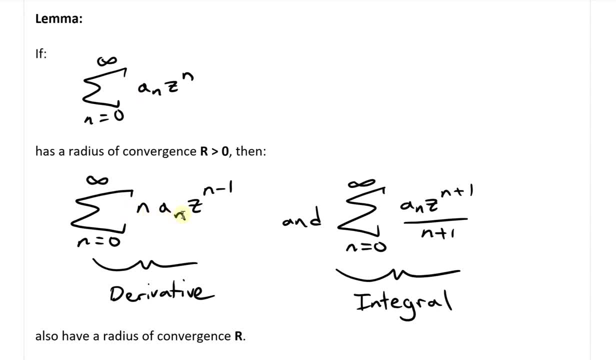 then so does the series of this one here: n times a n times z to the power of n minus one, and so does here the uh integral part: uh a n times z to the power of n plus one, all divided by n plus one. all right, so now let's just scroll down to the uh integral proof, and the integral proof is: uh very. 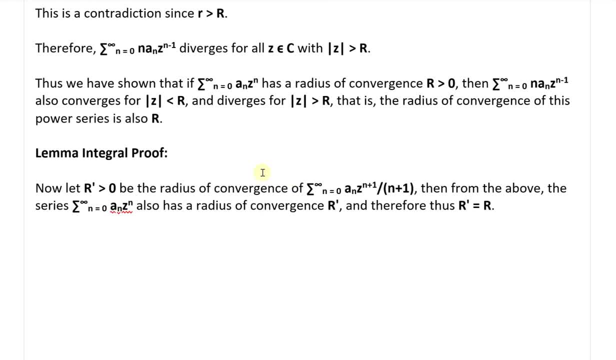 straightforward: it's uh just a follow-through from the uh from the derivative proof. so, lemma, integral proof. so now let r capital r prime be the radius of convergence of uh, the integral integral part. so the summation from n equals zero to infinity of a n times z to power of n plus one. 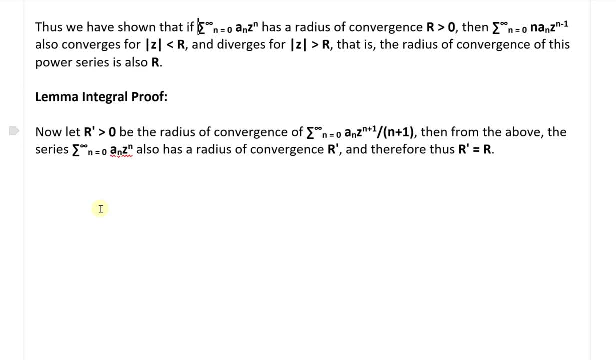 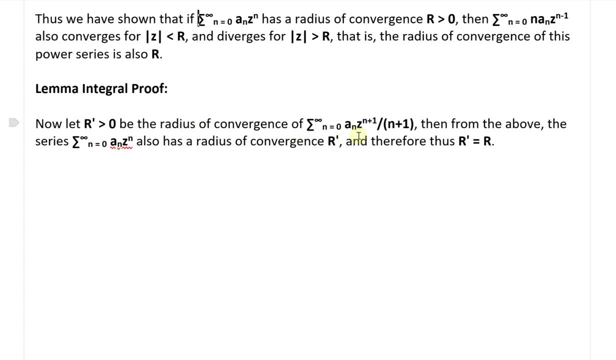 all divided by n plus one, then from the above the series, uh, the summation from n equals zero to infinity, of a n times z, to the power of n plus one, all divided by n plus one, and then from the n times z, and also has a radius of convergence, r prime, or uh r dash like that, and this is uh, this. 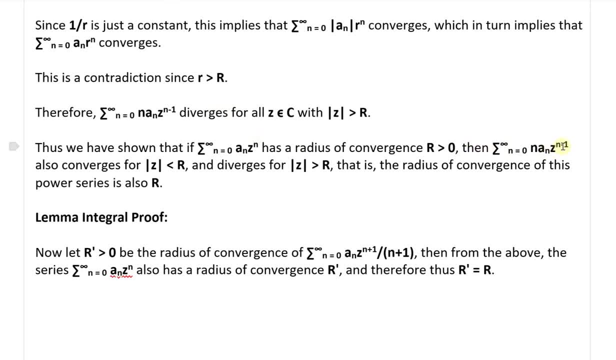 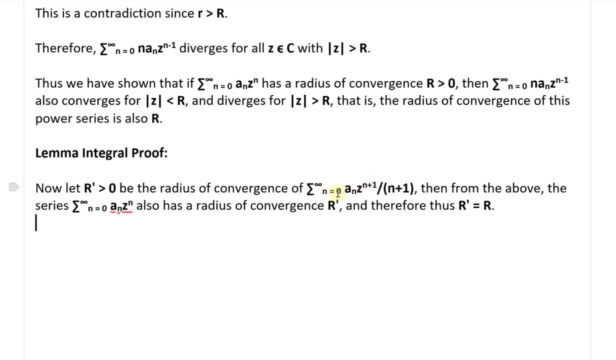 is strictly because, uh, what we're doing here we're just lowering, uh, we're just taking the n, putting it down and subtracting by one. so we're doing that here as well, but this time we're taking the n plus one down, subtracting by one, and then these would end up canceling, and then this will get this right. 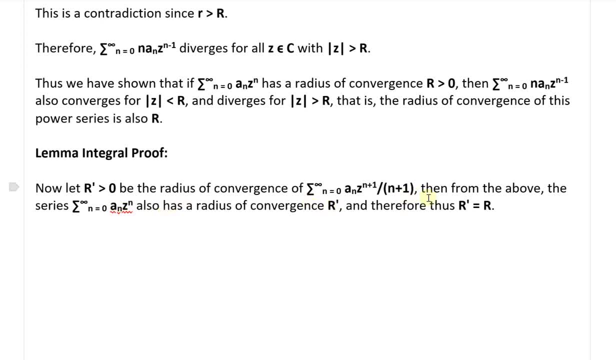 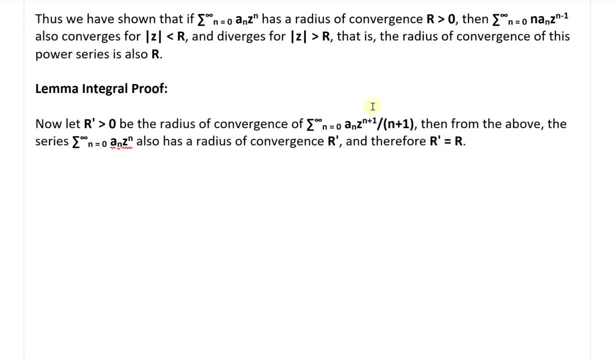 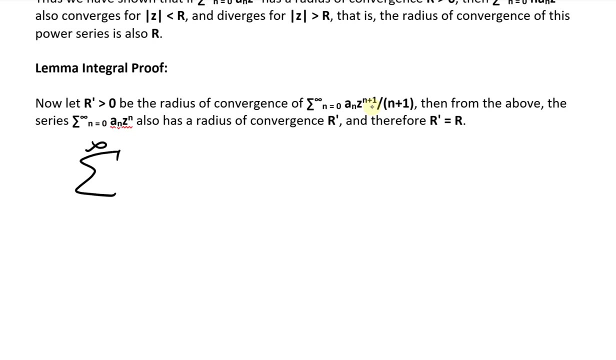 here, and it also has radius convergence, r prime and therefore uh, and therefore uh, r prime equals to r and to illustrate this better, this is what the pdf proofs stated: uh, it's basically what this is saying is: we're showing this, uh, graphically, so we showed that. uh, so the lemma, we showed that. if 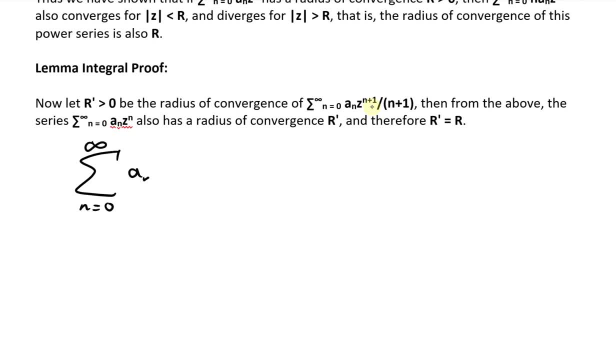 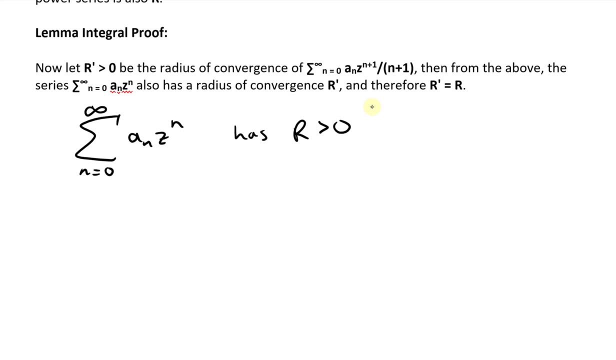 n equals zero up to infinity of the series. uh, a, n, z, power of n and this has r greater than i mean just regular r greater than zero, then uh, yeah, so if we have this one here, so what follows is is: uh, is that uh? if we take this here and uh, infinity n equals zero, and then just bring the n down, or 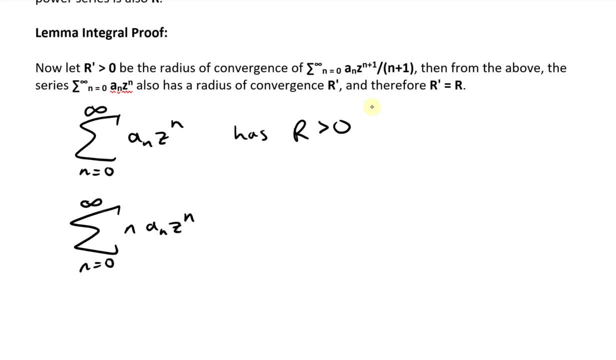 uh, just just write down exactly here: so uh n times a, n z, uh z to the power of n minus one. yeah, now this uh- yeah, this also has this right here- also has r greater than zero. so these are the exact same ones. so both of these have r is greater than zero. yeah, so they both have radius. 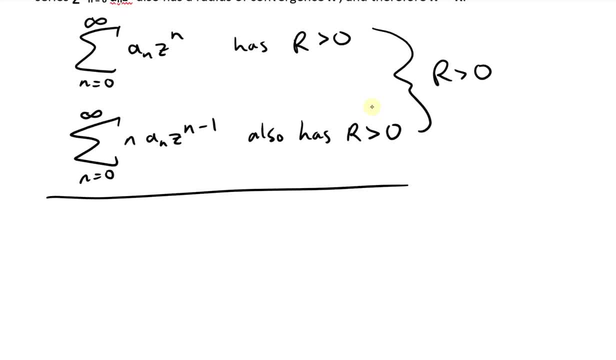 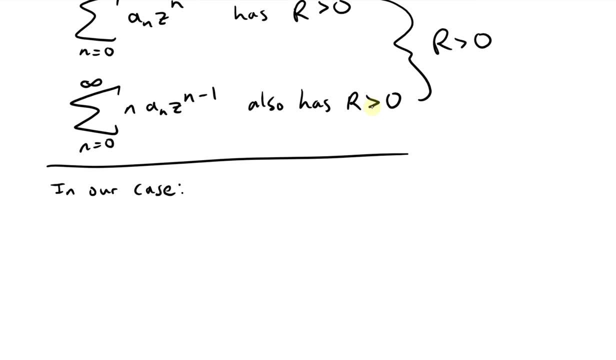 convergence: uh, capital r greater than zero. so then we can do the exact same thing. we can do the exact same thing for our case. so i'll write that uh down in our case and also here: uh, so we have. uh, let's write: move this over to the right number. what if? 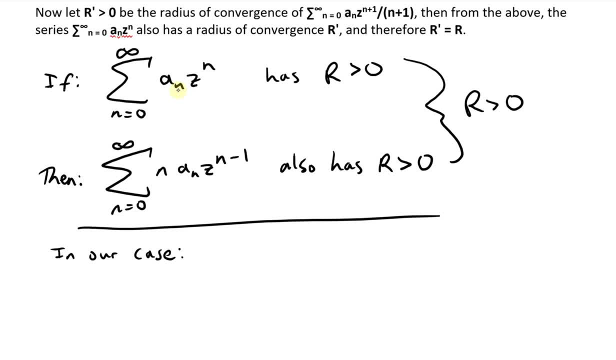 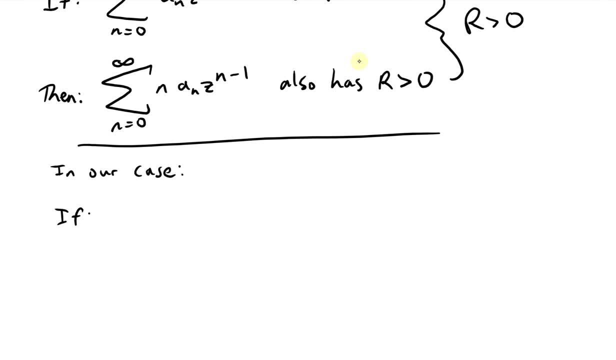 we have that from the lemma, then this is what we prove. thus, in our case, what we have is: we're starting off with the integral part, so, uh, this right there. so, in our case, if, if, right here, summation from n equals, uh, zero to infinity of a n, and then we have 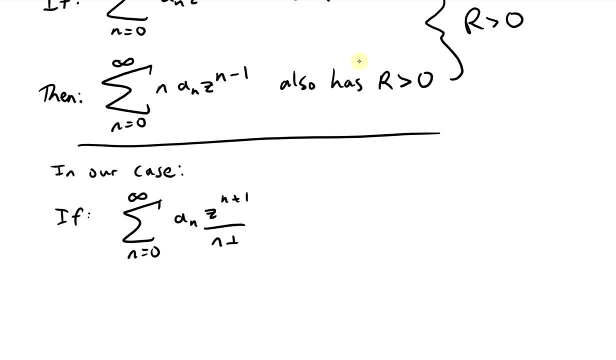 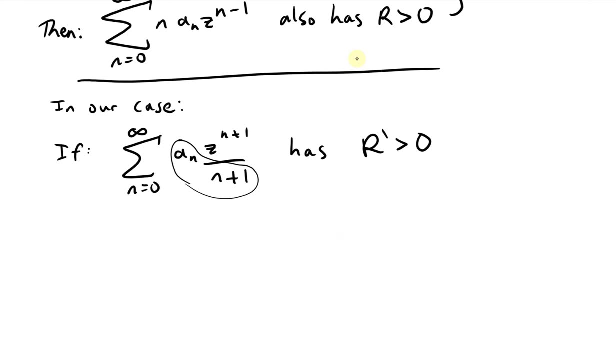 z n plus one over n plus one, and if this one has r prime greater than zero, so assuming it's different than this one, yes, then what we could do is, well, we could just circle this part right here. this is the same thing as saying, uh, because, remember, this is a n divided by n plus one. 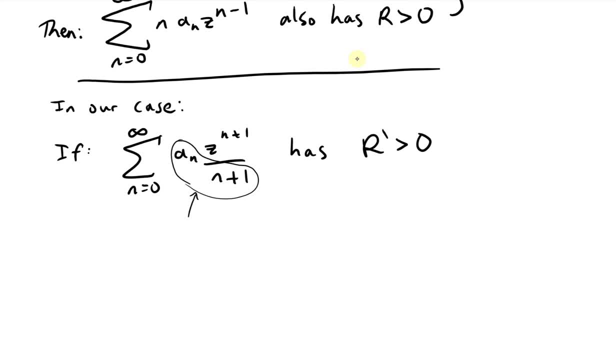 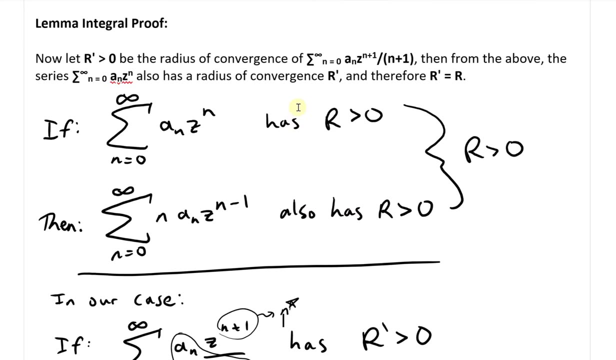 these are still coefficients. these are just still going to be constants when we add these up to infinity. so this is going to be- let's just call this a and a star, to indicate that it's that. and then this: right, here we're gonna. let's just call this n star. yeah, so here we're just applying this exact uh theorem. 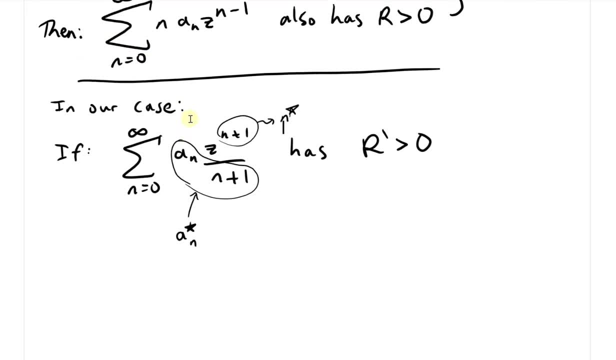 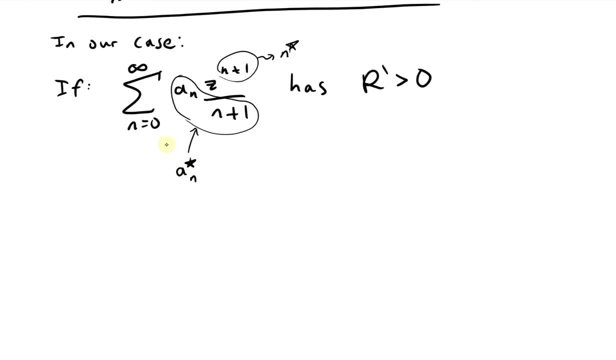 there or this exact lemma. so if this, then we're gonna have uh, this right here, but in this case we're gonna call that n star. we got a top part n star, this one uh a n star. so i'll say, if this uh, then in bracket here or the giant bracket. so this is going to be the same thing as saying: 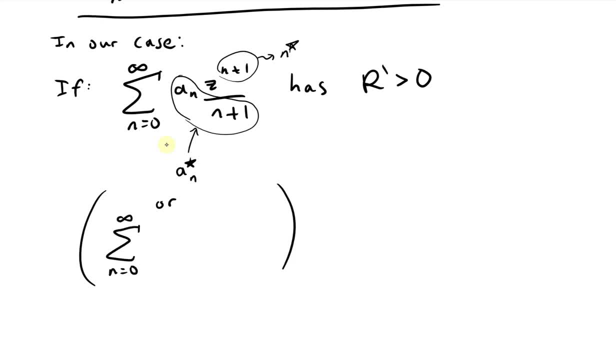 summation from n equals to zero up to, uh, infinity, and this is going to be a, and star, uh, this is going to be z. i'm just showing that it's exactly the same thing, just the power series, uh, and start like that. yeah, so here, i just uh, moved it around, moved it over here, so this is. 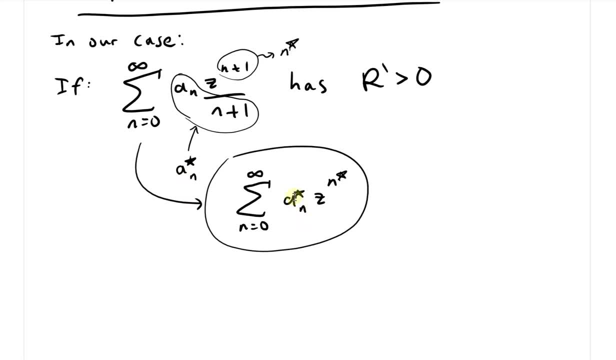 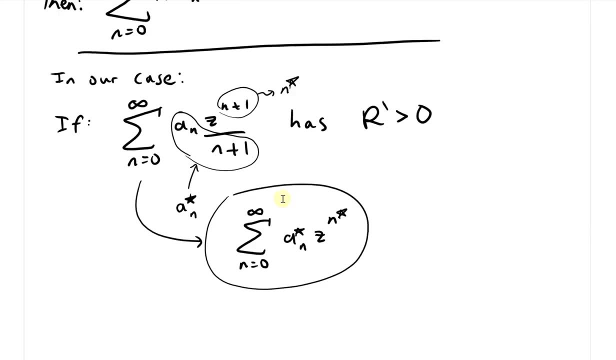 the same thing saying is: summation from n equals zero up to infinity of a, a star, n, like that, and then z and star, where, anytime you have n, you're going to switch them over to this one. so that means, according to this theorem, then we can just bring down the n and then we'll have n minus 4. 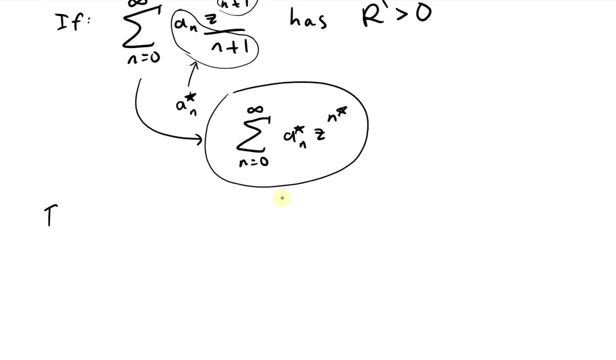 n star there subtracted. so this is just going to be then. then, uh, summation up to infinity: n equals to 0. then we could bring the n star like that, this is going to be a and star z and star subtract by 1.. and yeah, so then this one right here, this: 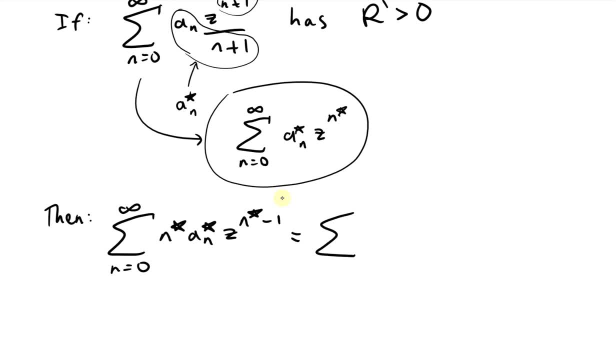 also has our prime, and where this one is just merely equal to. just plug in everything. this is going to be: n equals 0 up to infinity, and this is going to be n star is going to be our n, like that, and then add this: a n star is going to be: is this going to be a n? regular, then divided by? 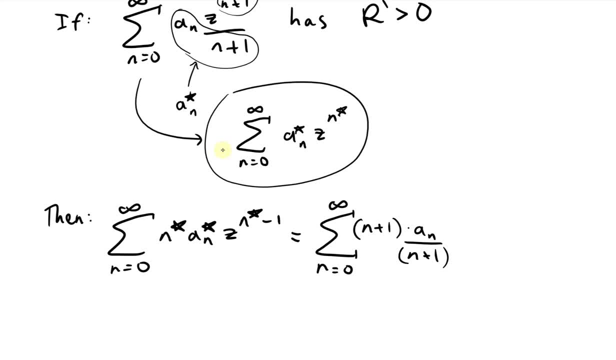 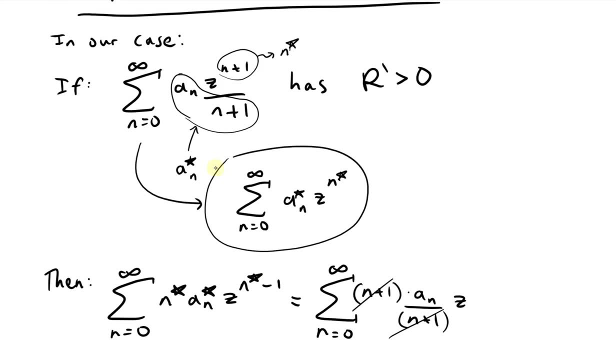 n plus 1.. so we have, these are going to cancel, so this is going to cancel, and then this is going to be: uh, times it by z, and then n star is going to be n plus 1. we're subtracting by 1. this is going to 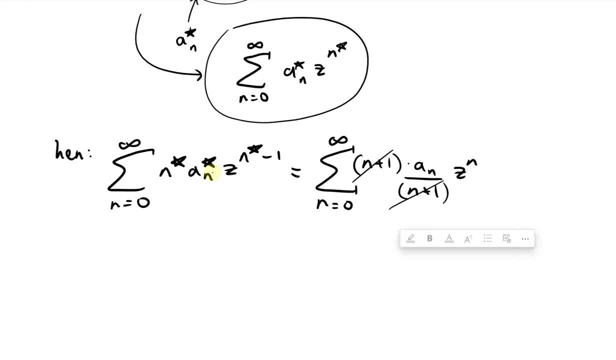 be z, n, so on. and here i'm going to move this over, or actually i'll just keep it here and then: just right, then this equals 2, these cancel. this is going to be n plus 1, and then we're subtracting. this is going to be equal to summation from n equals 0 of a n, z, n, like that. so if we have uh, 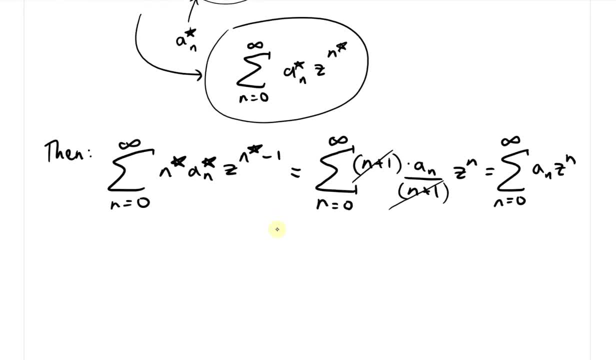 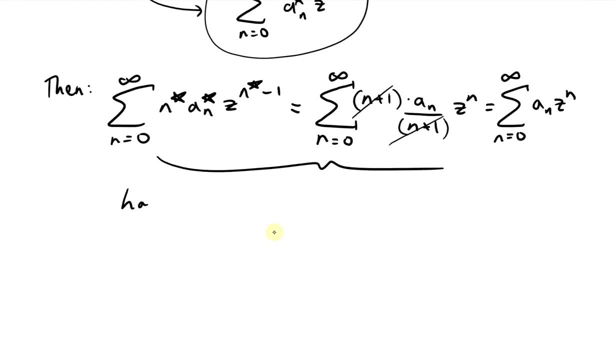 if we start from here, this has a radius of convergence r prime, then so does here. then then this right here: this is this whole thing. uh also has also has r prime greater than zero. but then this one here. we already know that, uh, this one is already given. this is a summation from n to infinity and this is going to be equal to summation. 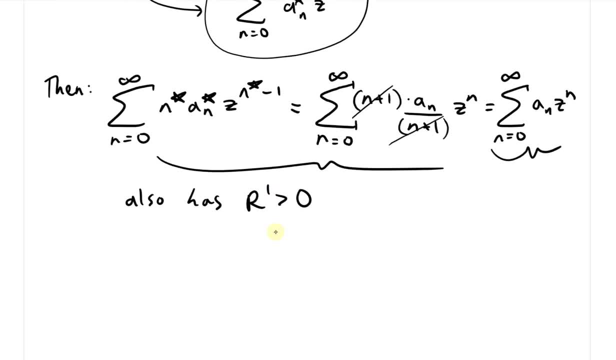 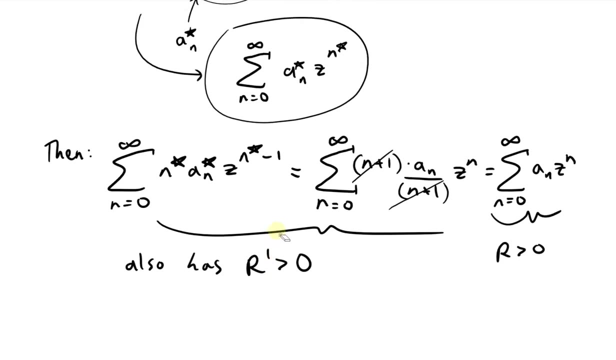 from n equals 0 to infinity of a n z power of n. this one already has uh r. uh r is greater than zero, so this, so thus these are. these are exact same things. yeah, so this one's already that. yeah, so then these are r prime and this r uh without the prime is exact same one, so also has this. 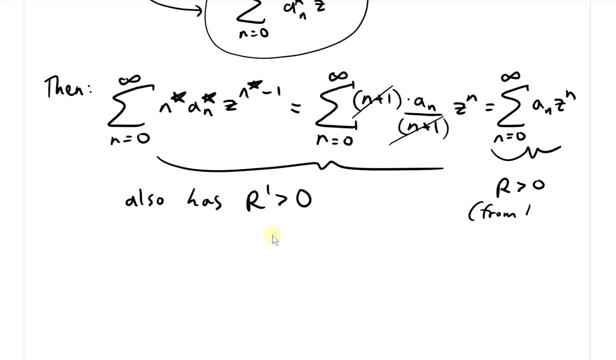 uh, this is from the lemma, or the or the derivative part of lemma. uh, just, uh reset. so so this is pretty much it. just the hits is a bit convoluted here. uh, thus r prime equals r, so it's just, it's still power series. this is, this is just dealing with different uh n plus one terms, because again you're going to 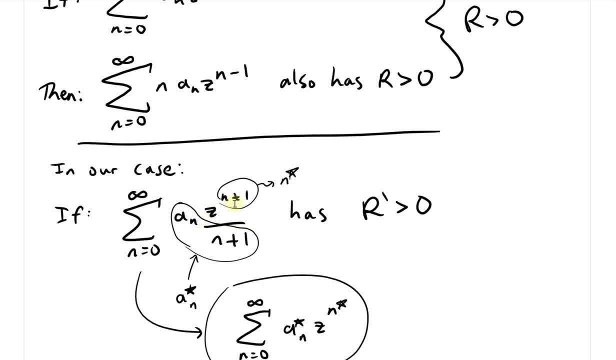 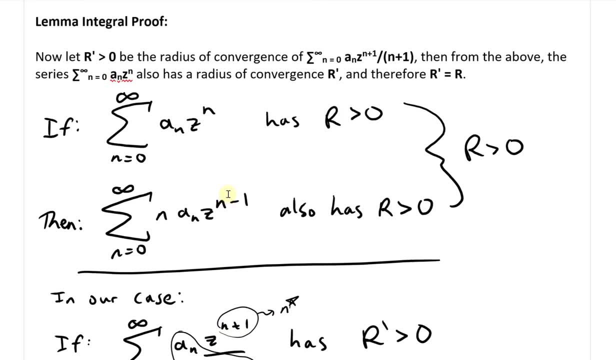 infinity. these are all just going to be coefficients. this one's going to be, uh, your powers of this going to be power of one, two, three, four, five, et cetera. so, then, this minus one might be starting from, uh, slightly earlier, but it's all going to infinity. 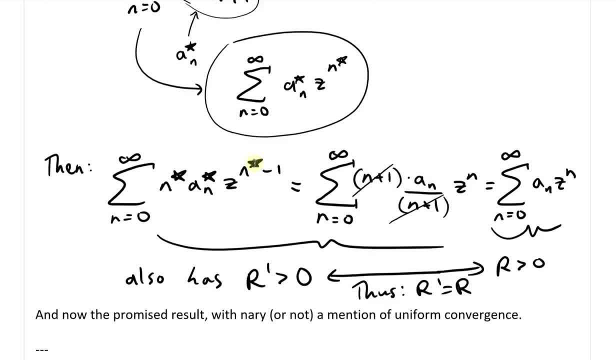 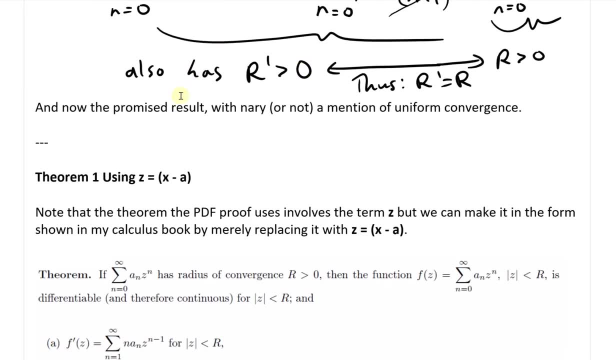 so, yes, we could just do all that. so, yeah, i just wanted to uh illustrate that graphically exactly what they were stating here from my calculus. that's all they wrote, uh, but it's uh should be pretty straightforward. and now the promised result with uh, nary or uh, not a mention of uniform. 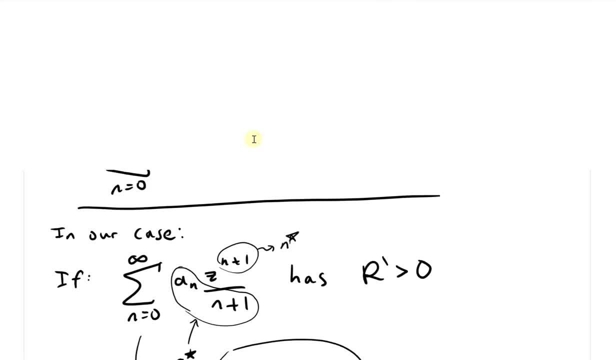 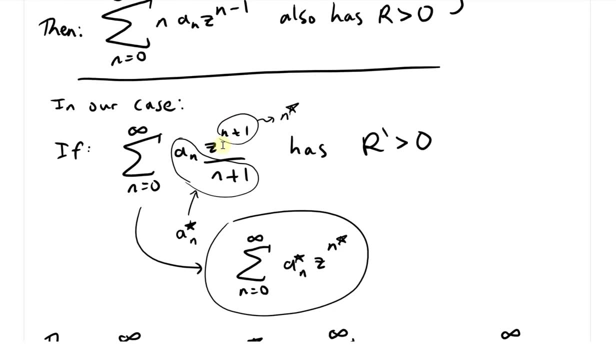 convergence, uh, uniform convergences, uh, the this would, we would what we were just going over. so then, all these a n z n? uh, series of n? a n z n? uh minus the power of n minus one, and also this one a n z, the power of n plus one, all divided by n? 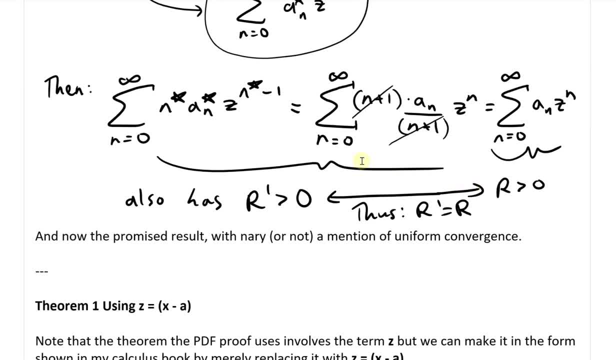 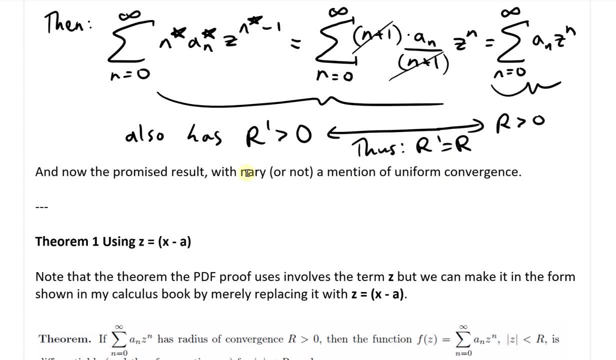 plus one, they all have the same radius of convergence if uh r is greater than zero. so yeah, so that's uniform convergence. and here this nary is: uh. this word is used in my uh the pdf proof and it's not part of my vocabulary. well, until now what that is. so anyways, let's jump right. 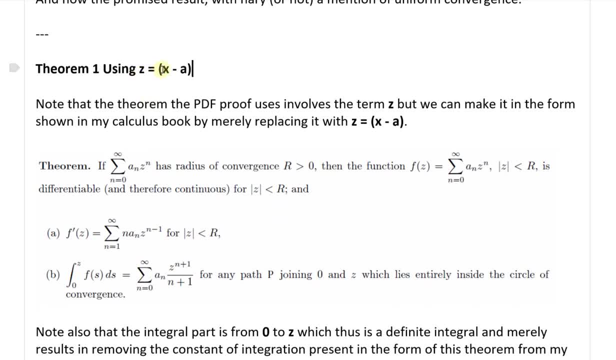 and so theorem one- and this is again using z- equals uh, x minus a. uh, yeah, so my calculus book has that uh in the form x minus a. but then this pdf proof just uses z, but nonetheless, you can just replace it, you can substitute it and you'll get the same result. 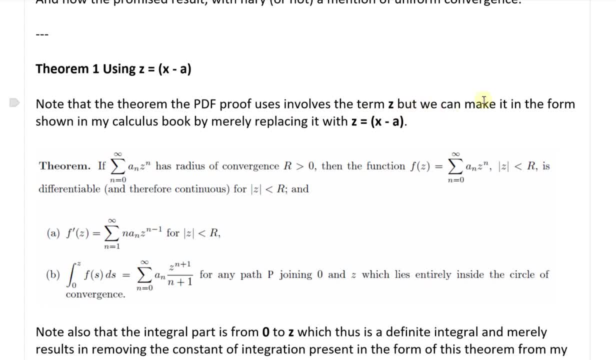 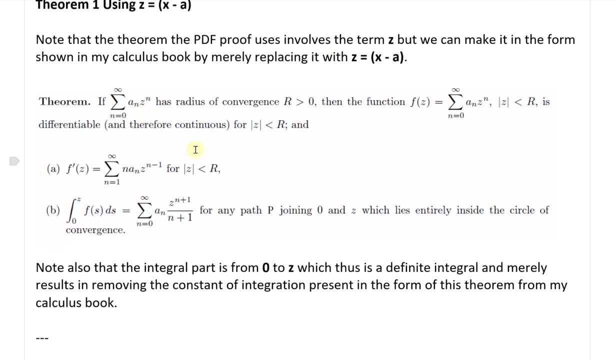 so note that the theorem the pdf proof uses involves the term z, but we can make it in the form shown in my calculus book by merely replacing it with z equals x minus a. so here i just uh screenshot or just took an image from the pdf proof. so theorem: if the summation from n equals: 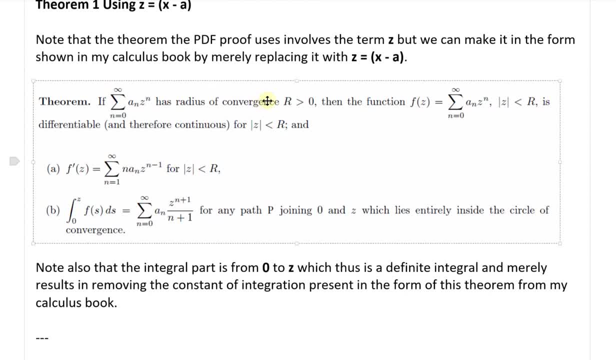 zero to infinity of a, n, z. the power of n has radius of convergence. r is greater than zero, then the function f of z equals to n. equals zero up to infinity of a, n, z, n. yeah, z to the power of n. this is writing this as a function, uh, where absolute value of z is less. 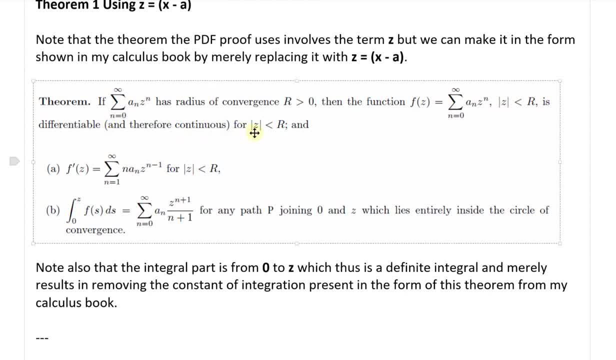 than r is differentiable and therefore continuous, for this absolute value of z is less than this radius of convergence r, and we have. so this is the theorem. yeah, so if this function is differentiable and therefore continuous, uh for uh, it's uh, for one absolute value of z is within the 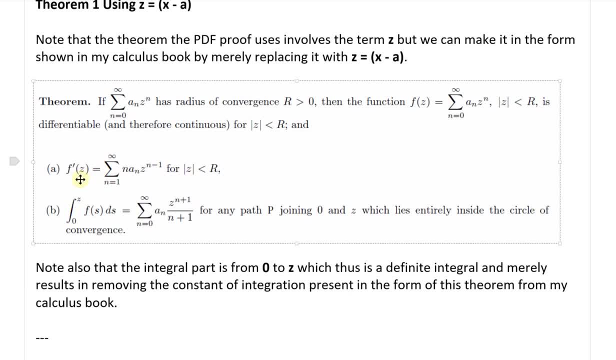 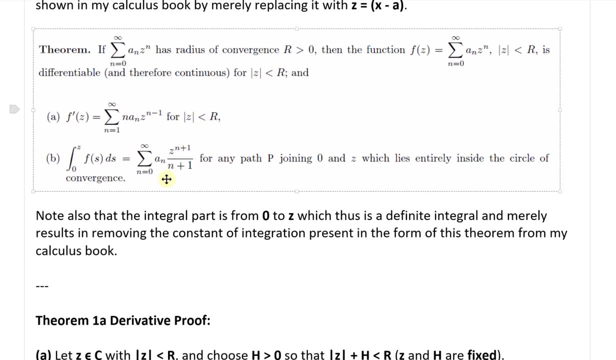 radius of convergence. and then we could take the derivative. so then a f, prime of z, or the derivative. first derivative, uh equals two, the summation from n equals one to infinity, of n, a, n, z to power of n minus one. for uh, absolute value of z is less than r. and then for part b, uh, the integral. 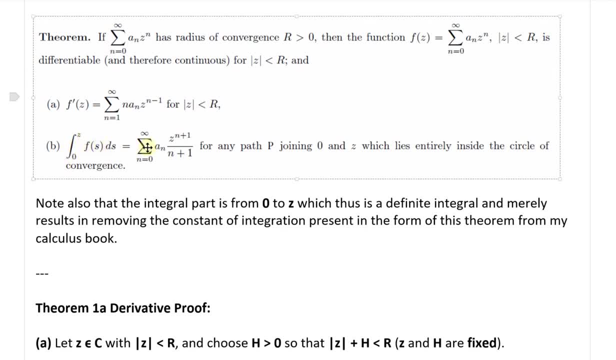 from zero to z of f of s, d. s is equal to the summation- n equals zero to infinity- of a n. uh. this is the integral part times z to power, n plus one, all divided by n plus one for any path, p joining the circle of convergence and uh. note also that the integral part is from zero to z in this uh. 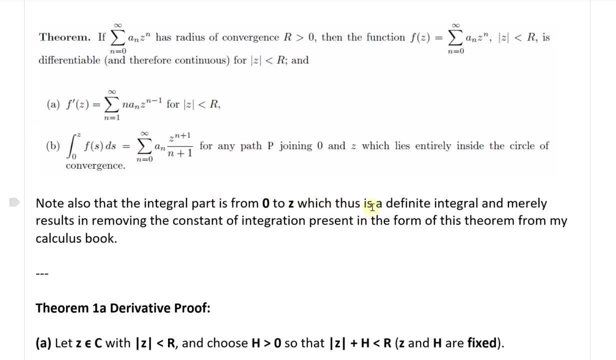 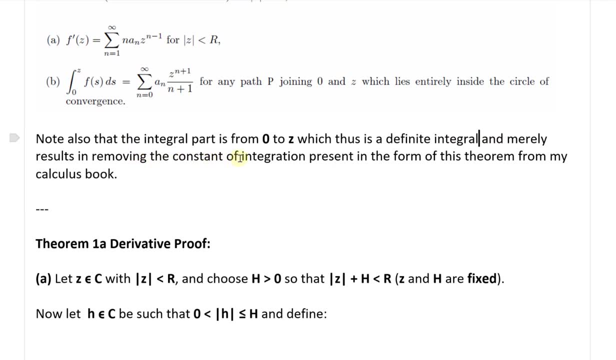 derivation or this theorem that pdf proof uses uh, which uh thus is a definite integral as opposed to the indefinite one uh shown before, and merely results in removing the constant of integration present in the form of this theorem from my calculus book, so this one doesn't have the 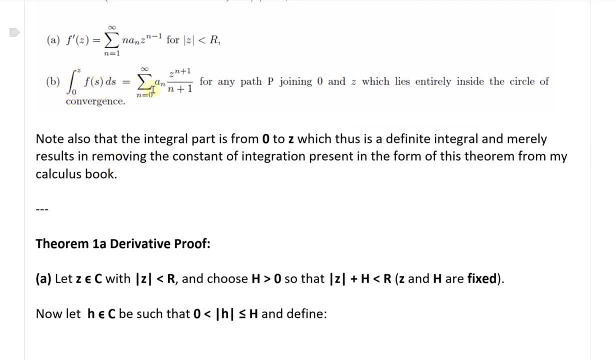 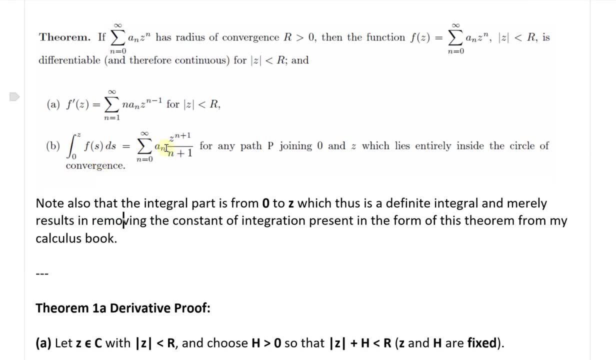 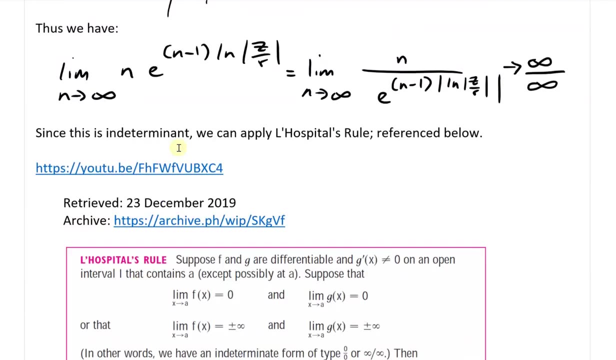 constant integration, the definite form, and when you have it from zero to z. well, if you plug in zero and into this uh z area, this all just becomes zero. so, uh, yeah, so then then you're just going to be left with this and no constant integration. and let's just scroll up to the earlier one, where i screen grab just to show you the constant of. 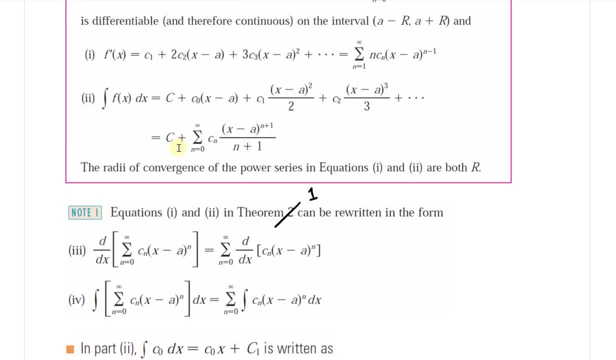 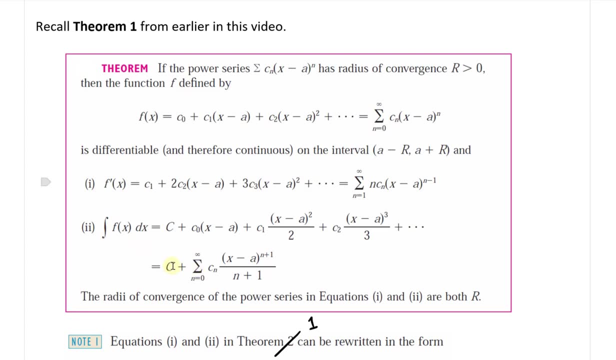 integration. and where this? where the one from my calculus book is over here. this one just used the general, uh, just a general indefinite integral, so you have the constant integration there. but then the other one: you're going to be subtracting uh, this, and then from when uh equals, from when? 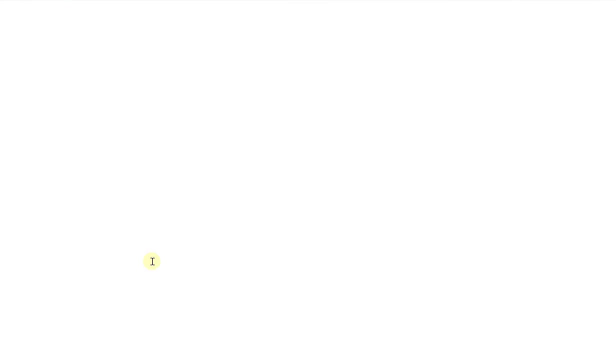 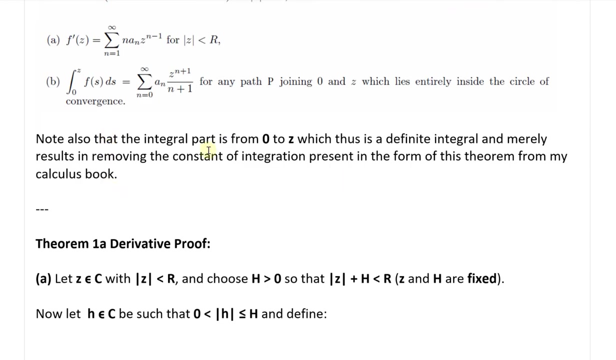 z is replaced with zero, so it's from zero to z. anyways, i'll- i'll be getting into that uh later in this proof, all right, so let's just keep scrolling uh right to it and see what we can come up with. so where is the proof? all right. so now that we got, uh, yeah, just shown that just. 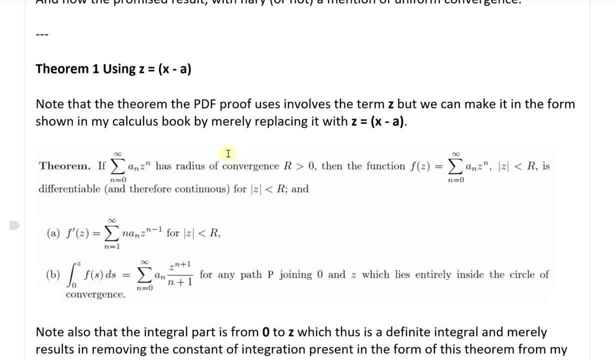 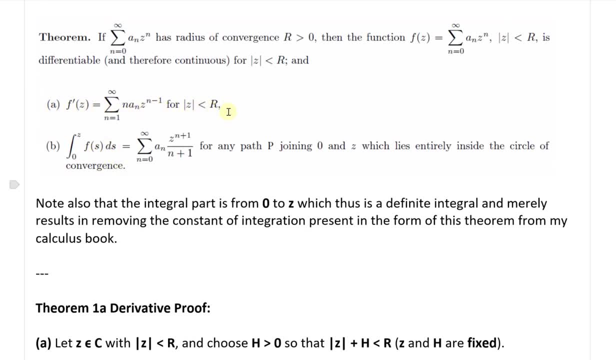 show the differences between the uh, the theorem and my calculus book, how it's presented in the theorem and the pdf. but they're the same thing. so now let's look at theorem 1a, which is the derivative proof. so look at this part right here. so let's said, be an element of all numbers. 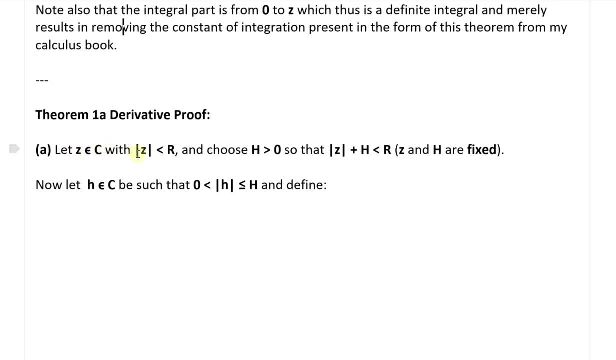 again, this is all. numbers are all real or complex, with absolute value of z is less than r, where that's a radius of convergence and choose capital, h is greater than zero, so that we have this scenario where you have absolute value of z plus absolute plus h is less than r. yeah, so where? 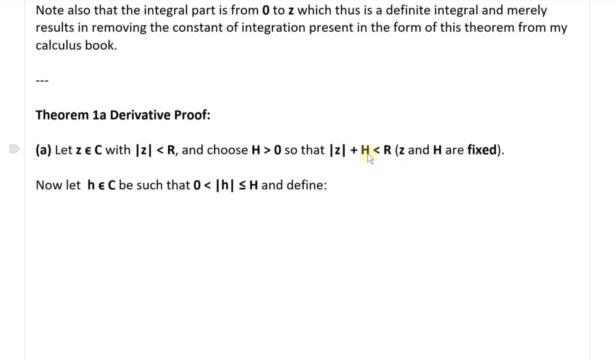 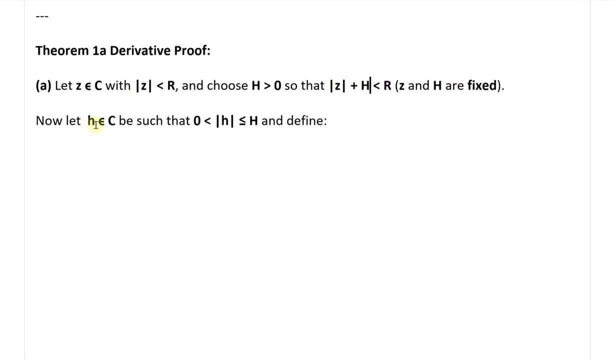 z and h are fixed. so we're just setting this, defining this h such that when you add it with absolute value of z, it's still going to be less than the radius of convergence, and this all makes sense as i get through this. and now let h be an element of- uh, yeah, also an element of all numbers. 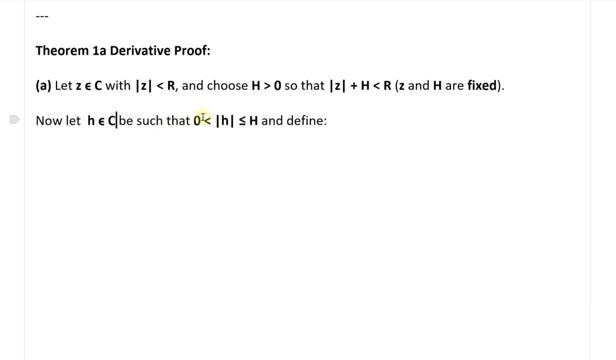 all real or complex- be such that, yeah, such that the absolute value of this h is greater than zero, and uh, it's, yeah, it's greater than zero, and it's less than or equal to capital h. so it's going to be, yeah, smaller than this one right here. uh, so that when you add as this absolute value of h to 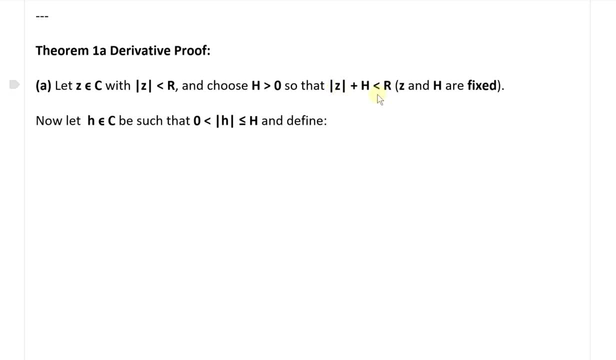 this absolute value of z. it's going to be less than the radius of convergence and we're going to define. so what we'll do is define f1. yeah, we'll define. f1 of z is equal to, equal to the summation here, and we're going to go from. 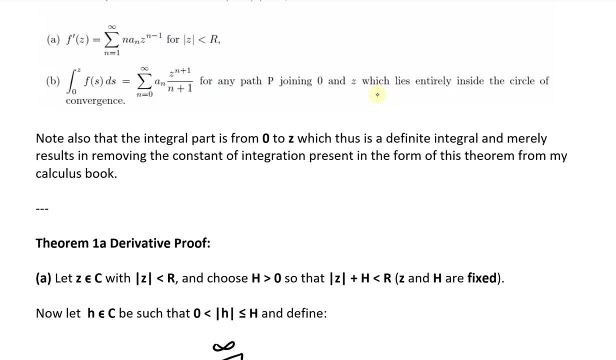 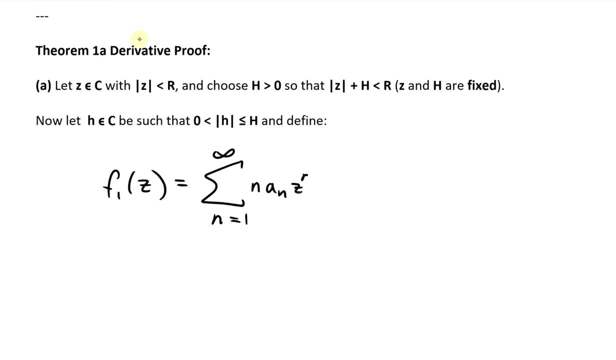 n equals to 1 up to infinity, and we're going to just set it as the inside term right here of this derivative there. so n, a, n and then z to the power of n minus 1. and this is for, uh, this is for when absolute value of z is less than r, the radius of convergence. yeah, so essentially we're just 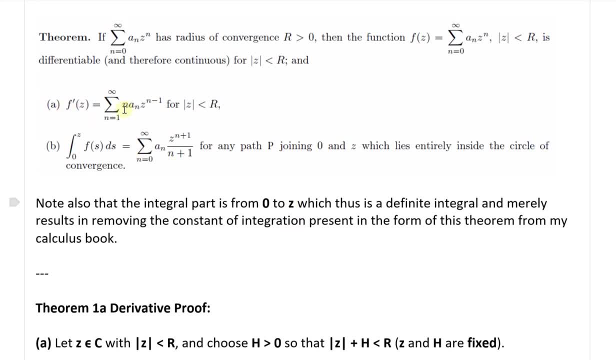 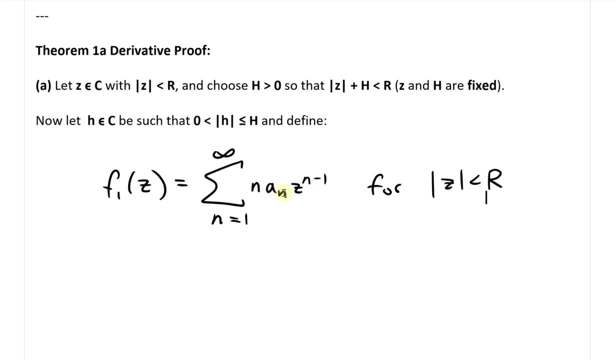 defining this function here and we're going to set it as the inside term right here of this derivative as this: and now we got to prove that it's actually the derivative of this function that's written as a series of this: a, z, n. so we're just going to define this function right now and then this: 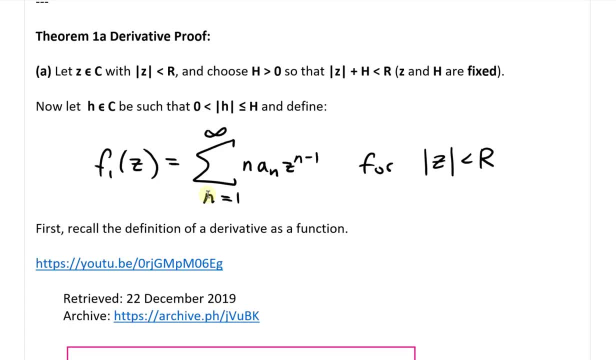 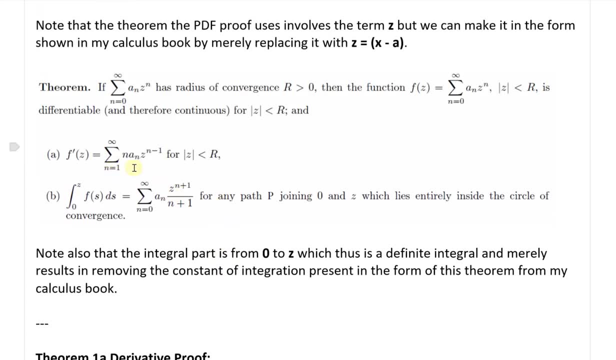 for the radius of convergence, absolute value of z is less than r. yes, and also another thing i want to note is that this one starts from n equals to 1. so if you scroll up here, this is from n equals to 1, just because if it's n equals to 0, it's just going to go advantage to 0, so that doesn't matter. 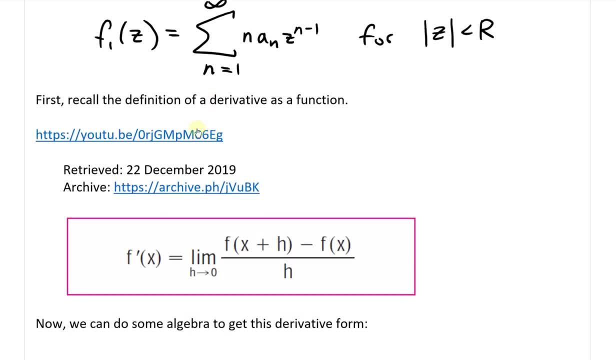 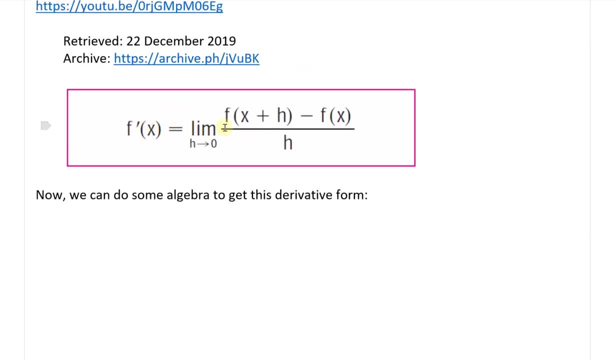 which one you use, but anyways, we'll just jump right in with. n equals to 1. so now, first we want to define the derivative, we want to find the derivative, and that's what we're going to find here. so the derivative is equal to the limit as h approaches 0, and hence why we have h, uh, this. 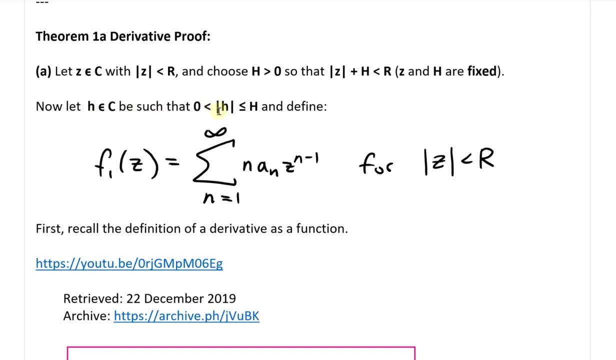 absolute value of h is greater than zero and it's going to be less than this term there, just to later. we'll ensure that it's all within the radius of convergence. so we're going to have this h there. so when you take the limit as h approaches, 0 of f of x plus h minus uh, f of x, all the way up to. 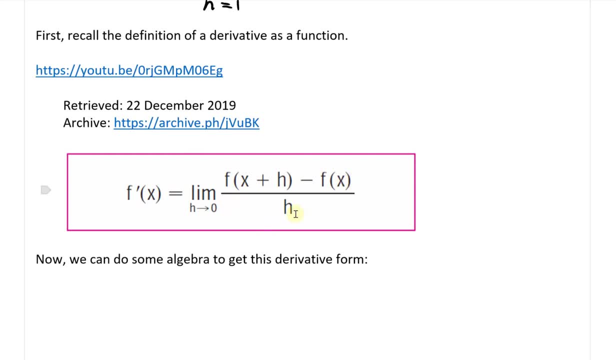 zero. so that's the whole idea of the absolute value of h. so that's the whole idea of the limit. so we're going to think of the definition of the derivative as a function from my earlier video and divided by h. in other words, here we're adding this, here this is just a slope, so we're just taking the. 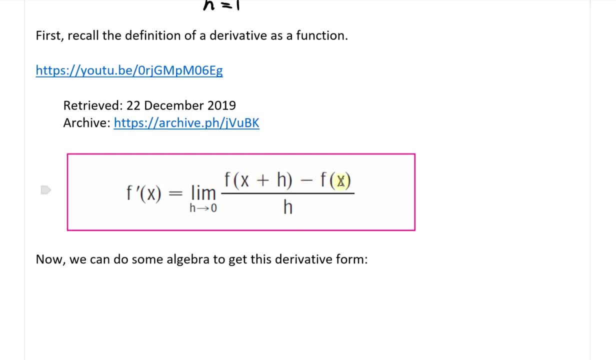 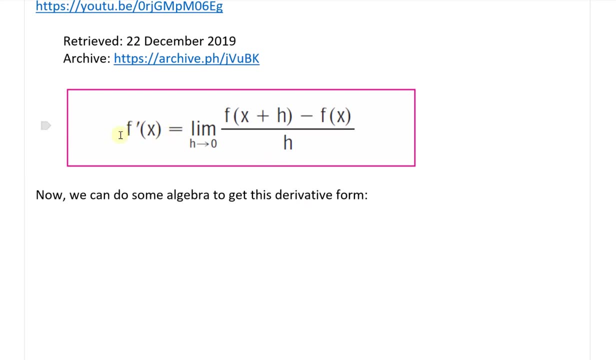 you're taking the limit of this h, where the top is just going to be a change in f of x, so the difference between fx plus h minus fx, and then as a slope as you make this h go to zero, that that is our derivative or our instantaneous slope. so now we can do some algebra to get this derivative form. 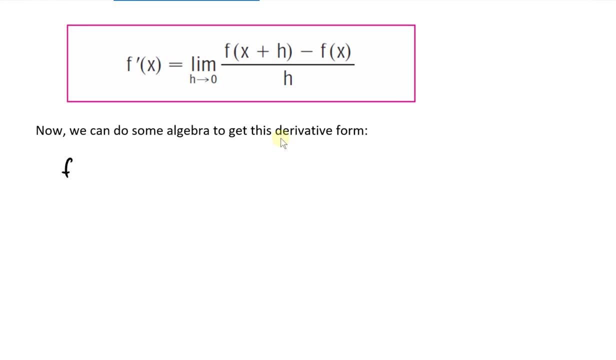 yeah, so what i'm going to do is uh, write this like this: i'm going to write f of z plus h, and i'm going to minus this by f of z. so this is our function. uh, this is our function: a z, n. so that's. 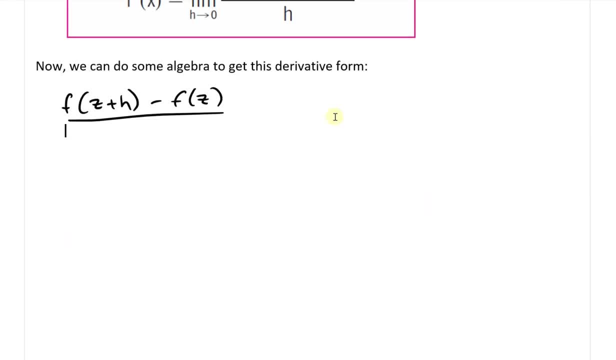 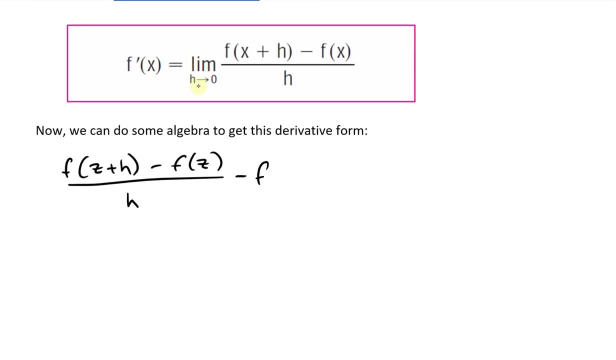 this one right here, and then divide this by h, then now i'm going to subtract by the uh f1, which is our derivative that we've got to prove. so then we're going to subtract this by f1 of x, like that. now what this ends up equaling when you write this in series notation: uh, this left side right here. 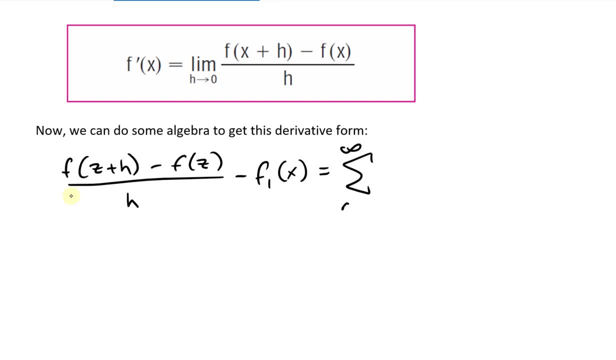 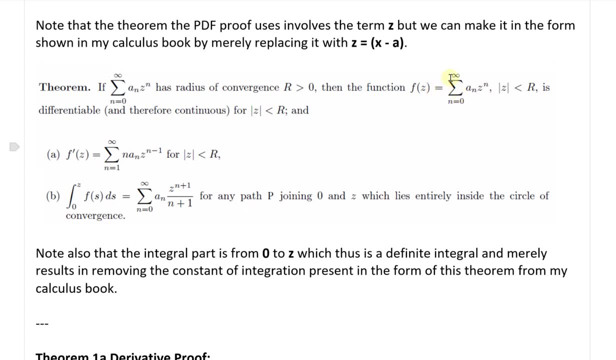 this is just going to be uh from infinity, from starting to the left side. right here, this is just going to be from infinity from starting from zero. so that's our uh function. right here, f, f of z equals to uh. the summation from n equals zero to infinity of a, n, z, n, uh, z to power of n. so now what we're going to have is well, uh. 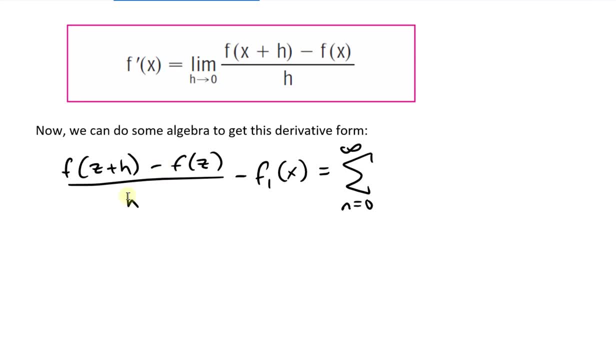 when we just put this all inside the same bracket. so, uh, this, this case, right here, this f, uh, f f of z plus h and this f of z have the same a n, so we just factored that out. this is going to be now. uh, this is going to be the inside. here is going to be. 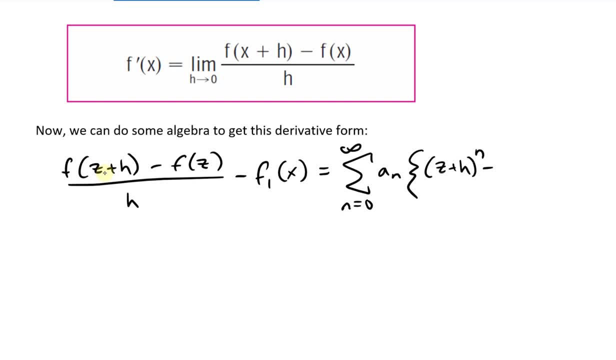 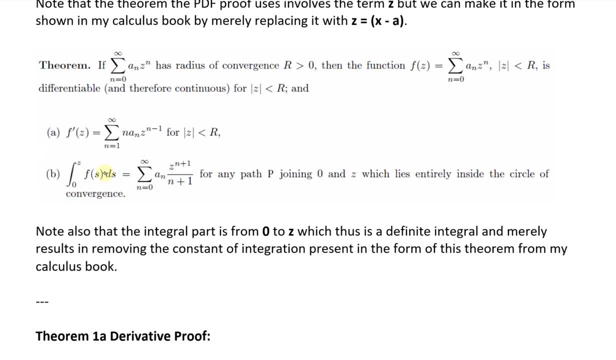 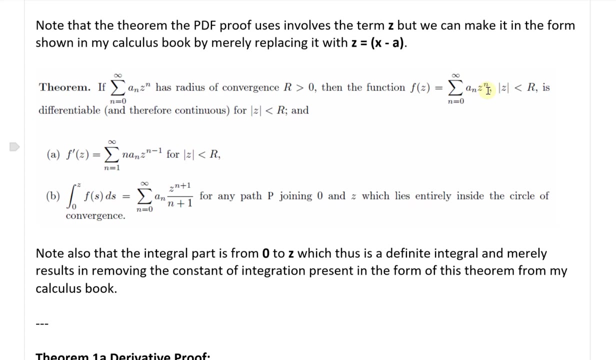 z plus h to power of n, and then minus just z to power of n, all divided by h. right there, like that. and and again, that's just this, uh, right here. so when you plug in uh a, this is a n. so when you plug in z plus h, and then then we're going to subtract by the z to power of n only, and then 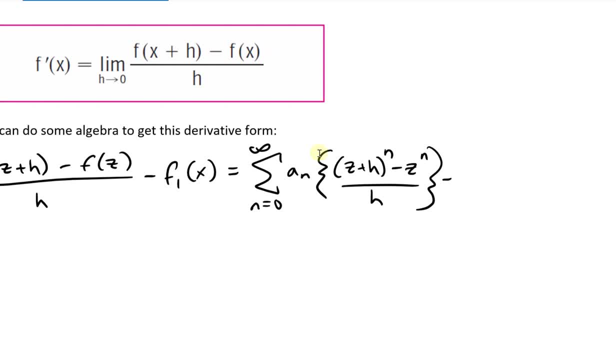 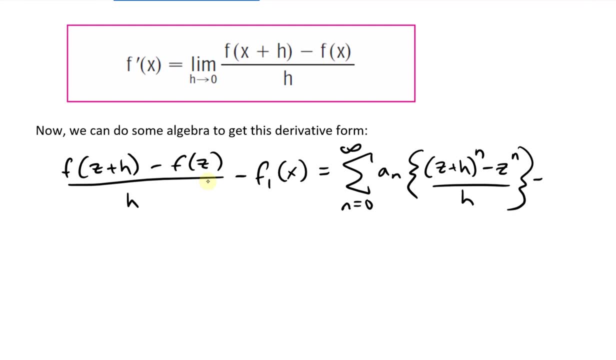 now we're going to subtract this by the difference and, uh, the idea here is: uh, we want to make, the we want to make, if we take the limit and make sure that this is: uh, yeah, these are equal to each other. in other words, that the, the, when you subtract this, should equal to zero. uh, or less, or yes, or. 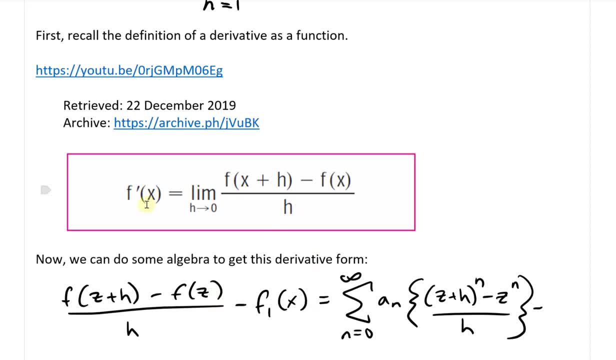 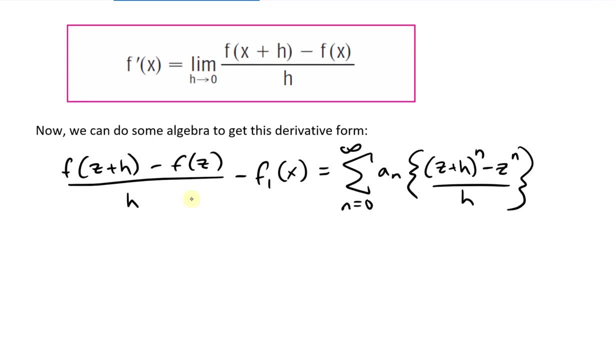 something like that, as i'll get through the proof and then we can just move this around and show that this f1 of x is actually the derivative. if you want to jump ahead, there's no room there, so i'm just going to subtract here now, subtract from f1 of x, and f1 of x is we're defining it as this. 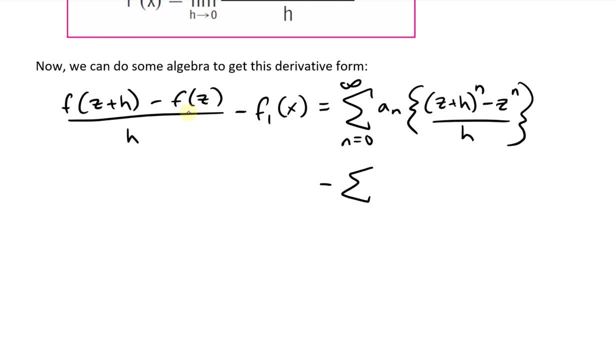 right here. so that's going to be the summation up to infinity of n equals to 1, so start from here. n, z, n, uh, minus one. so yes, that's exactly this right here. also the a, n. so let's, yeah, so n, a n, z and minus one. yeah, actually, on my the pdf proof. actually, i forgot to add in a n there. 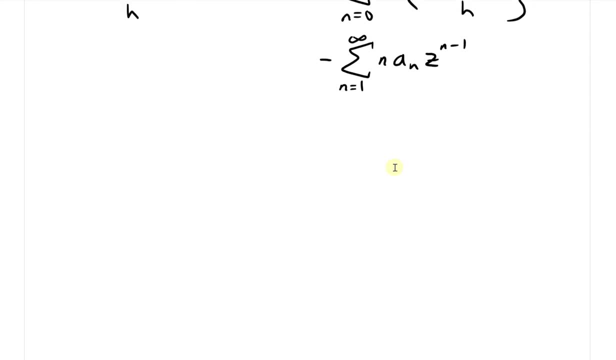 uh, so it had a type: yeah, so now what we could do is, uh, we could uh, multiply the top and bottom. yeah, multiply the top and bottom of this one right here by uh h over h, but uh, we'll do that in the next step, actually. so now what we have here is this gonna equal two, and uh, let's just 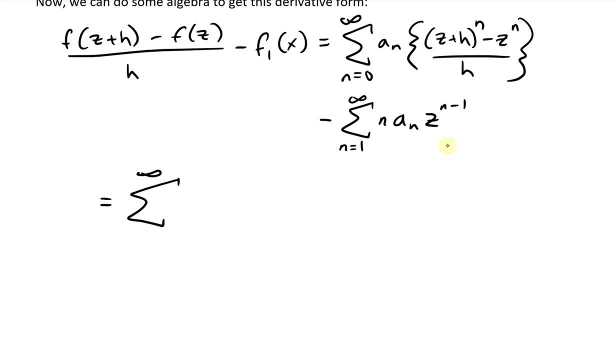 put this all in on one line. uh, the summation from this is uh infinity. um, i'm gonna write n equals two and in fact this is gonna be n equals to one. i just wanna make these exact same starting points: n equals to one, and we can do that because this summation right here, or? uh, yeah, the summation. 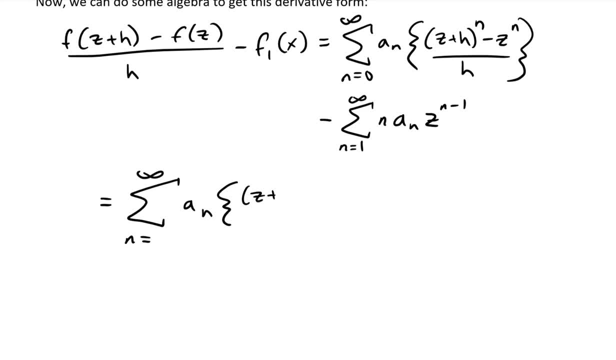 let's write this down: uh z plus h n minus z n. uh, this is. i'll divide this by uh h. so at when you plug in n equals uh, zero. there, what do we end up having is uh, that we're gonna have um. uh z plus h is zero. so let's write this: 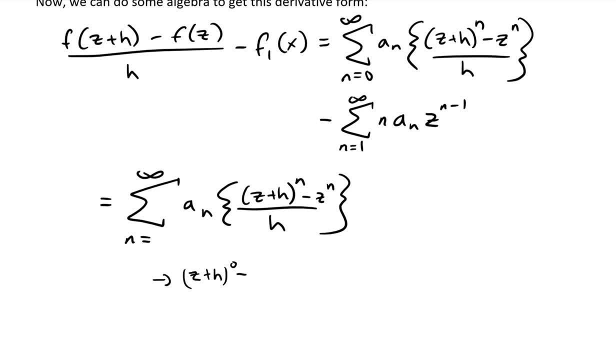 down z plus h to power of zero minus. uh, right here, z to the zero. this is gonna be a. one minus one is equals to one minus one, anything. power of zero is one subtract that we get zero. so this all vanishes. so we just start from here. 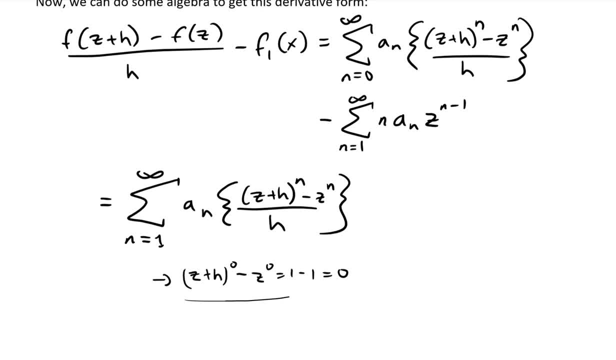 like that. i'll just put this in uh, bold, or just a circle as lightly. yes, we'll have a zero times an, a n, uh divided by h, doesn't matter, this one's non-zero, so this all vanishes. so we'll just make this so that it's the same: n equals one there and now we subtract this by this term, like here: 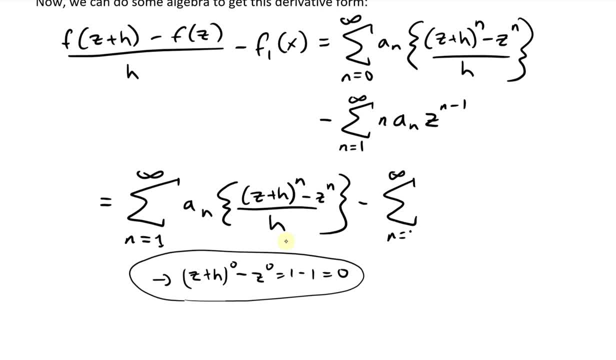 yeah, so here, a from infinity up to n equals one, and then i'm gonna again multiply this by, so i have the same common denominator there. i'm going to multiply this by h over, uh, h. let's multiply this h over h so that we can combine all of these powers. i mean, we can just 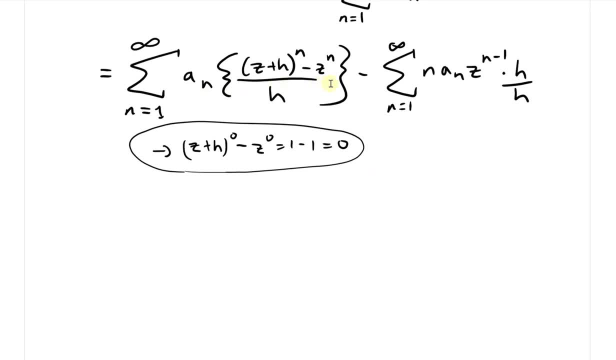 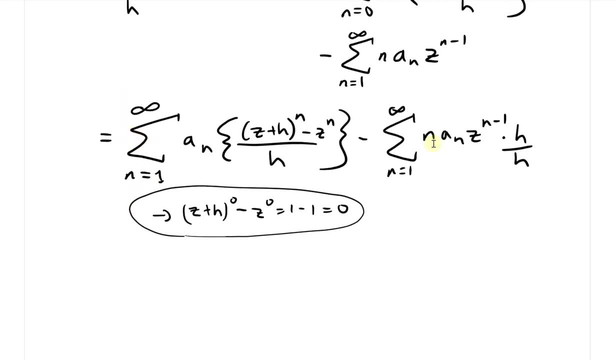 combine these all in the the same fraction, uh. but also now, because these series are the same, we can add these up according to the earlier theorem i uh. i referenced uh before, where if you have a subtraction or addition, you could just sum these up together when these are, from start, same starting. 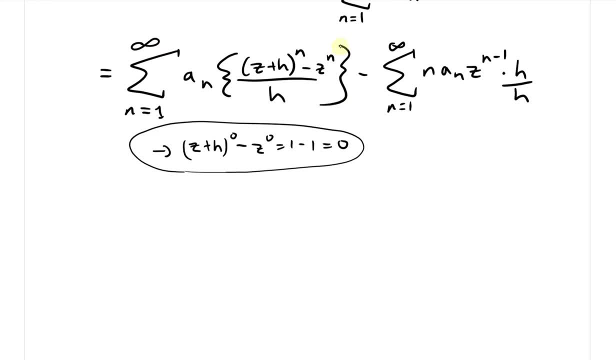 points: n equals one to infinity. n equals one to infinity, and also now we have the same common denominator there, so this is going to equal to now. the summation of n equals one to infinity, and also now we have the same common denominator there, so this is going to equal to now. 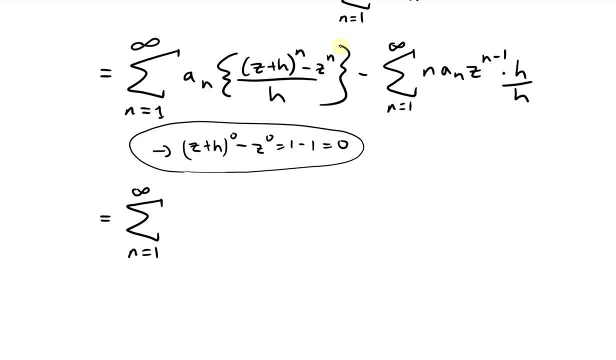 up to infinity of n equals to one starting point, and this is going to be a n. and now a n is factored out on all sides like that: now it's going to be a z plus h to the power of n minus z, n, and now we're going to minus this part right here. and then we factored: 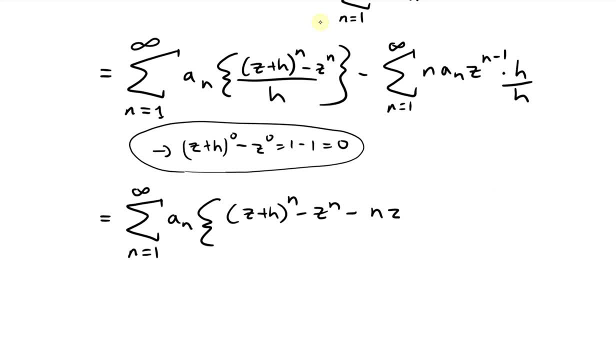 out the a, uh, the a n out. so we're just going to be left with n, z, n minus 1, and then we're going to have a z plus h, so h. so yeah, multiply this by h, all over now the same common denominator of h. 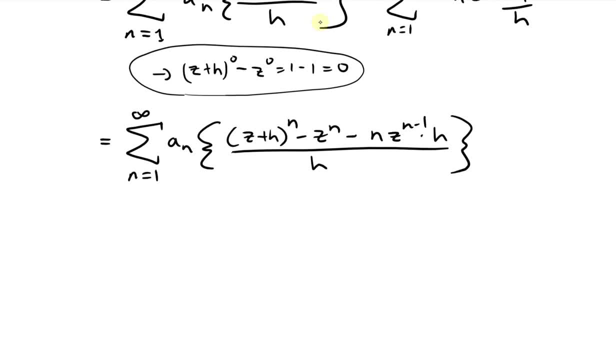 like that. and now this is uh, from n equals one, but what we could do is- well, you know, notice, what we could do is uh, yeah. so to go even further, we have another part where we can do a zero. so instead of putting one there, uh. so note here: 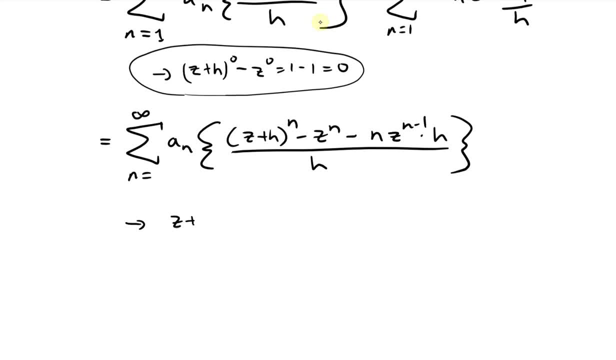 if, uh, if n equals to one, we have a z plus h to the power of one minus a z. one minus a one times this is going to be z to the zero. uh, yeah, one minus one is zero, and then times it by h. so, in other words, what we end up having is this: equals to z plus h minus z. 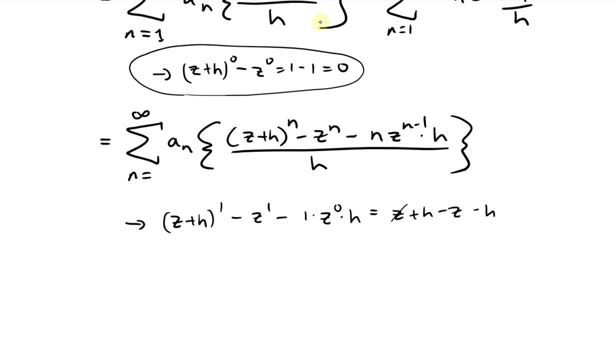 minus. this is goes to one minus h. so in other words, this is going to cancel, this will cancel. oh yeah, so these all cancel, the z cancel and the h's cancel. this equals to zero. so this becomes trivial. that goes to zero. so we just start from. n equals two instead, so start from there. 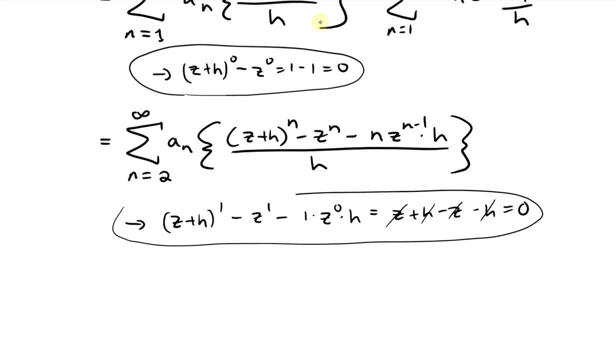 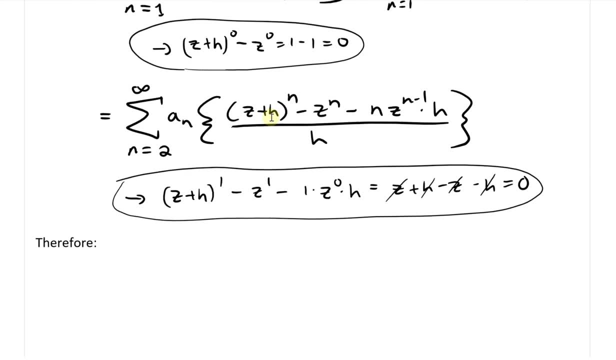 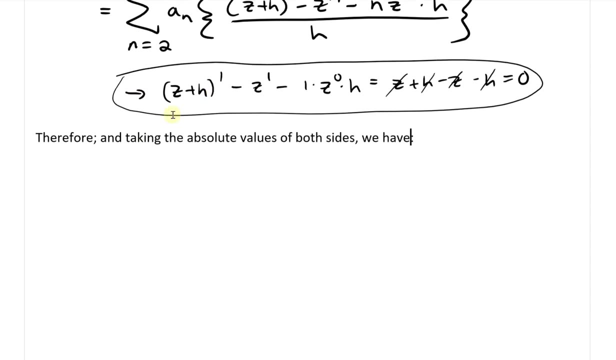 instead of the other one and again bold this one out like that. all right, so now, therefore, what we have, and just put this all into one line. so put this starting point and then this big giant summation there. so therefore, uh, the yeah when you take both sides, and also, uh, you're afraid. 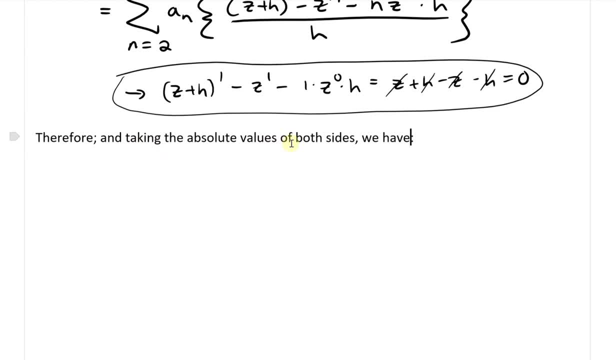 to mention this. so, and taking the absolute values of both sides. so let's take the absolute value of this and, uh, that's going to be equal to the absolute value on both sides. so let's write this all out. so this is going to be f of f of z, but it's also going to add these three first things. 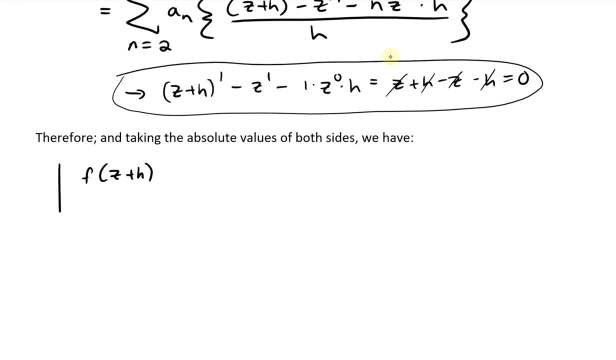 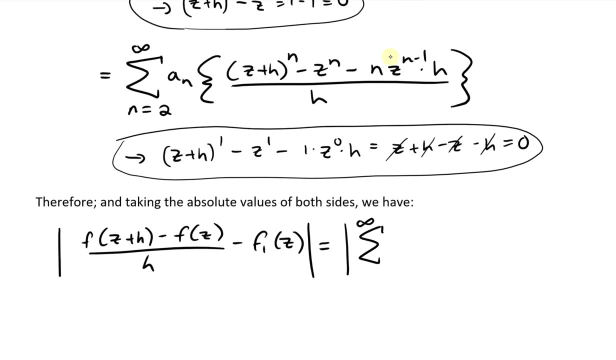 and then this is going to be equal to f of z, and then this is going to be equal to the sum of the of z plus h minus f of z. i'll divide this by h minus f1 of z, so now this absolute value equals to the absolute value of this entire thing. there, the summation from n equals to 2, up to infinity. 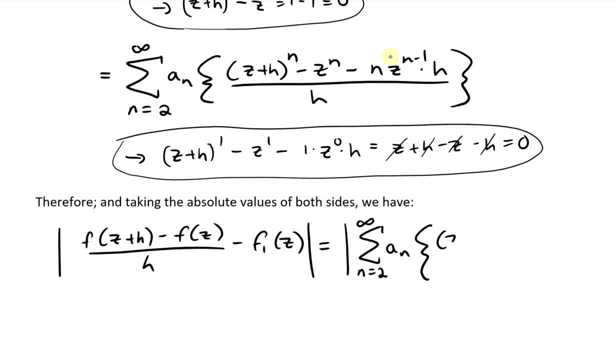 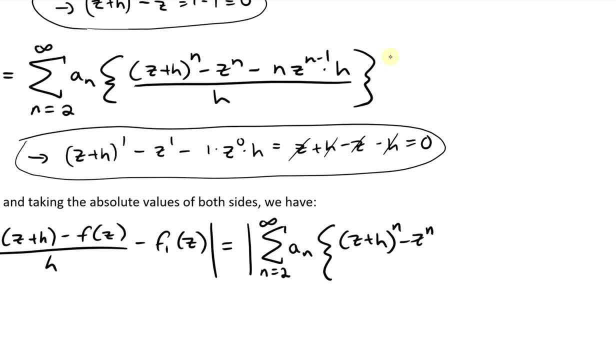 of a n, then giant bracket. we'll have a z plus h, power of n minus z n. now we're going to move this over: minus n z, n minus 1 h. i'll divide this by h and then close bracket like that, and then absolute value of the whole thing. so, yes, a big giant uh series right there, all right. so now that we have 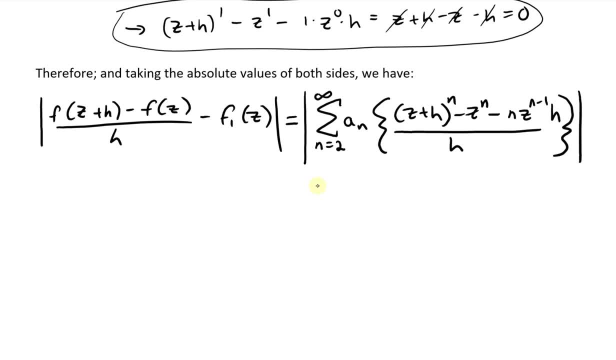 this part and how. this were the pdf you proof, uh, doesn't uh explain at all, but uh, it jumps right away to this point, this point, right here, and it does this, uh, using the binomial theorem, which i'll go overview after. i just write this down just to show how i was confused at what just happened. so from n equals to infinity. 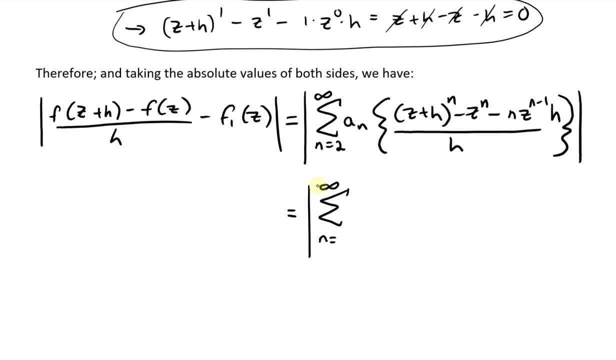 yeah, summation from- i mean summation from n equals to 2, to infinity, and now we'll have a n, and then what it did was it adds another summation inside. uh, so then it's going to be a summation, and it starts from k equals to 2 up to n. so this is summation, this one. 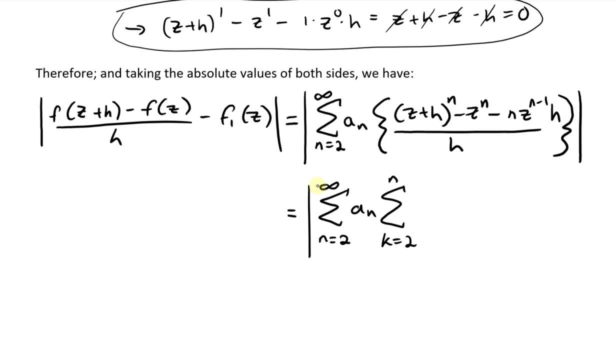 then uh, where this n depends on this one right here, and then we have a double summation right here. then it uses a uh n choose k factorial to be able to understand what this was, just because i haven't uh done this in a long time. so what we have is now z to the um n minus k and then h k minus. 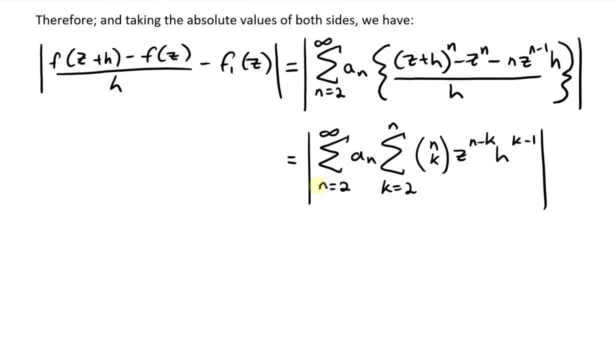 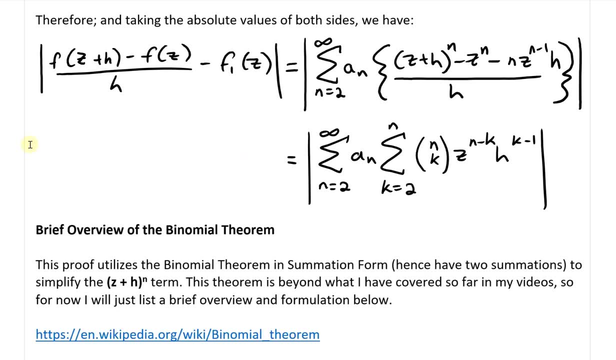 1, all absolute values, and then we have a double summation right here, and then we have a double summation value. so now to illustrate what this, uh, this, uh mumbo jumbo is and uh, yeah, now, before i go over the brief overview of the of the binomial theorem, what i'm going to do is i'm going to write: uh. 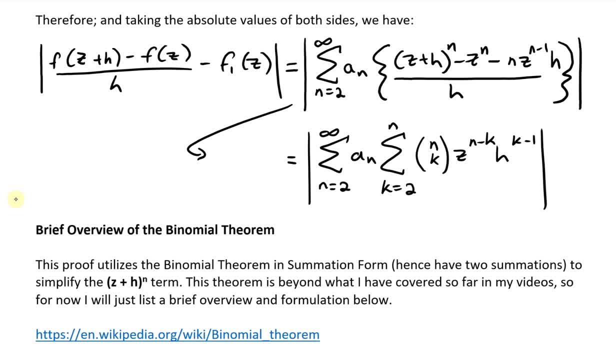 the pdf proof: uh, magically jumps to here. so it goes from here and magically jumps there, with zero explanation, magically jumps to, or here's where i rewrote that. so pdf proof magically jumps to. uh, yeah, it jumps to that one here. so i'll circle it and i'll do it again, and i'll do it again, and i'll do it again, and i'll do it. 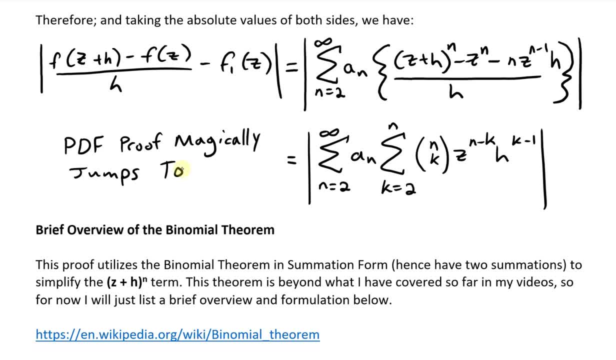 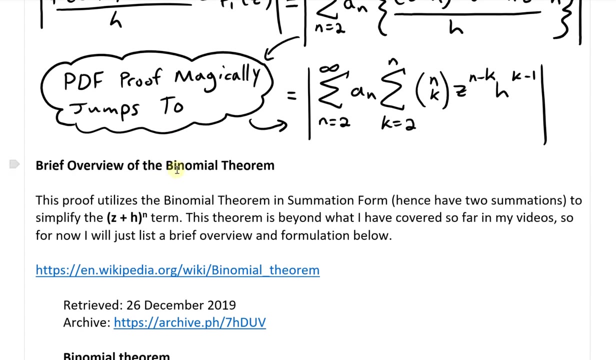 all this. or uh, put a cloud, actually for magic, so it just magically just jumps from here, yeah, ignores all the stuff that got into putting this and again- and this is matthew's solution. so here at mes, uh, we actually have to uh derive the magic. so, uh, here's a quick, brief overview of the binomial theorem. so this proof utilizes the. 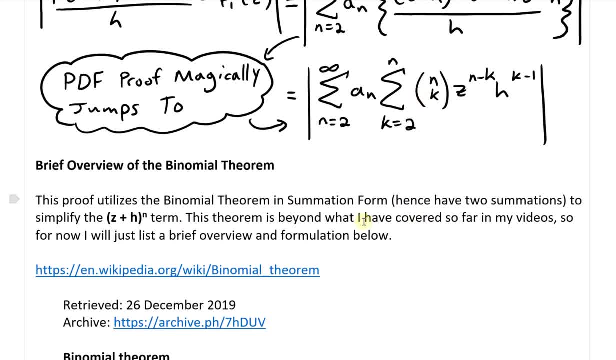 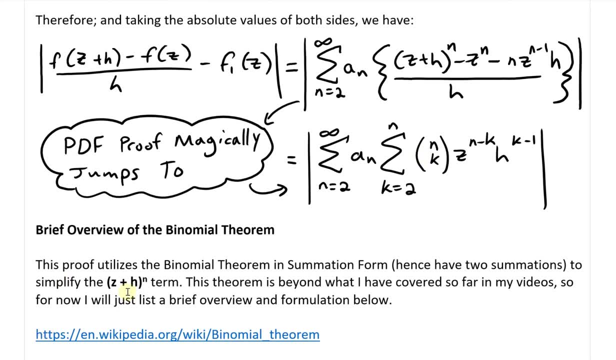 binomial theorem in summation form. hence we're going to have two summations. to simplify this term is zero 1 minus j, is zero plus n, and just 2 plus 1 minus t, and then we'll give y to the power. zero plus n is nothing but the z going up here. so when we look at it again, 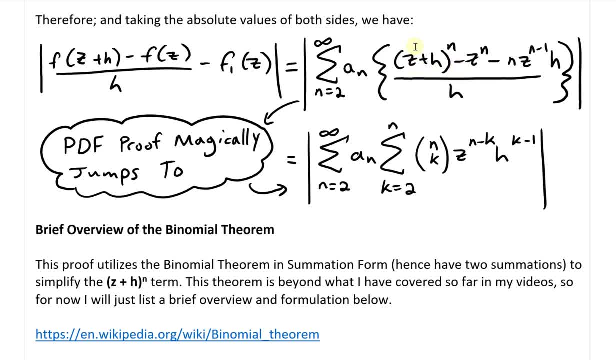 we should still, rather than looking at it again, say that j is the number of hours out of the binomial theorem. so it's gone higher. so we have one zero zero. decrease is one zero. zero minus zero. this is also essentially aอ. so what we're going to do is build back a部分. we're going to 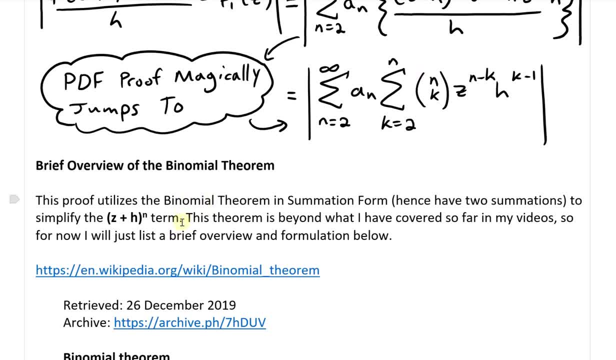 put in n and its transform into the prime derivative of r by n. this is the relative Iran weighted product of power of r. yeah, this time the expression of the n is a negative perché? uh, because at zero times, zero is negative, because the root of r is negative and then, when I apply this, profund is negative, so the root factor will transmit and push up toirezian. 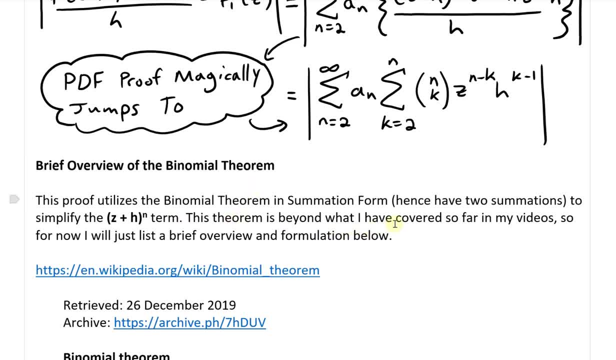 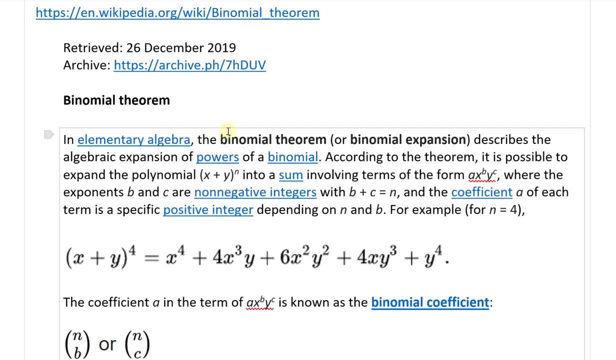 minus 2, etc. so this theorem is beyond what i've covered so far in my videos. so for now i will just list a brief overview and formulation below. series from wiki: uh- binomial theorem. in elementary algebra the binomial theorem or binomial binomial expansion uh describes: just make this um ignore. 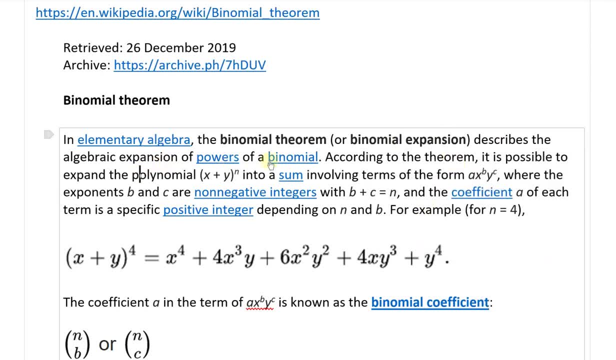 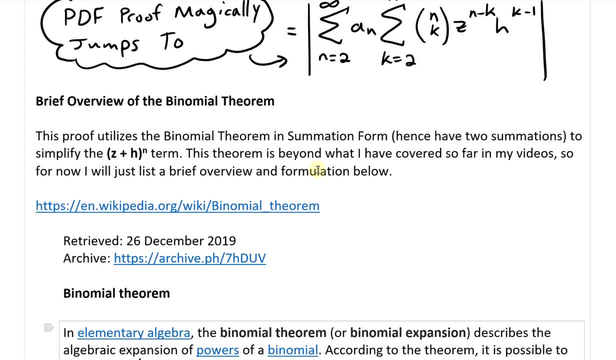 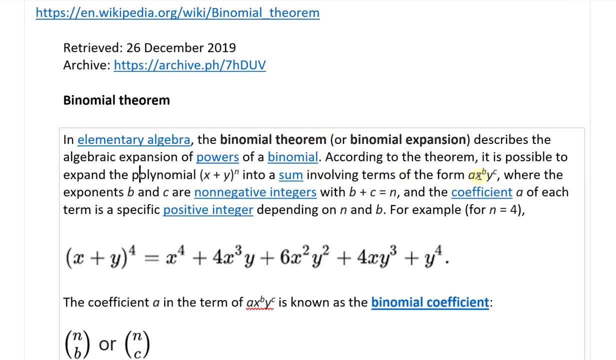 describes the algebraic expansion of powers of a binomial. according to the theorem, it is possible to expand the polynomial x plus y to the power of n. so again this is, but ours is z plus h to the power of n, into a sum involving terms of the form a times x, x to the power of b times y to the power. 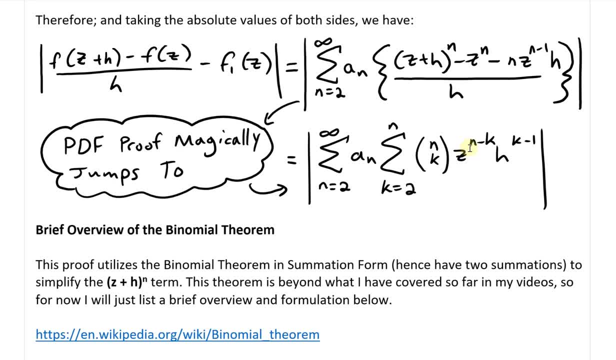 of c, so you can combine these all into this form actually z and h, so z and h there. yeah, plus coefficients a there and in fact this n choose k, uh this, uh this vector looking uh notation down here, and then you can combine these all into this form actually z and h, so z and h there. 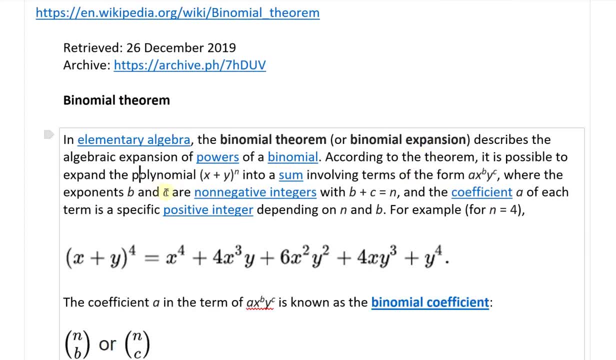 that's actually the coefficients, uh, where the exponents b and c are non-negative integers, with b plus c equals to n. so when you add those all, they're all equal to n. and the coefficient of a of each term is a specific positive integer depending on n and b. for example, for n equals. 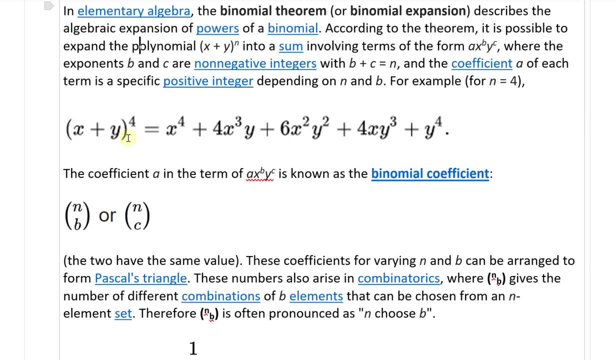 to 4. so we have this, if we expand this out, so x plus y to power 4 equals to uh x to the power 4 plus 4 x, 3 plus uh, yeah, plus 4. x to the power of 3 times y plus 6. 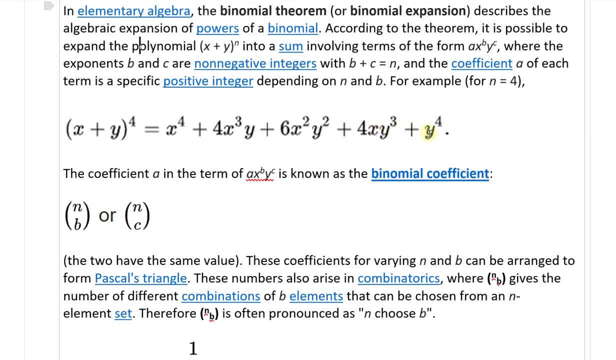 x squared, y squared plus 4, x, y cubed plus 4. i need a plus. lastly, y to power 4. so notice symmetry here goes from x4 all the way to y4 and at the end one has 4, x, y cubed, but this one has. 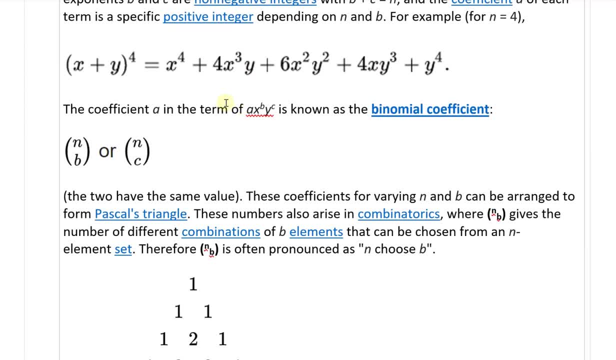 4 x cubed y, so it's very, very uh symmetric. so the coefficient a in the term a, x to power b times y to power c is known as the binomial coefficient and it's written as n choose b or n choose c. in fact these two both have the same value. 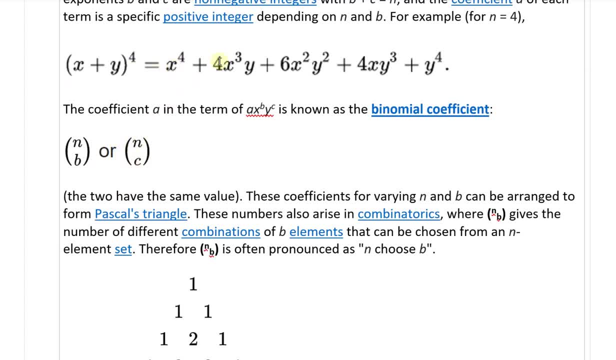 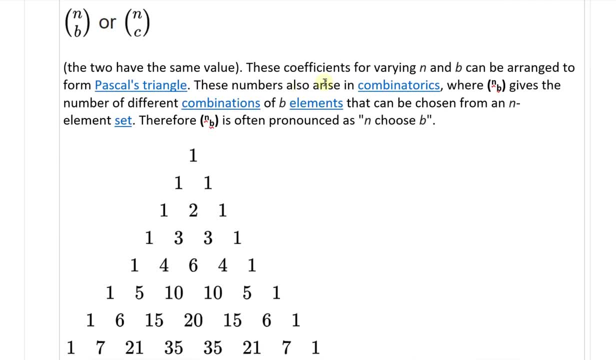 so this is just a notation for this coefficient, so it would expand out such that it equals to: uh, this right here. so this one's gonna be one, four, six, four, one, uh, these coefficients for varying n and b can be rearranged here or can be arranged to form pascal's triangle. uh, yeah, the famous. 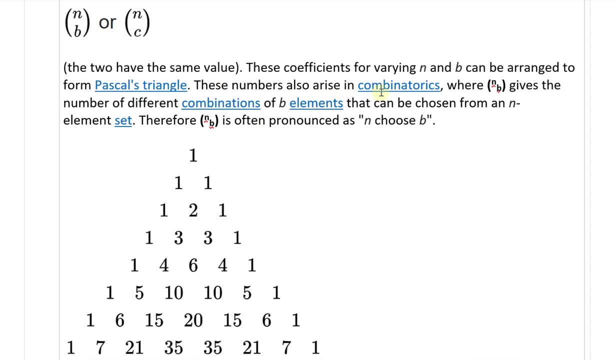 triangle, so these numbers also rise in combinatorics or probability. uh, where n choose b gives the uh. you just wrote it like that, i can't write it easiest for me to ignore. uh, so n choose b gives the number of different combinations of b elements that could be chosen. yeah, so there's a. 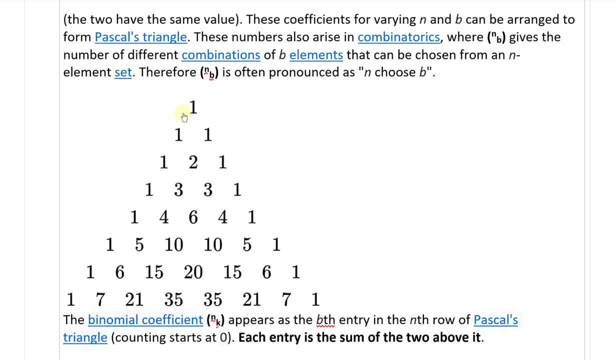 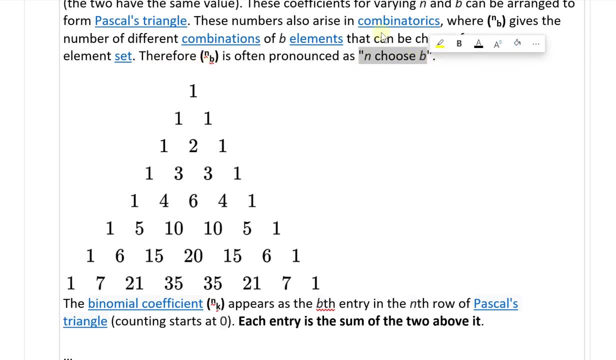 number of b elements to be chosen from an n element set. and again, yeah, this is beyond what i've covered so far- uh. therefore n choose b is often pronounced as uh yeah and choose b, so yeah. in combinatorics or probability, uh theory, uh this, uh, this number. right here, uh gives a number of 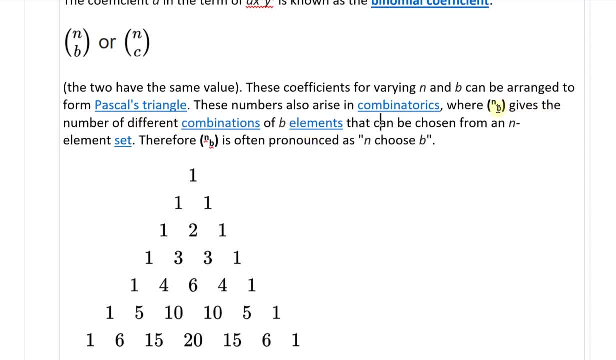 different combinations of b elements. if you have uh b elements, three inside there, for example, this is, let's say, five and it chooses. this shows the number of elements that could be chosen from an n element set. so, yes, uh, interesting stuff. so, anyways, i will be going over this. 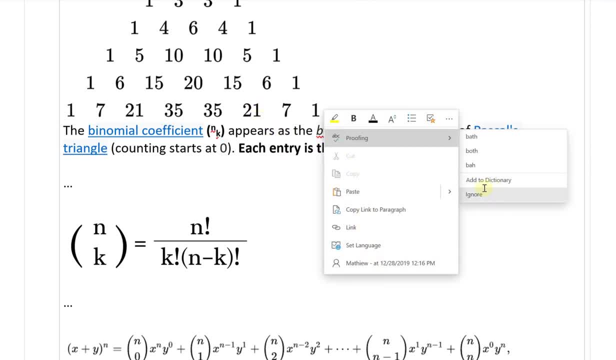 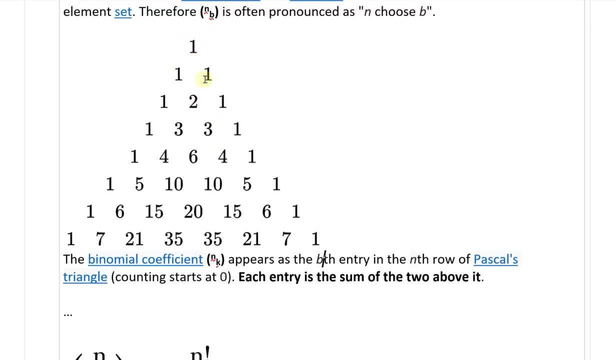 maybe in the future in detail, but uh, it's just a bit beyond what i've covered. so the binomial coefficient uh and choose k. so notice here, right here. so it goes from one, then one plus one, and this is gonna be uh, one, two, one, and then one, three, three, one, one, four, six, four, one, and this part. 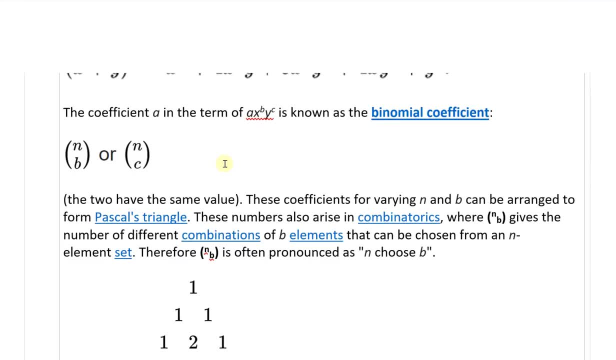 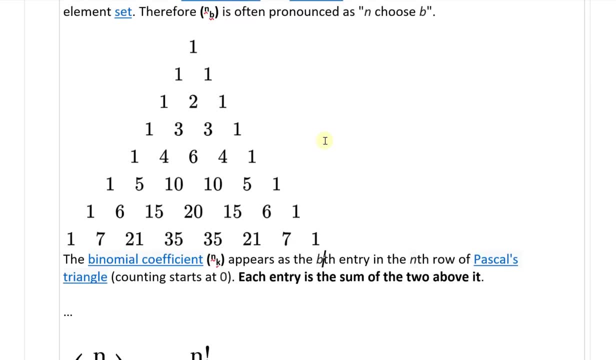 right here is the uh n to the power of four. so one four, six, four, one. that's the n to the power of. is uh, just right here, that's one, four, six, four one. so yeah, this one is the one we just uh in the example it showed, and then so on. it keeps going on and uh, yeah, so the binomial coefficient and choose. 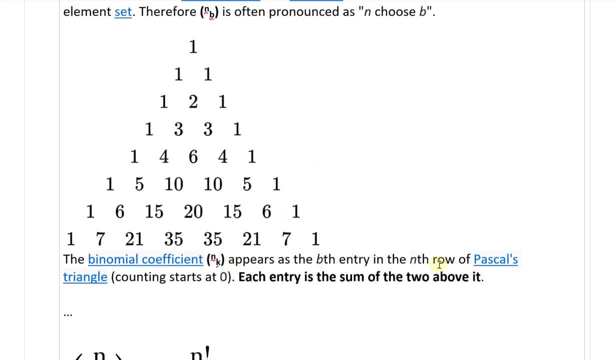 k appears as the bth entry in the nth row, so b would be a, one, two, three, four, all the way to n. and of pascal's triangles, counting starts at zero. uh, each term is a sum of the two above it. so this is a very, very interesting one. yeah, it's actually the sum of the two uh above it. so if you have, 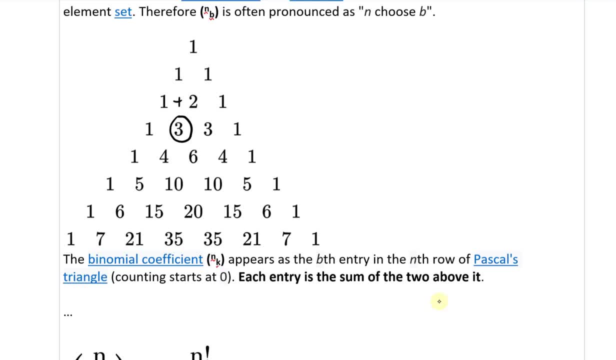 here this is equal to one plus two is three. so you can find the coefficients. so this one here 20 is going to be 10 plus 10 is 20.. interestingly, if you have here one, this is going to be well, uh, zero plus one is one. likewise, if you have here this is going to be one plus five is uh six, and so on. so 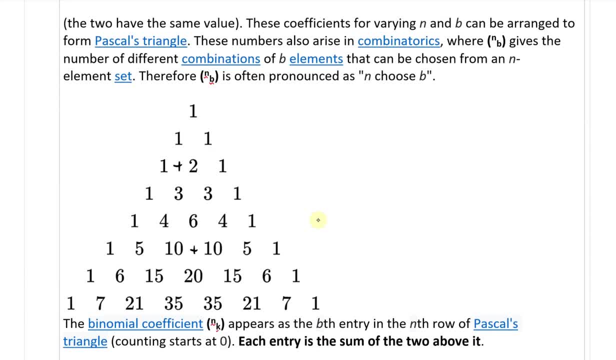 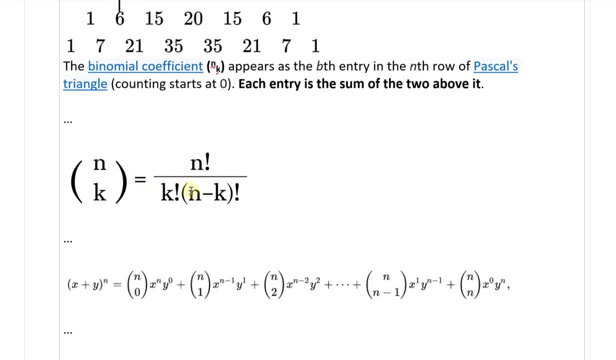 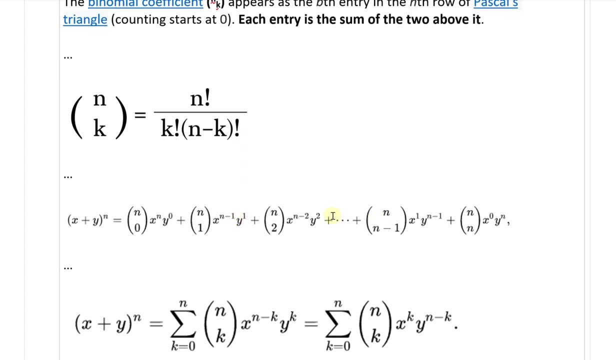 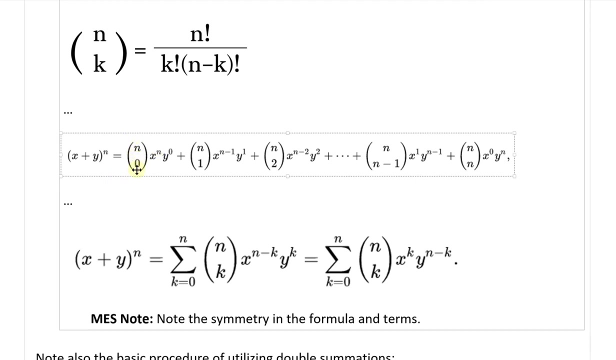 that's very interesting. so that helps how you go from here. it's actually quite interesting to see, uh, which part. but the difference between okay, so the variance factor here is going to be zero, and then we're going to go through, um, the знаю waiting bits. so i'm going to go into the interpol project here. here's a u, g of z, which 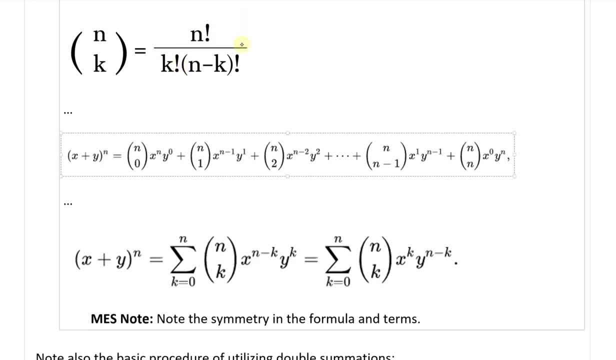 is going to be, um, your n minus zero, so that's gonna be n factorial, and so on. so, uh, this can be written as: again, i'm just showing the formulations, because, uh, this is beyond what i've covered so far, but anyways, you can write it as: n choose zero, x, uh, x to the x power of n times y to. 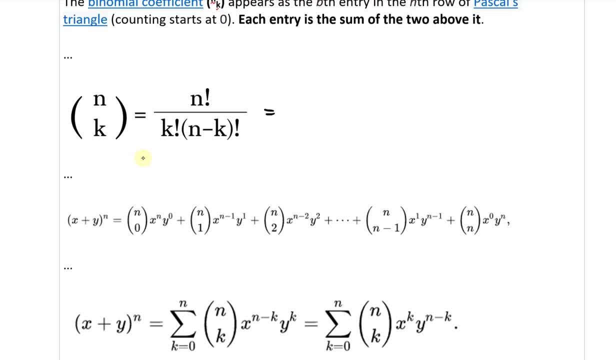 the power of zero. and this one here: n choose zero. actually, let's just write that down quickly. so, n choose zero. this one's going to be equal to n factorial over zero. uh, factorial, which equals to one. then now here we have n minus zero, so it just becomes n factorial. this cancels, so this. 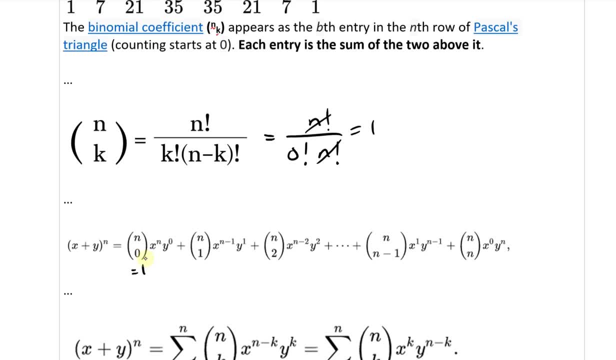 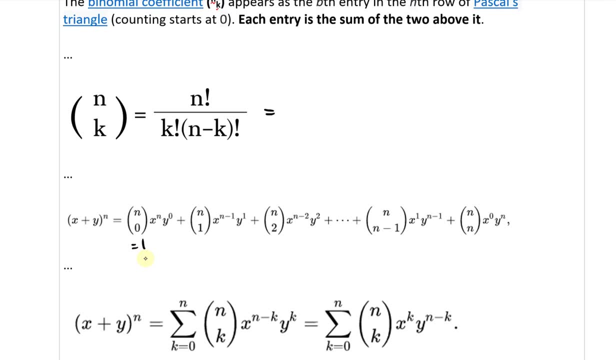 equals to one. so this coefficient is going to equal to one, and the first one again, that's that's our one, in every single starting point there. and also n, choose n. that's also going to be uh, zero and it's also going to be one. just by looking at this, you'll have a n divided by this can be. 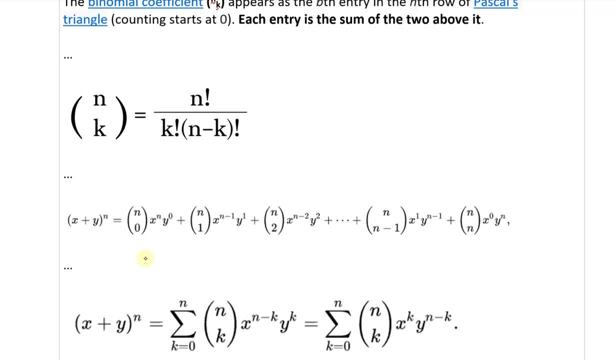 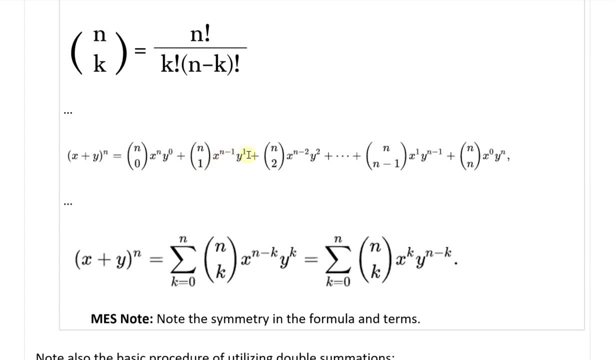 n. this one will be n minus n, zero, so we'll have n over n anyways. so then then, after that we have n, n, choose one x. uh, then we have x to the n minus one. this is y one. so notice this one that starts from n. then 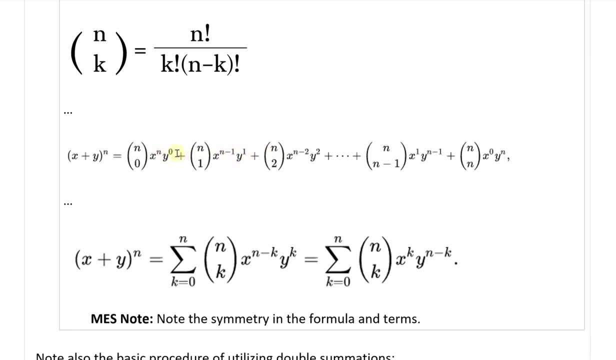 starts going lower and lower. and this one starts from: y is power of zero- and it starts getting higher and higher all the way to yn, and then xn goes zero, and then this n choose two and and choose n minus one, all the way to n choose n. so the n keeps going up, up and up. so, in other words, 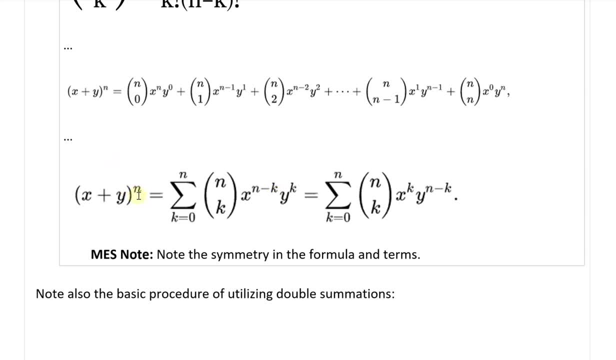 if you write this in series notation, so x plus y to power of n is equal to summation: from k equals zero to n of n. choose k, x to the n minus k, initially zero, so we'll have n, then when it's one, we'll have n minus one, and so 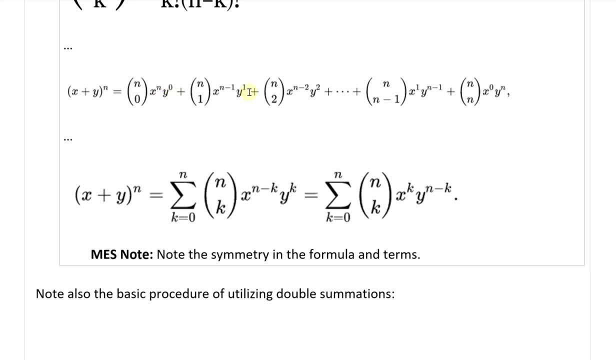 on where this starts out at. k is zero and k is one, with a for the y. so you could write it as here: times x to the power of n minus k, times y to power of k, now this equals two. the summation: uh, k equals zero. to uh, up to n of n, choose k and you could just rearrange this so this could be k. 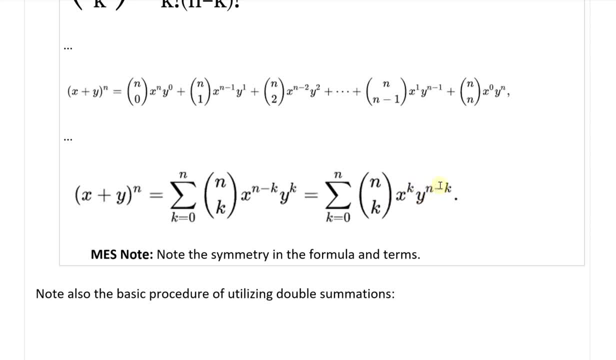 and this could be y, the power of n minus k, because you're just starting off from here instead. so y, n minus k, this is zero, that's going to be n, and then this one's zero, and then, when you add this up, this is this: just works backwards. so note the symmetry in the formula and terms you could use. 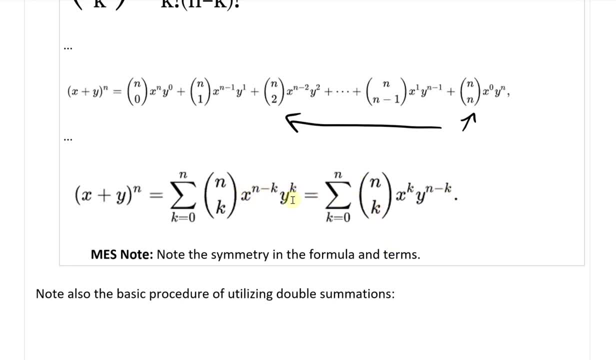 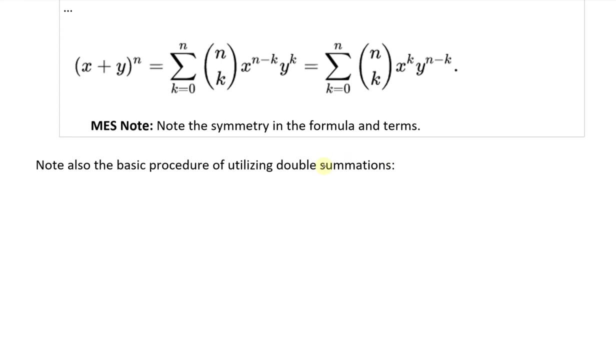 either uh n minus k on the x or um and then y and then k on the y, or reverse it: k on the x and y has n minus k, and you're all you're doing is going backwards like that. so note also the basic procedure of utilizing double summation. just, we're going to write this down, yeah, so just a lot of uh. 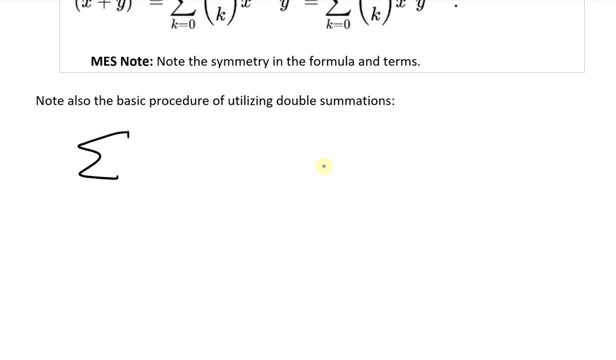 summations if you just have something like this, just to demystify what it looks like. so if you have something that starts from i equals one to two of the summation, uh, right here up to four, uh, where uh, let's say we have j equals to three and we just have i times j. so now this is going. 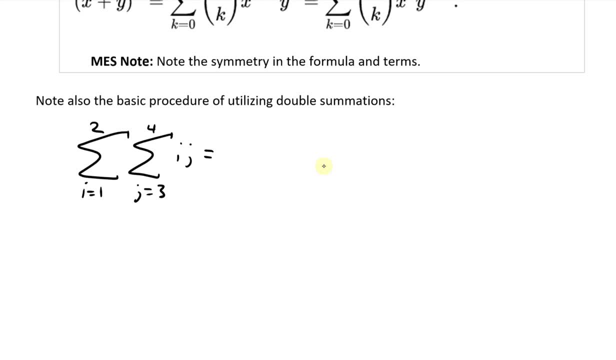 to equal two. yeah, this is going to equal two initially. we'll have, let's say, i is equal to one, so this is going to equal to four. we'll just create a matrix, so we'll have: i equals one times it by j, which is three, plus i is again one, j is four. so then you would increment, uh, the j's all first and combine them. 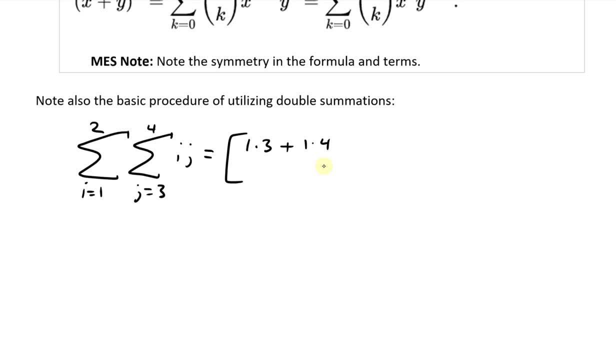 so one times four. and now, uh, this summation right here is equal to seven. and now we do. the next one is four, two, so for i is two times by, j is three plus. so now this: yes, so basically the i's increment downwards and then the j's increments to the side. so now plus two times four, this is going to be yes. 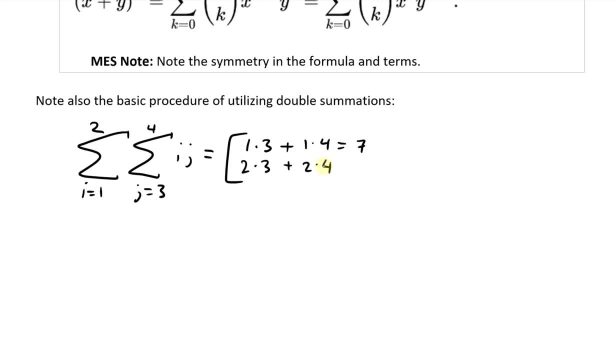 this is three plus four to seven. this one is going to be now two times three, is going to be two times three is six plus uh, two times four is eight. so eight plus six is going to be uh, fourteen. yeah, eight plus six is fourteen, and then we can combine these to seven plus fourteen. uh, this is going to 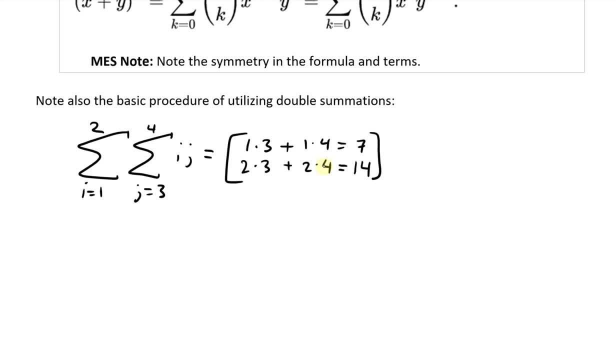 equal to uh, or just put an equal sign: equals to seven plus fourteen. so you just add up all the terms. now this is going to be equal to 21.. so that's just using a double, uh, double summation. all right, so now that we've got over the brief, the overview. 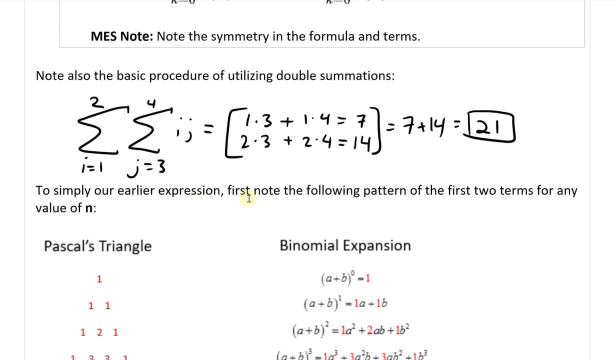 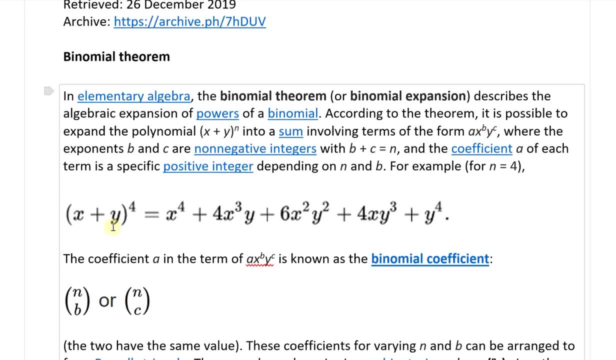 uh, uh, briefly. so now to simplify our earlier, our earlier expression: uh. first note the following pattern: the first two terms for any value of n: uh, before i get to that, just uh, notice here, because again this magically jumps from here to here: uh, it puts all of this, all these, all these terms. 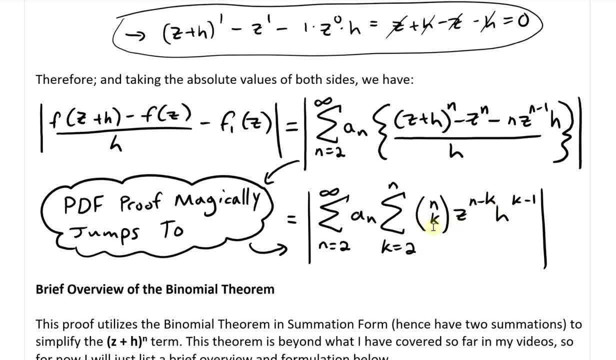 inside this binomial uh, uh, yeah, this, this binomial, uh, expansion, uh, in, in, uh, in summation notation. so so it puts all that it combined, it goes: it starts at k equals to two. so so what i'll do is: uh, i can, i'll show you how to transform this into this where uh, it goes from k equals to two, because 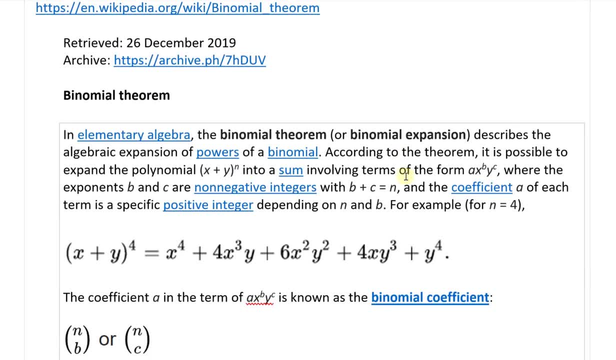 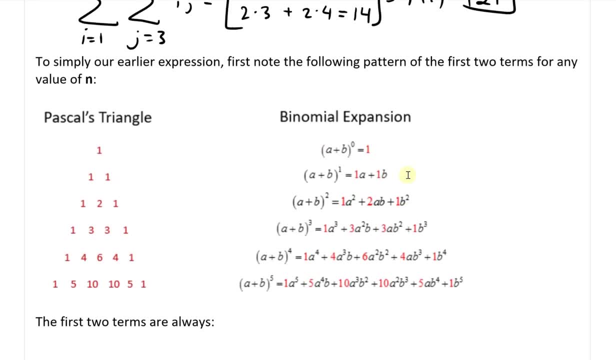 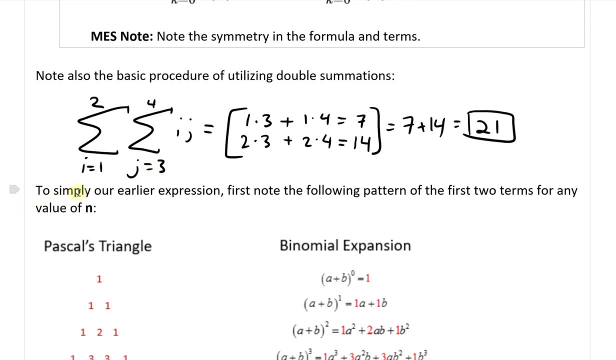 uh, k equals to zero, uh, or uh, yeah, or i'll show you what happens to the: k equals to zero, and so on, and k equals to one. so let's just scroll down here: yeah, so to simplify our, uh, to simplify, yeah, spell this wrong. to simplify: yeah, our, our earlier expression, uh, our earlier expression first. 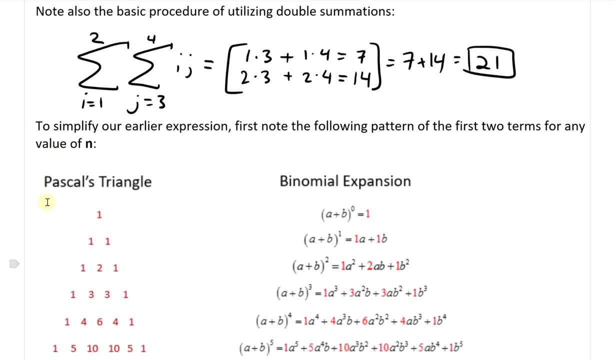 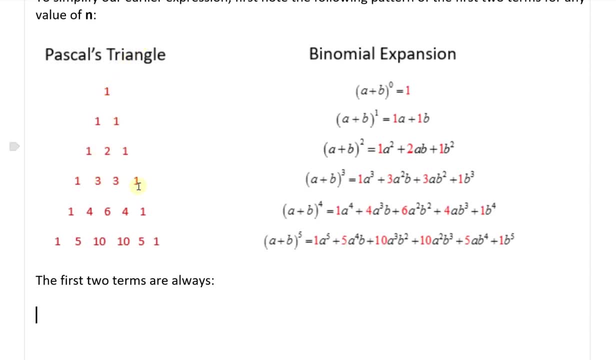 is the following pattern of of the first two terms for any values of n: yeah, so here is uh pascal's triangle. so it just goes one uh one, one, one, one, two, one, one, three, three, one. this is one, four, six, four, one, et cetera. then it goes to one, five, ten uh, ten, five uh one. so this is from uh a plus b to 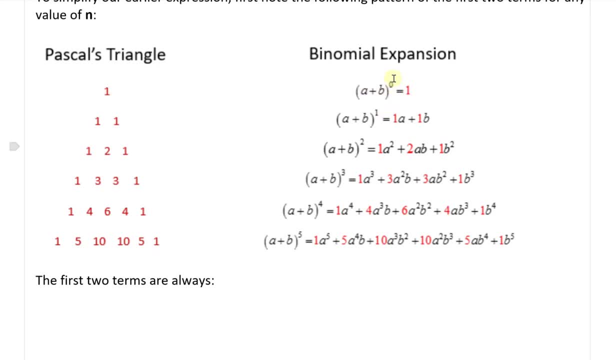 power of zero. this equals to one. uh, yeah, this is, this is anything. power of zero is one. and then a plus b to power of one is: is this going to be well, one a plus one b. and then when you uh square this one and it factors out to one plus two, uh, a, b and so on, and it goes to one three and 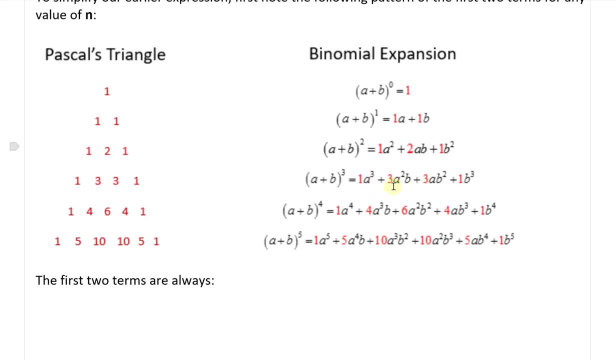 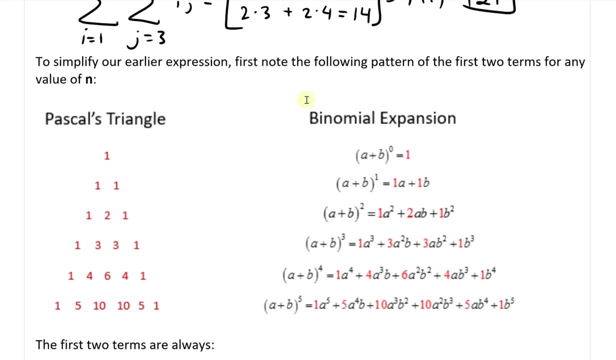 then yeah, then it goes to a a cubed plus three a square, b plus three, a b squared plus um, then it's gonna be one b cube. so for no first note the following pattern of the first two. i'll highlight this: first two terms, uh, for any value of n. so this is going to be n equals zero, this is n equals zero. 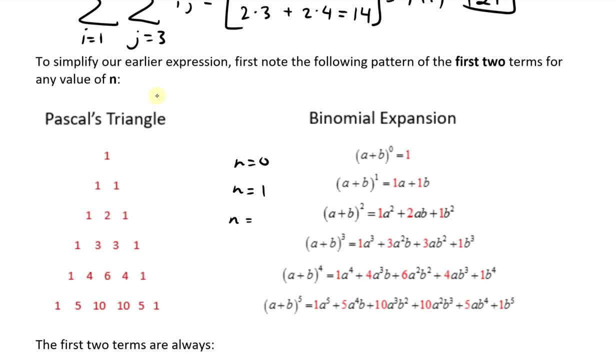 n equals to uh one and this is n equals to two, et cetera. and notice what happens here to the first two terms: this is gonna be one, and then uh. the next one is: uh, yeah, it's gone there, so this is gonna be one and then this one's gonna be- actually, i'm not gonna be more broad- uh, because it's the. 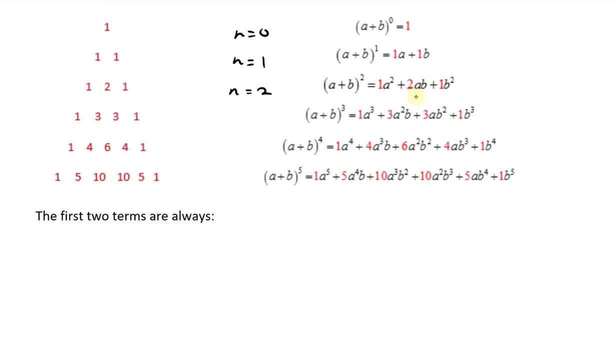 first two terms: uh. so let's just look at uh, a bigger one here. so if we have here, this is gonna be one a five plus five a four b, and this one here is one a four plus four a uh three b. so for this is the uh n equals to three. this is n equals to four, this 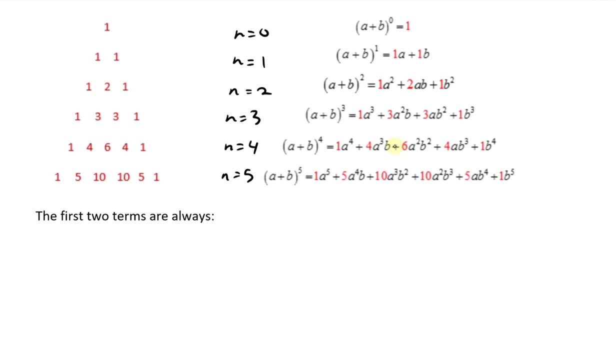 n equals to five. so now we have this: n equals to five. the second term is: is n? it's always n the. this one, this four is always to the four, so it's always n. three is always to the n. this one right here is always n, this one's always n, and so on, and likewise the first term is always going to. 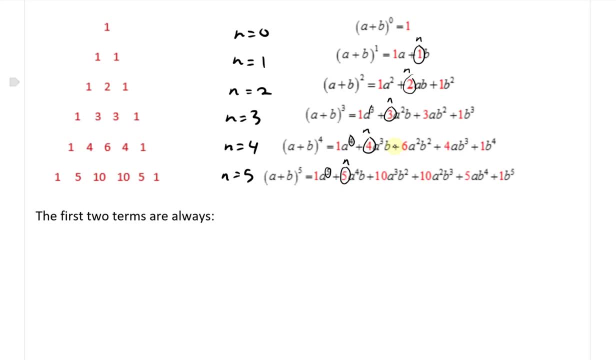 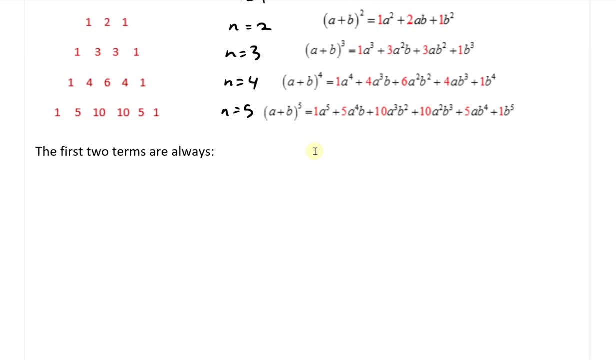 be n. so there's always a to the n, a to the n. they're both n. so all these are are all n? uh. so what, uh? what i'll do here. so the first two terms are always, and they're always going to be: if you have a plus b to the power of n right here, this is always going to equal two, uh, the. 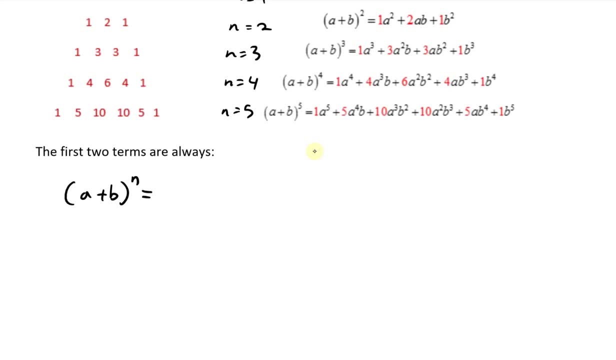 first term is going to be one, so it's going to be. i'll just write this down as one times a, uh, yeah, or just ignore the one. so it's always going to be a to the n. then, plus, the second term is always going to be: there's going to be an n there. 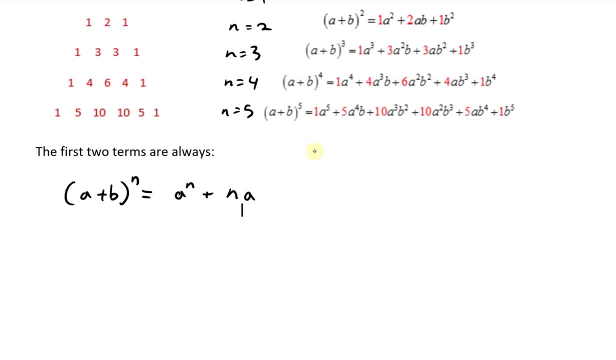 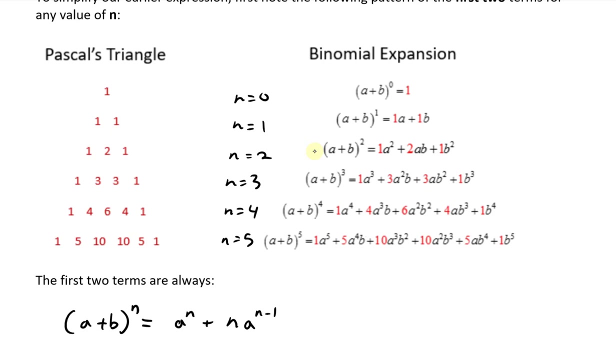 and then it's going to be a: a to the n minus one- i mean a to the uh, a to the n minus one there- and then the b is always power of one. every single one of this is power of one. power of one, power of one, and so on. so the b is always power of one. so this is going to be plus b, the power of one. 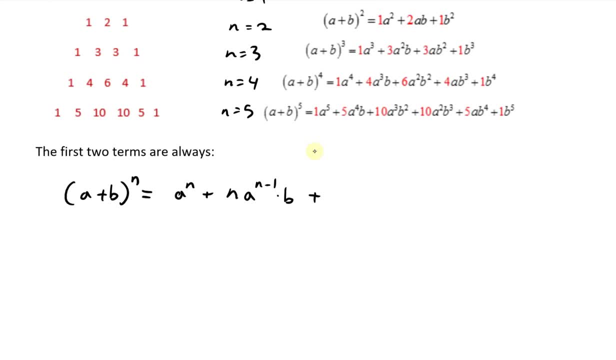 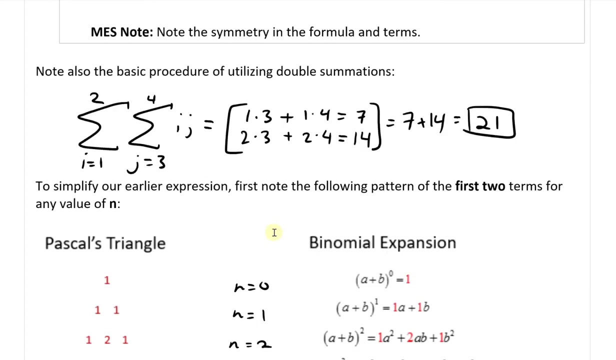 so this is the then, then afterwards we can add it. so this one is when k equals to zero. so notice what happens: at k equals to zero, we're going to have, uh, yeah, we're going to have a n minus uh, this number of the formula. we're going to have a n minus k, which is zero, so a n minus zero. 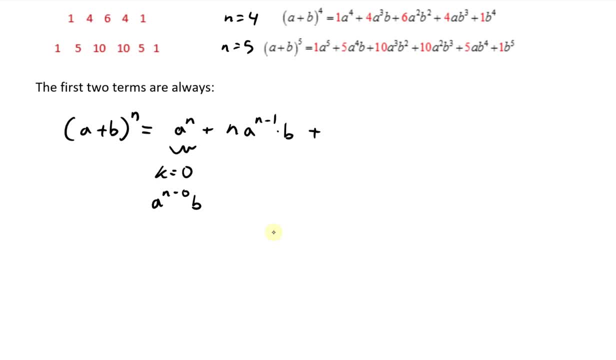 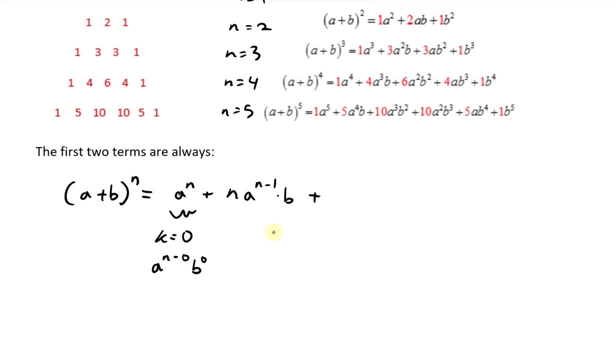 and then we're going to have a b, a b to the power of zero. so then, uh, yeah, that just vanishes. so this just equals to uh, yeah, just a n, uh. so now this is going to be a n minus k, which is zero. this, this part right here, this whole thing, is when k equals to to one. so when you have k equals. 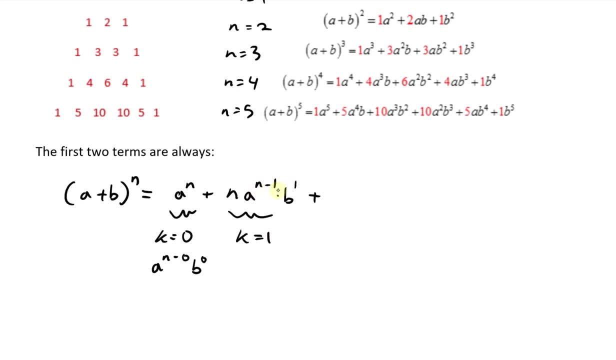 to one. so now there's this n minus one, this one here, b to the power of one, uh, etc. and then, lastly, we'll have the remainder, the. so all this remainder afterwards is going to be just a summation: up to uh, up to n. so, yeah, so this always goes to uh. n equals five all the way to b to the power of n. 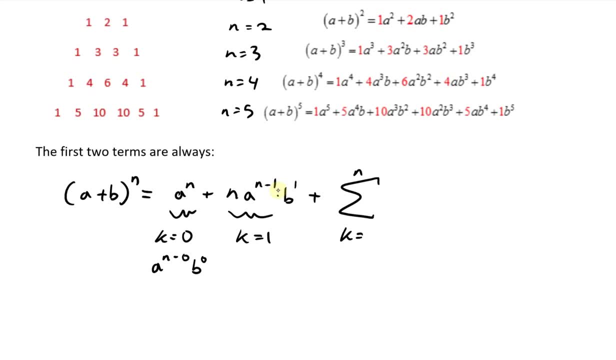 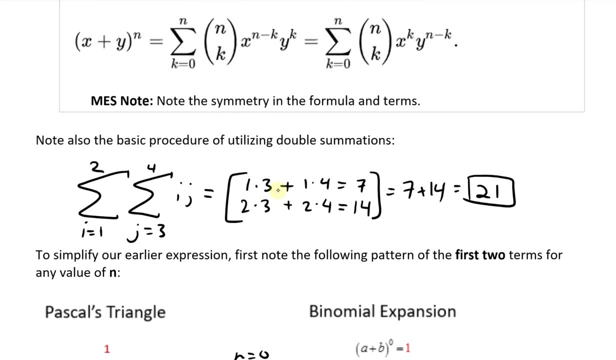 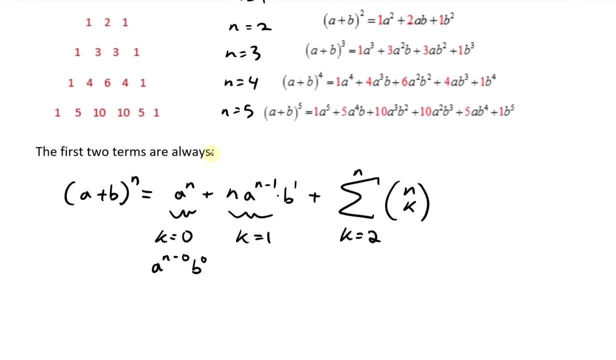 so now it's going to be the remainder. and now now the starting point here is: k equals two. so if this k equals two, now this, this formula and series notation- i mean in uh, in summation notation- is this: uh and choose k, x, n minus k and then y, k, so this is going to be um x, or this case. 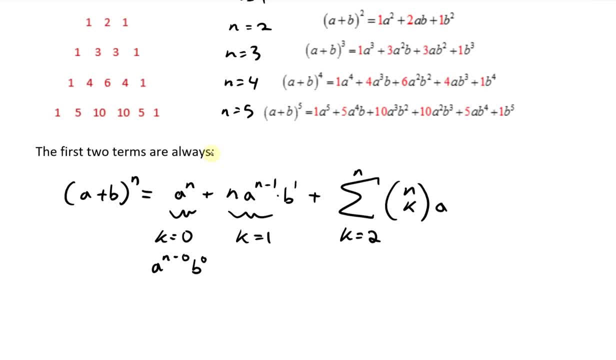 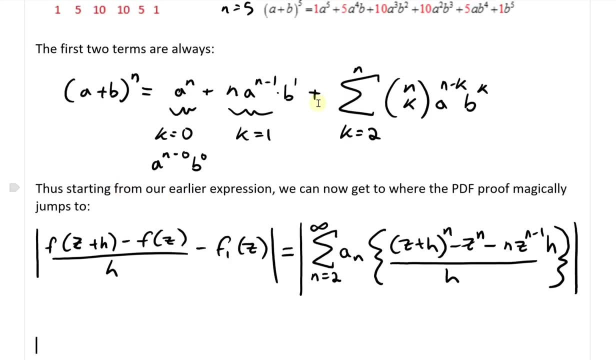 a. just to make the same as that. uh, this is going to be uh n minus k, and then b? k. all right, so now, thus we have this all uh wrapped around our brains. so thus, starting from our earlier expression, we can now get to where the p is, and then we can get to where the b is, and then we can get to where the. 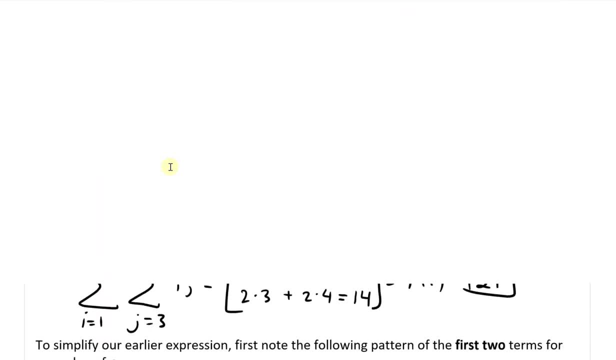 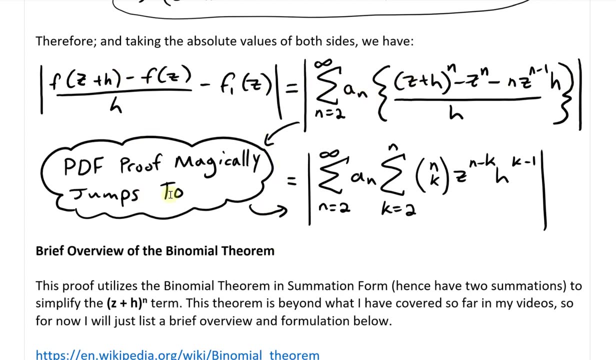 pdf- uh proof- magically jumps to. so yes, go back up here, let's keep scrolling up. so here, uh. so we went from all the way to this big giant thing. so i just copy and paste it at the bottom and it jumps to all the way here where we start from. k equals two and this is just uh, and then also here. 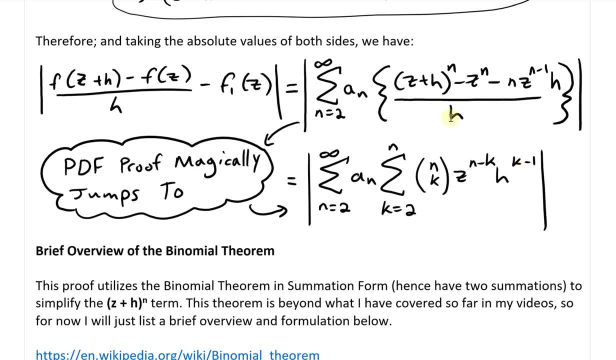 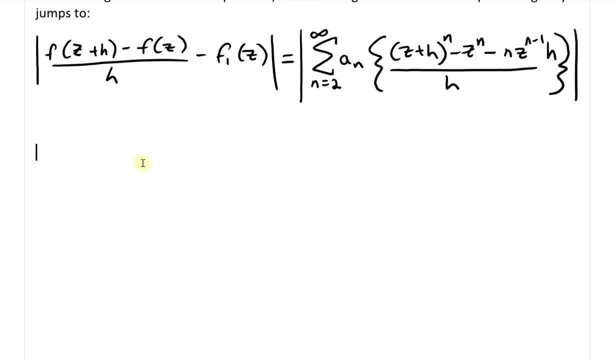 we have a h minus h to the power of k minus one, and you can see that because we're going to be dividing by h there. so let's see how it gets magically there and let's just expand from that starting point. all right, so now this entire thing on the right side. this is going to equal to: 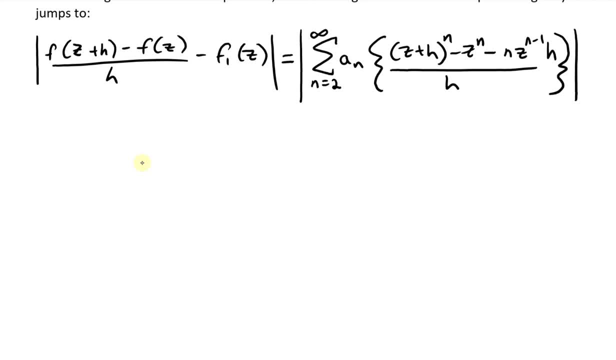 well, let's just write this out as the absolute value. it's actually, it's going to be pretty big, so i'll write this as equals to the- uh, absolute value of this series. let's, let's write it like this: um, or even, i'm gonna need more space, or may need more space. uh, summation, yeah. summation from. 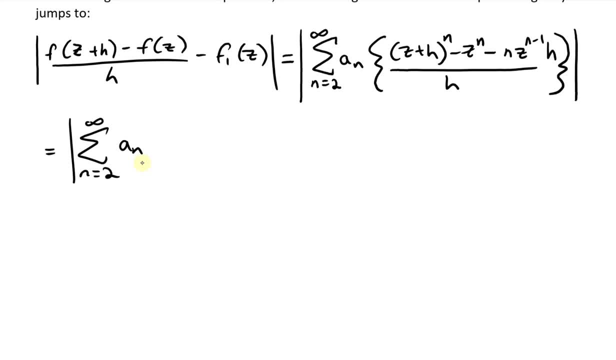 n equals to two of a n, and now what we'll do is, yeah, so inside this bracket, we're gonna have, so we're gonna expand this, uh, this, this power right there, so this z plus h, the power of n, we're going to write this in, uh, you know, and this is all going to be. 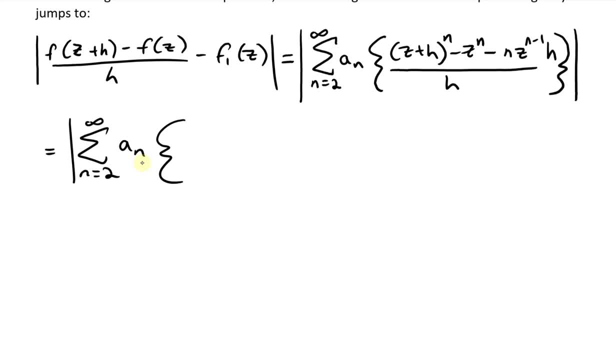 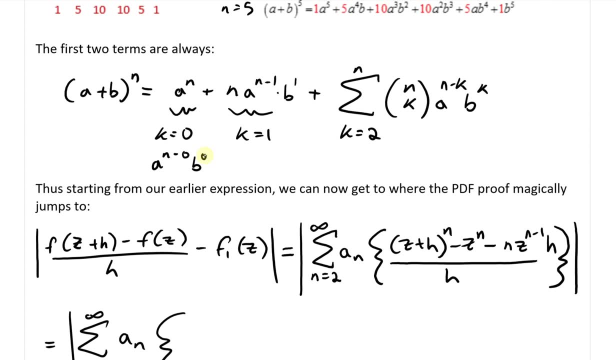 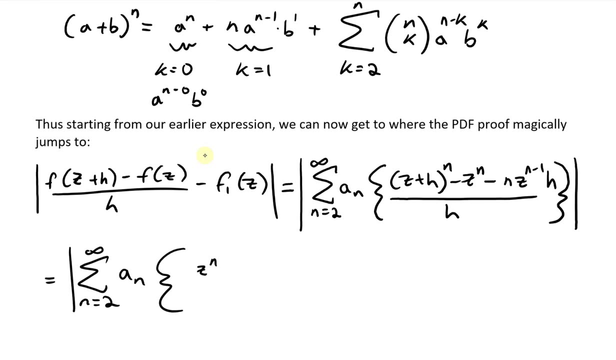 divided by h. so i'll do that uh afterwards. so this is going to- we're going to expand this out. so z plus h, the power of n, this is going to equal to- we're going to write it in terms of this. so instead of a and b, we'll write z and h. so this equals to uh, z, n plus. so the first two terms: uh. 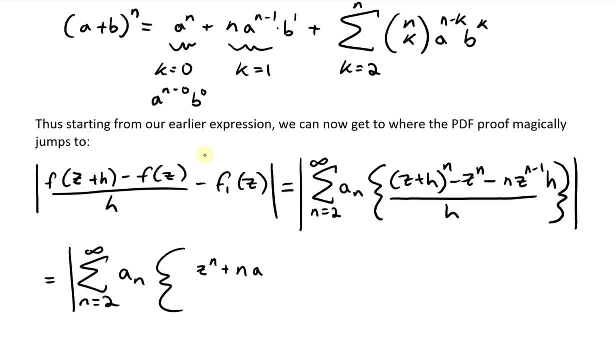 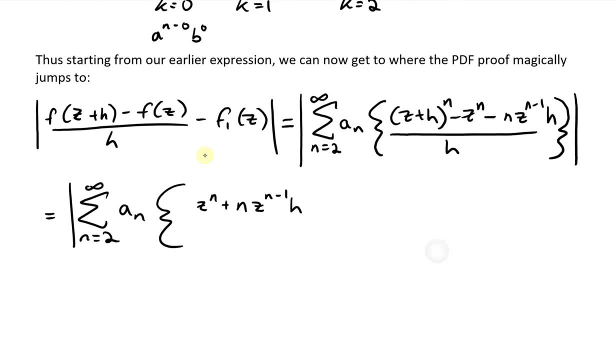 n a, uh, yeah, so n a z, this is the power of n minus one, and then times b, which is h, like that, and now we're going to subtract this. i'm, now we're going to add this entire thing right here. so we're going to add: 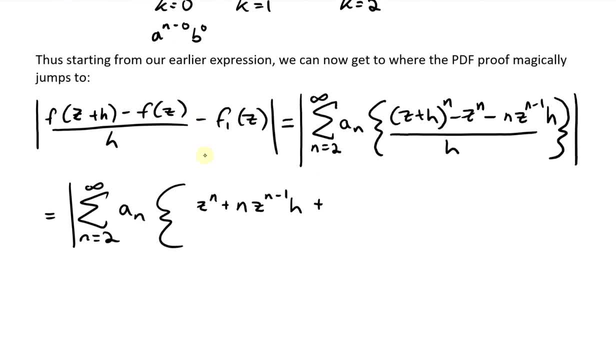 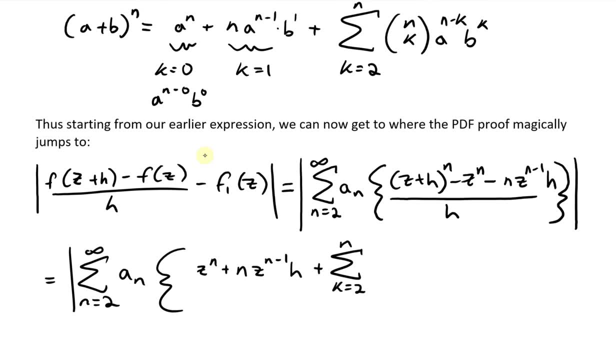 that. so we add the first two terms and then plus yeah. so hopefully this is all coming together. so plus k equals a two of the summation up to n of n choose k. yeah, so n choose k. and now we have uh z to power of n minus k, and then b is going to be our h, so h k like that, yeah. so those are the first. 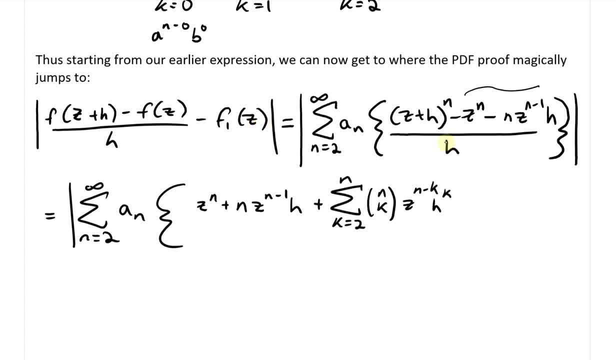 two terms. but then we also have these, these part right here. so this part here we have, where my calculus book just magically, uh, it just ignores. so we have these and let's just, uh, i'll just put it like that, so we need this part and that's going to be our minus. so this is outside of this. this 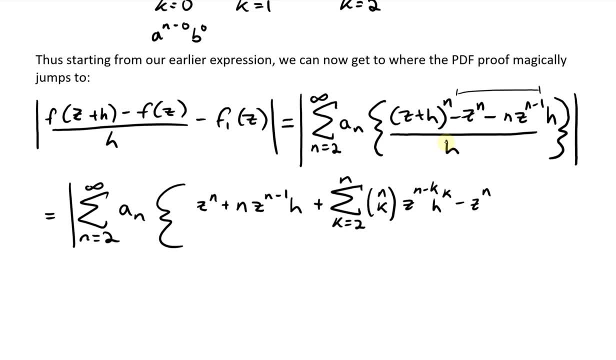 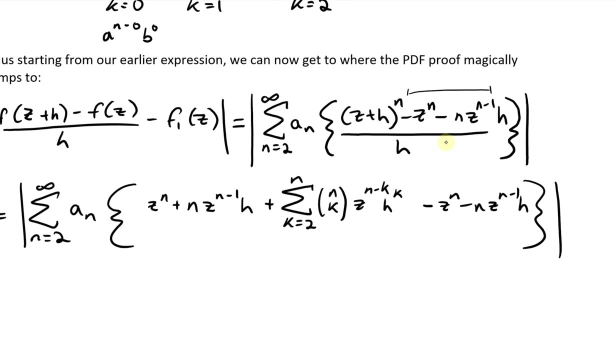 summation. so just inside the other one, this is that n, and then we're going to add this to the. let's just move, make it a separate. so minus z n, uh, minus n z n, minus one h, and this is all going to be inside this giant bracket, and then all all absolute value, yes, and lastly, we got to divide. 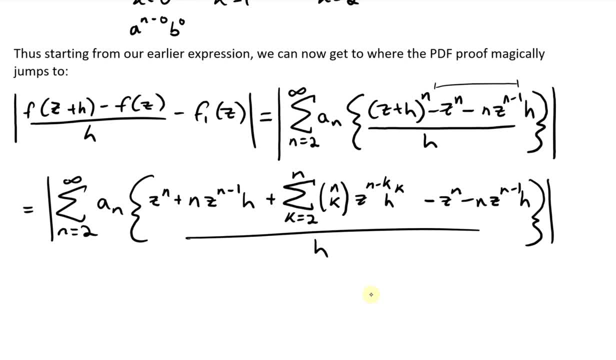 this all by h. so we have that h there. so let's see, yeah, this entire thing, same common denominator of h, all divided by h. and now look what happens: we have the z and the first term cancels with this. i'll just make it a bit. 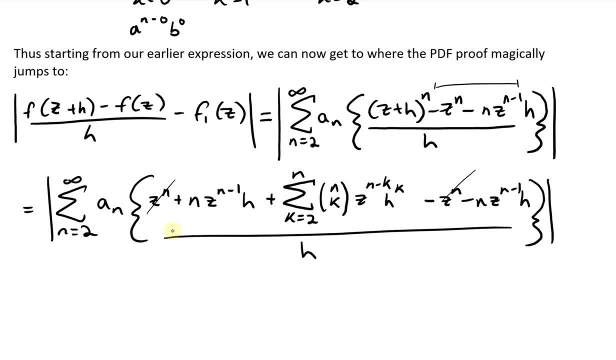 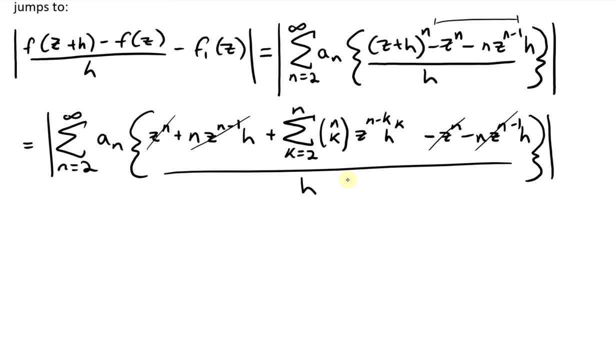 lighter. so this, this cancels with this. and then the next one right here: this is a n, not an r. and then the next one here: n z, n to the uh, i mean z to the power of n minus one times h. this cancels with this. so all these cancel. so all we're left with now is just this series, right there, and 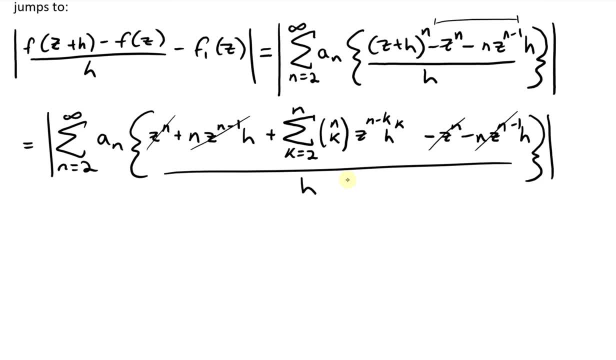 we have, uh, yeah, i mean the summation right there- but then this h, the power of k, but then we have a h, we have the r, right there, and then we have b. we have the h, the power of k, and then the sum of n and then the s, the power of n, which is a normal constant plus a, is a normal constant plus a, and 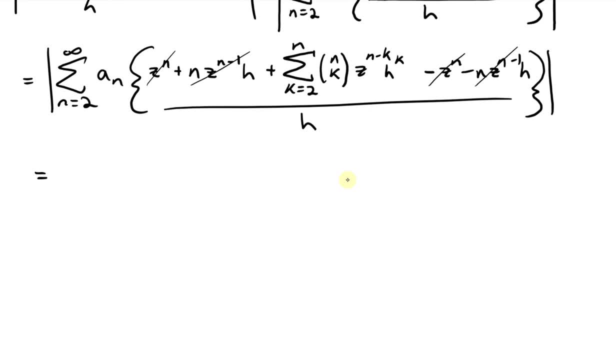 then we have the, so we can just subtract it from that. you can divide it by h there, on every single term, so we just subtract that by one. so this equals to: yeah, so this equals to. let's put it here now: this equals to the summation, that's the value of the summation. 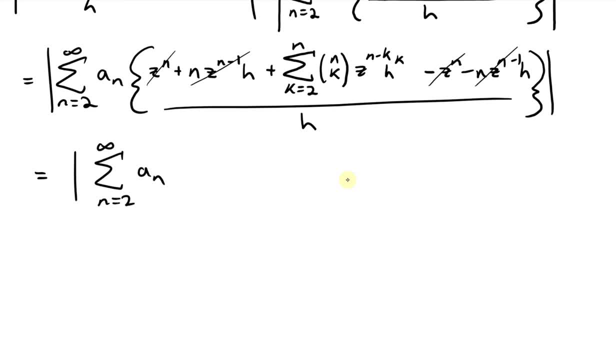 right here: infinity: n equals two of a n, and now this: uh, we can get rid of this giant bracket, and So this is going to be summation up to n, starting from k equals to two, And it's going to be n, choose k, some combinatorics there, And then this is gonna be z n minus k, h k minus one, And this: 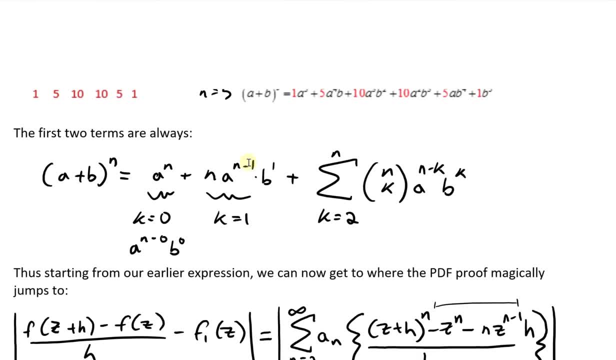 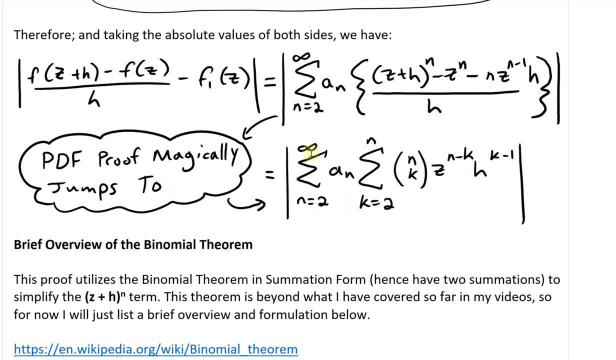 is exactly what we magically got. Let's just double check that one there, scroll up. So here so PDF proof magically jumps to this part right here. summation n equals to two up to infinity of a n, and then the summation from k equals two to n of n. choose k, z n minus k and then h k minus. 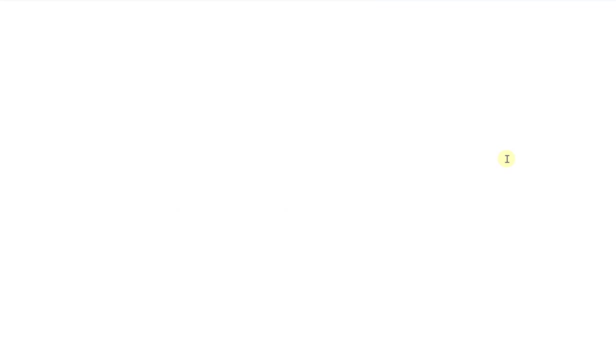 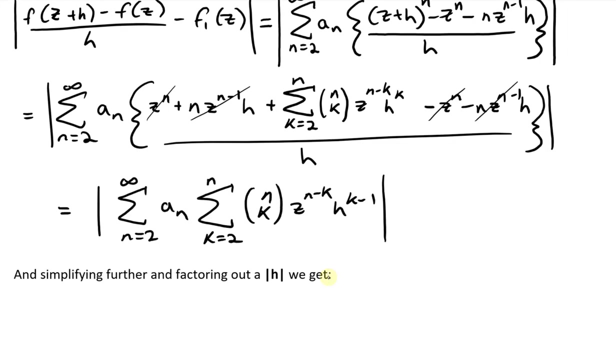 one And that's exactly what we have here. Yeah, this is exactly what we have right here And, yeah, it's fascinating stuff. So, yes, this is a pretty amazing. So let's just box this out, actually. So I'll just put a bubble, put a giant bubble around this And now put a hashtag: amazing. So it's pretty. 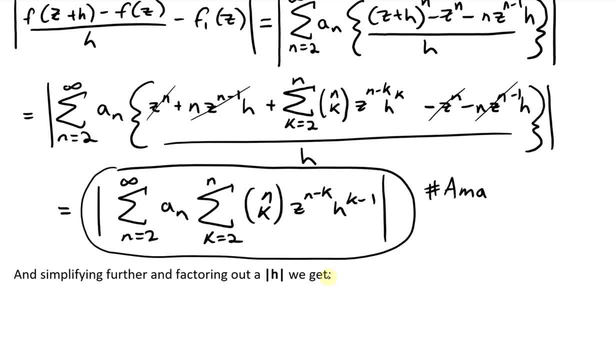 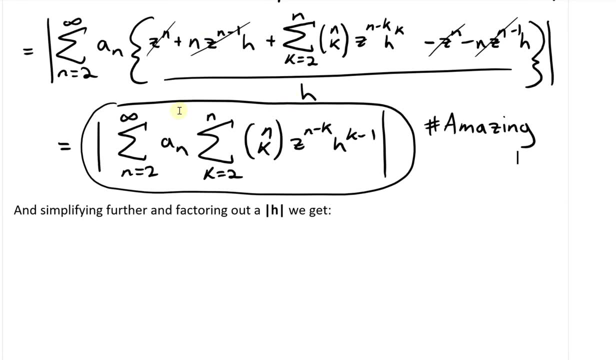 amazing, going forward from that giant, giant series- I'm giant summation to this call was slightly compact or somewhat compact, that double summation- And I'll see I going from this right here, merging all the terms, canceling them and getting to this right here, which is pretty amazing. So now simplifying. 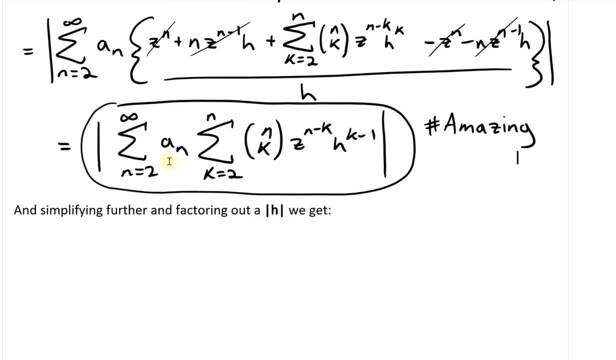 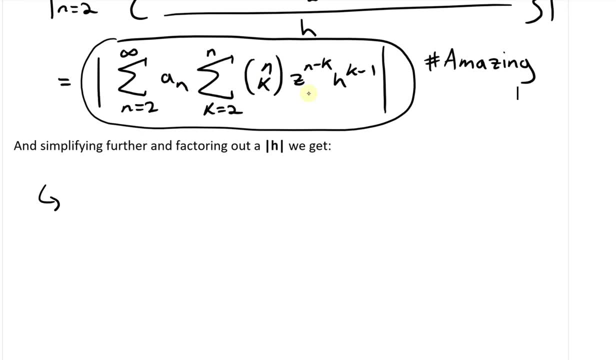 further and factoring out a absolute value of h and also putting an absolute value on every individual term, so that what we'll end up doing is: well, we can ensure that this part right here is going to be less than or equal to n. 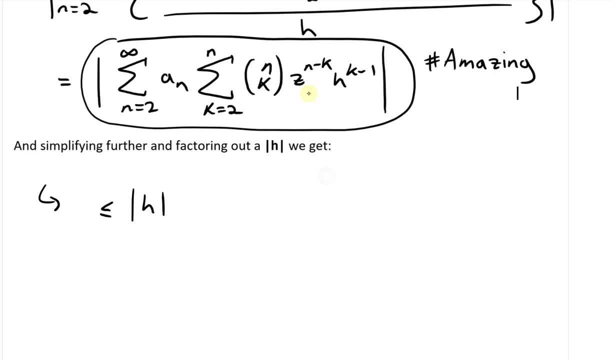 or equal to, and just factor out an h, because it's not dependent on n or k. So we could factor out an h and also take the absolute value of each individual one, So that this means that when you, when you have positive, positive numbers only inside, then this results always gonna be greater. 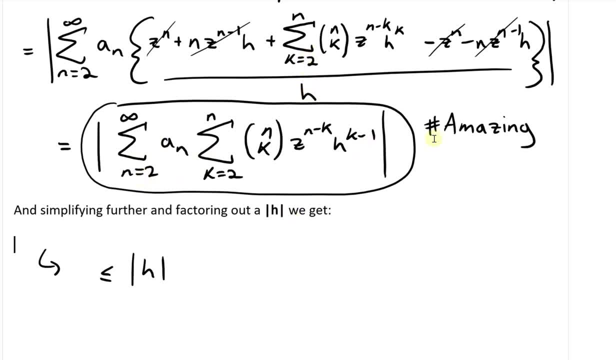 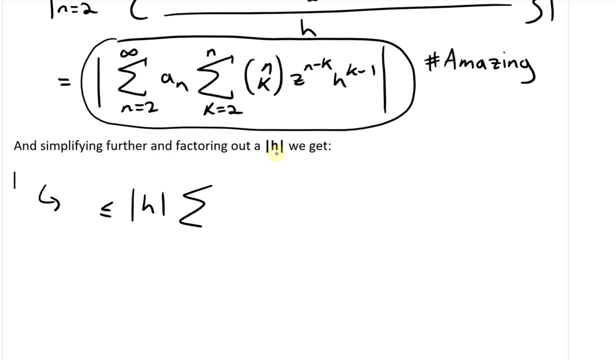 than or equal to, yet to a few, then just taking absolute value of the final result. So we're gonna do have the each individual term. So this can be less than or equal to, and this is going to be from infinity nossos checkbox. So the real thing, we just take an absolute value of an and on to a few276. 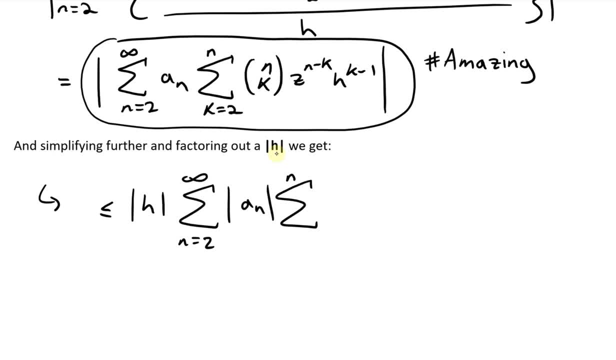 conviction, so on, is gonna give us photos that have any of the essence: n equals the two, or absolute value of a, n, And now what we have is times the by the. this is going to be now the, which put this like this: this is going to be a double summation. So up to n of K equals two. and now what we have as n choose K. these are all positive, So we don't need an absolute value. but the Z could be negative or not. so n? n power. I'm this absolute y of z to the power of n minus k. times it by absolute value of a two times. 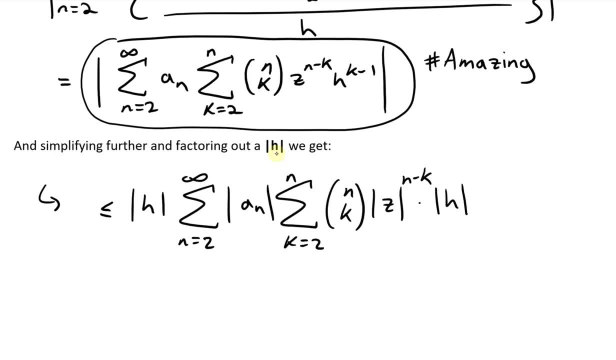 Nik technique, k plus k times n is equal to p2 squared by the sum of a two. so we're gonna get to the Kit comer신 superst Bitte es dieradik. times it by absolute value of h. now what we'll have is: this is going to be k minus two, because 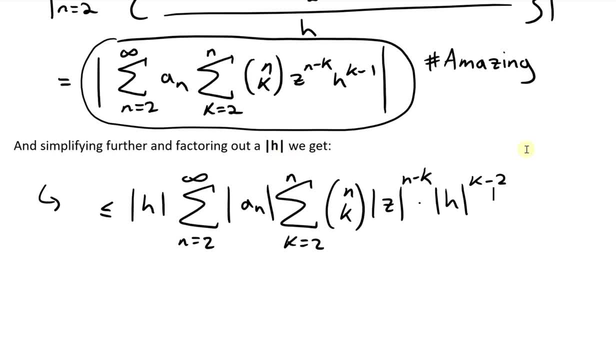 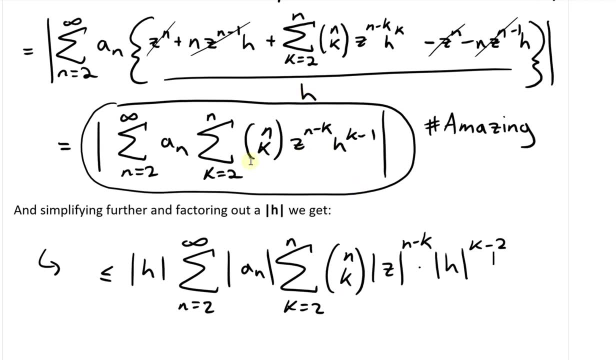 we factored one out. so this value- because every single one of these we're forcing to be positive inside can- is always going to be greater than or equal to um, uh than if we just took the absolute value at the end, because some of these could be negative and they can cancel out and so on. 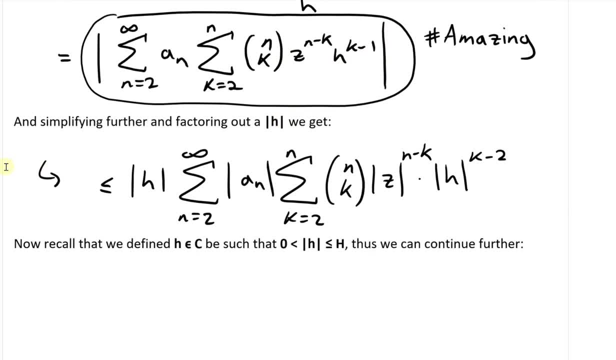 and hence absolute value is signed there. all right. so now recall that we defined h as an element of all numbers, uh, real or complex, all numbers. c, uh, be such that, uh, so we define that this is, uh, yeah, so, defined a element of all numbers. be such that the absolute value of h is greater than. 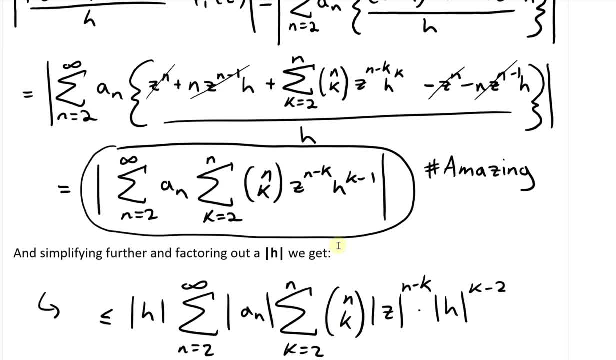 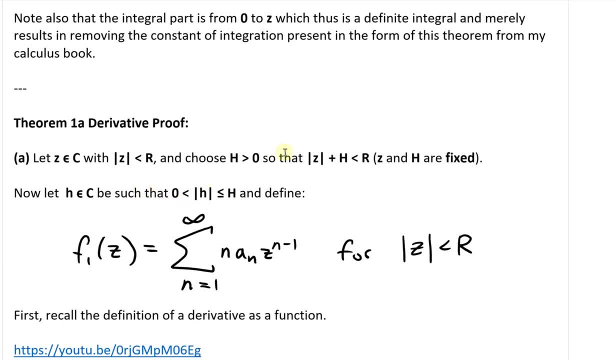 zero and is less than or equal to this capital h. thus, we can continue further and let's just scroll all the way up to where we define that. let's see if we find it. yeah, so we defined it here. where, uh, absolute value of h is less than or equal to capital h and where, again, h, uh, h plus uh. 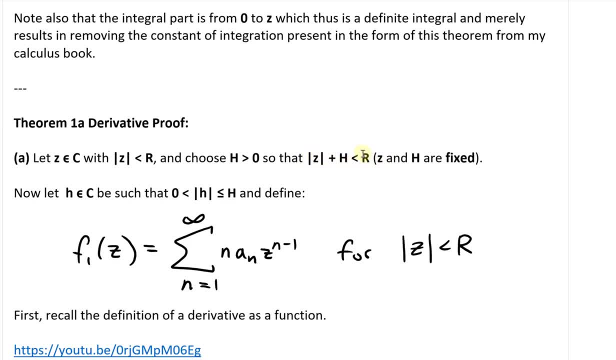 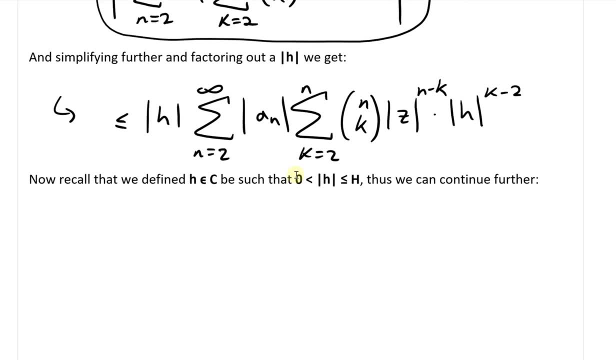 capital, h plus absolute value of z is going to be less than the uh radius of convergence. so, and where h is fixed, yeah, so thus we can continue further by even having a further inequality. so this term right here above is going to be less than, yes, this one's going to be less than or equal. 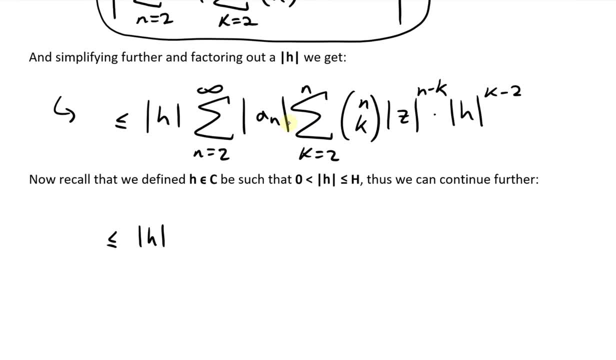 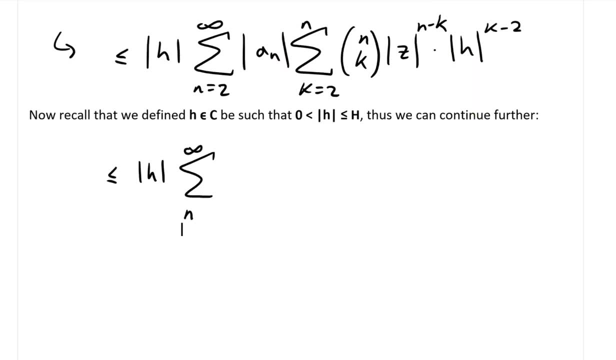 to uh, this is going to be absolute value of h. again, this is, this is right. everything, everything's going to be the same, except we'll replace this with uh, capital h. we're going to replace, yeah, this one with capital h. so we get is equal to two. uh, absolute value of a, n summation up to n of k equals to two, and then this is going. 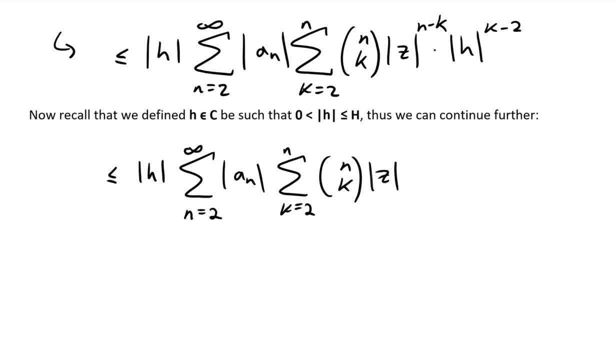 to be n. choose k, absolute value of z, n to the power of k, and now we have absolute value of capital h which is greater than or equal to absolute value of h, and we don't even need the absolute value sign because it's we know it's greater than the absolute value of that, so it's. 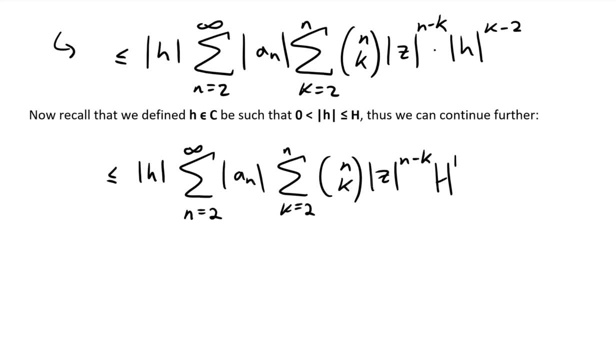 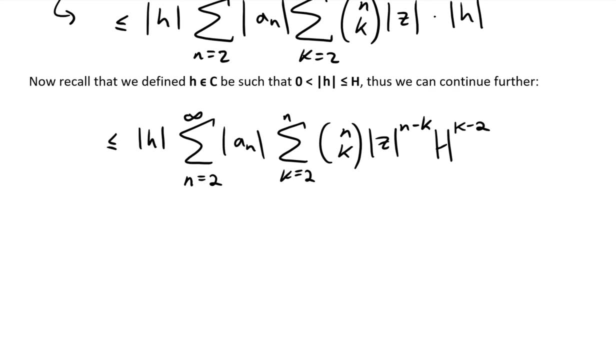 always positive. so we just put capital h, uh, power of k, minus two, and reason is: uh, we'll become evident soon- uh, what we'll do is this is going to equal two. uh, absolute value of h is factor out this, uh, capital h. there, so two of them so that we get. 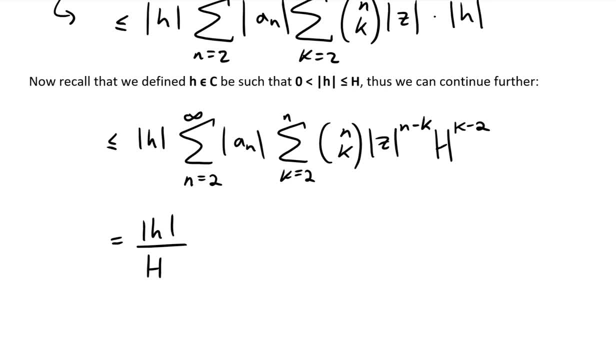 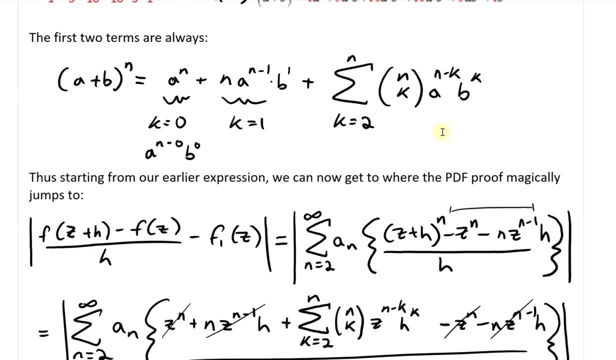 rid of uh this minus two there, yeah, and in fact the reason is so that we'll have uh h power of k, so that it will look exactly like our uh combination formula there, or this, this formula right here, and so we'll look exactly like this. so we want this uh y to power of k, so we're 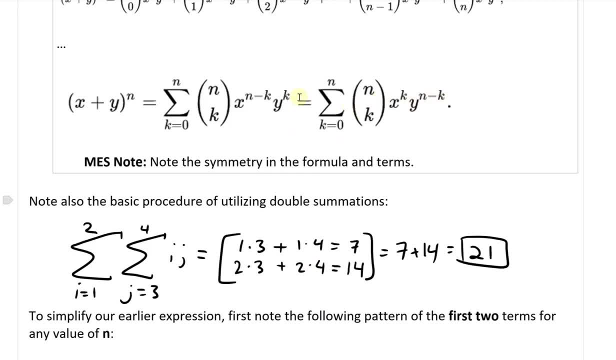 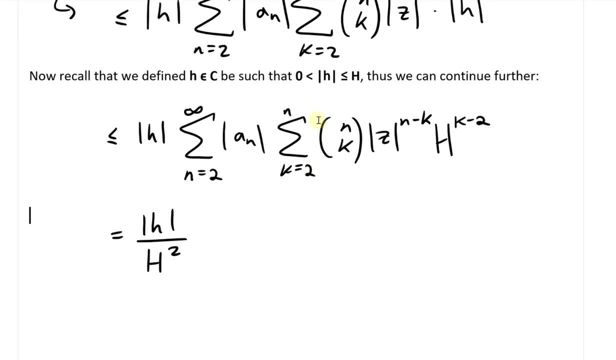 going to, we're going to, we're going to use this uh, and now this uh. this is going to equal uh. So right now we have k minus 2.. So we got rid of it. So we get rid of this minus 2 so that we can go work backwards. 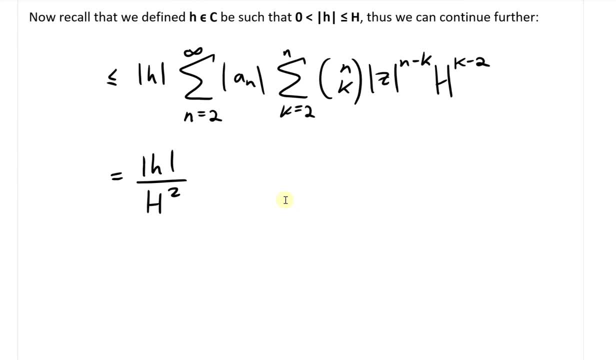 before the binomial expansion of that: a plus b, power of n and so on. But in this case it will be z plus h, So let's just write this out. So this is going to be so. we factored that out. 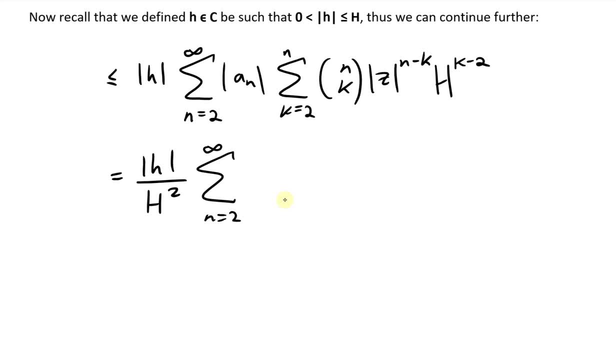 This is going to be infinity, from n equals 2 up to infinity of a, n, And this is going to be now the double summation. So n, k equals 2, n choose k, And now this is going to be absolute value of z, power of n minus k. 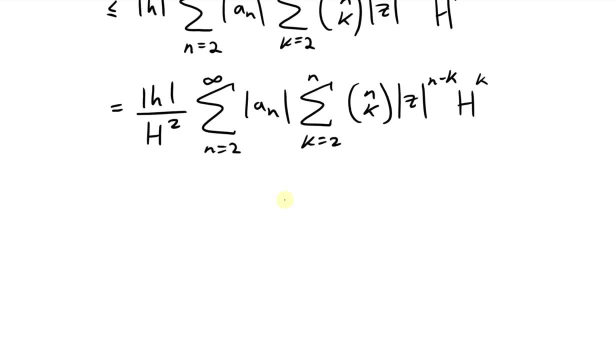 And then this is going to be h k. Yeah, so now what we have? we have an n equals 2 there And we also have a k equals 2.. But remember that the f1 function that we defined and also the derivative that we're trying to derive- 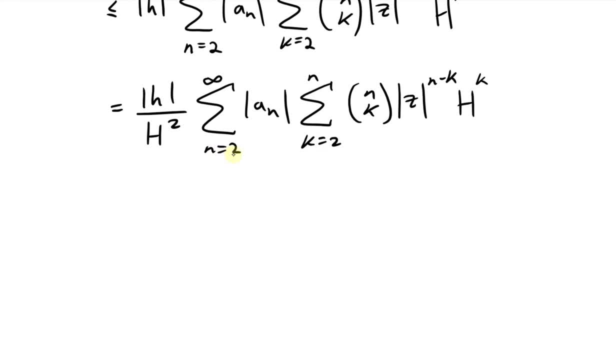 starts from: n equals to 1, just to make it all the same, And this one, we want this to equal to k, equals to 0.. So what that means is, since all of these terms are positive, if we have extra terms, that means it's going to be greater than. 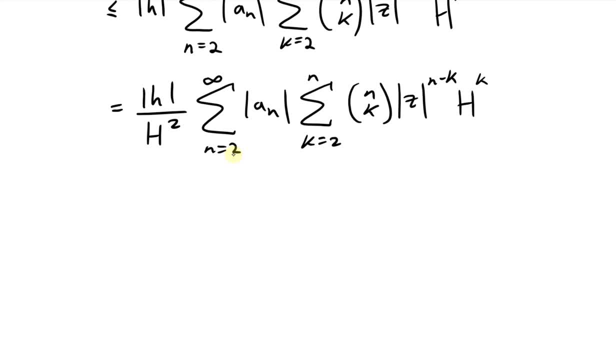 It's going to be greater than this term right there. So, in other words, this right here is going to be less than or equal to the same exact formulation, but with more terms. So this is going to be less than or equal to absolute value of h over h squared. 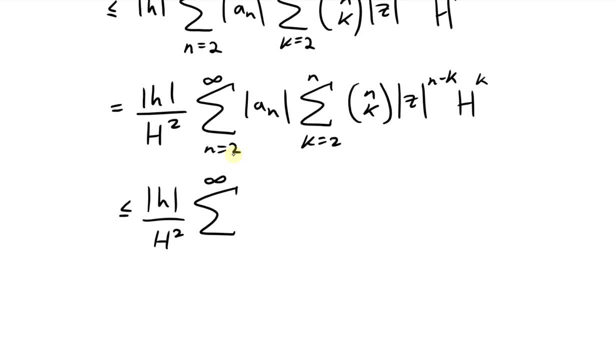 And this is going to be summation: n equals to n equals to 0.. Yeah, we're going to start from n equals to 1 here, So we'll have an extra term up to infinity, of absolute value of a- n. So this is going to be less than this, because it has more terms. 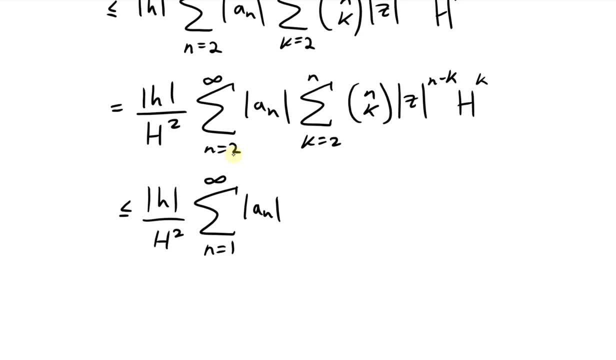 And they're all positive. So it has to be greater than or equal to this over there. So now we have the starting point here. k equals to 0 up to n, And this is going to be n, k, n, choose, k. 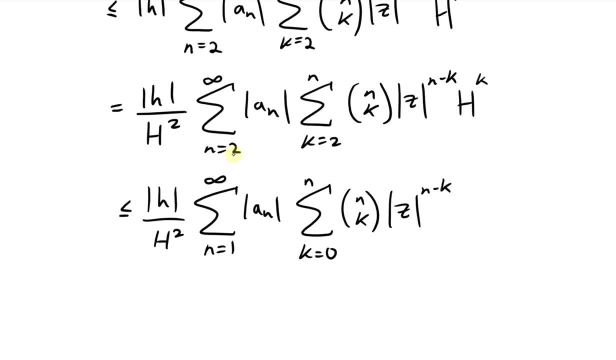 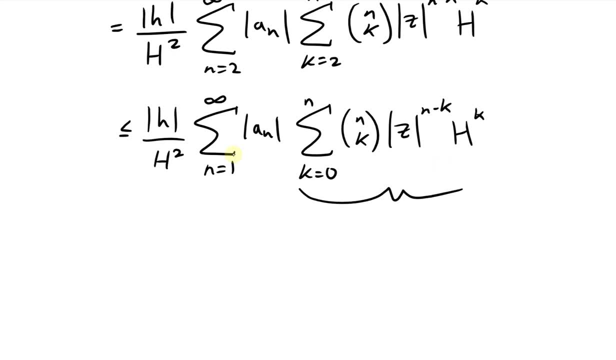 absolute value of z. now n minus k, This is going to be h k. Yeah, so in other words, this entire thing. this is just our binomial expansion. So this is binomial expansion of absolute value of z plus this capital H there. 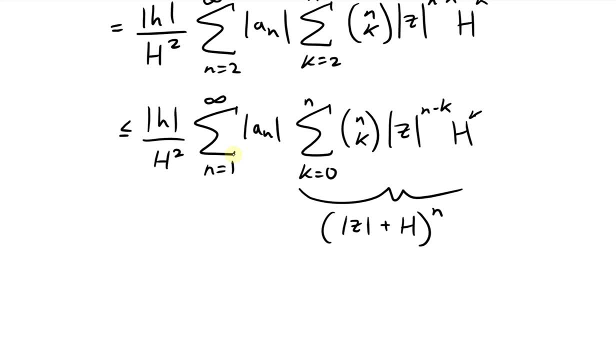 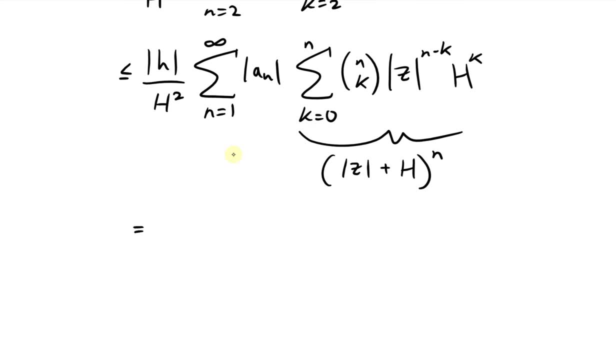 And then this is the power of n. It's exactly the formula, So we can get rid of that all. So now what we have is: yeah, get rid of that entire series. Now what we have is equals to absolute value of h. 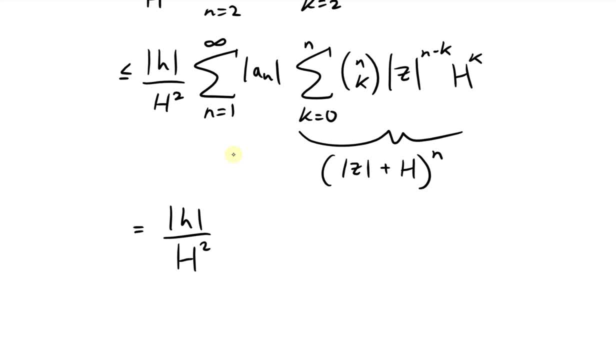 So this whole thing equals to this divided by capital. H squared Summation, now Summation up to infinity, From n equals to 1 of a n, like that. So absolute value of a n times it by. and this is going to be well, I'll just put it in bracket. 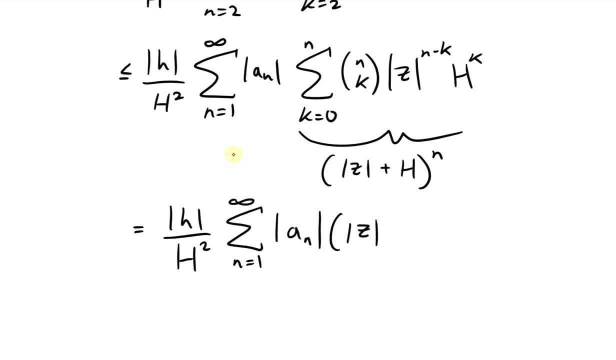 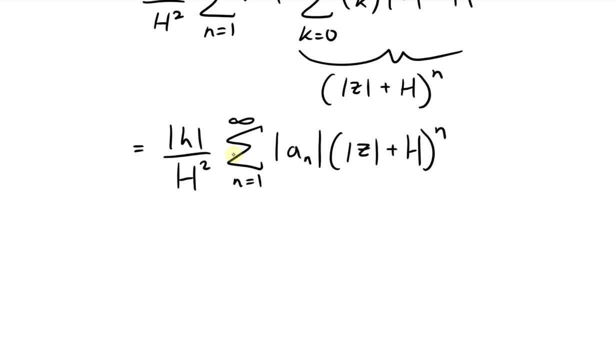 like that. absolute value of z plus capital H, power of n. And now recall that this part right here, a capital Z, I mean absolute value of z plus capital H. This is entirely within the radius of convergence. So in other words, 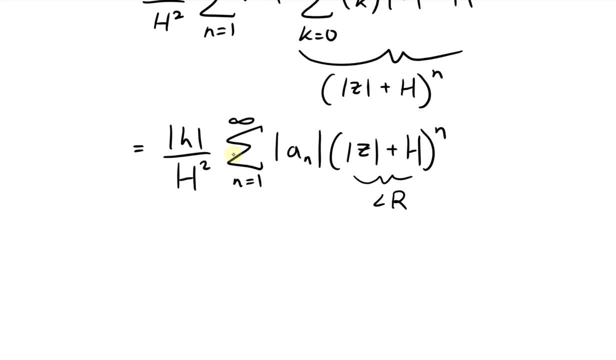 this series. this is just absolute value of a. n times it by this absolute value of z plus H, power of n. This is a convergent series. So that's what we have is so here, yeah, so this part right here is going to be well less than or equal to 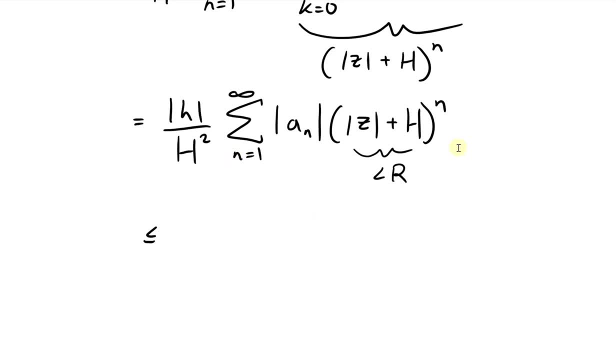 the limit of this as this converges, Because, remember, this series is going to be convergent, because absolute value of z plus H is less than the radius of convergence, So thus we can write this as a number. So this is going to be always going to be less than or equal to. 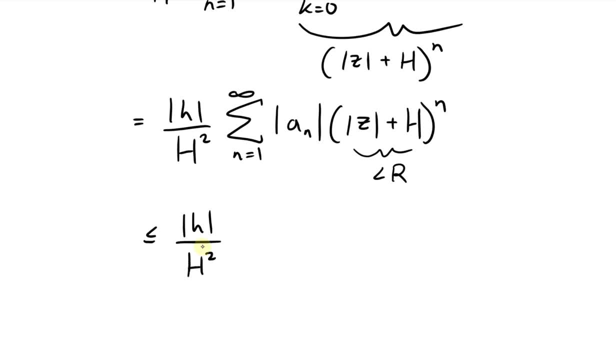 absolute value of a n times H, power of n, H divided by capital, H squared. And we'll just pick a number here- times m, like this: where so this is going to be less than or equal to it? where m is going to be equal to the summation up to infinity. 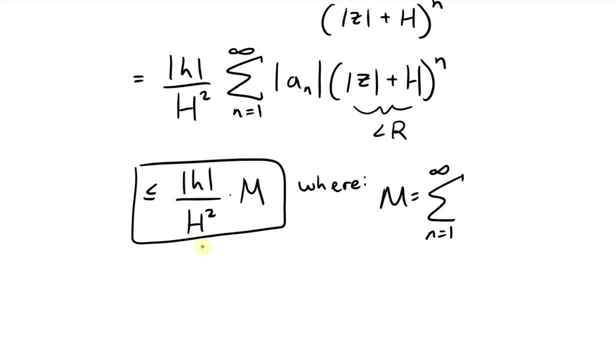 of n equals one. In other words, just the yeah, just the limit there or where it converges to And right here is going to be of yeah, this is going to be absolute value of a, n, and then this is going to be absolute value of z. 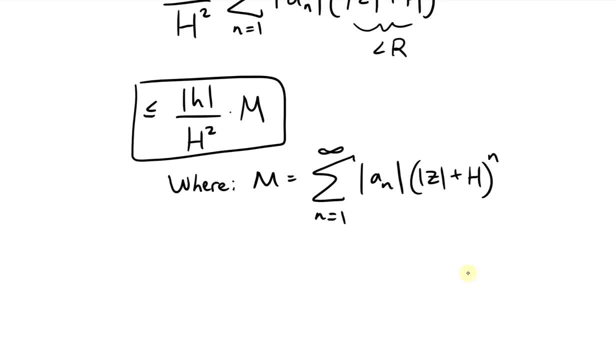 plus capital H, power of n. Yeah, and here I just moved it over here to make some room. And now, where this m equals to the summation up to infinity, where this is going to be less than infinity, In other words, this converges: 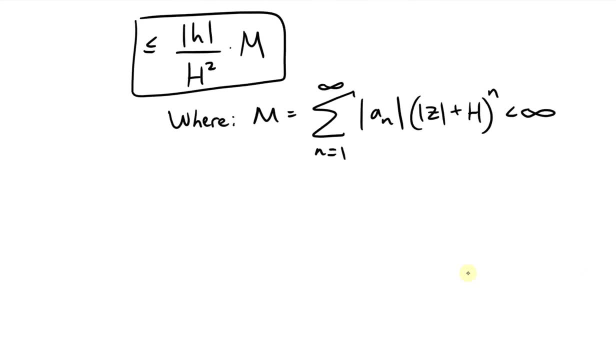 Yeah, so this would be less than infinity. And this is all, since we chose or we defined capital H, since absolute value of z plus capital H is less than the radius of convergence R, So it's convergent. So in other words, we're going to be less than infinity. 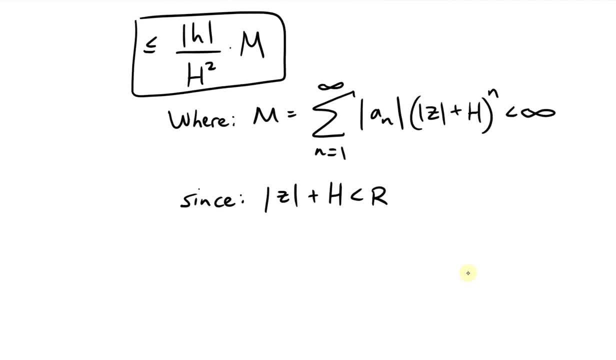 We're going to have to have that limit, I mean the starting point going to be less than or equal to this right here. Well, yeah, these numbers are over there and let's just put it all together. Yeah, so putting it all together is therefore: 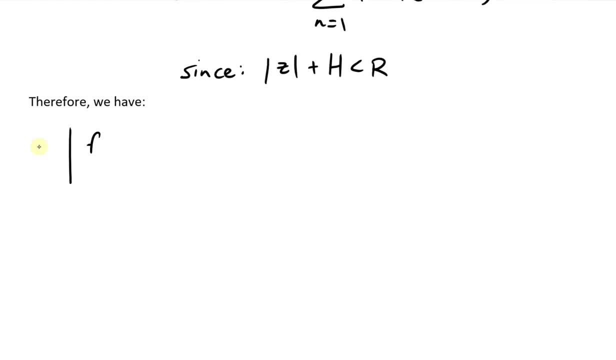 we have a number of. the starting point was just the absolute value of z plus H minus f of z, or the difference, and then divide this by H and subtract it by f1 of z. right there, absolute value. Yeah, so that's putting it all together. 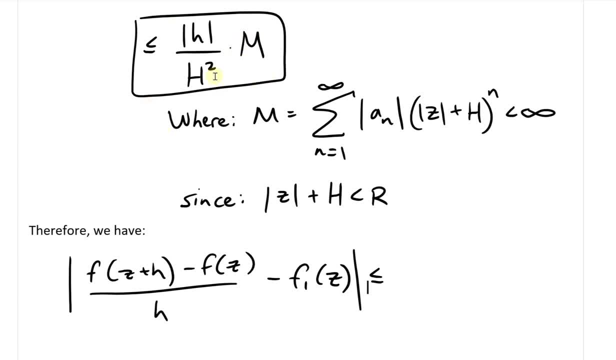 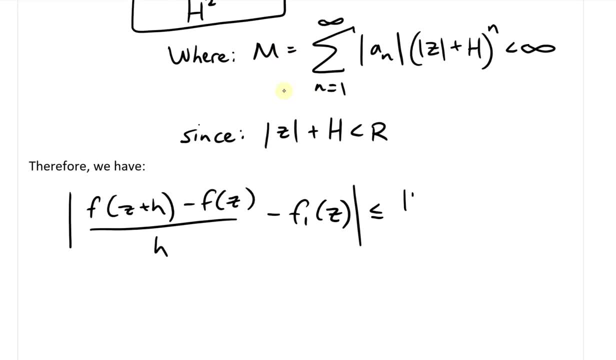 This is going to be less than or equal to this, where we completely got rid of all of the series notation, or I mean the summation notation. So this is going to be equal to absolute value of H over H squared, and this is going to be M times by M. 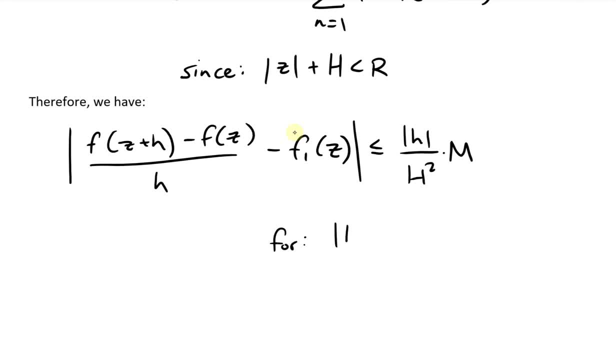 And yeah, this is all, for absolute value of H is less than right here is less than capital H, So where we defined that as well earlier. So this is what we have. So this is actually pretty epic, epic notation there. So we put this all together, put a circle like that. 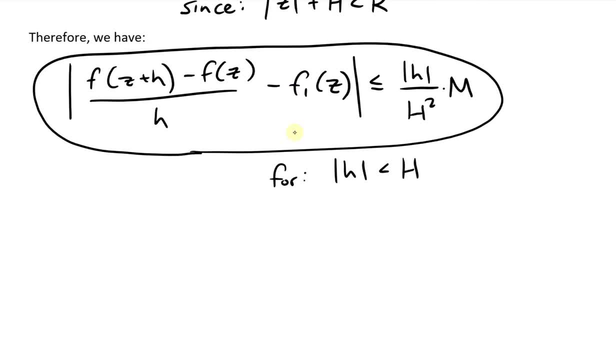 because it's we have absolute value sign. So yeah, this is some pretty epic stuff there. Actually, I got rid of that circling It's because it just seems a bit more just a bit convoluted or just a bit messy. 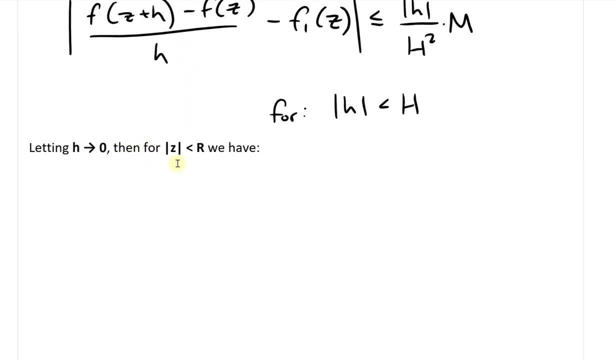 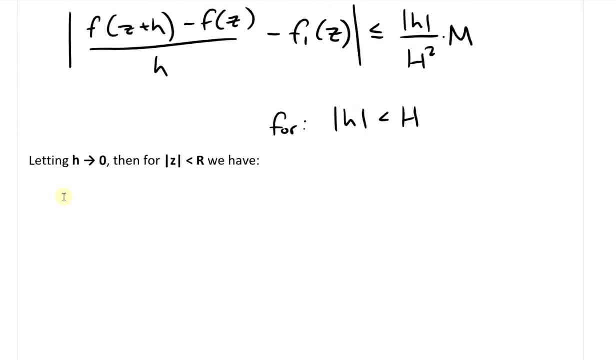 we have kind of the same thing going on in the left side. This is just H, so that that goes to zero. So in other words, yeah, in other words, you know, when we take the limit on both sides and this one. 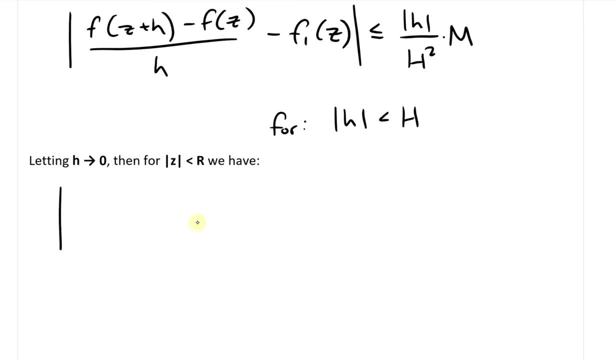 the only thing that's dependent on H is that inside function, so what we can do is write this as absolute value of the limit of yeah limit as H approaches zero, like this: of f of z plus H minus f of z. I'll divide this by H. 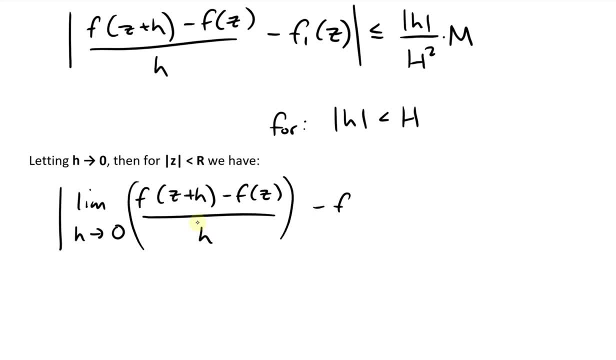 And now separately, we're going to have a minus- just put this in bracket like that- minus f1 of Zed right here. so now this is gonna be absolute value. it's gonna be less than or equal to the limit, as H approaches 0, of absolute value of H over a capital H squared M. so these are all. 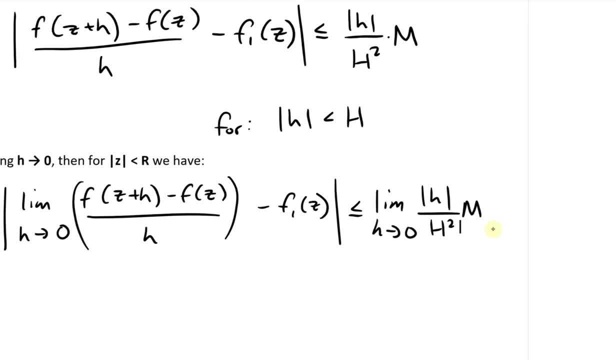 just gonna be numbers there. yes, these are just gonna be numbers where this absolute value of H- now remember this, this- a capital H squared is gonna be- well, it's always gonna be greater than this absolute value of H, so that, in other words, it's not gonna be dividing by 0. so that does this limit is gonna. 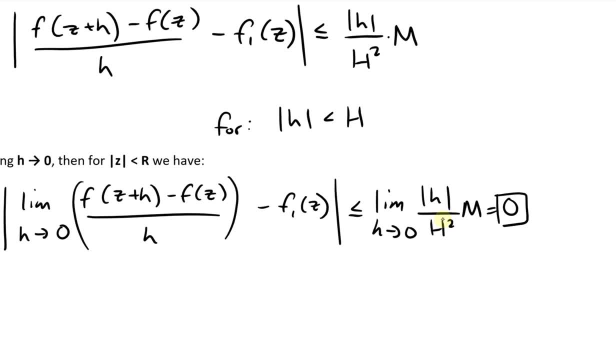 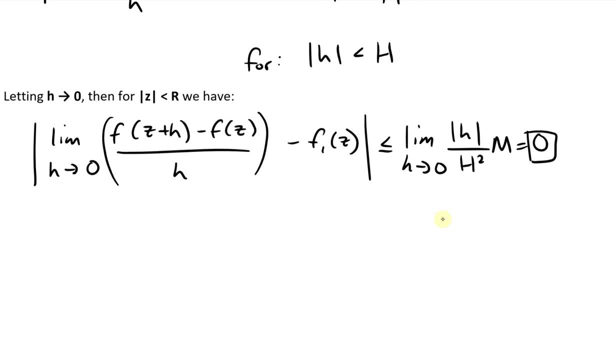 approach 0, so this equals to 0, and the only way this is gonna be equal to 0 is if our only way this is equal to 0 is if these are equal to each other. yeah, so we have this. all zeros as this H up survive. H goes to 0, that just goes to 0. this. 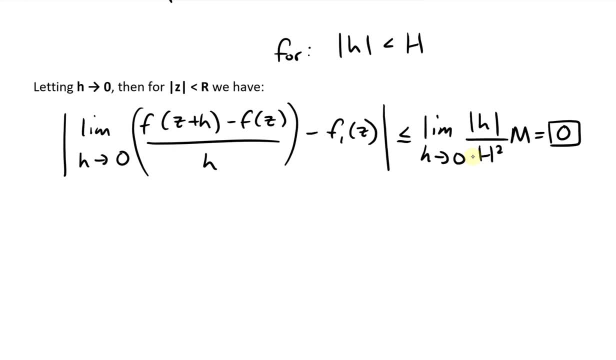 capital H is bigger than it, so then these have to equal each other. so this inside has to approach 0, 0, and so that's what we have. is this: it has to equal to the F ones. that, yes, so that's the limit as H approaches infinity of this entire bracket there. 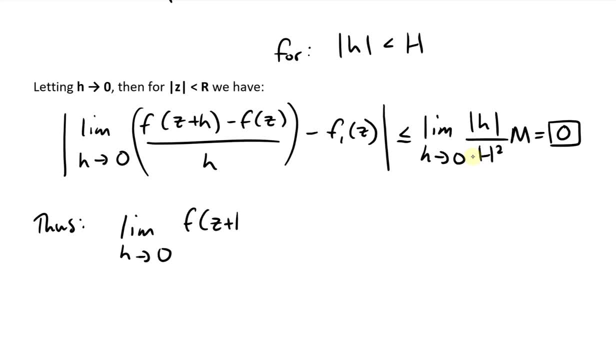 I'll just write this as F- F of Z plus H minus F of Z. divide this by H has to equal to this, so it's only way it's gonna be 0 or approaching 0. so this equals to F 1 Z. in other words, this is: this is just a derivative. 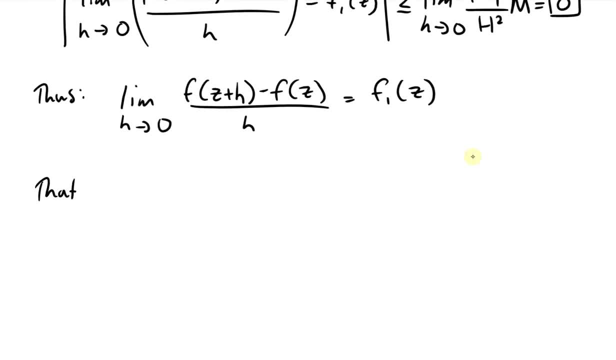 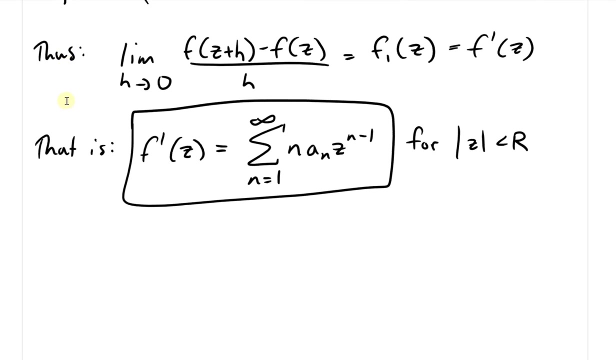 X. so this, that is basically. this is just. this is just a derivative, it's just R. And yes, there is the proof. I'll scroll to it at the end of this video. Okay, this is another epic long video. So this is for absolute value of Zed is less than R And yeah, this. 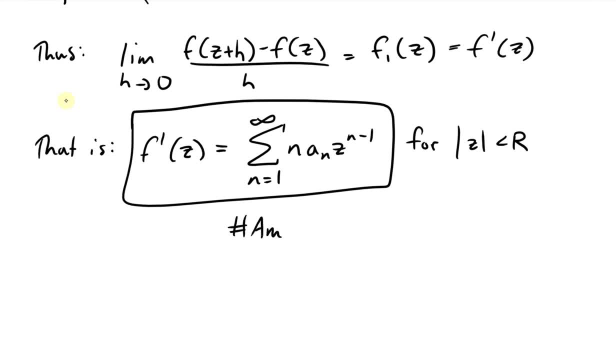 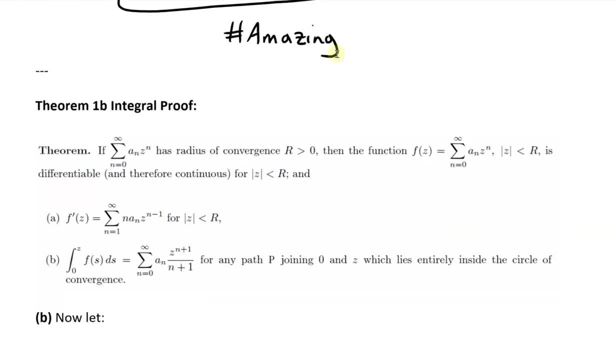 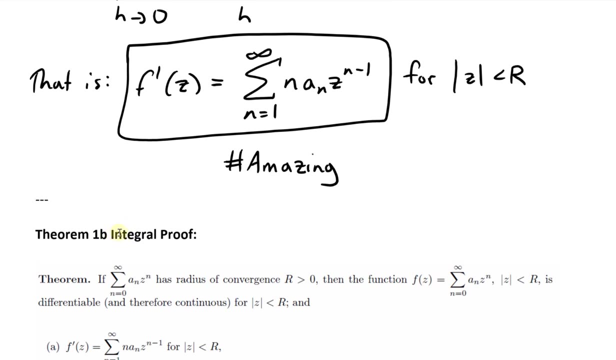 this final result deserves a hashtag: Amazing. There's some pretty epic derivations going on here, And now let's finally finish off this video by going over the last part of this video, And that's theorem one B, which looks at the integral proof or the integral part of theorem one, And let's just quickly refresh it Again. 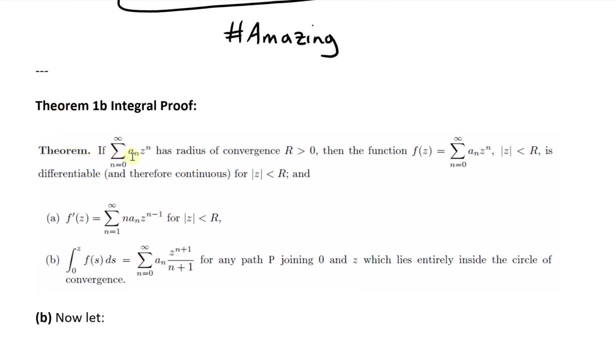 this is a screen grab, again from the PDF proof, And again it uses Zed instead of the x minus a which was in my calculus book. So anyways, so theorem. so if the series a and Zed power of n has radius of convergence are greater than zero, then the function f of Zed equals. 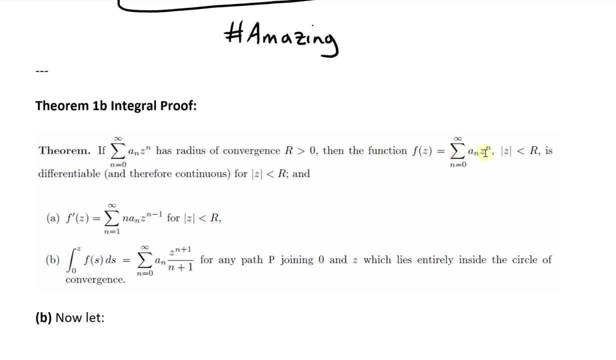 to. so we set that function equals to the series a and Zed. power of n, where absolute value of Zed is less than the radius of convergence capital, R, And it's differentiable and therefore continuous, for absolute value of Zed is less than R And we have a. so then what we're gonna have. 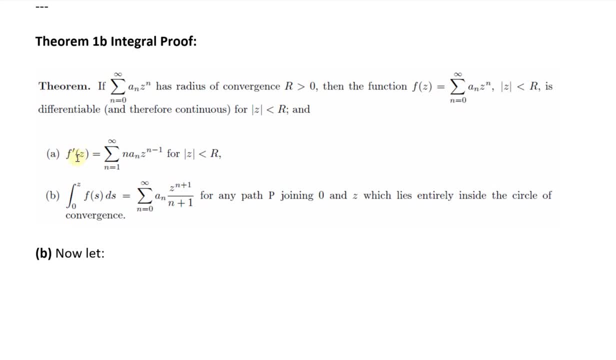 is a, the derivative of this function. So f prime of Zed is equal to the, the series now from the n times a sub n times Zed, power of n minus one for the same radius of convergence. And now we're at this inside term. 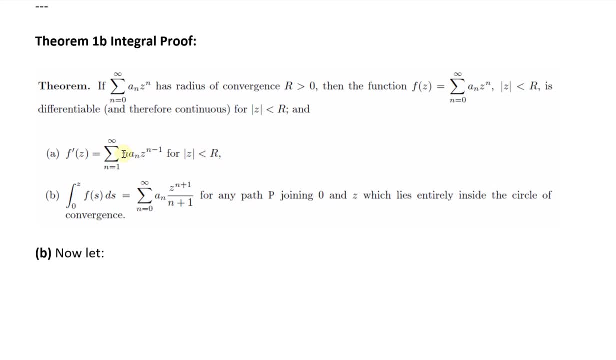 So this is what we're going to have as the derivative of each term. So this is pretty much summing up the derivative of each term And it's a saying that the derivative of the entire series, entire function, is, can be the derivative of the sum of each terms is the. 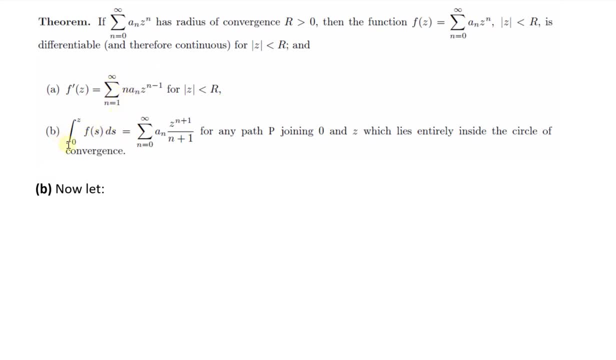 sum of the derivative of each terms. And likewise now part B, which we'll look at. they have the definite integral from zero to Zed And again number of the calculus. my calculus book use the indefinite one size constant of integration. But when you deal with definite, 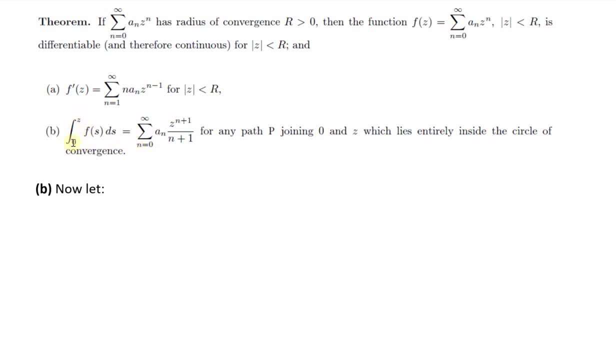 ones. what happens is the constant of integration. And again that's the same thing. the integral integration cancels. and here this proof looks at from 0 to z, but nonetheless illustrates the principle. So integral from 0 to z, of f, of s, ds, equals to the summation, from n equals 0 to infinity. 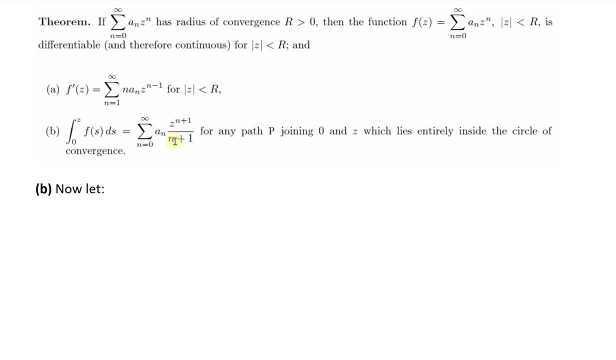 of a n times z to the power of n plus 1, divided by all, divided by n plus 1.. In other words, this is pretty much the integral. This is the integral of each term. So basically it's saying that the integral of the entire function, which is the series. 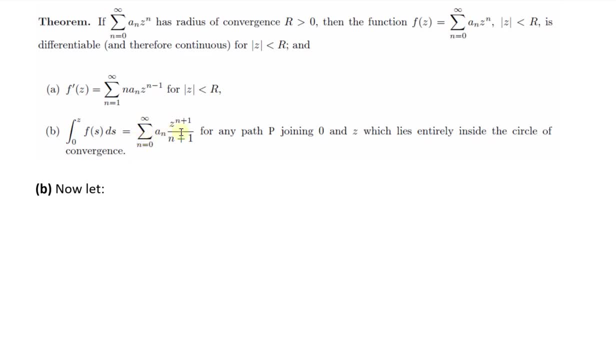 is equal to the summation of the integral of each term. So term by term, hence the term by term: differentiation and integration. So this is the theorem for it. So now part b states: this is for any path, p joining 0 and z, which lies entirely inside. 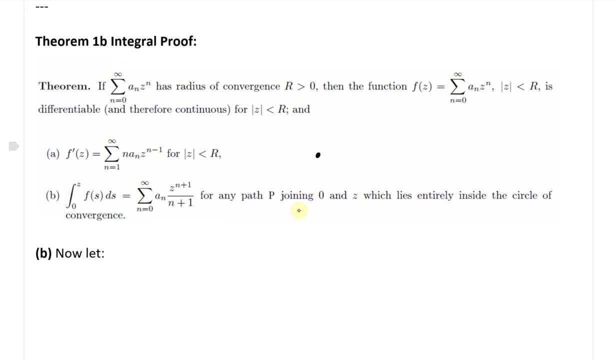 the circle of convergence. This basically means if you have the point z right here and the point 0 is point z, this is any path connecting it, So long as the entire path's within radius of convergence, So within the capital R there. 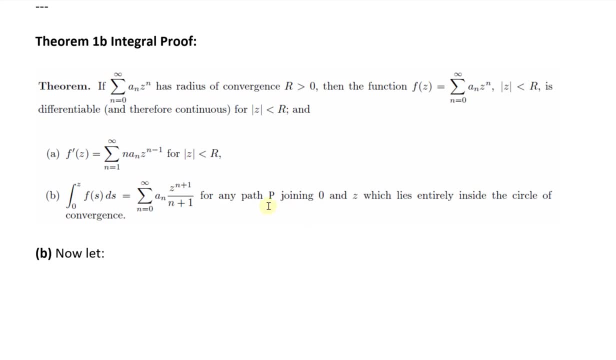 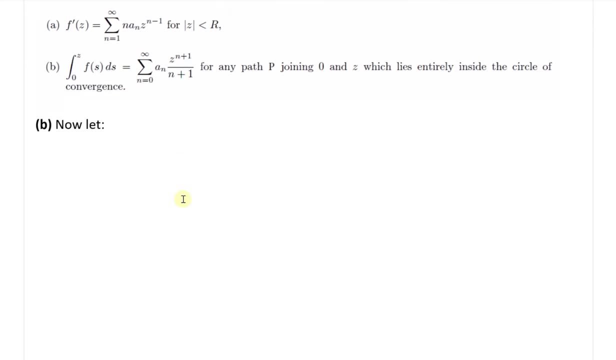 So as long as it's within, then you could take the definite integral of it And then this will equal this series right here. So let's take a look at this proof right here. So now let, yeah, let- lowercase f, so f of z equals 2, and we'll write this as the 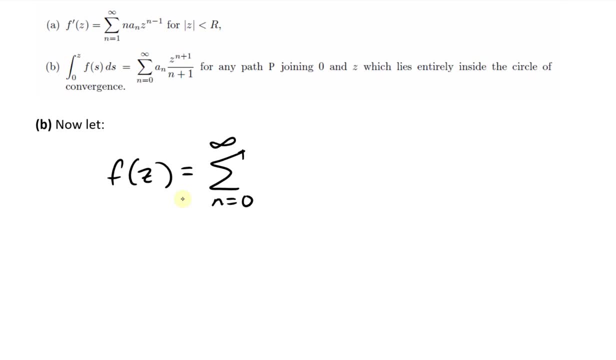 summation up to infinity of n equals to 0 of a, n, z, n. And then we'll write this: And this is for the radius of convergence. so absolute value of z is less than radius of convergence capital R. All right, so now we let this one here. this is from the same one as the theorem right. 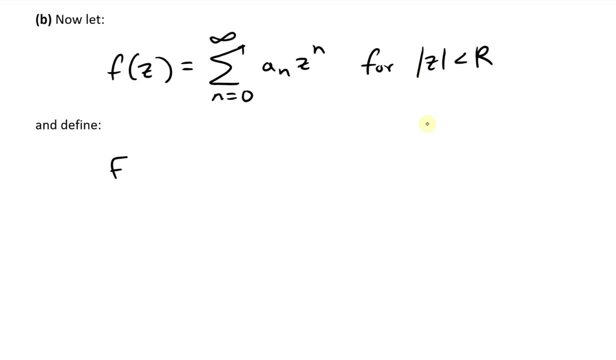 there. So now what we'll do is we're going to define capital F, and which I'll show later. this is just the anti-derivative of that function. So capital F, right here, equals to the summation from n. equals to 0 up to infinity. 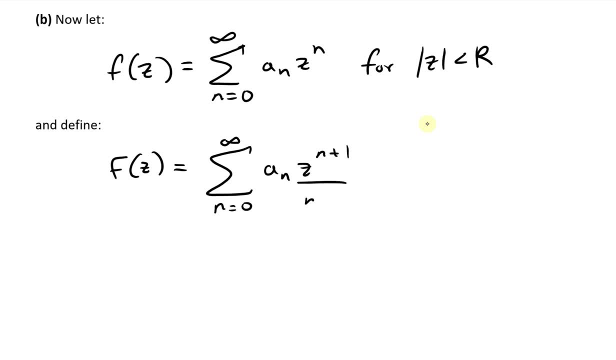 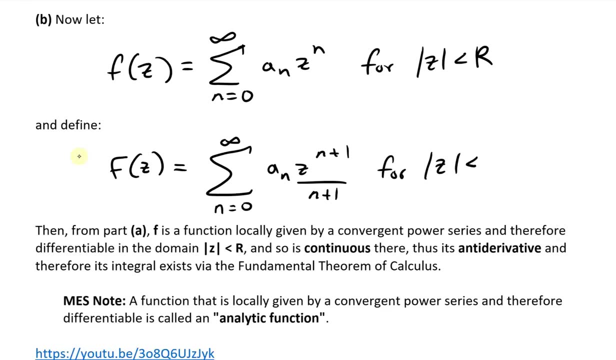 And we're going to call this a n, z, n plus 1.. I'll divide this by n plus 1.. And this one, here you're defining it for all. yeah and again, this is for absolute value of z is less than radius of convergence R, like that. 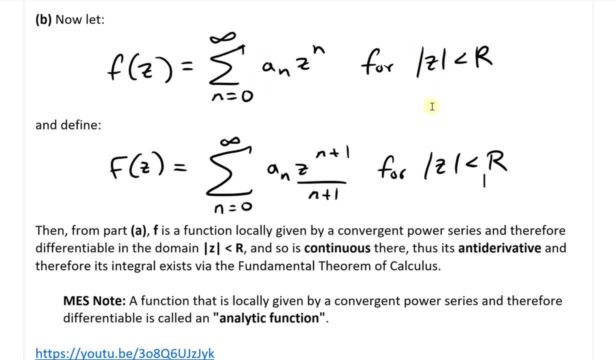 And the lemma shows that these two R have the exact same radius of convergence. So then now from part A, F is a function locally given by convergent power series. So, yes, we're given that it's radius of convergence. right here where absolute is. 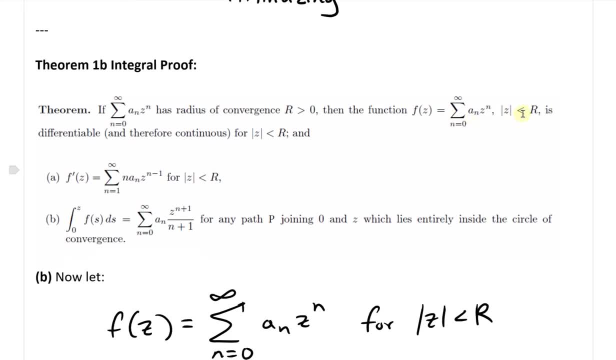 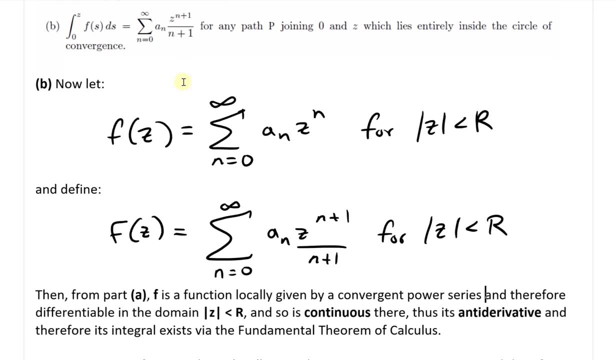 R gradient 0, where absolute value of z is less than R. So it's locally convergent within this radius of convergence. So therefore it's differentiable, or it is differentiable and therefore continuous. And yeah, just read it here. 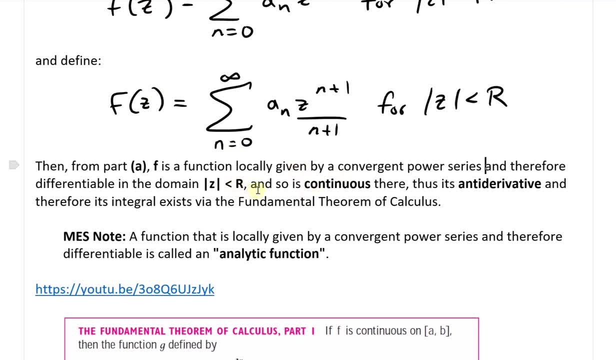 So and therefore differentiable in the domain absolute value of z less than R, and so it's continuous there. thus it's anti-derivative. So again a reference from my earlier video that if it's differentiable then it's continuous. 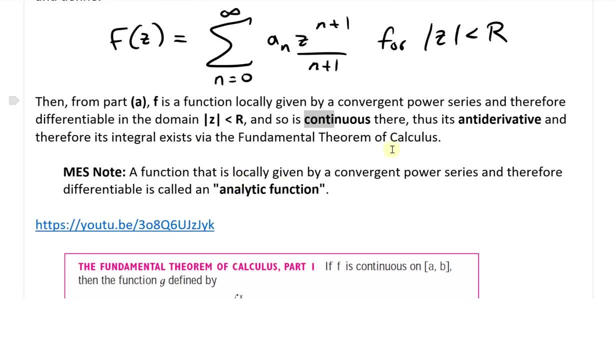 So thus it's anti-derivative And therefore it's integral, exists via the fundamental theorem of calculus and put our reference below And also MES. note: a function that is locally given by convergent power series and therefore differentiable, is called an quote analytic function. 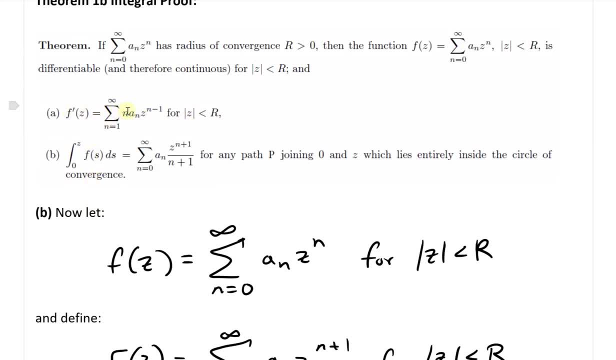 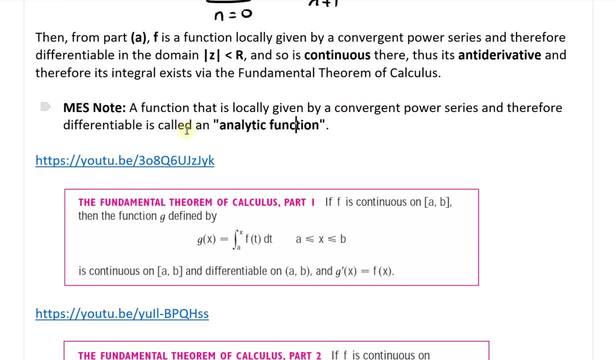 And this differentiable one- we just proved that it's a derivative- is equal to that right there. So we could take a derivative within the radius of convergence And if it's- yeah, so if you have a convergent power series, then therefore it's differentiable. 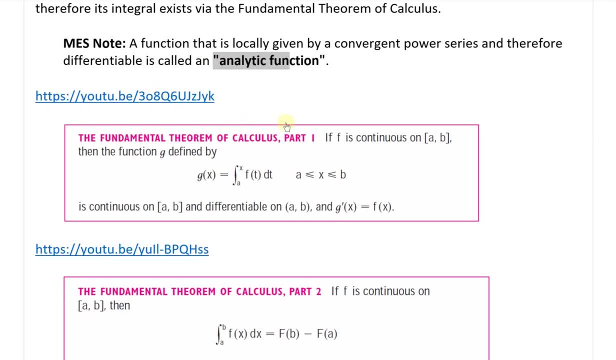 and it's called an analytic function. So in any way. So the fundamental theorem of calculus. recall part one: if F is continuous on a closed interval, A to B, then the function G, defined by G of X, equals to the integral from A to X of F. 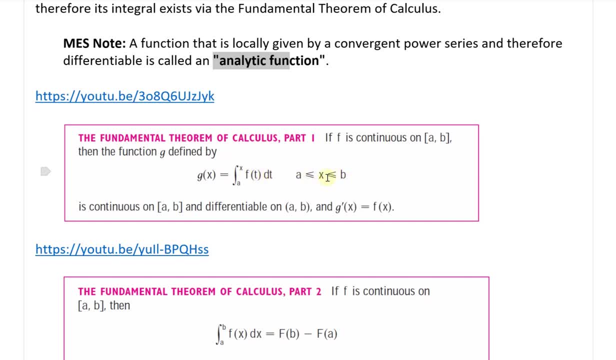 of T, DT between X from X is between A and B, is continuous on A and B closed interval and differentiable on open interval A and B. And therefore, and also G, prime of X equals to F of X. In other words, that's the anti-derivative. 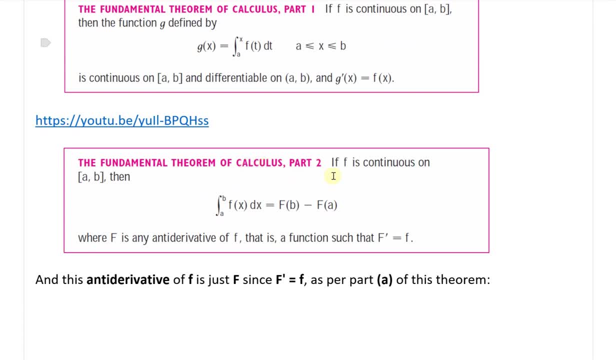 And then from part two of the fundamental theorem of calculus. Okay, So if we look at the integral of calculus, if F is continuous on a closed interval, A to B, then the integral from A to B- F of X, DX- equals to capital, F of B minus the capital. 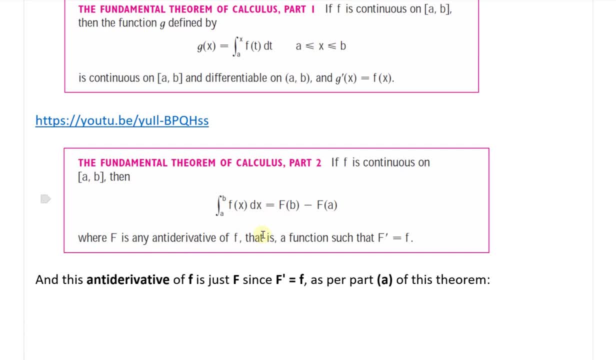 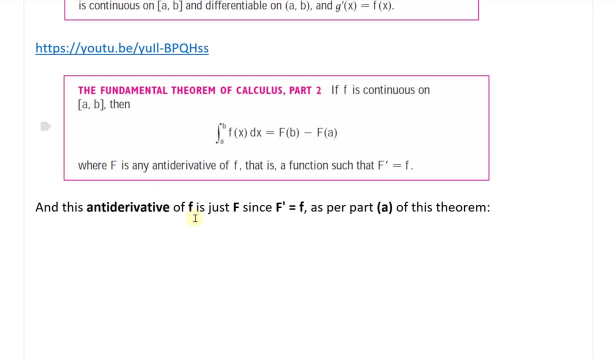 F of A, where capital F is any anti-derivative of F, that is, a function such that the derivative F prime equals to F. Yes, And this anti-derivative of F is just going to be capital F, since F prime equals to F. 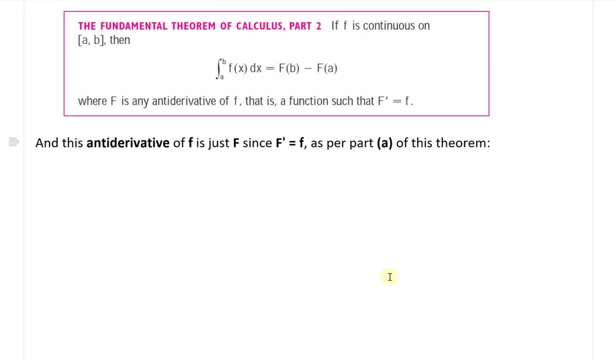 as per part A of this theorem. In other words, Uh, basically, if we have, uh, yeah, so F like that, So F prime of Z, this just equals to D over D, Z of F, where we know that uh, F of Z is. 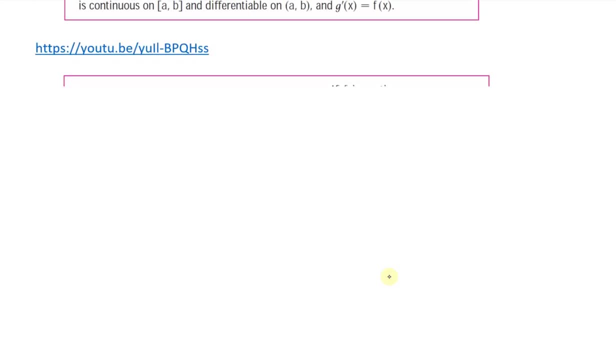 right here. So a and the summation from N equals zero to N equals zero to infinity. So I'll just write this as the same thing as writing: uh, this is N equals to zero, a and Z and plus one over N plus one. 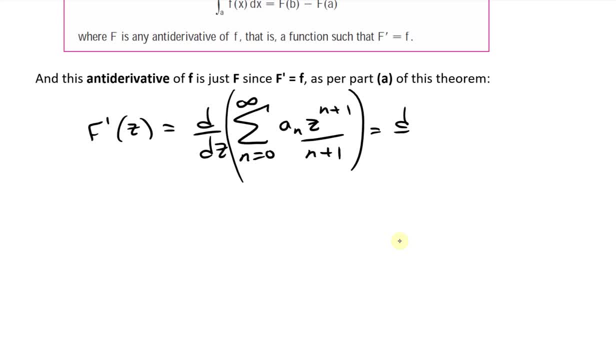 Uh. so This is the derivative of the outside. It's going to be the derivative of the inside. So this summation N equals to zero of D over D Z. This is, uh, the notation uh that I went over earlier from my calculus book. 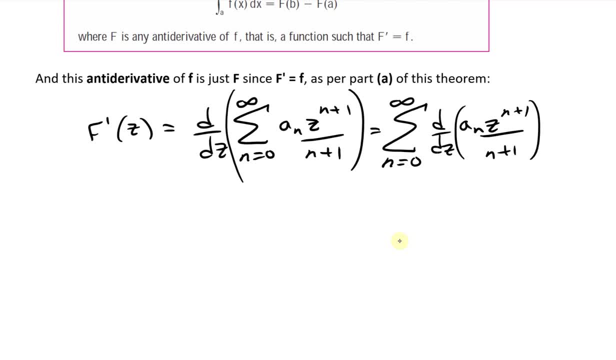 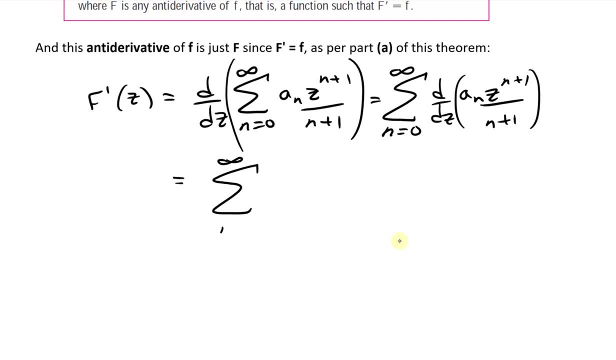 But anyways, this is going to be. you could write it as this: uh, and now this equals to uh, this is going to equal to. you could just bring that down: summation N equals zero, And then this is going to be. 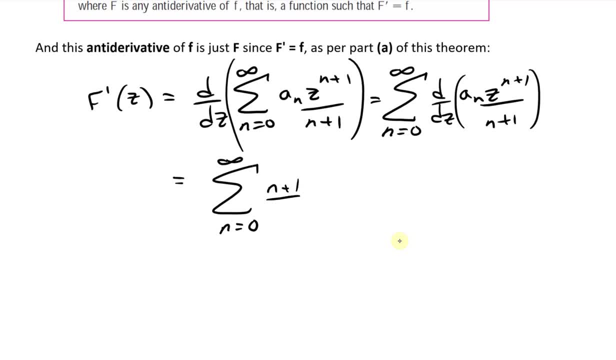 Okay, Well, uh, and plus one over- yes, bring it down. and plus one a, N, and then this is going to be subtracted by one, So Z, and so, in other words, this equals to like that and equals to zero up to yeah. 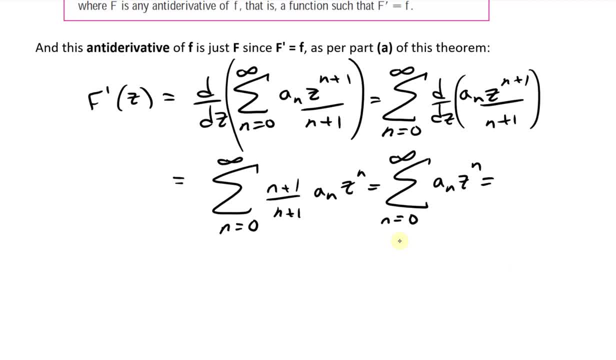 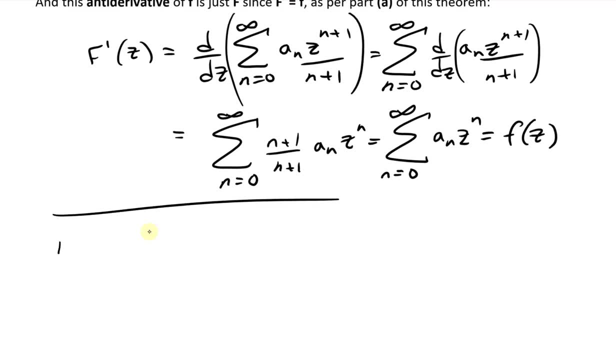 this is this: just cancels a and Z and this equals to well, F of Z I got. And also note for clarity: uh, note, we could uh do what we did earlier for the uh integral proof of the lemma. 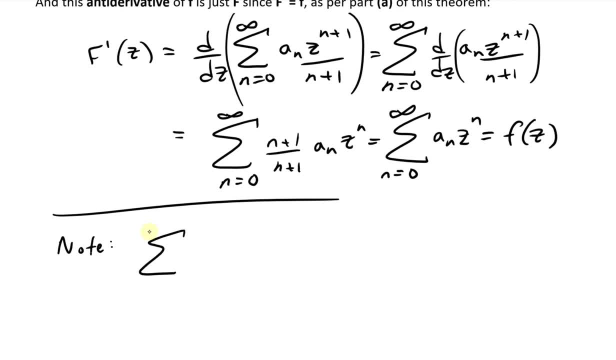 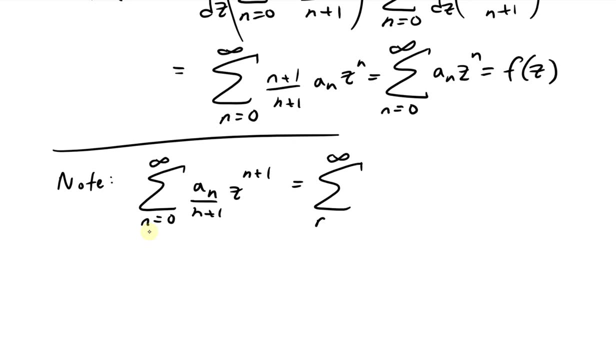 So we'd note we could view this as: let's just write this as a summation: and equals zero of a N over N plus one, And then this is going to be Z and plus one, like that, And let's just view this, uh, as equaling to. so similarly, as as before, just to show. 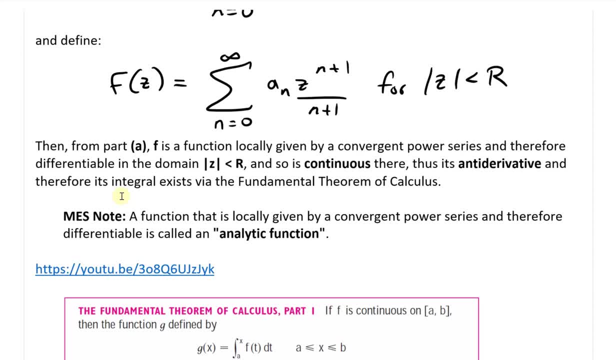 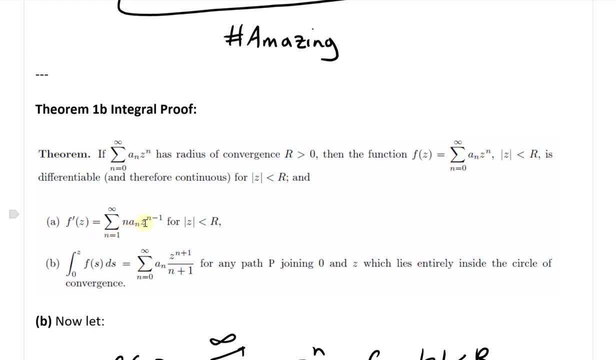 you that? it's exactly just to show that it looks in the same appearance as a this theorem right there. So we have, um, yeah, starting from a N Z, and then make it look like N a N Z. Uh, power of N minus one. 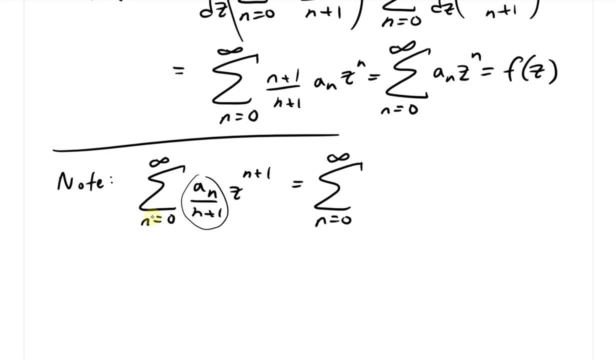 Yeah, So the same thing as writing: let's just call this right here and we'll call this a star, and and this one right here, um and star, oops and star, like that. just write this here and star. 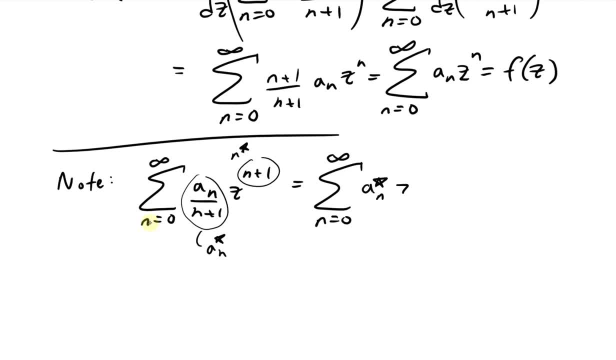 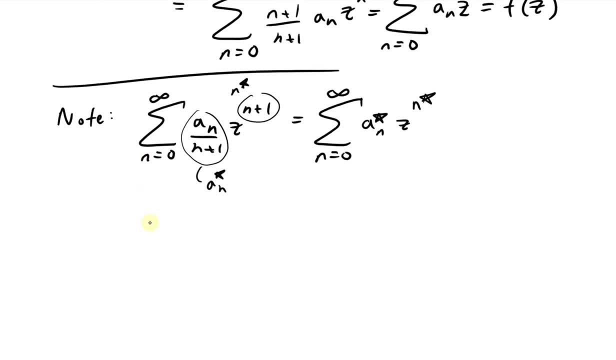 This can be sending is writing a and star, Zed and star, like that. Okay, Okay, So thus, uh, the derivative is going to be equal to. now, right here, derivative D over D Zed of this function: a and star, Zed and star. 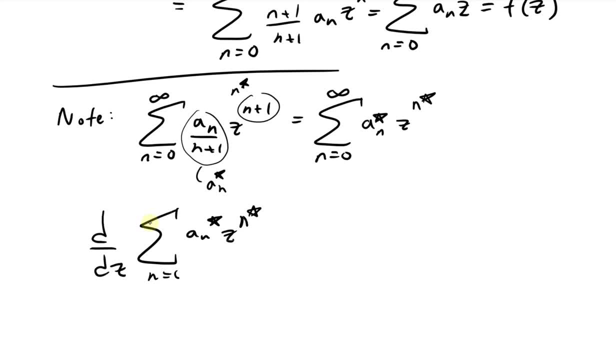 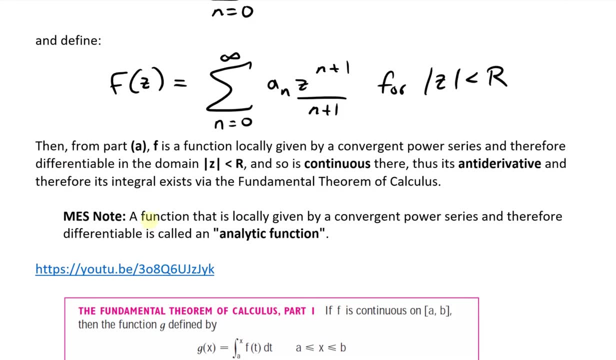 This is mainly, uh, try to make it clear in my head as well. Uh, so N equals zero to infinity of a and stars that and stars- exactly the same notation as this one above. And then we just bring down- uh, this is bring down an N. 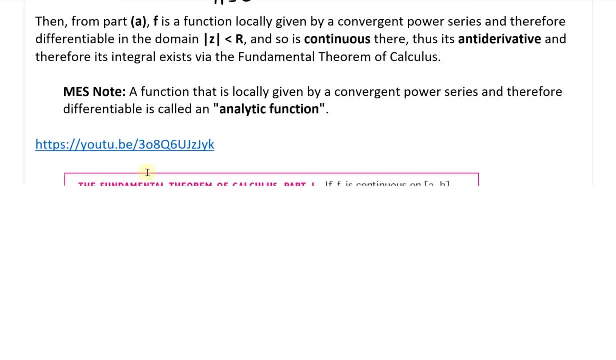 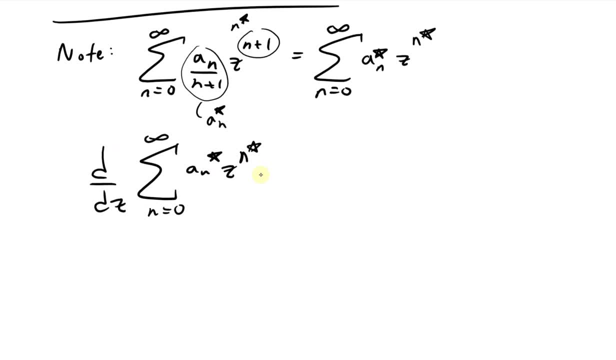 Okay, Yeah, It's the same thing as this one. Just bring down an N and we subtract by one And, interestingly, they had the derivative. even if you're taking driven to be the exact same thing as this, uh, it's, the derivative is based on the Zed. 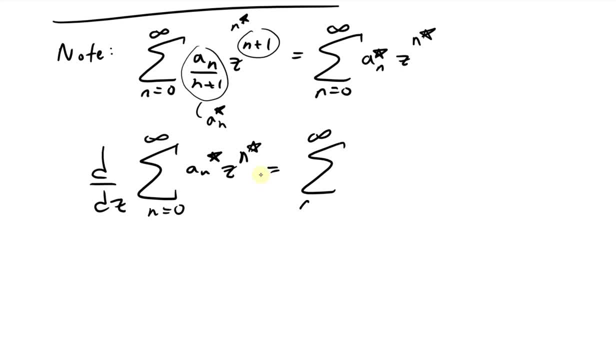 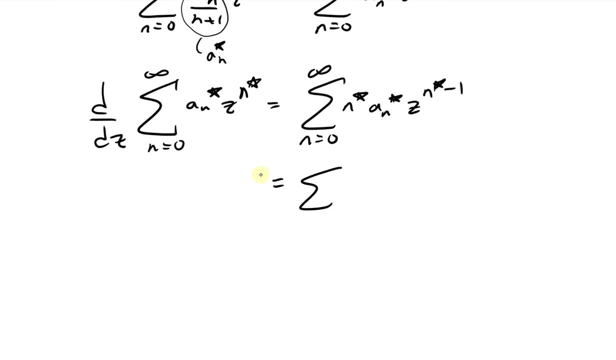 So this just equals, to just bring it down, infinity, and equals zero and star a and star Zed and star minus one, like that. And uh, then we just combine them all together. This just equals to summation, or just fill in the blanks. 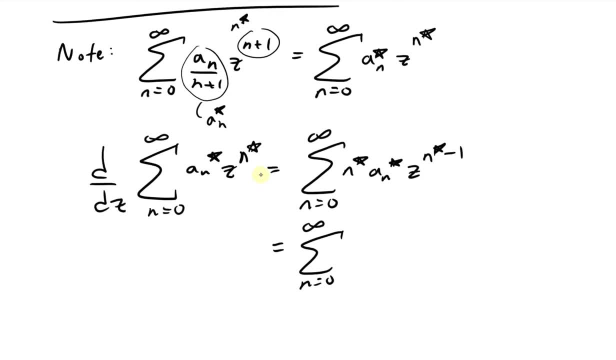 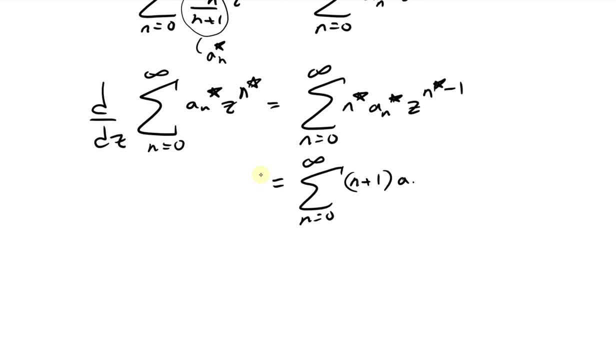 Okay, Okay, Thanks again. So N star is going to be our uh N plus one. So N plus one, and then uh times it. by now we have a N N plus one. That's just this. one times it by Zed, and plus one minus one is going to be Zed. 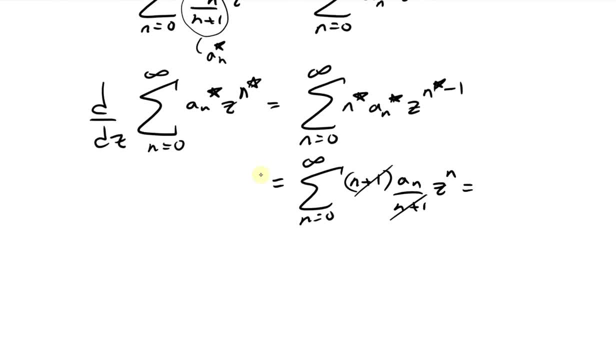 So these cancel and, uh, this just equals to our um, uh, F of Zed. So, right here, Yeah, So those cancels, just write this as F of Zed now, and then this right here is equal to F prime of Zed. 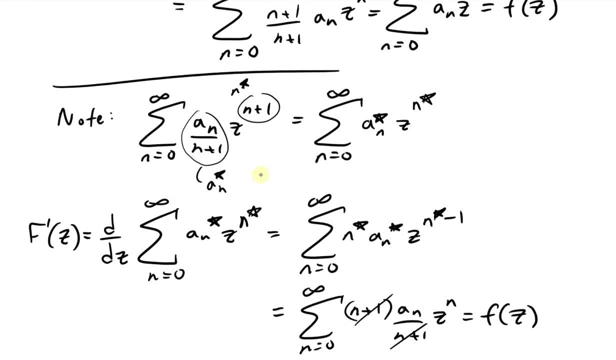 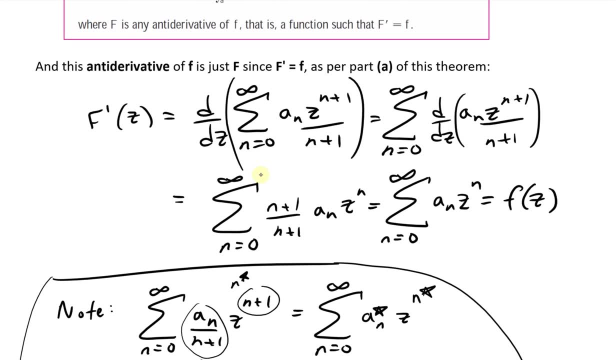 Okay, Yeah, So hence these are. these are the exact same things. I'm just going to uh circle this one here just to illustrate that. this is just to further clarify the point. All right, So, uh, that's what we have is a capital. F is an anti-derivative of lowercase F in the 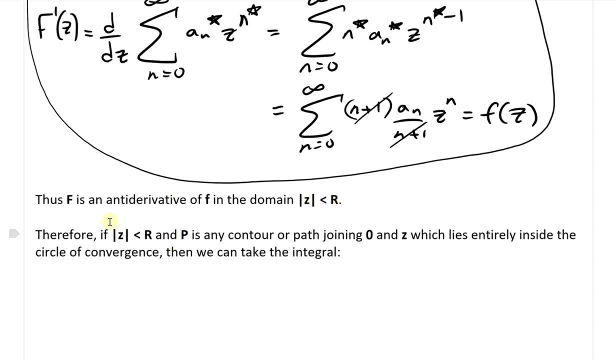 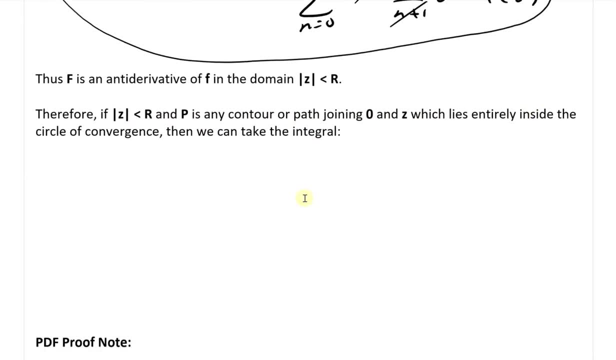 domain, absolute value of Zed is less than capital R. So therefore, if the absolute value of Zed is less than a capital R and P, is any contour or path joining zero to Zed which lies entirely inside the circle of convergence? Yeah, 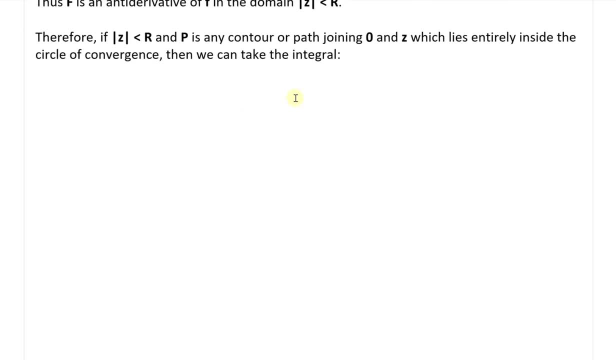 Then we can take the integral or the uh definite integral and this is uh. we'll write it like this Calculus book has it like this, or the PDF proof has it like uh. so the path P integral for the path P of F of Zed, uh, D, actually F of SDS, equals to the integral from zero. 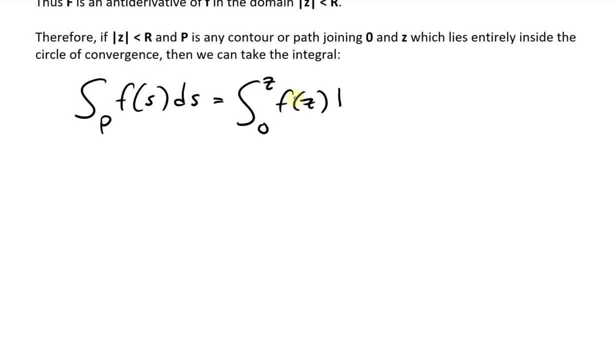 to Zed, of F of Zed, uh D Zed. This just equals to now capital F, the anti-derivative uh of Zed, any of them, minus anti-derivative any of them. They're all just separated by coefficients, uh, the, the constants of integration. 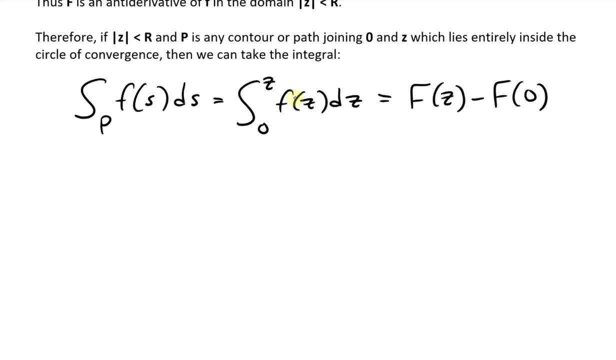 So capital F of Zed, minus F of zero, and and uh, this equals two. So this is going to be equal to, um, you know our function, capital uh F, which is just our a and Zed, the N plus one all over and plus one. 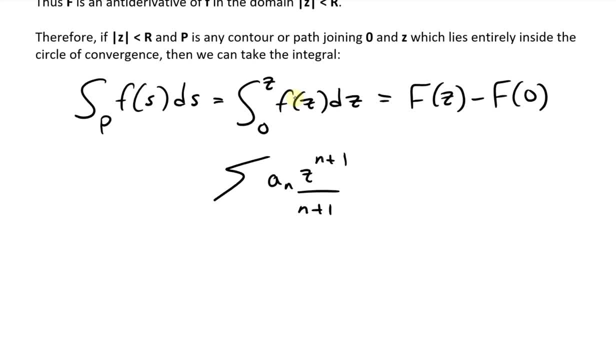 And uh, yeah, this, this the summation of it, uh, summation of a series. this will be defined it as: N equals zero up to infinity of a N Zed and plus one divided by N plus one, like that. 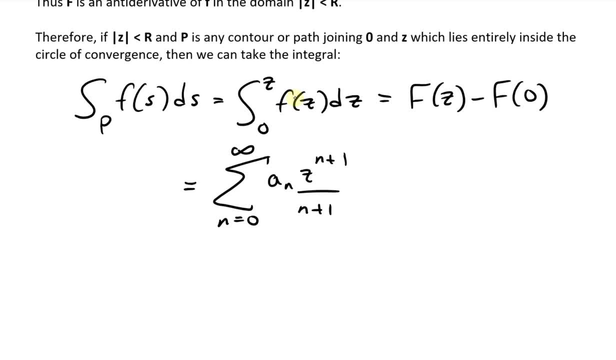 And uh, this is just an equal sign. And then we subtract when you plug in the zero one inside. So when you plug in zero, we're just going to get a well, minus a zero, So minus a, and a summation: a and zero. a N times zero, uh uh, N plus one, et cetera. 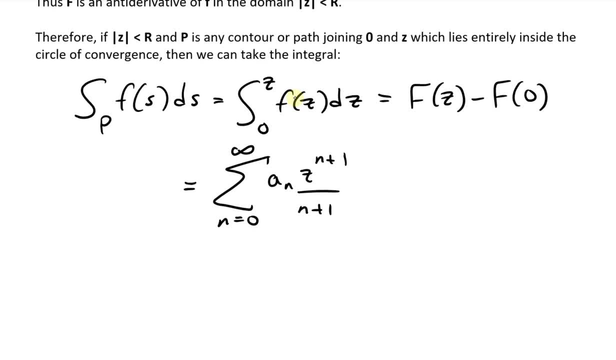 This is all. vanishes is zero. So I'll just ignore that and I'll just highlight this and I'll just put this all together. So this is going to equal two. Put an arrow, Um. so thus we have the integral from zero to Zed of F, of Zed, uh uh. F of S, yeah F. 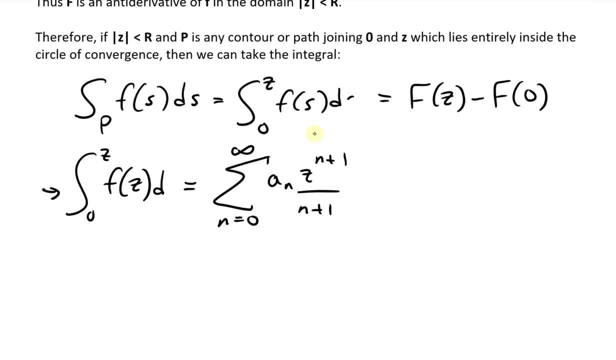 of S. yes, or remove those with F of S D S. this is going to be F of S D S, like that, And because we're going to plug in the variables that inside and this is a yeah, so this is what we have. 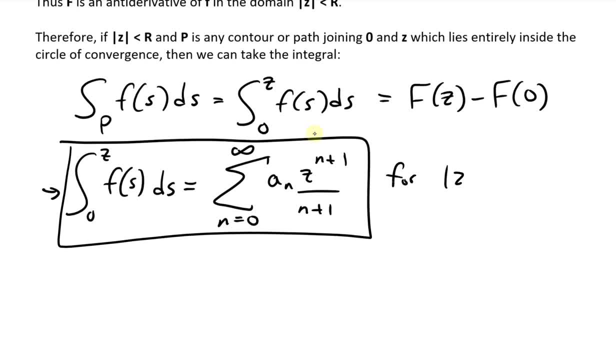 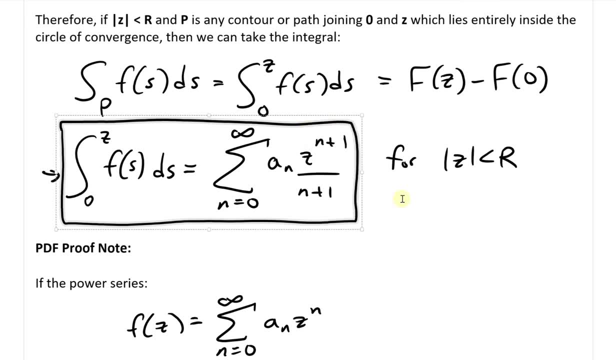 Sparks this out. This is four. Uh. opposite value of Zed is less than the radius of convergence. are So yes And uh. there completes the uh theorem. uh pretty epic, uh, epic uh derivation. 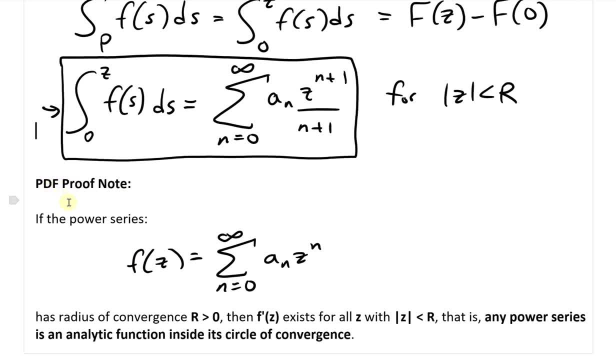 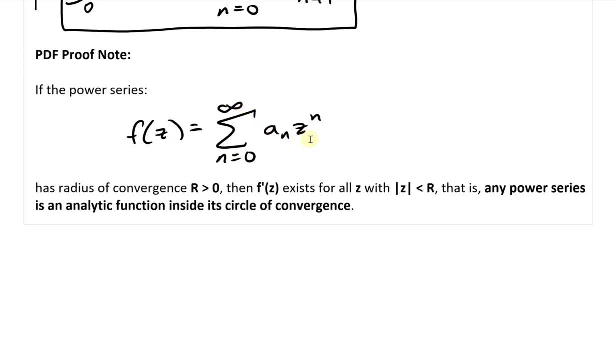 to get here And uh, also just a PDF proof. knows from the PDF proof, uh, if the power series F of Zed equals to the summation, and equals zero to infinity, of a N uh Zed and has a radius of convergence, uh, or a capital R is greater than zero, 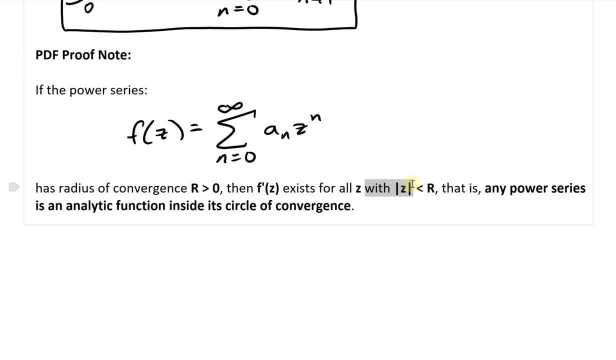 Then F prime of Zed exists for all Zed. with uh, absolute value of Zed is within the radius of convergence, That is, any power series is an, an analytic function inside its circle of convergence. In other words, any power series can be written as a convergent power series. uh, IE itself.